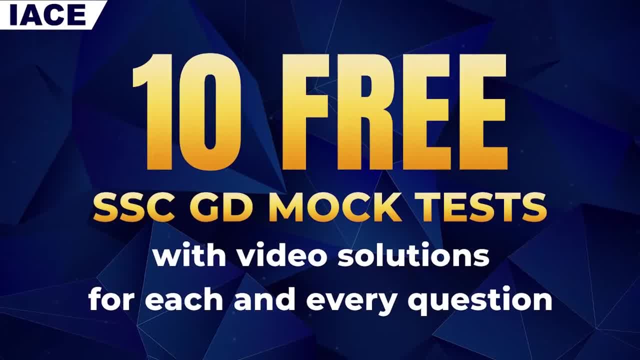 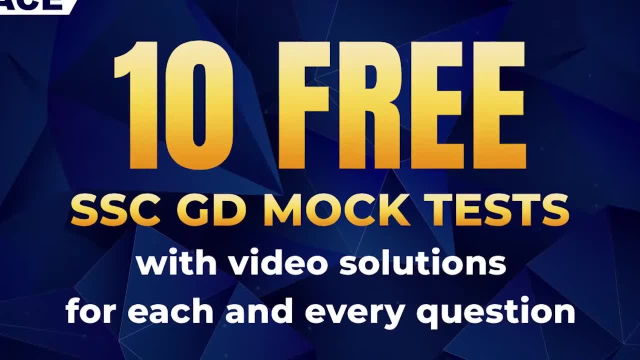 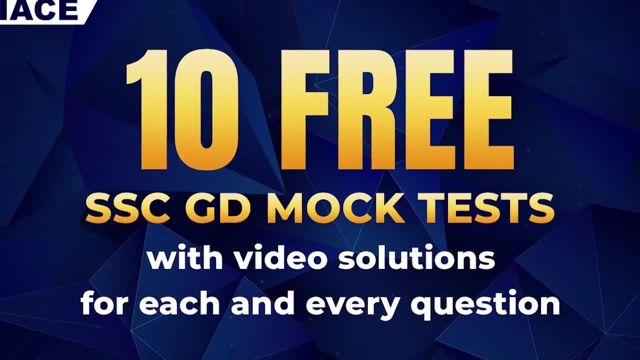 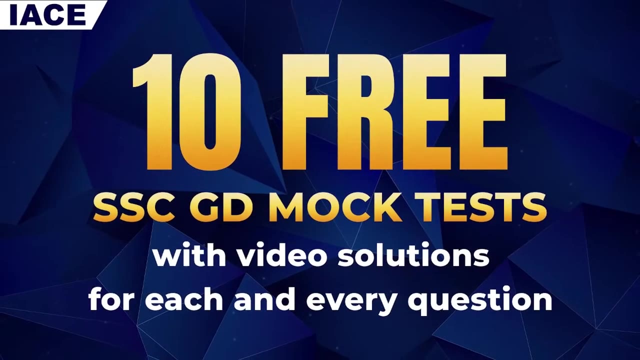 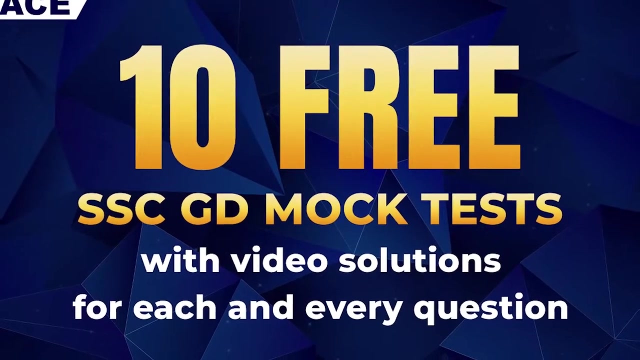 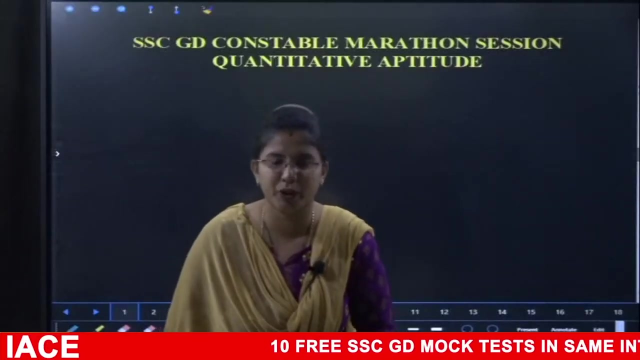 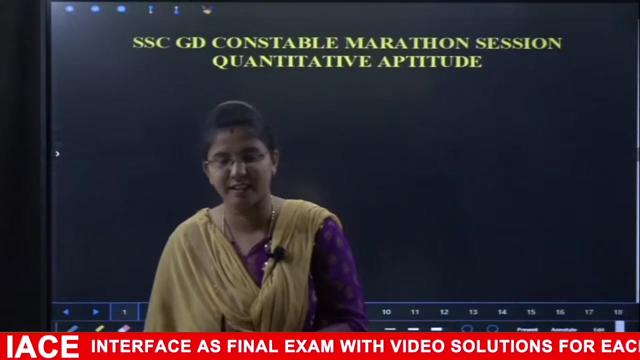 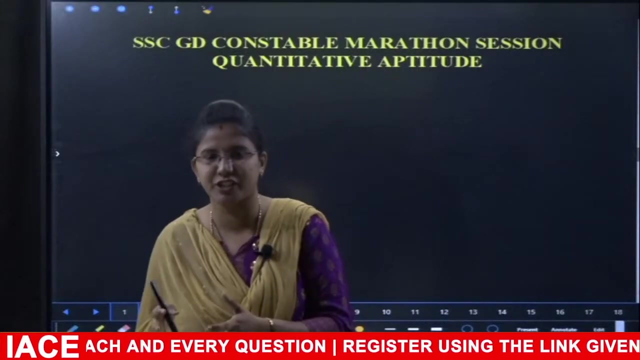 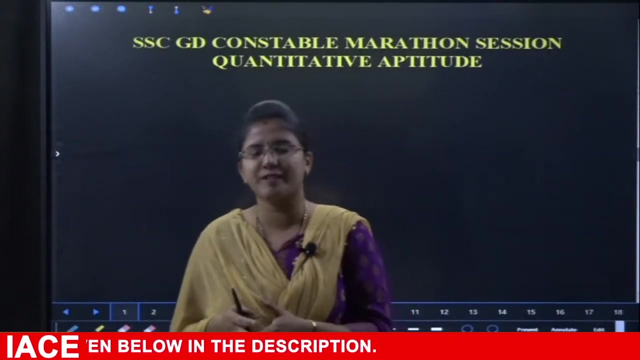 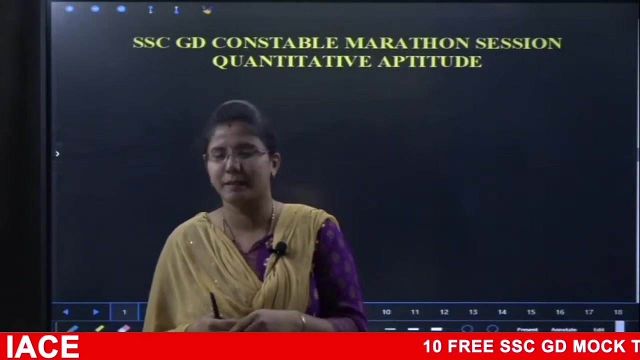 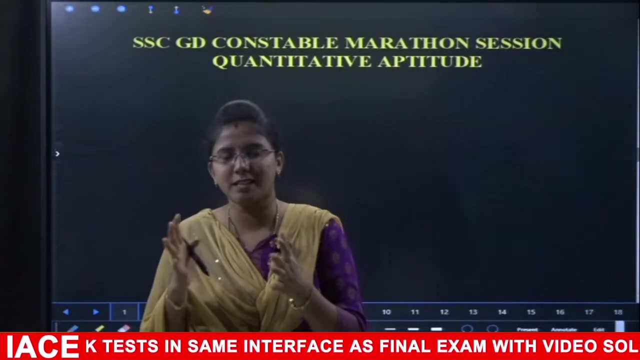 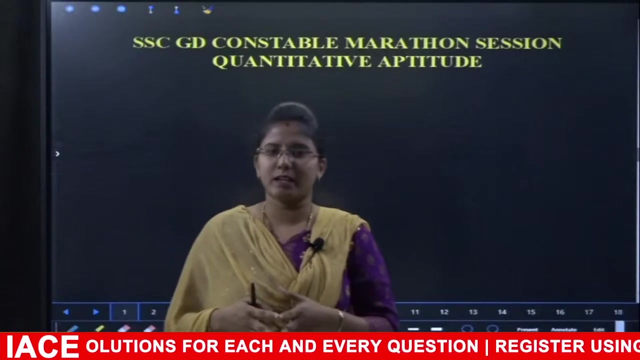 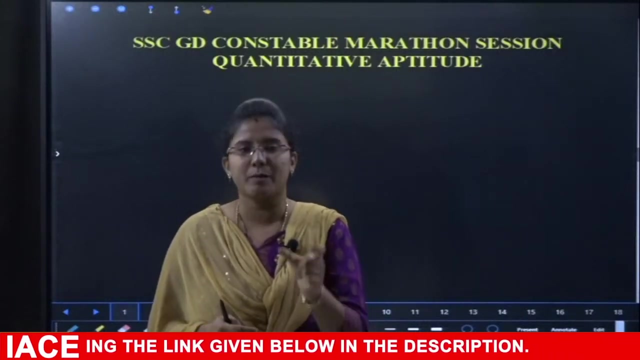 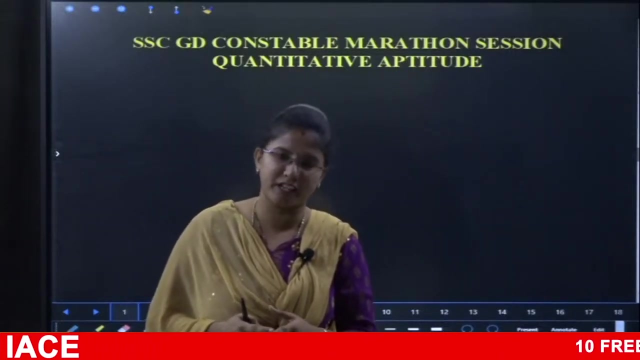 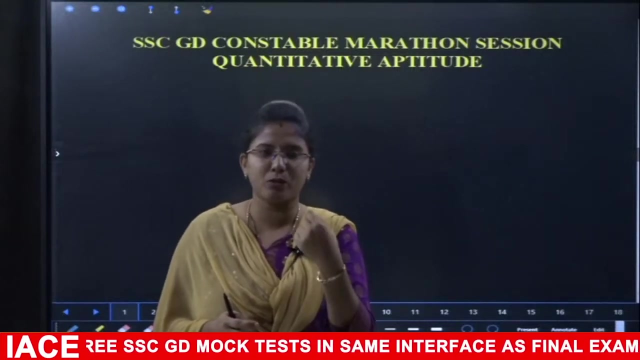 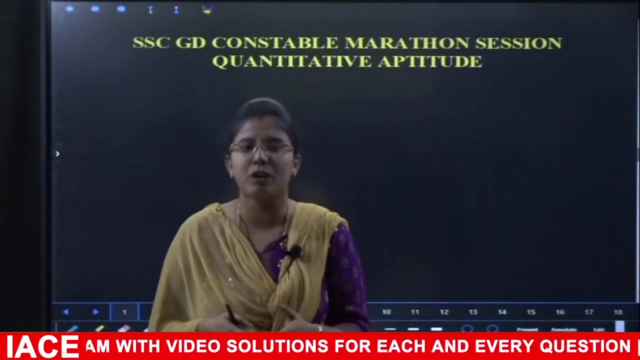 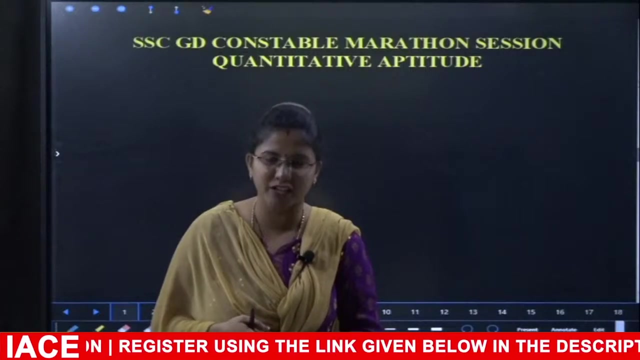 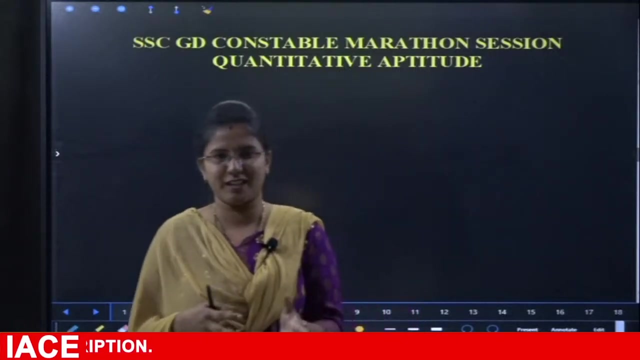 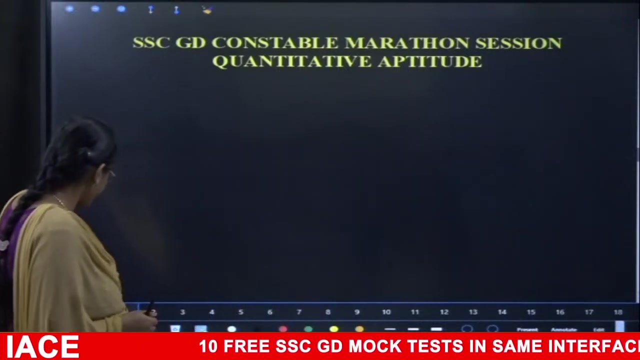 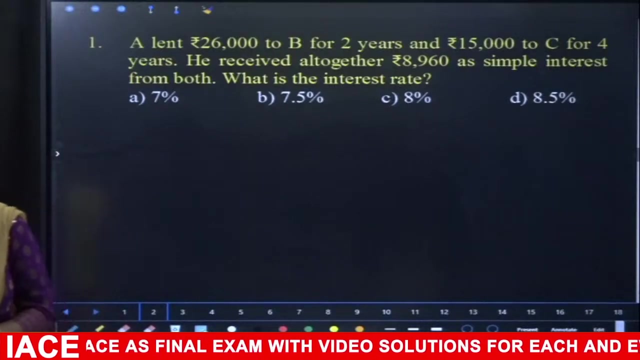 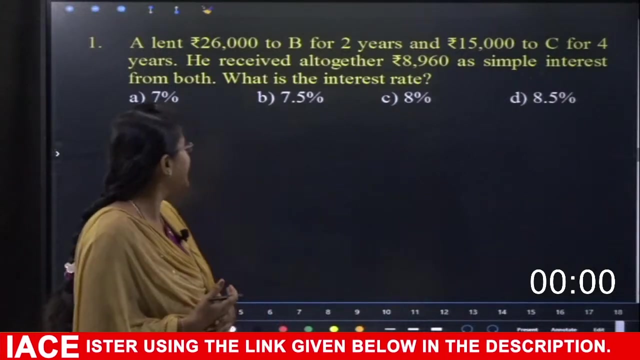 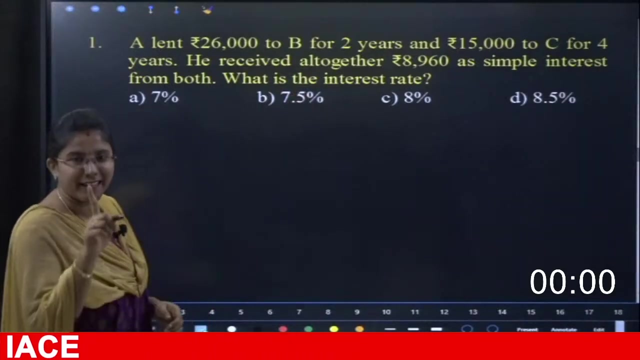 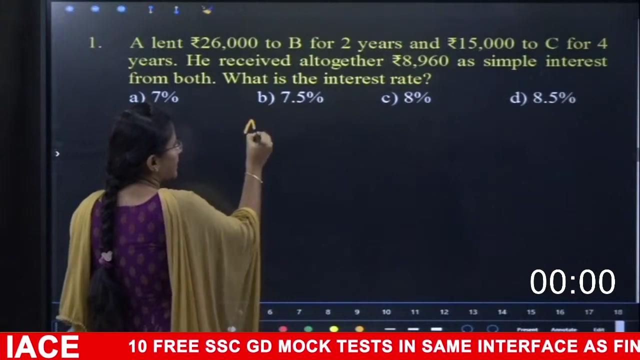 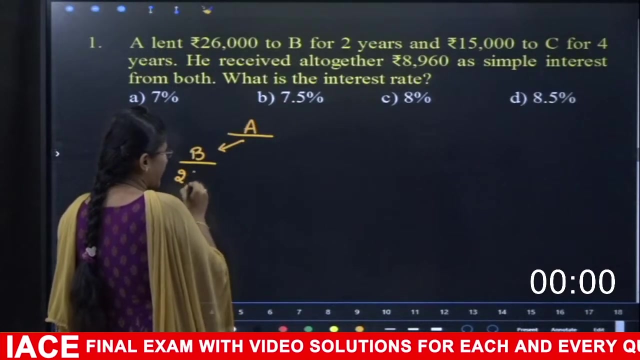 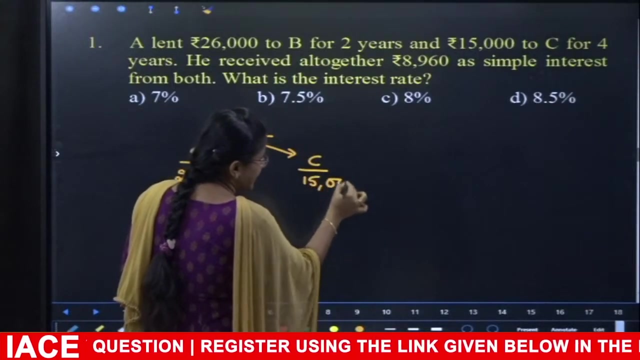 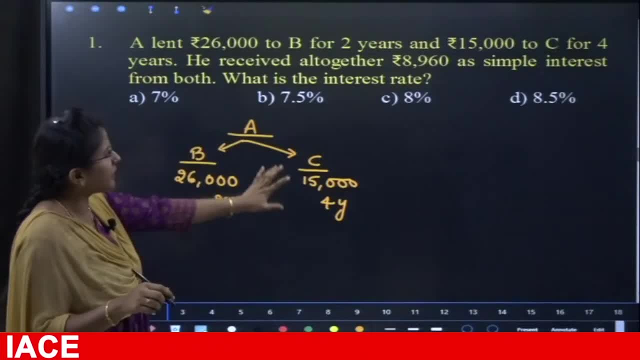 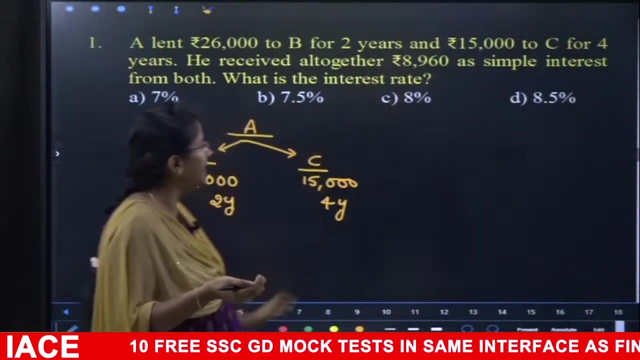 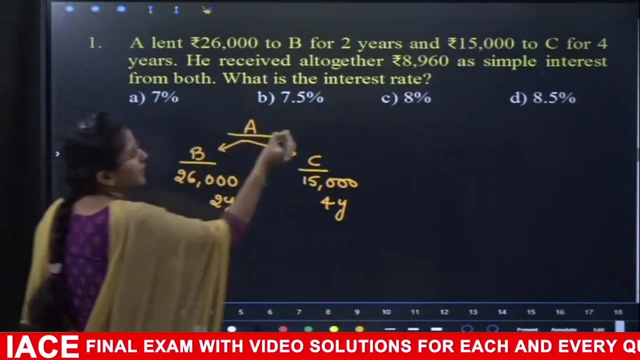 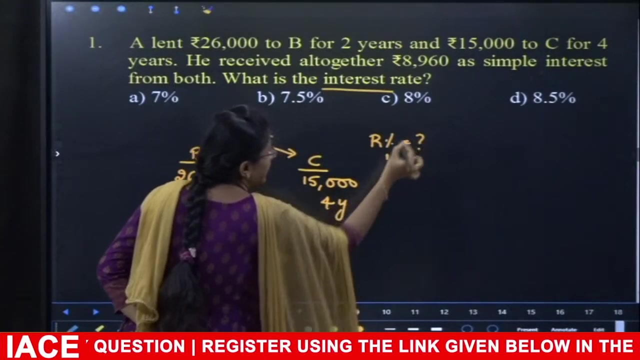 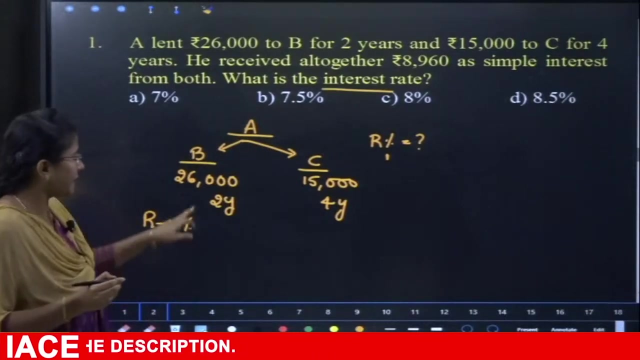 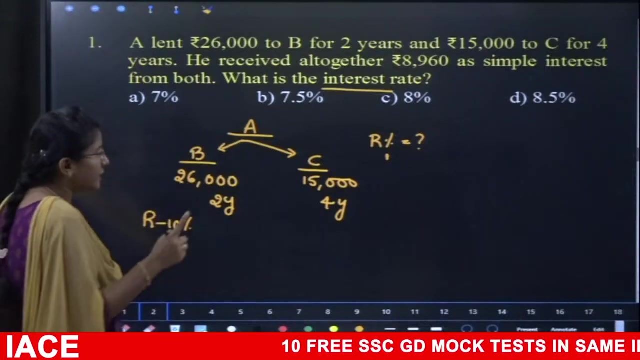 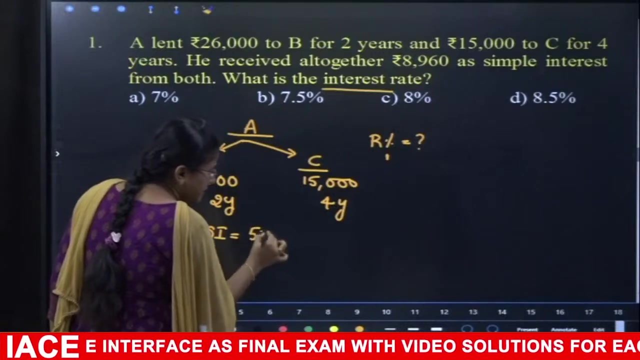 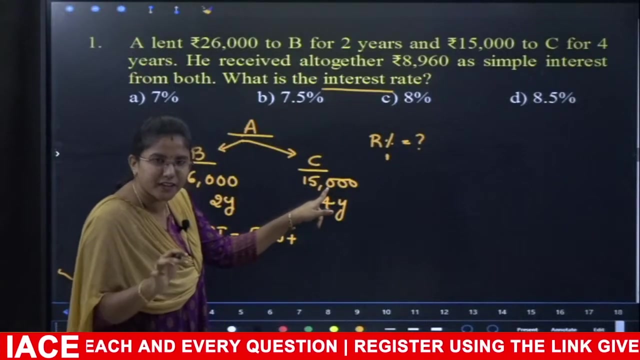 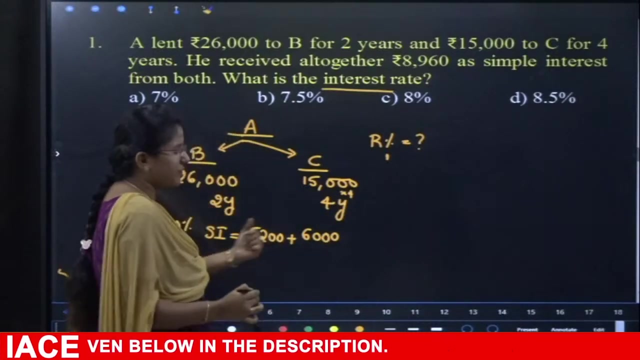 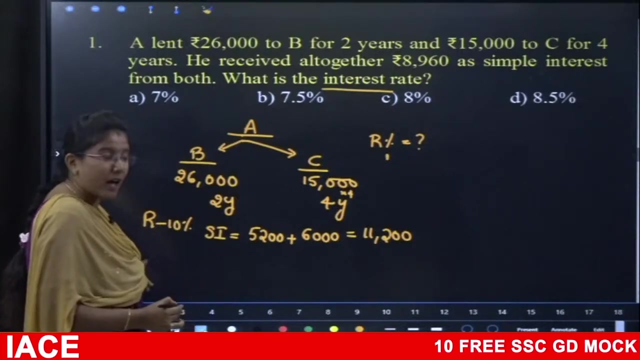 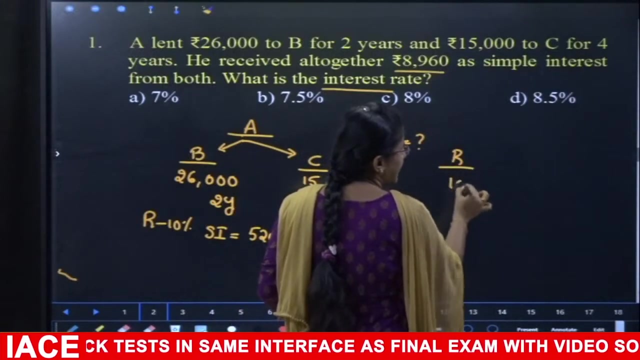 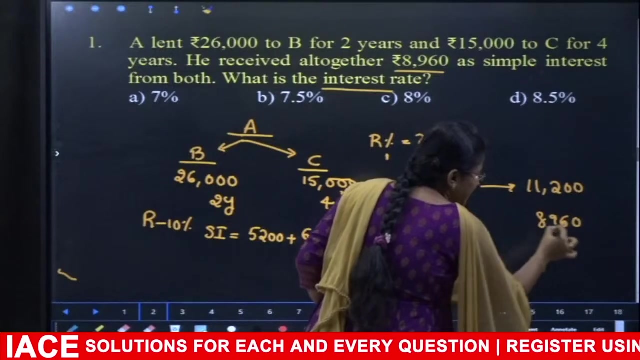 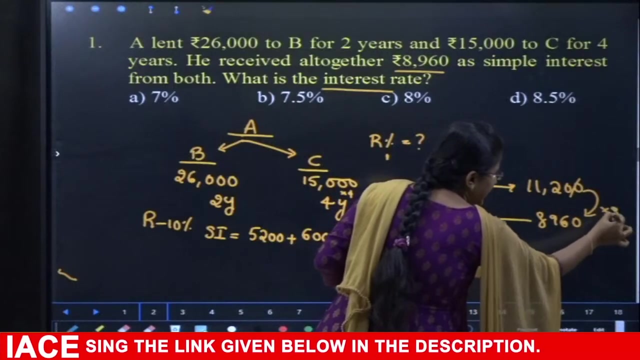 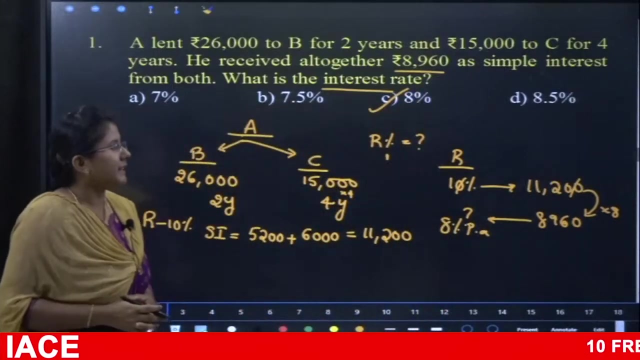 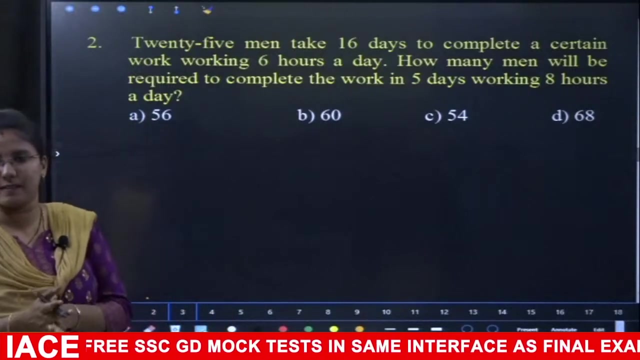 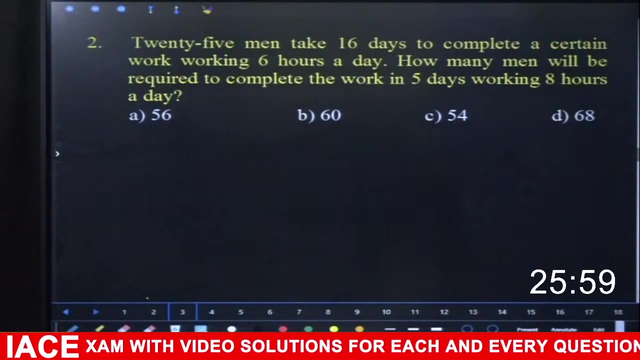 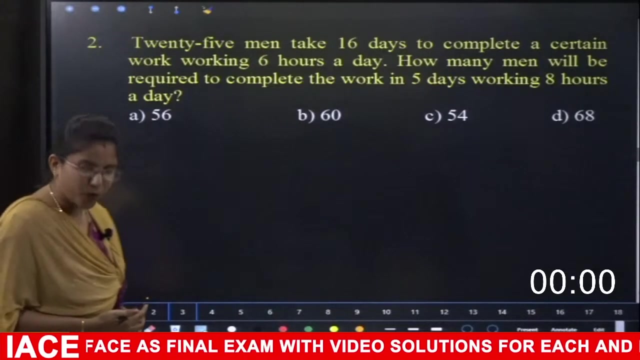 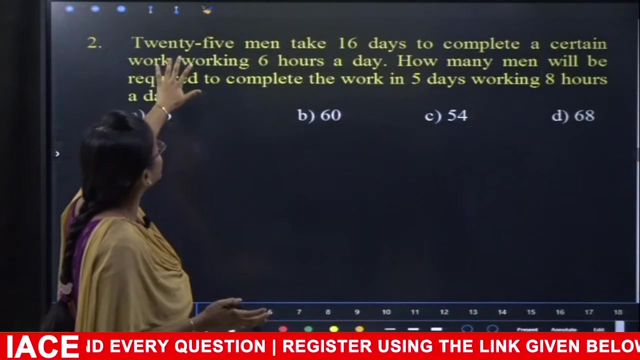 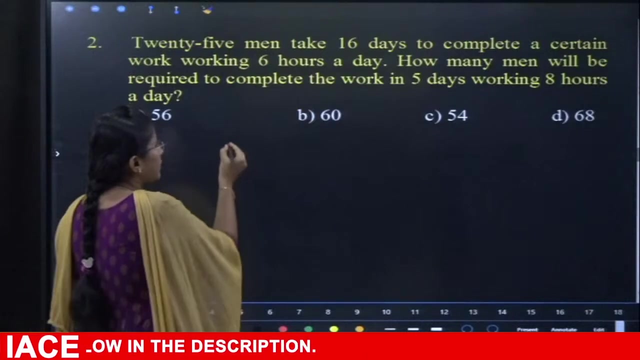 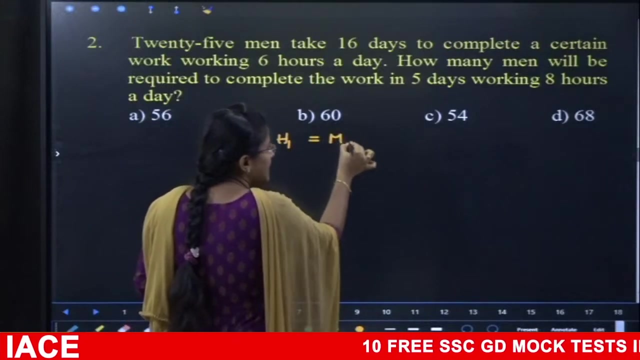 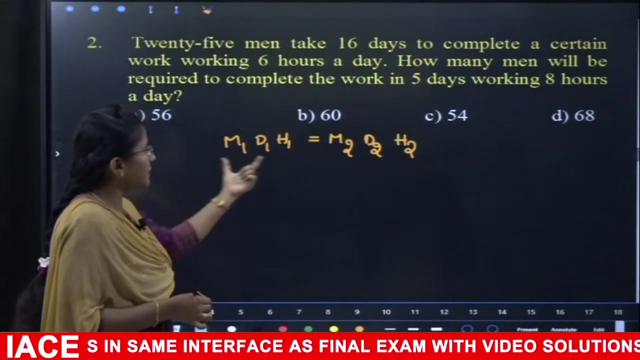 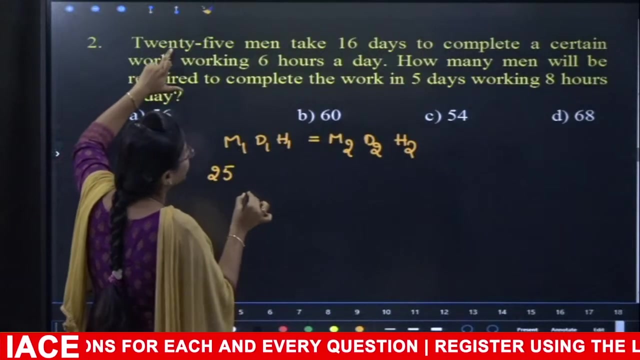 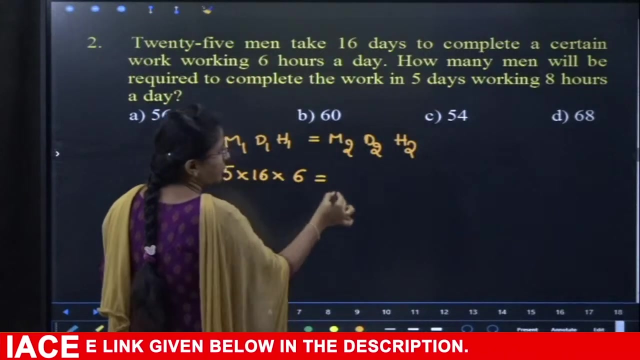 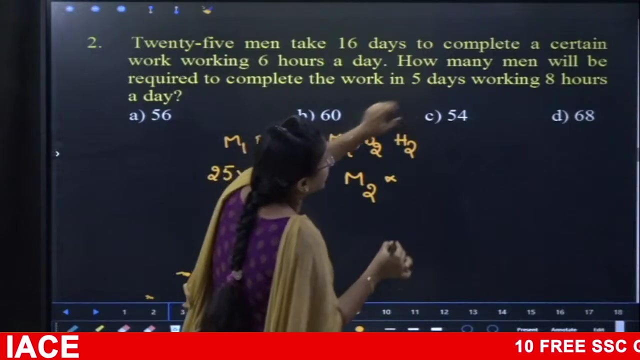 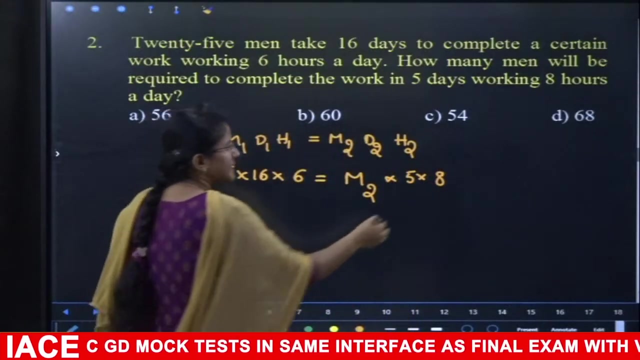 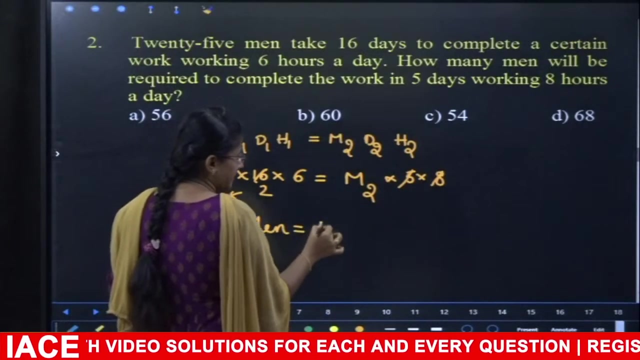 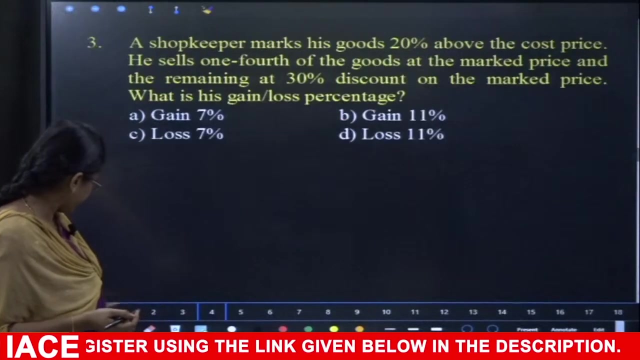 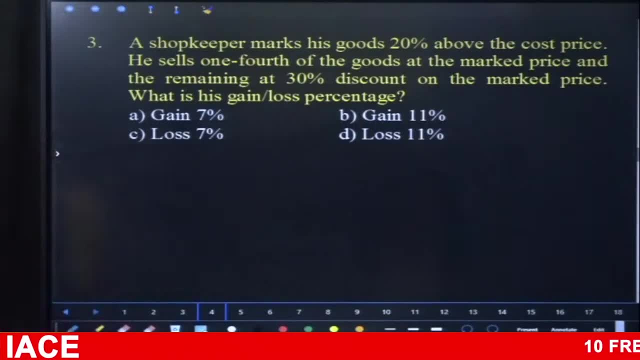 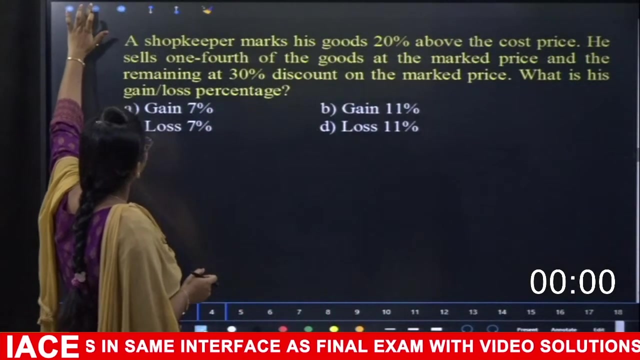 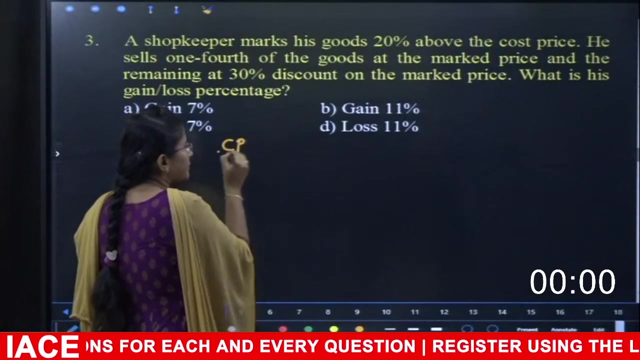 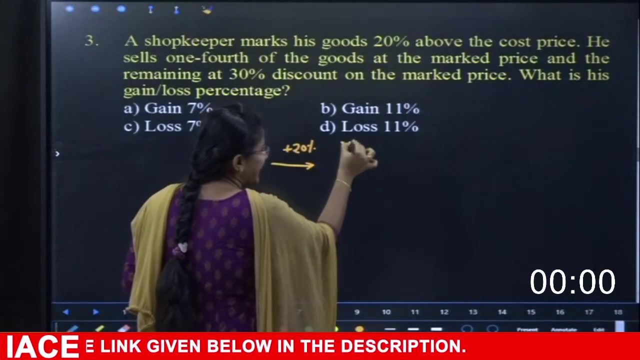 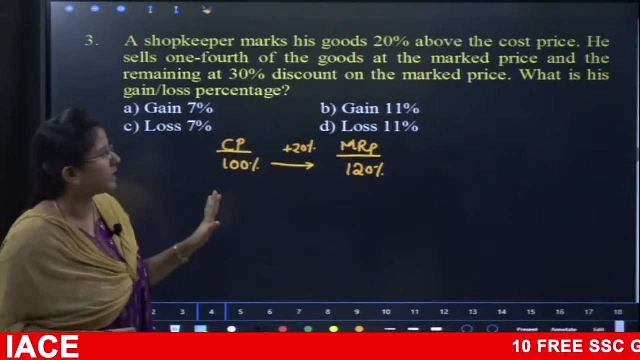 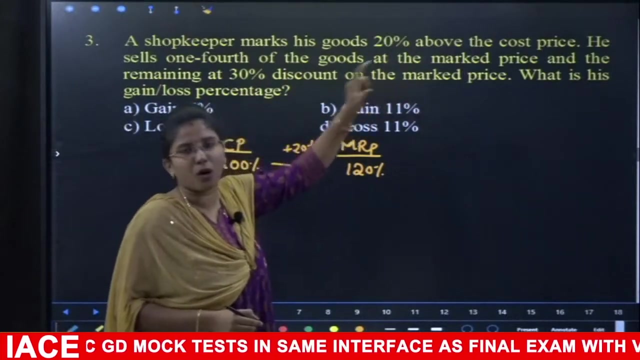 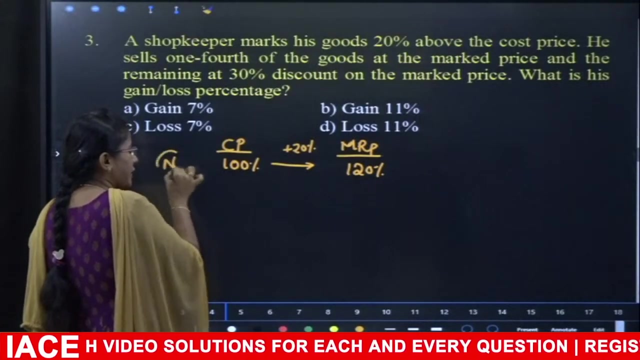 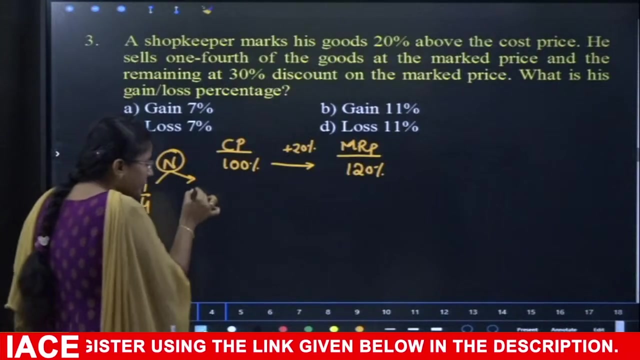 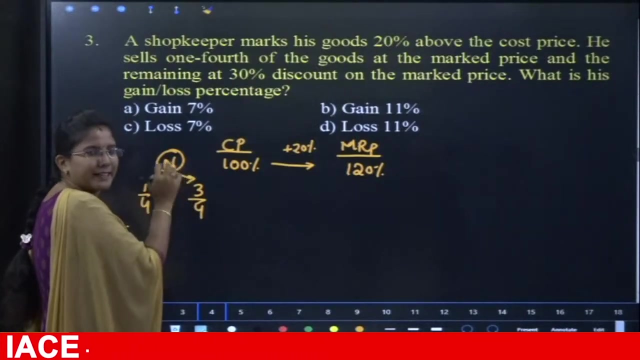 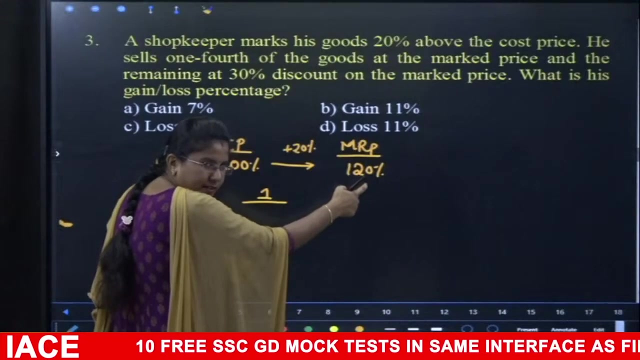 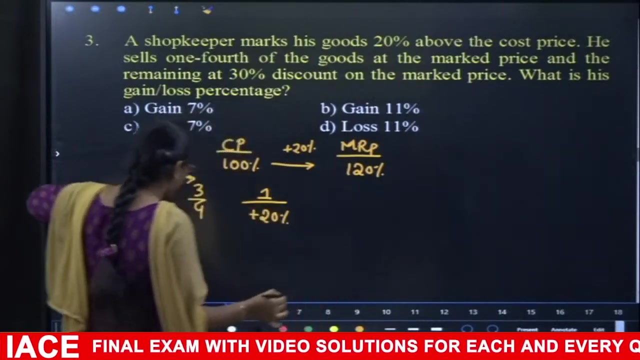 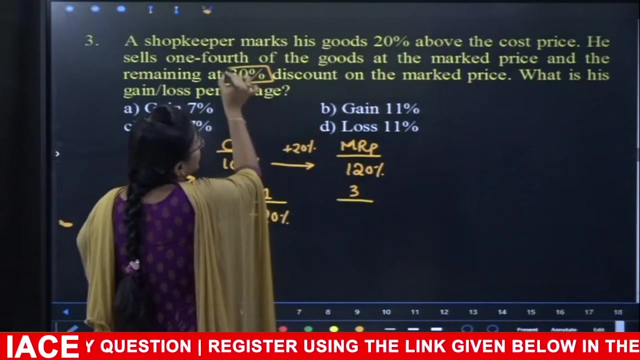 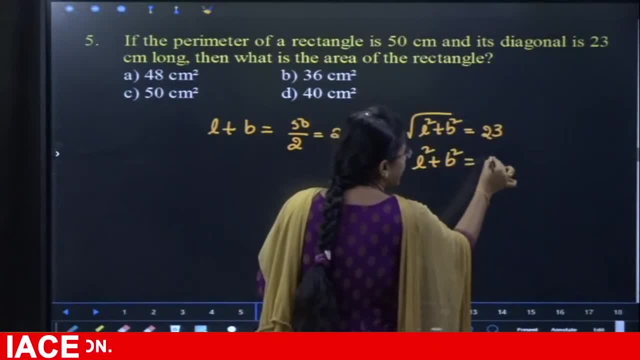 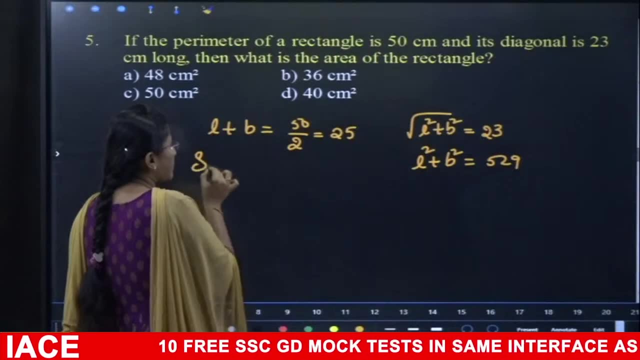 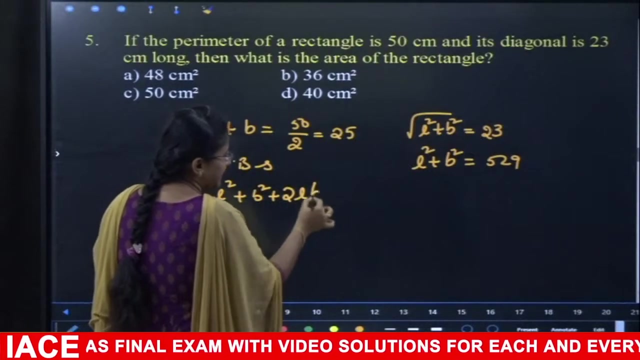 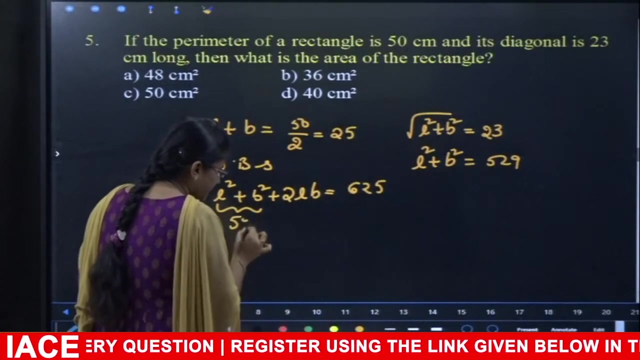 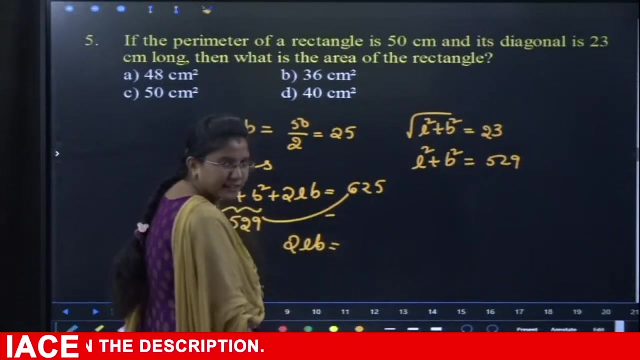 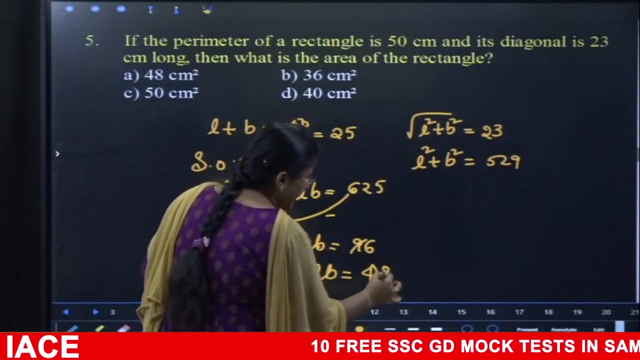 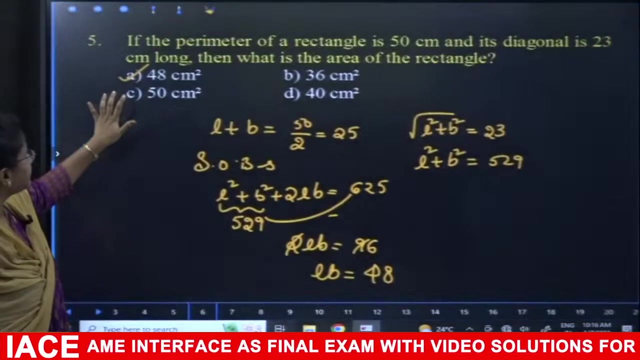 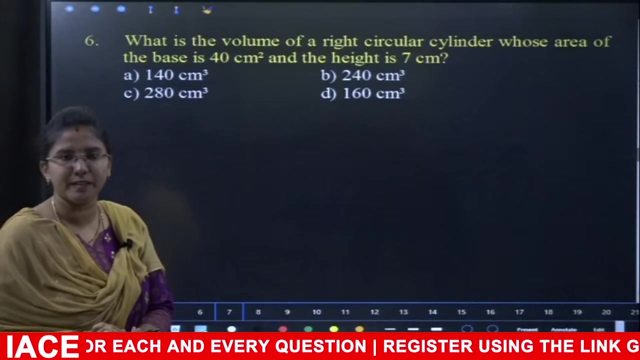 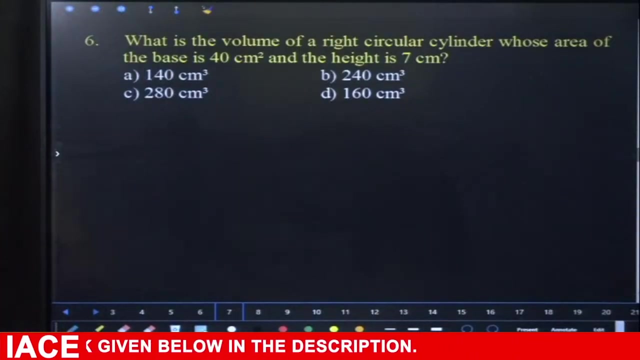 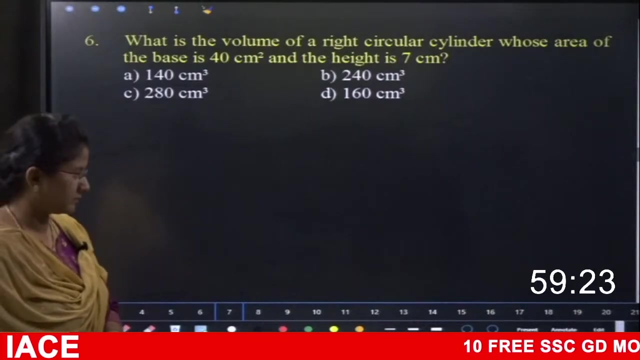 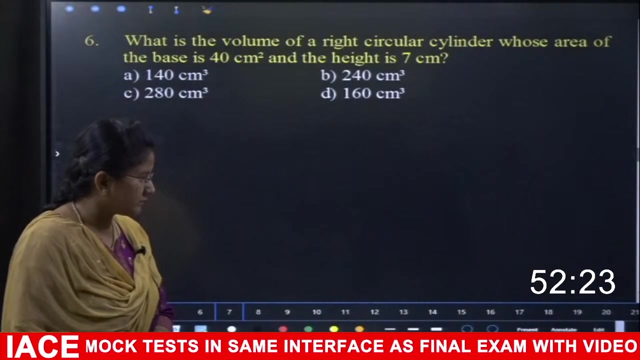 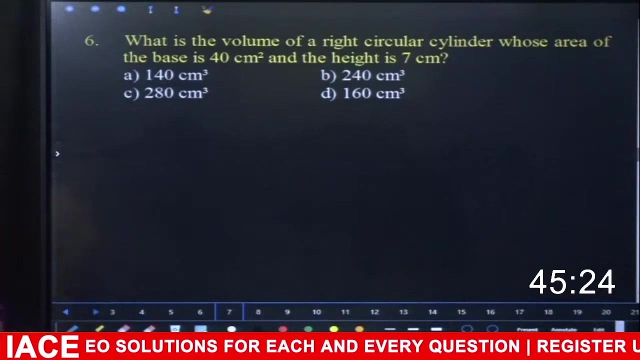 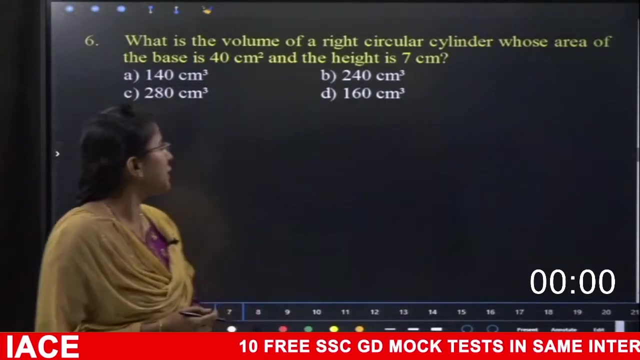 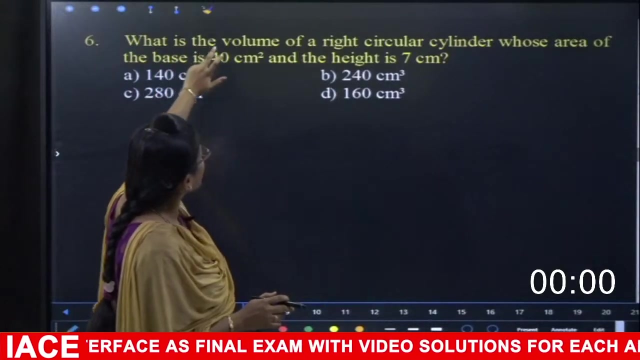 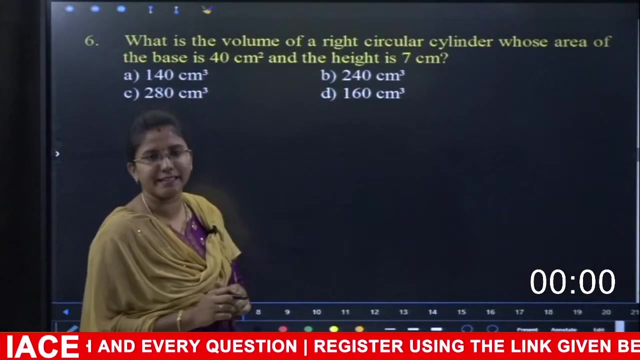 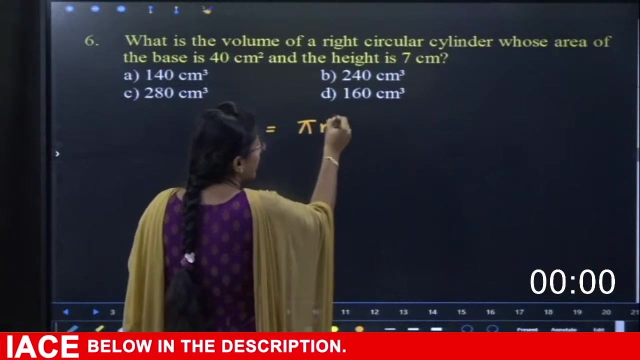 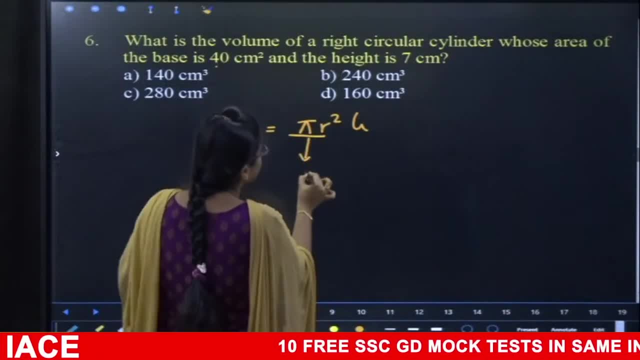 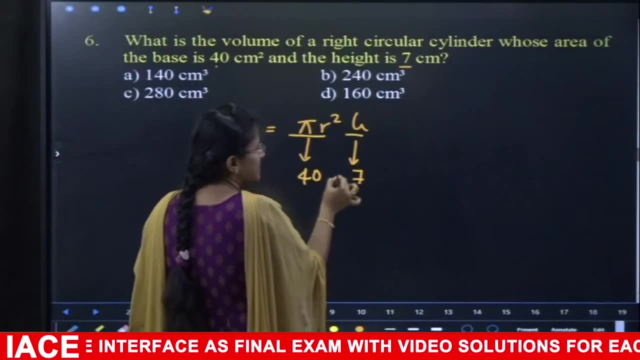 How much area has he given to that circle in the equation? Area of base is 40. Yes. Next, how much height has he given to the equation 7.. So height is 7.. These two can be simply multiplied Just 47.. Answer is 280 cm3. 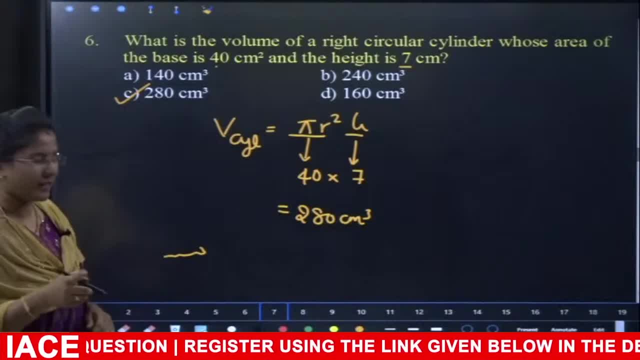 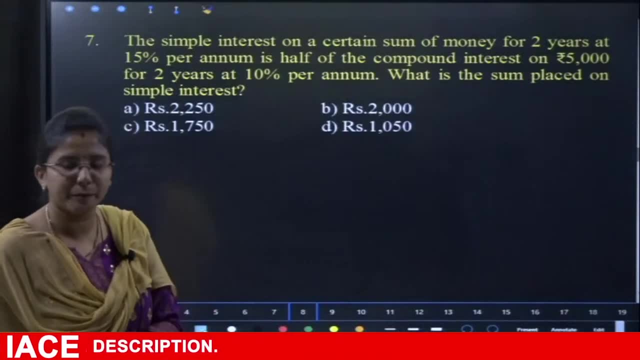 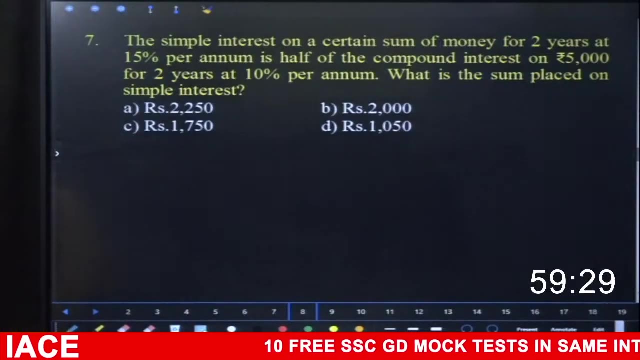 So answer option C, Ok, Next, Ok, Try this question from simple compound interest topic. One minute timer, please. How much area has he given to that circle in the equation? Area of base is U, That'swhile R square h times U value. 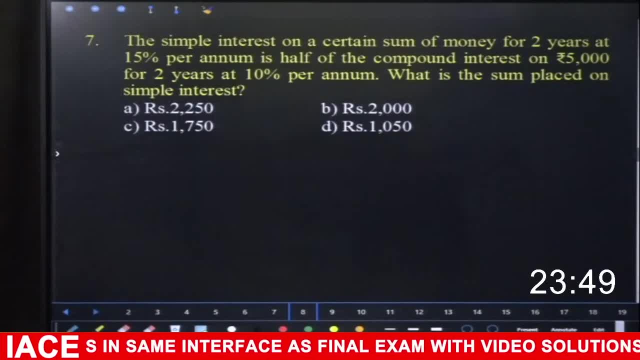 Then one into 2 minus 3 is 2.. All right, Ok, Now we fill this. Okay, All right, All right, So know we're there. And what is the area of base function Array, as you did earlier? 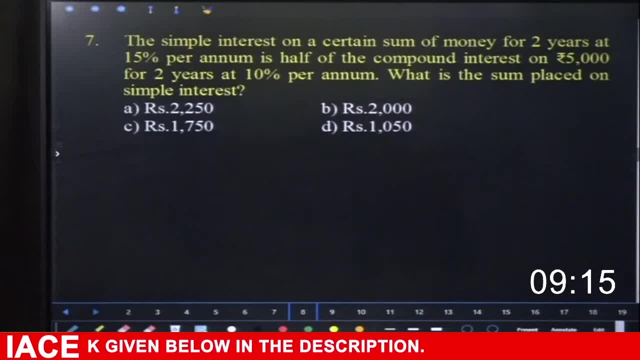 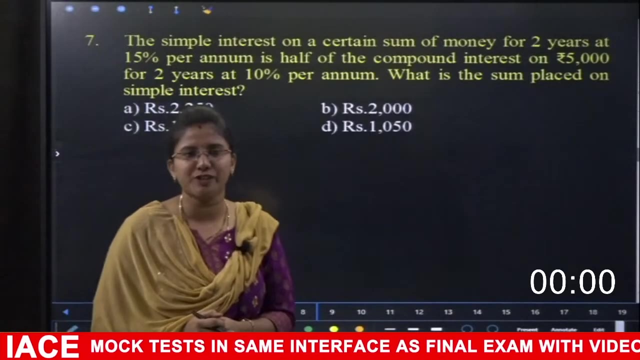 Do not give part number. Write it first. Write something Only. Do not give part number. Write all of the rewrite of the speak, the format of the strike space in the last column. Okay, your time is up, so let's solve this question. it is from topic, simple and compound. 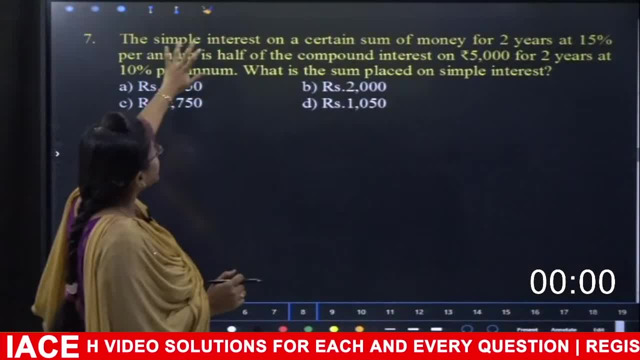 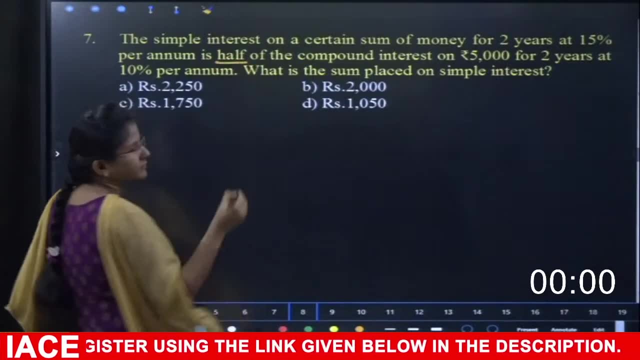 interest Here. question given. let's see it clearly simple: interest on a certain sum of money for 2 years at the rate of 15% per annum is half, what is given Half. he gave a relation like half, three-fourth, one-fourth. for us, half is 1 by 2, so let's. 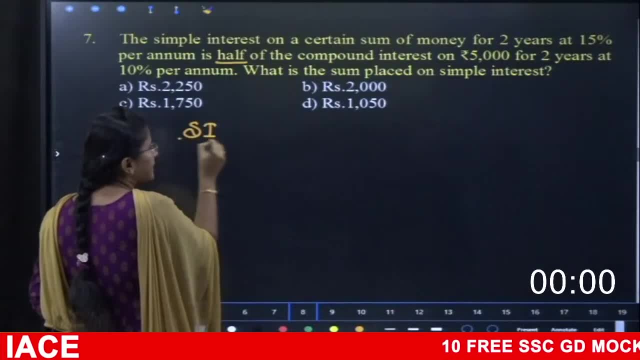 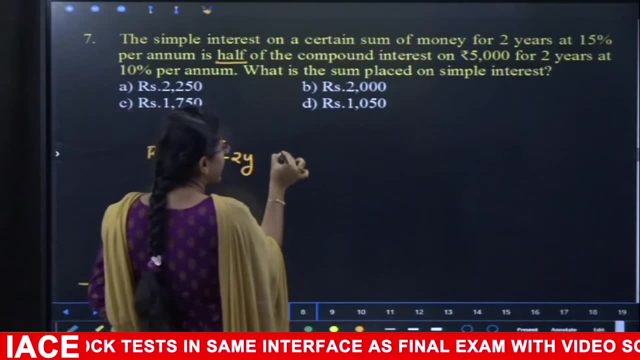 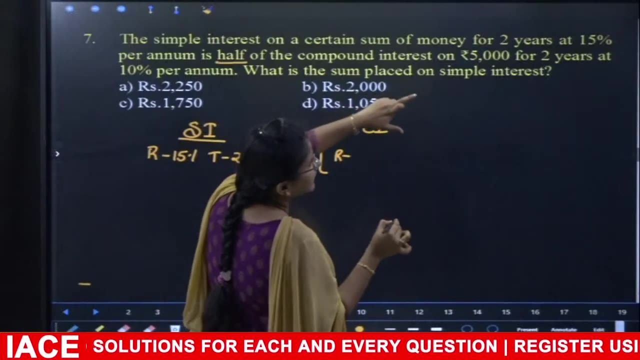 write the information given. clearly, simple interest given at the rate of how much percent? 15% for how many years? 2 years. So this simple interest is equal to that is half of on what is half compound interest at the rate of given rate: 10% per annum, 10% per annum. time in years is 2 years and the principle of compound interest is 10% per annum. 10% per annum. time in years is 2 years and the principle of compound interest is 2 years- 15% per annum. time in years is 2 years and the principle of compound interest is 2 years. 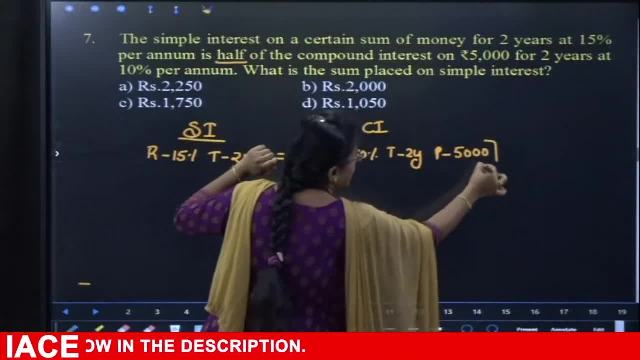 15% per annum. time in years is 2 years and the principle of compound interest is 2 years. So what is the value of the simple interest? Five thousand, five thousand for two years, 10% interest, how much compound interest will? 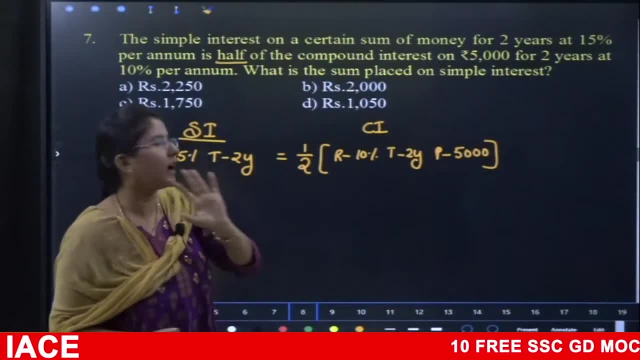 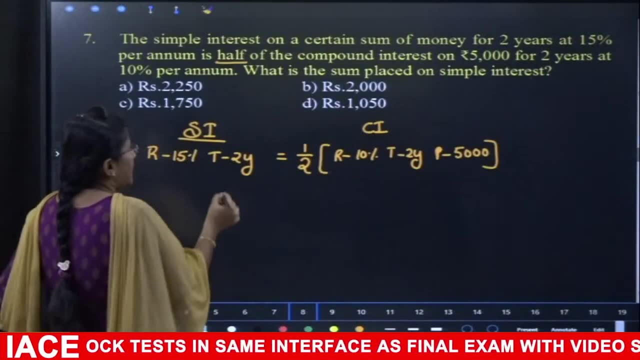 be given, in that the simple interest is half. so let's find the value first see. okay. So here, 15% is 2 years and since the simple interest is constant, we are paying 15%. for this year, in which 15% is always 100% principle, we are paying 15%. 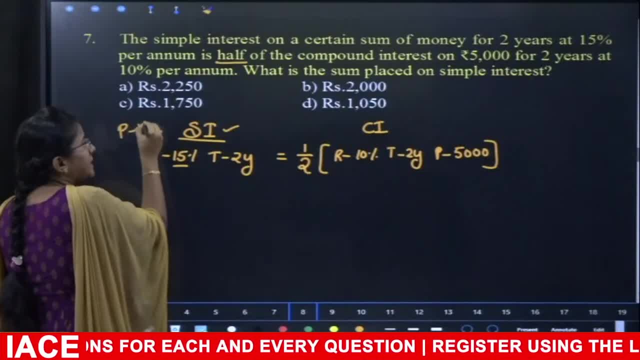 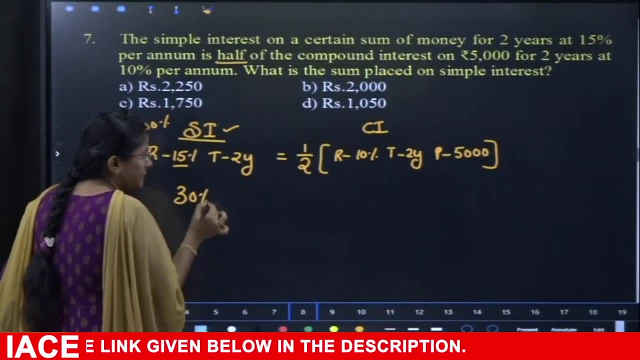 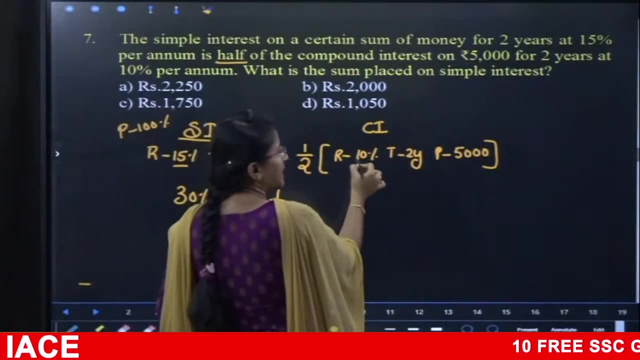 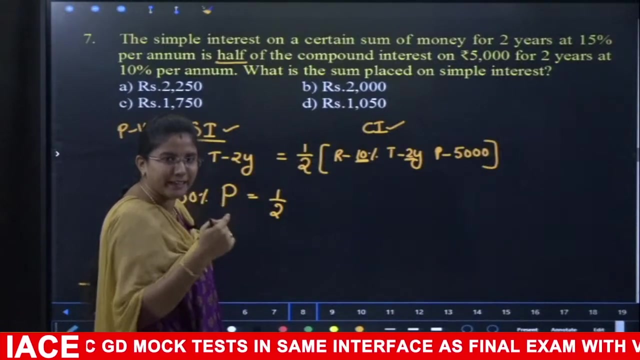 So every year. 15% for 2 years means the value is 5 percent, so we are paying 15%. The value is how much? 30%? 30% of this principle is equal to half of. let's directly calculate this every year. 10% is 2 years, but since it is compound interest, what is the overall percentage? 10.. 10.. 10% out of 10 is 1.. 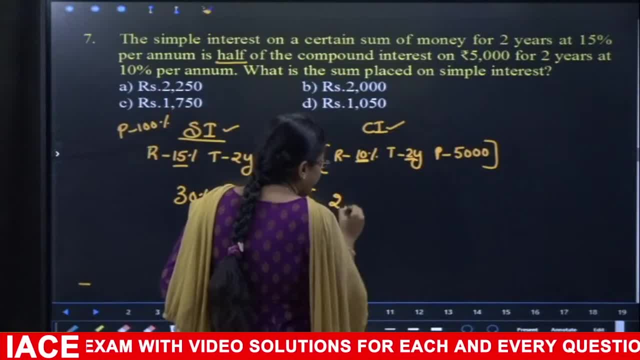 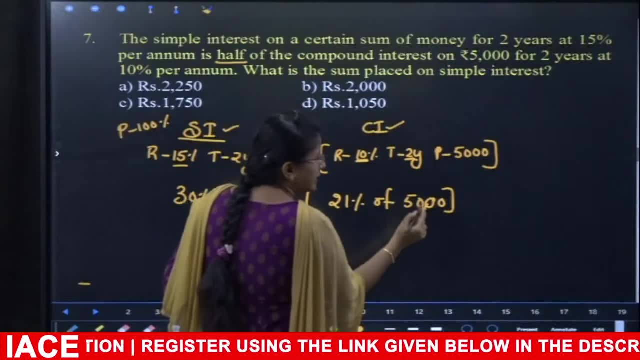 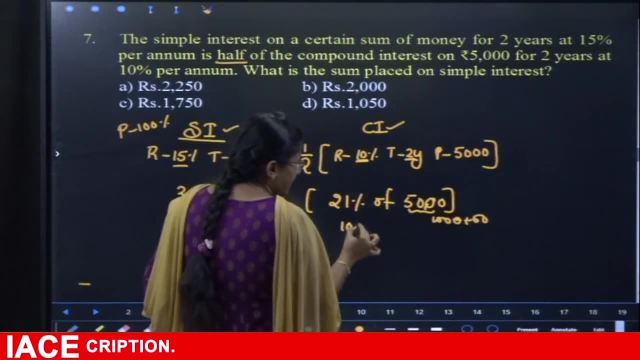 Overall. we can directly write it as: 21% is of how much? Principle: 5000.. In 5000, what is the 21% value? Higher 20%, 1000, 1%, 50. So overall interest is 1050.. In 1050, what is the half value: 525. 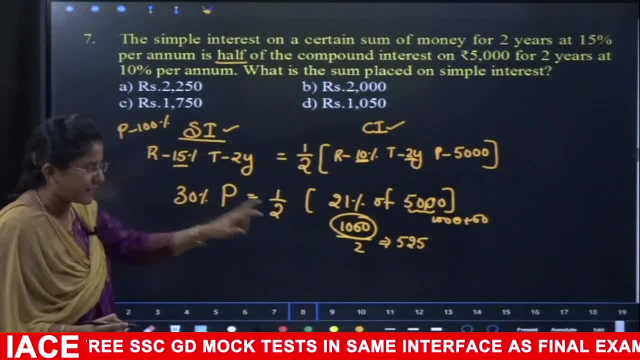 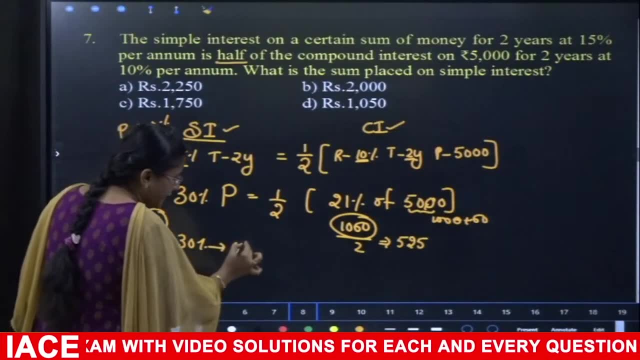 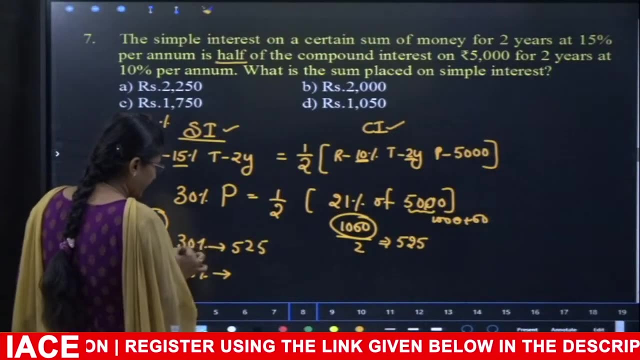 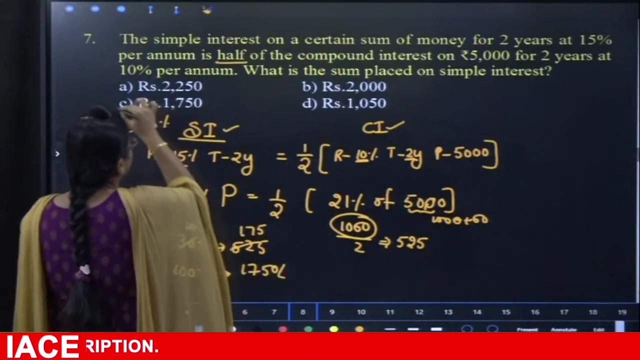 So in this principle, 30% value of simple interest is 525.. So we can directly write it as principle. So in this principle, 30% value is 525.. So how much is the principle 100%? 100% value will be here. It will be. we will do 10 times out of 3.. This will be cancelled by 175 times. So the answer is 1750 rupees. principle Answer option C. 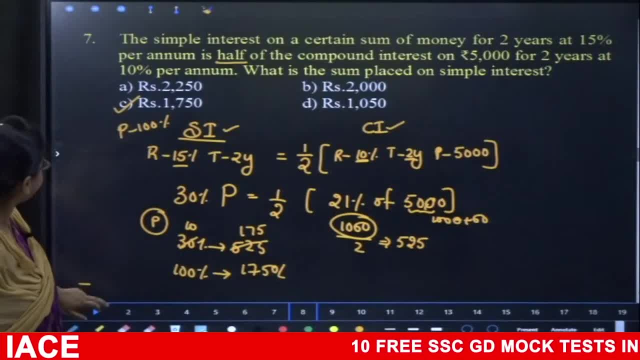 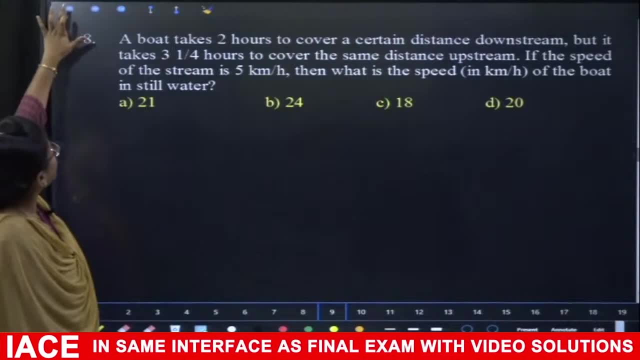 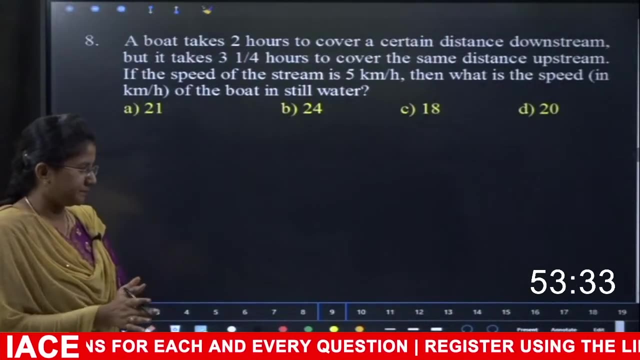 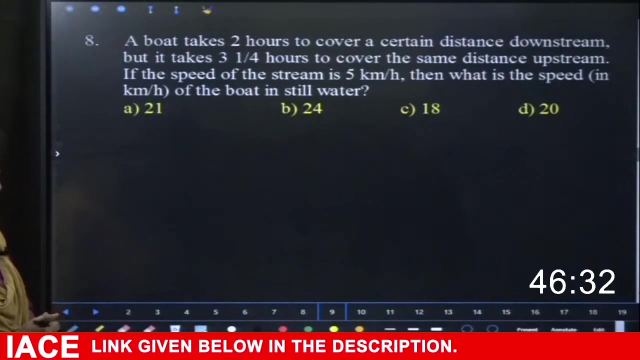 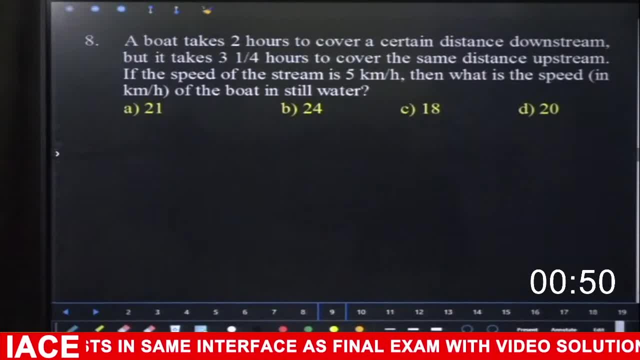 Okay, let us have a look on next question. 8 from topic boards and streams. Try it One minute timer please. Okay, let us have a look on next question. 8 from topic boards and streams. Try it One minute timer, please. 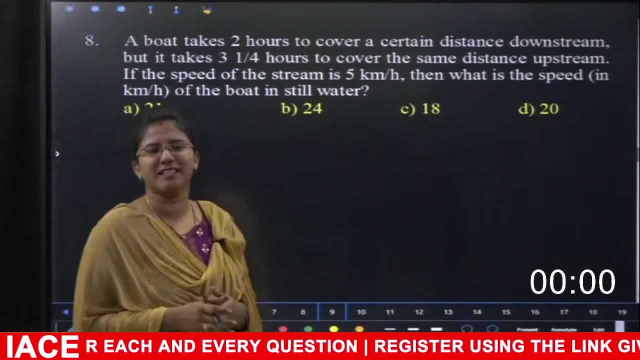 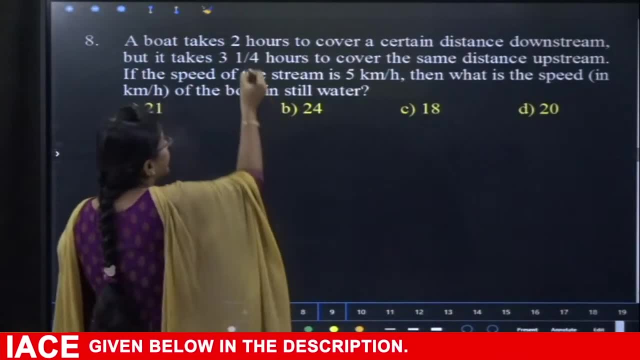 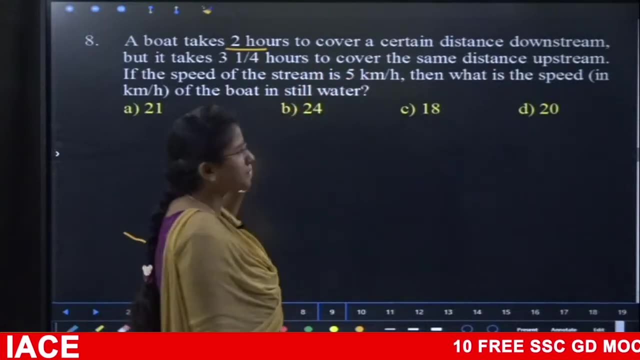 Okay, your time is up. We have understood board and stream from topic of this video. This is a very easy question. It seems very easy to understand. A board takes 2 hours to cover a certain distance downstream, But it takes 3 x 1 x 4 hours to cover same distance upstream. 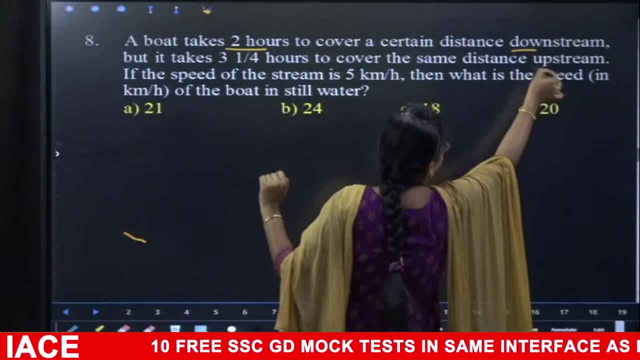 A board takes 2 hours for going downstream And it takes 2 hours for going upstream, But it takes 3 x 3 x 1 x 4 hours for going downstream. 3, 1 by 4 hours time is taken. 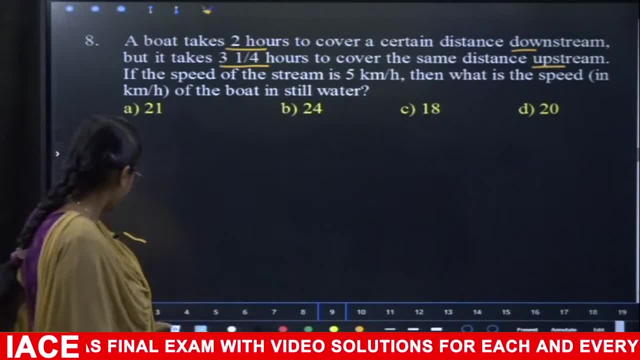 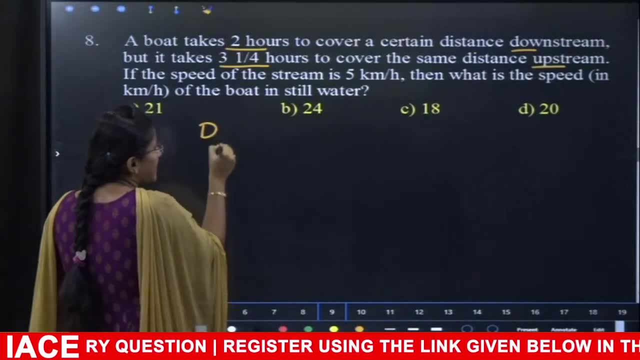 If the same distance is seen, we can solve it easily in the ratio See. Ok, So he gave downstream time. How many hours time did he give us? Downstream time is 2 hours And he also gave upstream time in the question. 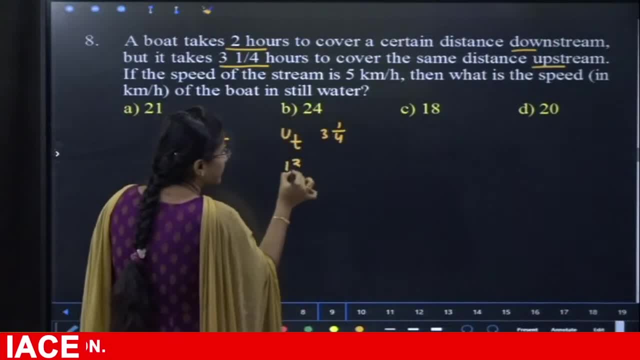 How many hours did he give? 3, 1 by 4.. 3, 1 by 4 is nothing but 12 plus 1.. 13 by 4.. Yes, 13 by 4.. Here, what will be the time's ratio? 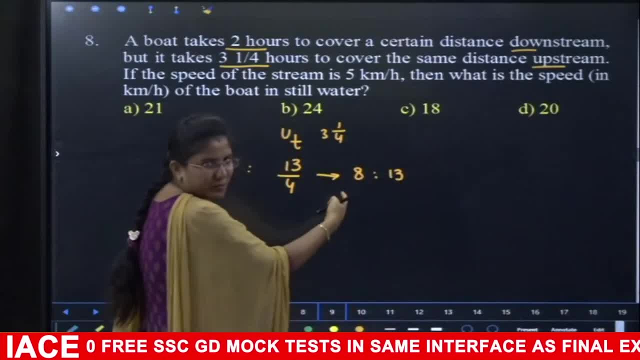 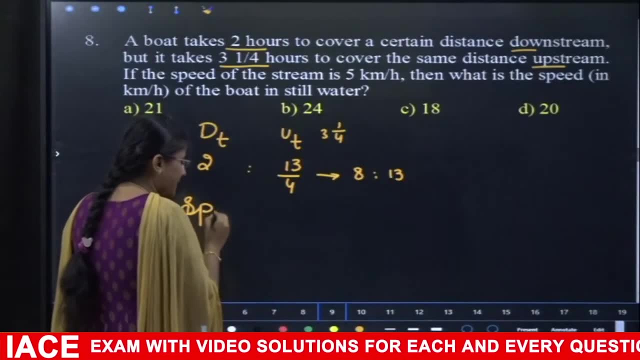 8 is to 13.. If 8 parts of time falls downstream, 13 parts of time falls upstream. So if time's ratio is 8 is to 13,. in the case of same distance, what will be the speed's ratio? 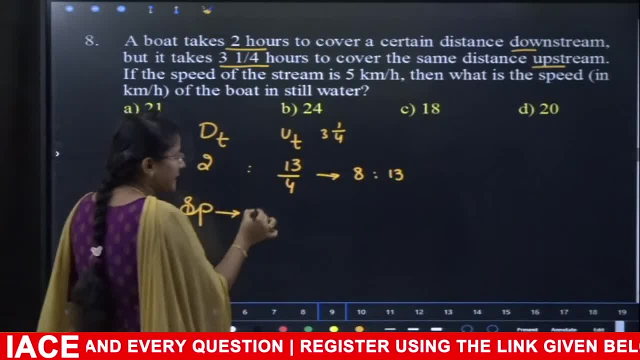 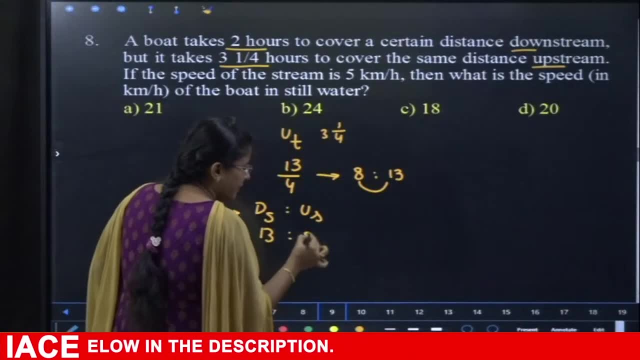 It will be inversely proportional to time. So, downstream speed and upstream speed, What will be the speed's ratio? That will be 13 is to 8.. From this downstream and upstream speed's ratio we can directly write: M is to W. 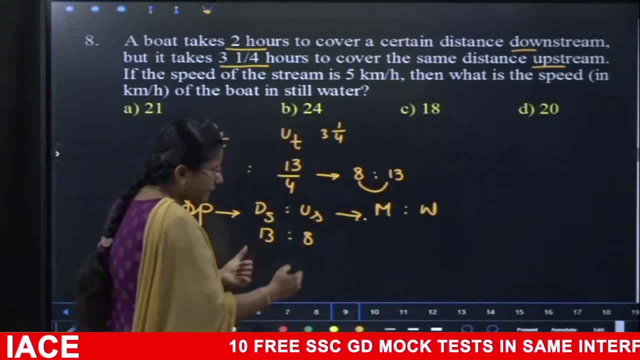 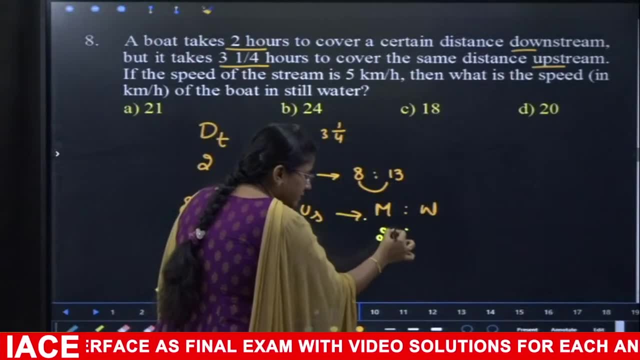 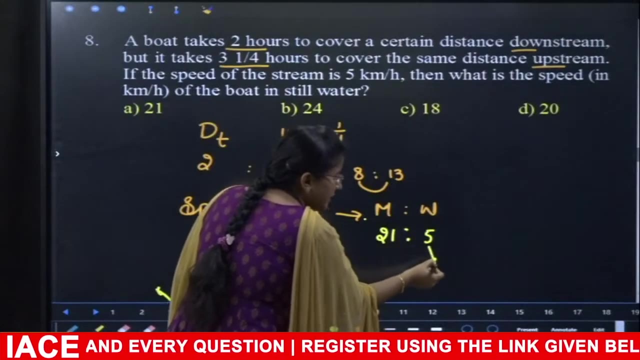 That is boat speed and water speed. If we want boat speed, add it once. If we want water speed, add it once. If we add 13 plus 8, that will be how much 21.. If we add 13 minus 8,. 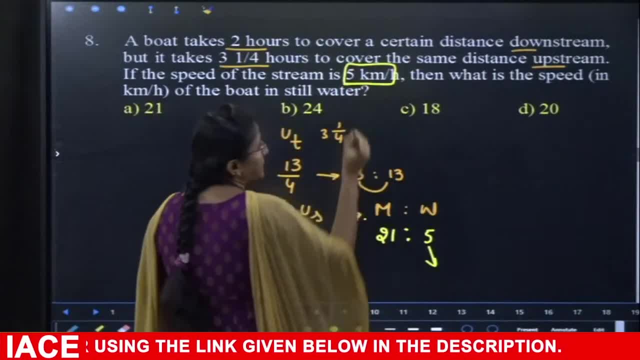 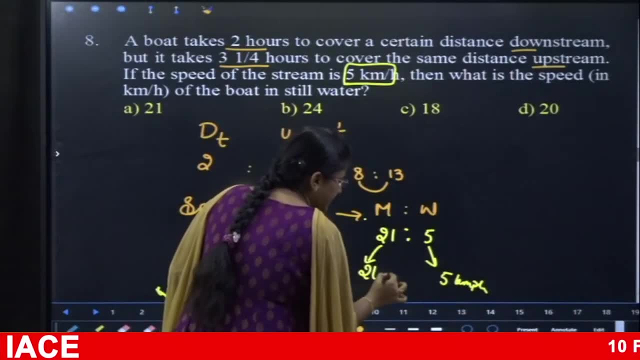 that will be how much? 5.. So we got 5 parts of water speed. He gave the same question: clearly, What is the value of 5 parts, 5 kmph? So if 5 parts is 5 kmph, 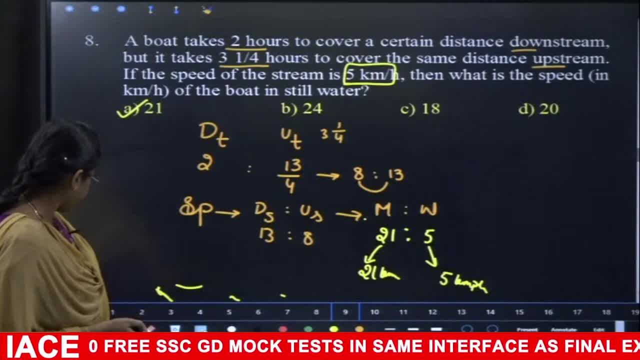 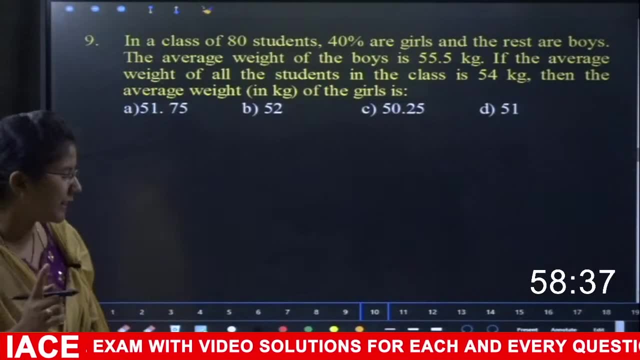 the answer is 21 parts is also 21 kmph. Let's go for next question From average topic. try it Display the timer please. There will be 1 minute timer. Try it seriously. So we have 4 minutes for each part of the time only. 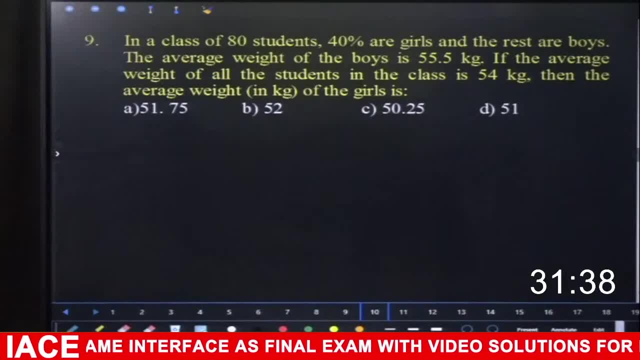 How many parts? Which part of the time? 1., 2., 3., 4., 5., 6., 7., 8., 9., 10., 11., 12., 13., 9.. 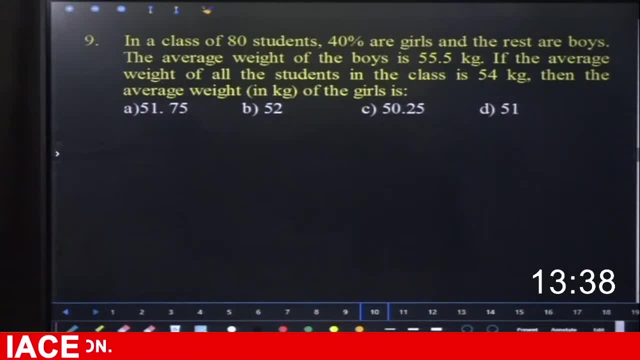 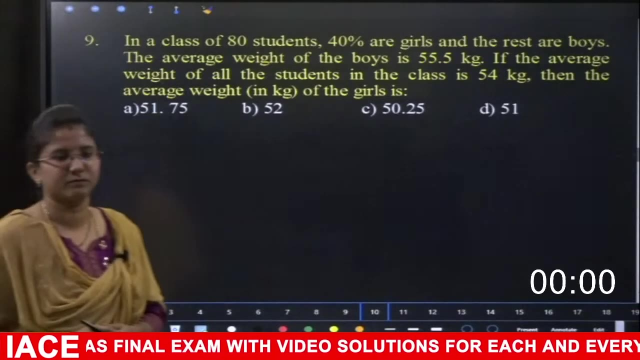 1. 10. 11. 11. 9. 2., 5. 2. 1. 1.. Okay, your time is up, So this question has come from the averages topic, So let's solve this. 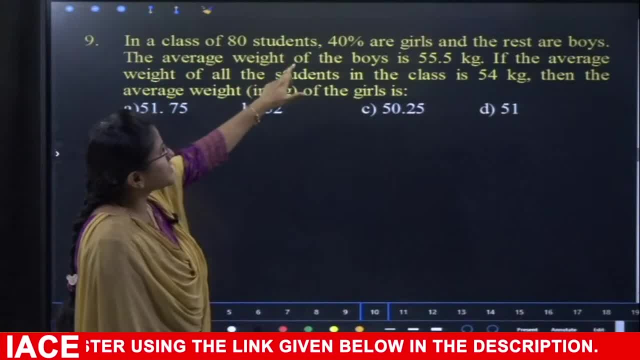 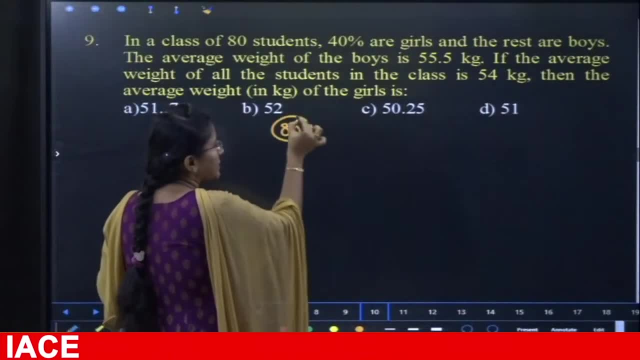 See, In a class of 80 students, 40% are girls and rest are boys. Let's write the first sentence: Number of students: 80 members are there. In 80 members, girls are 40% Boys. how much percentage are remaining? 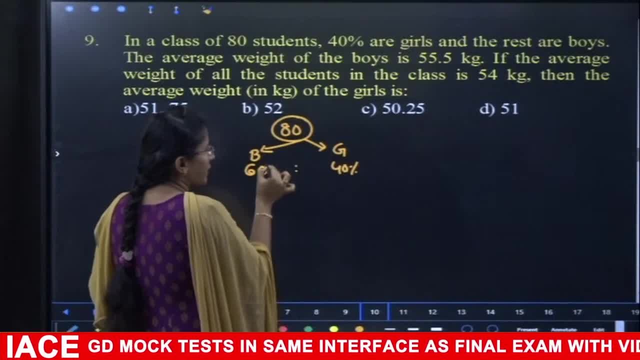 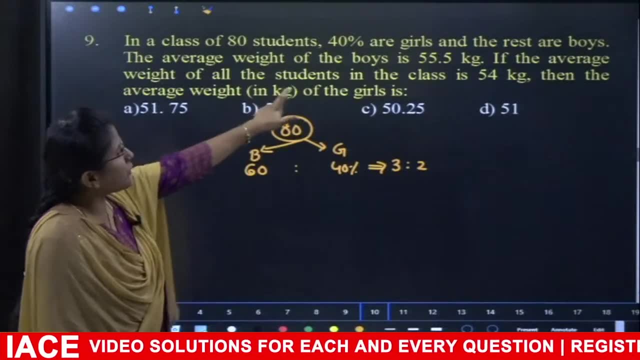 Yes, 60% is. So ratio will be 60 and 40. If we write the ratio, it is clearly 3 to 2.. Next, Average weight of boys is 55.5 kgs And average weight of all the students is 54 kgs. 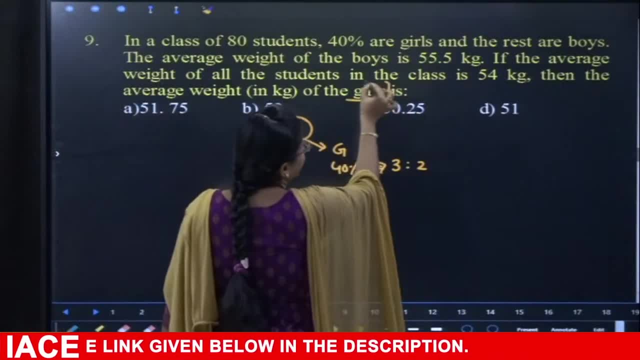 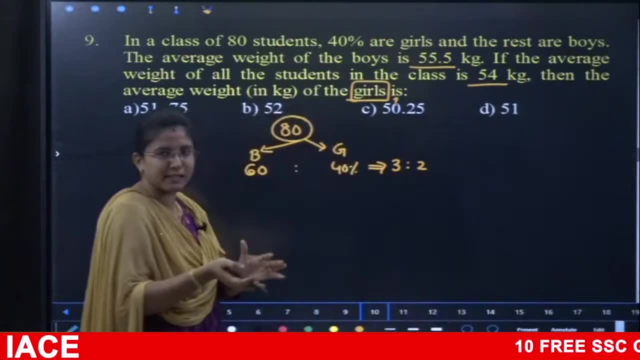 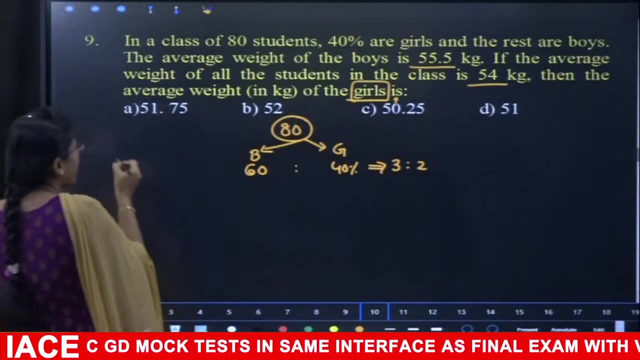 The question asked is: what is the average weight of girls? There is a question on girls. Boys averaged 55.5.. And all students, boys and girls, averaged 54. So we can use the allegation rule. See here. in the allegation rule the average weight of the boys is 55.5 kgs. 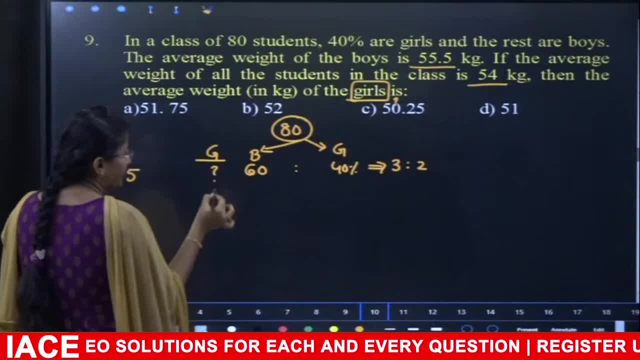 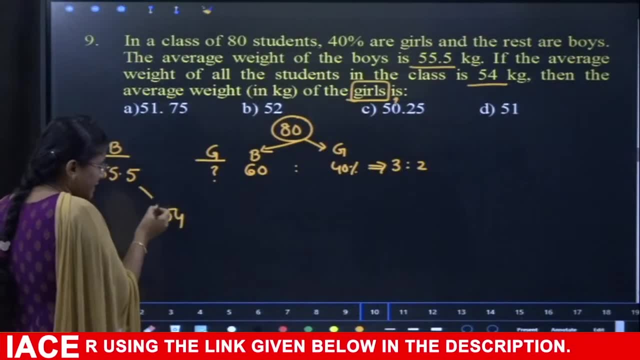 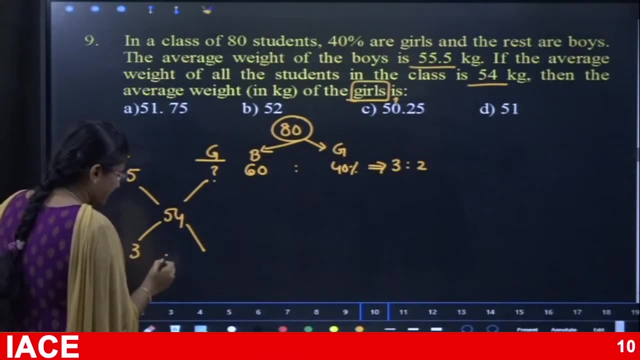 Girls average. we do not know about it, We need to find it out- And overall average in the class is given 54. If we write the averages, we can write the number of boys and girls. So we have already written it: 3 to 2.. 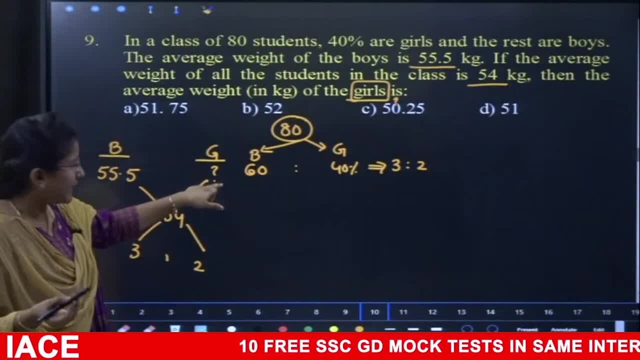 So, whether we can give this, you can verify it with the options given here, Or else we can write the ratio of the boys and girls, Since we know one side, 55.5 and 54. Difference is how much. 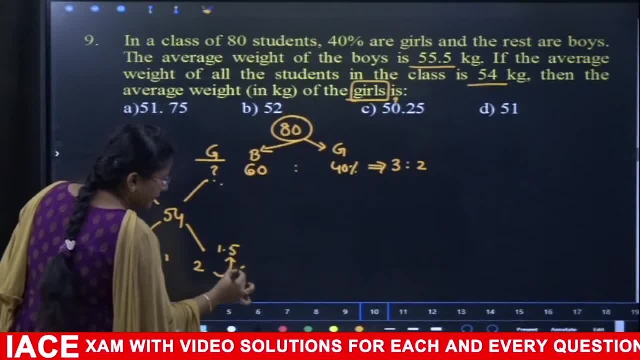 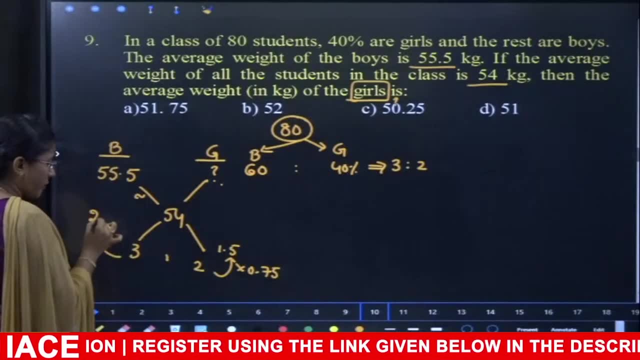 1.5.. So if two parts value is 1.5, then one part value is 0.75.. Next, if we do 0.75 three times, that will be how much 2.25.. 3 into 0.75, how much is it? 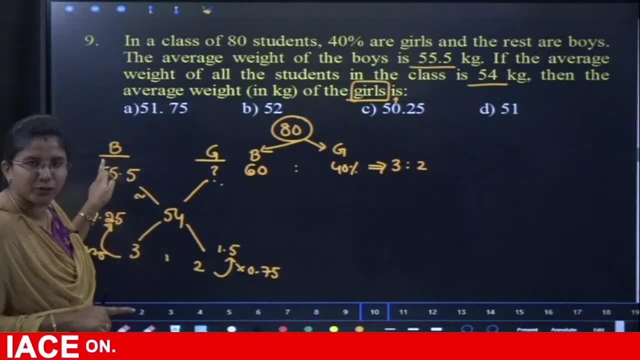 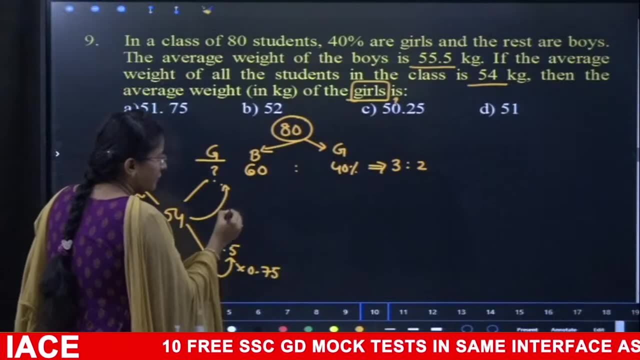 Clearly 2.25.. So since 54 has a bigger value, it will definitely be a smaller value. How much difference will there be? 2.25.. So answer is 54 minus 2.25, that is 51.75.. 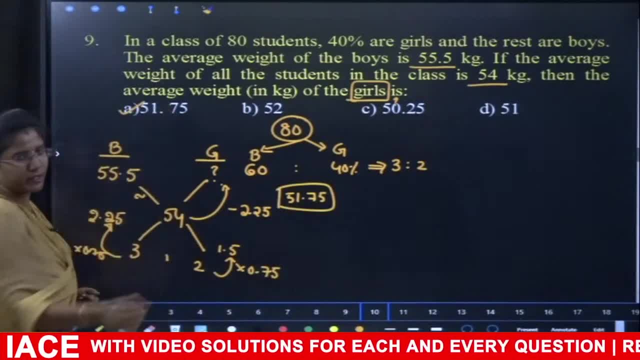 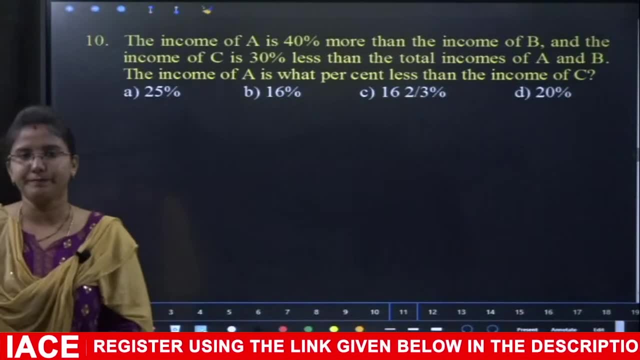 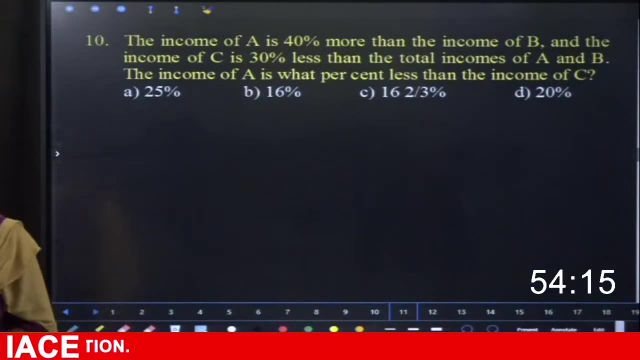 Option. enter nandi, option number A. Okay, understand all of you. Next Let us go for 10th equation. So equation tries: JND: one minute timer. display the timer, please. How much is the mass? 53 x 62 and 800. 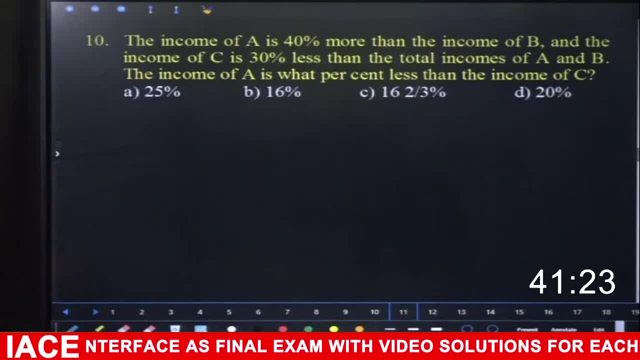 5x that 9.. There is 3, 2.5 inside 2.6.. Why is the k-1? It is a ratio of negative 2.5, 1 to the k-2 minus 1.. So 2 x k-2 minus 2 is not a value of 1.. 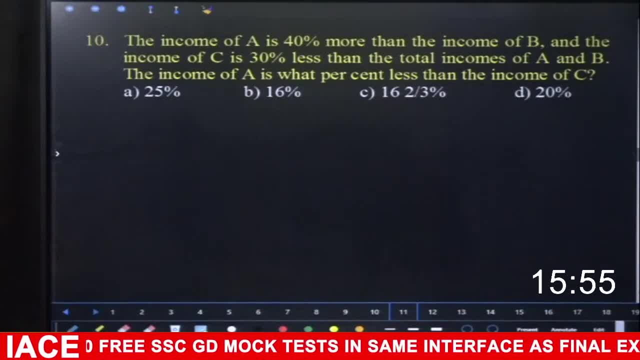 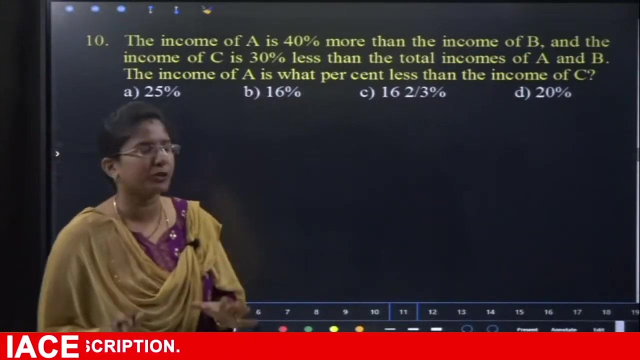 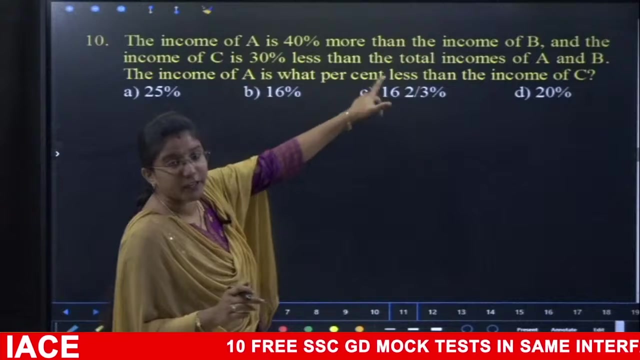 Okay, your time is up. This is the equation from the percentages. It's a very easy equation. Here, income of A is 40% more than income of B, And income of C is 30% less than total incomes of A and B. 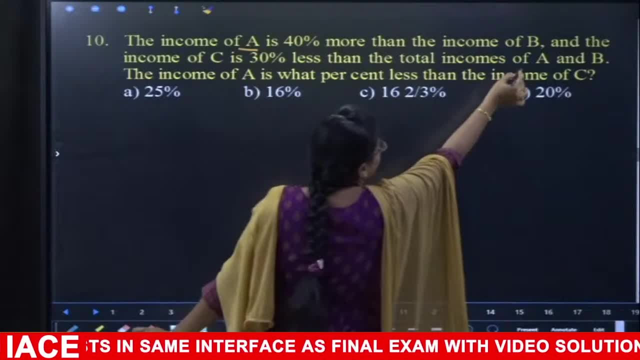 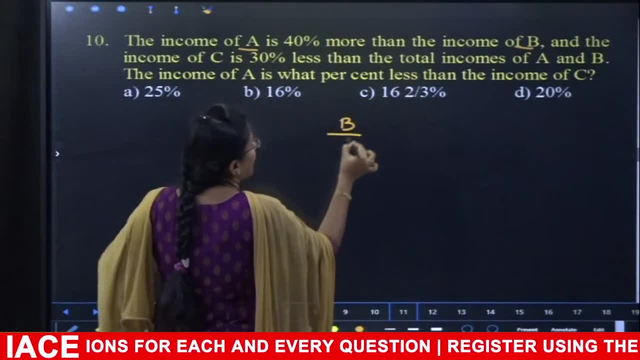 First sentence is in the relation: Income of A is 40% more than income of B. He gave the relation to A and B, So we will clearly write A and B. A is 40% more than B, So A is 40 more than B. 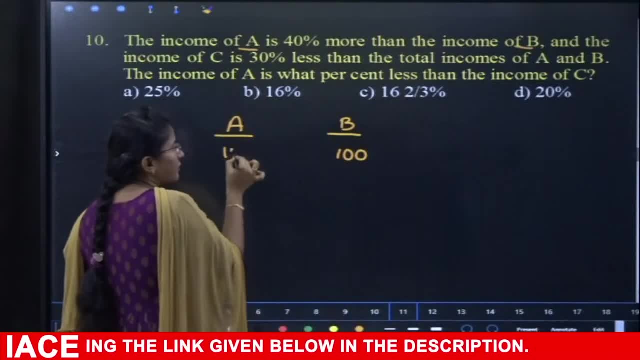 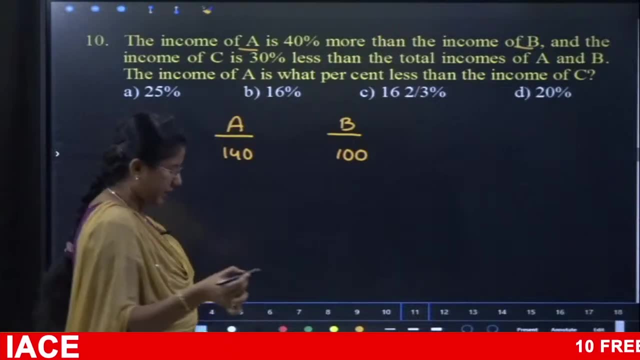 So if I take B as 100, A will be how much 140.. Okay, Next sentence is: income of C is 30% less than total incomes of A and B. How does C income exist? It is less than total A and B. 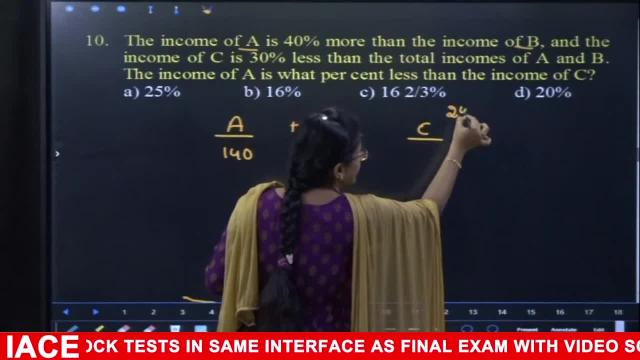 If both A and B are combined, how much is 140 and 100?? It is 240.. It is less than 240.. It means it is less. We will put minus How much less is it? It is 30%. 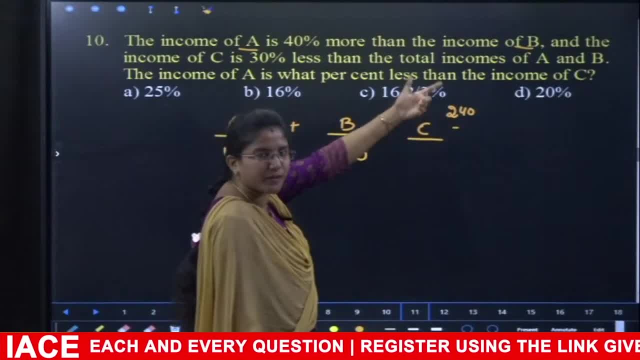 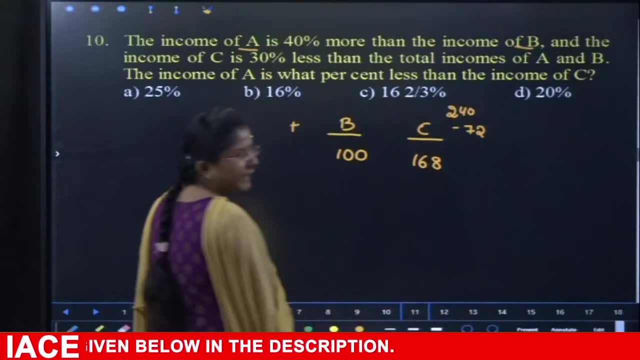 We have to see 30% in this. So 24: 3s. 30% means 24: 3s How much 72. So if we deduct 72, it is 168.. So here, if we think one number is 100, all 3 or 4.. 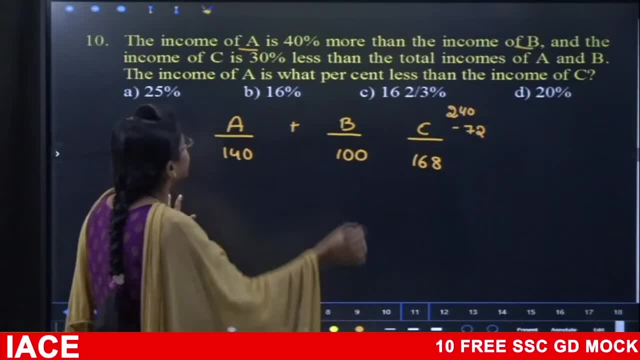 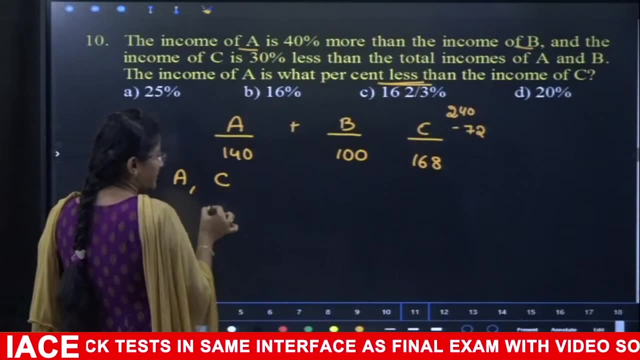 No matter how many relations we give, all those numbers will be deducted. So question is: what is the income of C Income? is what percent less? what percent less than income of C? Which income, How much percentage, is less than the C income? 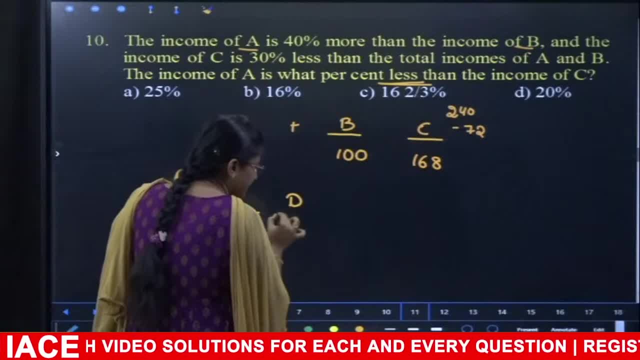 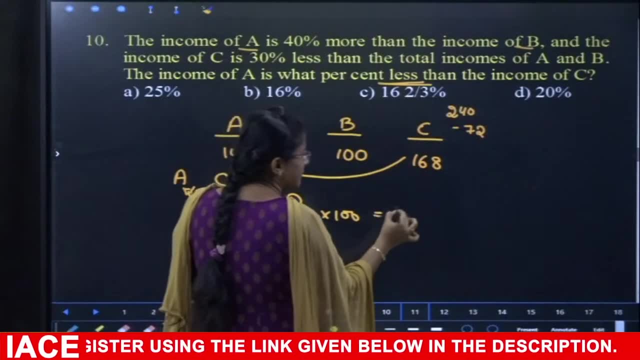 He is asking for less percentage. What is the less percentage? We will write it: Difference by highest value into 100. Difference between the numbers is how much? 140 and 168.. What is the difference between the numbers? 28.. 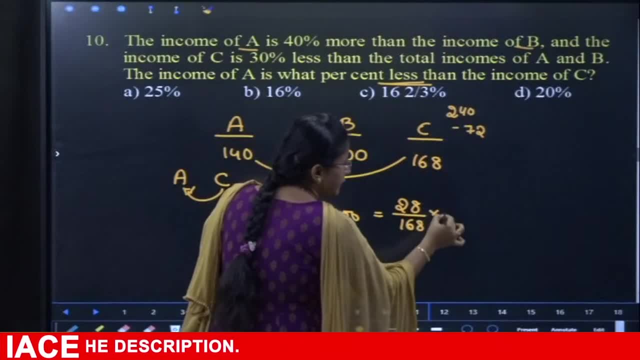 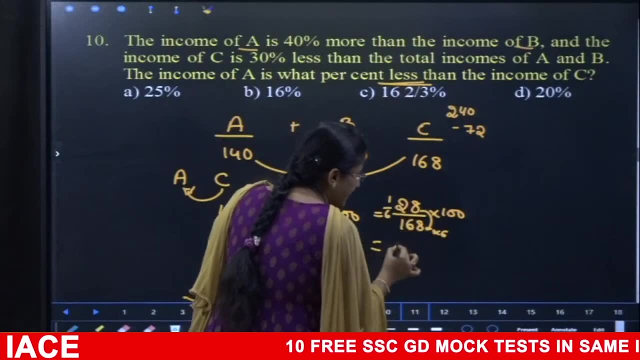 And here denominator highest value among them is 168 into 100.. 28,, 168.. Clearly it is 6 times more. So 1 by 2., 1 by 6.. 1 by 6 and the answer will be 16.. 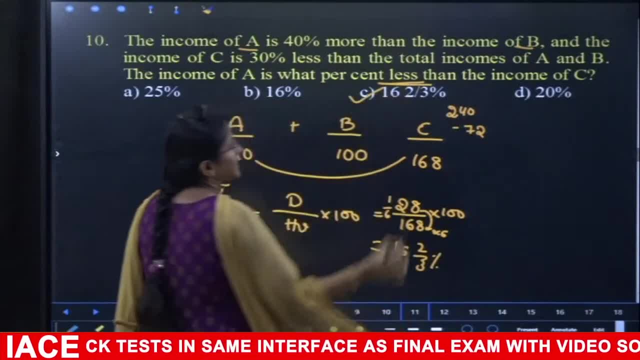 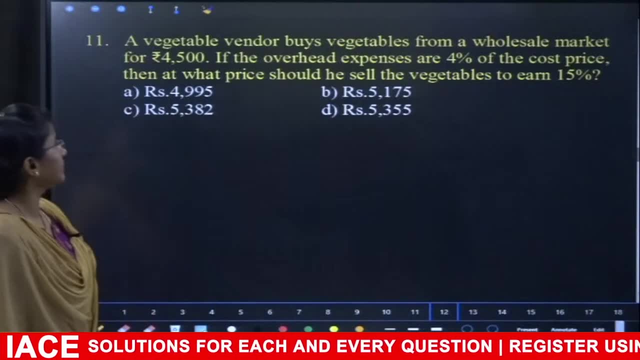 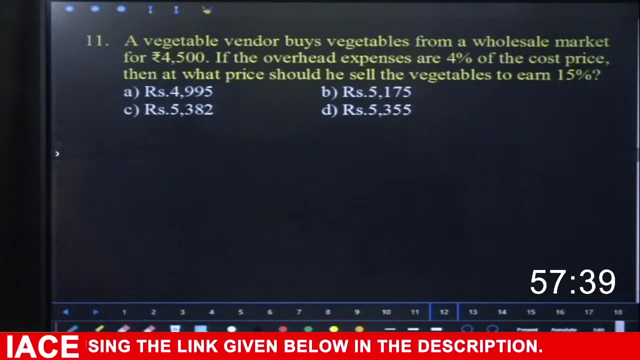 2 by 3 percent. So that is option C. Okay, all of you. Next. Next go for 11th question. Okay, try this question. There is a one minute timer. Display the timer please: 1, 2, 3, 4,, 5,, 6,, 7,, 8, 9.. 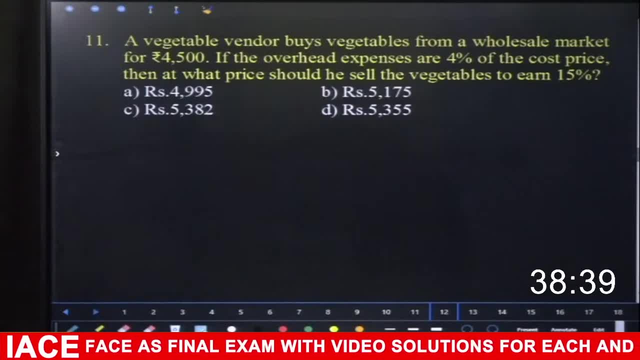 Is any one of you using the timer when you are not on call hours and on call time? Yes, All of you are using the timer. All of you are using the timer. We will now do the questions and answers. These will be given to the questions, to the questions. 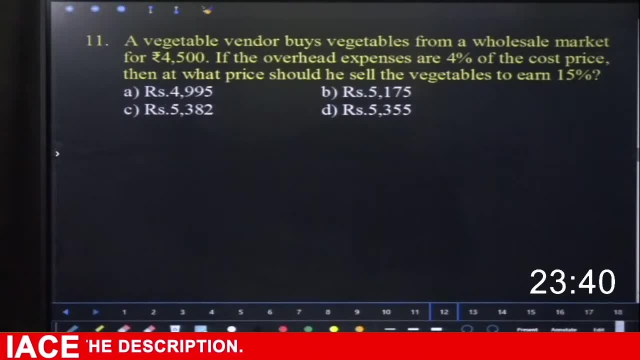 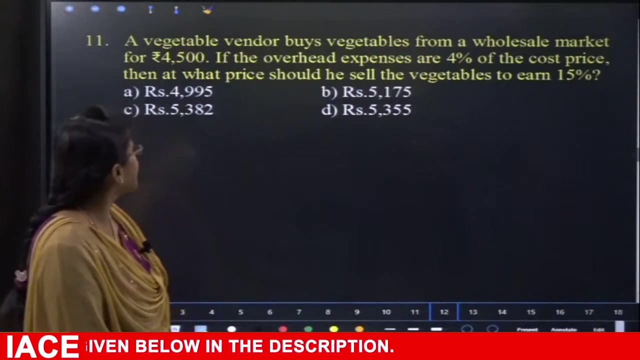 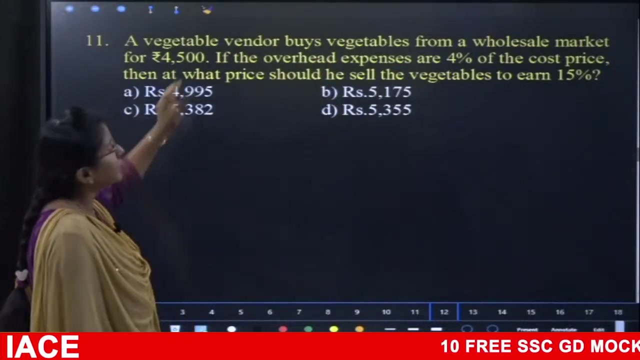 On and off. we will give our answers. We will give them our answers. Are the questions answered? Yes, Okay, your time is up. So equation judandama: very easy. equation chala: easy. A vegetable vendor buys vegetables from the wholesale market for 4500. 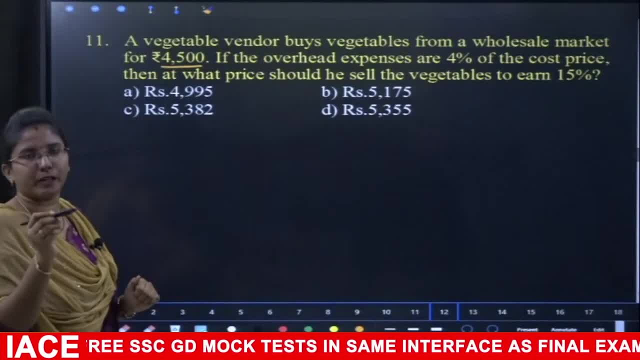 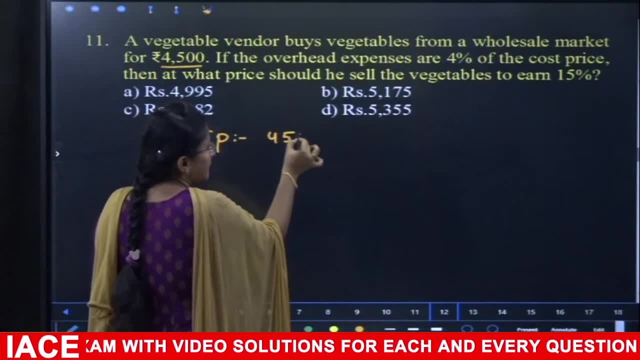 Buys means bought, bought vegetables for 4500 rupees. So because bought means bought, that is nothing. but what Cost to price? cost to price, given 4500.. If he gets overhead expenses on this, 4500, means transportation or something like that. 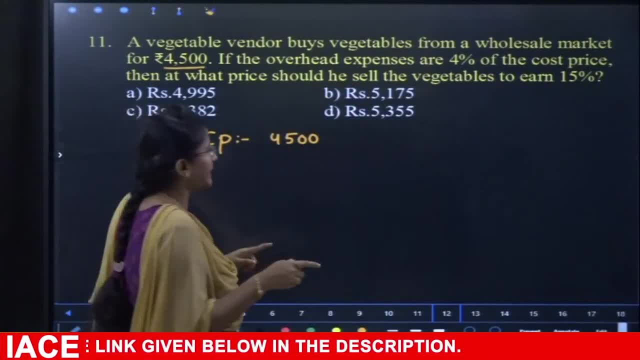 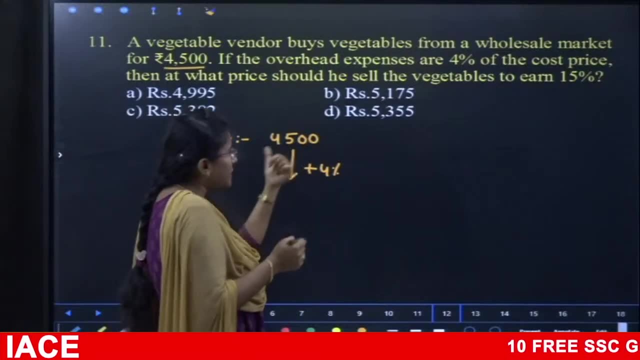 we call it overhead expense. we calculate that also in cost price. So here it is given 4%. So 4% on 4500.. So 1% means 45.. If you multiply 45 four times 45, four cities 180.. 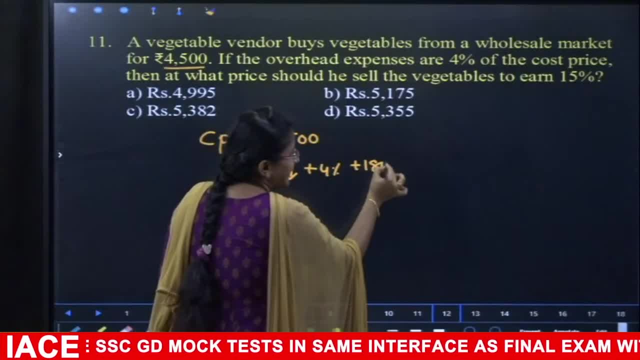 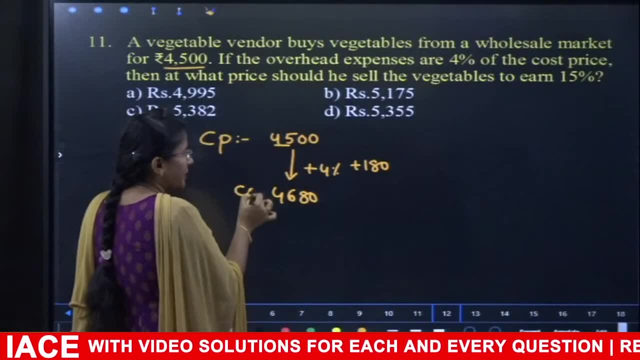 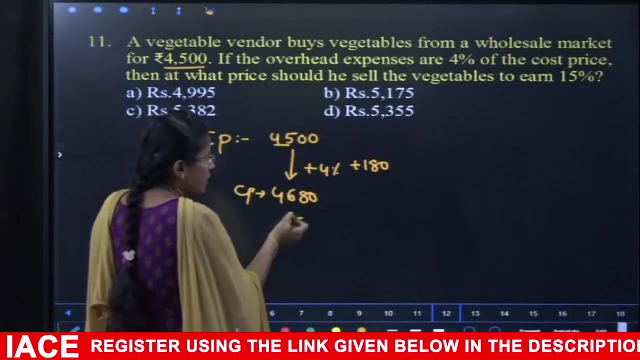 So that will be total 4680 rupees expense. This is total cost price. So now, if you have to sell these vegetables, you have to see profit or loss in it, only On this 4650.. See how much profit do you want to get on this 4650?. 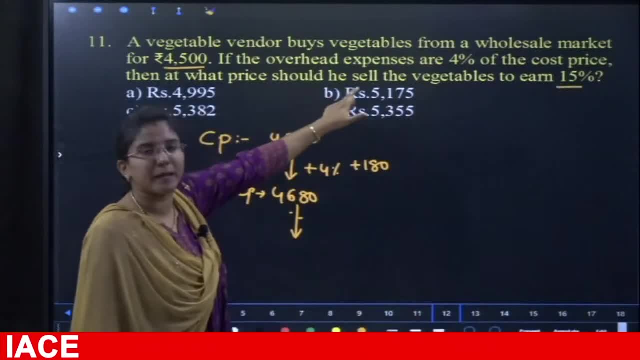 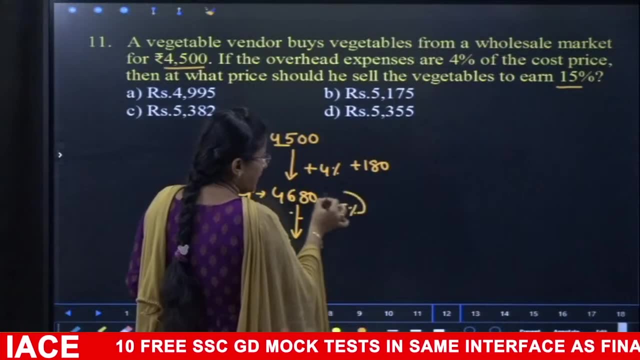 15%. So what is the selling price? How much is the selling price? 15% profit. So let's take 15% in this, 15% value on 4680.. 10% is 468.. 5% is half in this. 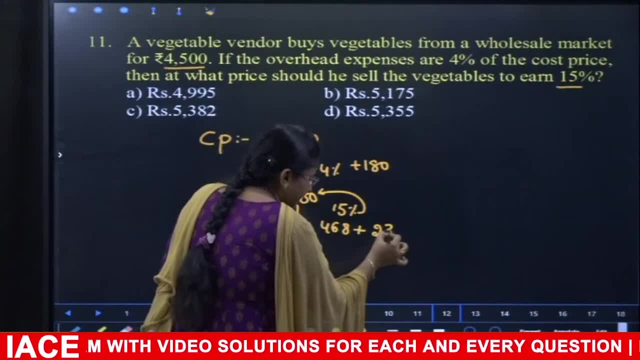 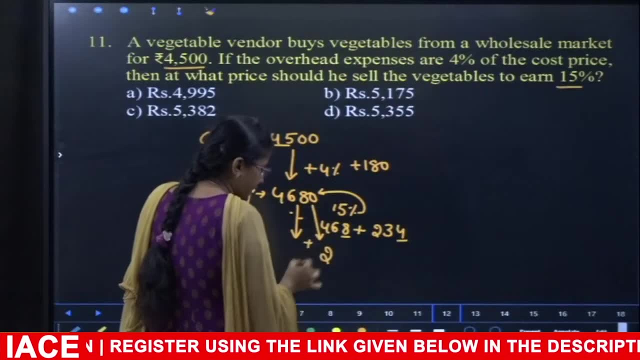 How much is half 234.. So 4 and 8.. If we add, the unit digit will definitely be 2.. Since there is already 0 here, 0 plus 2. Unit digit of answer will be 2.. 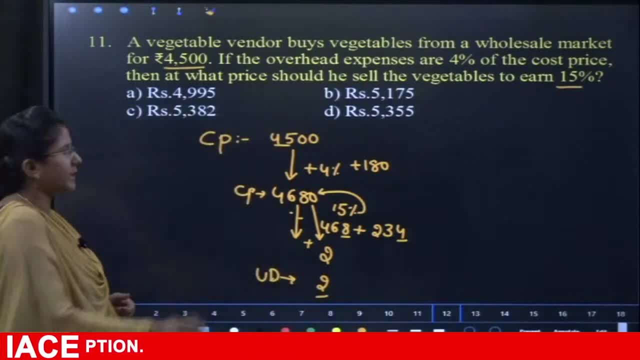 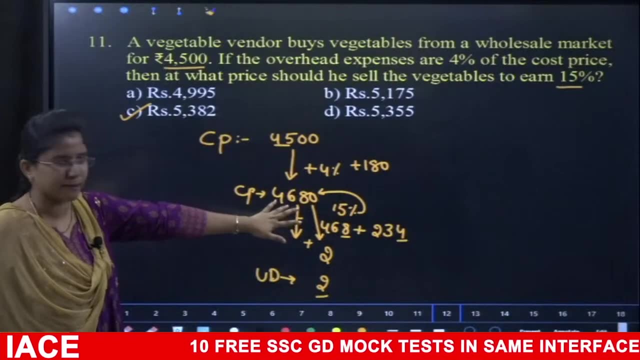 If there is only one option like that, we will put only one answer. So the answer is we have only one option: C 5382.. That is it So? cost price: we have added overexcited expenses and we have filed selling price. 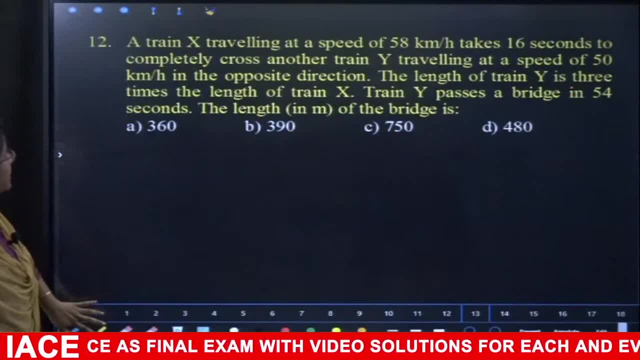 So understand all of you. Next, Let's see the next question. It came from trains, topic 12th one. So one minute timer, please Try it. One minute timer has started. Let's see the next question. Are you free to ask questions in the chat? 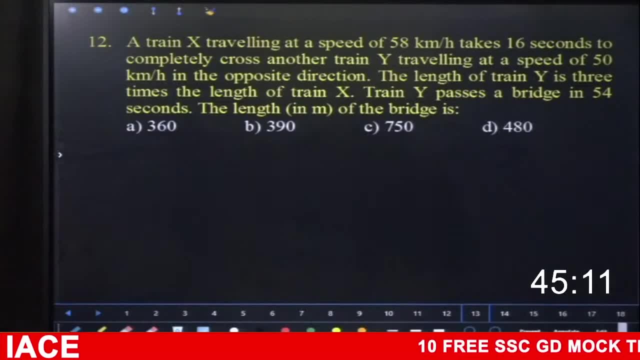 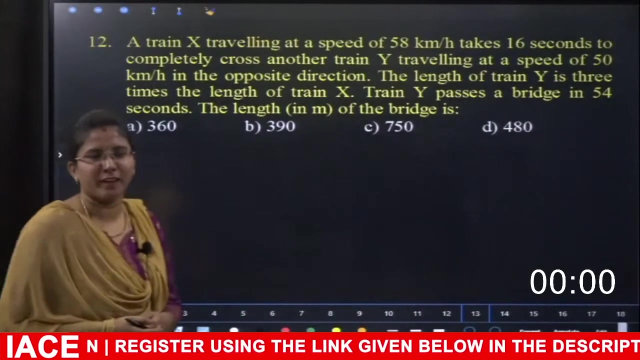 If you did not answer. the next question is from the audience. Caution for the next question. our next question is from its own name. Okay, your time is up, So let's solve the equation from the topic of trains. 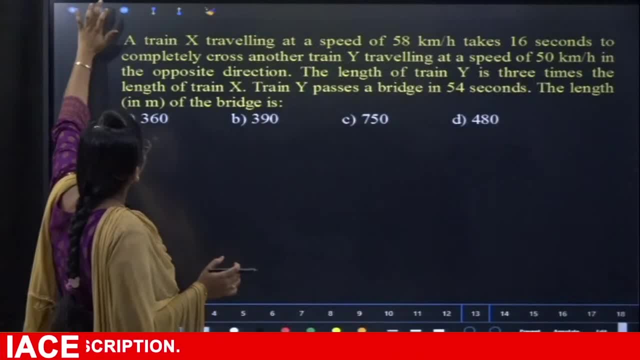 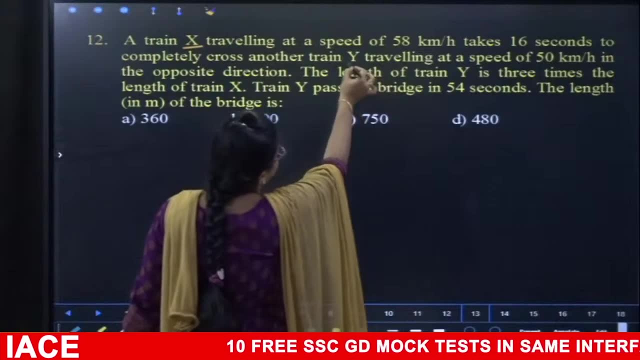 So let's solve the equation from the topic of trains. A train X traveling at a speed of 58 kmph takes 16 seconds to completely cross another train Y traveling at a speed of 50 kmph. The first sentence is very clear. 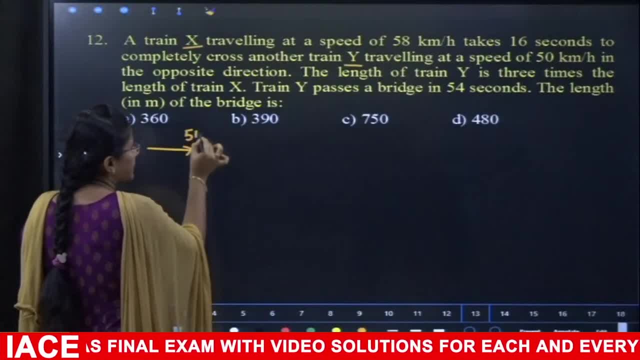 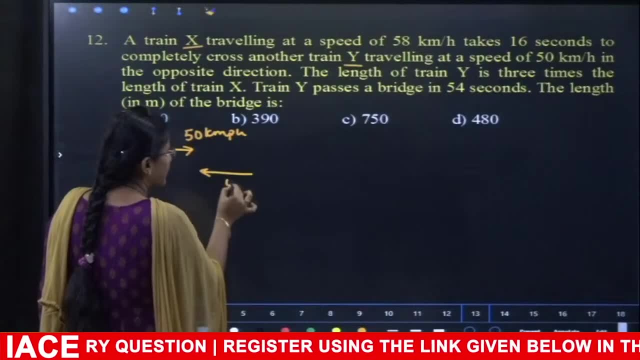 There is a train called X. How fast will the train go? 50 kmph. Let's write the direction in which it crossed. He said opposite direction. So it is crossing train Y traveling at a speed of 50 kmph. So it is crossing train Y traveling at a speed of 50 kmph. 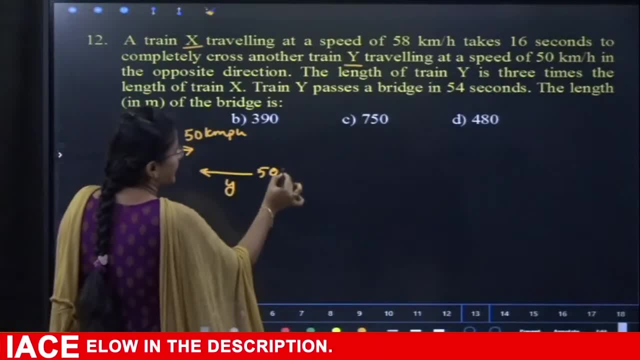 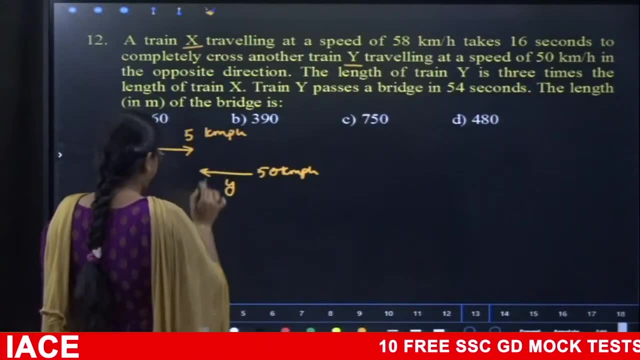 So it is crossing train Y, traveling at a speed of 50 kmph. So this is speed of 50 kmph. Next I'll change the line X to 58, okay, So since it crossed in the opposite direction, what is the distance travelled? 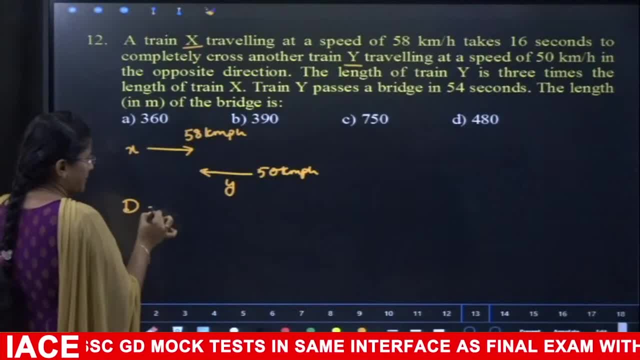 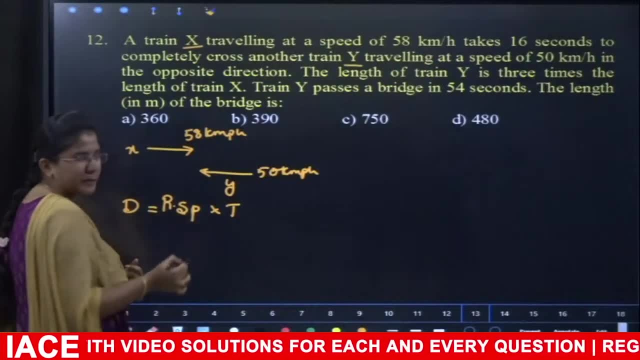 Since it crossed in the opposite direction. what is the distance travelled? Let's write it. We know the formula of distance travelled, equal to the speed times time. So this is how the speed in the moving train is снatched and the relative speed nessecured to the other two train member. 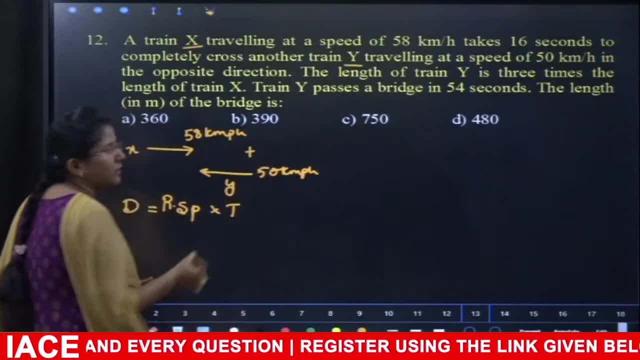 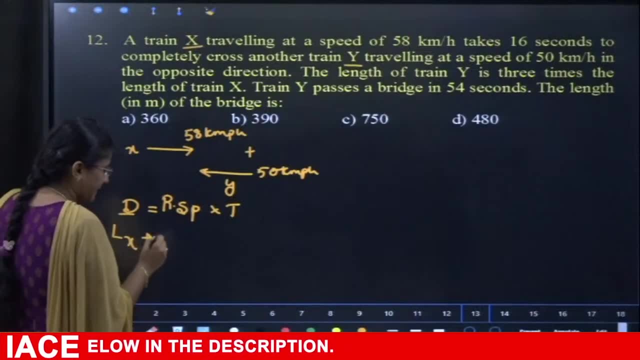 Since they are at the opposite direction, we will add two speeds just in time. So here, compliment: Distance travelled equals to the speed you have is kmsh-30.. will be E train, E train across Jason, and a length of train X and plus length of. 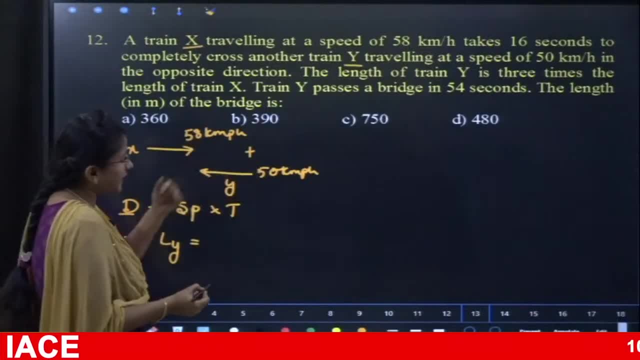 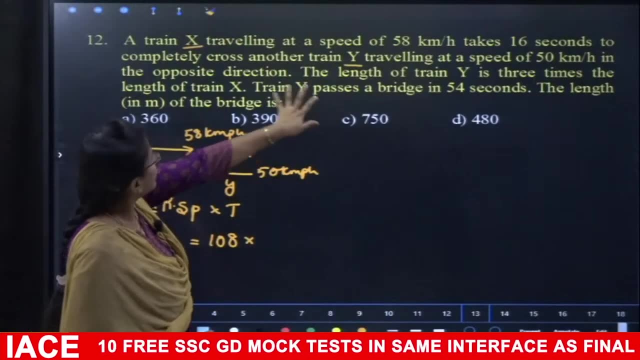 train Y is equal to delay, to speed. 58 plus 50 dot latches the 108 kilometer per hour into each net. I'm any second slow? no, it is crossed in how many seconds. 16 seconds, and you can enjoy. only take 16 seconds, 16 seconds on to. 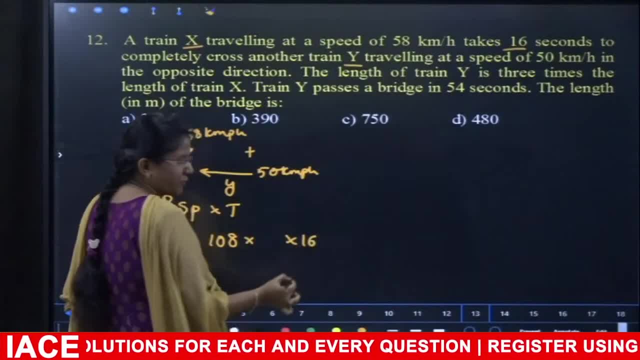 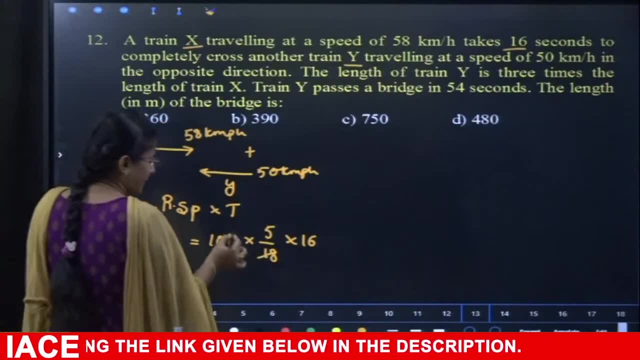 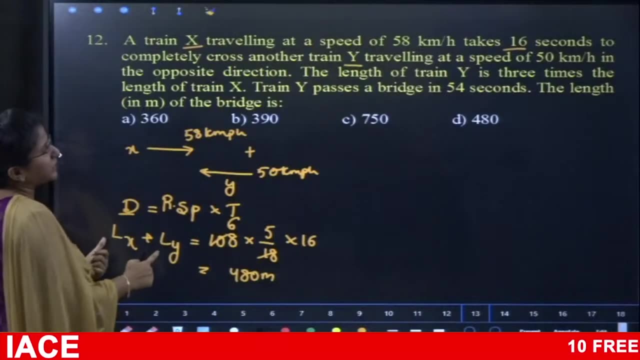 not cover T into 16 waste amo. I did the KMPS loan in seconds long the cover T into monica для m the second of March 11ez, five weight in�. so here it will be six times. then it is a for 80 for 80 meters Shh preview. it's a relational along date trainer length. 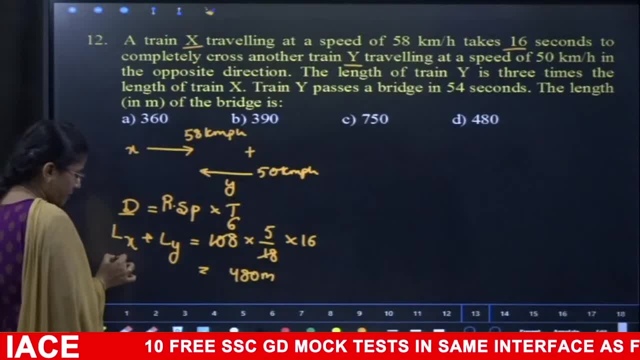 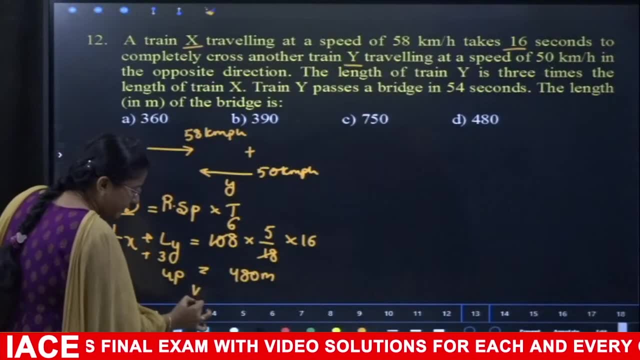 of trained Y's. 3 times length of train X&R. empty, the 1 part winter, the three times capacity, three parts. so one plus three, totalzza by 4 parts or 184 parts, or it is then will be 1 part value. yes, 120 meters universe. so length of train. 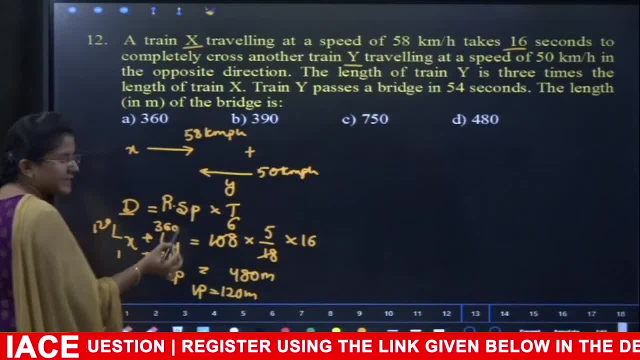 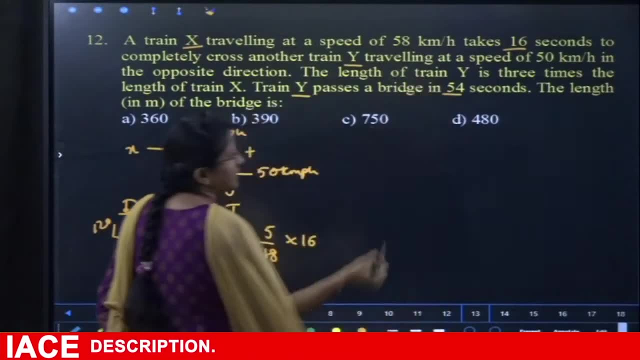 Esdanen length of train way is 3 times 123 is 360.. Next question is: that is the train way passes the bridge in 54 seconds, then what is the length of the bridge? This is the same train way. this time it crosses the bridge. 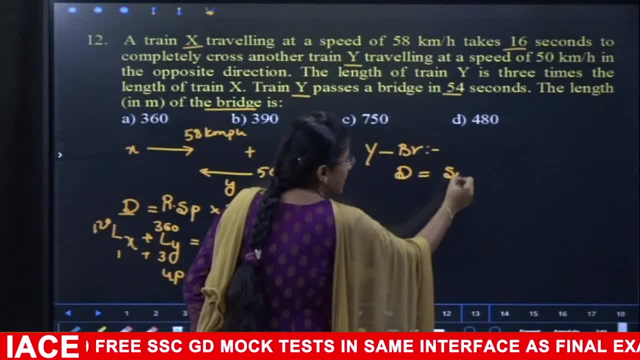 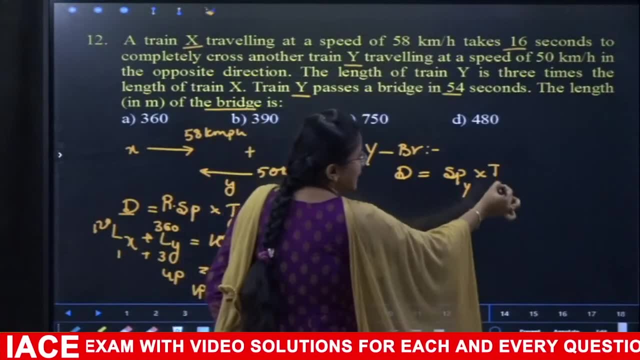 Here again we will write the same formula: Distance equal to speed into time Who is crossing the train: Y. So we will take speed of Y. Second time he used is 54.. Distance: we have to write If the train comes and crosses the bridge. 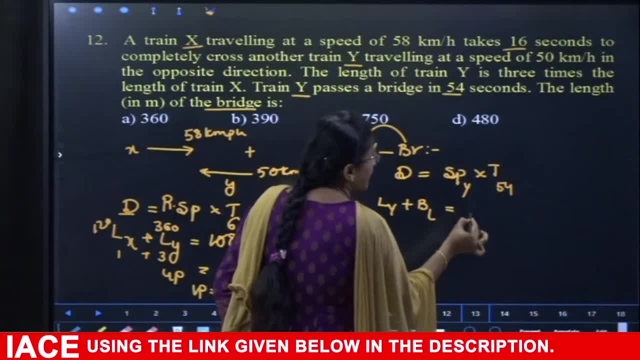 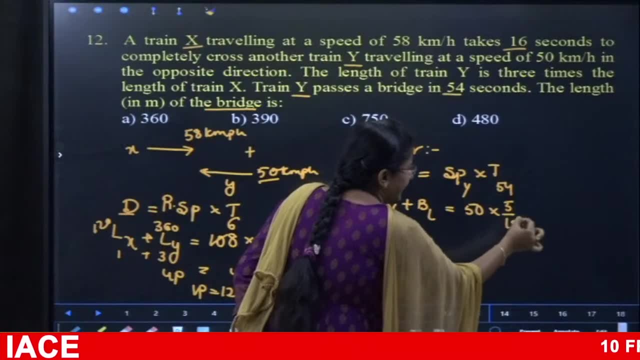 length of Y plus bridge length equal to speed of Y. how much did he do Already, given in starting itself 50 kmph, 50 into 5, by 18, into time, given 54.. Here length of Y we already got, so we will write 360.. 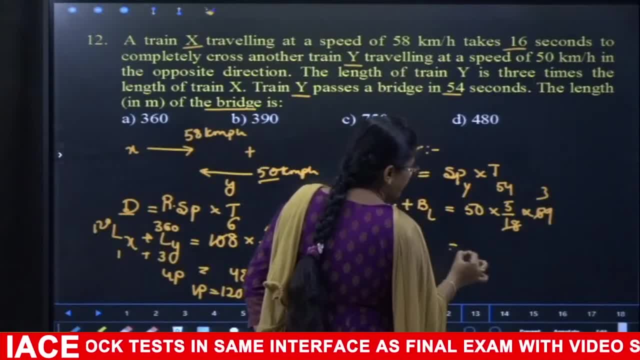 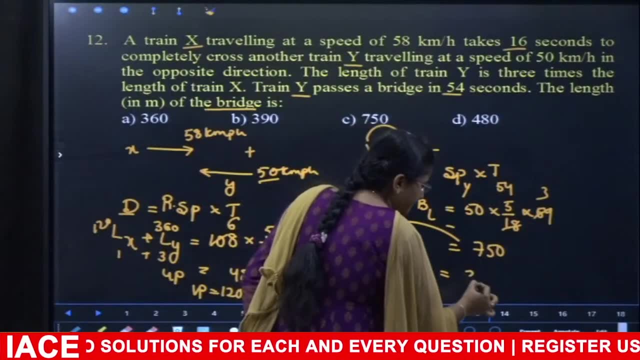 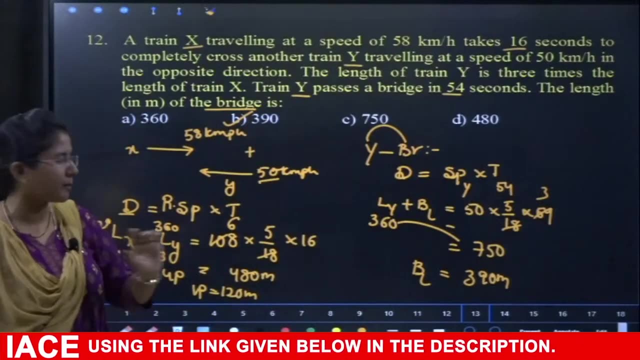 So 18, 54 will be for 3 times, So 253 is 750.. So bridge length will be answer: 750 minus 360.. Answer is what? 3 90 meters, Option B, So distance equal to speed. into time, We will use only one formula. 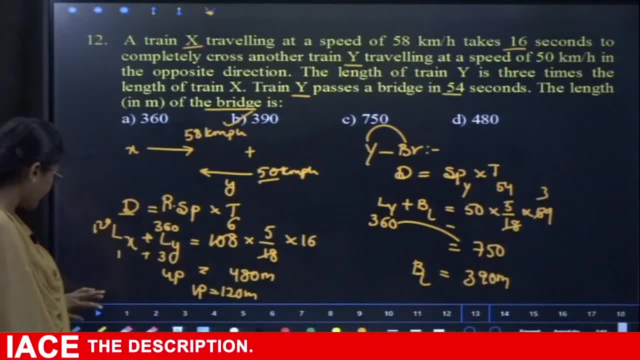 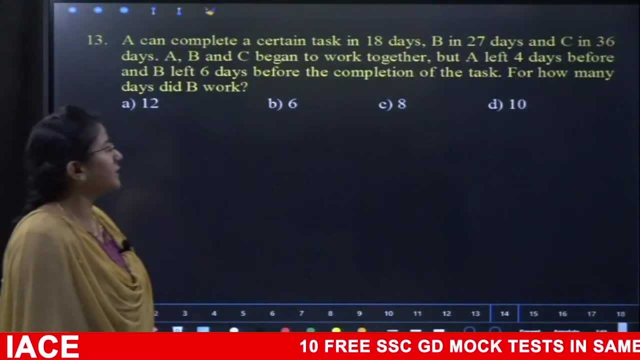 in this equation- So easy. There is nothing else in this. Let us see the next equation. Let us have a look on it. 13th one from time and work topic. Try it Display the timer, please. One minute timer. 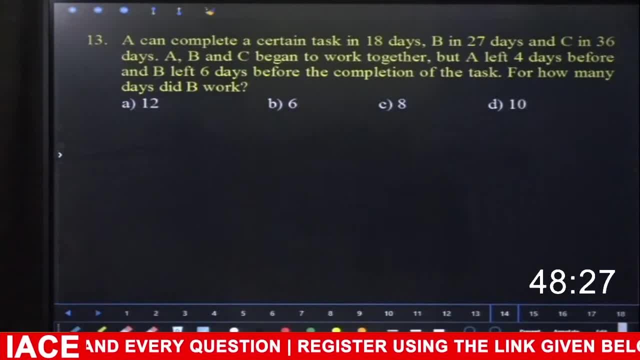 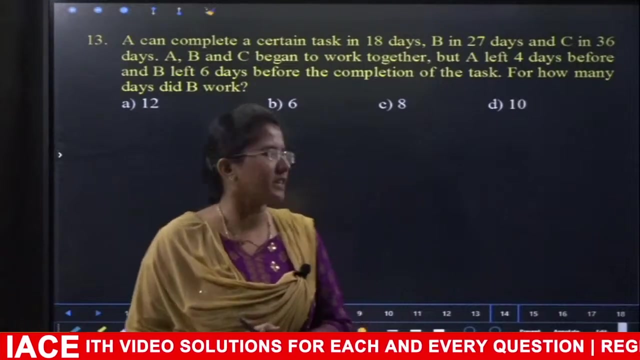 1 minute and 20 seconds Difference here. Notice that. So okay, your time is up. So equation solve: chetamandi C time and work topic: ninchi, very important. model A can complete a certain task in 18 days. 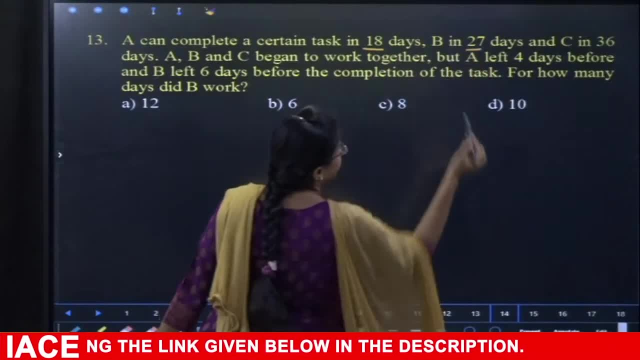 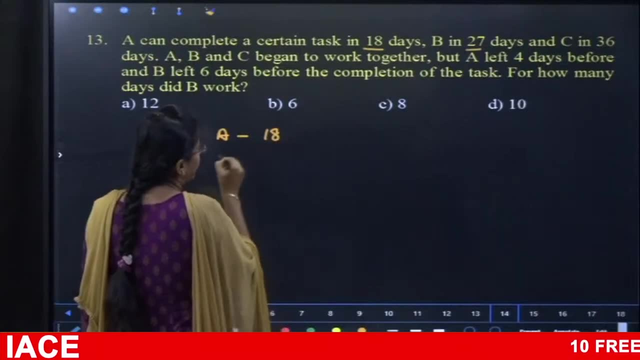 So A can complete a task in how many days? 18.. B in 27 days and C in 36 days, itchinadu. So, number of days given itchasadu gabutti, A is taking how many days, 18.. 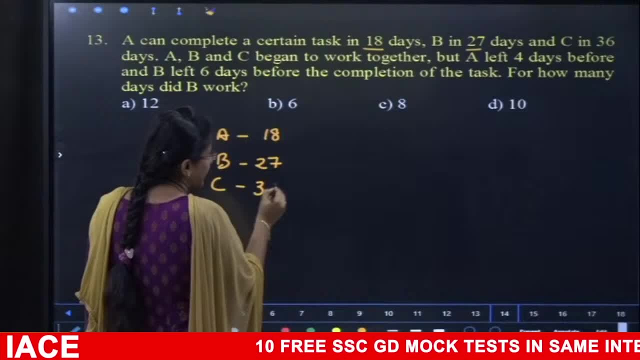 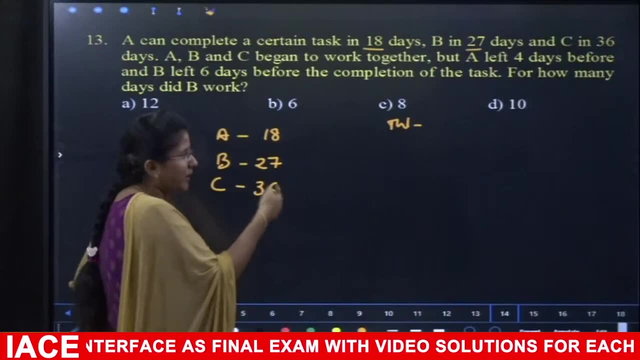 B 27.. C can complete the same task in 36 days. Here LCM method use chestamani total workni 18 ki 27 ki 36.. KLCM cheskuntavumma 18,, 27,, 36.. 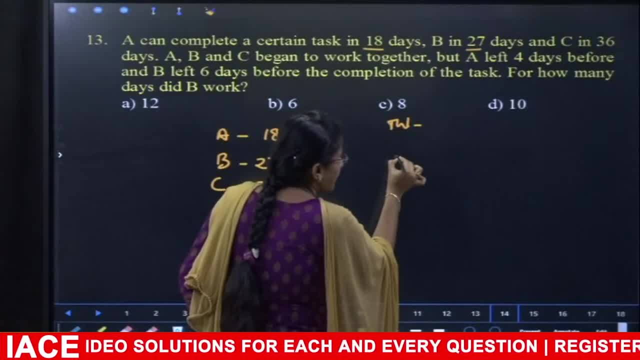 KLCM cheskuntavumma 3 ki otchi 2 ki otchi. 2 ki otchi 2 ki otchi. Common number LCM avaronti 108.. 108 units mani teisikuntatla itte. 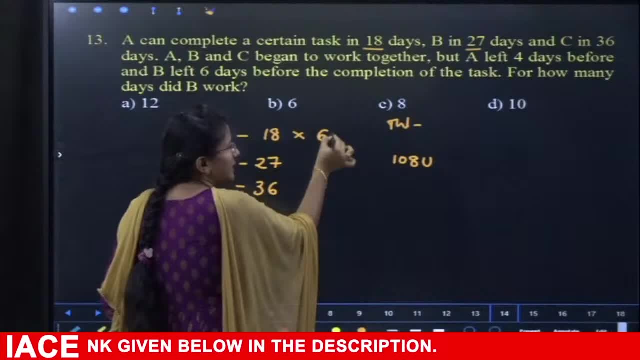 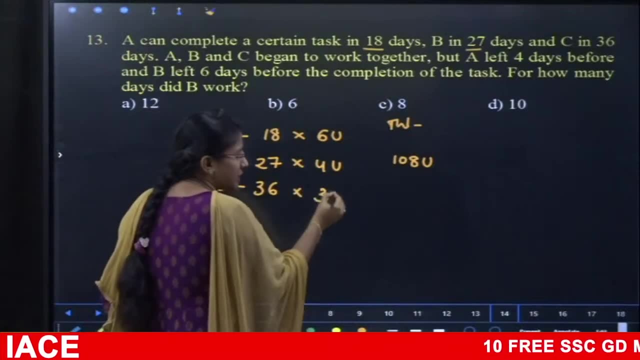 18,. A will do 1 day ki eni units cheskuntandi 6. Adhe B will do 1 day ki 4.. C will do 108,. 36 will be how many units? – 3 units. 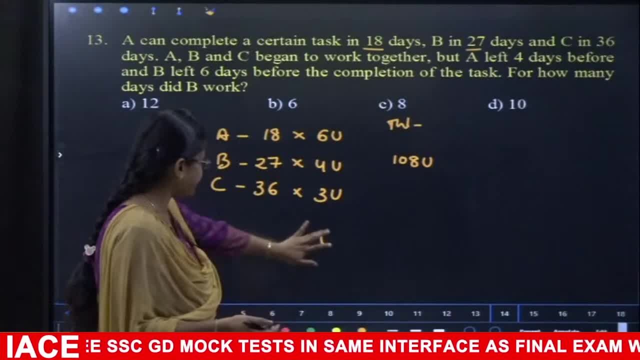 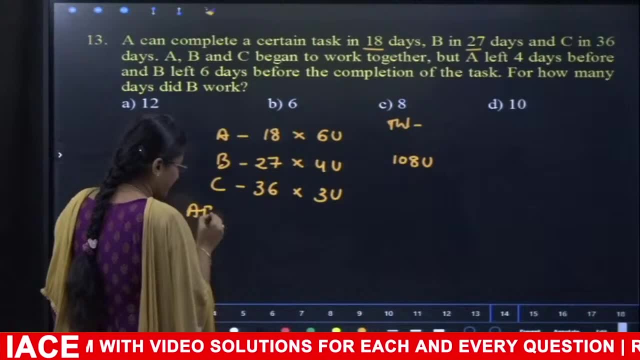 First LCM teskuntavumu efficiencies. fill up chesese sin tharavatha itpuda question. model chetitavumma See question itchininti inti ABC began the work 12. So the group started working. 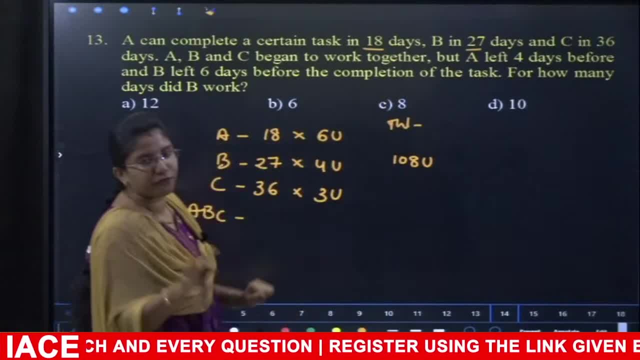 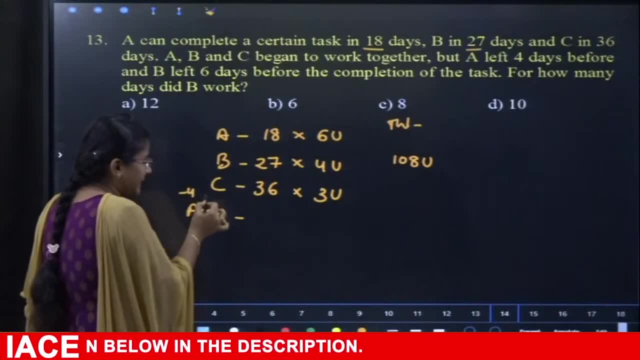 So the people who left the group were: A left 4 days before and B left 6 days before When the work was about to be completed. if A left 4 days before, B left 6 days before, So 4 days before and 6 days before. 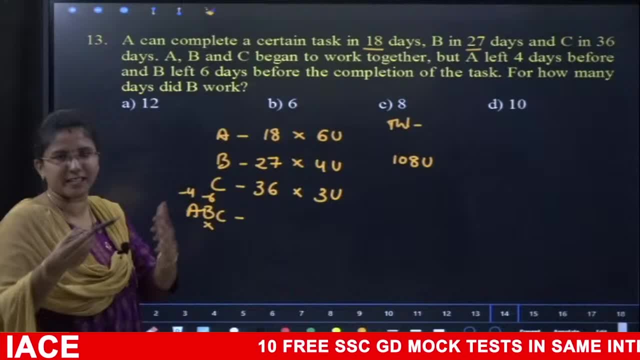 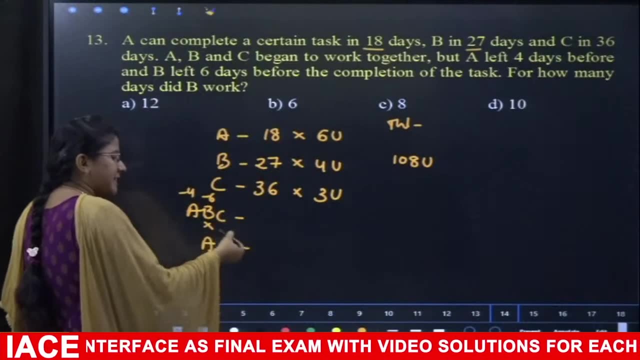 The first person who left from A to B was B. This is the person who left 6 days before, So B left. So who were the remaining people? A and C. So A and C stayed until A completed the work. 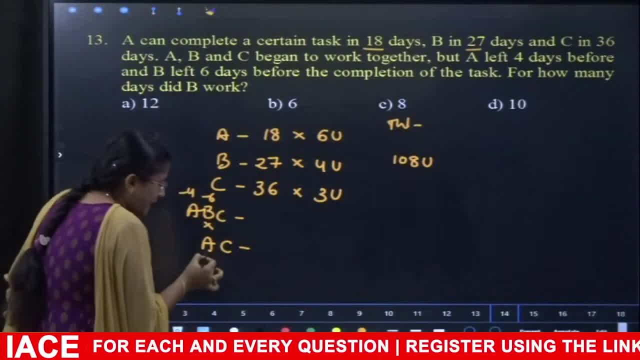 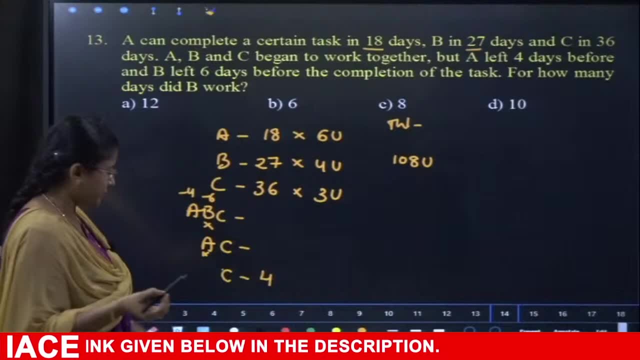 No, How many days before? A left 4 days. So the next person who left from this group was A. So A left 4 days before. So that particular 4 days C worked alone. B left 6 days. 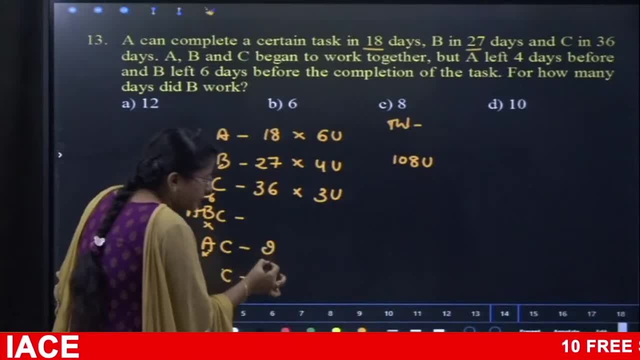 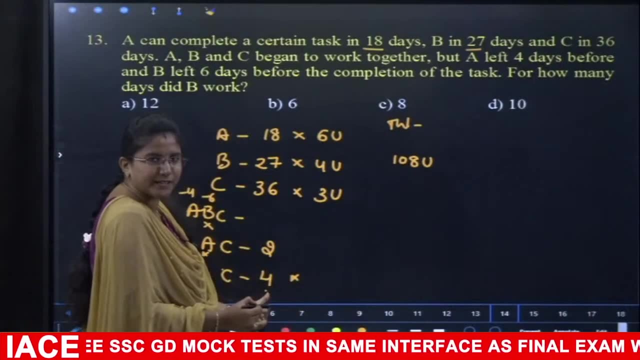 Here already 4 days are there. 6 days means A and C worked for remaining 2.. 4 plus 2 is 6.. So here the problem is filling up the efficiencies. C worked single for 4 days, 4 days efficiency 3.. 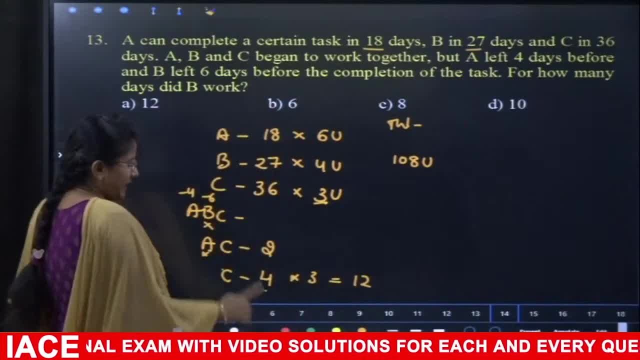 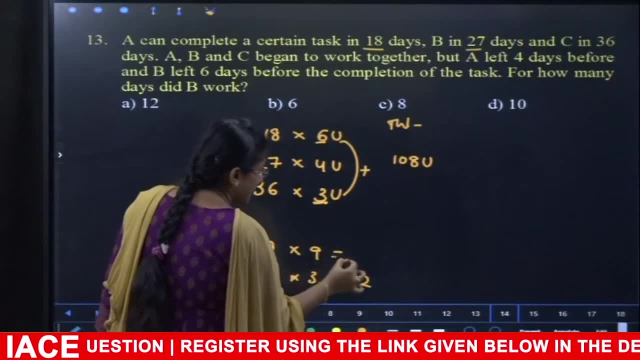 4 and 3, how many units? How many units will be completed? 12. Next, what if both of them work? A6, C3.. If 2 are combined, 6 plus 3? 9. Since they worked for 2 days, how much is 2 and 9?? 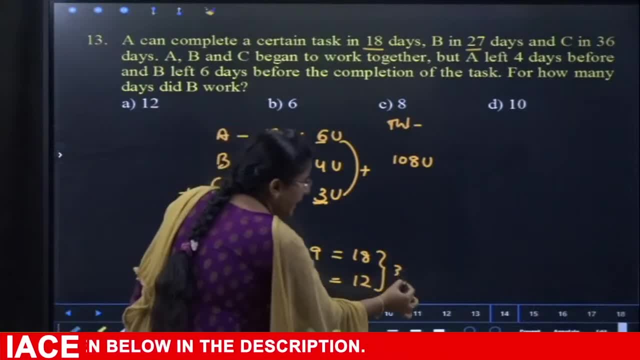 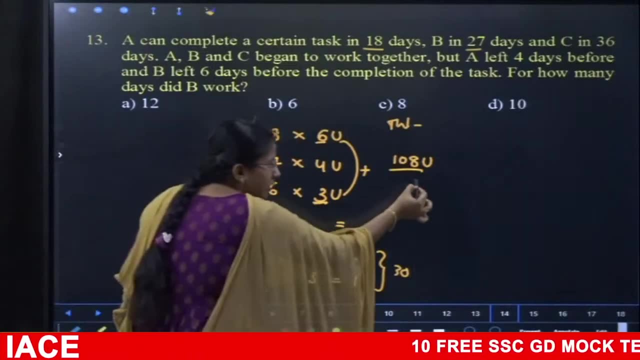 18.. So here, 18 plus 12.. Total work completed is 30 out of 108.. If 30 work is done in 108, how much is the work done by 3 people? 108 minus 30,, that is how much. 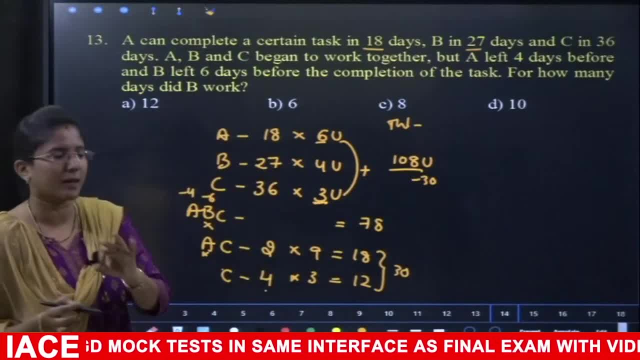 78. That means these 78 units were completed as a group by 3 people, So they are doing 78. If 3 people work together, the work will be completed For 1 day. 6 plus 4 is 10.. 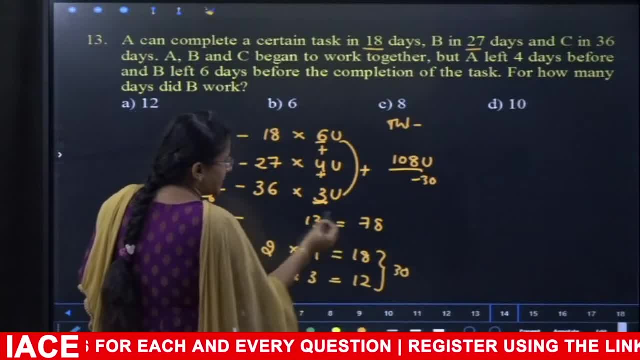 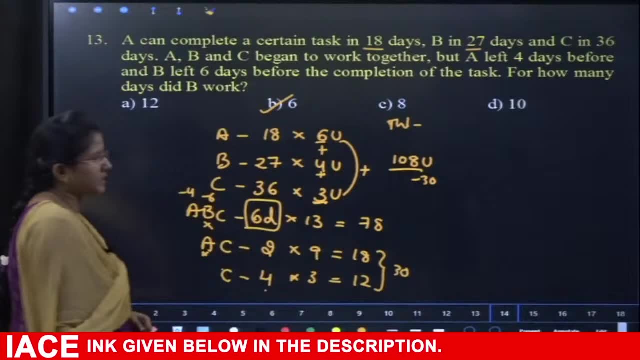 10 plus 3 is 13.. Since you completed 78, how many days do you have to work? So the answer is clearly 6 days. Option B: So, in LCM method, just pick a number and fill up these numbers. 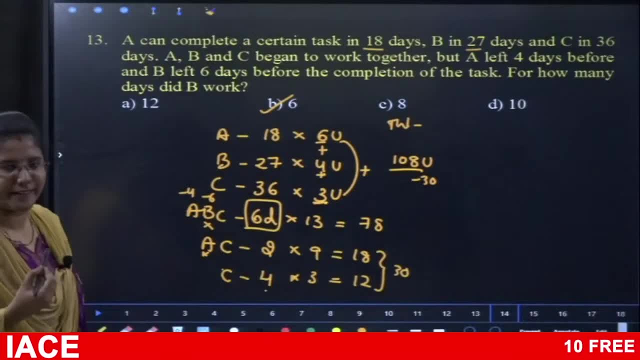 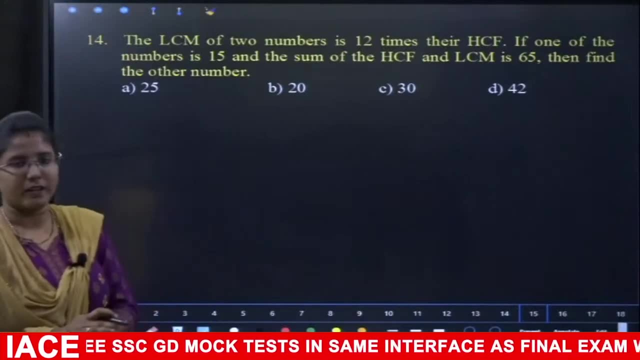 It is an easy equation, You can solve it very easily. Okay, Understand all of you. Next, Let's go for next one. 14th equation: Try it Display the timer please. Okay, This was the timer. This was the timer please. 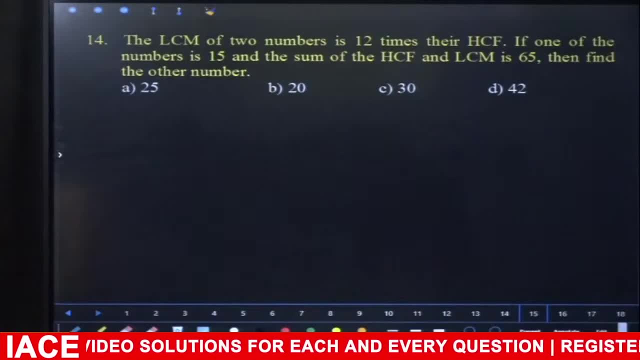 Easiest equation: 30 seconds Enough, 30 seconds timer. Try it Okay, You can try it Okay. Please try it Okay. Try it Okay, You can try it, Please try it, Try it Okay. 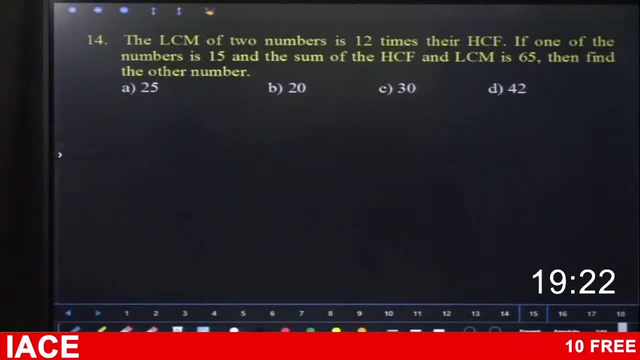 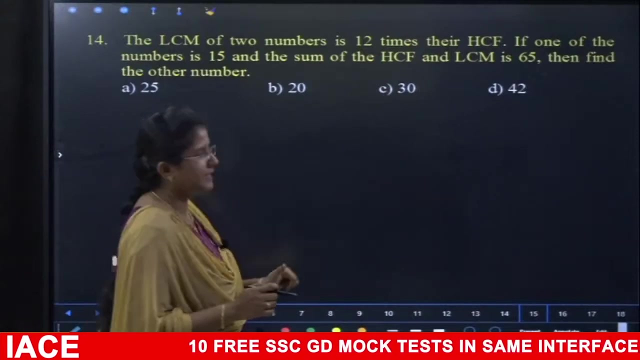 You can try it. Okay, Please try it. Try it. Okay, Your time is up. LCM- HCF topic is very easy question: See First sentence. to them, LCM of 2 number C is 12 times their HCF. If one of the number C is 15 and sum of LCM, HCF is 65.. LCM of 2 number C is 12. 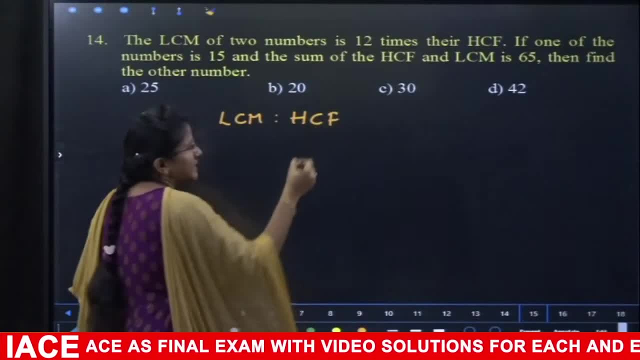 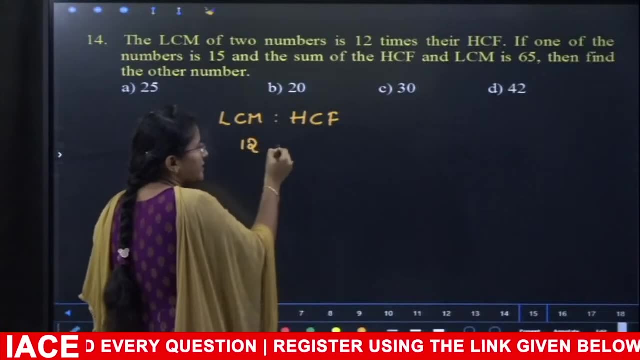 times their HCF. From that sentence we can write LCM, HCF ratio: How many times HCF has LCM. 12 times 12 times means ratio will be 2 is to 1.. We write double is 2 is to 1, triple. 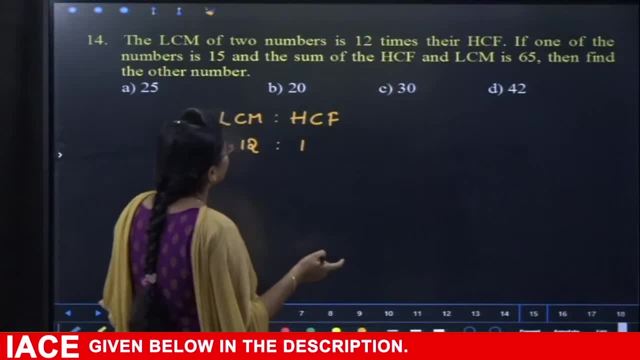 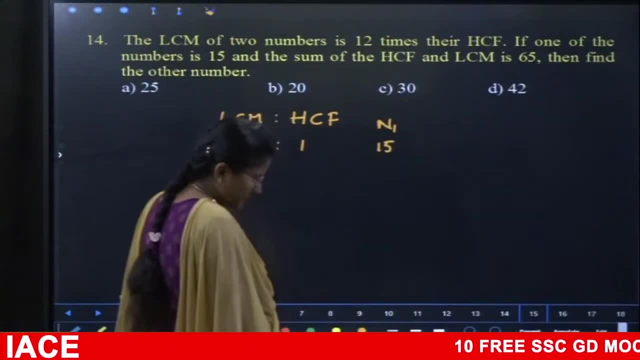 is 3 is to 1.. So 12 times is 12 is to 1.. Next, one of the number is given, Two numbers. so one number is given to us. How much is it 15.. Sum of LCM: HCF is given How much. 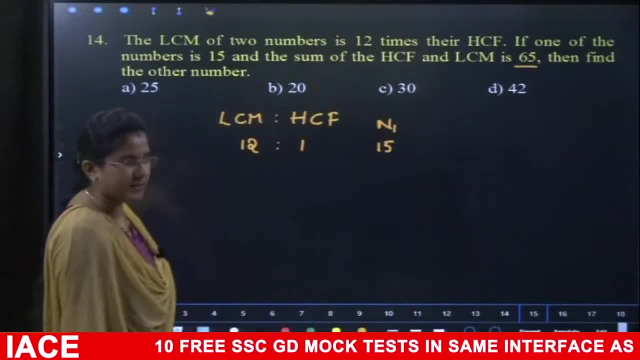 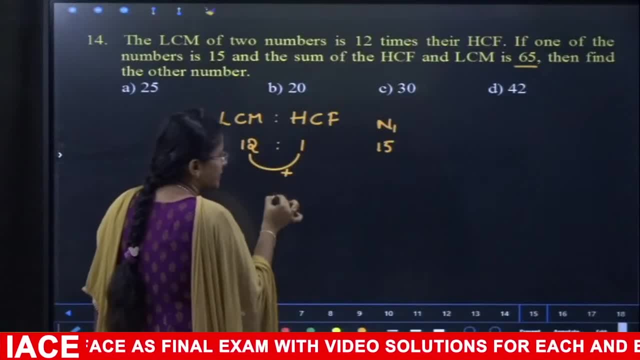 HCF is given, So LCM HCF is given, So LCM is given, So LCM HCF is given. Now, how many are cleft? and then some are kept, and again the number is given, So 13 times 2 is to. 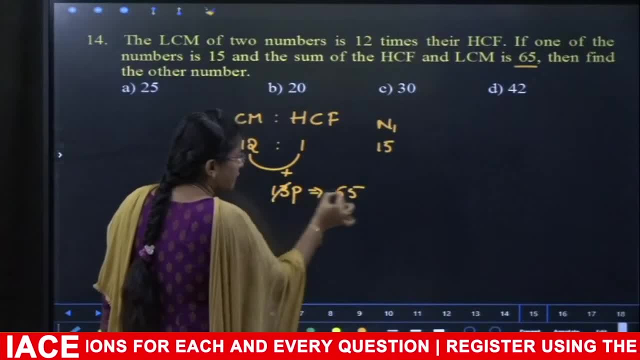 5. We will add 12 plus 4 times 9 plus 3 times 8 times 5, and here blue is the number above it. so 11 equals 5 centimeters to 1.. Next, 5 is higher than 5. That is equal to 5 centimeters. 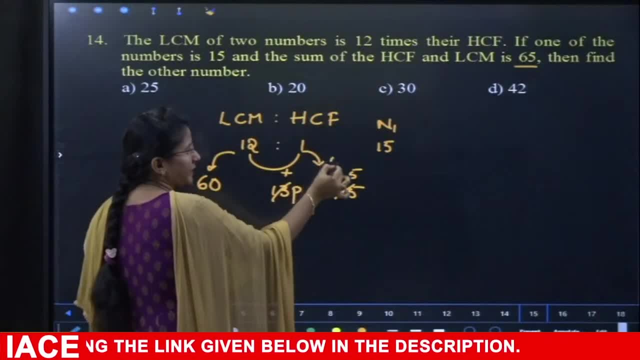 higher than 9 days, 15 times Now. once again we will show how many are given. So let not forget that 3 a did Now first we will add that 5 is higher than 5 so that it becomes 3. we have to do the subtraction Now. we will do a little for an example. so if you want, 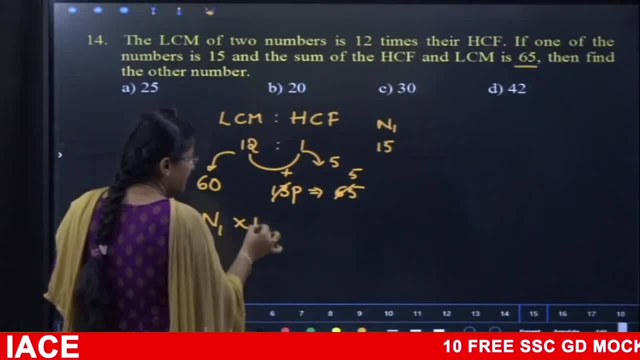 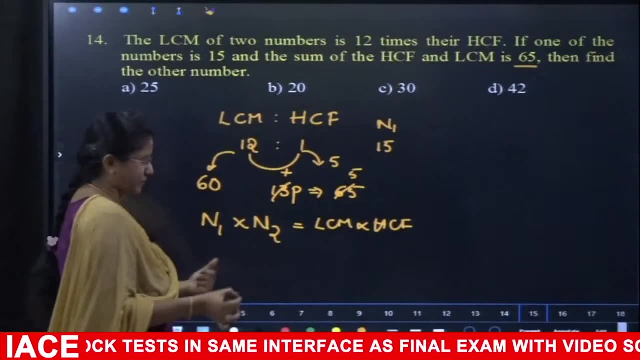 to with a bar number and a number. we can add the number we walked up because okay, in analog N1 into N2, equal to LCM into HCF. So simply, we will substitute that We will find out another number, N1, given 15.. 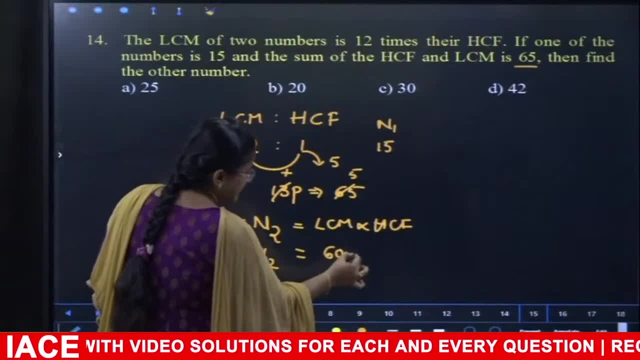 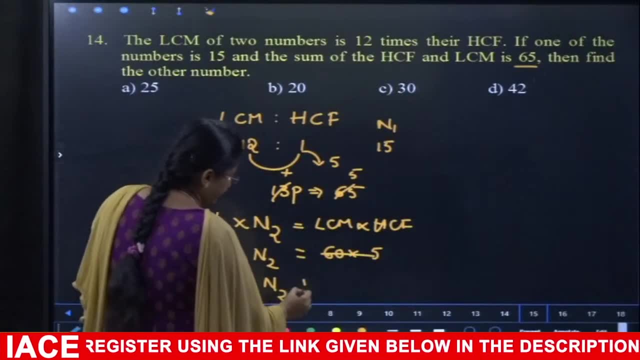 N2, we should find it out. LCM: we got 60.. HCF: we got 5.. So here that will be answer. N2 is 20.. So N number will be 20.. Option D: Okay, Next. 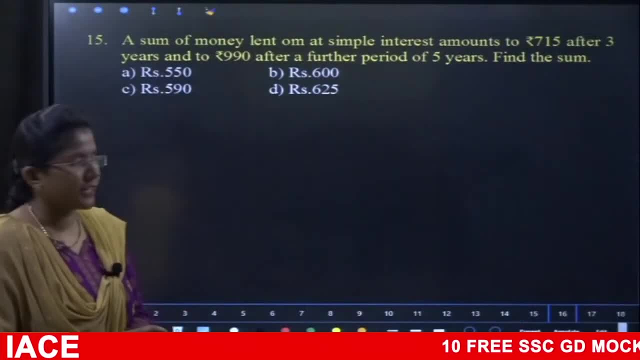 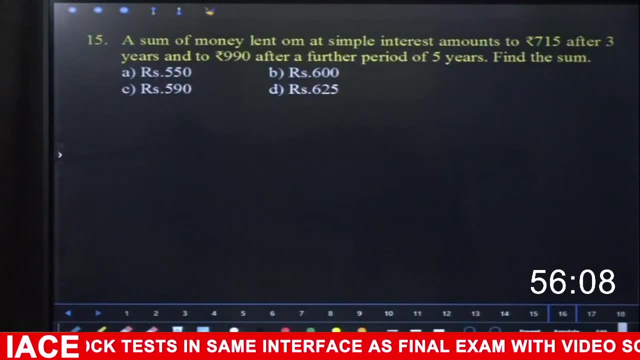 Let us go for next one, 15.. So try the equation: One minute timer. Display the timer, please. Did you get the answer? Nada Theان görün Thin, Thin, Thin, Thin, Thin Thin. 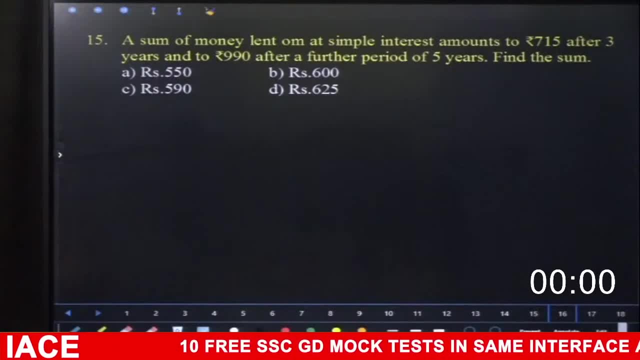 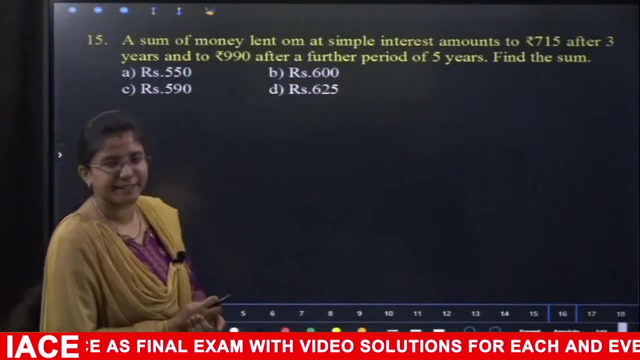 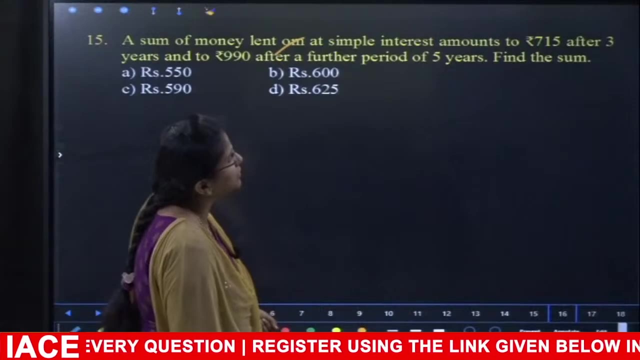 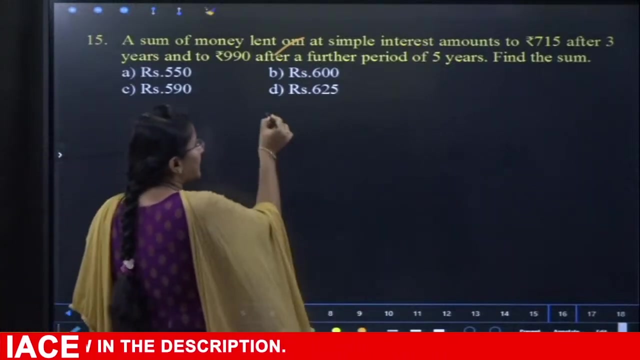 okay, your time is up. so here the question given from simple interest topic, easiest question, and see, try to them. a sum of money lent at simple interest amounts to 715 after three years and 990 after further period of five years. find this sum sum on the principle and the principle in the 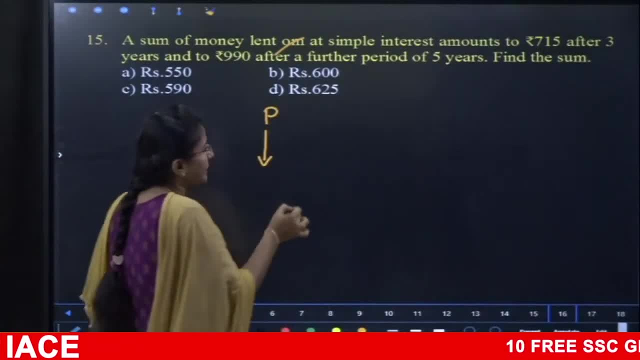 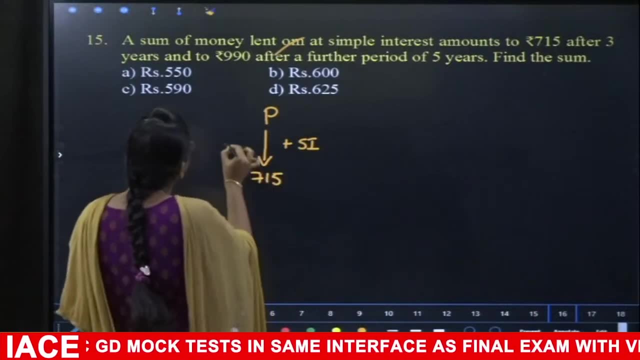 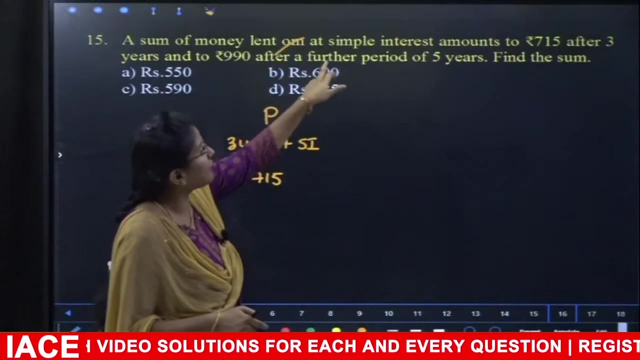 it amounts to, and the principle plus interest: Calipi, total amount, each other amount and each other and a 715. in how many years? a period of three years, three years, low, 750, 90 are they principally 990 in the in the amount of 990 after further five years. after five years, only the after. 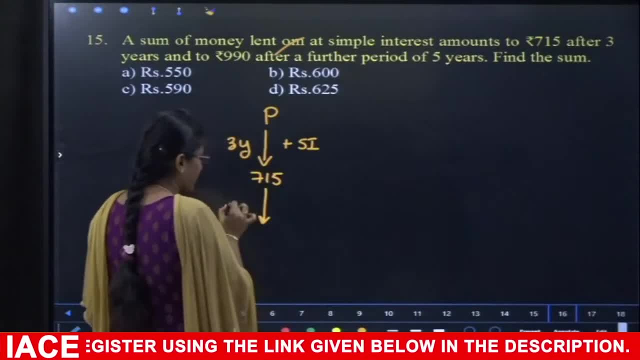 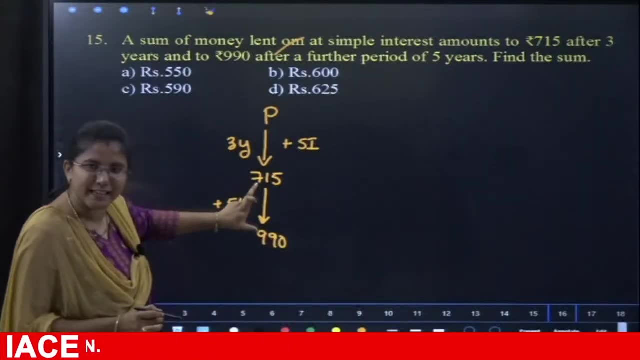 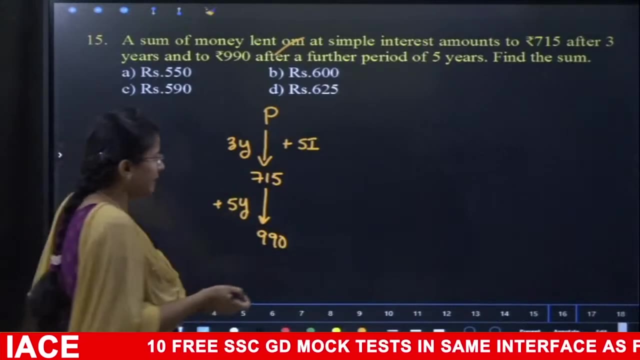 further five years and the economy, she in Coco, five years in Coco, five years, third of our teaching amount and the chant, and nine hundred and ninety and the easy second sentence into clear. that else both in the seven, fifteen, nine, ninety, and then the interest, find that part of the, in the simple interest, five years, part of the difference is going to. 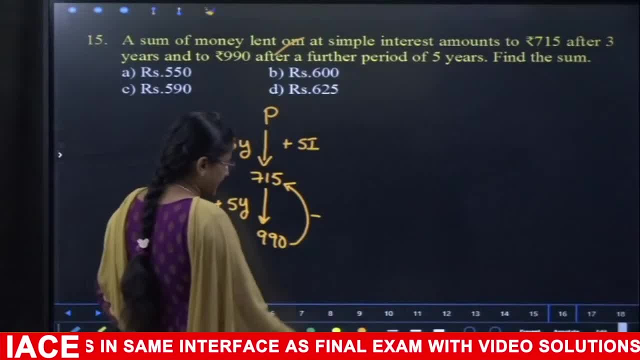 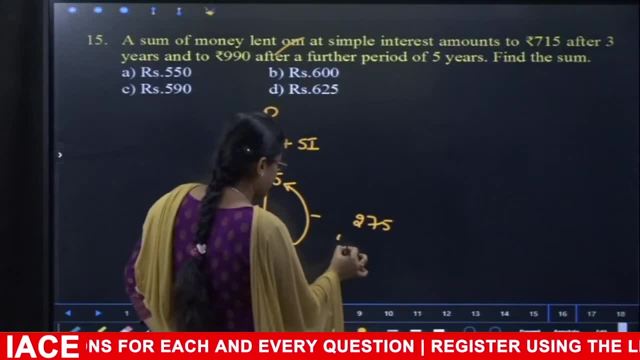 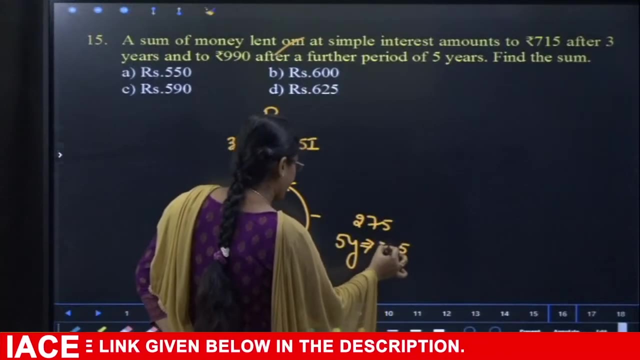 support them. so difference is nine ninety minus seven hundred and fifty, that is 75, it is two to 75, so five years to key interest will be five. it is eight, one, seven, two, two, seventy five, so five years, k 275 and that then one year key, the interest will be. 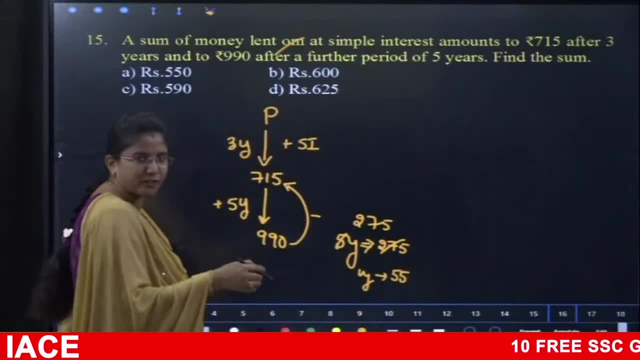 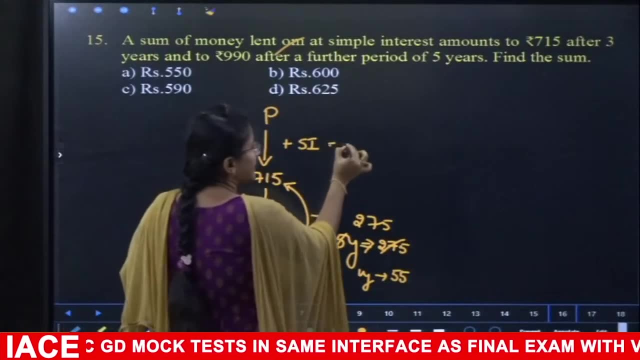 fifty-five. so one year, coach is simple, interest fifty-five. so every year, and they want to the cavity could find out J system. one year, key fifty-five with a three years can't interest for, don't Dali? so answer is: one year, fifty-five, Allah, three years, cover to fifty-five trees in. 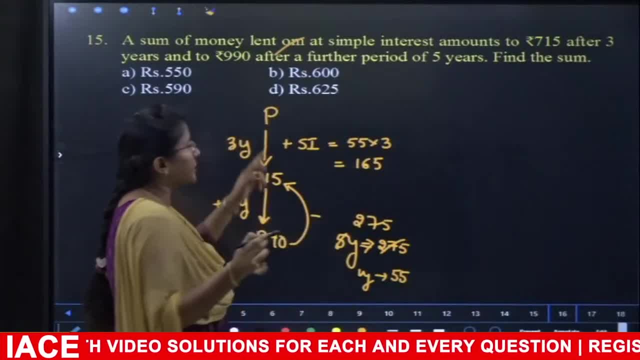 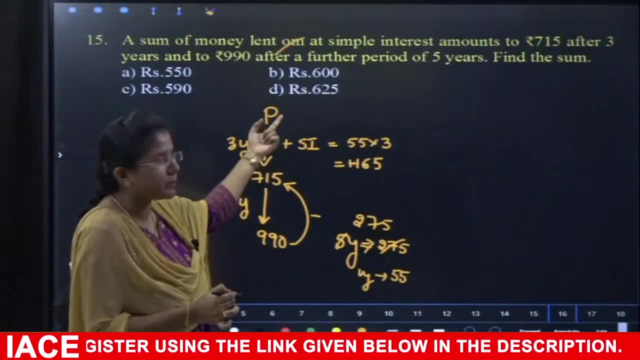 candy, yes, one sixty-five. and take a principle either only the principle made a one sixty-five interest to put in the amount of Cindy seven fifteen. so answer will be: and then I do not principle, and then I do not know. so my name back a lot of a party. they seven fifty loon she amount. 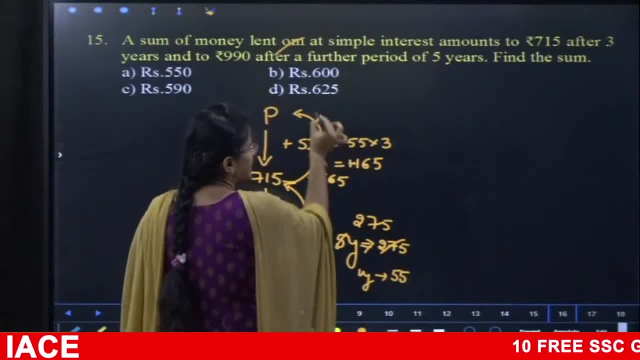 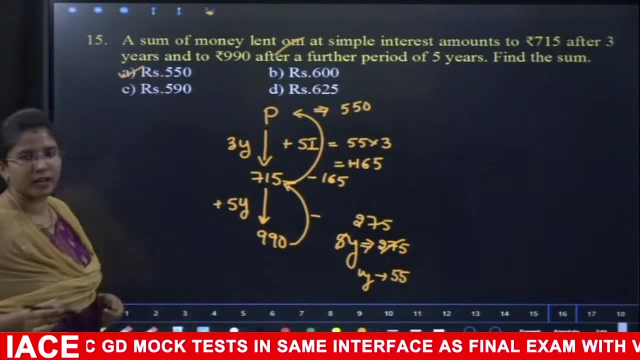 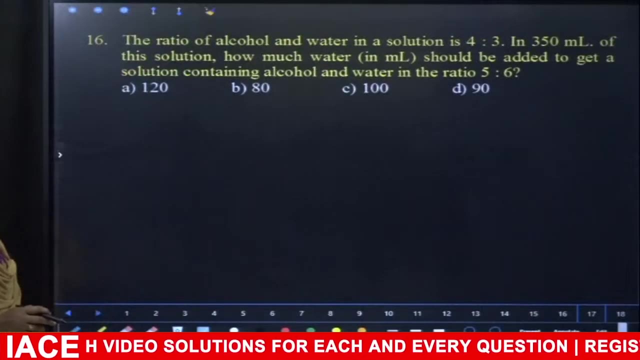 minus six is seven, fifty minus one, sixty-five. so principle is five hundred and fifty. five hundred and fifty, it is options eight. okay, understand all of you. very easy question and the simple interest account easy. I plus all just say it's one mixed. go for next equation 16. so it is from ratios. 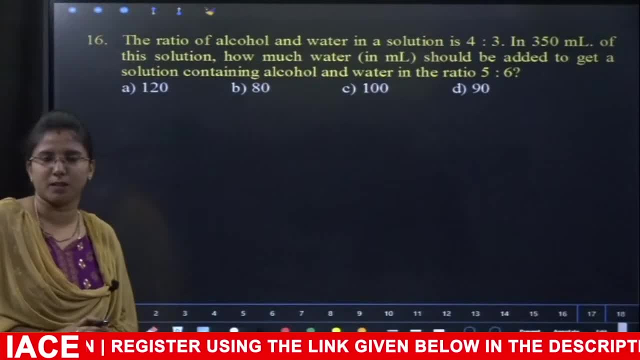 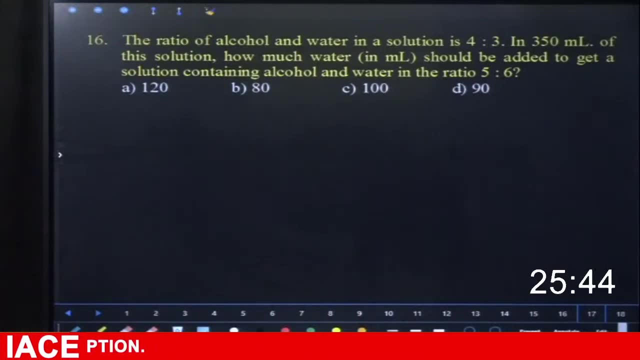 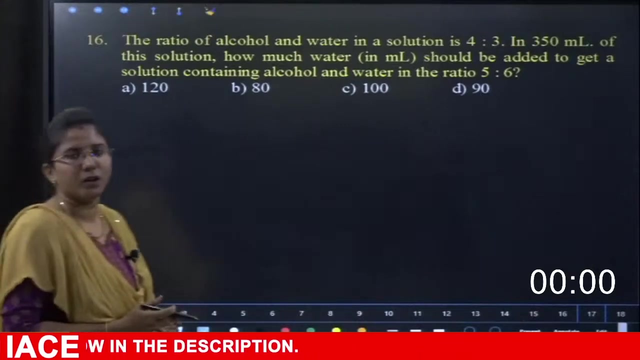 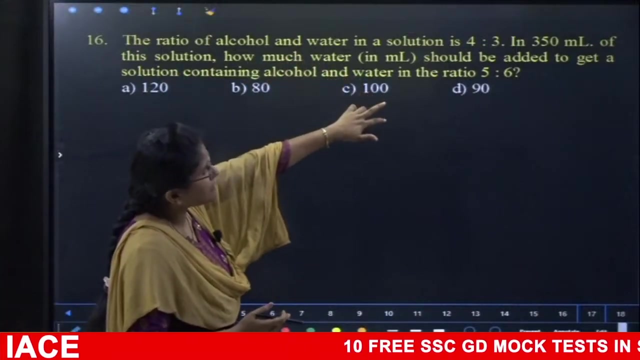 topic: easy question and D, so 30 seconds timer. these fundamental easy gas all change to display the timer, please. okay, your time is up, so equation J them very easy. ratio of alcohol to water in a solution is four is to three. in 350 ml of the solution, how much water should be added to get the solution containing alcohol to? 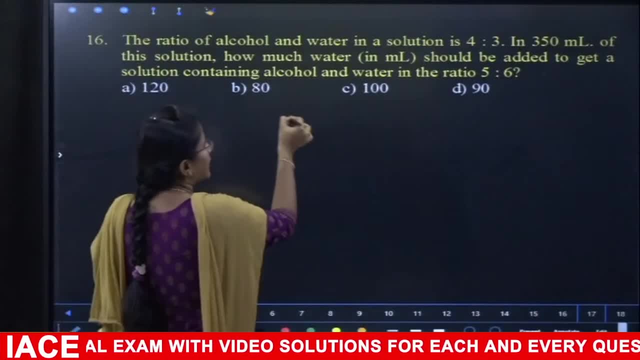 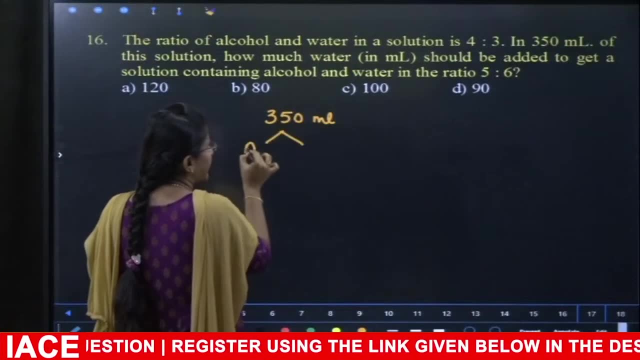 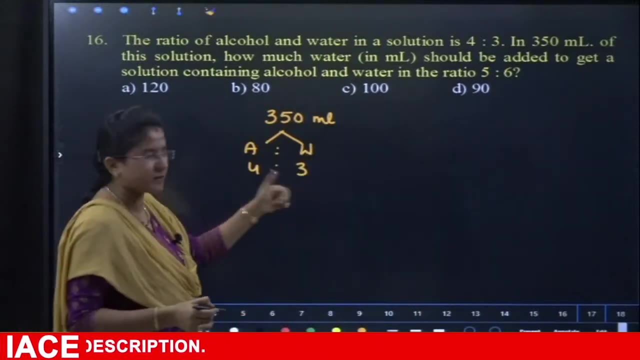 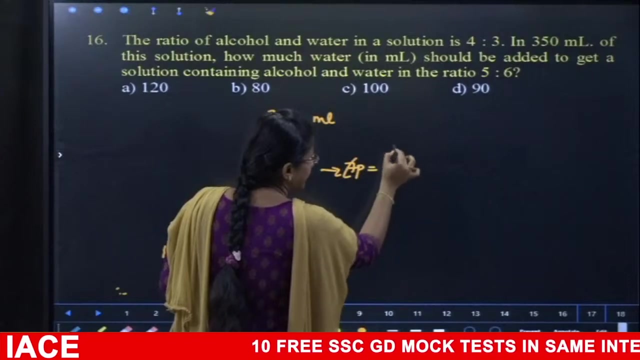 water in the ratio five is to six. alcohol water: kitchen ratio four is to three. so 350 ml of the solution. low ratio of alcohol to water each other and the alcohol four parts water, three parts. so ratio is four is to three. four parts, three parts total, how many parts? seven parts, seven parts equal to 350, I think. what is the value of one part? it is. 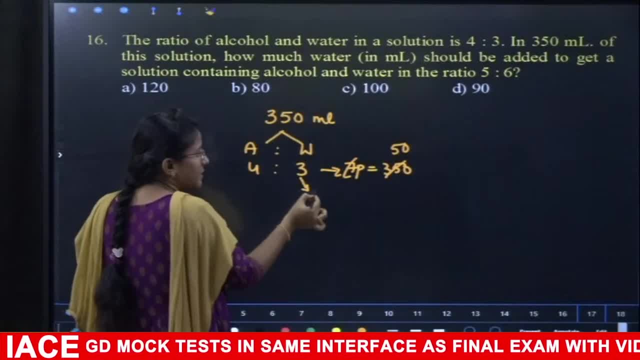 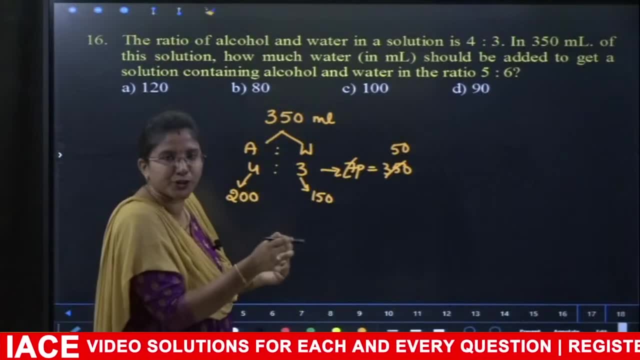 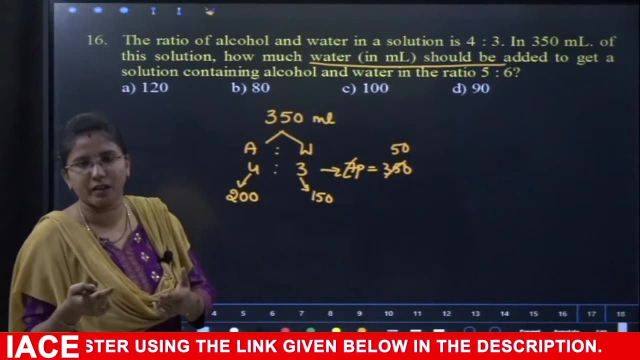 fifty, one part, fifty go. but the water present in the solution is 150 and alcohol present in the solution is 200. so 200, 150 classification, a solution, low key question I do to me how much water should be added? water master match a mountain or alcohol match a minute, little piece a minute. 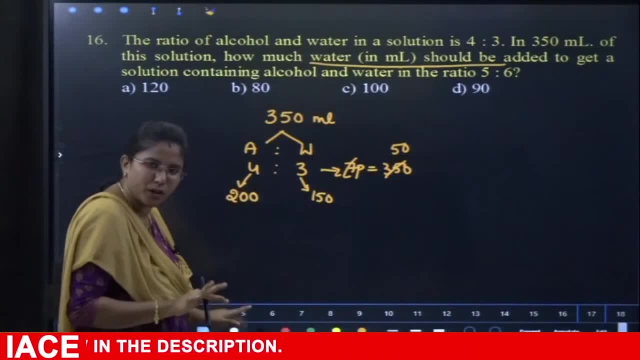 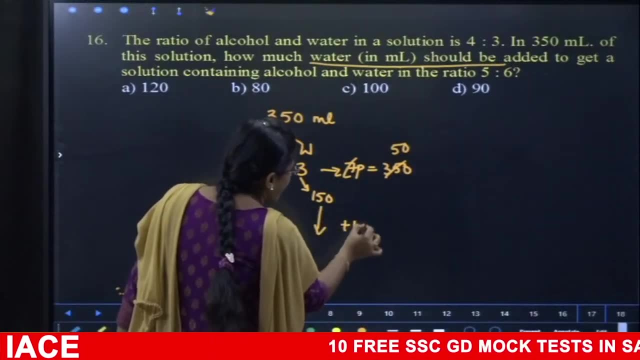 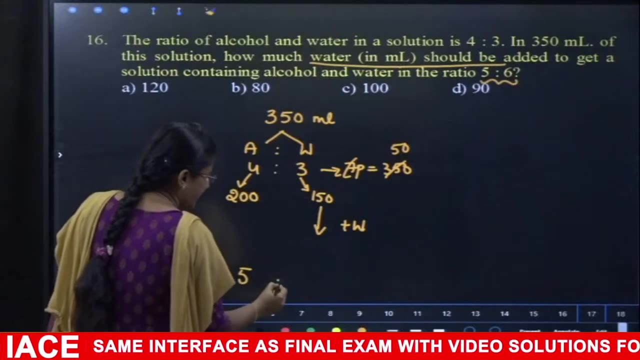 little Santa alcoholic. a 200 on. take five, hello Coda two hundred. I went to the point so I pay in the water. at chile, la una Dini key, I pay. ratio of alcohol to water should be come along darling. five is to six. so alcohol to water ratio should be five is to six, out of the way. so 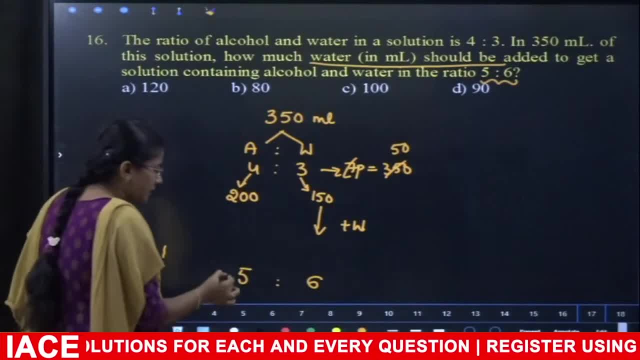 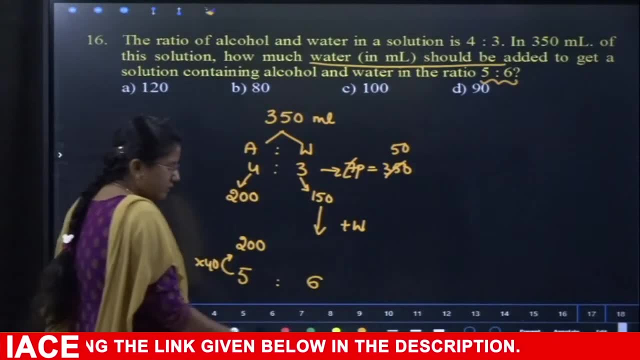 water matter matches, not about the alcohol stays constant. so many five parts value 200 inches them. so five parts 200, I do. what is the value of one part 40? so six forties will be in the middle and you grow six into forty. eight is a two forty. 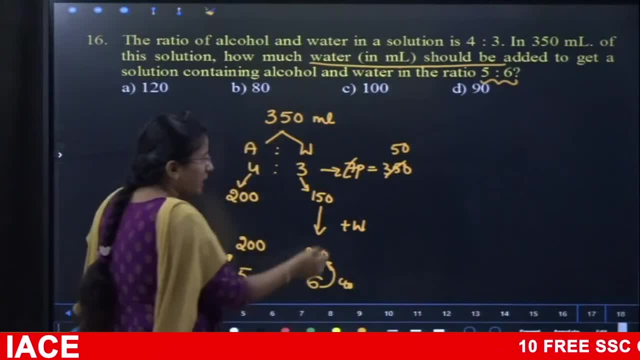 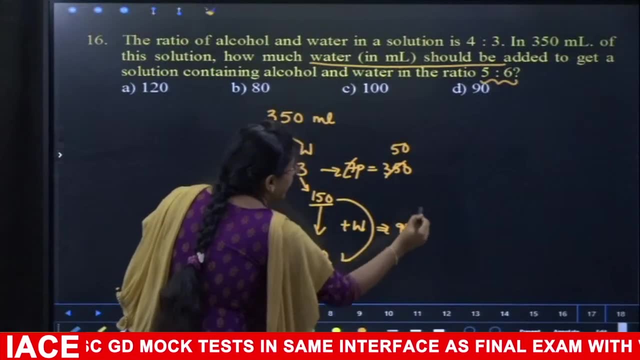 so water should be two, forty and any ratio it loves me, one, fifty, one dozen water to forty and then take some addition journey and then that is in andy, ninety, ninety, eight or so water should be added. if we add 90 liters of water, then we will get ratio five is to six. that simple as. 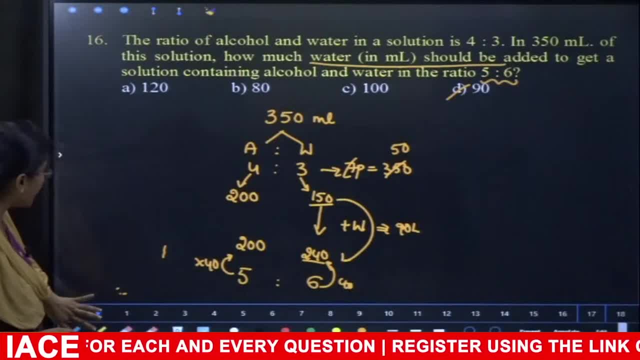 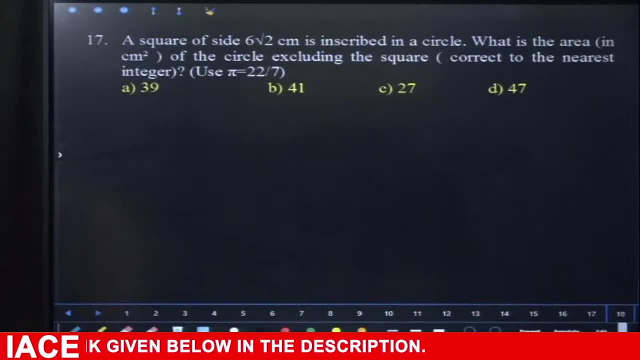 that my next equation to them, question number 17. try chain and equation or display the timer. please take a minute. I don't know what the answer is, but the answer is I am going to go ahead and do it. I am going to go ahead and do it and take a minute to give it a second look here. 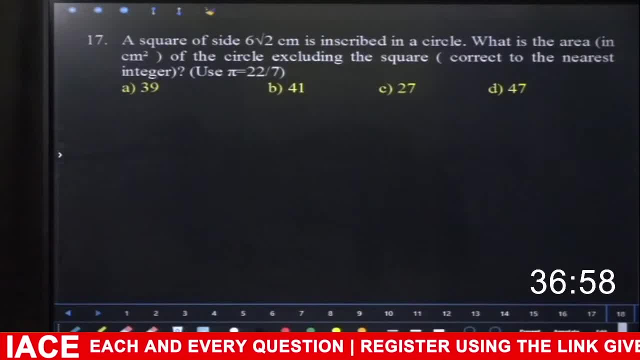 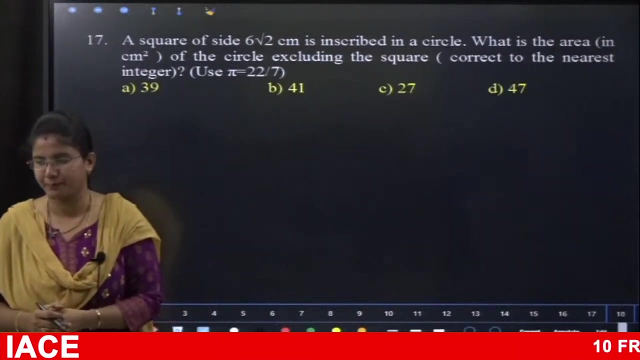 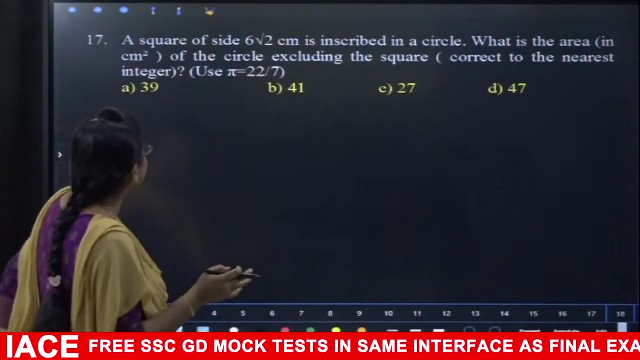 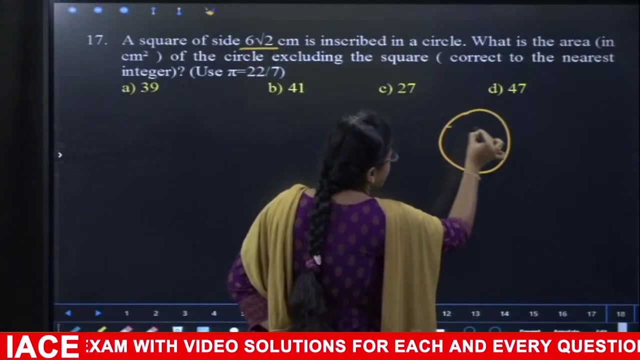 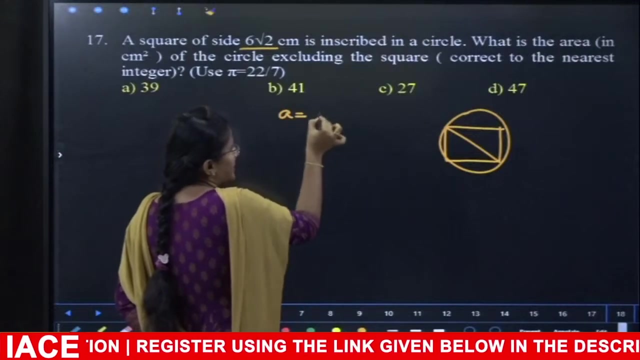 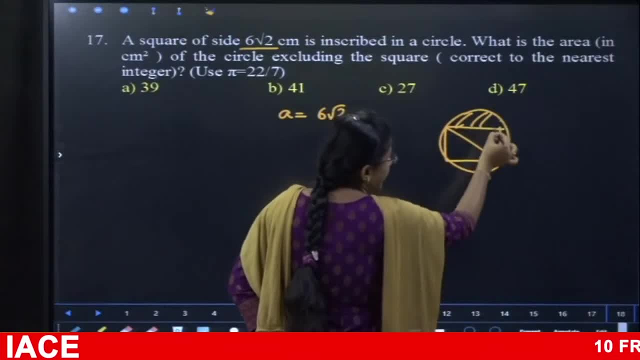 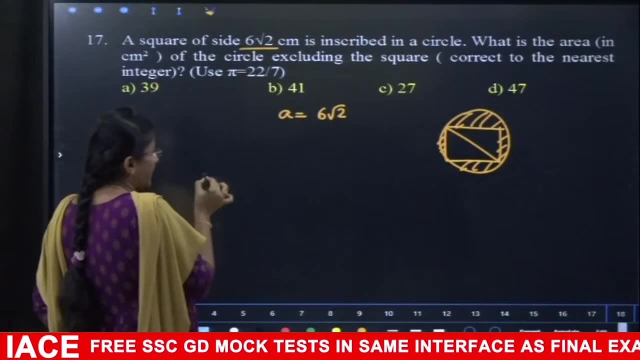 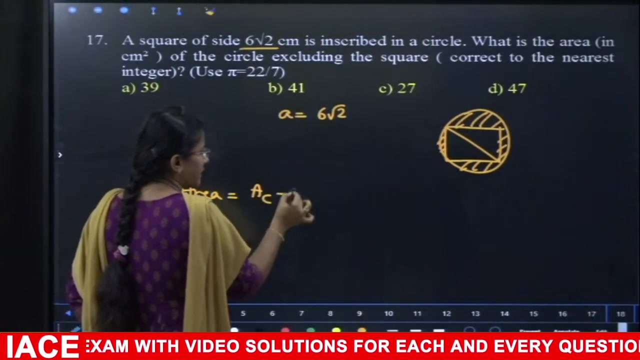 We are asking a question. We have to find out the circle area and exclude that square. That is this portion. We have to find out the area for this portion. So finding out the area of that portion is nothing but area of that region equal to total circle area. From that we will deduct the square area. That is all We know how to find out the square area and circle area. What is the difference? 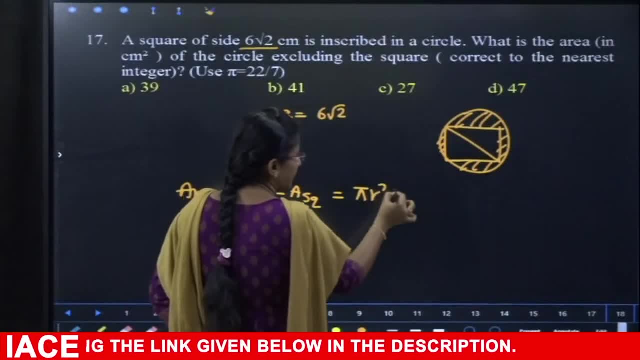 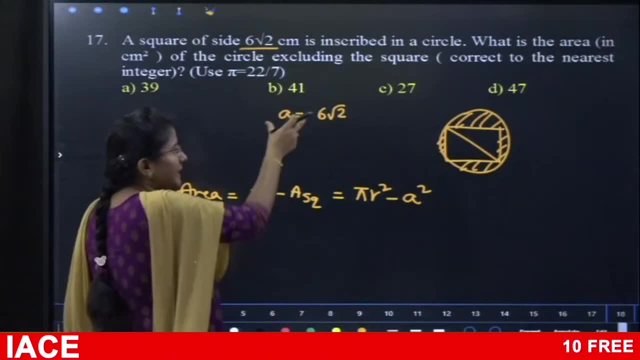 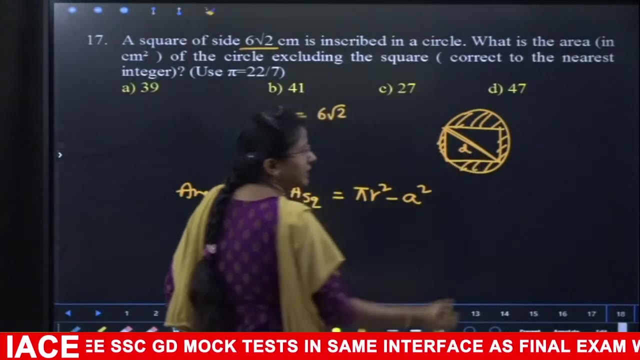 Circle area will be. that is pi r square minus square area will be a square. We know the side. We know pi r square And radius of the circle. we have to find out We will use the side for that. So when we take a square and inscribe it in a circle, that square diagonal will be there. That diagonal will be diameter of the circle. 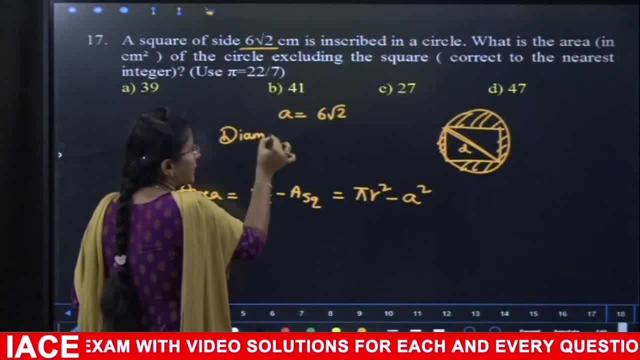 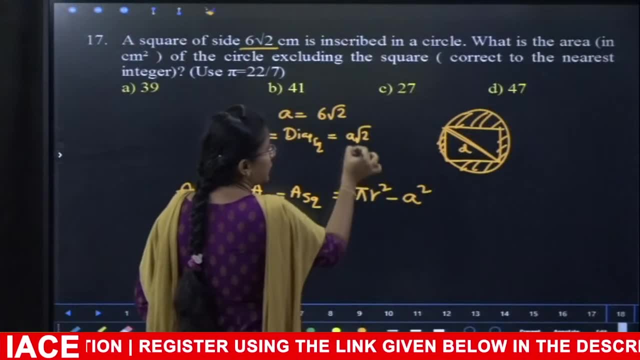 So diameter of the circle will be equal to diagonal of square. So we know the formula of square diagonal. What is that? Yes, a root 2.. So a is already given 6 root 2 into root 2.. That is. 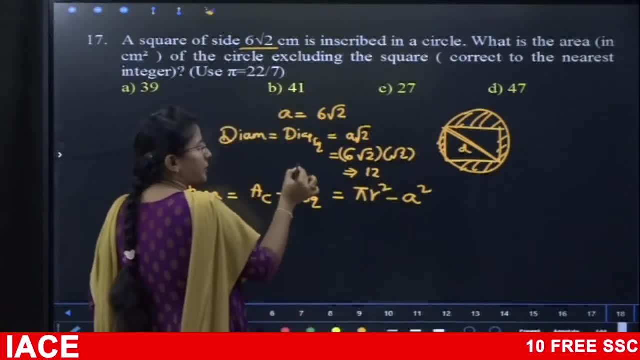 6 root 2 is 12.. When diameter is 12, diameter means 2 times of radius. When 2 times of radius is 12, radius will be how much It will be 6.. We will use that 6 here. 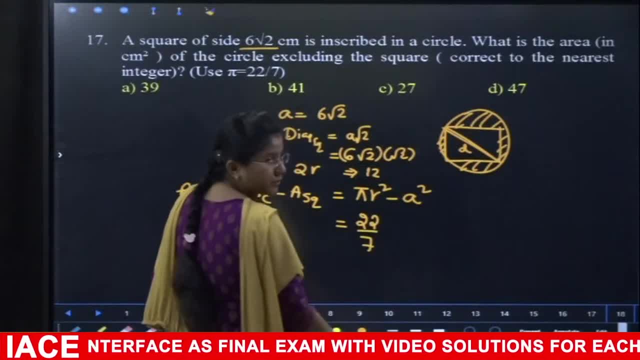 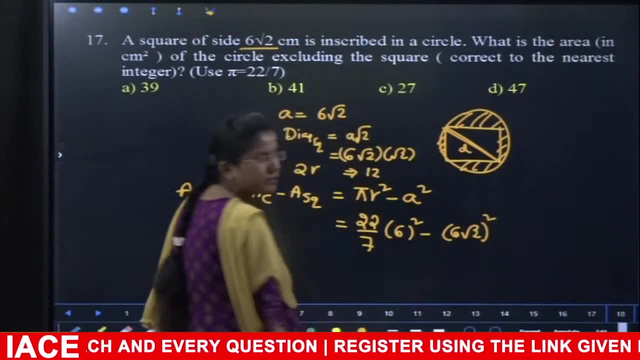 So pi will be what Use 22 by 7.. We will use that Into 6 square minus. a square is already given. How much is it? 6 root 2 whole square. So that is normally we have to solve. 6 square will be 36.. 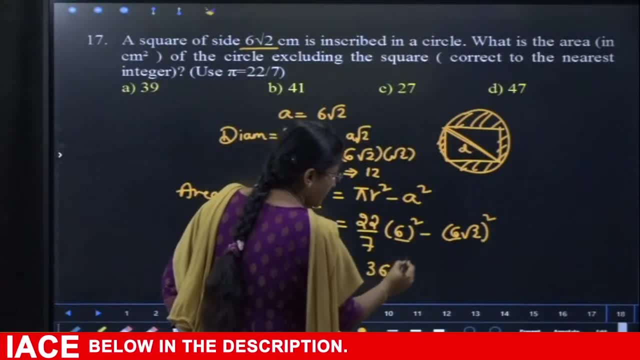 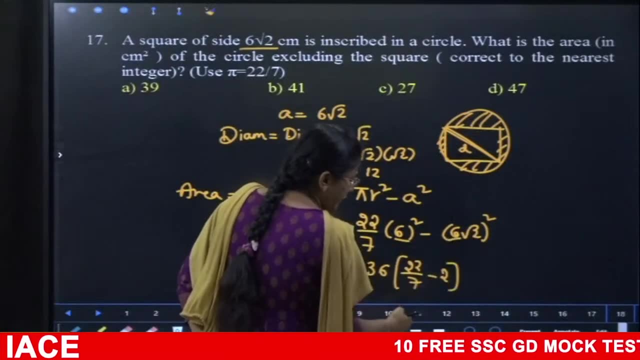 36 will come in this and 36 will come in this, So 36 we will take as common. 22 by 7 minus root 2 square, That will be 2. 22 by 7. 22 minus 14 will be 8.. 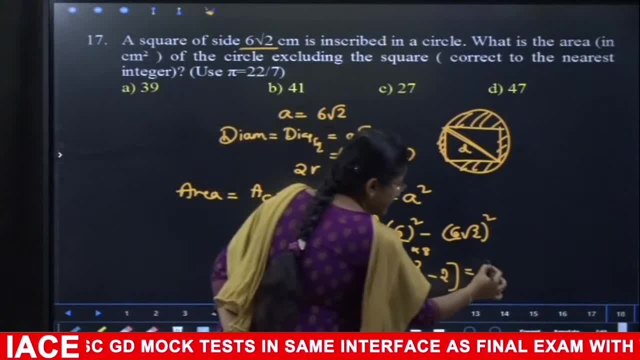 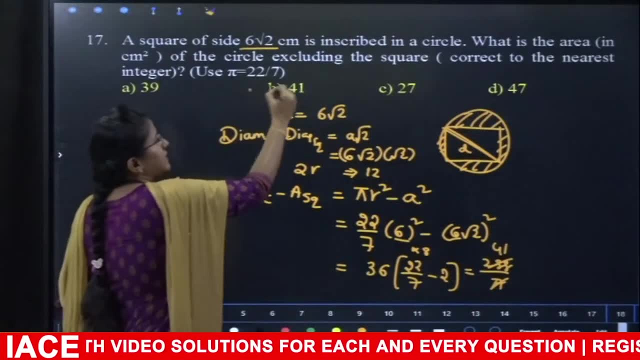 That means 36 into 8 by 7.. 36 8s, that is 288.. 288 by 7 will be 41 times 41. point will be approximately nearest integer is option B41.. Okay, Next, Let us move on to next one. 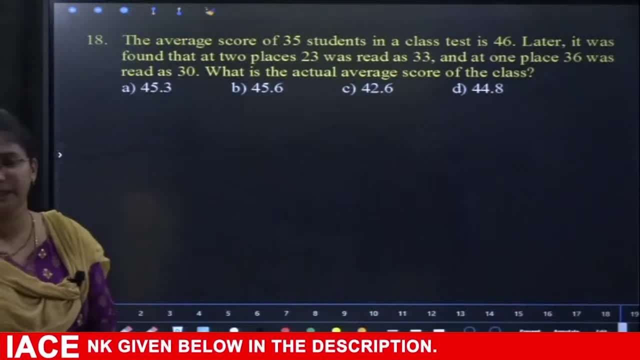 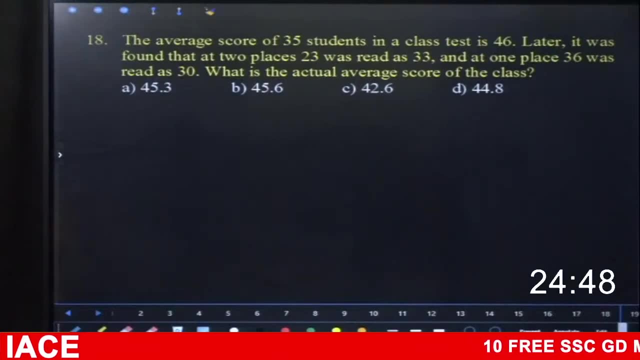 18th average is topic mentioned. Try it 30 seconds time, please. Thank you, We are in moment. Hold for 2 seconds: Okay. 20 seconds. 30 seconds: Okay. 1, 2, 2, 1.. 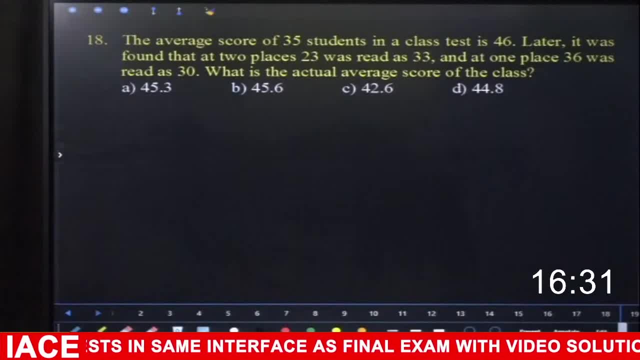 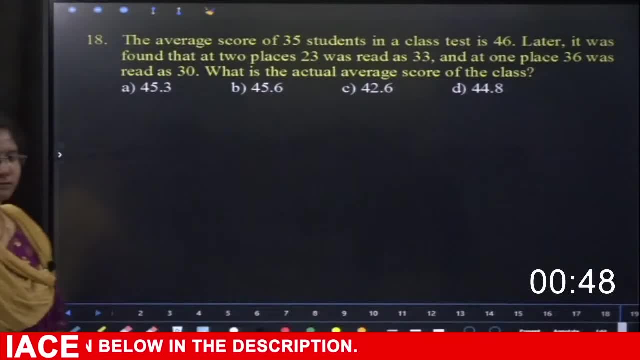 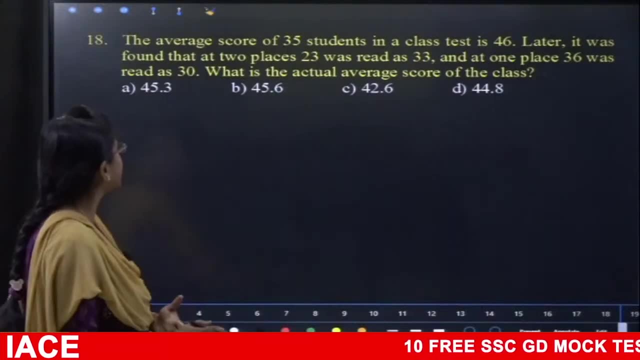 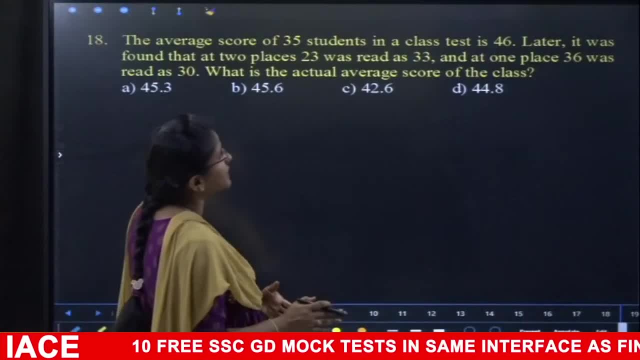 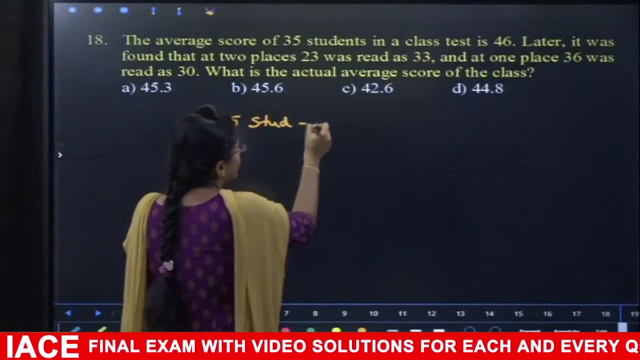 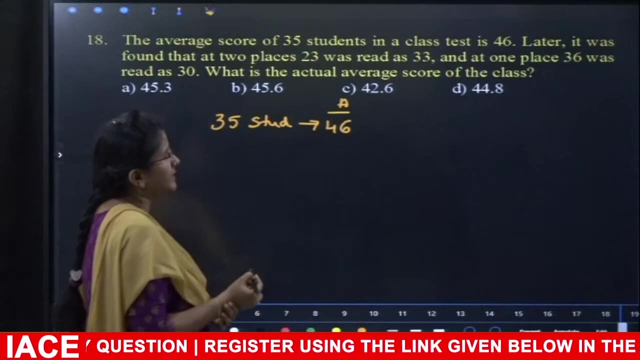 So average score of 35 students in a class test is 46.. In our class there are 35 students. He gave the initial average to 35 students. Average is 46.. Next, later it was found that at two places 23 was read as 33. 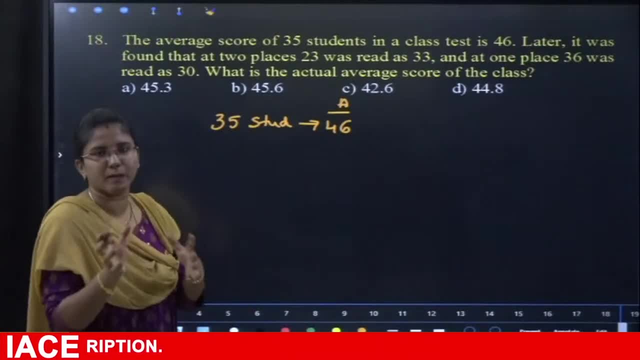 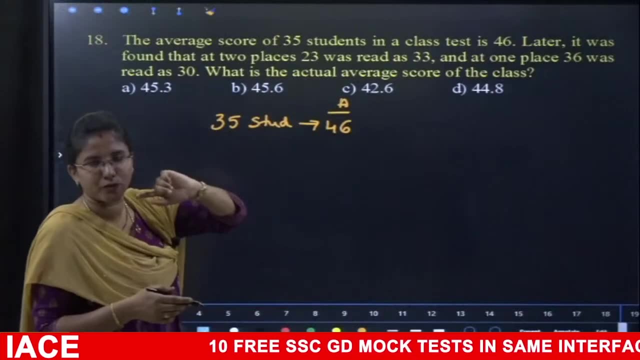 and at one place 36 was read as 30. It means correction. Some will get wrong marks in some places without getting correct marks After correction. the question is: what is the actual average of this class Most frequent question? So let us write the sentence we were given. 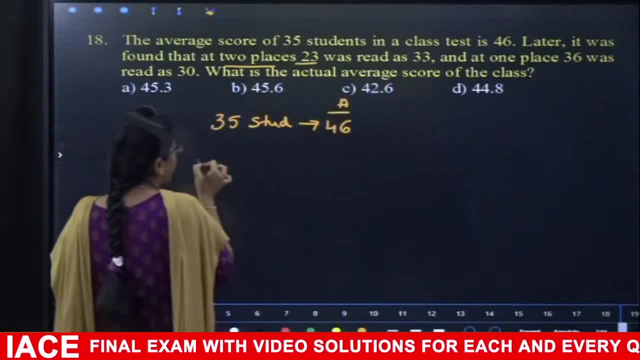 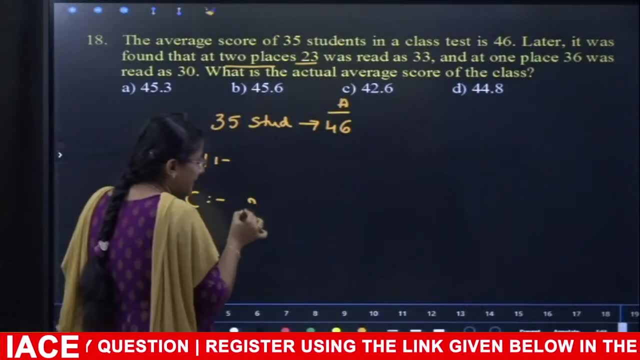 It is found that at two places 23 was read as 33.. So we read 23 as 33.. If we read 23 as 33, it means 23 is correct and 33 is wrong. In how many places did it happen? 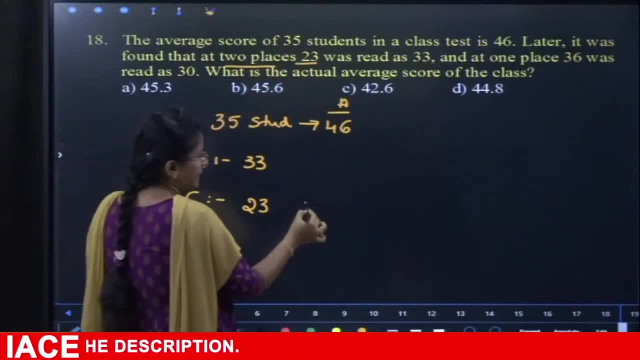 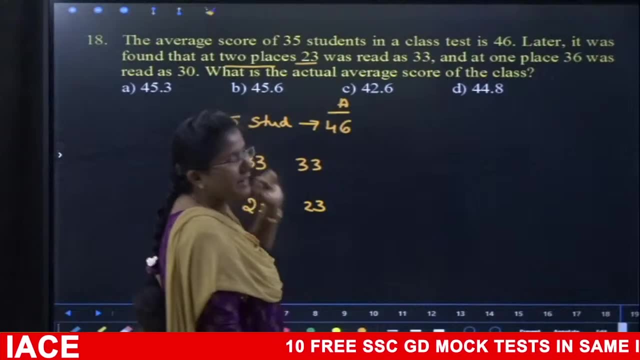 It happened in two places. So 23 was read as 33.. See the next question. At one place, 36 was read as 30. We read 36 as 30. So 36 was read as 30.. 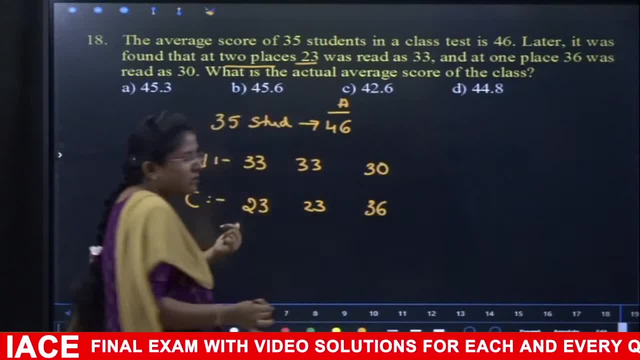 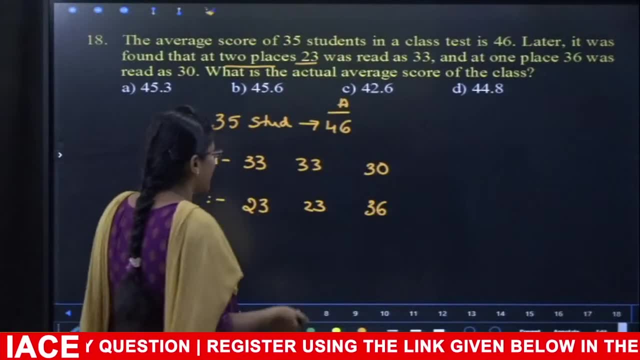 It means 36 is correct and 30 is wrong. It is very easy to know which is correct and which is wrong. So the average is 46 initially. The average will definitely change due to these deviations. Let us see the difference between the numbers. 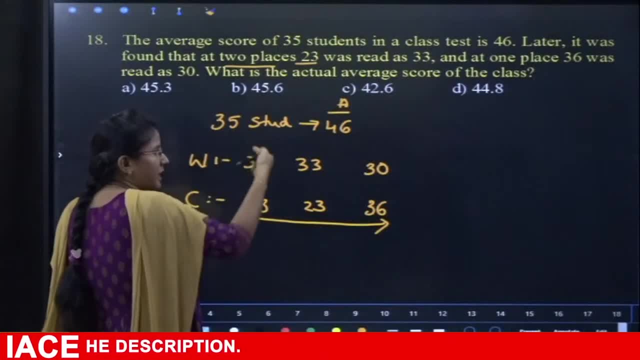 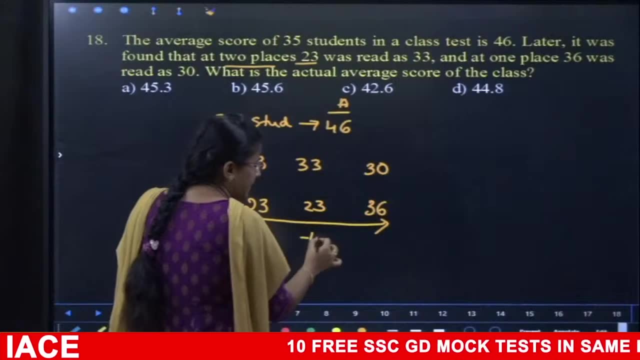 So it is 23 and 33.. When we are doing correction, what should we do? Since it is more than it should be, I will write 10.. Similarly, it is same here. I will write 10 and 10.. 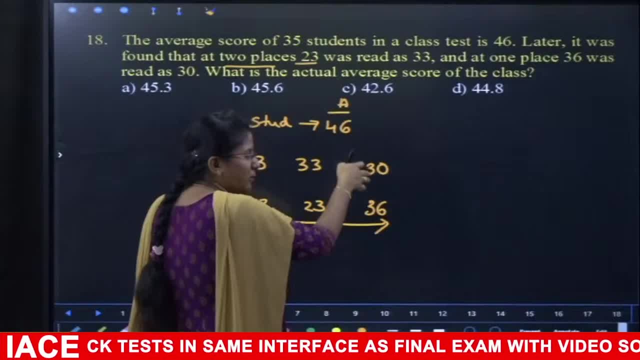 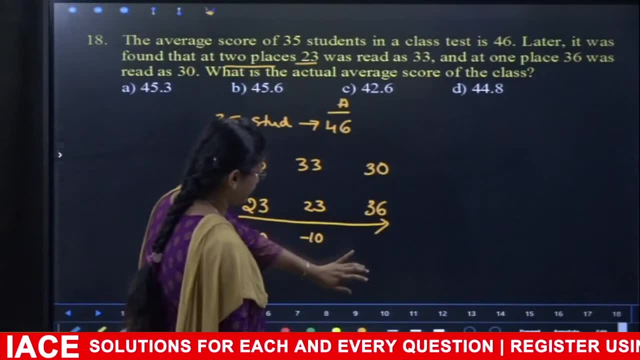 I wrote 36 less than it should be. So what should we do while doing correction? We should add How much should be added? We should add 6.. So there are three people here. We should add How much? 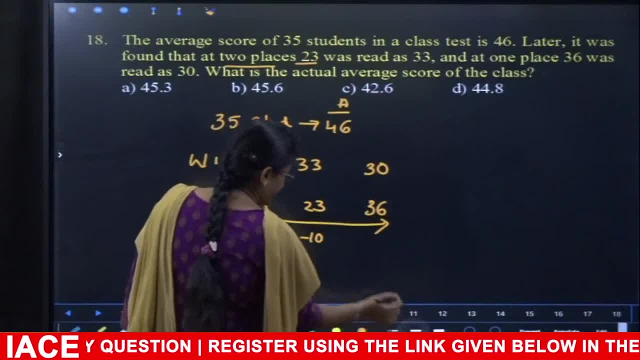 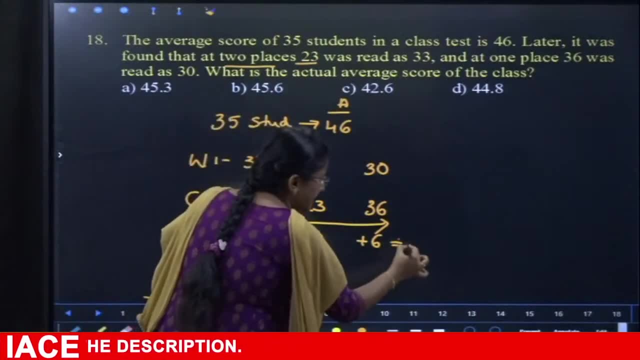 How much We should add. How much We should add. How much should we add? We should add. So, overall, the deviation of 3 people is minus 20 plus 6.. What is minus 20 plus 6?? 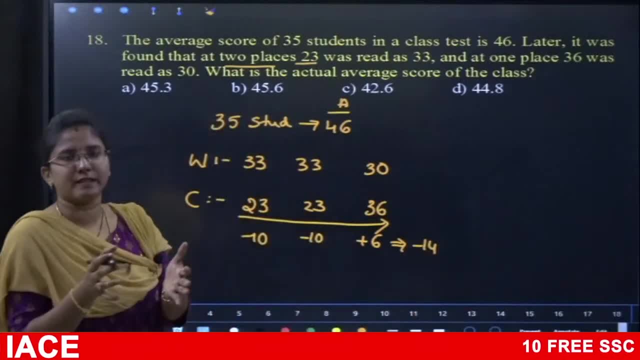 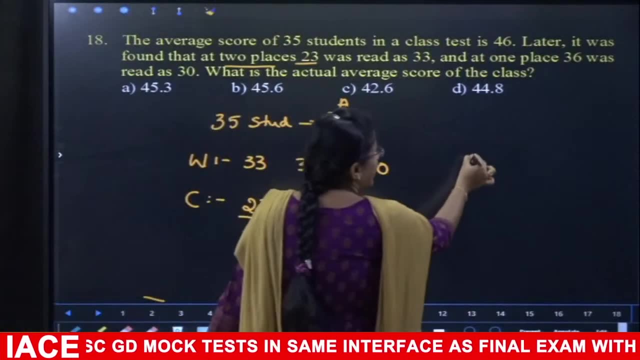 That is minus 14.. We have to take out the deviation of 14 from 35 students. We have to reduce it. How do we do that? We have to do it equally. So taking out 14 equally from how many students. 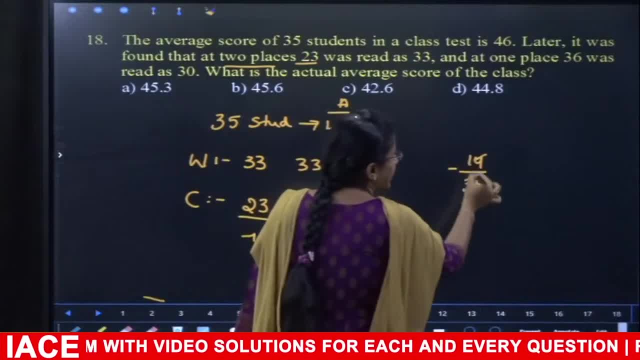 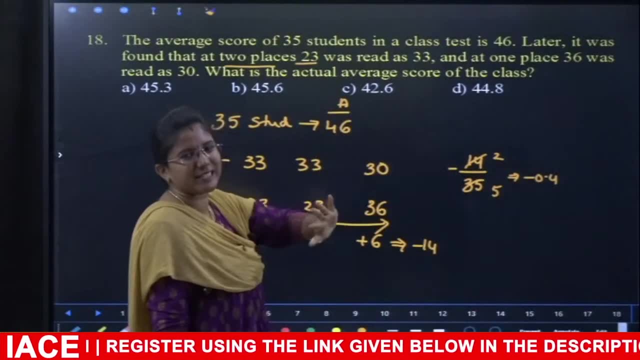 35 students. So minus 14 by 35 will be 2 by 5.. 2 by 5 is nothing but 0.4.. So we will subtract the point from the already existing average part. So the answer will be what. 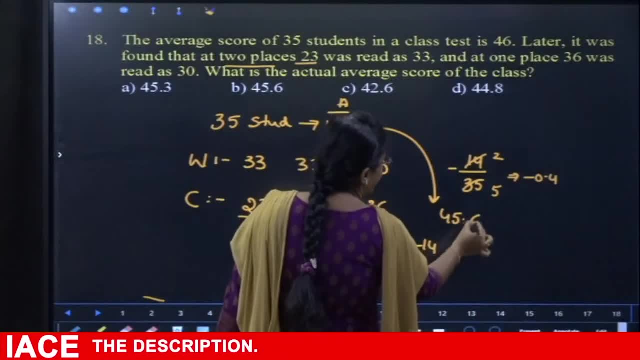 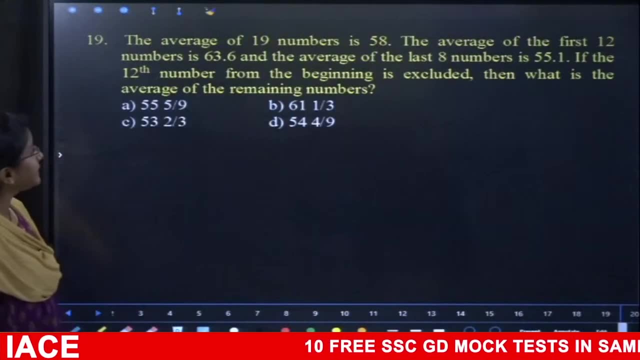 46 minus 0.4 will be 45.6.. So option B Answer is B. Okay, Next Go for next one. 19th. That is also from averages topic. Try this One minute timer please. 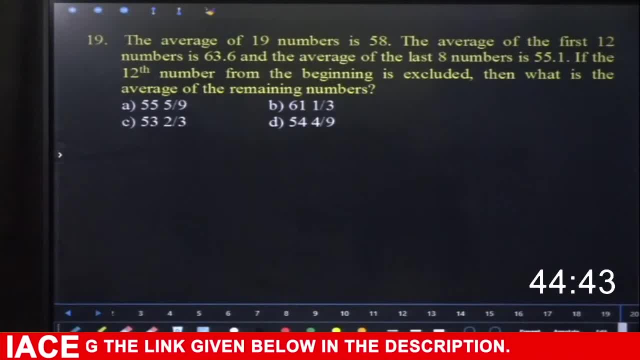 If you came through my lab today I will not make up as much for you with the answers I missed to those of the 30 questions. What is maximum in average average over the type that makes FFB- Let's says 0. simpler. 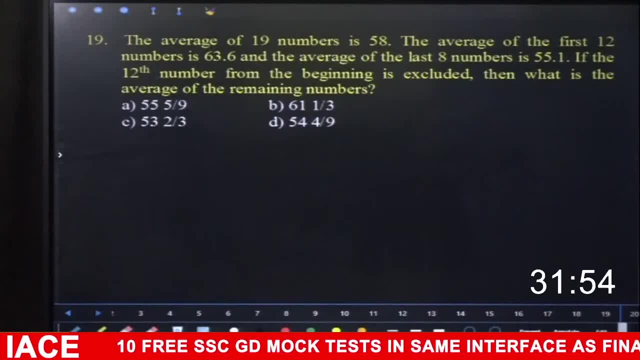 Not true. 1. Not true. Is this the same as M Cannon object? Sorry, Say it again. Very specific These: What are the categories that we have here? Number 1. unloaded irgendwo. 2. other. 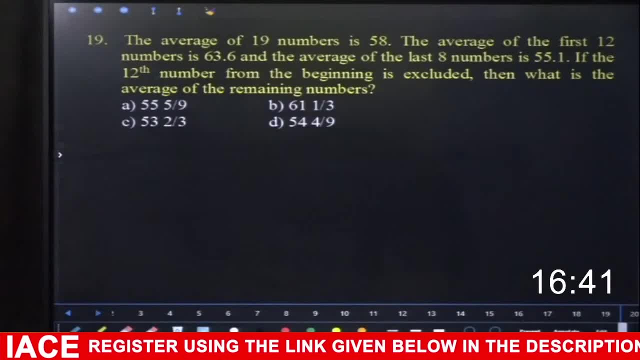 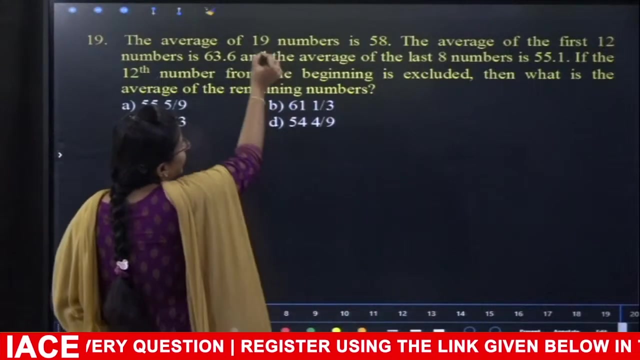 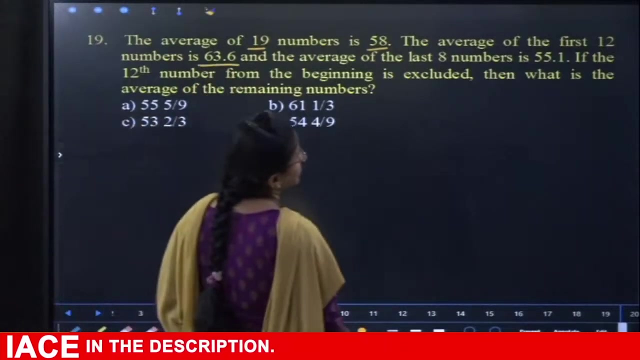 denk保u Over there. Okay, so this question is also from the average age topic, So let's find out the answer. C: Average of 19 numbers is 58,. average of first 12 numbers is 63.6 and last 8 numbers is 55.1.. 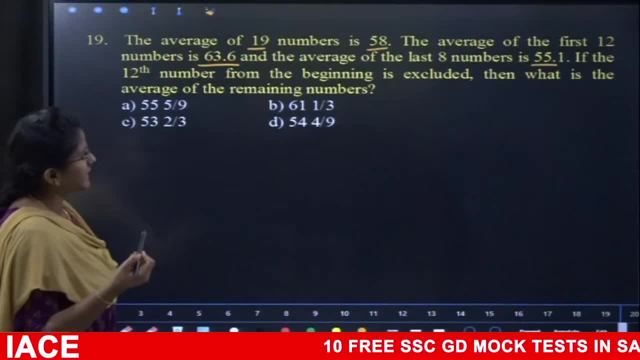 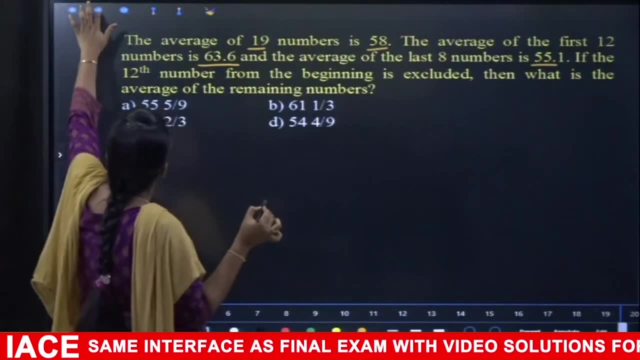 If the 12th number- is from the beginning- is excluded, then what is the average of the remaining numbers? The total number of numbers we have is 19.. Okay, there are 19 numbers. He gave an average of 19 numbers, So let's write the average. 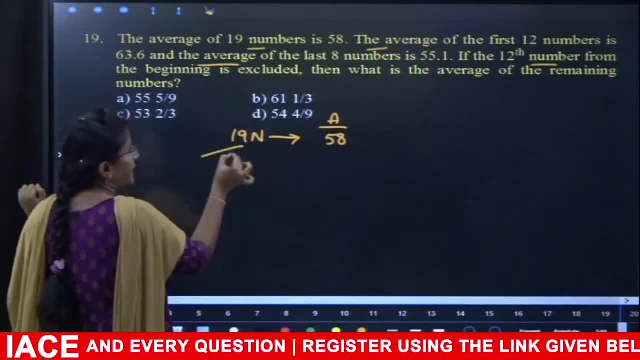 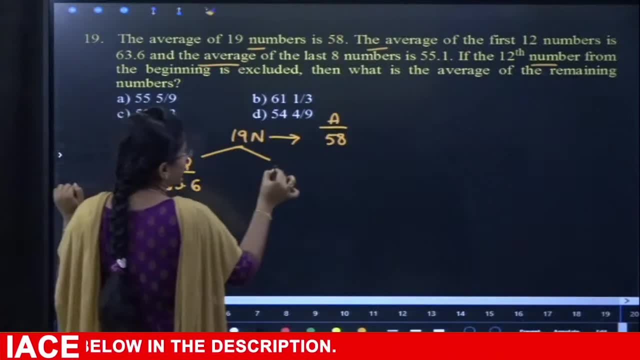 Average is given what? 58.. Alright, in these 58 numbers, he gave an average of 12 numbers separately. The average of 12 numbers is 63.6 and the average of the remaining 8 numbers is 55.1.. 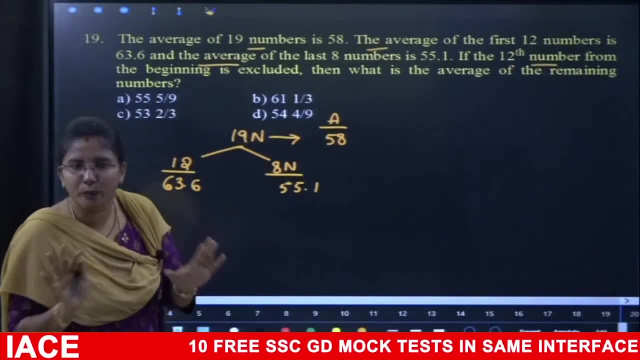 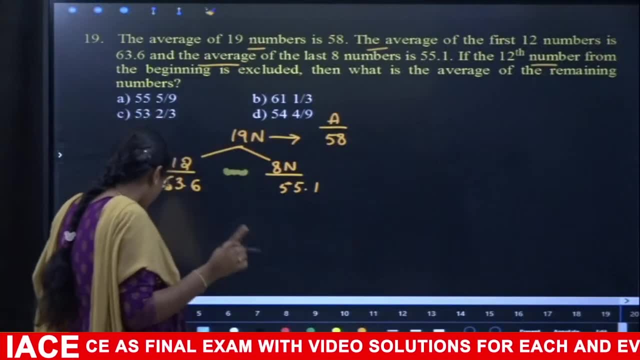 So here there are 12 numbers and 8 numbers. In this group there are only 19 numbers. If there are only 19 numbers, then how should the 12th number in the middle be? It should be common, So that common number is 12th number. 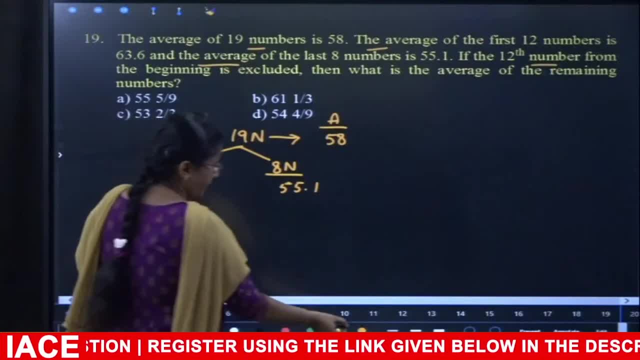 Okay, so let's find out what is that 12th number. If we know what is the weight of that 12th number, the problem will be completed. What is the exact weight of the 12th number? There is no 58.. 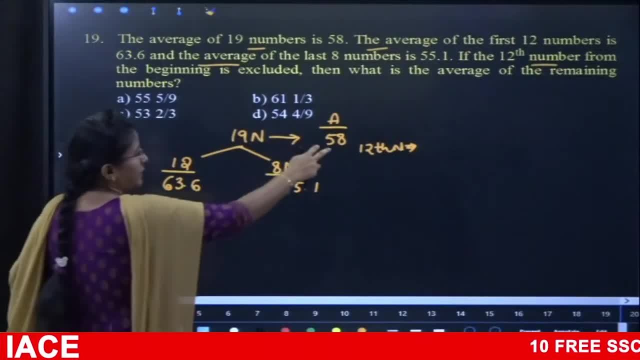 There is more or less than 58. There is something, Let's find out- that. So if we compare it with 58, there is an average of 63.6.. It is more here, So how much is more? 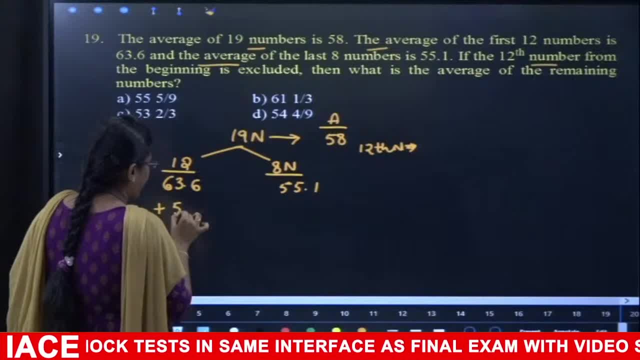 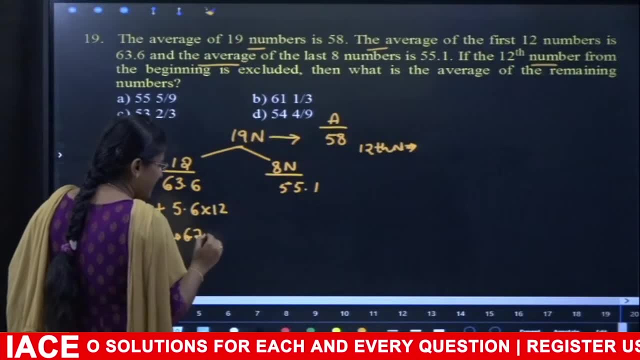 Plus 5.6 for each number. How many numbers are more? It is more for these 12 numbers, So 5.6 into 12 will be. that is. the extra weight here is 67.2.. Next, if we compare it with 58,, it is less here. 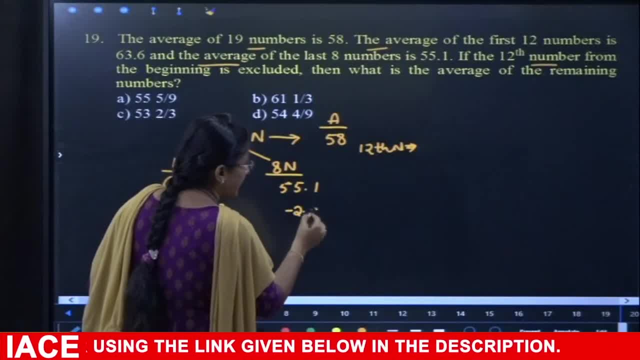 How much is there? If we subtract from 58,, it is minus 2.9.. Less How many numbers are there? There are 8 numbers. That will be 7.. That is 23.2.. It is less. 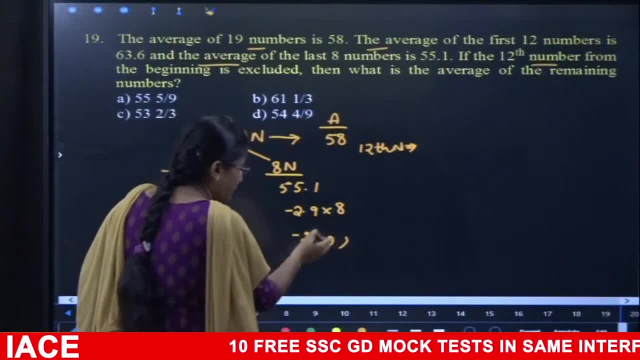 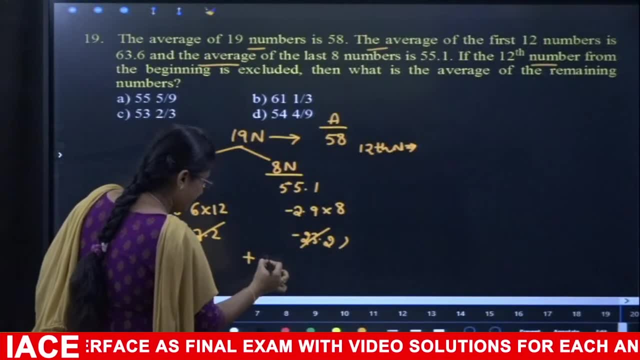 So here we have more than 67.2.. Here 23.2 is less, So there is a deviation for both. If we subtract from this amount, here there is a difference for both. That is 67 minus 23 is 44.. 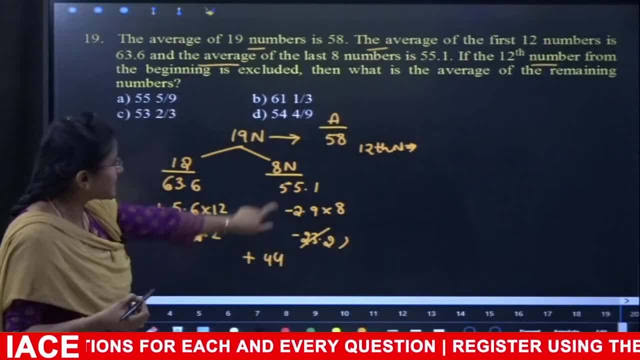 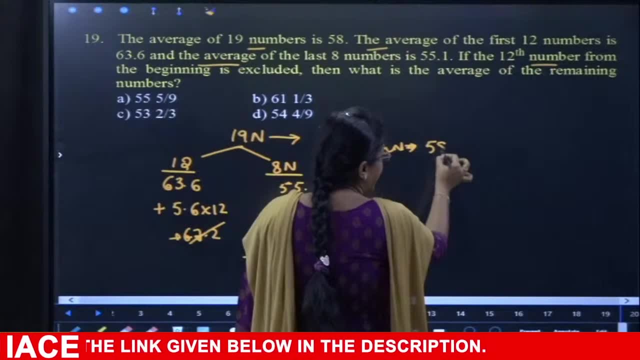 There is an extra 44. This extra 44 will be. This extra 44 weight is the weight of the 12th number in the middle, So that particular 12th number is not 58.. Here, if we get a plus, we will add a plus. 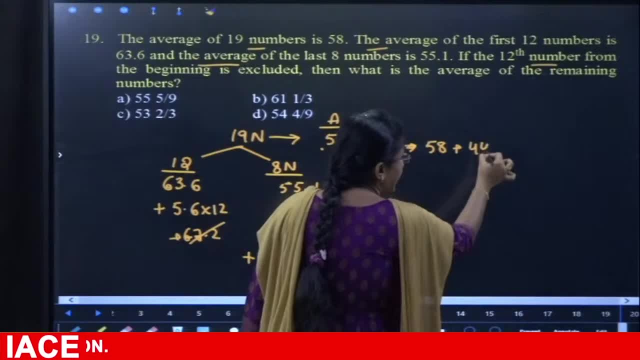 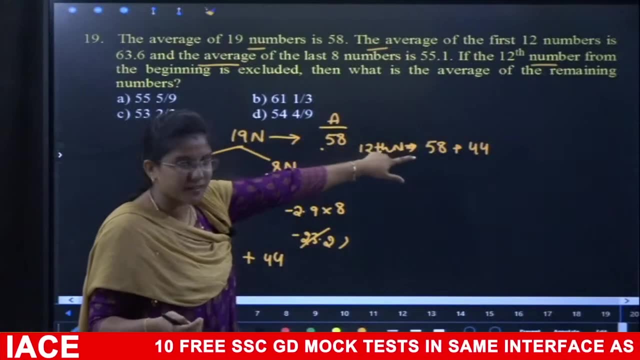 If we get a minus, we will do a minus. That is, this number is not 58. There is an extra 44. If we exclude that number from the extra 44, the already available average is 44. So it is decreasing. 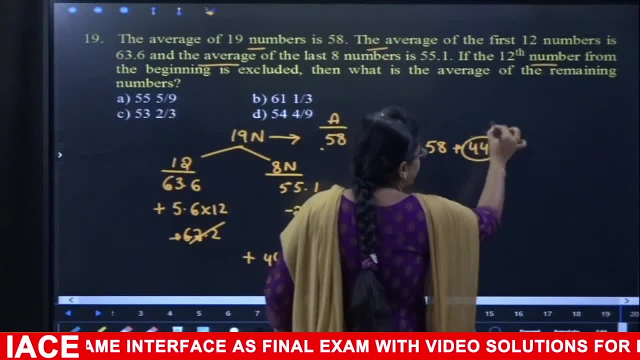 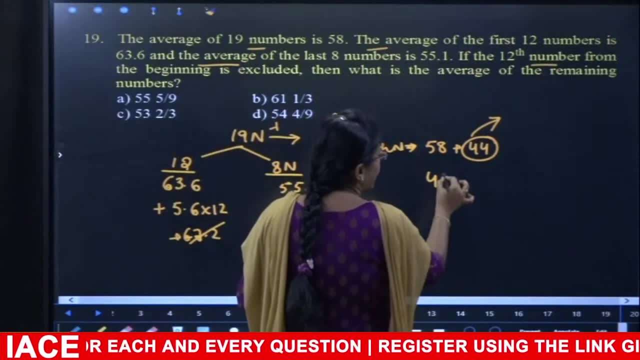 It is decreasing. What is the decrease? This 44 is going out? From how many remaining numbers If we subtract from 19,. that one If we subtract the 12th number From the remaining 18 numbers. So taking out: 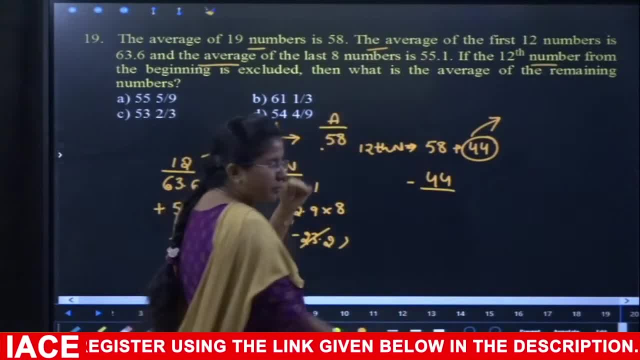 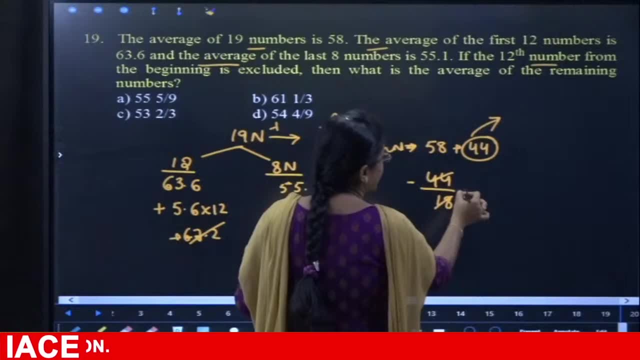 We will subtract 44. How many numbers are there? How many remaining numbers are there when 12th goes out of 19?? From 18 numbers, We will take it out equally. So if we take it out equally, How many are there from each number? 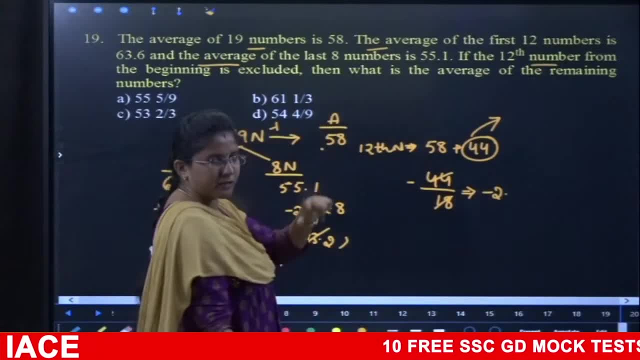 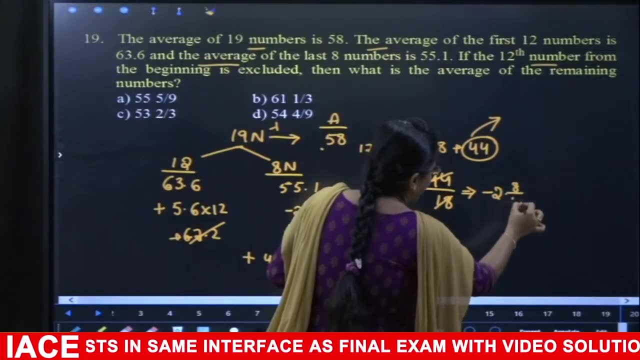 Approximately 2 points. It is like that, Or else because we gave it in mixed fraction, The options will be 2.. If 36 goes, remaining 44 and 36.. 8 by 18.. 8 by 18 will be nothing but 4 by 9.. 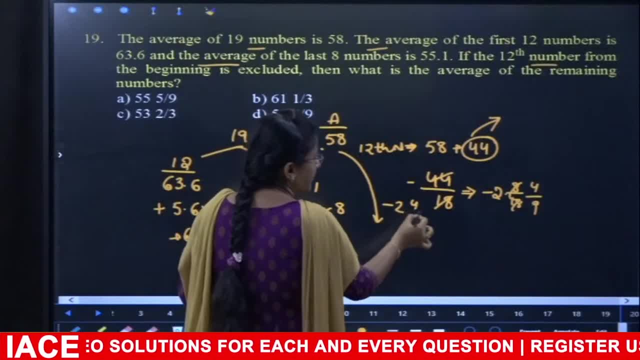 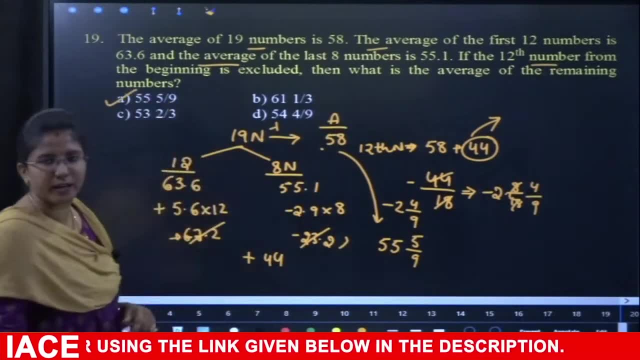 So from the remaining 58, how many we have to subtract 2. 4 by 9.. That is answer 55.. 5 by 9.. Option number 8.. Ok, I understand all of you. 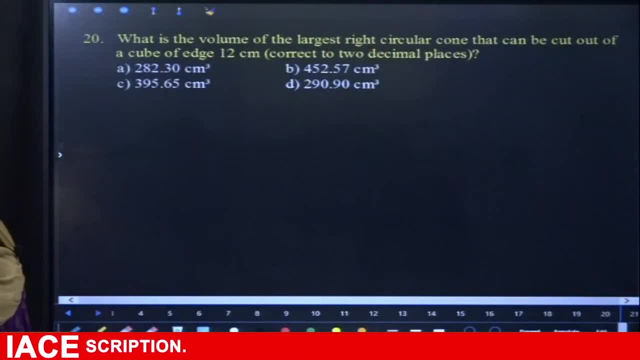 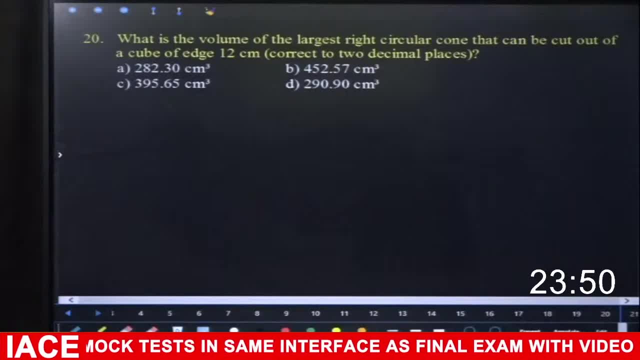 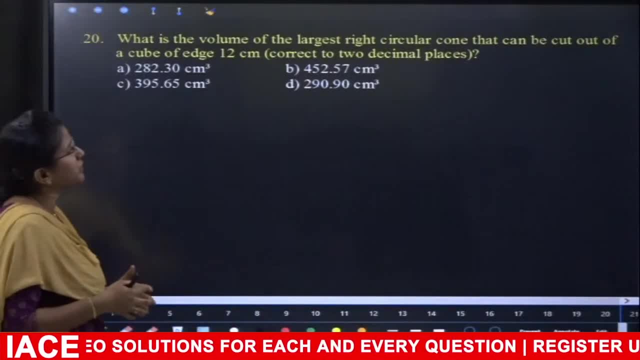 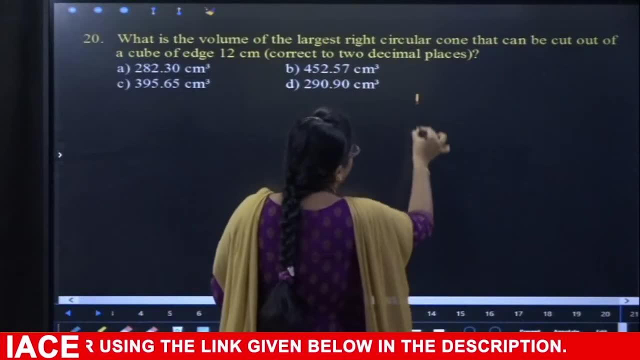 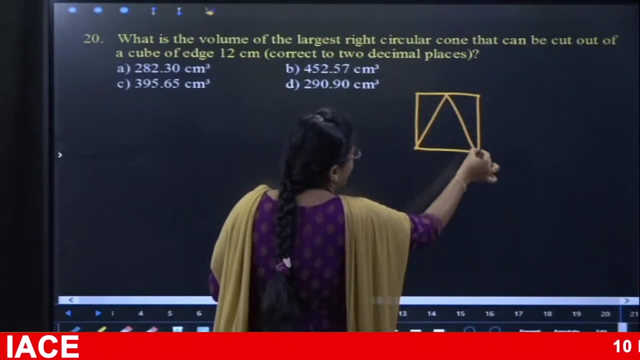 right circular cone that can be cut out of a cube of age 12 centimeters. So decimals. are the points So correct to approximately find out? So nearest answer: Cube. What is the volume of largest right circular cone that can be cut from a cube of side 12? So? 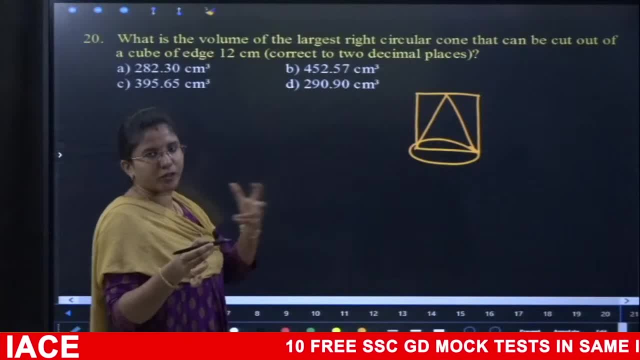 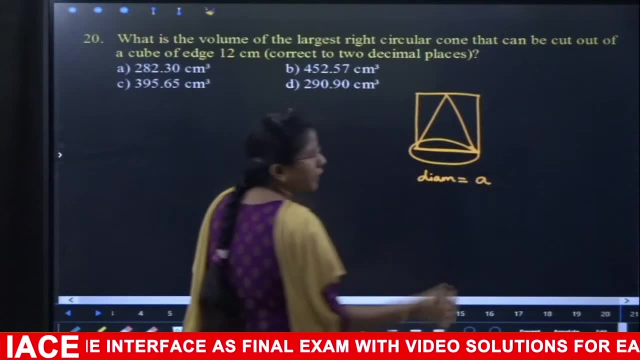 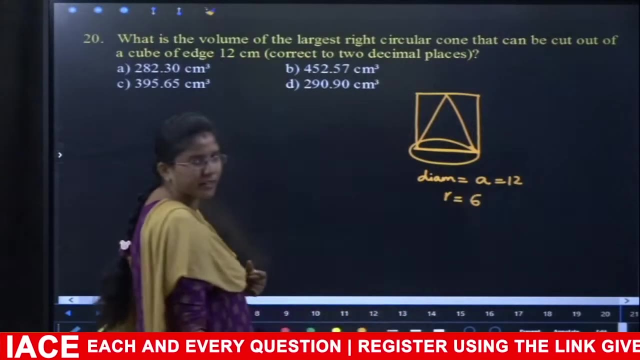 side 12 cube, largest possible circular cone. we have to cut that circular cone's diameter. that diameter should be equal to side of the cube, So side of the cube A will be what did he give already? 12 gave. So diameter, 12, what is the radius? Half right, 6.. So 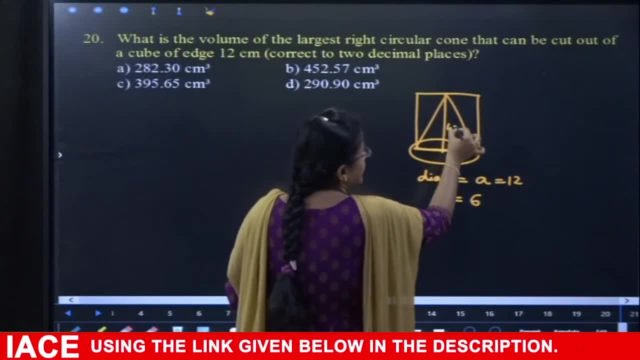 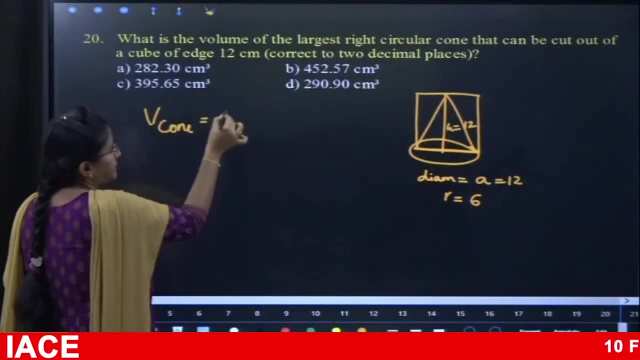 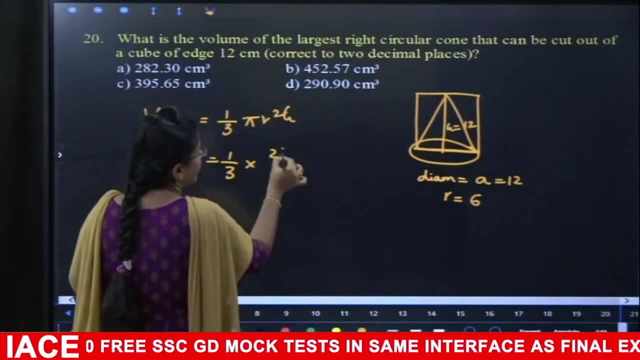 height of the cone also. already what is happening, That is side only 12.. So volume, find out. so volume of cone, we all know formula What 1 third pi r square h 1 third pi will be, that is, 22 by. 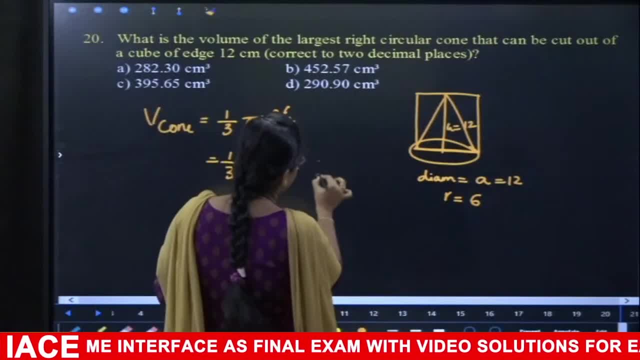 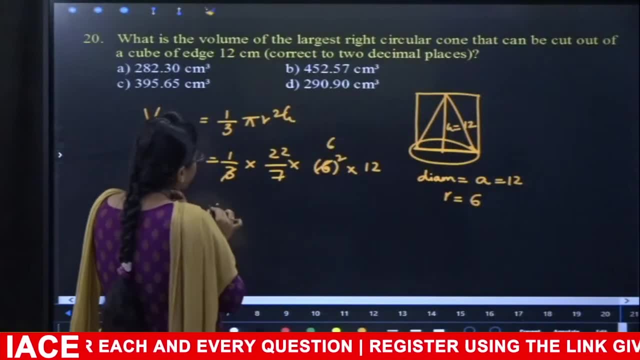 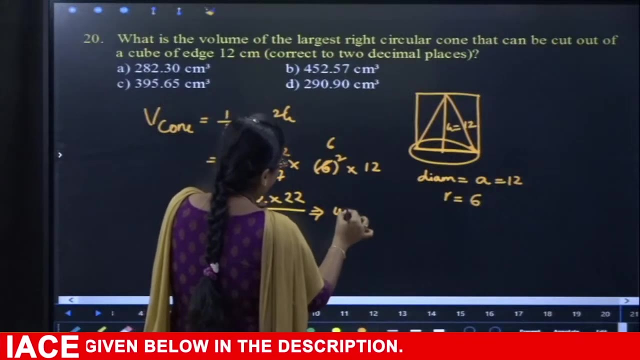 7. r square is 6, square Height will be what? 12.. So here, if we cancel out one 6, there will be another 6. That is 12672 into 22 by 7.. Approximately we get 446 points. Since. 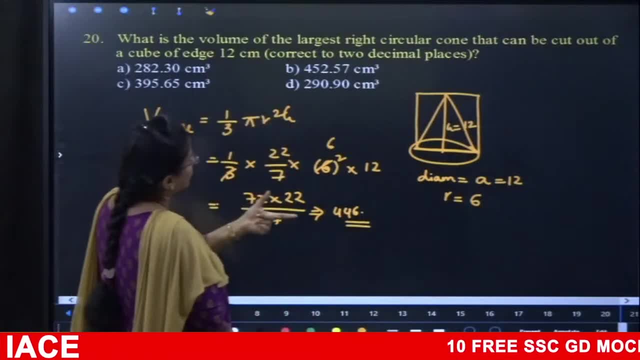 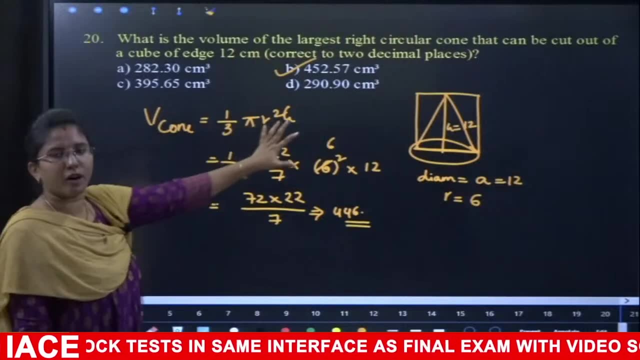 nearest integer is said we have 442.. We can see unit digit only. Since there is only one option, we cannot cancel out 4 times, So answer 452.. 5.57.. Just a formula, substitution only. We call it as height and radius only. Okay, Next. 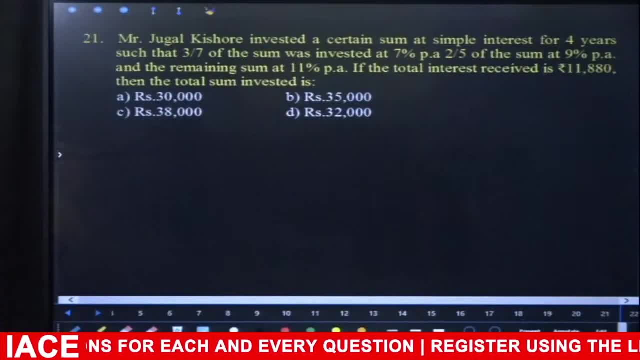 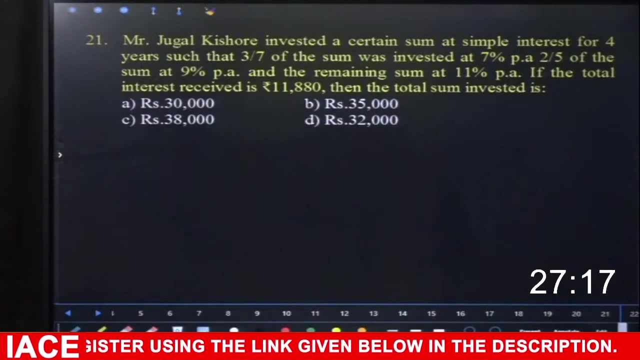 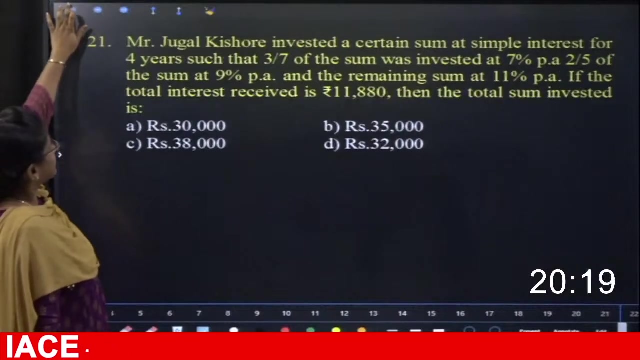 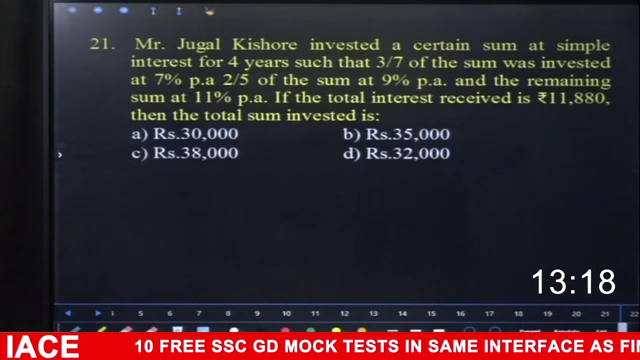 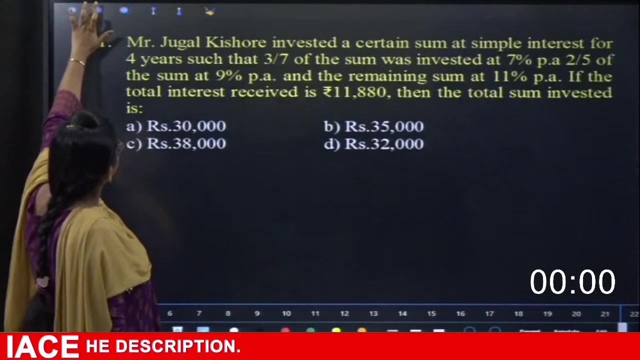 Next we will try 21.. Equation: one minute timer please. Yep. Step 3. magic club�, Step 3. magic clubben, Step 3.. magic clubben, Step 3.. magic clubben. Biff G on C. Okay, here this question comes from the topic of simple interest. 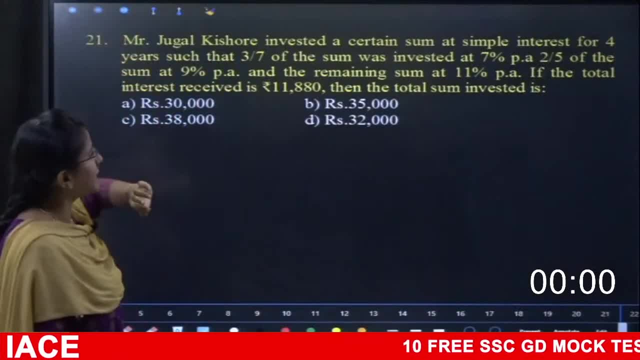 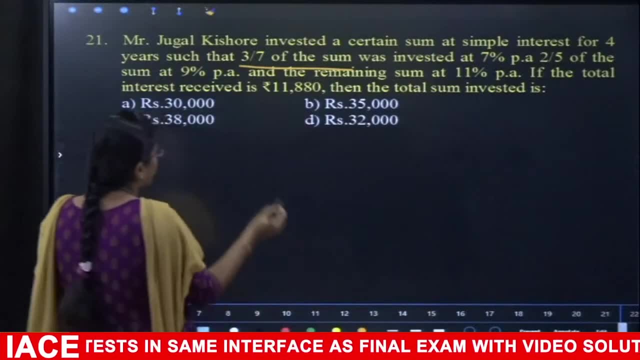 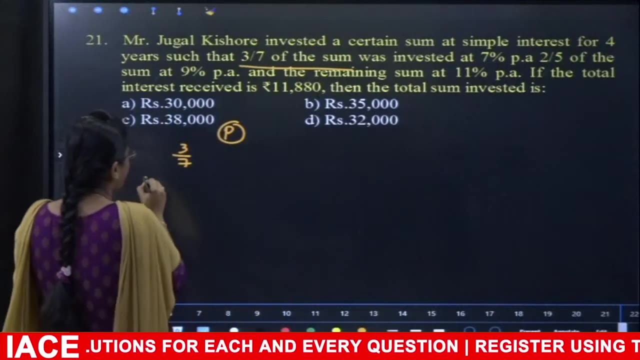 Mr Jugal Kishore invested a certain sum at simple interest. for how many years? 4 years, such that 3, 7th of this sum was invested at 7% per annum. We have a principle in which 3, 7th of this sum is invested at the rate of 7% per annum. 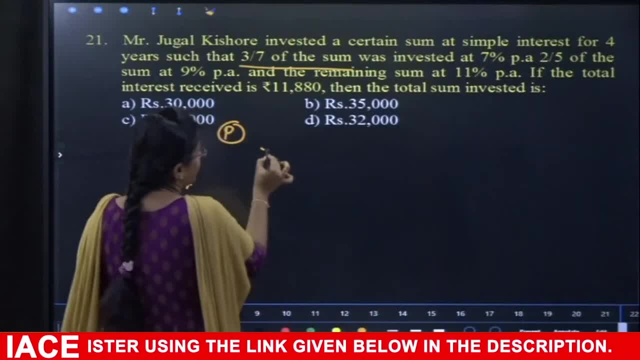 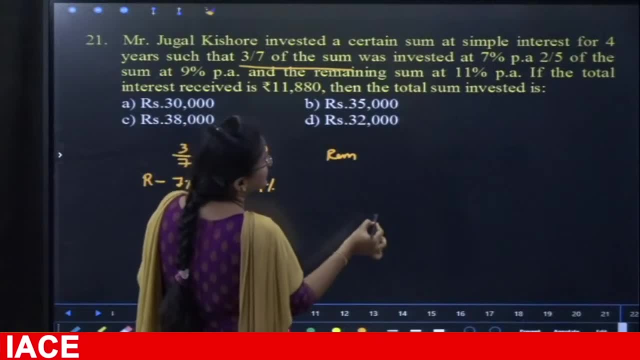 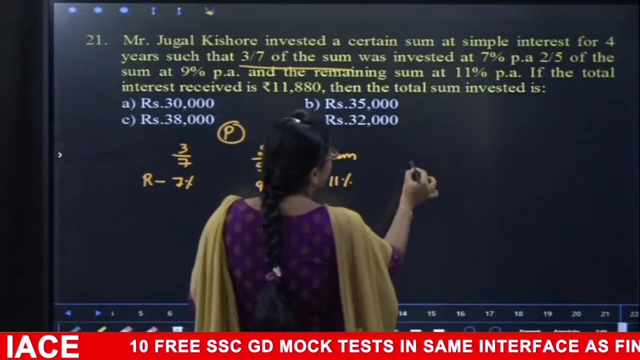 And next 2: 5th of principle is invested at the rate of 9% per annum. After these two, he invested remaining remaining amount at the rate of 11% per annum. What is the total we got? Mr Jugal Kishore gave simple interest at 4 years. 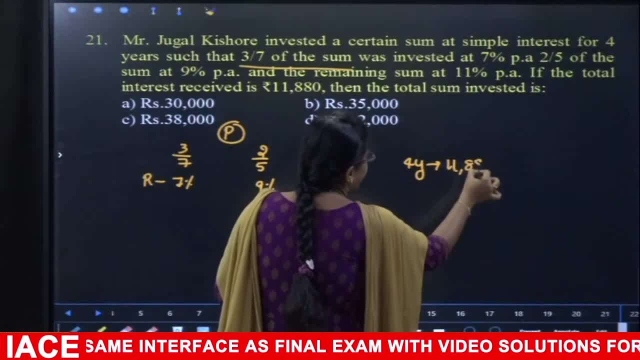 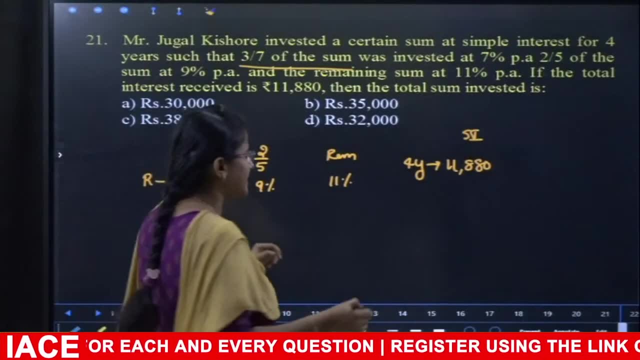 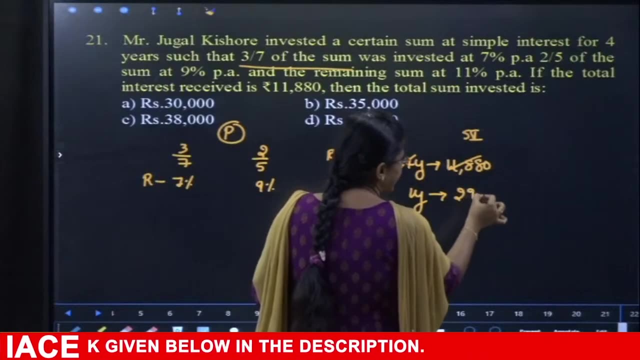 What is the total interest? we got 11,880.. Simple interest for how many years? 4 years. Simple interest is constant every year, right? So let us write it as 1 year. If it is 11,880 for 4 years, it is 2970. 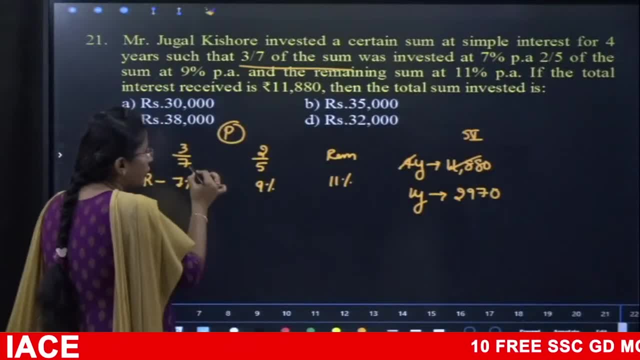 So let us see it as 1 year. So we can catch the option of 3- 7th and 2- 5th by using the denominator Here. 7 and 5 means 35 should definitely be there. 35 is the only one. 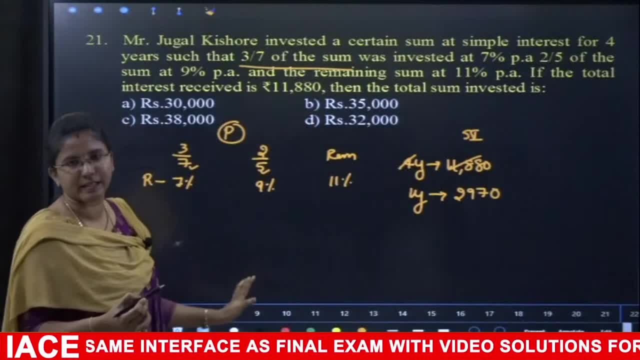 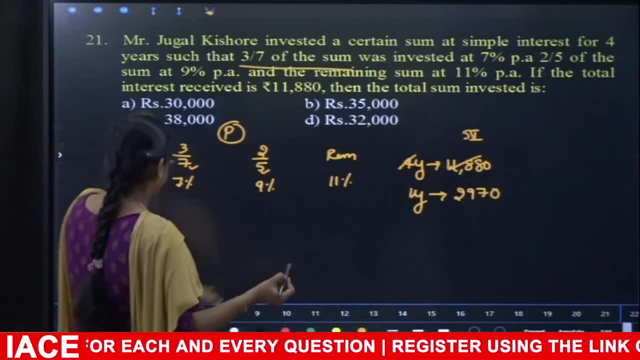 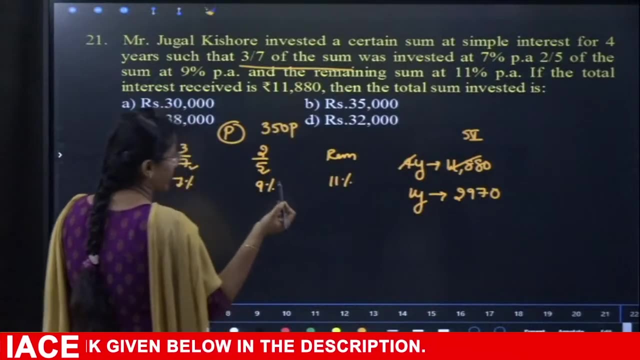 Option. we can take 35000. It will be enough if we check it. Or else, as 7 and 5 is 35, take some 350X. It can be 35 parts or 350 parts. I prefer 350 parts, P or X. 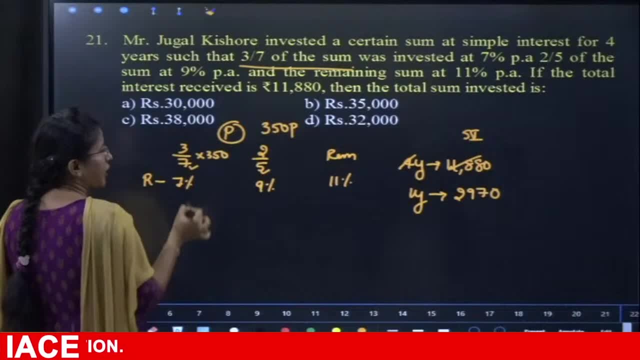 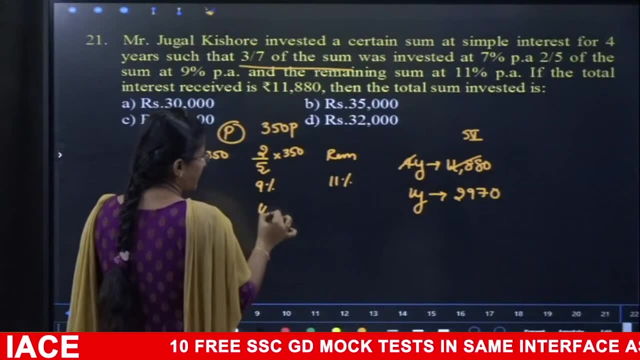 In 350 parts. when we say 3, 7th and 350, that will be how many parts? 150 parts. Next here, when we say 2, 5th, 2, 5th of 350, that is 140 parts. 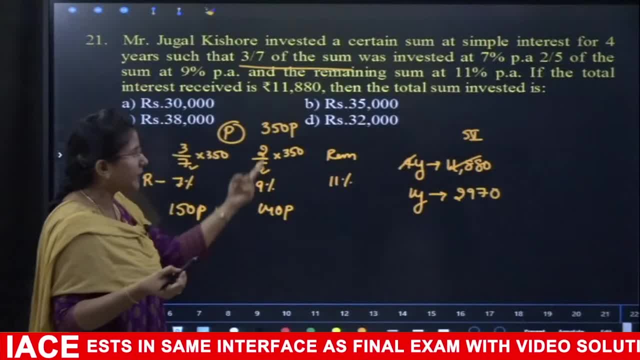 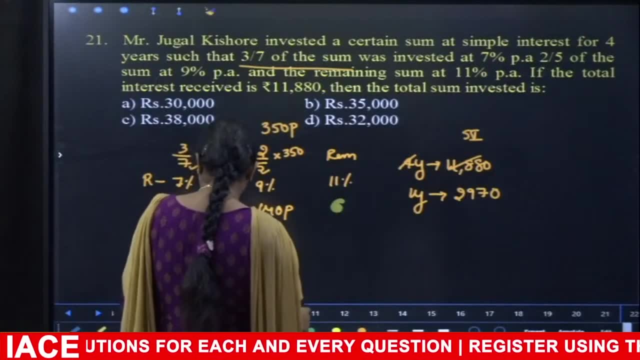 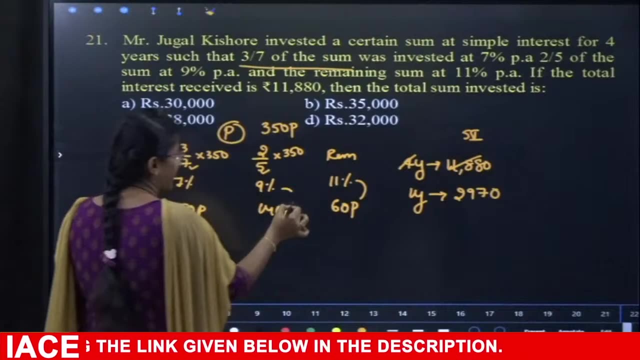 So here we have 150, 140, 290.. Out of 350,, 290 is completed. If 290 is completed, how much will be remaining? 60 parts 60. In these 60 parts, you can take 11%, 9% and 7%. 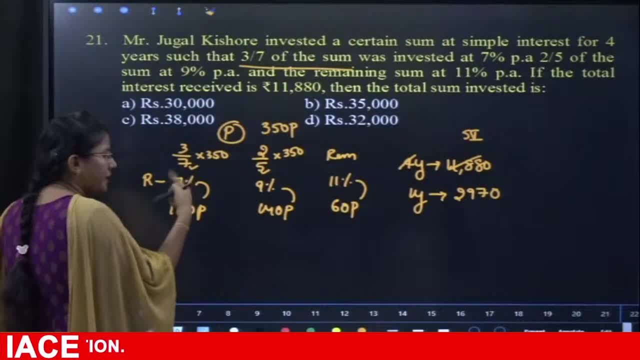 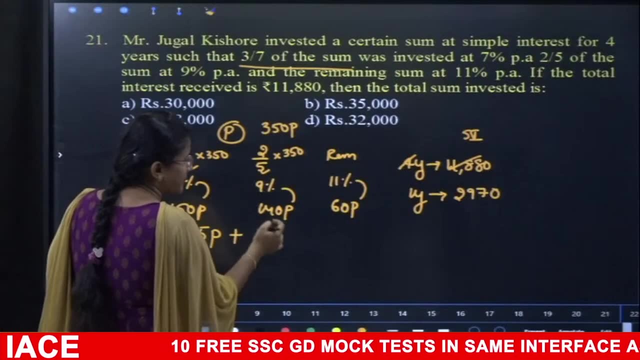 So let me tell you: 1507% means 1.57 times 1.57 times, That is 10.5 parts. Next, 149% will be 1.4 into 9.. 1.4 into 9 will be 12.6 parts. 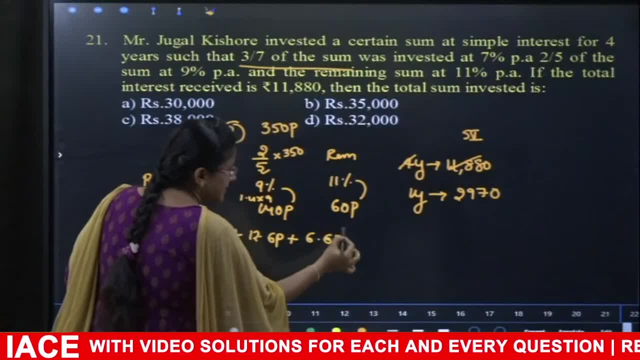 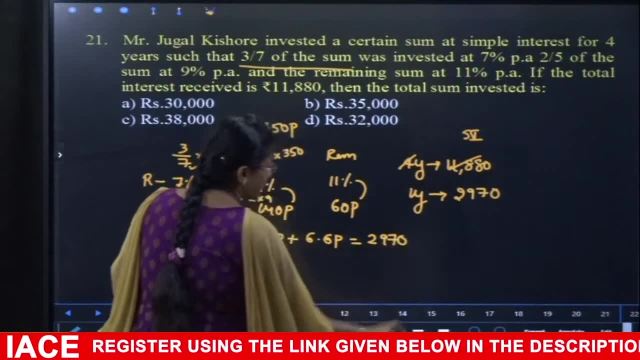 Then in this 11% will be 6.6 parts Simple interest. We will add the rate of interest directly, The total interest given is 2970.. So if we add all these we will get 29.7 parts. 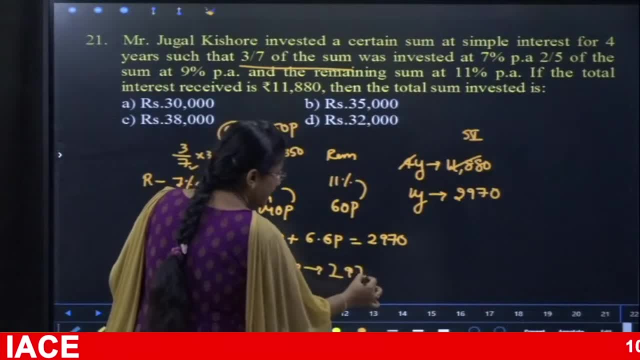 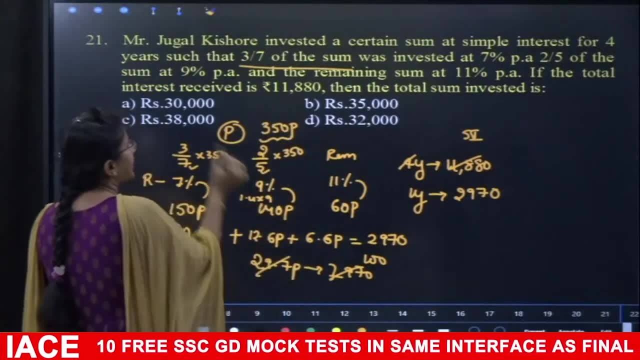 If 29.7 parts is 2970, then each part value will be 100.. Since it is 100, one part is 100.. Since I took 350 parts, 350 into 100 will be. the answer is 35000.. 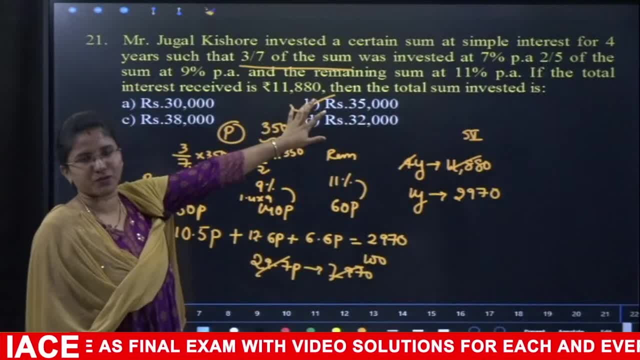 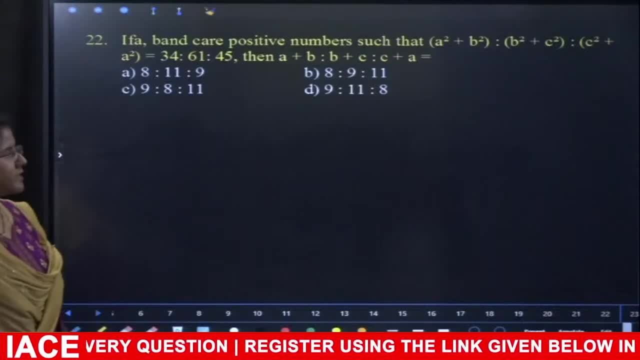 We can put the option we choose immediately- Please check the verification- Or we can solve the process like this: Next Go for next one- 22.. Easiest question: 30 seconds timer please. Please try 30 seconds timer please. 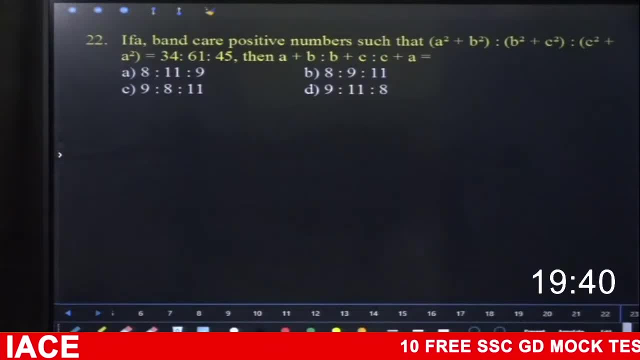 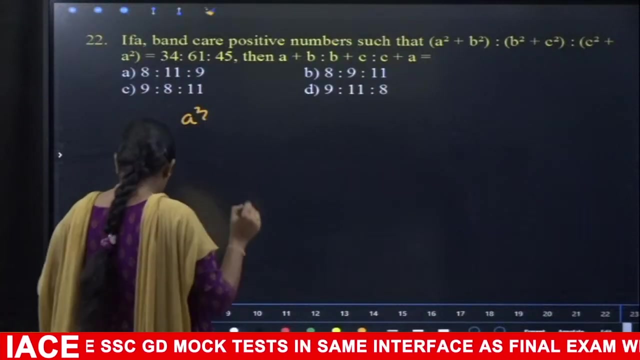 Okay, So your timer is up. Then, given in the question if A, B, C are positive numbers, such that A square plus B square, B square plus C square, C square plus A square, So once the ratio given is A square plus B square, 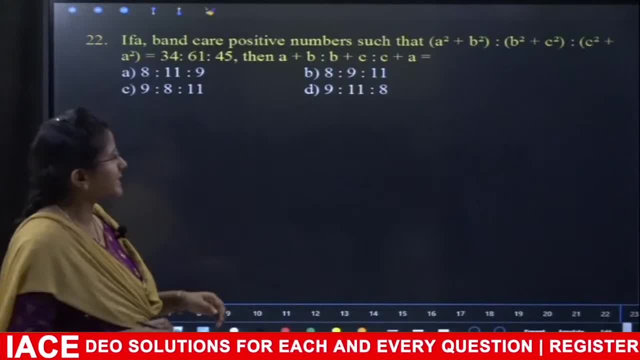 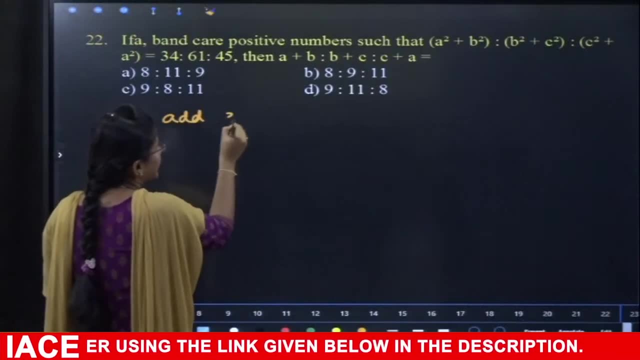 If we directly add all the parts given in the ratio A square plus B square, B square plus C square, C square plus A square, Add all three. If we add all three, A square will be 2 times, B square will be 2 times. 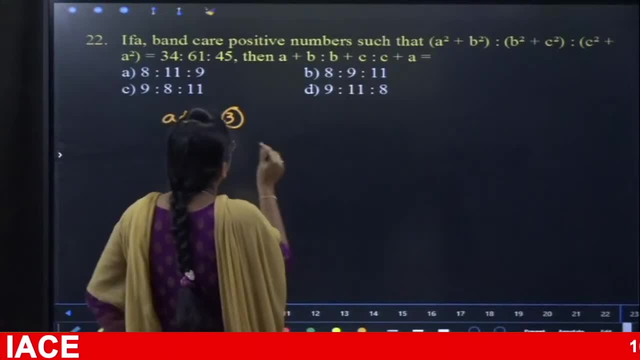 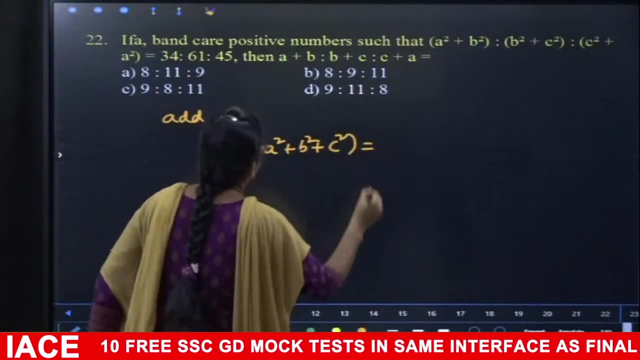 C square will also be 2 times. So since it will be 2 times, we can directly write 2 into A square plus B square plus C square. So if we add all the parts 34 to 61, that is 95.. 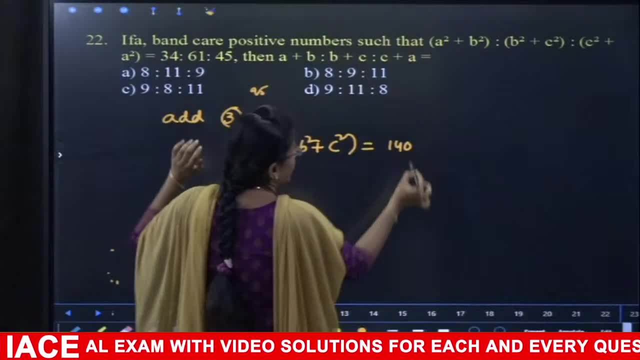 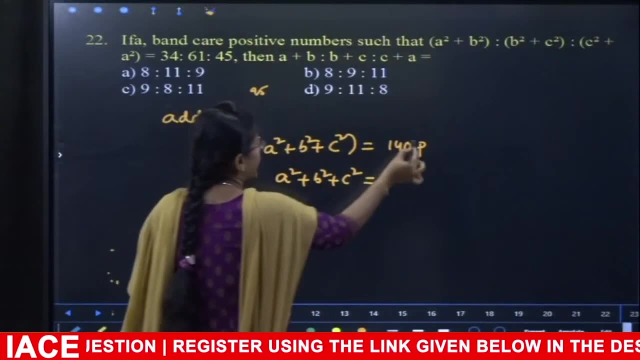 95 to 45,, that is 140.. 140 parts, So that will be A square plus B square plus C square. If we want it to be one single, we will divide it by 2.. How many parts are there? 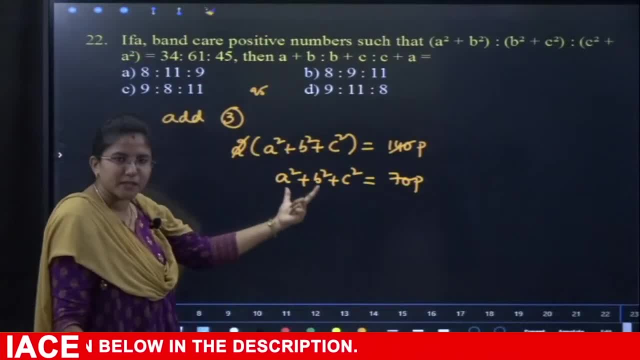 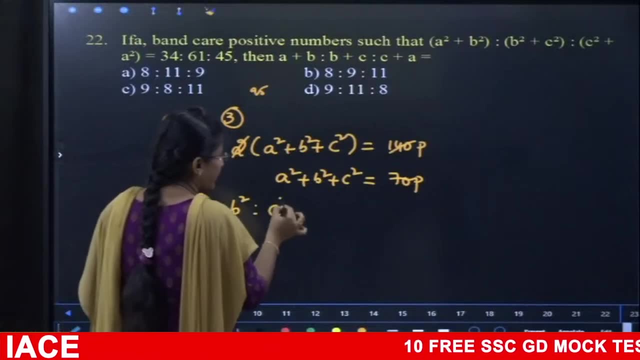 70 parts. So this one A square plus B square plus C square. from these 70 parts directly we can take: A square is 2, B square is 2, C square, Write it down. How do we write it? 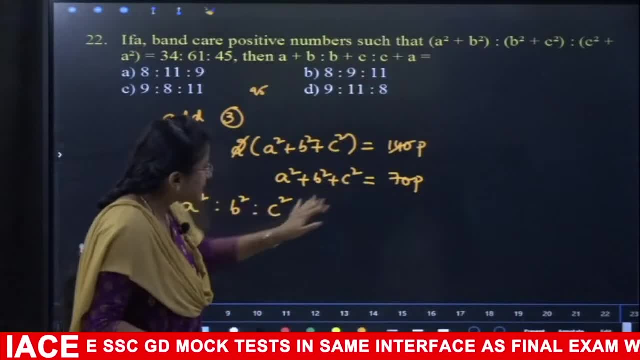 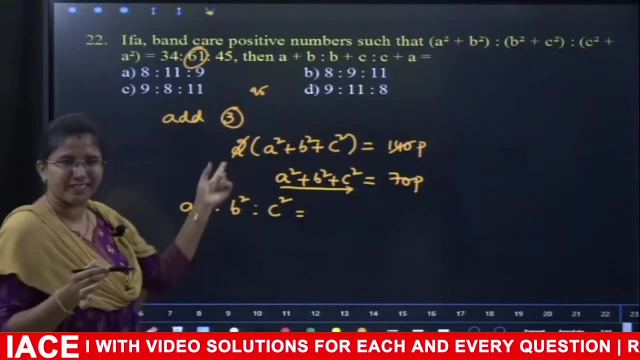 If I want A square specifically from this sum of A square plus B square plus C square, if I want A square only if there is B square plus C square, how many parts are there? There is 61.. I will deduct it. 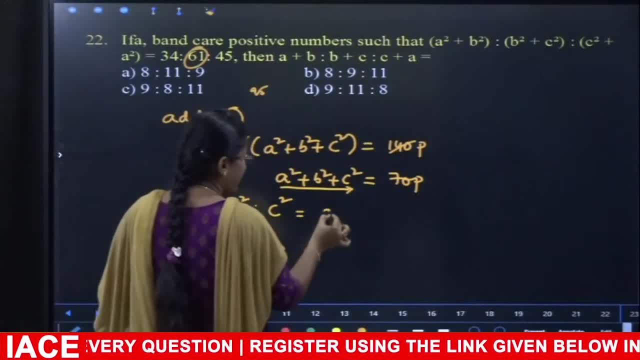 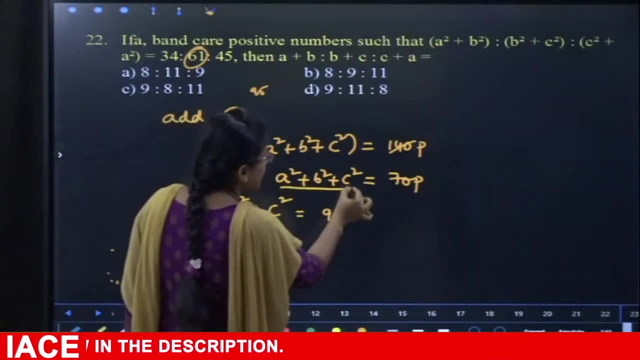 So 70 minus 61. If I subtract 61, how many parts are there? 9.. So next, I want B square. If I want B square specifically, what will we deduct from the already existing sum This time? 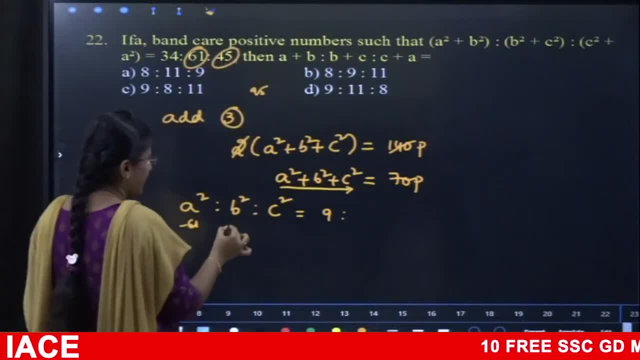 we will deduct A square plus C square. That means how many parts do we have to subtract Minus 45.. How many parts are there already? 70.. If we subtract 45 from 70, how many parts are there? 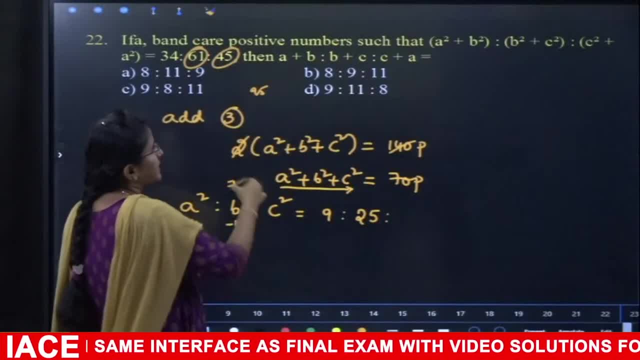 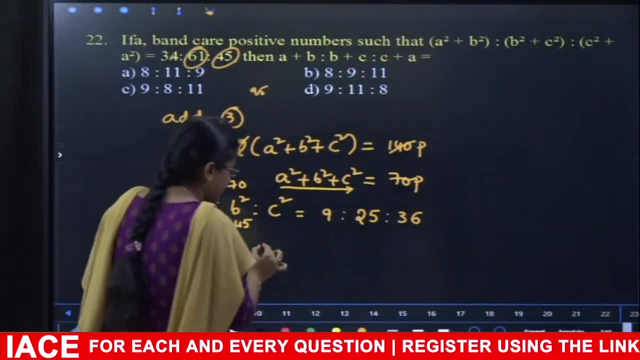 Yes, 25.. Similarly, what do we have to deduct from the last part, 70?? This time we will subtract 34.. How many 36.. If the ratio of squares is 9 to 12,, 25 to 36,? 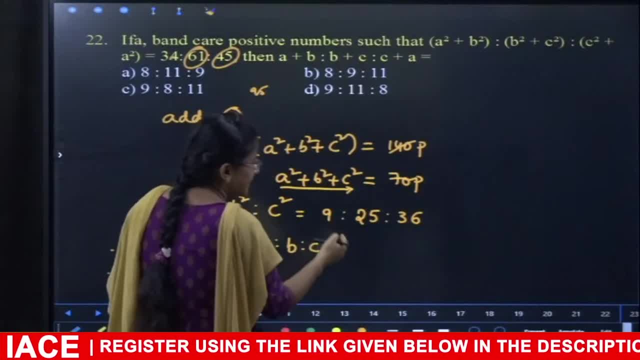 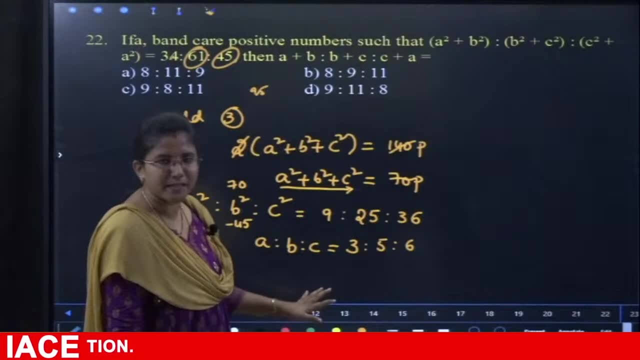 A to B to C, the square root is 7.. What is 9 square? If we subtract 25, it is 36.. If we subtract 46,, it is 6.. So now we will add: Since A plus B. 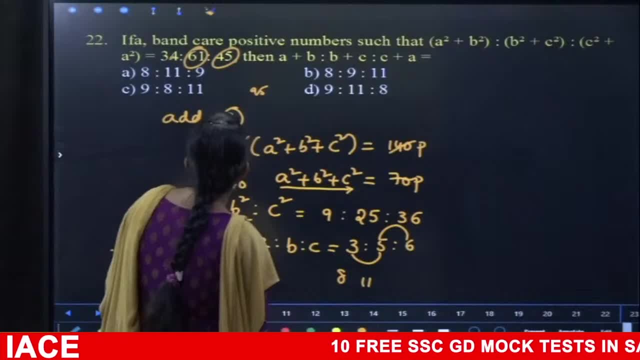 B plus C, C plus C, he asked. A plus B is 8.. B plus C is 11.. Next, C plus A is 9.. That is option A. 8 is to 11 is to 9.. Okay. 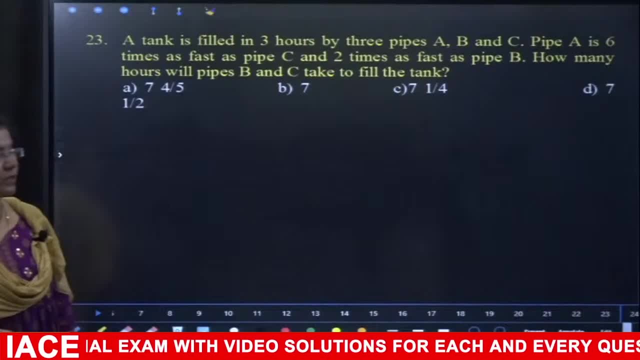 Next, Next one: 23.. Try it dear: 30 seconds. One minute timer. Try the equation from Pipes and Systems. topic: One minute timer. Okay, Next one. 23.. Try it dear: 1,, 2,. 3,, 4,, 5,, 6,, 7,, 8,, 9,, 10,, 11,, 12,, 13,, 14,, 15,, 16,, 17,, 18,, 19,. 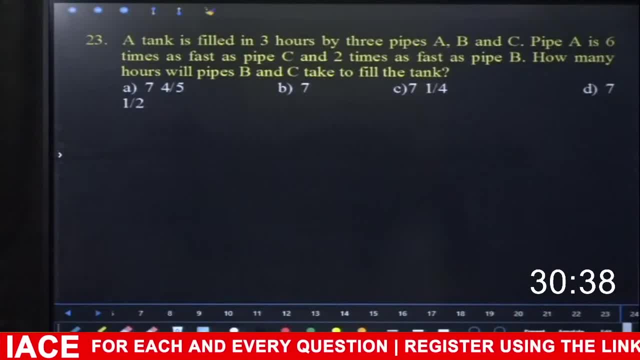 20,, 21,, 22,, 23,, 24,, 25,, 26,, 27,, 28,, 29,, 30,, 31,, 32,, 33,, 34,, 35,, 36,. 37,, 38,, 39,, 40,, 41,, 42,, 43,, 44,, 45,, 46,, 47,, 48,, 49,, 50,, 51,, 52,, 53,. 54,, 55,, 56,, 57,, 58,, 59,, 60,, 61,, 62,, 63,, 64,, 65,, 67,, 68,, 69,, 70,, 71,. 62,, 63,, 64,, 65,, 66,, 67,, 68,, 69,, 70,, 71,, 72,, 73,, 74,, 75,, 76,, 77,, 78,. 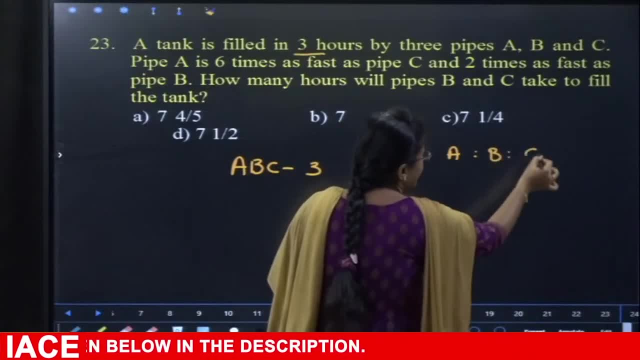 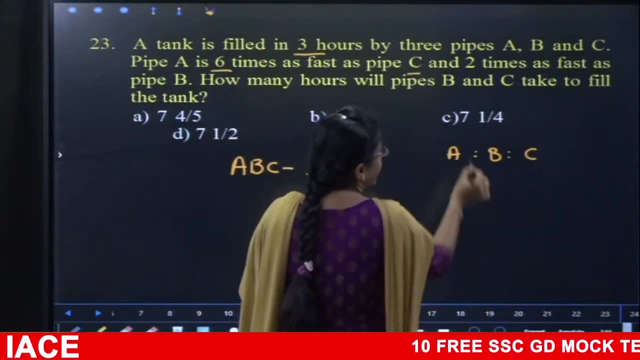 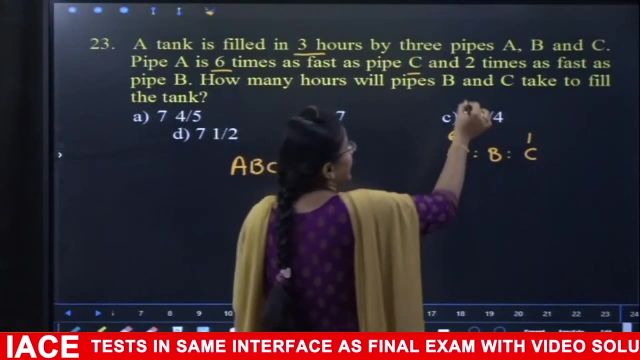 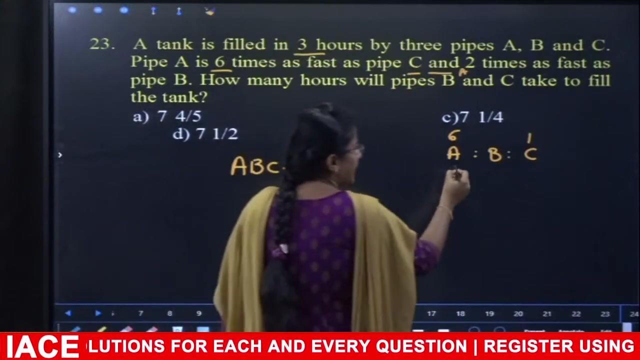 79,, 80,, 90,, 91,, 91,, 92,, 92,, 93,, 94,, 95,, 96,, 97,, 98,, 99,, 100,, 140,, 85,. 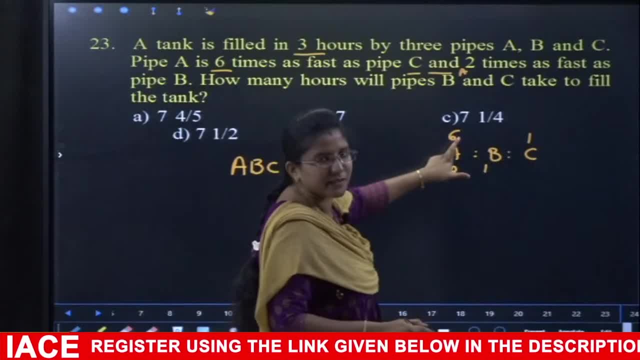 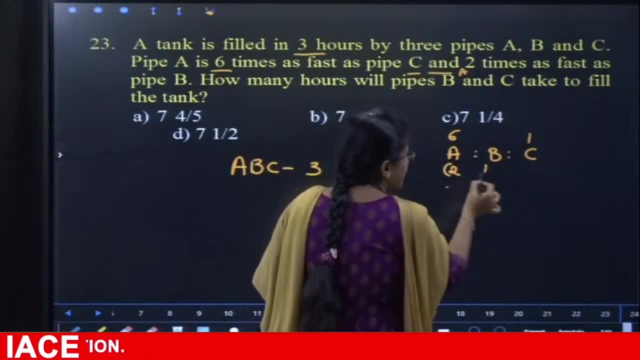 110,, 100,, 102,, 101,, 120,. 2 will not be like that. Since it is a pipe that fills, we will do the same efficiency. Since we can do 2 by 6 in this ratio, we will do 2 by 3.. So here A will be. 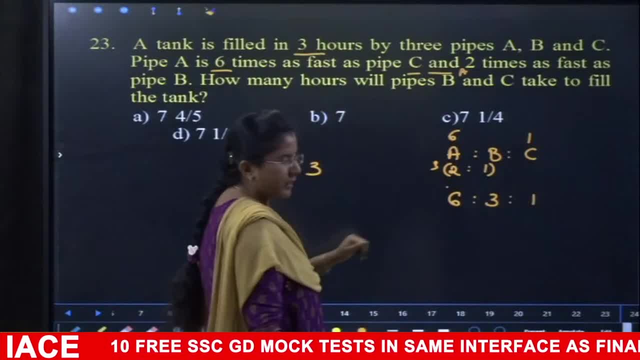 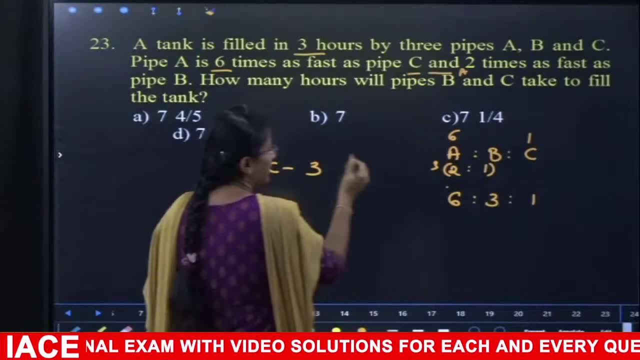 6, B will be 3, C will be same: 1. So C has 6 times and B has 2 times. Since the efficiency has come: A, 6, B, 3, C, 1. If we mix 3,, 10 liters will be filled 3 into 10, how many liters tank is there? 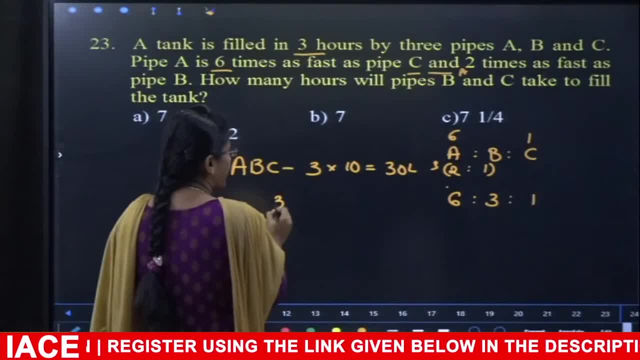 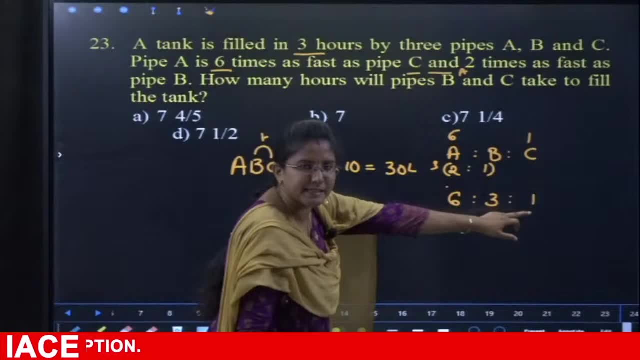 30 liters is there. Now whoever wants to work to fill the same tank with 30 liters. they have B and C. So B and C efficiency is to be added. B, 3, C, 1.. So 3 plus 1, total 4.. So how much time is it taking? 30 by 4, it is. 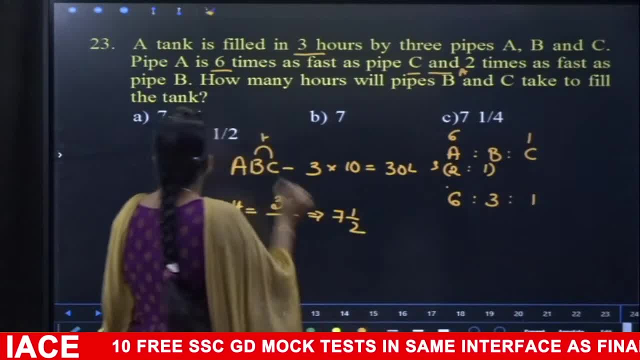 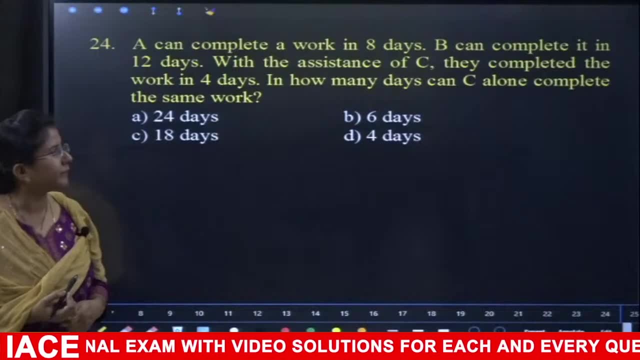 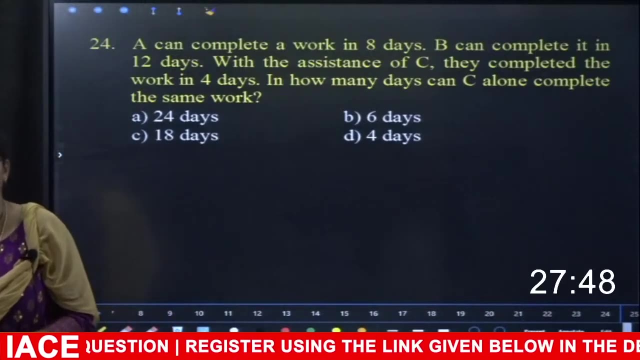 7 and half hours. Option D: 7.5.. Ok, Very easy equation. Next Go for next one: 24.. Try it. So this is also a very easy equation: 30 seconds timer. 30 seconds timer, please. 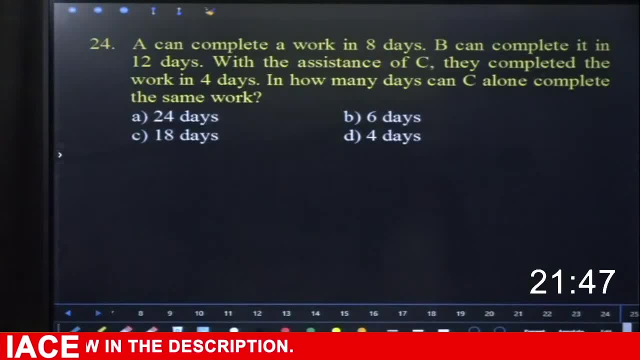 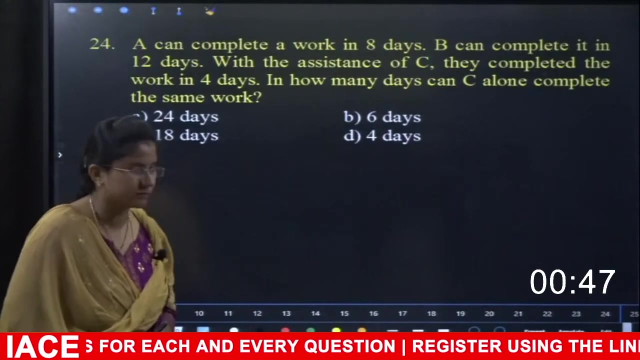 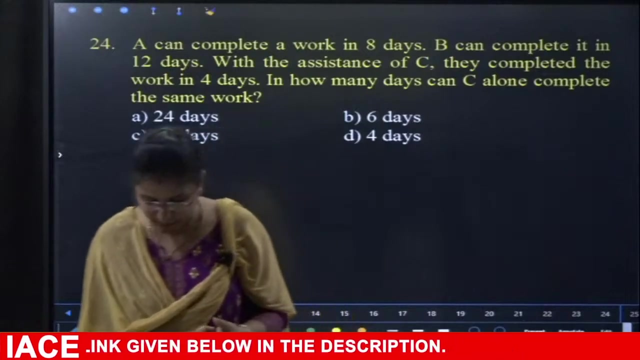 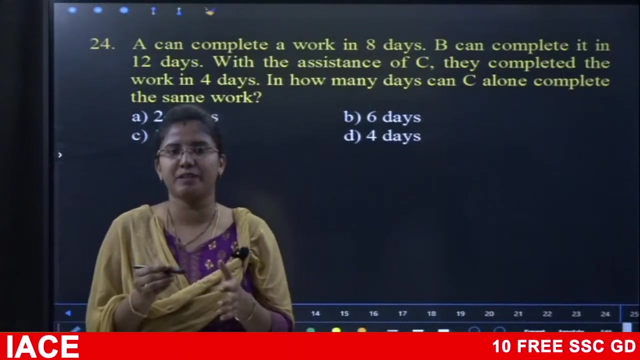 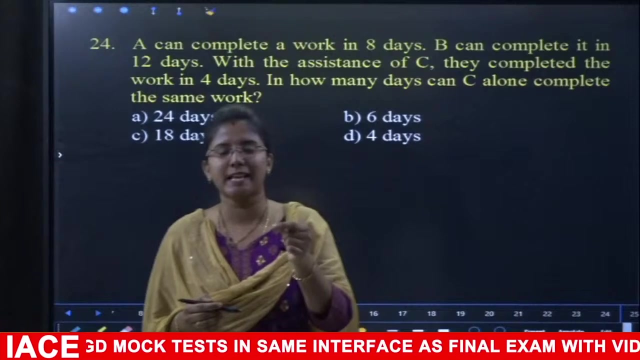 Ok, So I will remind you once again: Our IACE team, SSC GD Constable, is providing 10 free mock tests with video explanations. All the details related to that video are provided in the link description. Visit the link in the description once. These 10 free mock tests will help you a lot for the exam. 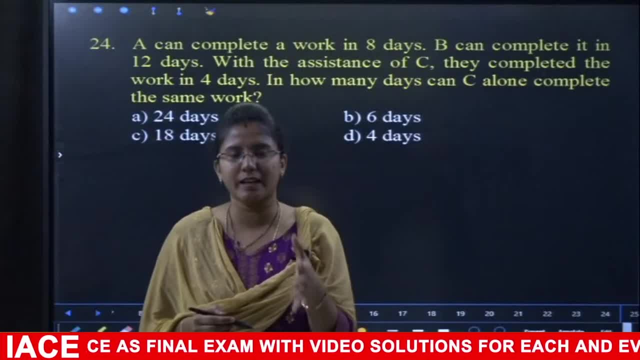 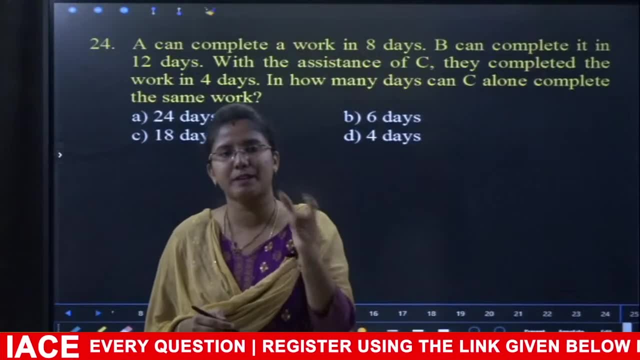 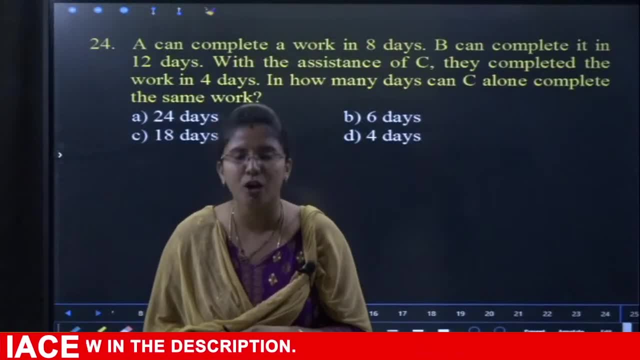 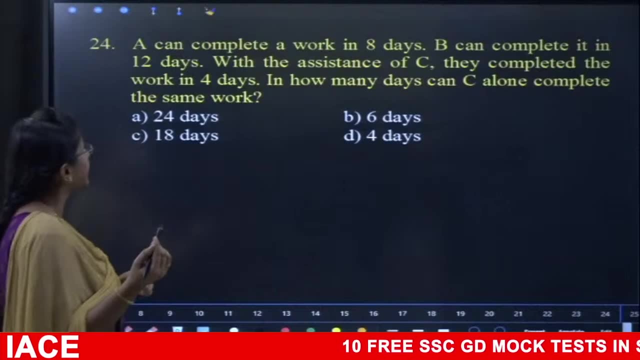 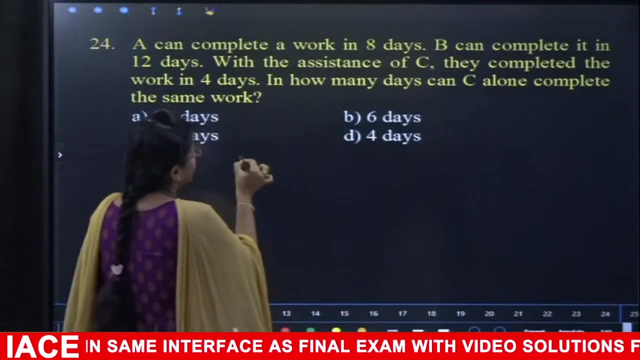 All the other details will be done in our team within 48 hours, So please utilize this opportunity. So next let us try this question. So did you answer it very easily? Ok, A can complete a work in 80 days and B can complete it in 12 days. 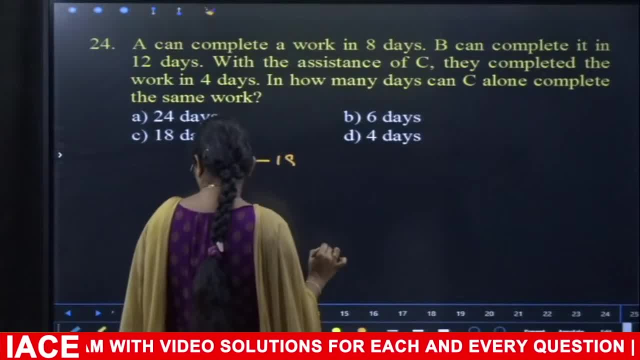 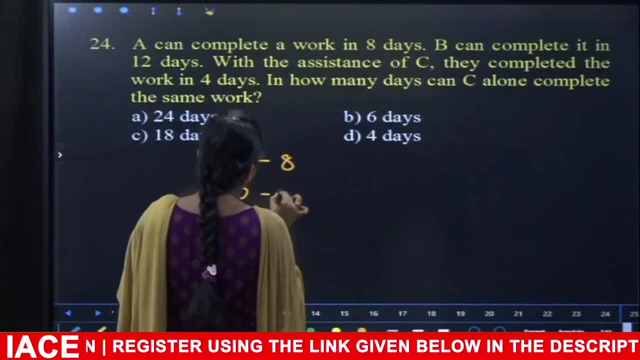 A can complete a task in 8 days. Ok, 8 days. Next, B can complete the same work in how many days? 12 days. It is saying How many days, 12 days. With the assistance of C, they completed the work in 4 days. 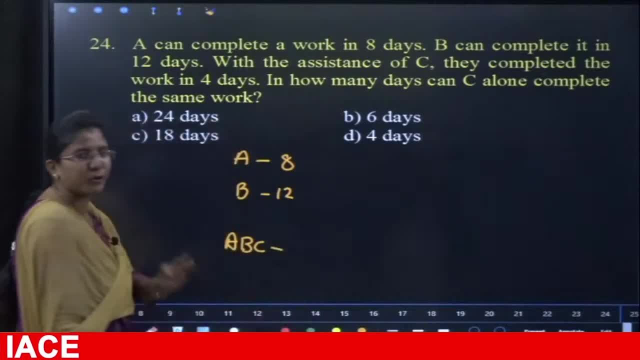 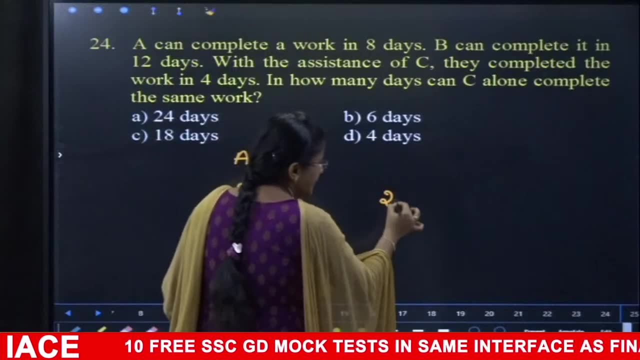 With the assistance of C A B, 2 took C help and 3 worked together. So A B C completed the work in how many days? 4 days, So 8 to 12, 4 multiple, just 24.. 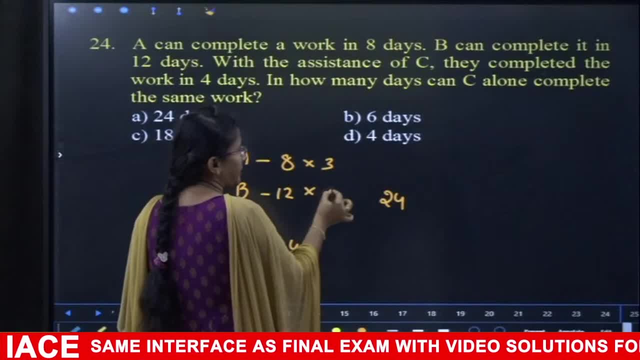 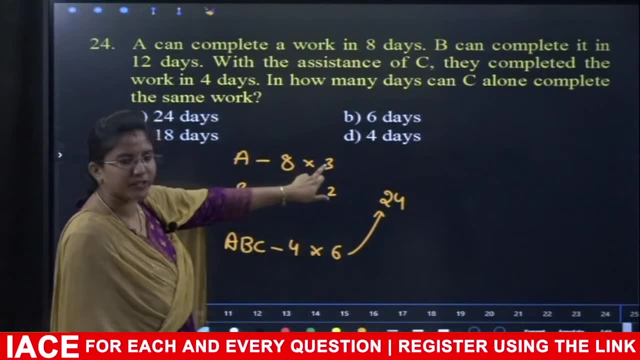 So if we take 24, efficiency of A becomes 3, B becomes 2, efficiency of A, B, C all together 4 to 24, how many times? 6 times. So if we take A, 3 units, B, 2 units, E, B, C, A B C, all together they completed 6.. 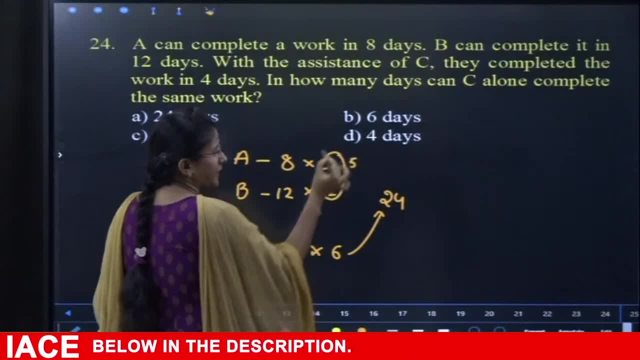 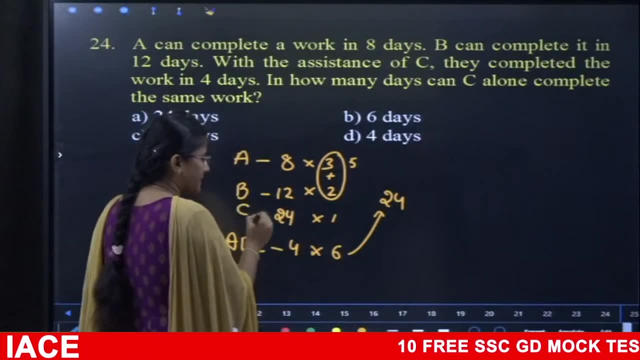 So in that A B work already we know 3 plus 2, how many 5.. If 5 units in 6, they completed C work will be 1 unit. Since they completed 1 unit in 1 day, 24 units should be completed. how many days will it take? 24, that is it. 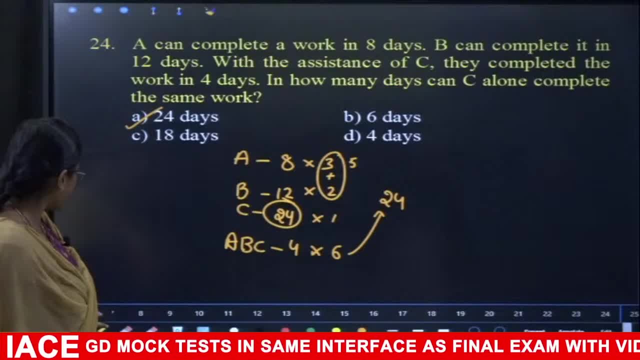 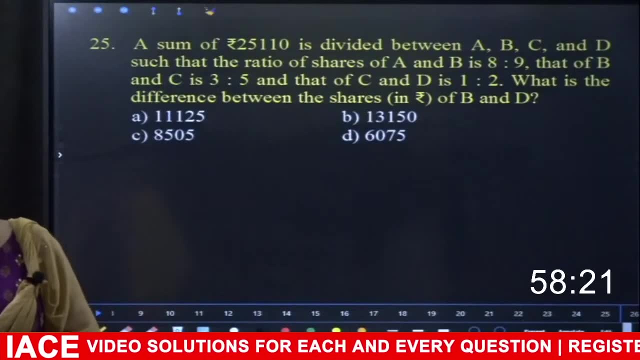 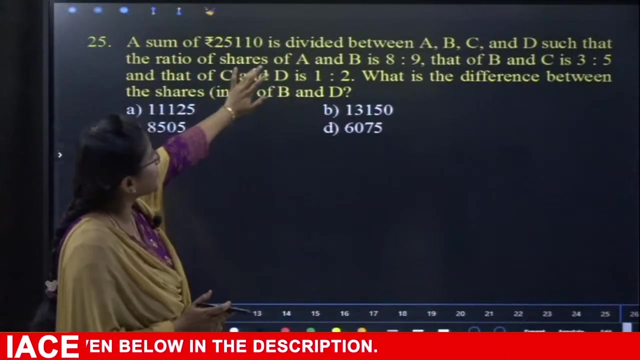 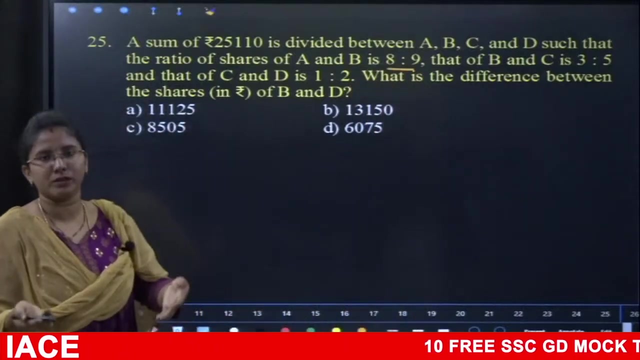 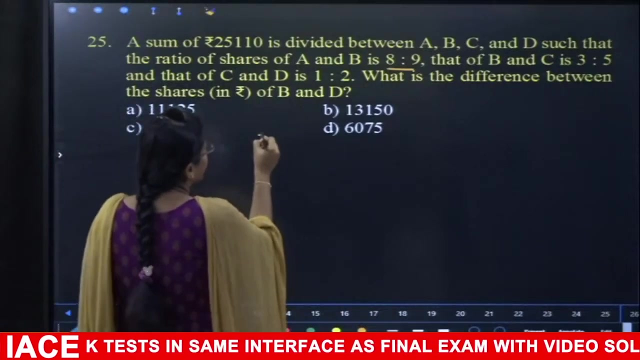 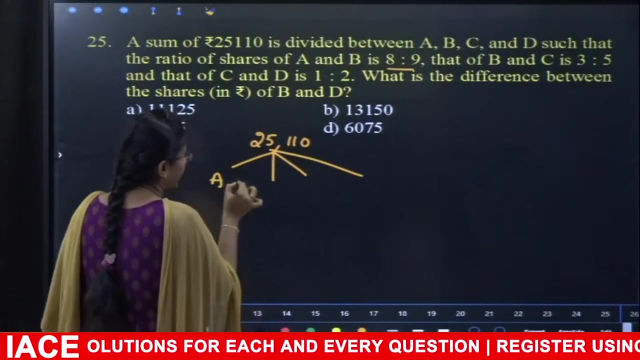 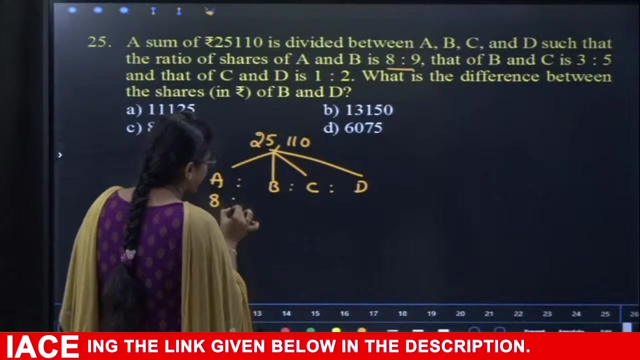 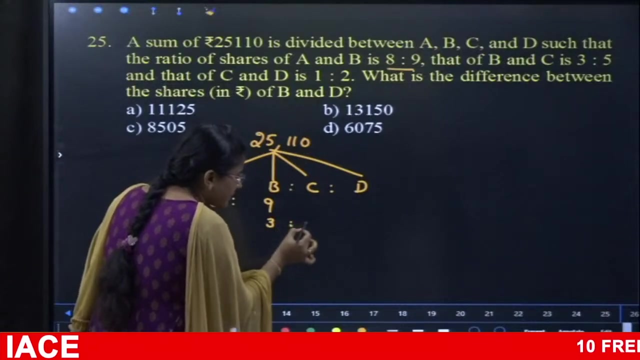 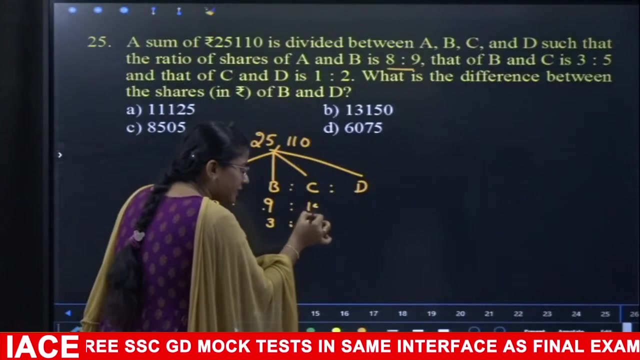 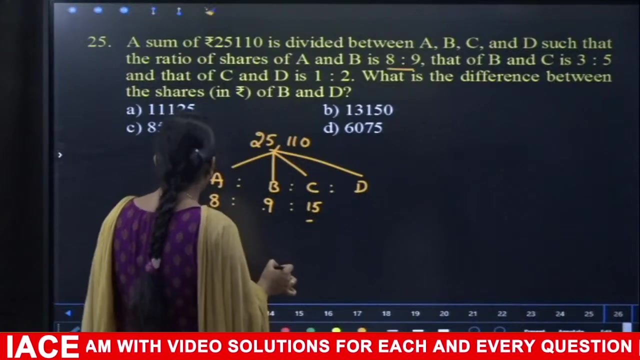 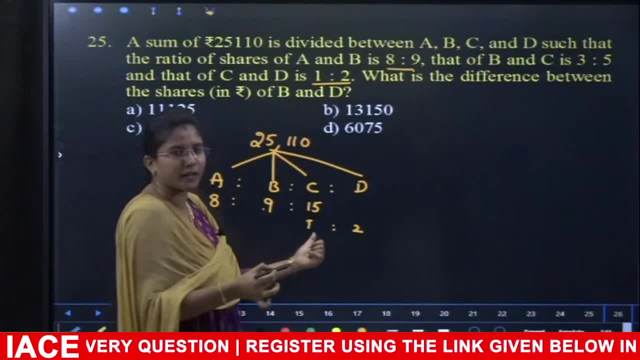 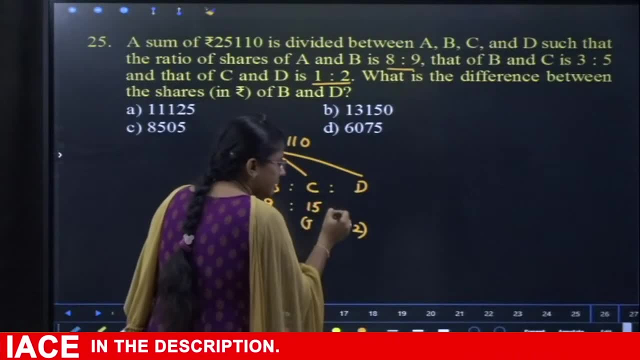 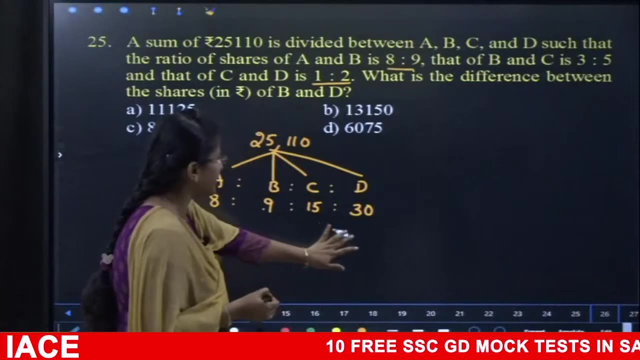 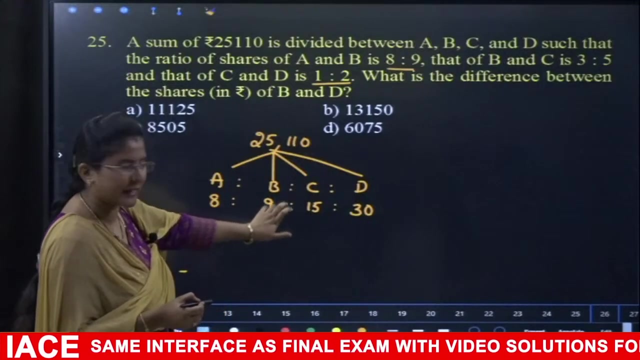 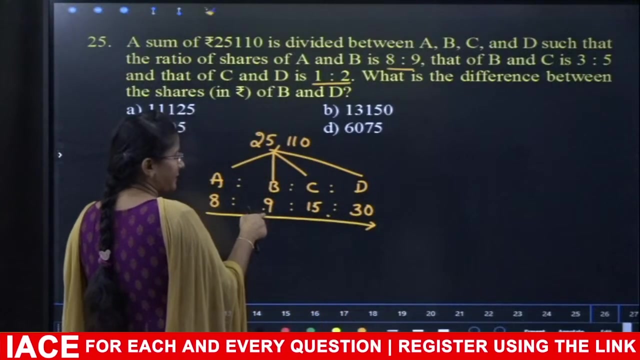 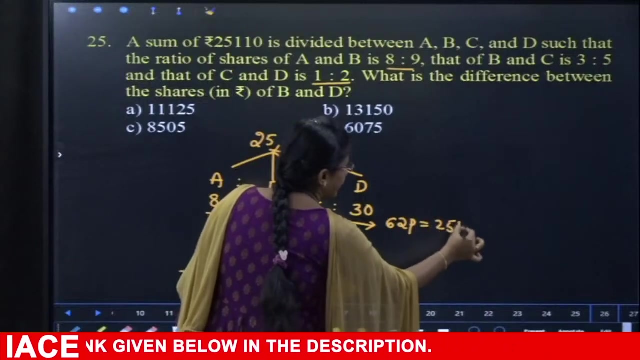 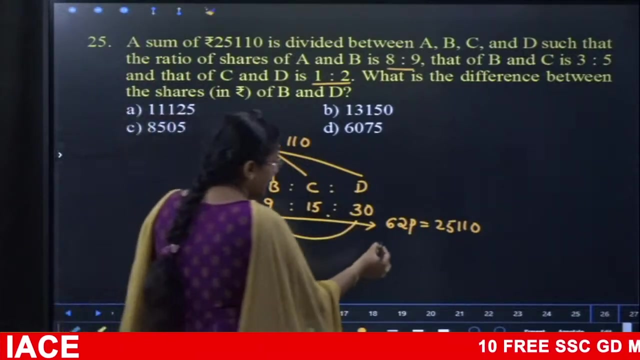 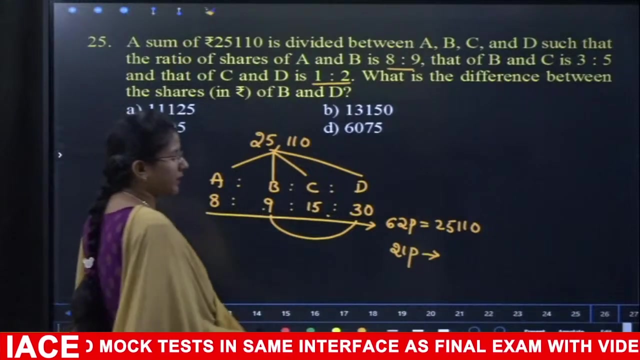 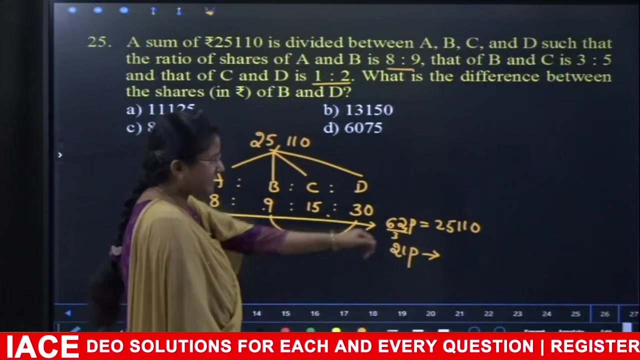 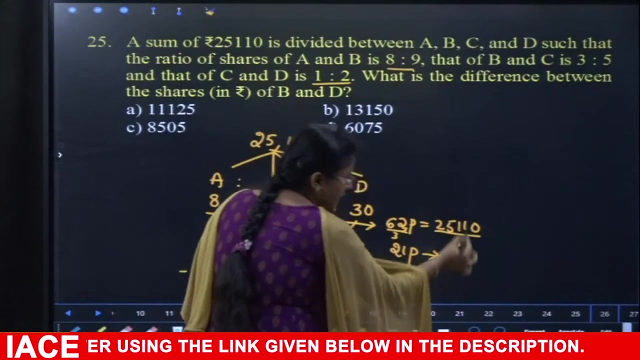 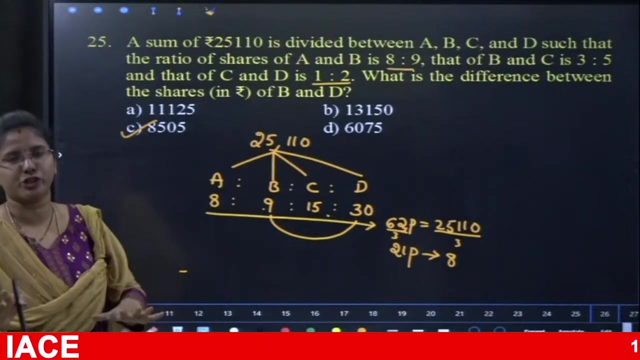 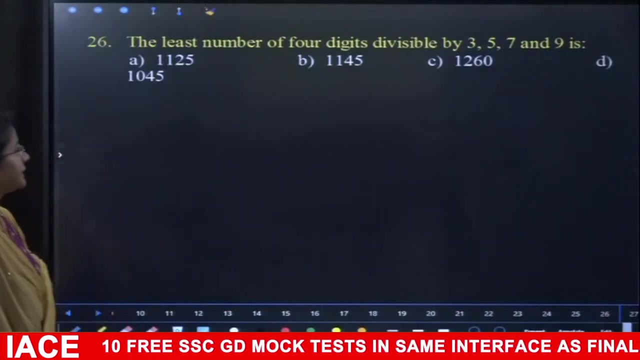 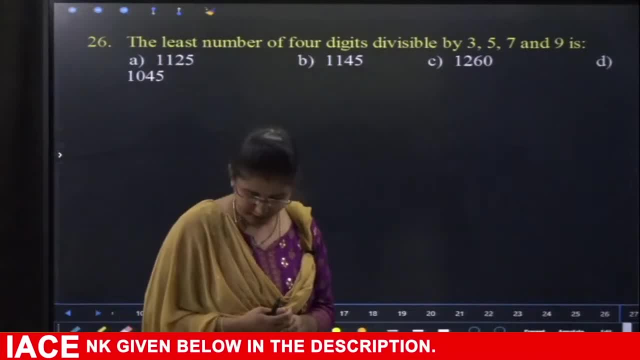 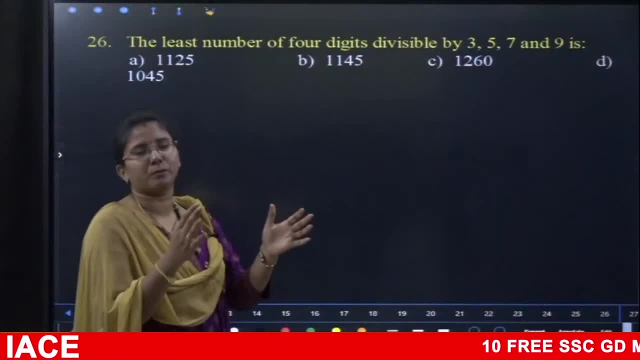 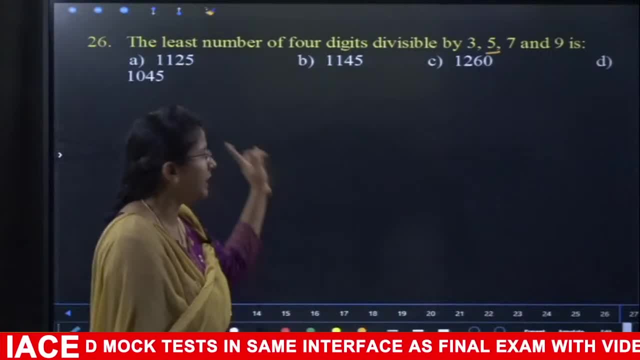 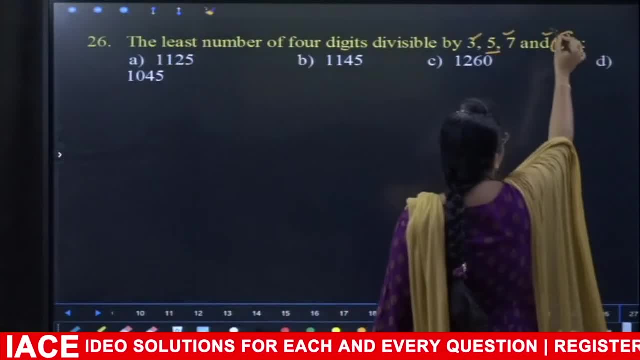 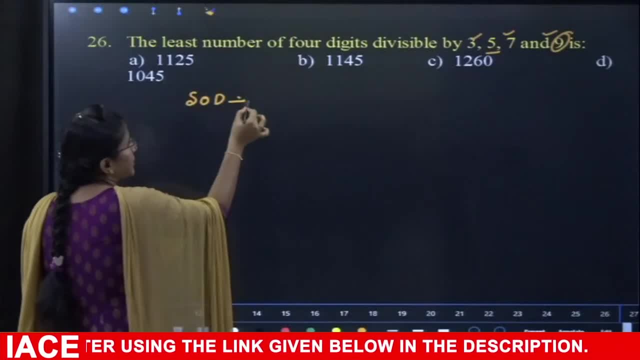 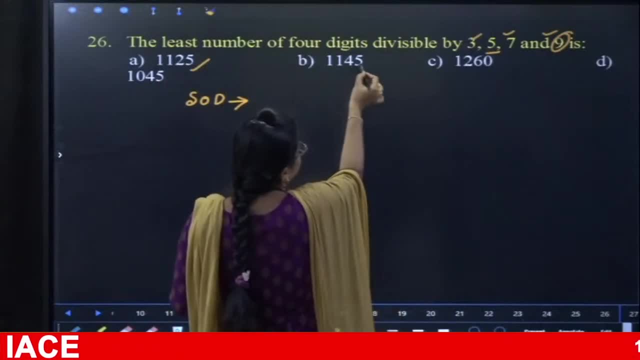 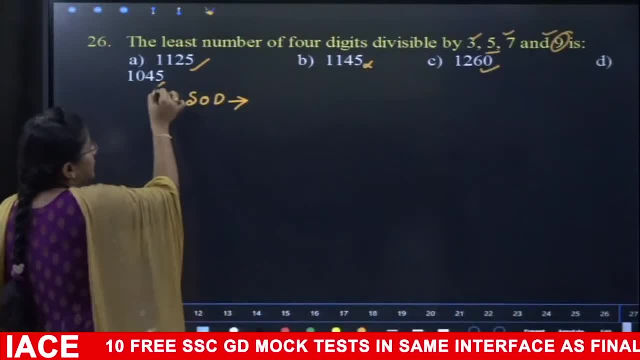 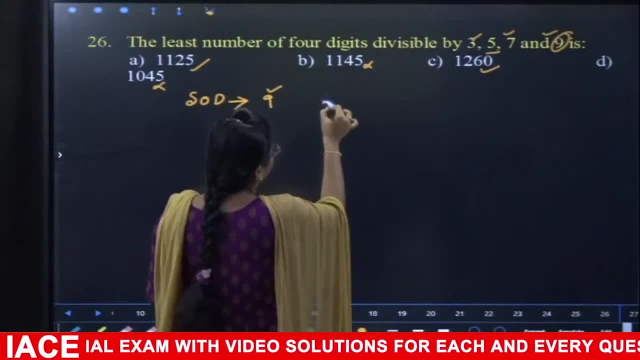 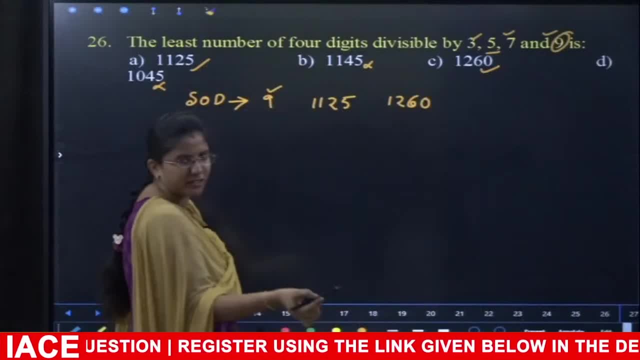 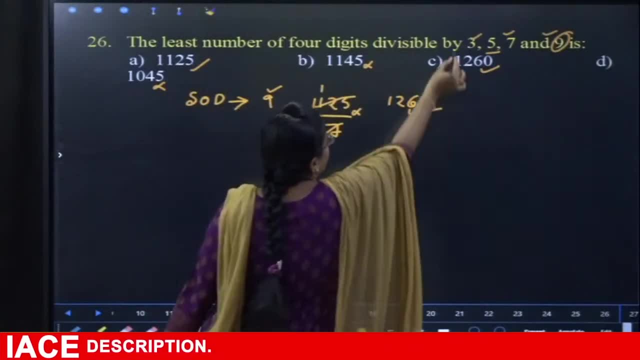 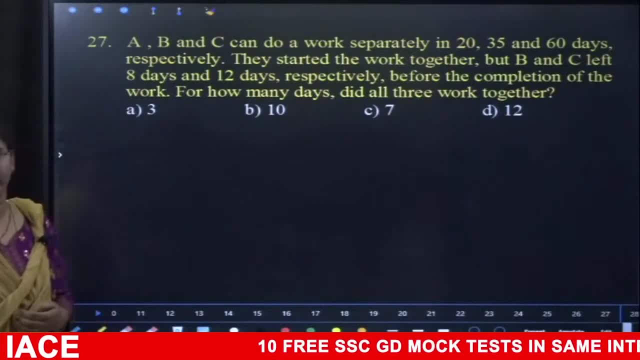 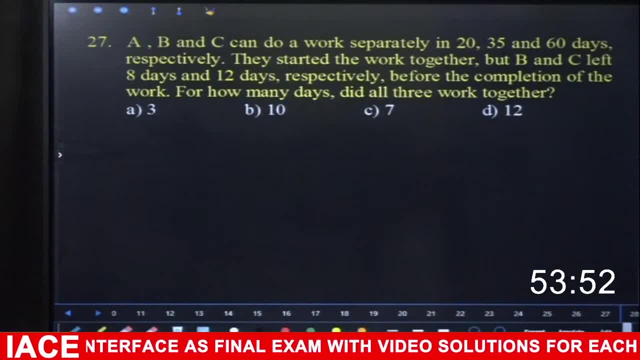 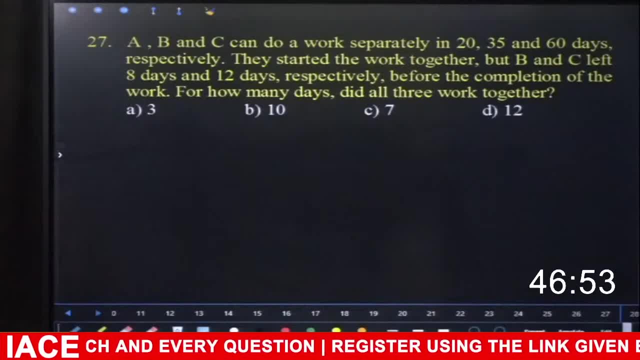 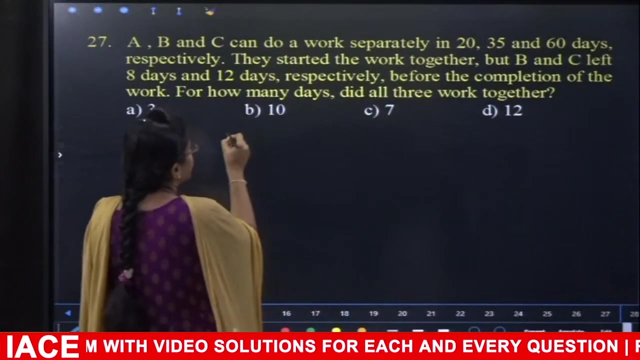 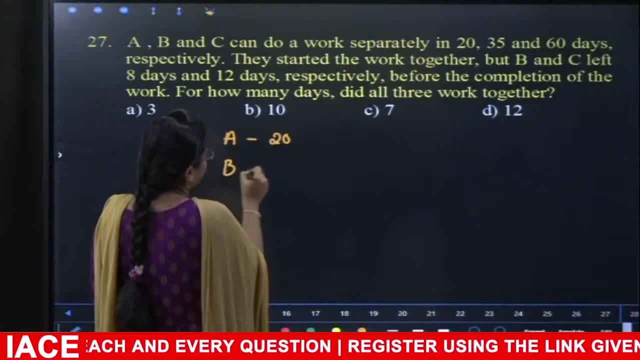 A can do a work in 20 days, B 30,, 5.. C can complete the same work in 60 days. First, in the total work LCM method, we choose LCM for 20,, 35 and 60.. 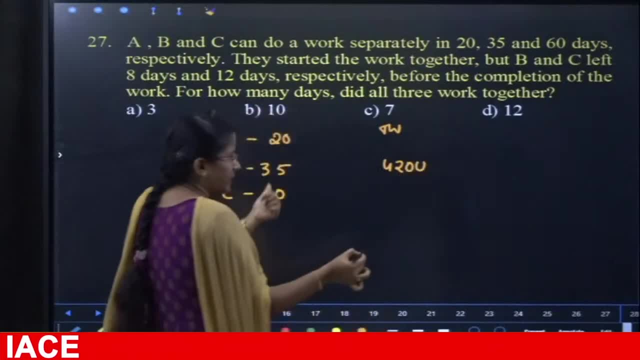 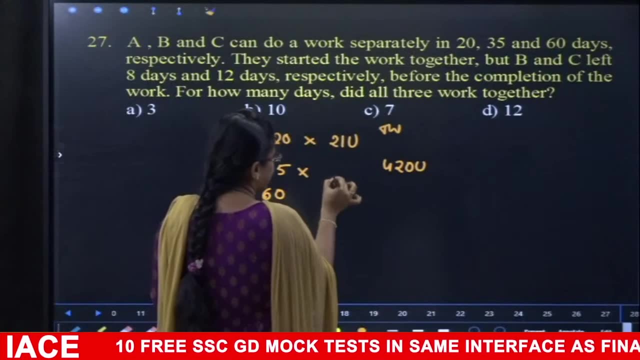 That is for 20 units LCM. It comes in all of them commonly, So 20 times 21 units. work is A, B, 35, 4, 20 will be 12 units. Next, 60 is 7 times. 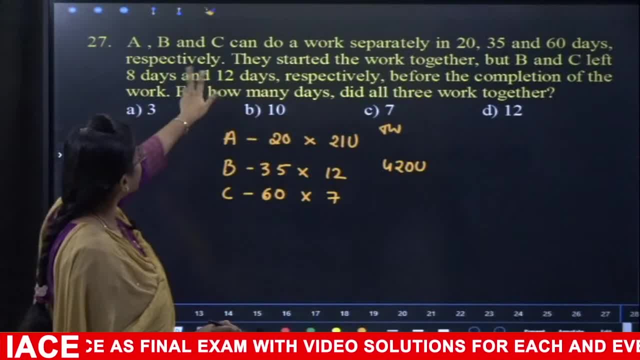 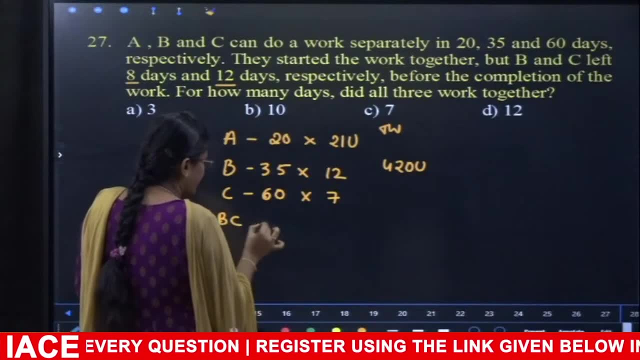 Efficiency is filled up. They started the work together, But B and C 8 days and 12 days respectively Before the completion of work. A, B, C, 3 of them started the work, But among them, 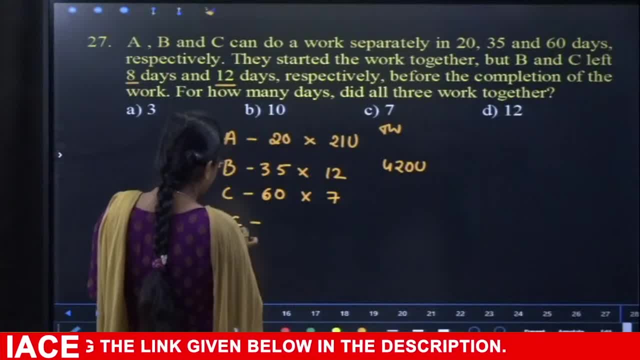 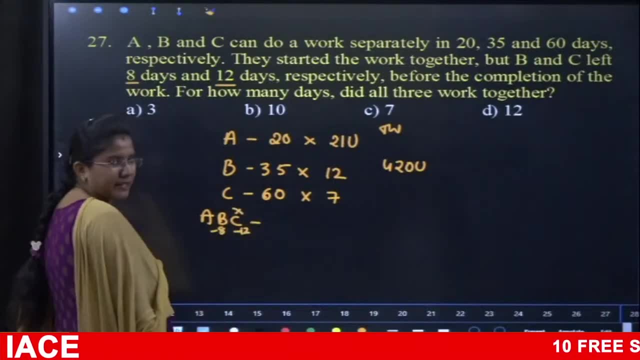 B left and exited after 8 days. C exited after 12 days. B 8 days before. C 12 days before. That means C is the first to exit. C left and A. B will work. B left 8 days before. 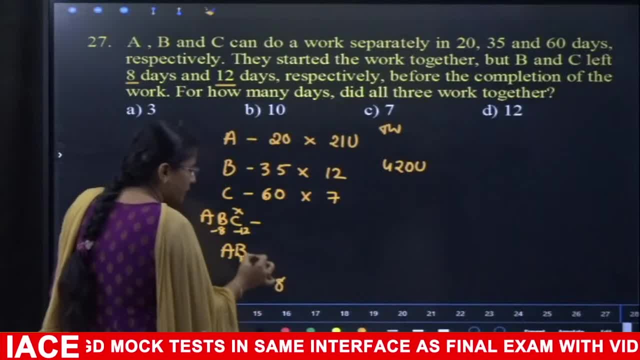 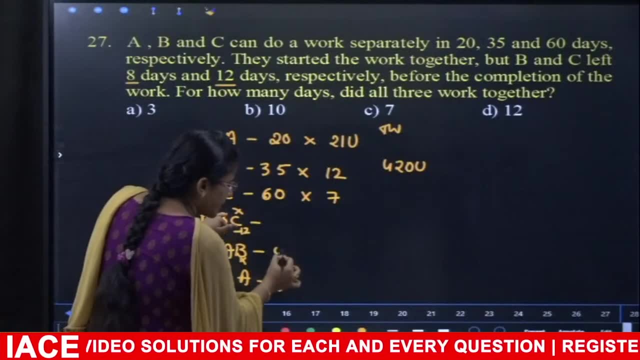 So B exited and A worked How many days before? All days work individually, So we wrote 8 first. In total, C left 12 days before, So here Already there are 8 days. A, B worked for remaining 4 days. 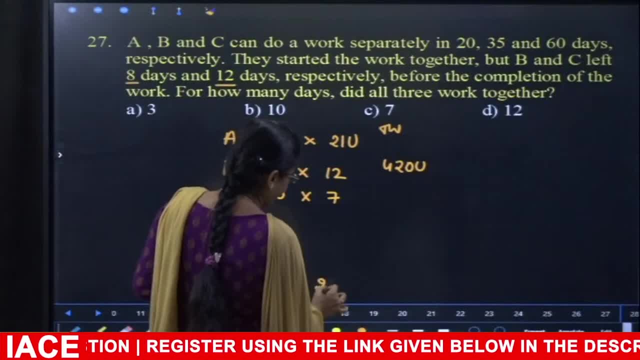 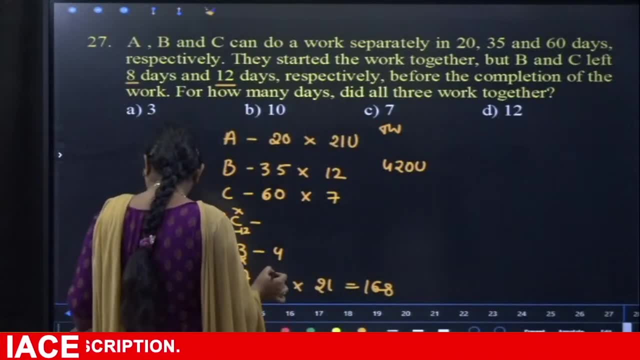 So let's fill the efficiencies. A will be 21.. 8 x 21, 168 units completed out of 420.. Next, if A- B works 2 times, If A B works 2 times 21 plus 12, total work is 33.. 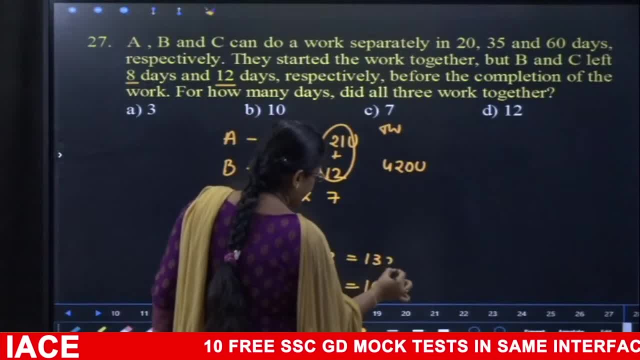 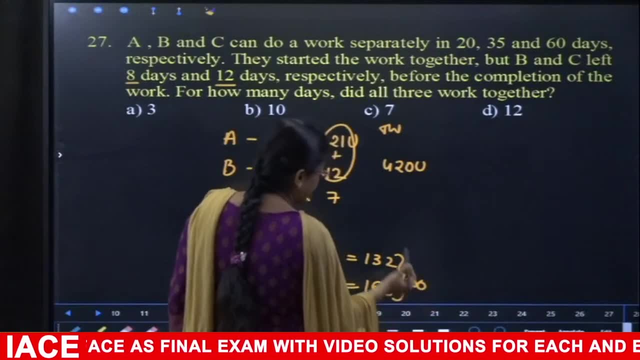 4 x 33,, that is 132.. So 132 and 168.. Total work will be 300 units completed, 300.. In 420, 300.. So here what we will see is: In 420, 300 units completed. 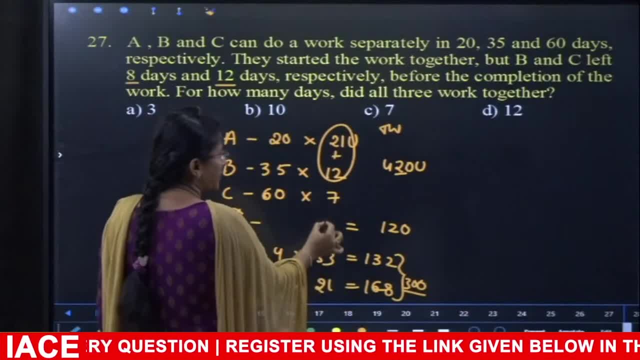 If A? B works for remaining 3 days, B will work for 120.. If A? B works for remaining 3 days, 33 plus 7, total. how much work will it take? 40 for 1 day. 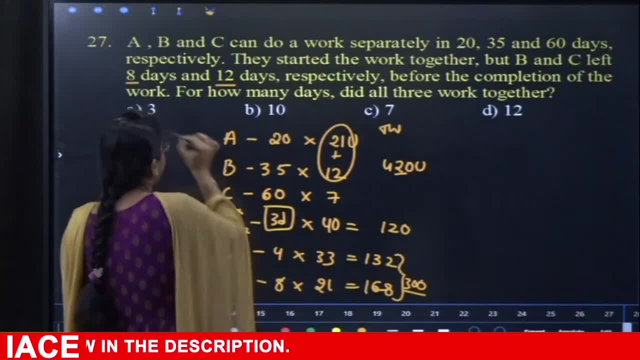 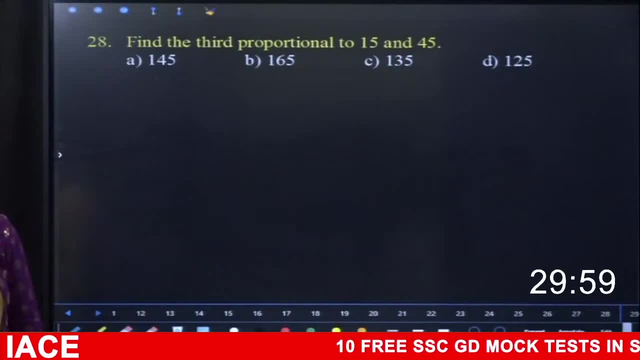 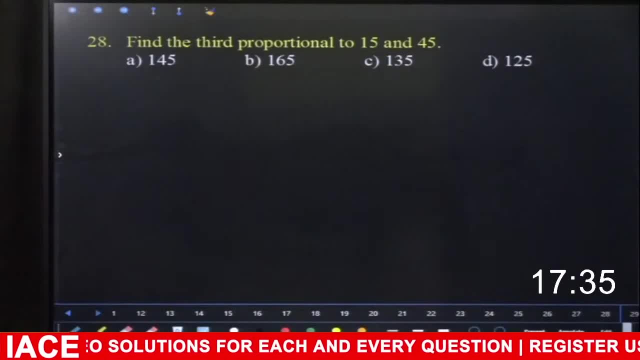 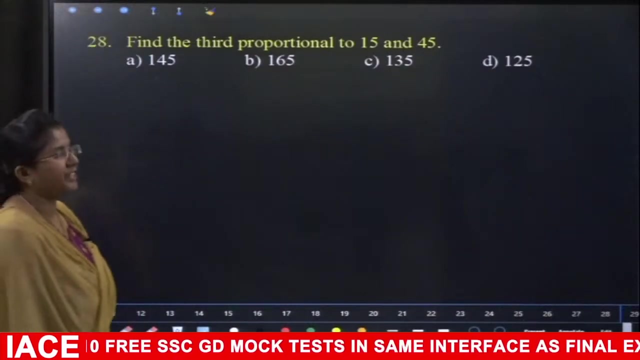 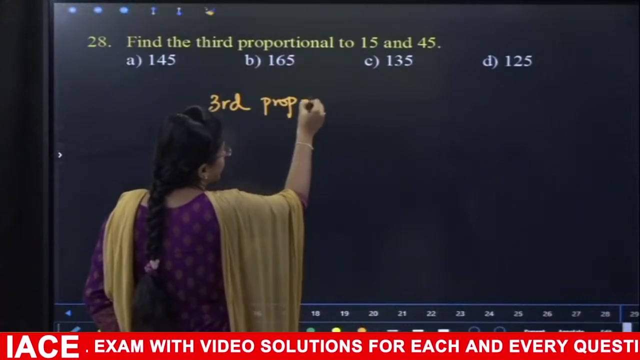 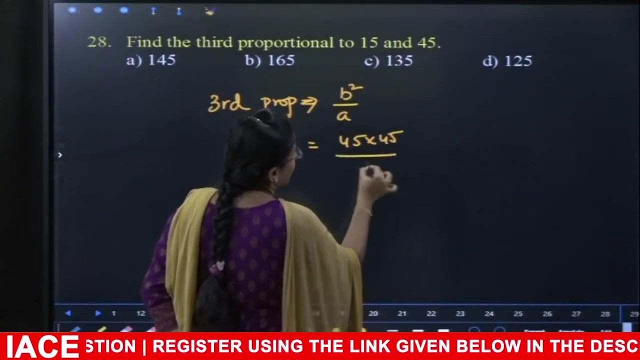 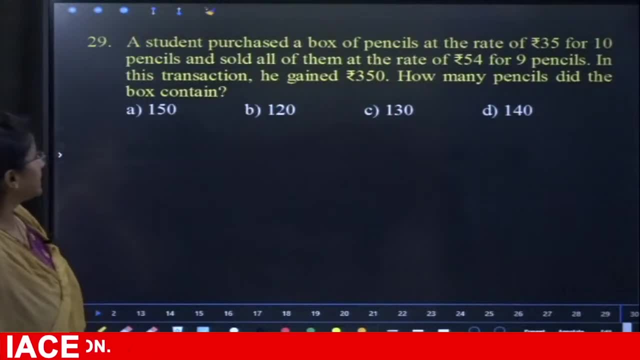 option c: okay, next 29. so equation: try 30 seconds time. oh please, easy. equation: 30 seconds time: oh please, okay, so your time is up. next, a student purchased a box of pencils at the rate of 35 rupees for 10 pencils, and so on. 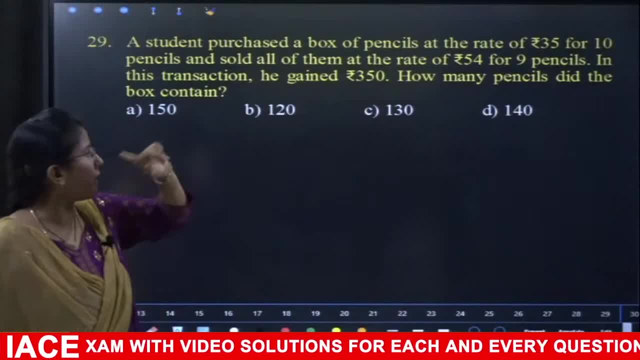 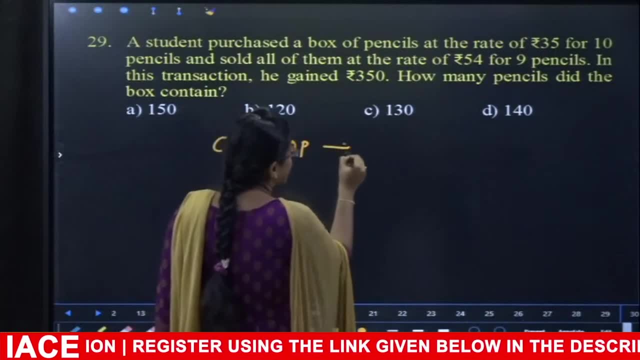 ok, so your time is up. next, a student purchased a box of pencils at the rate of 35 rupees for 10 pencils, and so on. He sold all of them at the rate of 54 for 9 pencils. He bought at the cost price of 10 pencils for 35 rupees. 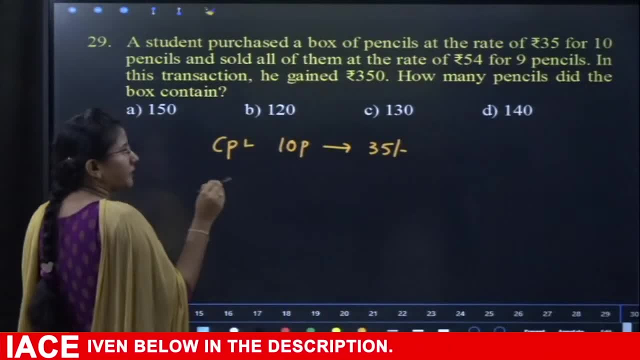 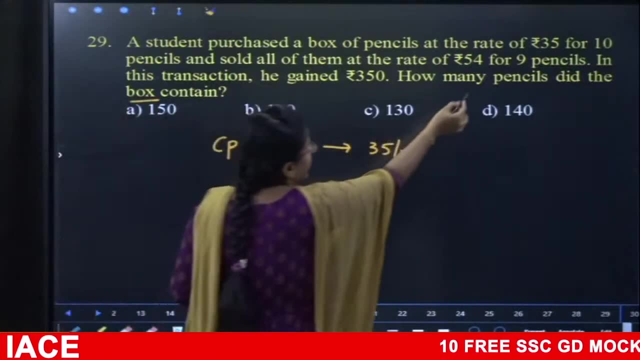 Next, he sold all of them, for 10 pencils for 35 rupees. He didn't tell how many pencils. He asked the same question: How many pencils does the box contain? He asked how many pencils are there in the box. He sold all of them at the cost of 10 pencils for 35 rupees. 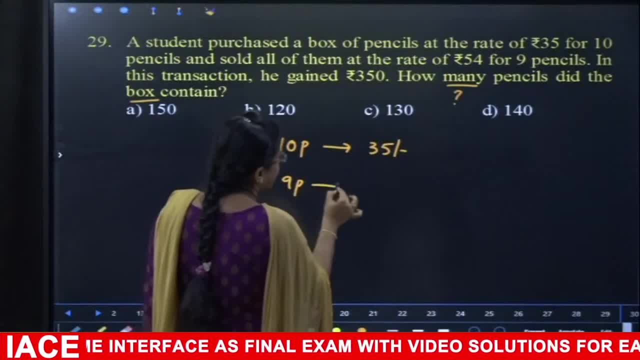 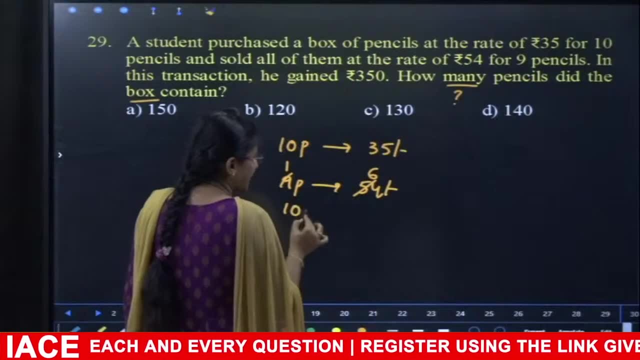 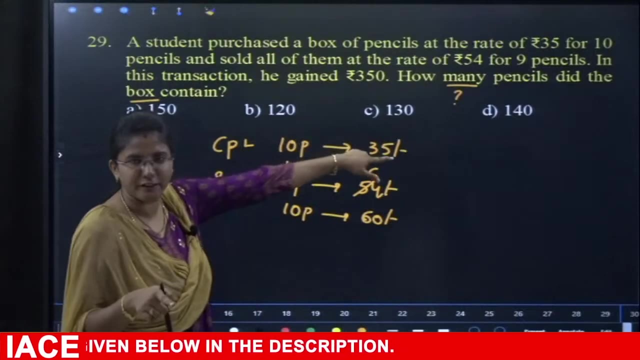 He sold all of them at the cost of 54 for 9 pencils. Each pencil will cost 6 rupees. How many pencils will cost 10 pencils for 60 rupees? He bought 10 pencils for 35 rupees. He sold 10 pencils for 60 rupees. 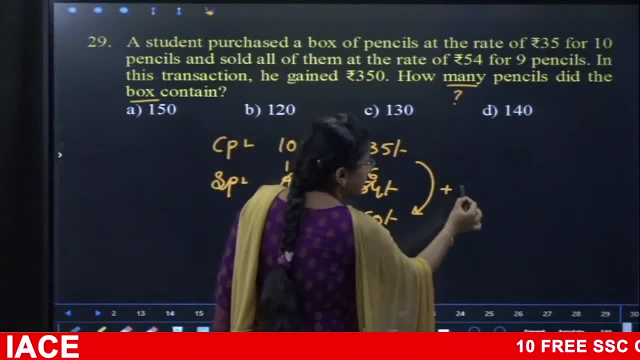 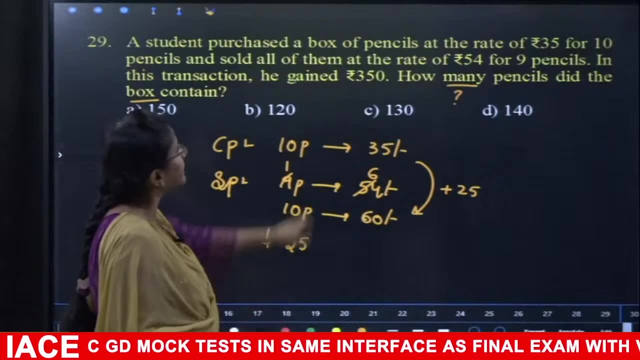 He got 25 for 10 pencils. If I take the number of pencils as 10, I got profit as 25.. How much profit should I get? He gained 350.. How many times should I get 350?? How many times should I get 25 and 350?? 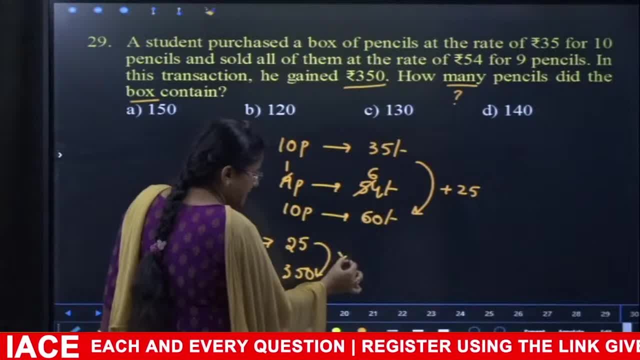 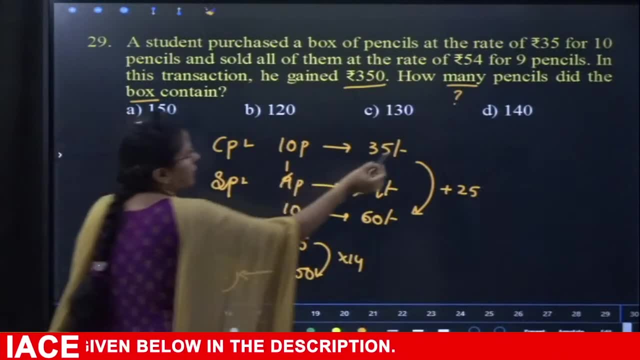 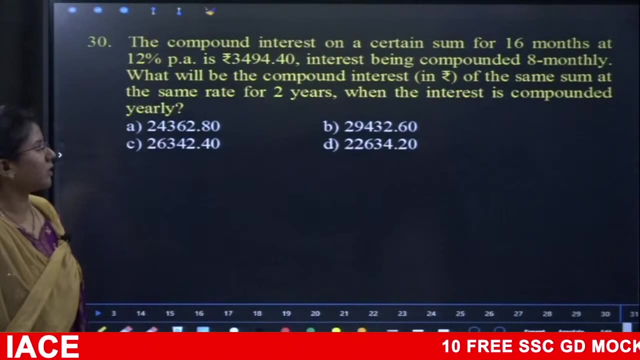 10 times 250 is 14 times, So the answer is 10 for 14.. 140 pencils are there for a box. Very easy question. Answer option D. Next one Go for 30. This is a compound interest problem. 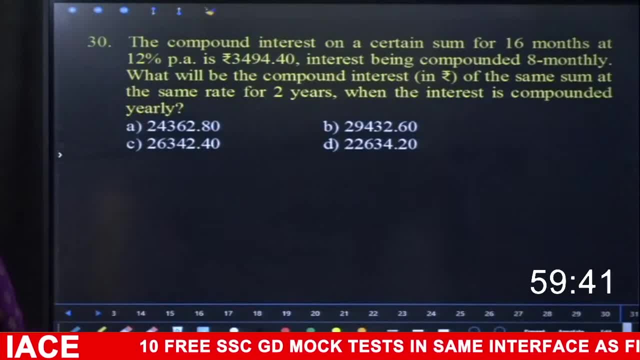 Try it. 1 minute timer please. One minute timer please. How many pencils are there? 10., 30., 3., 4., 5., 6., 7., 8., 9., 10., 10.. 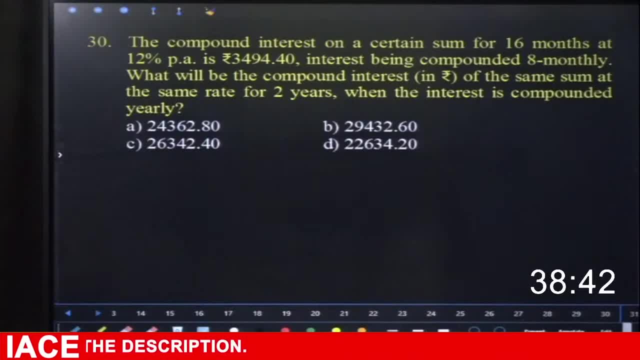 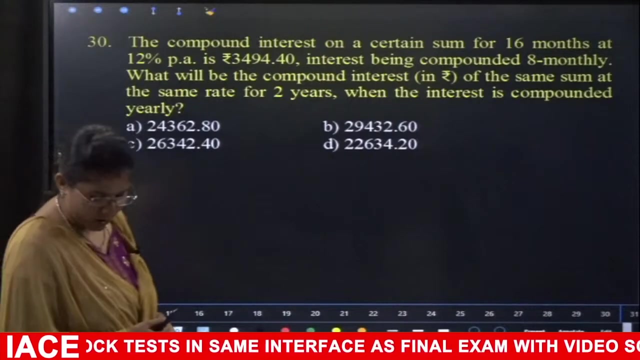 10., 11., 11., 11., 12., 13., 14., 15., 16. 17.. Okay, so this is the compound interest problem, a bit calculated, but we can sort this problem with the unit result. 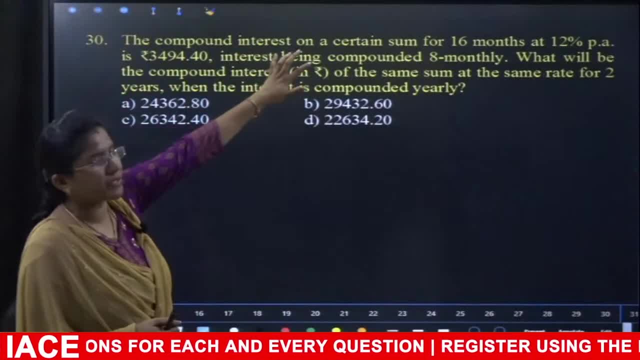 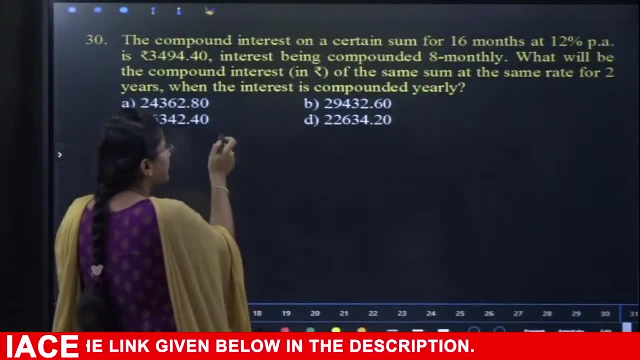 See: the compound interest on a certain sum for 16 months at 12% per annum is 3494.4,, interest being compounded 8 monthly. So, compared to the time period given, he calculated the interest for 16 months at the rate of 12% for 1 year. 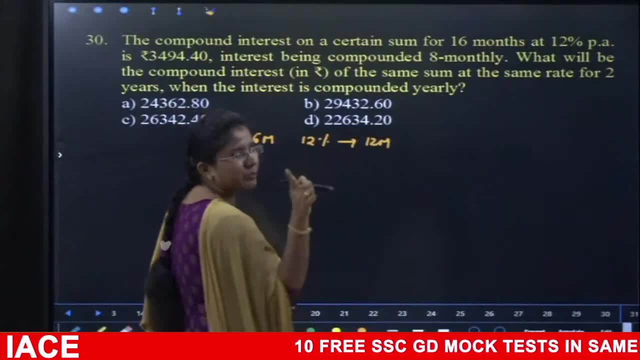 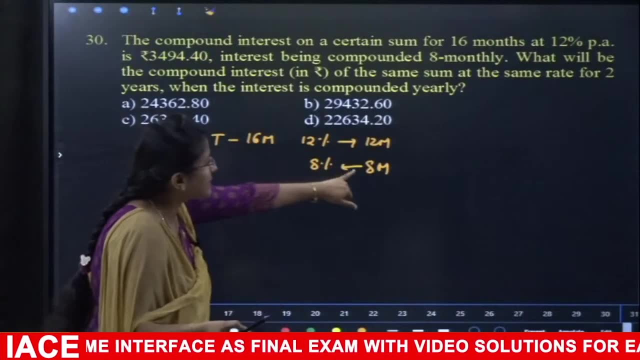 1 year means 12 months, 12% for 12 months and 1% for 1 month. So if compound interest is taken for 8 months, the rate of interest will be 8% itself. Similarly, if we calculate 8% for 8 months, we get 3494 rupees for 16 months of compound interest. 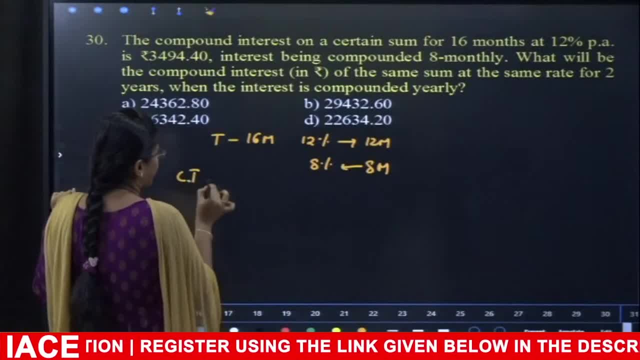 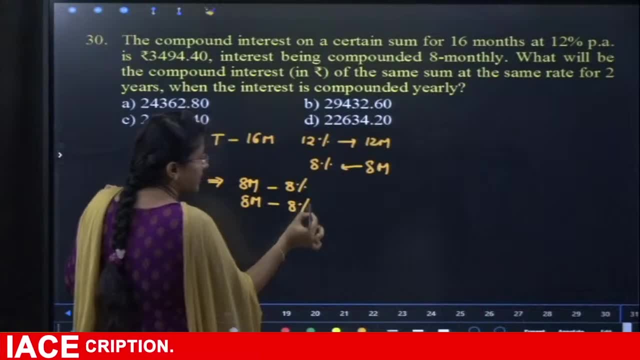 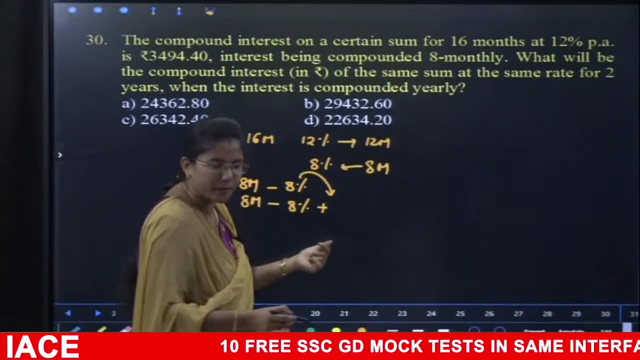 So it amounts to. so total compound interest is there For 16 months, first 8 months and second 8 months. first we pay 8% on the principal. second also we pay 8% for 8 months. Let us again write: 8% on the first interest, 8864,. percentage is by 100, that will be 0.64. 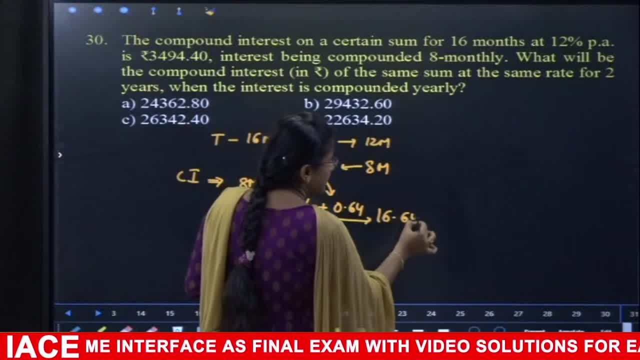 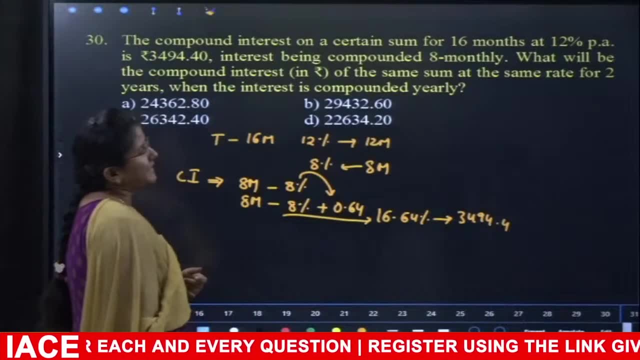 So overall the compound interest here is 16.64% value given in the question, What he gave is 3494.4.. Next, what will be the compound interest on the same sum at same rate for 2 years. Interest compounded this time is yearly. 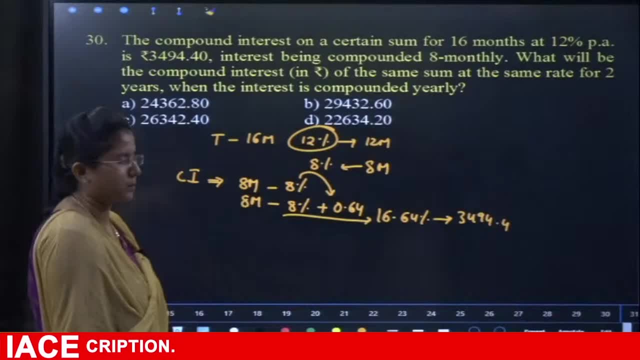 Since it is yearly, we will take 12% as usual. So 12% is there. So if we take 12% on the first year, 12% on the second year and 12% on this again, 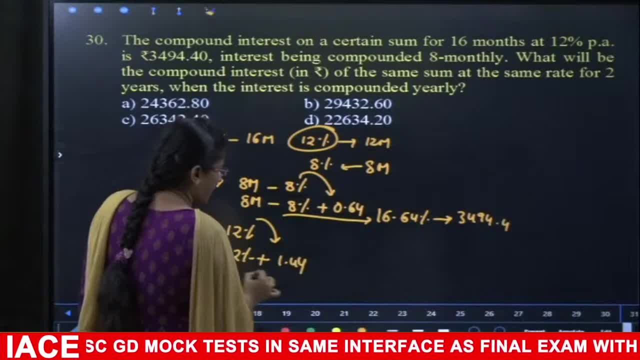 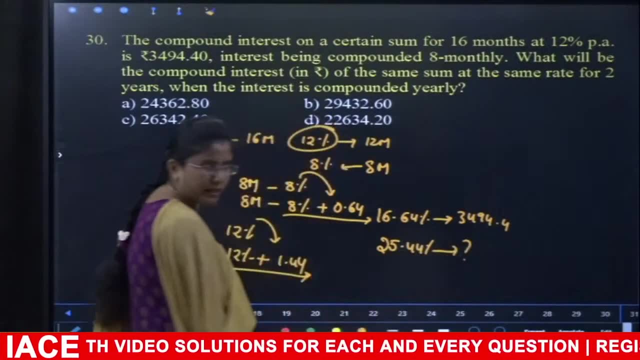 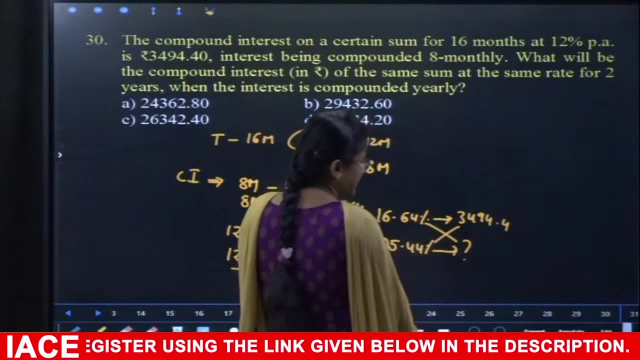 144 by 100, 1.44.. The overall interest there is 25.44 percentage value. We have to find out and answer it. So let us do the complete calculation. The numbers are very lengthy Since our calculation takes a lot of time. when we multiply these two, we will get 4 and 4.. 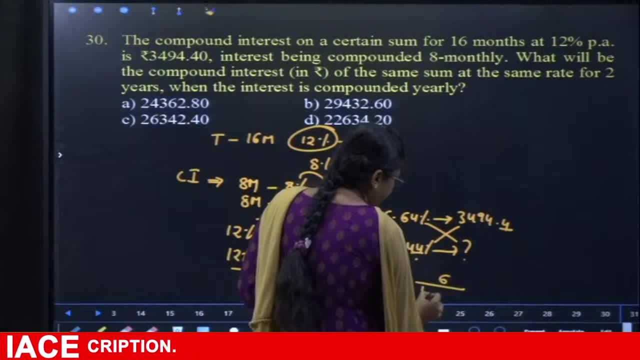 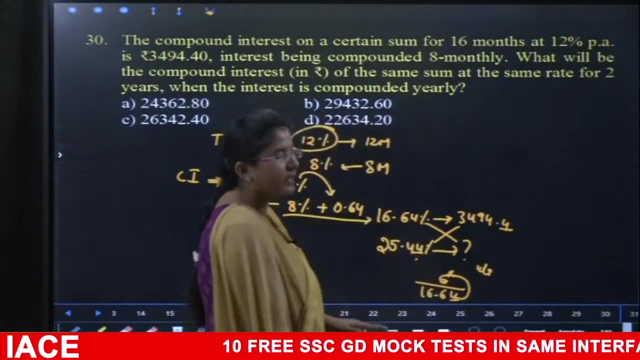 Unit digit as 6 in the numerator. In the denominator we have 16.64.4.. When 4 and 6 are cancelled, there should be either 4 or 9 unit digit. Since there is no 9, the option is here: 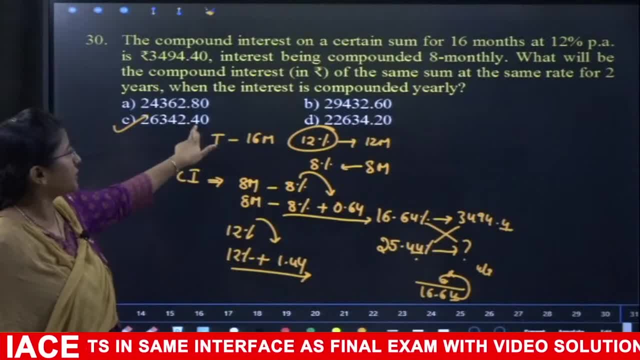 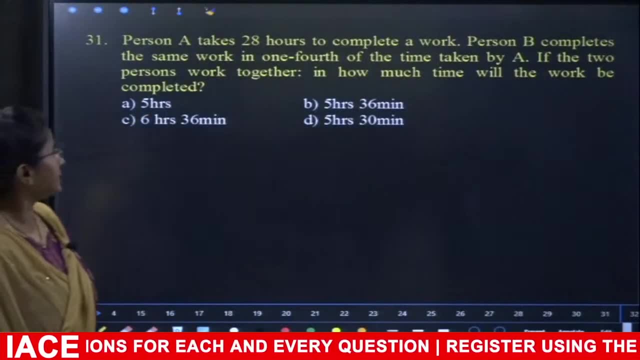 26342.4.. Unit digit is 4.. We have to calculate and answer it. Okay, Next, Next, 31. Try, 31.. Very easy question. 30 seconds time please. 30 seconds time please. 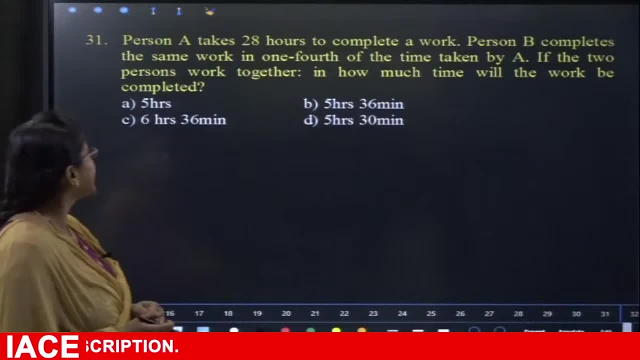 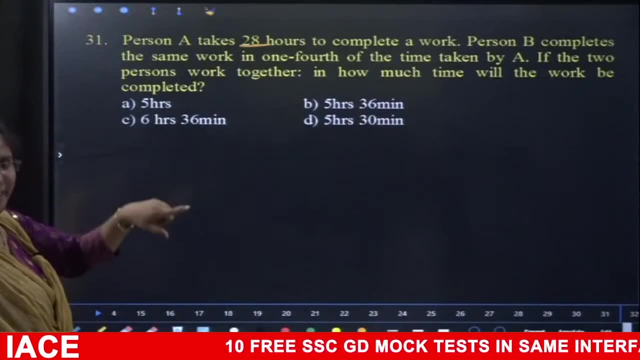 Okay, So time and work means equation Very easy. Let us solve it. Person A takes 28 hours to complete the work And B completes the same work in one-fourth time, taken by A. So A completes the work in n hours. 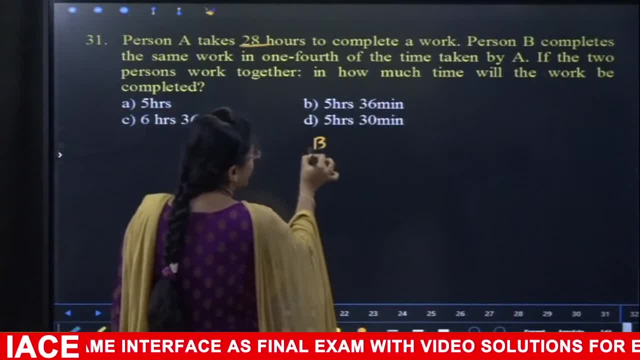 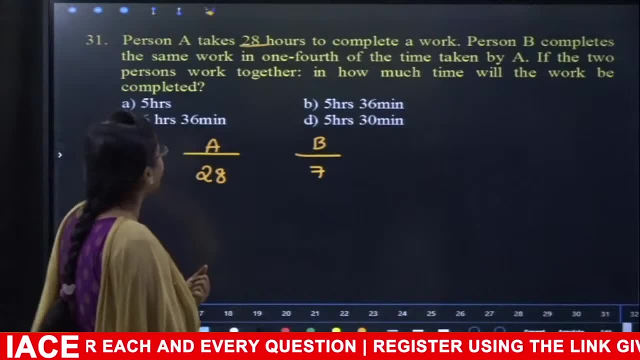 That means she completes the work in 20 hours. To complete B's work, she takes one-fourth time in this. That means 28 by 4.. How many hours? 7 hours? Question is: if two persons work together, in how much time the work will be completed? 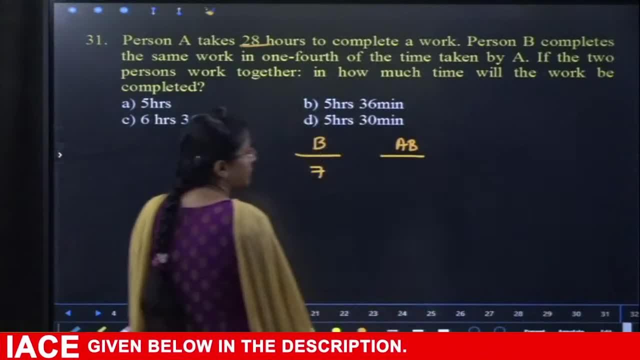 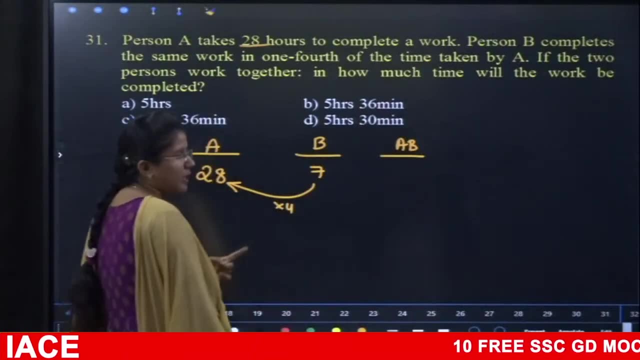 If A and B work together, how much time will the work be completed? So 7 by 28.. These two are direct multiples: 7 and 28.. 7 and 28.. How many times are there? There are four times. 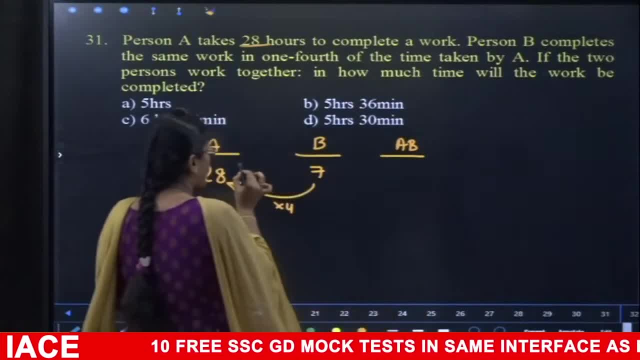 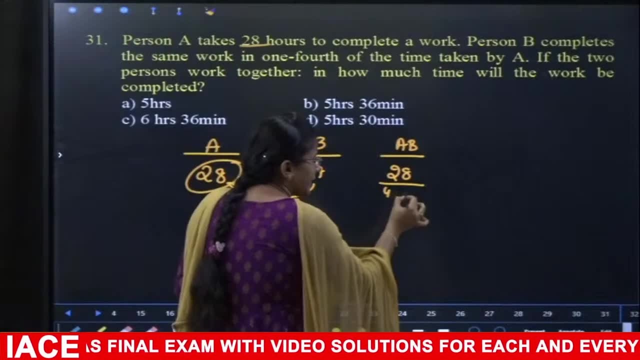 So if two persons work together, in how many days will they complete the work? Number of time, days taken. who takes more? We will write that 28.. How many times are there? There are four times, So you have to write in denominator. 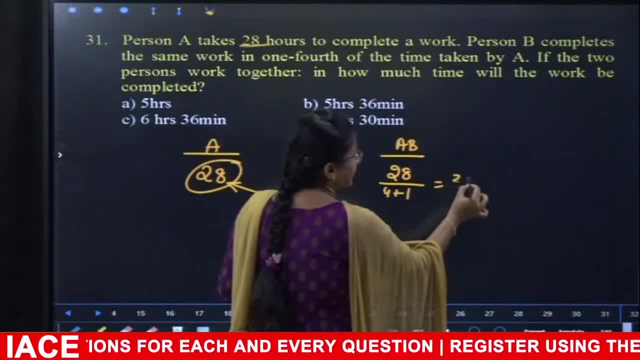 You have to write plus 1.. How many times are there? There is plus 1 for that. Answer is 28 by 5.. 28 by 5 will be how many hours? 5 hours will definitely come Next. 3 by 5 will be there. 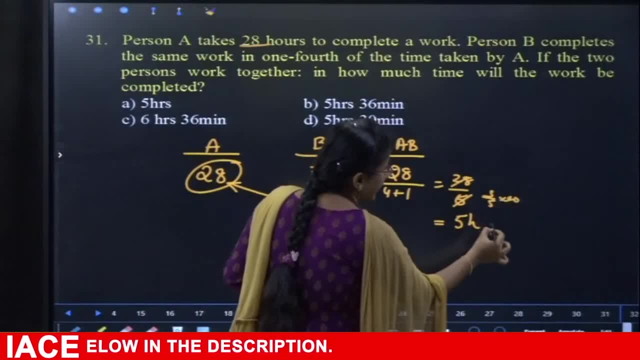 3 by 5 of 60 will be how much? 45.. 5 hours, 45 minutes. That is Wait, wait. 3 by 5.. 3 by 5 into 60.. 36 hours, 36 hours. 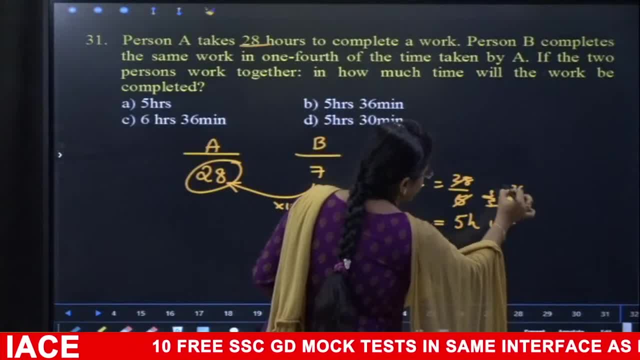 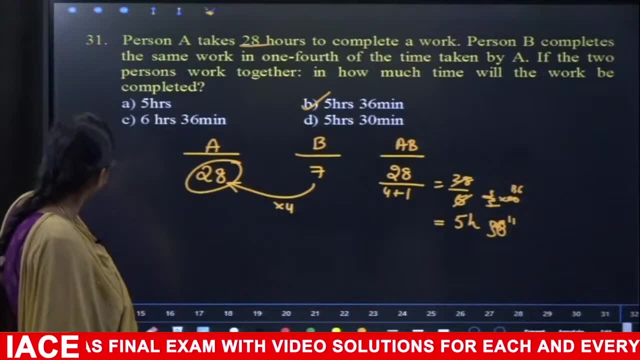 12 comes 36.. 3 hours, 5 hours, 36 minutes. Option B: Okay, Next 32.. Try it. The equation is also very easy. Time is 30 seconds, Please. Time is 30 seconds. 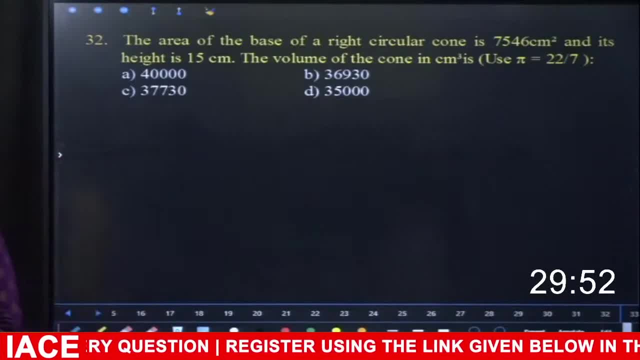 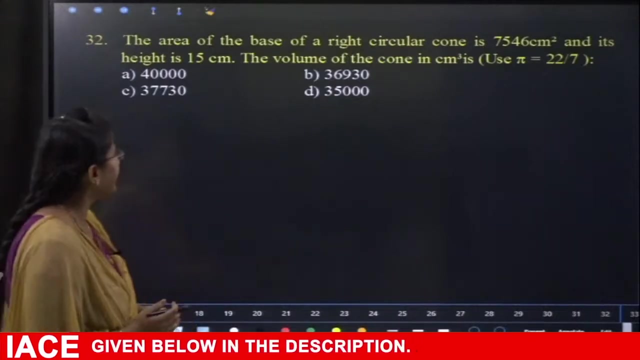 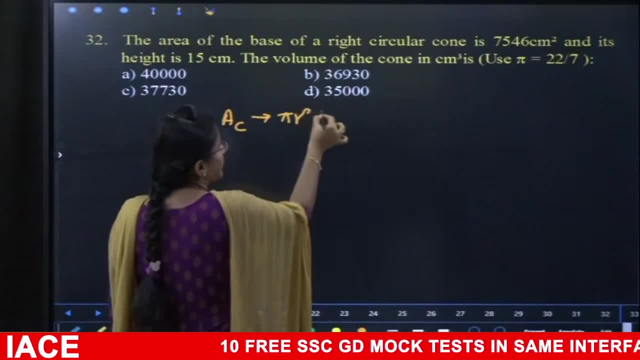 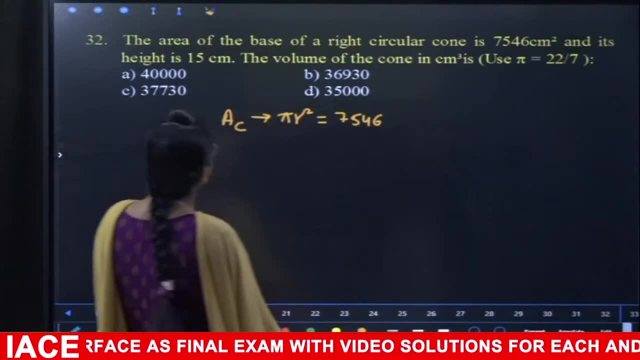 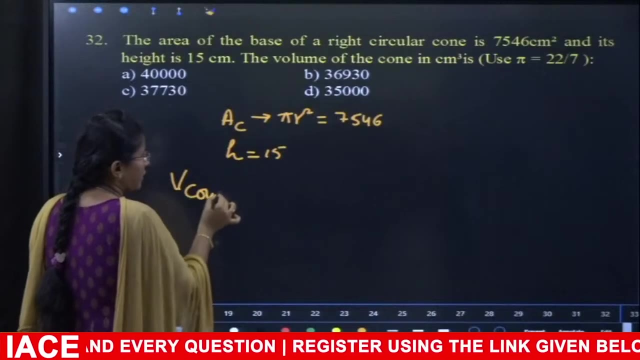 of base means circle. Since it is circular area is pi r square, given 7546.. Next, its height is 15 centimeters. Height is 15 inches. What is the volume of the cone He is asking? So nothing is there, Just multiplication Volume of cone formula is enough. What is it? Yes, 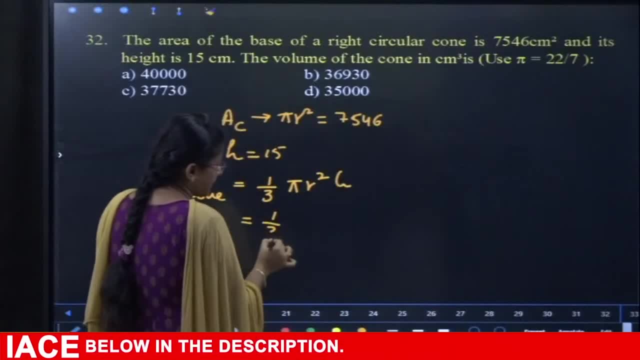 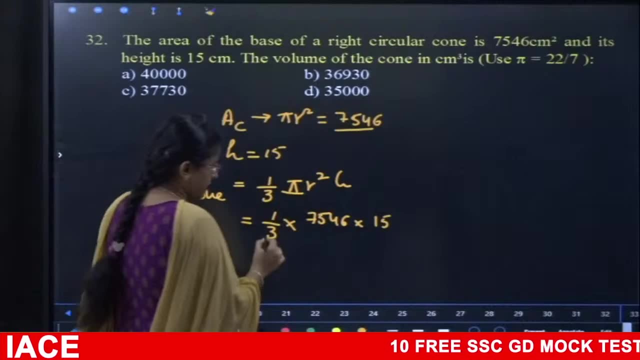 one-third pi r square h. So already given values are one-third. Let us keep it like that. What is the value of pi r square 7546.. Next height already given is 15.. So 315.. This 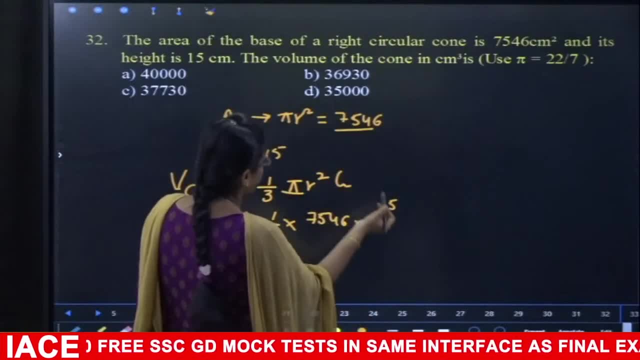 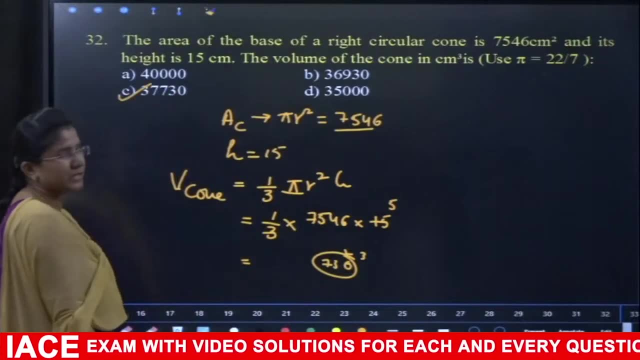 will be 5 times gets cancelled. And next unit: desert. For us, 3, 5 is 30.. 3, 5, 4 is 20.. 2, 27.. There will be 730.. There is only one option of 730.. 3, 7, 7, 3, 0. answer Okay. 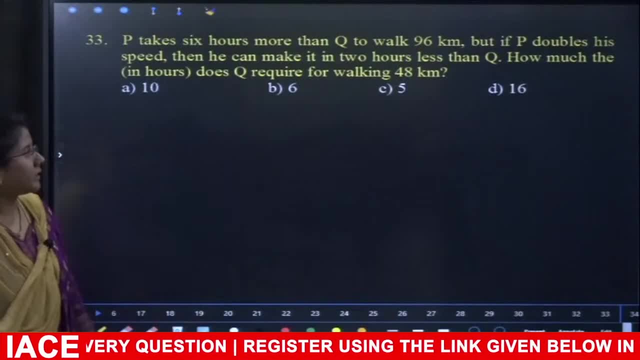 Next 33.. Try the next equation: One minute timer please. 1,, 2,, 3,, 4,, 5,, 6,, 7,, 8,, 9,, 10,, 11,, 12,, 13,, 14,, 15,, 16,, 17,, 18,, 19,, 20,, 21,, 22,, 23,, 24,, 25,. 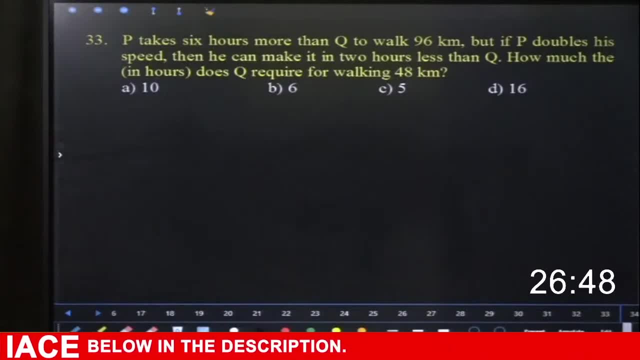 27,, 28,, 30,, 39,, 31, 32.. Okay, your time is up. So equation time and distance means see: P takes 6 hours more than Q to walk 96 kilometers. Then we will write it in written. 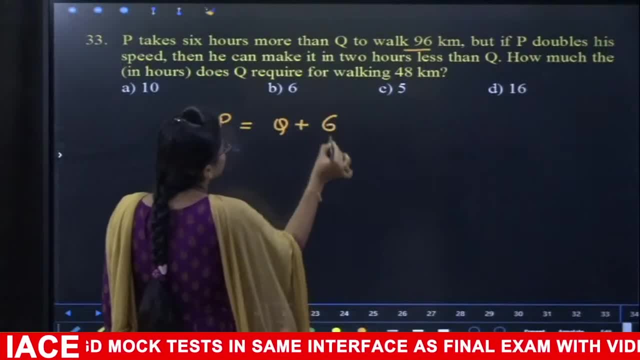 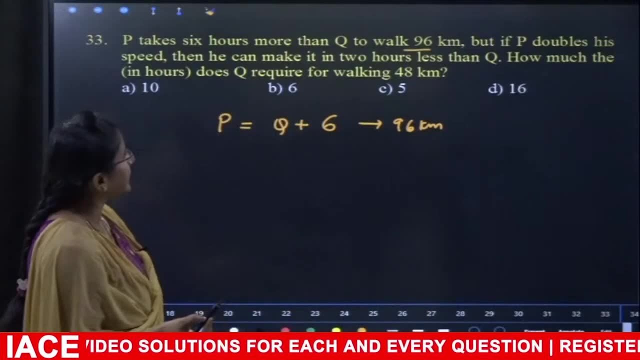 P is taking how many hours more than Q? It is taking 6 hours more than Q when traveling 96 kilometers. Next, if P doubles the speed, then he can make it 2 hours less than Q. If P doubles the speed, then it is 2P. 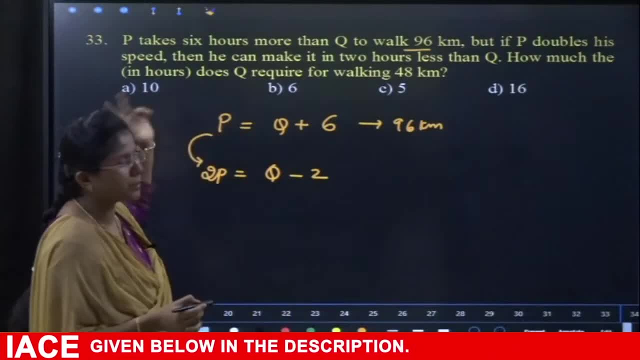 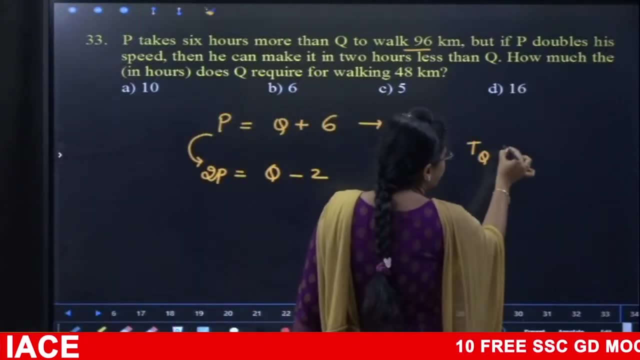 Then the time taken will be 2 hours less than Q. He gave these two and wrote these two. Next, how much time does Q require for walking 48 kilometers? He is asking time. He is asking time by taking Q. What is time equal to? 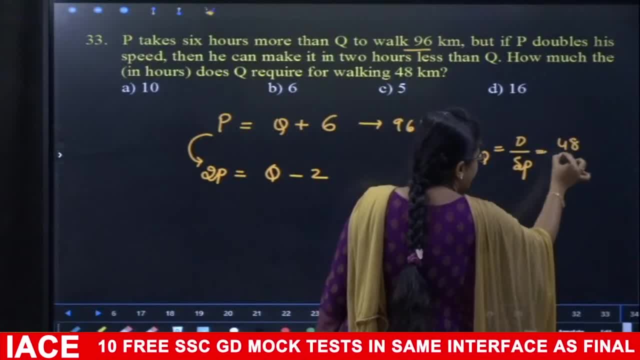 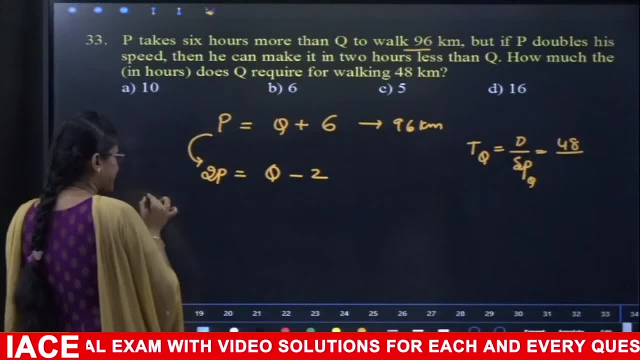 It is distance. by speed of Q. He gave distance 48.. Next, if we find out the speed of Q, we will get the answer. So that comes from these sentences. Next, if we take P speed, the speed of P ratio will be: 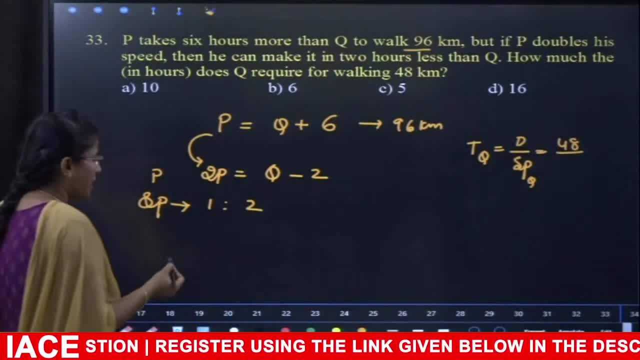 since it doubled here and there. that is, 1 is to 2.. If P speed ratio is 1 is to 2, then what is the time ratio? It is reverse. Since it is inverse, 2 is to 1.. 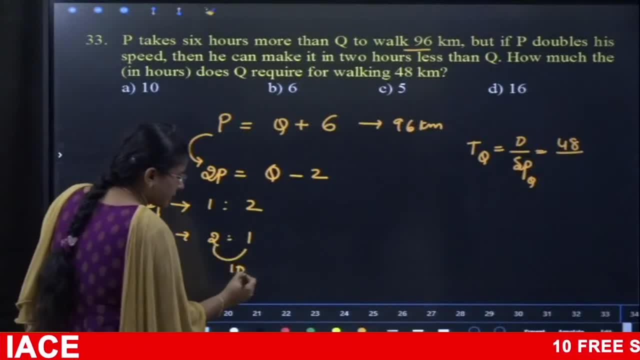 Here. how many parts are there for 2 parts and 1 part, 1 part. If 2 parts are there in the first case, then 1 part is there in the second case. The difference is 1 part. See here. time is 6 hours extra. 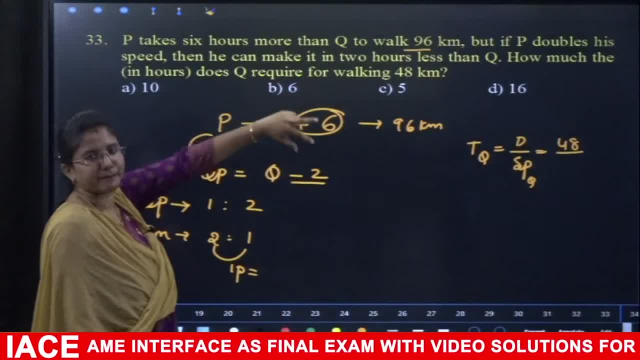 Here 2 hours is less, We will add the difference: 6 plus 2 is 8 hours. Since 1 part is 8 hours, 2 is 6 to 8.. In this case, time is 16 hours. 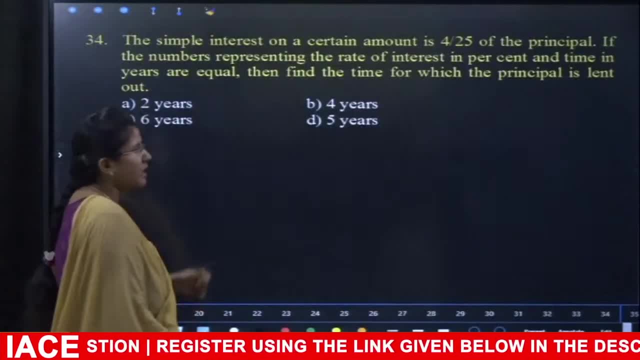 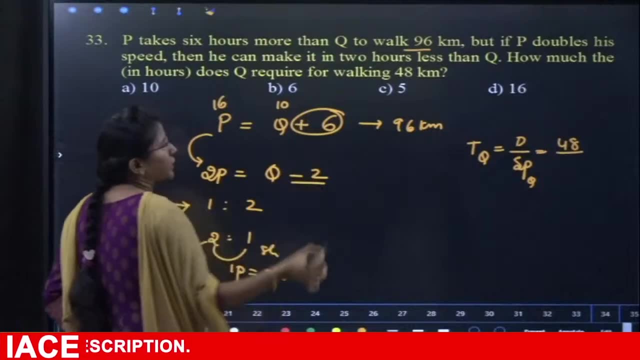 Here time is 16 hours. In this case time is 8 hours, So that 16 hours time is there. So, since 16 is here, since Q is plus 6, time taken by Q is 10 hours. 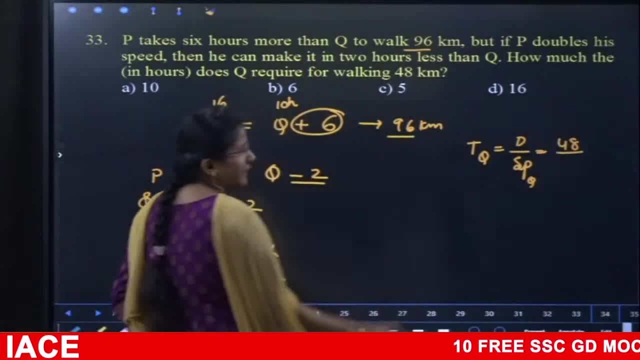 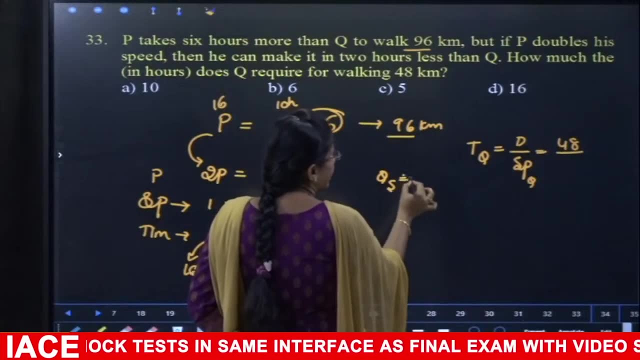 10 hours is the time taken? For how many kilometers? 96.. If 10 hours time is taken for 96 kilometers, we will say 1 hour is the speed. So what will be the speed of Q? 9.6 kilometers per hour. 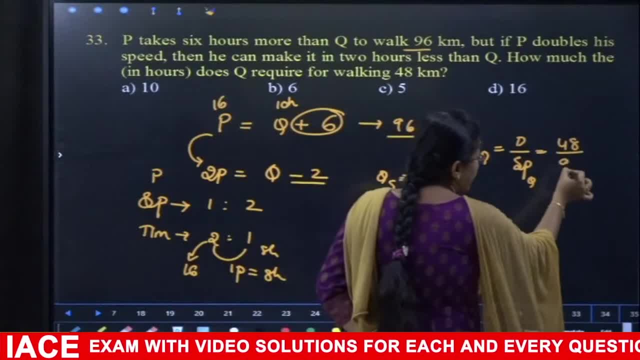 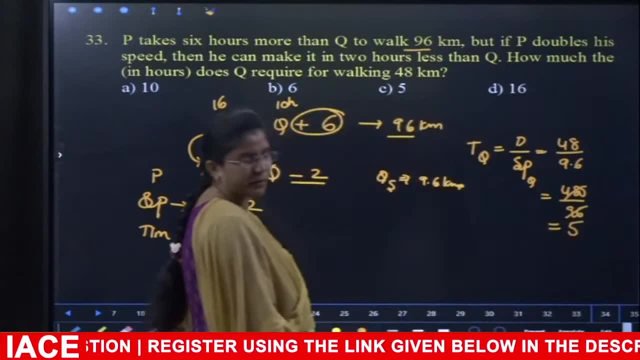 So 9.6 is there, 9.6.. So that will be 480 by 96.. 480 by 96 is the answer. How many hours? 5 hours. That is the time taken. Okay, So as it is for 96 kilometers, 10 hours time is taken. 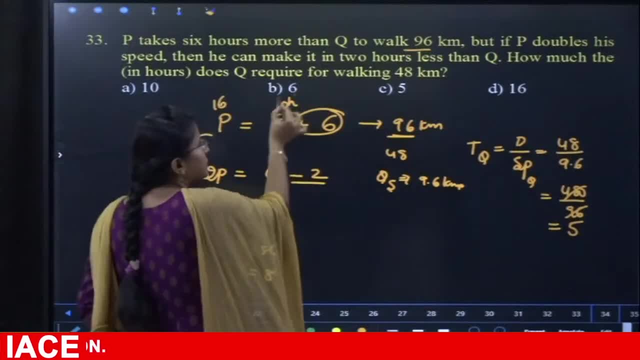 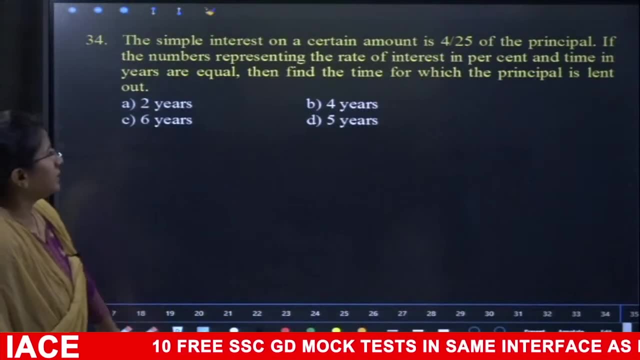 The question asked is 48 kilometers. right, There is half. So what is the time? We can directly put half in 10.. That is 5.. Okay, Next go for 34.. So try 34.. 30 seconds timer, please. 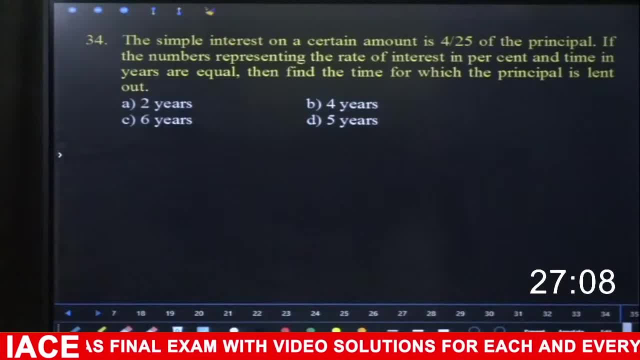 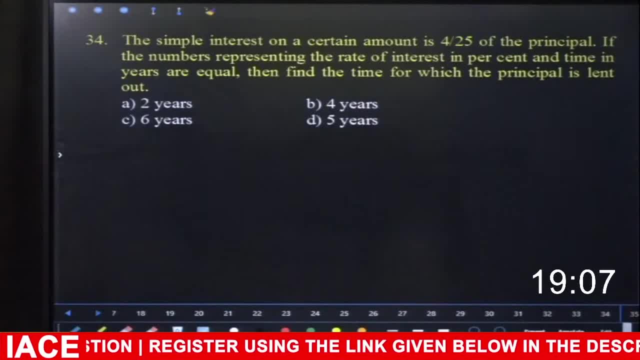 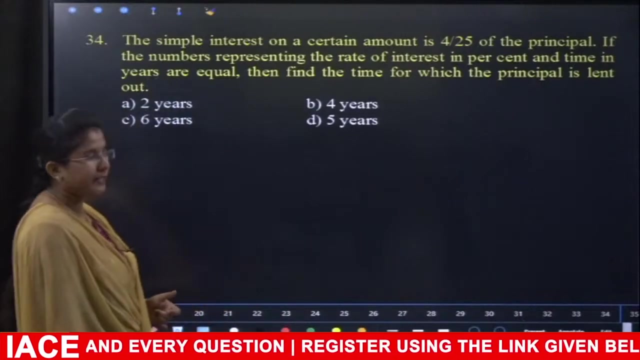 Next go for 34.. Next go for 34.. TOEAD Chair 14T. Okay, You've time missed. So equation is very easy from simple interest topic. This model is used very frequently. Observe it. simple interest on a certain sum amounts to 4 by 25th of the principle. 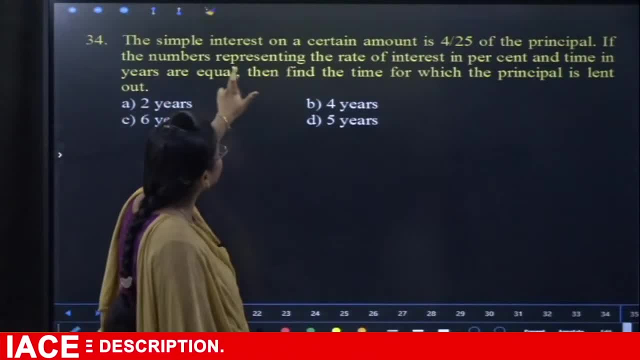 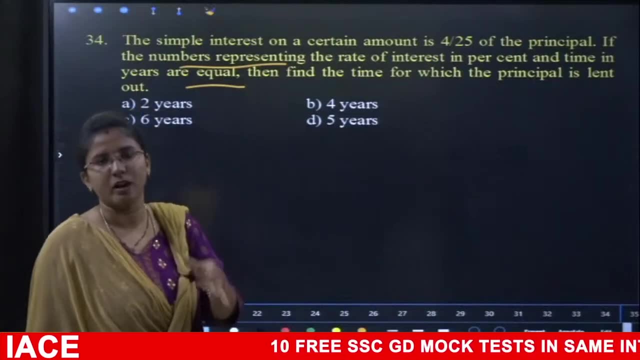 It's a simple interest principle of 4 by 25th. If number of years representing the rate of interest in percent and time are equal, Rate of interest and time are equal. If rate of interest is 10%, then time is 10 years. 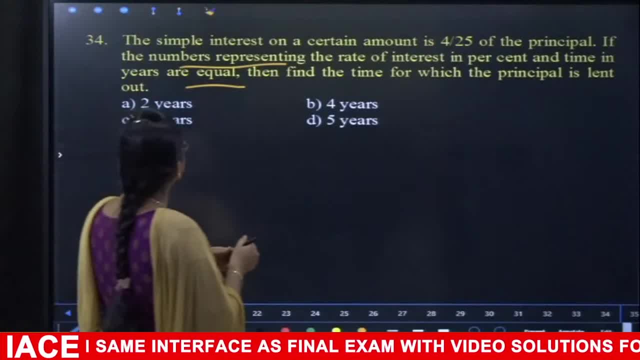 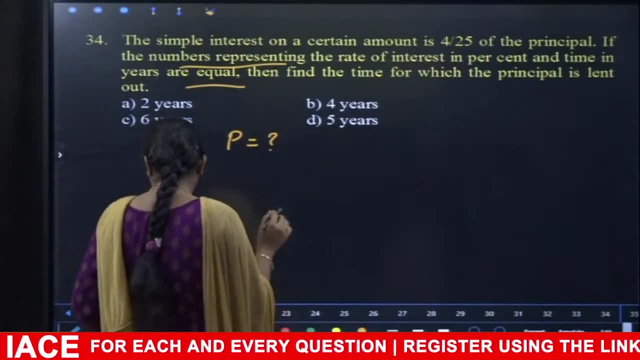 Numerically equal. Find the time for which the principle is lent out. The principle is not given to us, it's asked to find out. Find the time for which the principle is not given. it's asked to find out the time, How much time. 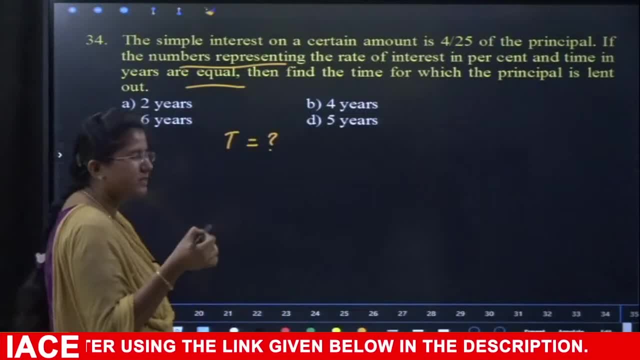 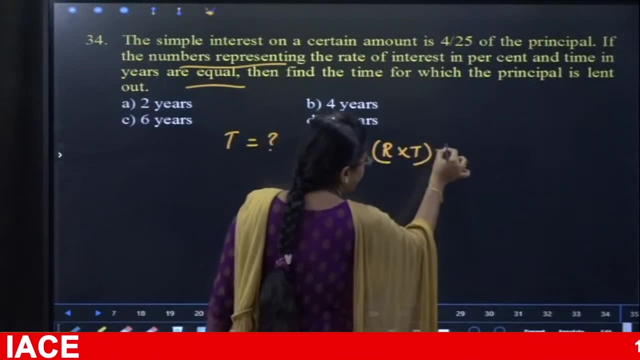 For how much time did we lend? It's asked to find out the time. So we have simple interest. we just write PTR by 100.. I am writing PTR by 100 in the form of changing it R into T. percent is of principle. 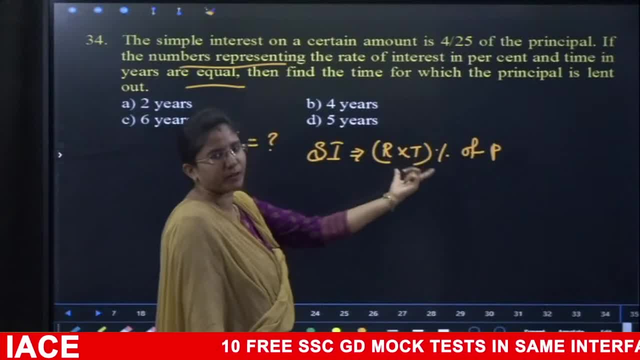 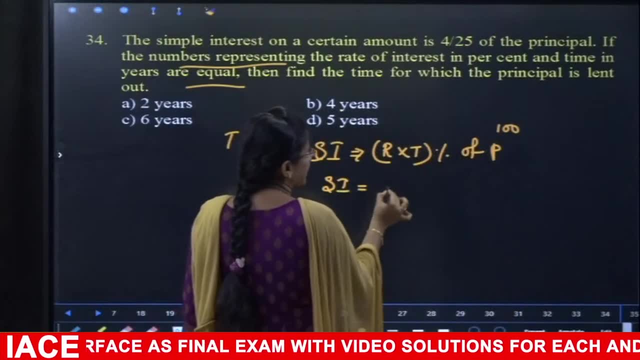 The principle is R into T percent. This is nothing but PTR by 100.. Since the principle is not given to us, I am taking 100.. How is the simple interest? 4 by 25th? In the principle there is 4 by 25th of 100. 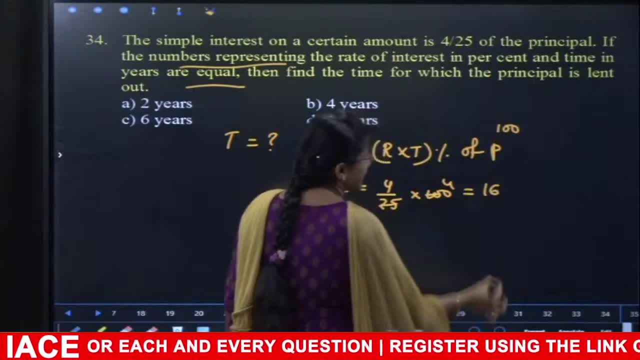 That will be 16.. How much is 4? 16.? There is no intention of taking 100.. If there is a percentage of 16 in 100, it will be 16 percent only. We don't have to calculate it separately. 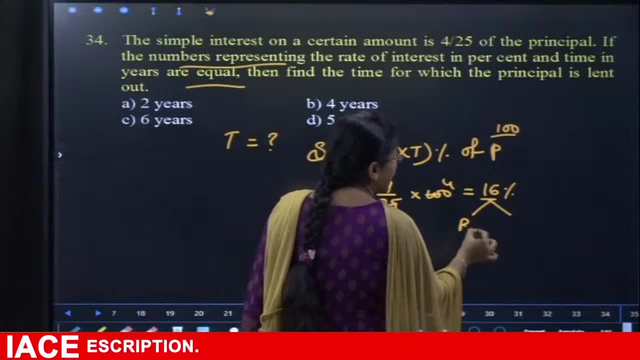 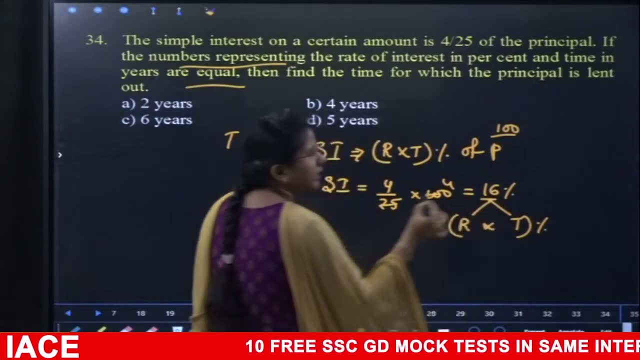 In this simple interest of 16 percent, what will be the multiplication of R and T? Since there is R and T percent, the rate of interest is 16.. He said that these two should be equal. So if we divide 16 equally, like this, it is 4 into 4.. 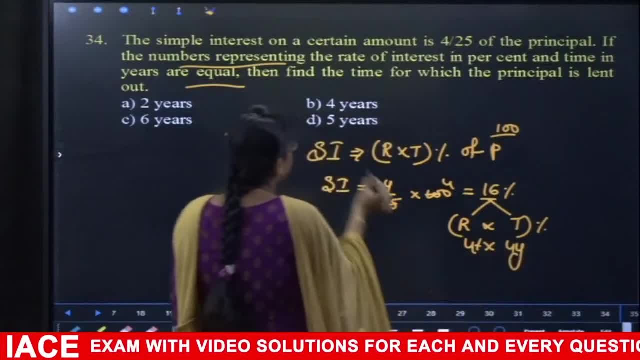 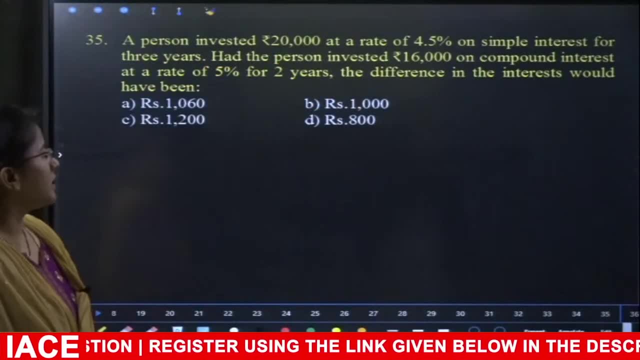 So if the rate of interest is 4 percent, then time is 4 years, So time is 4.. Option B: Okay, Next. Next we will go for next one, 35. Try to write the equation. 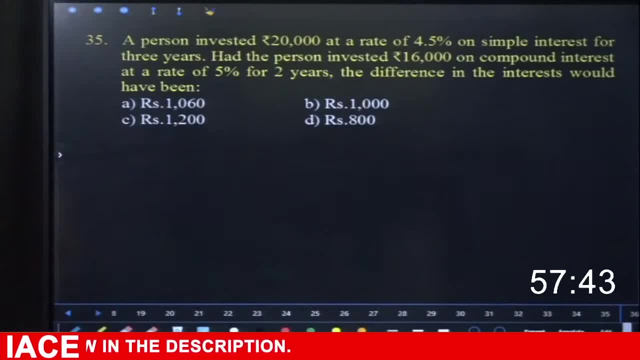 One minute timer please. Simple compound interest. Fine, Okay, I will write Y or Y zero as 1 to R, 1 byKY 2 times. Finally, y is a linear solution. What will be R of 0?? Rock is 1.. 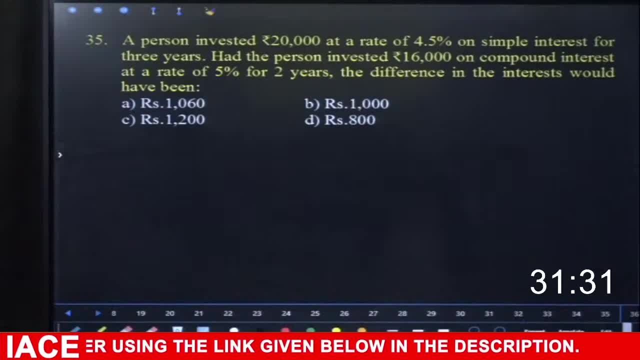 Rock is like a magnet. Uh huh, Rock by Krypton. Yes, Y is equal to 0.. Something happens to rise up little by little. Yes, Come on, Bring on what is Yes, the ball of y. Look at the position. 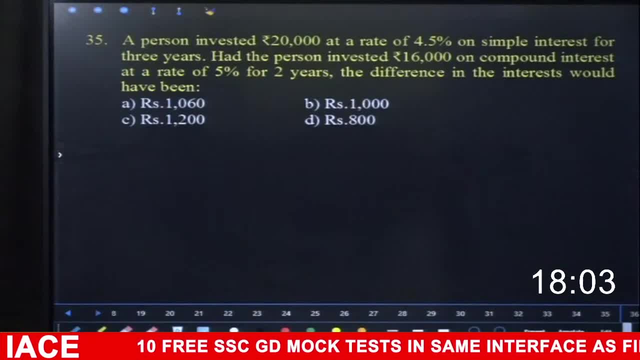 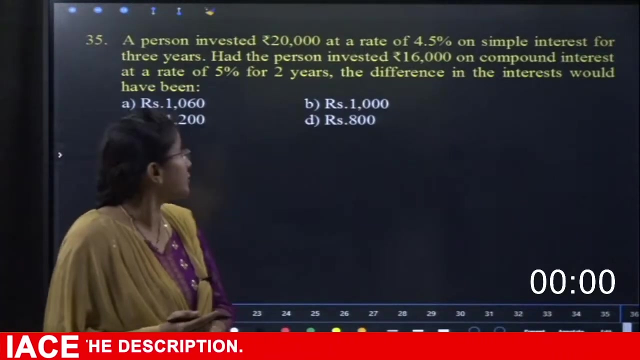 Look at the equilibrium. Yes, What's the equation of x minus 1 by 4?? Sometimes X and y get equal to 1 by 2. you always we will have three times. All right, okay, your time is up, so question shouldn't be. a person invested 20 000 at the rate of 4.5 percent. 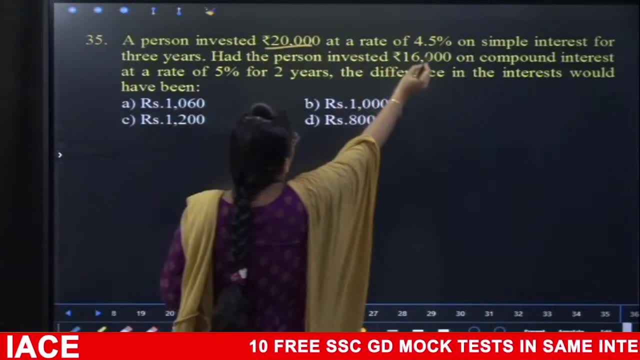 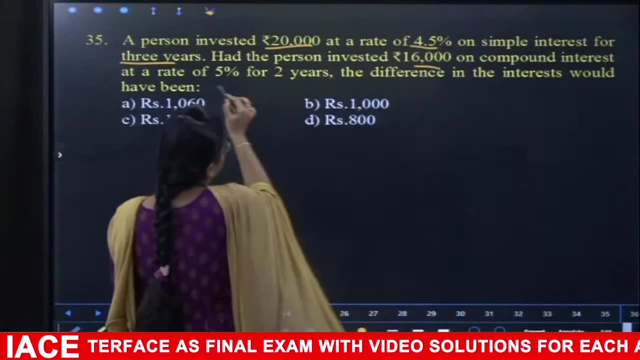 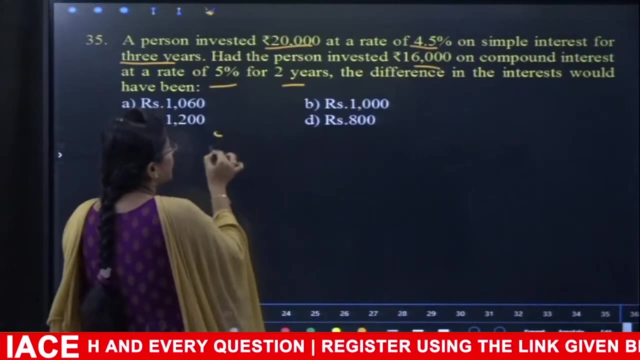 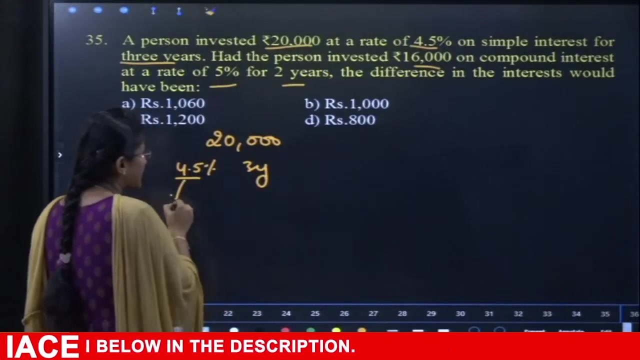 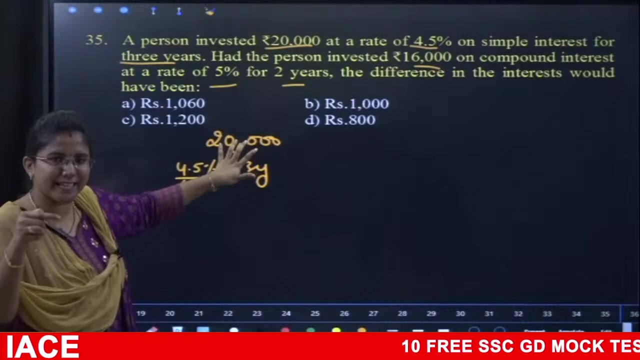 simple interest for three years: 20 000 principal 4.5 percent rate of interest in years, three years, had the person invested 16 000 non-compound interest for five percent two years. so principle 20 000, 20 000, three years, 4.5 percent, 20 000, 1 percent, 200, 4 percent will be 200 four times six, eight hundred. 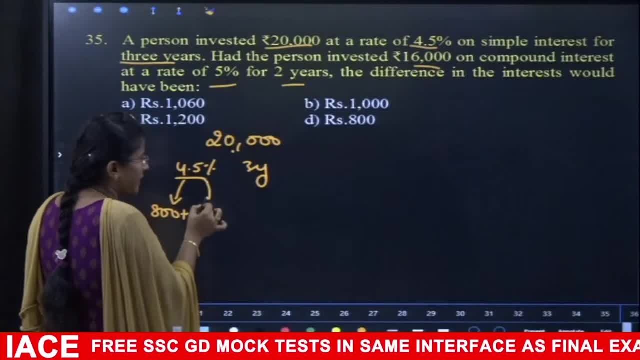 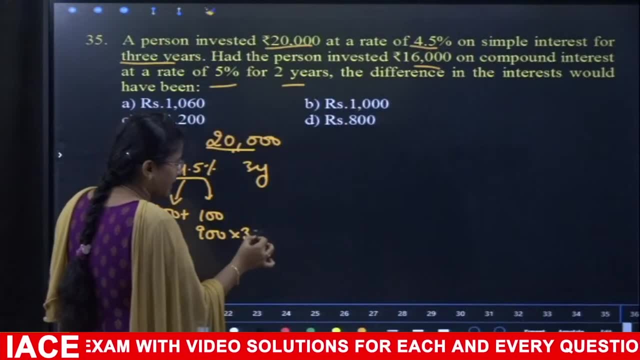 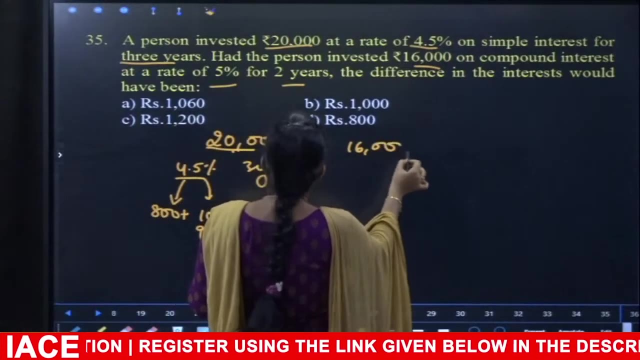 eight hundred four percent already in the two hundred me half chest, a hundred. so overall interest in nine hundred one year, three years, and not about in nine hundred, three cities, two thousand, seven hundred. next principle given to us is sixteen thousand, a sixteen thousand made a rate of interest monkey, five percent each other, or linear sir. 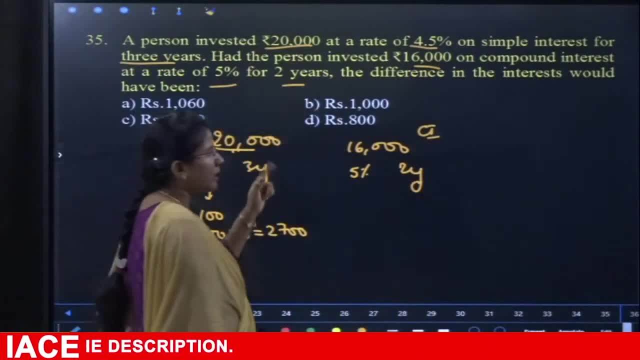 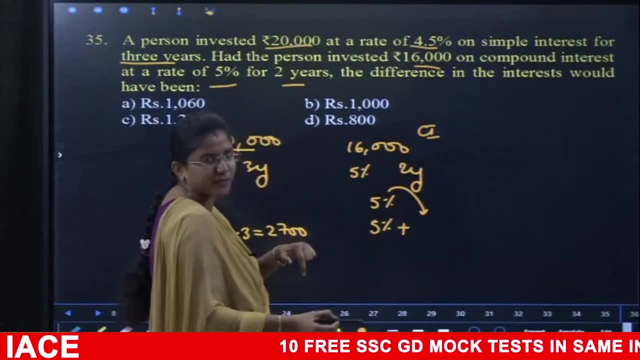 two years I paid a simple cargo compound, interesting compound, interesting to interest, medical interest. burden of our tea: first year five percent. second year five percent plus extra. the final multi five percent is some academic, is zero point two, five. so overall we could get ten point two, five percent of interest. 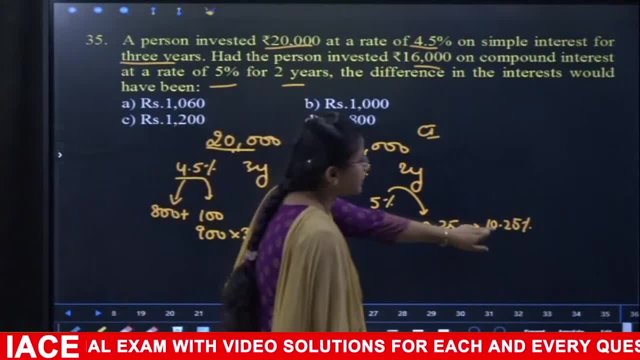 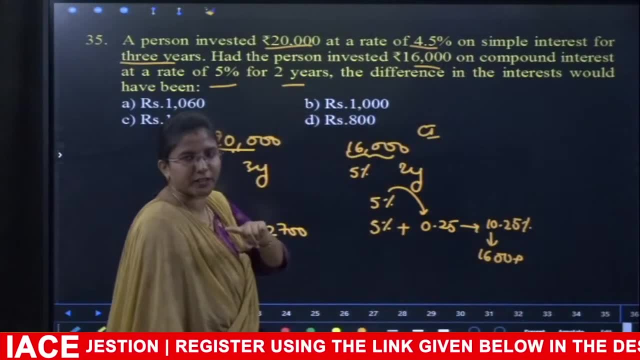 principle made and to the lesser the compound interest, or so that I come on the ten percent, process them. ten percent value is nothing but sixteen hundred plus zero point two, five, into one, fourth, Andy, already in the one percent value one sixty one together, zero point two, five and ten, and by for. 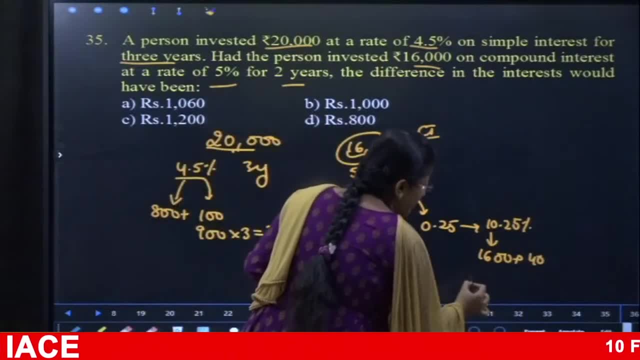 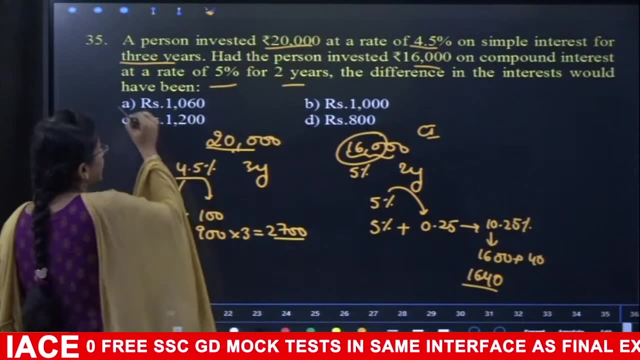 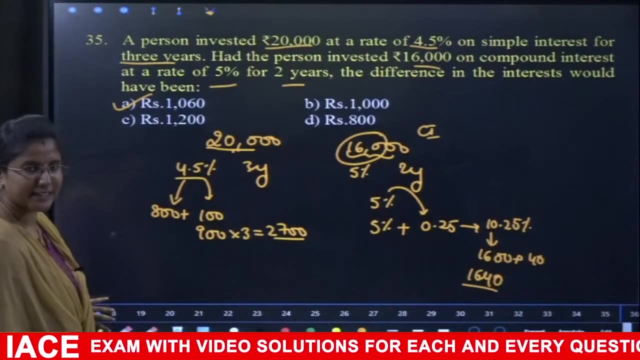 chidami, one sixteen by four chaser it is forty. so total compound interest we got sixteen, forty and here simple interest we got two thousand seven, hundred. then you can difference another. so that is one zero, six, zero across forty to hundred, and the sixty one option. you don't go down the option a. okay, next 36, so equation try. 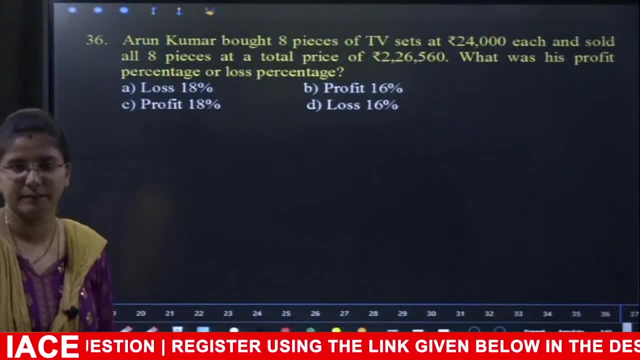 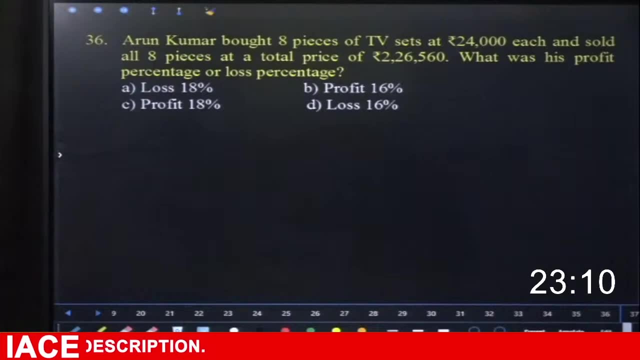 change. and, Andy, we put a very easy question: 30 seconds timer, please you, William. okay, so your time. he's up equation: Laman working Kumar. but eight pieces of TV sets are 24,000 each and sold all eight pieces at a total price of two Oooh las, 26,000 and five sixty. so what is? 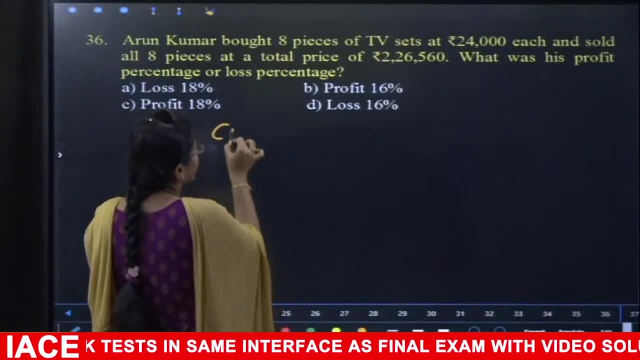 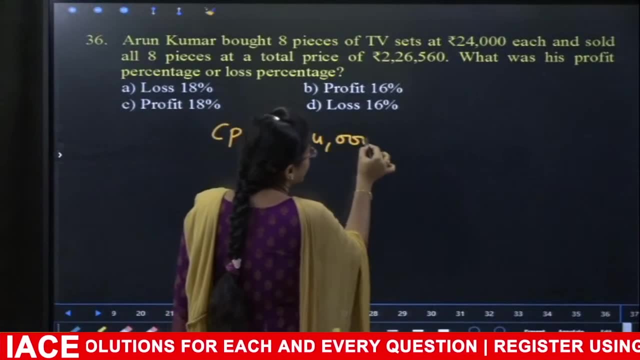 is profit percent or last person days are you got bought and another day cost price. and the eight pieces are each and another day, 24,000. total cost present with me: 24,000 into 8000, multiply- shame on inches. the next is selling price. he. 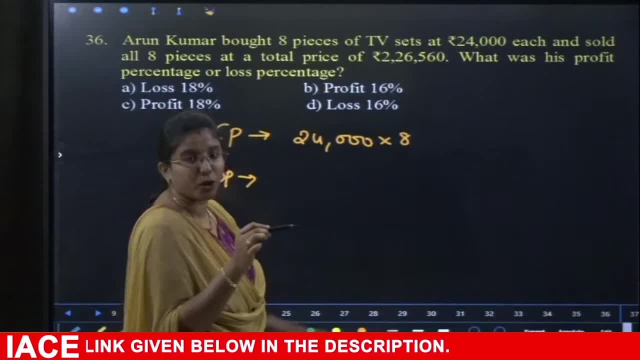 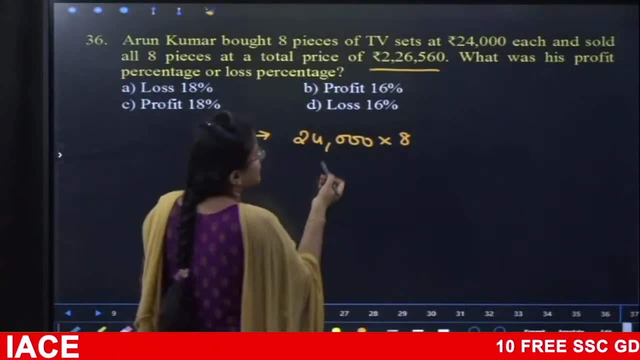 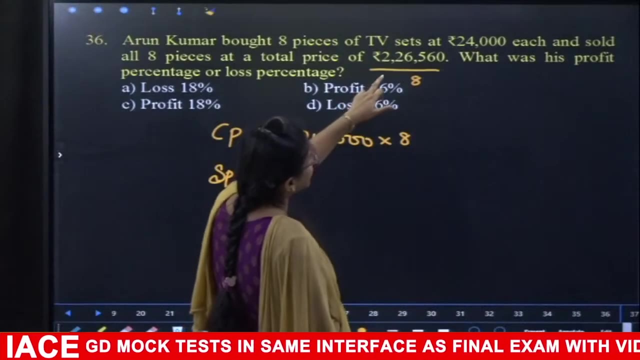 sold eight pieces at total price. inches and total price to lack 26,000 and 560 shadow it really into waiting on the gravity that would integrate the last one. so here my own thing is just teaching and I'm done by adjust. take multiple conversion, so eight multiple will be what a twos? that will be 16, 16. 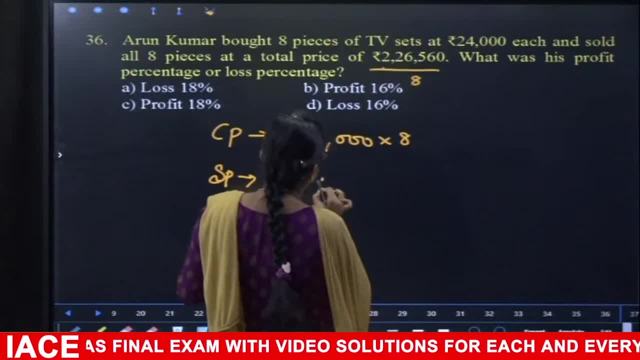 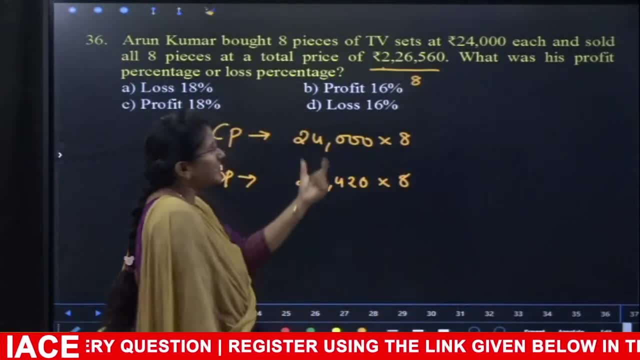 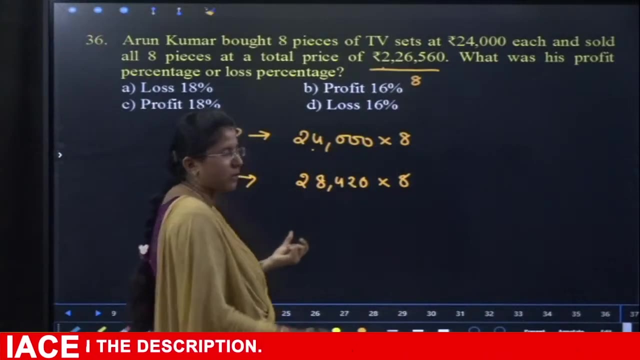 and here for and 666, 824, 25, 25 will be 4, 2, 0 into 8, the mission number, total price and a multiple Garasa. so here money to 24,000, gonna TV content, 20, 8000 and 422. cut a VM is on wood. so here that will be a normal profit or loss, or 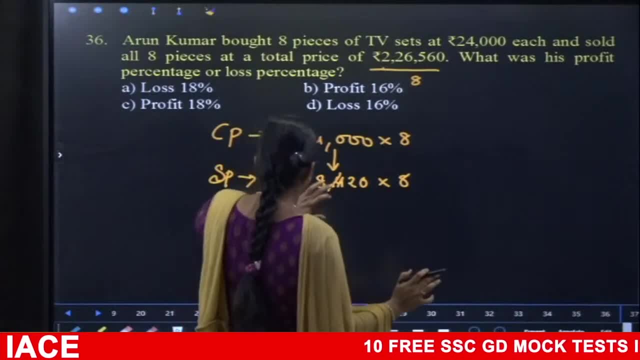 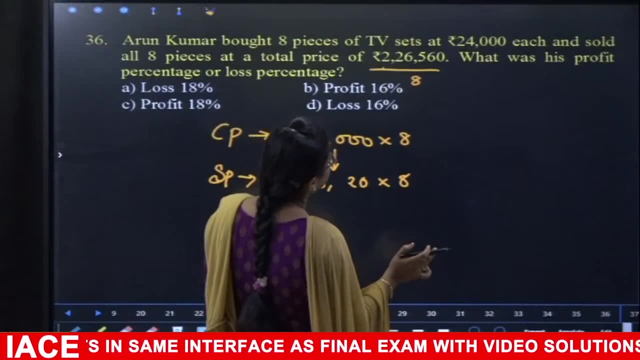 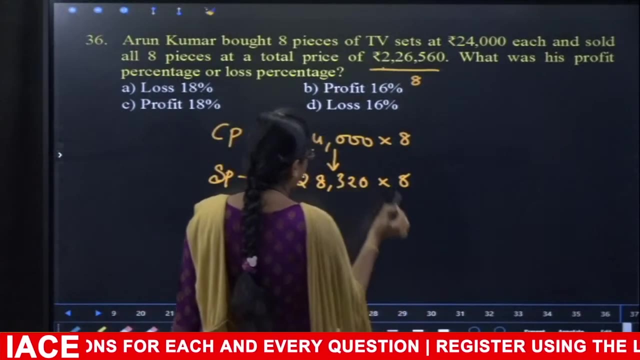 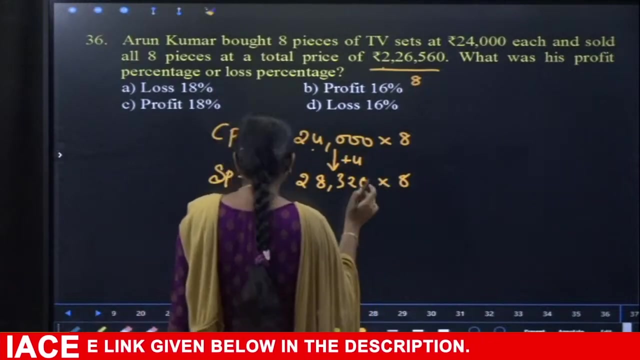 sooner profit. This is not 28,, 216,, 268, 25.. That will be 3.. That is not 4.. It is 3.. Okay, So the profit we get there is 4000 and 320.. 4000 and 320. 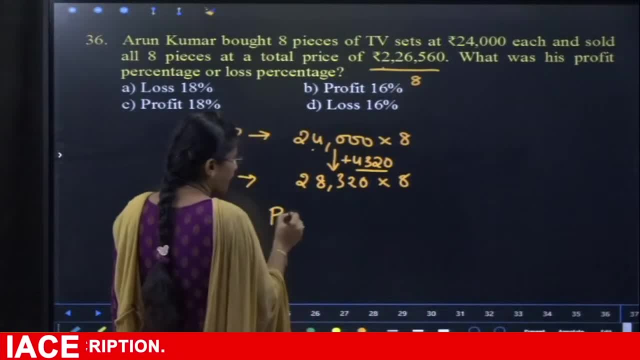 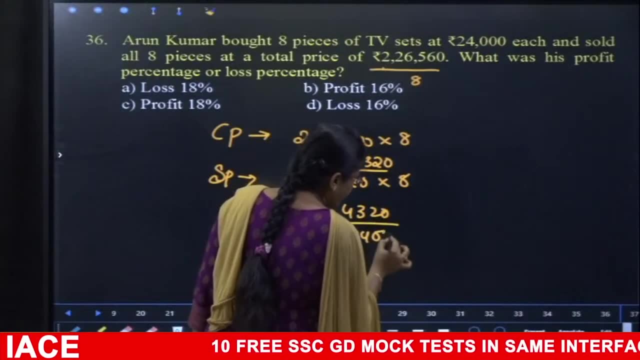 4000 and 320 profit on each TV. We know the formula for profit percentage: Profit by CP into 100.. Profit is 4320.. By cost price is 24000 into 100.. If we cancel out all zeros, 24 and 2 will be 18.. 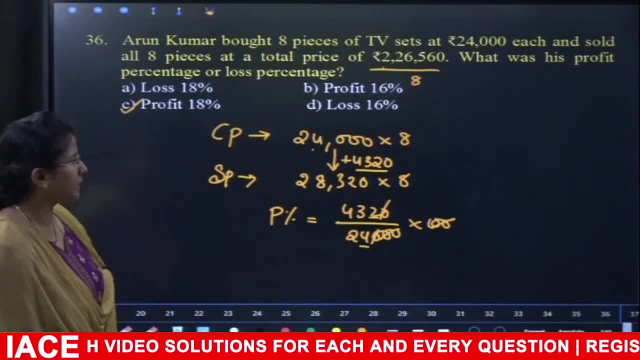 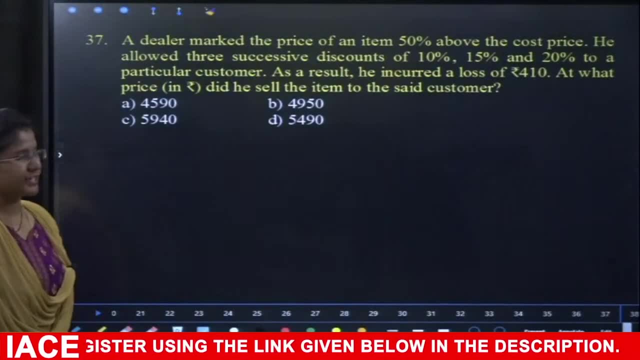 Unit digit will be profit percent of 18%. Okay, Easy question. Next, Go for 37.. Okay, Try this question. One minute timer please. Of course, in this analysis we have navel chart and plot. We know the result. we have the result. 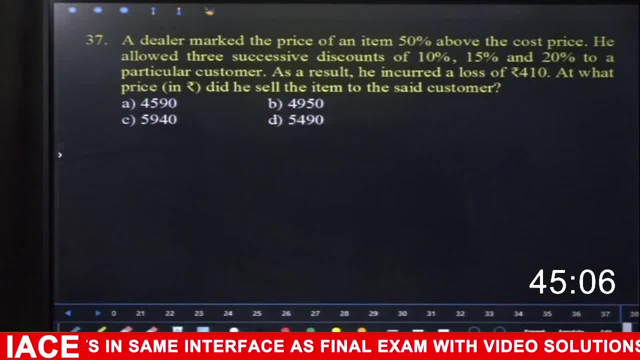 In real time for each channel. for each channel we have three channels, So we are trying to figure out. is there any net profit for each channel? This is a long term figure. Thank you for watching. Thank you for watching. 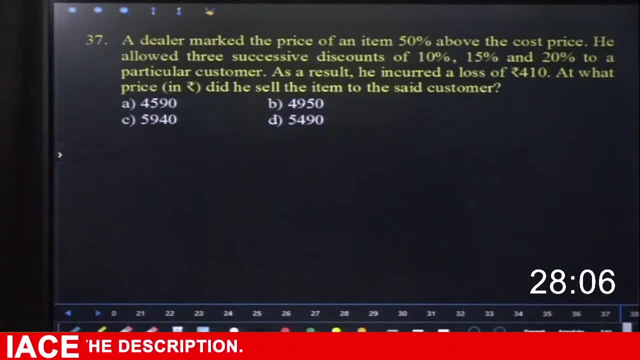 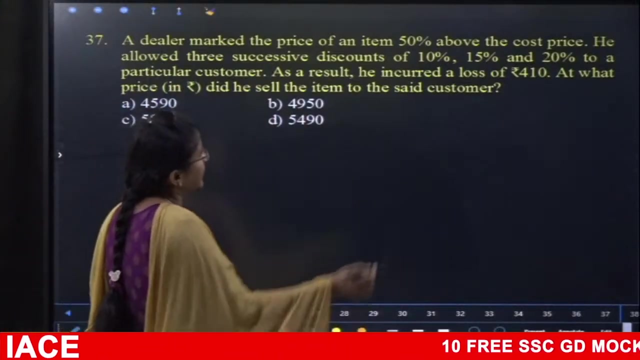 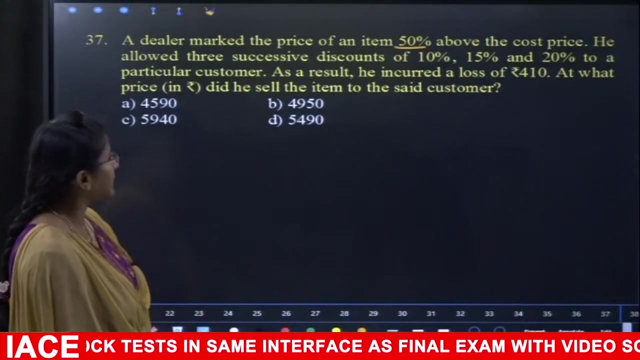 Thank you all. Thank you all. Okay, So next let's solve this question from the profit and loss topic. A dealer marked the price of an item 50% above the cost price and he allowed three successive discounts of 10,, 15, 20% to the particular customer. As a result, he incurred a loss of 410 rupees each. Then at what price did he sell the item to the said customer? At what price sell the item means he is asking the selling price. Our question is on the selling price. 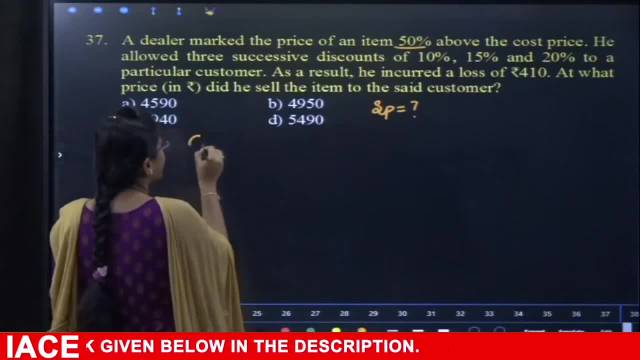 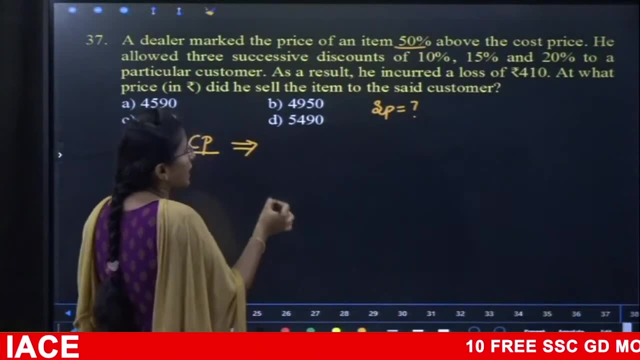 So let's just remove this directly from the parts. Initially he bought cost price. The cost price will always be for 100%. The successive changes you made to it is that you increased the already 100% to 50% above Increase. Then he successfully gave discounts on the increased value of 50%. Discounts are minus. That is, the first discount is 10% decrease. the second discount is 15% decrease. the next discount is 20% decrease. We will take these as a fraction. 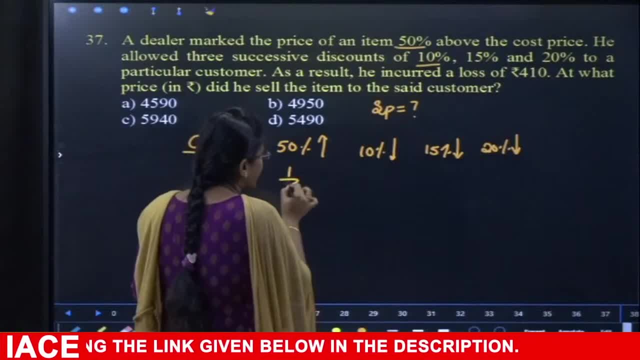 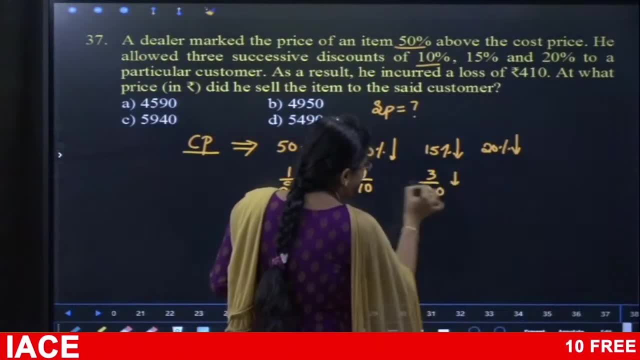 Let's try it. 50% above will be fraction 1 by 2.. 10% is a fraction 1 by 10.. This is 15 by 100.. 15 by 100 means that is 3 by 20 less. 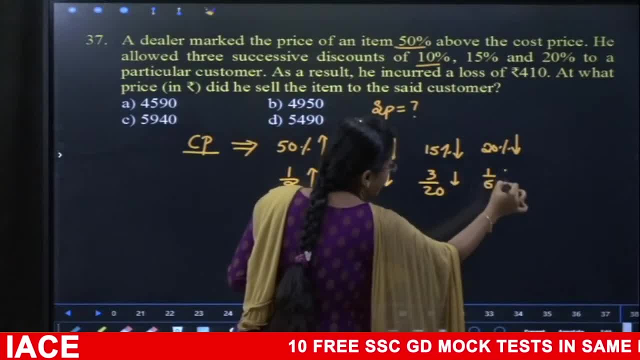 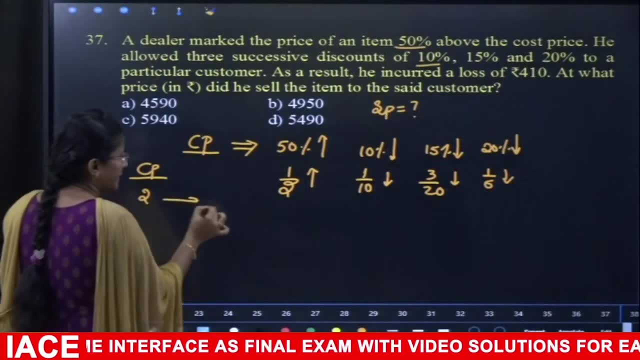 Less. This is increase And 20% will be, that is, 1 by 5 less. So he increased one part of the two parts, That is initially. he increased the cost price of the starting two parts by 3 parts. 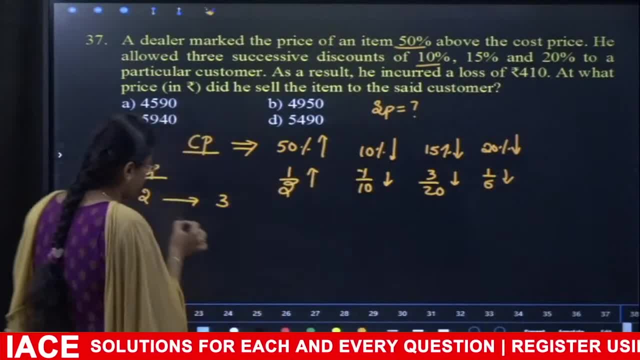 Next here: 1 by 10. He decreased the one with 10. That is, the one with 10, the next value is 1 decrease, that is 9.. Next, he decreased the one with 20 by 3.. 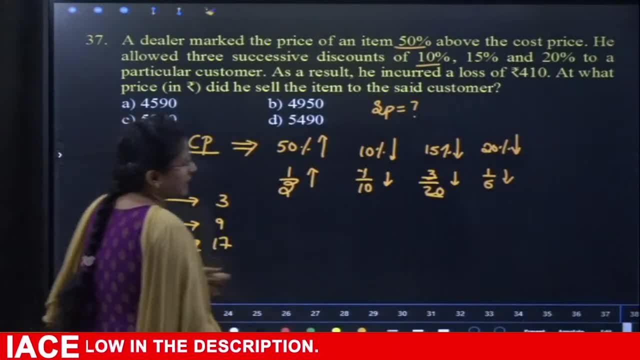 That is, he decreased 3 from 20.. That will be how much: 70.. Next, he decreased the one with 5.. This will be the one with 5 parts, Since he decreased the one with 1, it will be 4.. 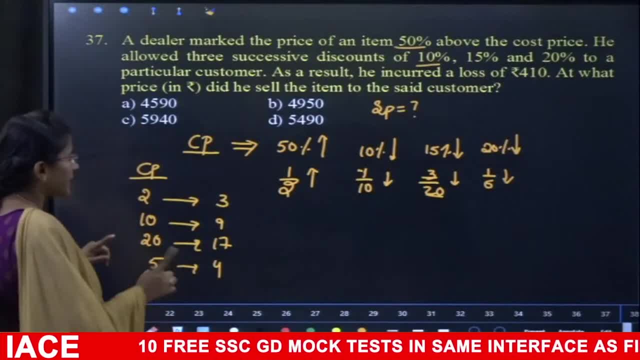 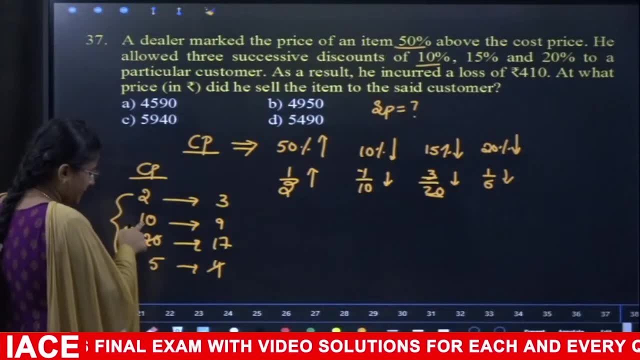 We will multiply all these in the sequence. If anything is cancelled, we have to see the alternate here. That is, since 4 is 25 times. So if we multiply all these, 25 by 10 is 252.. That is 500. 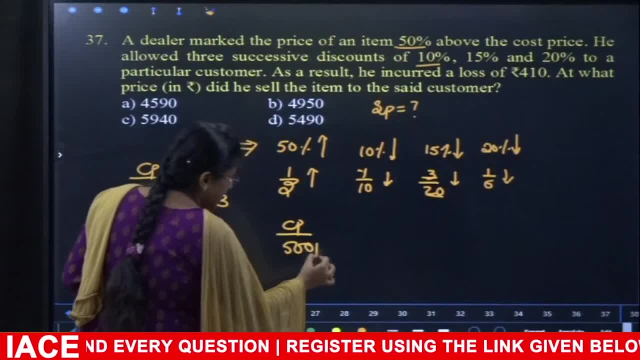 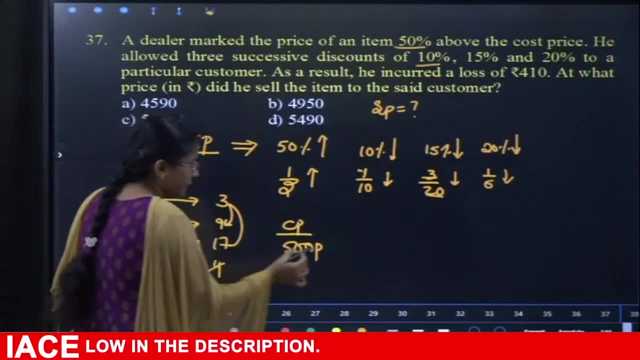 The total cost price we got here is 500 parts. We will multiply all these. If we multiply this side like that, we will get: 17 by 3 is 51.. 151 by 9 will be 459.. What is the selling price? 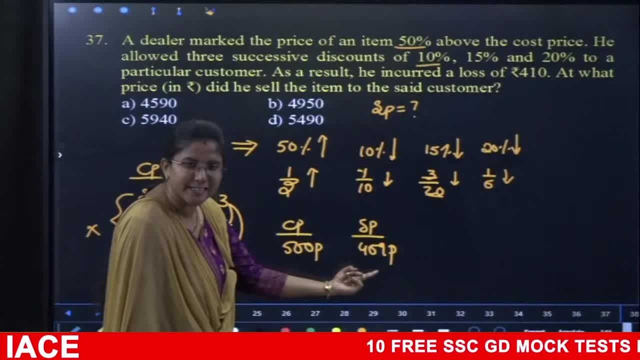 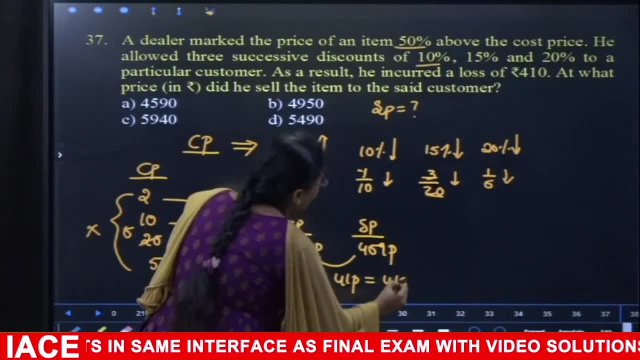 459 parts, Since we bought 500 parts. if we sell 459 parts, we will get the loss. What is the loss? 41.. How much is the value of 41 parts? He gave 410 rupees, So the one part value is 10, right. 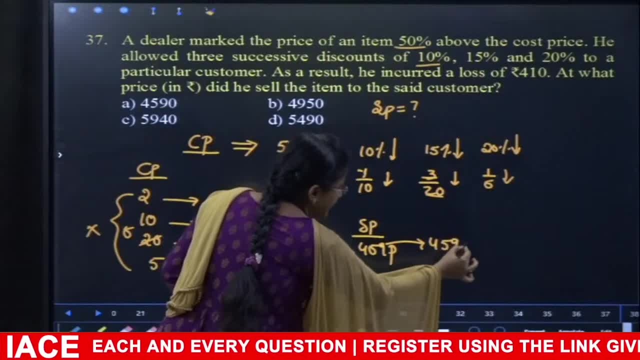 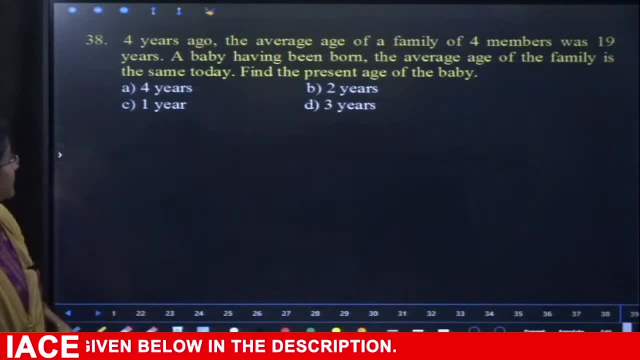 Since he asked the selling price, there are 459 parts, So the answer is nothing but 4590.. Option A: Okay. Next go for 38.. Please try to solve the equation in 30 seconds. I will ask the question in 30 seconds. 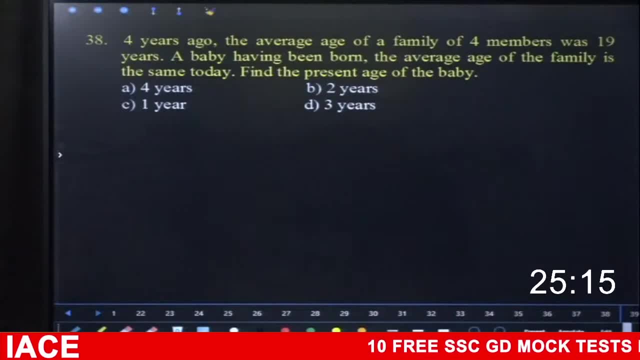 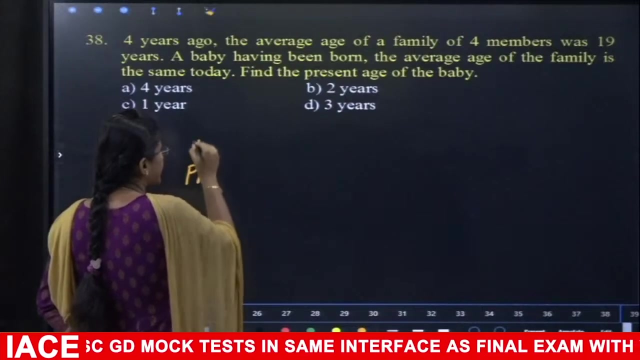 I will ask the question in 30 seconds. 38.. Try to solve the equation in 30 seconds, Please. 4 years ago, the average age of a family of 4 members is 19 years. From the present, the average age of a family of 4 members is 19 years. From the present, the average age of a family of 4 members is 19 years. From the present, the average age of a family of 4 members is 19 years. 5 members are equal to 19.. Here, the average age of 4 members is 16 years. 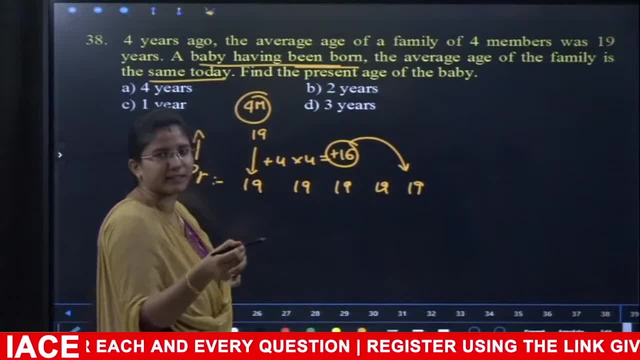 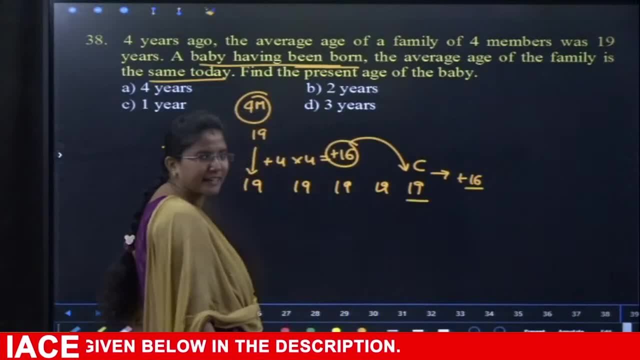 increase of all Cindy a baby can, addition jargon and bigger than 60, not chasing Taravata, that chain age become 19. I find the 16 edition chase a car, 99 that a initial age moon, the major original age of baby in years from. 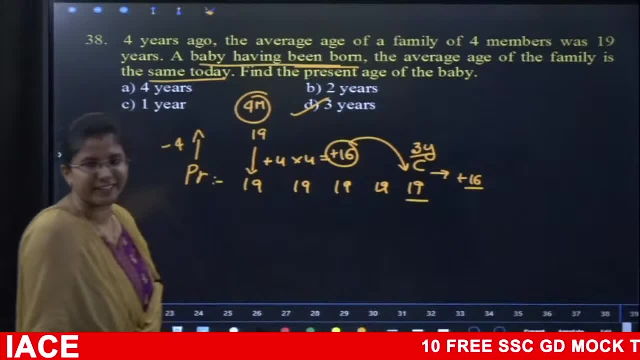 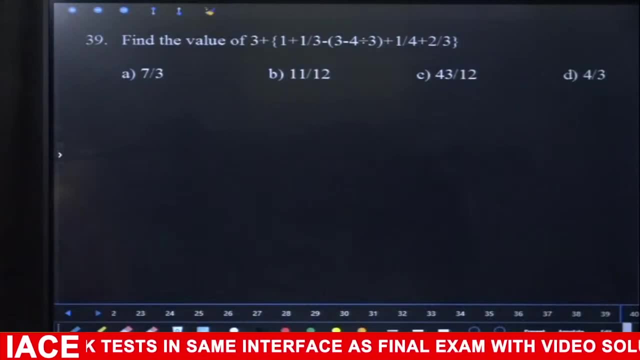 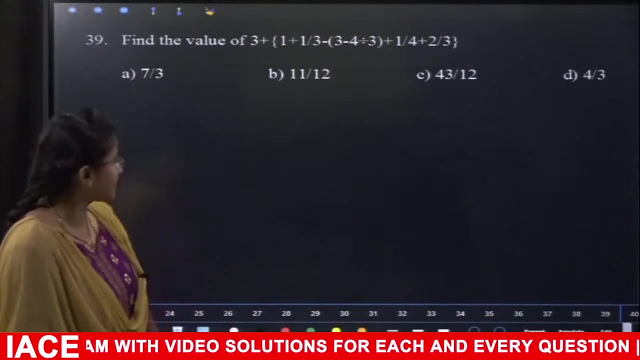 Darlene D, three years. so option is the be three years, very easy problem. next go for 39, the simplification bit, and each other easy 30 seconds time, oh, please you. so the very easy question in the simplification board, model board must rule. uses the under can answer which is: 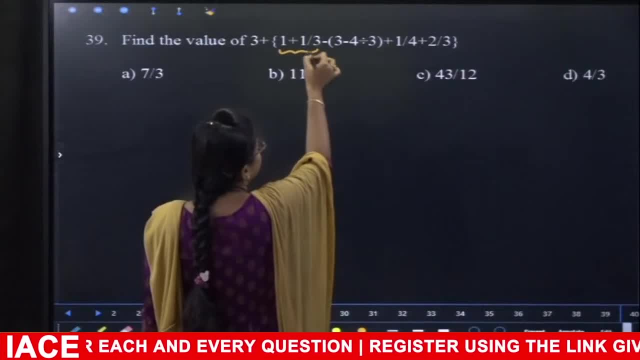 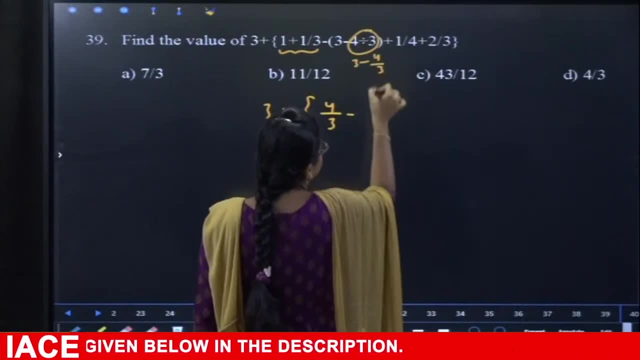 to me. Buster right, you know, I saw the system here. 1 plus 1 by 3, that is the 4 by 3. 3 plus 4 by 3 minus 4. 3 minus 4 by 3, that is the 9 minus 4, that is 5 by 4. 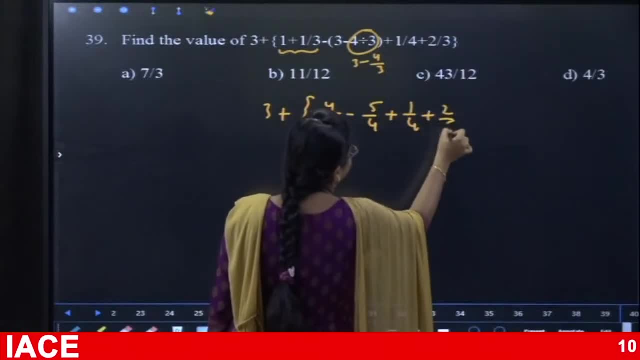 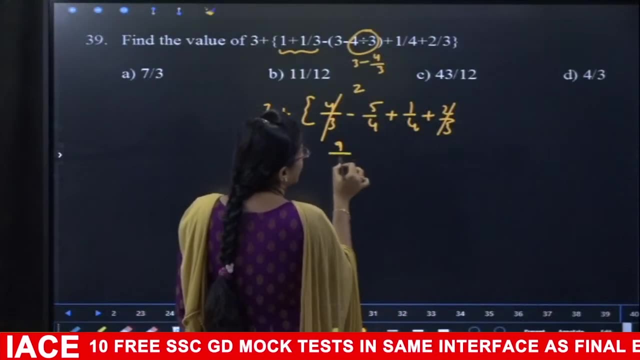 plus 1 by 4 plus 2 by 3, 1 D and E random on 3 denominators. this is a 6 by 3 or over to in the 2 plus 1 by 4, that is 9 by 4. so 9 by 4 minus 5 by 4, that is one. 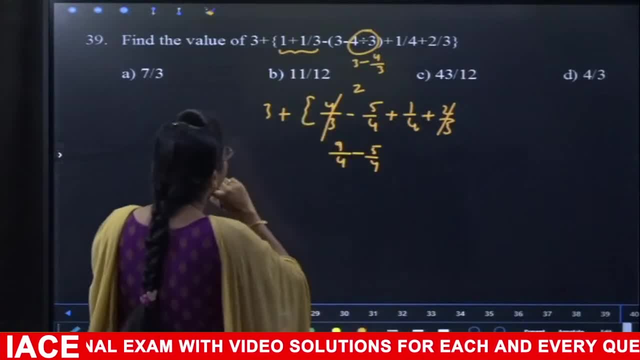 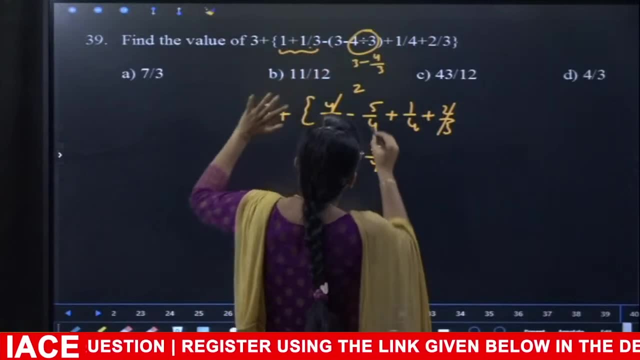 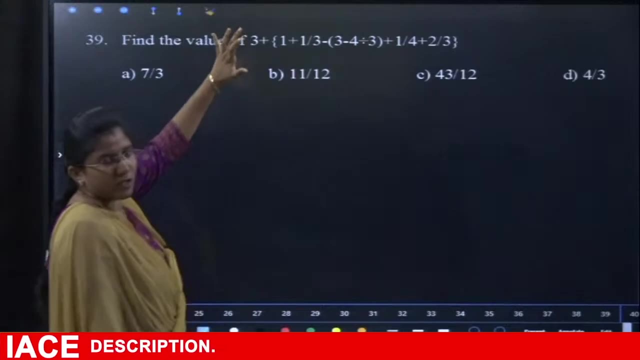 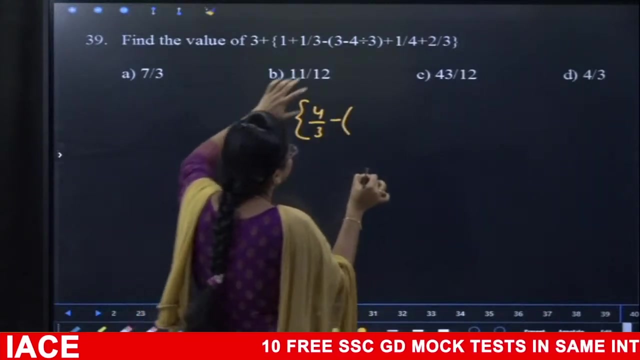 over all. go oh, 4 by 3 plus 2 by 3.. Majalok: 3 minus 3 minus 4 by 3.. So here that is 3 plus 1 plus 1 by 3, that is 4 by 3 minus 3 minus 4 by 3.. 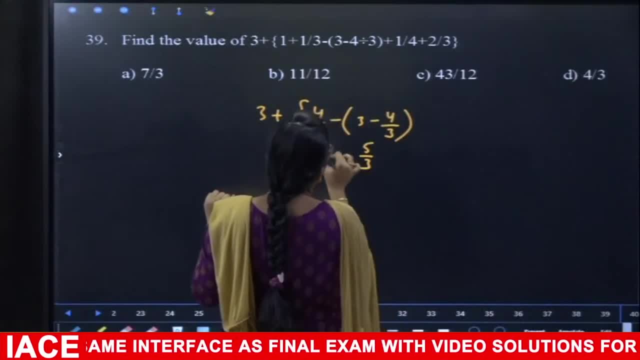 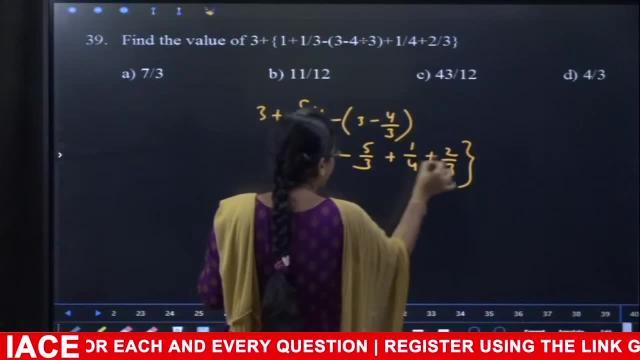 That is 9 minus 4 is 5 by 3.. Here it is 4 by 3 plus 1 by 4 plus 2 by 3.. In this overall board mass we can cancel out both and write C2 as minus 5 by 3 plus 1 by 4.. 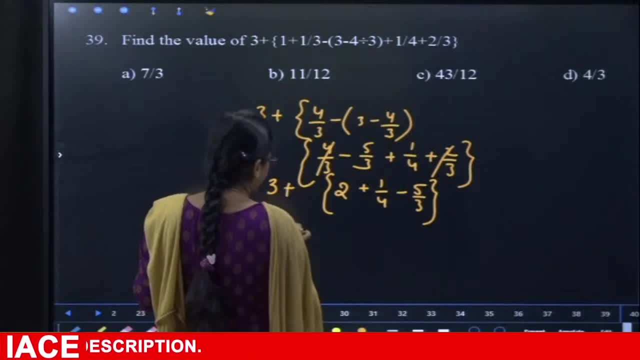 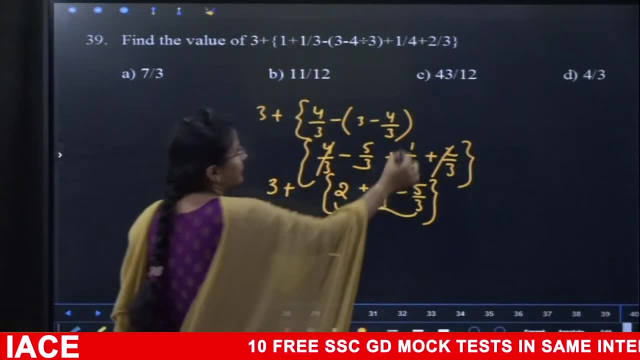 So here we already have 3. so if we solve this by taking LCM, we will get final answer 43 by 12.. So here 12 will be given 43 by 12. If we simplify this it will be fine. 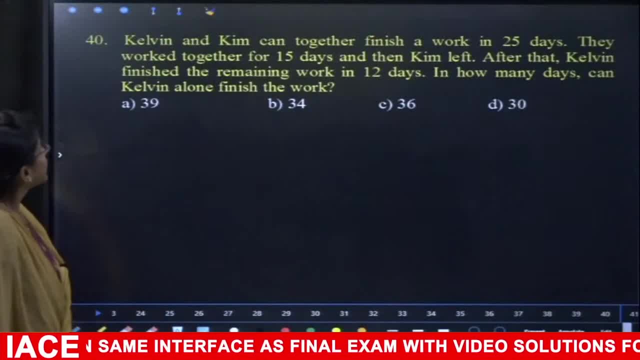 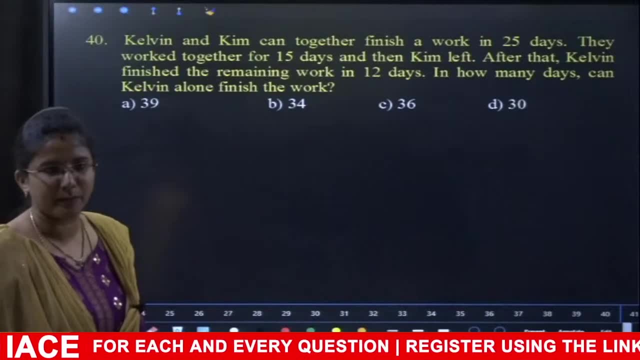 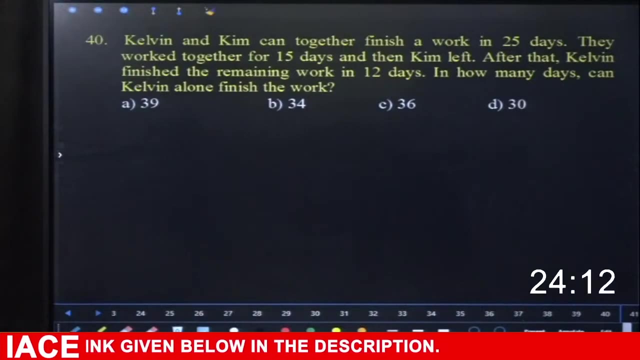 That is option C. Next Problem 40.. 40 is the equation. 30 seconds timer, please. Time and work topic means C. Okay, your time is up, So let's see the topic. Let's see the equation From time and work topic. 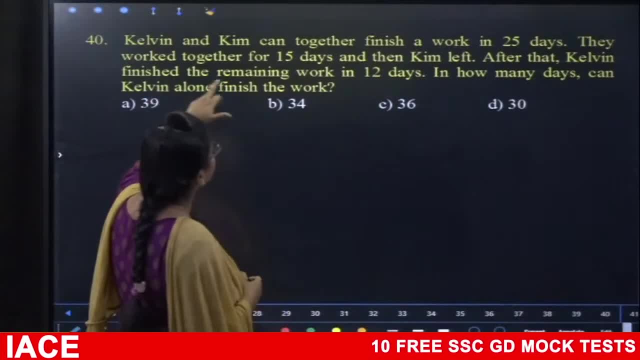 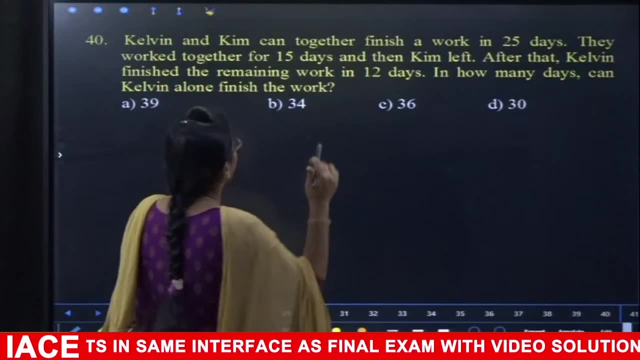 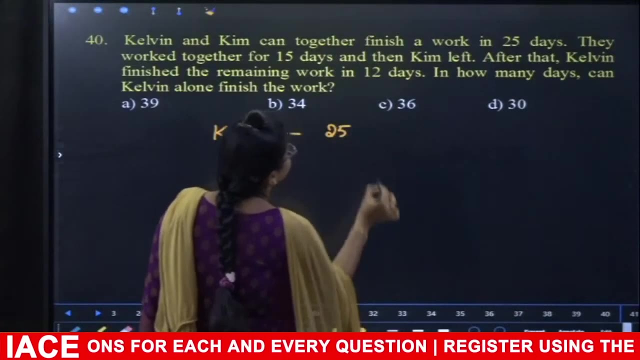 Calvin and Kim can together finish a work in 25 days. They work together for 15 days, and Kim left After that. Calvin finished the remaining work in 12 days, So Calvin and Kim can complete the work in 25 days. They work together for 15 days. 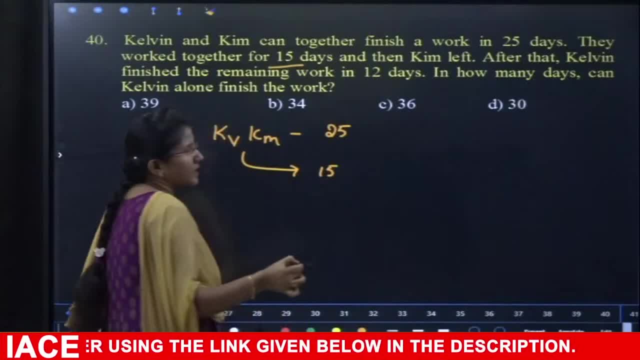 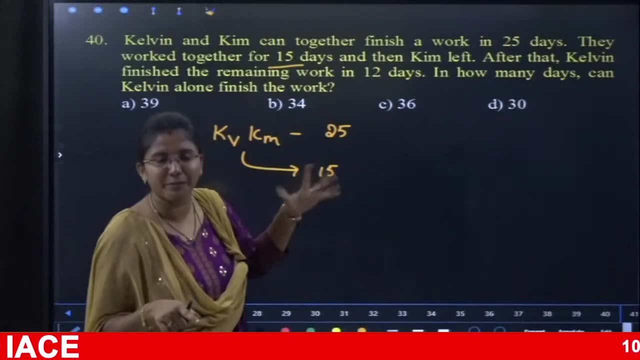 Likewise, they started the work and worked for 15 days. If they work together for 25 days, the work will be completed. If they work for 15 days, we can write how much part of the work was completed. How much part of the work was completed is 15 days. 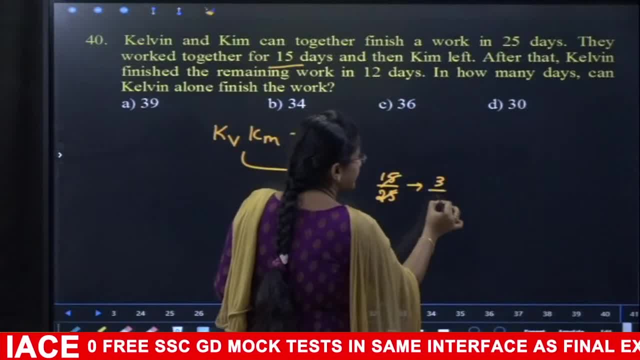 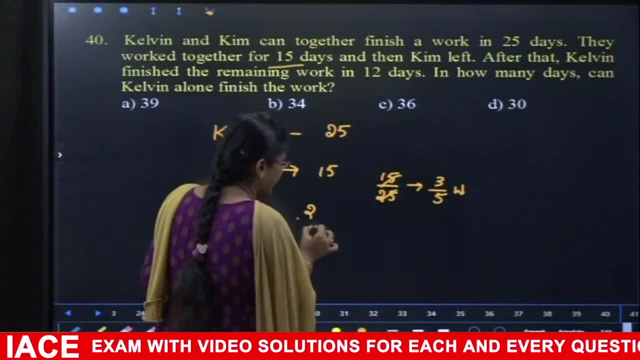 15 by 25. that is how much 3 fifth- 3 fifth of the work was completed. That is 5 parts. 3 parts were completed in 5 days. If it is 3 in 5, how many parts will be remaining? 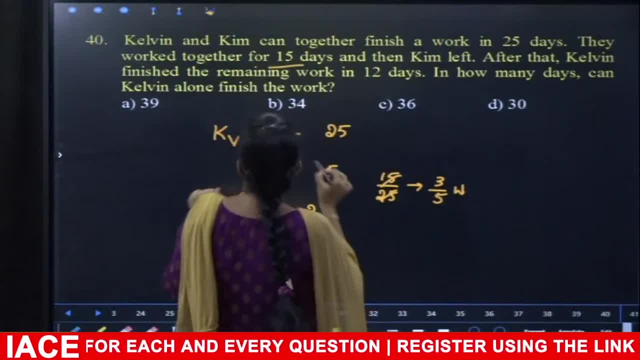 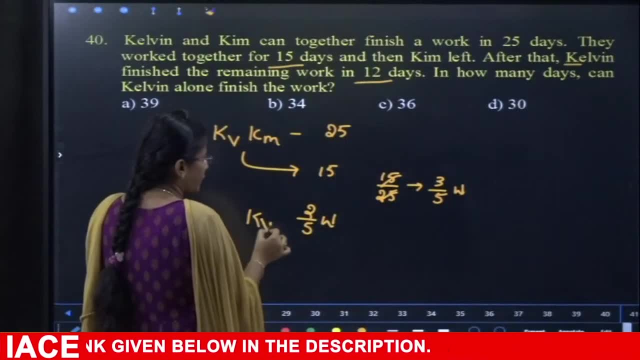 It would be 2 fifth of the work. That 2 fifth of the work was completed. Remaining work was completed. Who completed it? Calvin completed it. In how many days did he complete it? 12 days. So Calvin completed 2 fifth of the work in 12 days. 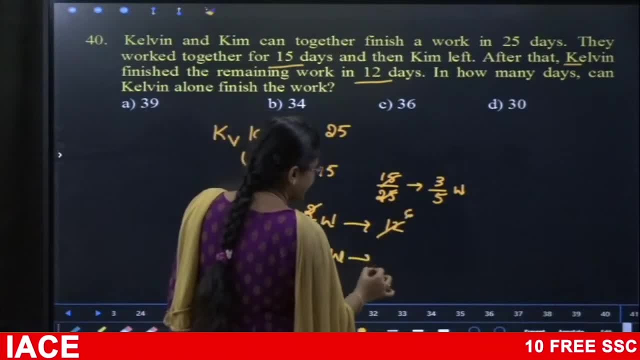 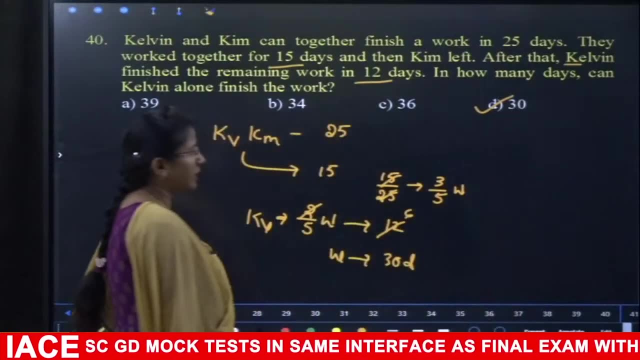 So that will be total work to be completed, He asked. so the answer is 6,, 5, 30 days. Okay, Option is 30.. Option is 30.. Okay, 3 fifth and 2 fifth were completed. 12 days were completed. 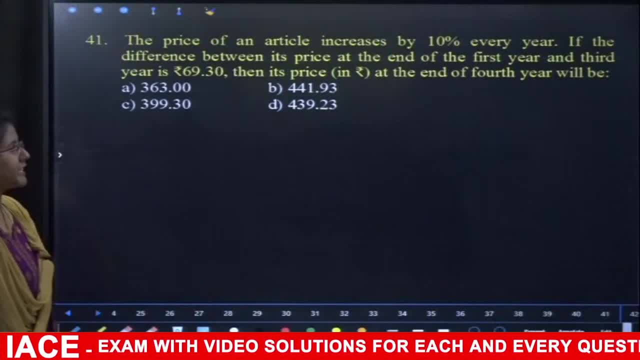 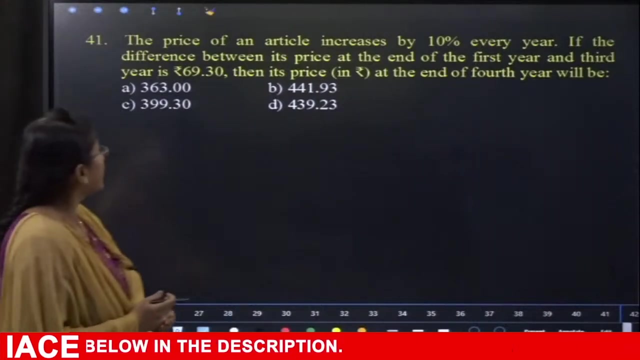 Total work was 30 days, Next one 41. Try it 41, 30 seconds timer, please, Okay. Okay, your time is up. Your time is up, So, equation, we will do it. 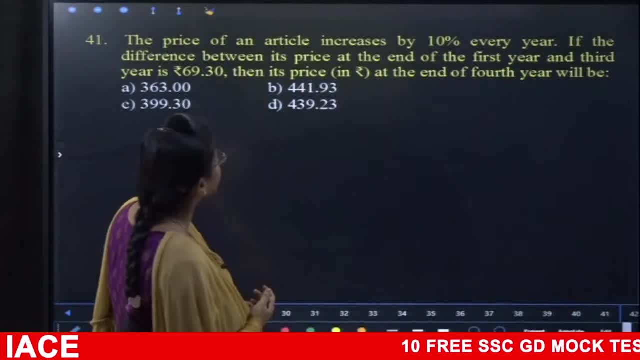 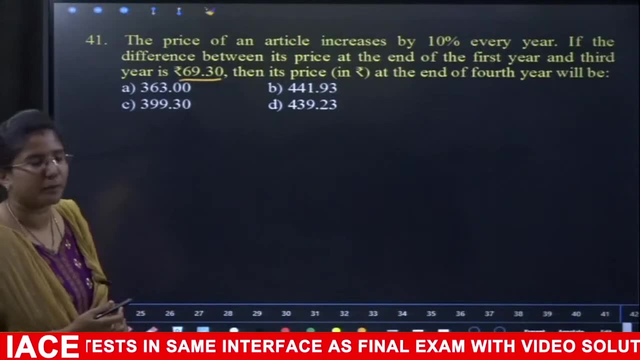 Price of an article increases by 10% every year. If the difference between its price at the end of first year and 3rd year is given 69.3,, then its price at the end of the fourth year will be: so every year. 10% increase of those Sunni. so in first. 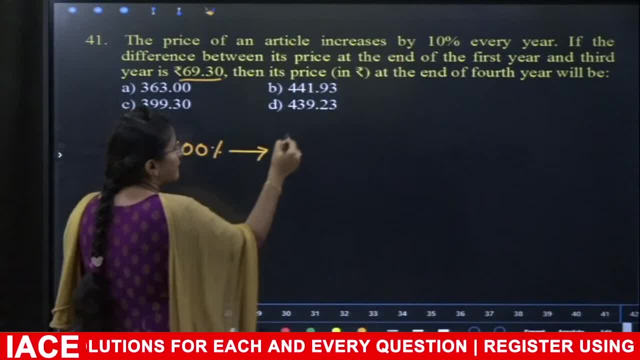 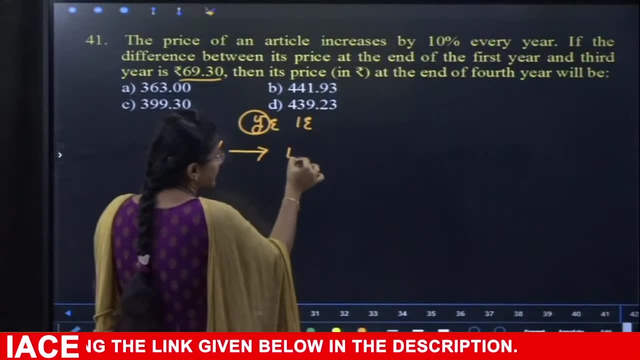 rastan, if it's value is some hundred percent only, and Kunti, first year end. coaches are key here and Radha money here and the first year and coaches are key. and though to the hundred key 10% pinch, then the yes, 110%, even 10% meta. 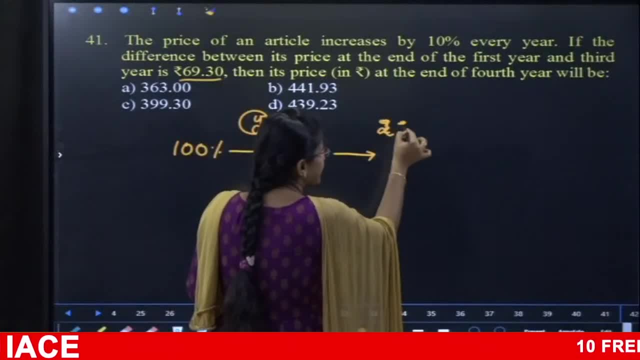 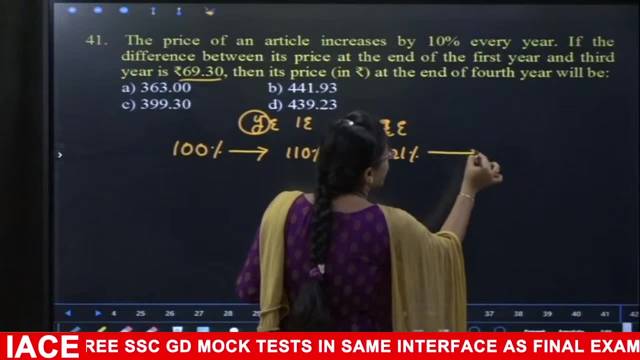 second year and coaches are key second year. and then one thing with a 10%- leonard chest and told me 120, one person top. next second year ending church in value in cook of one year key third year and also in third year and doctor key, okay, ten percent, twelve point. one man watches say that is totally one. 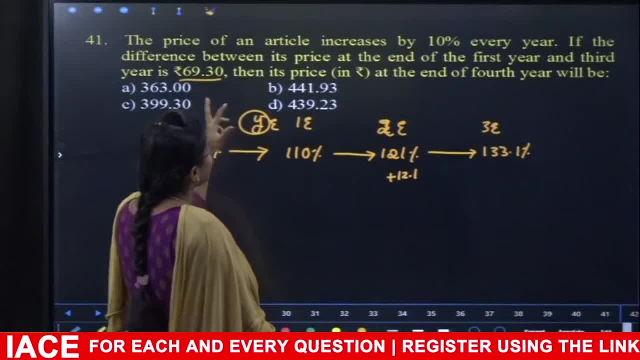 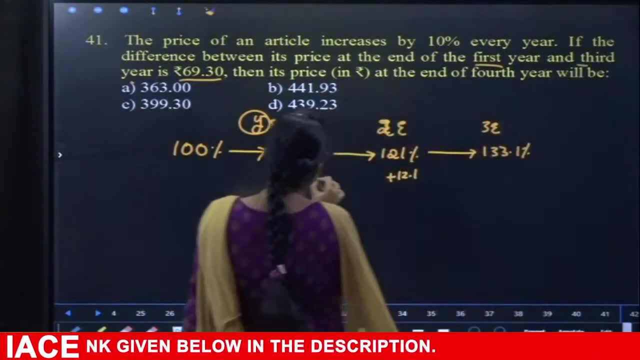 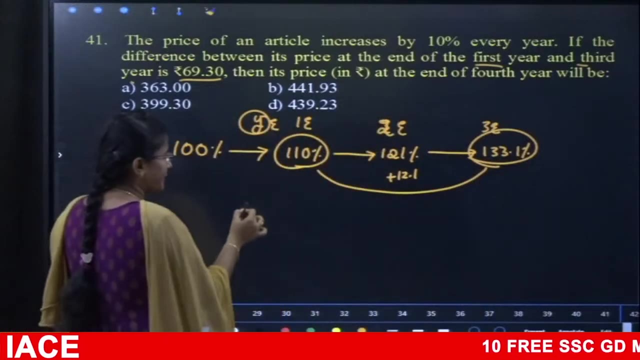 three, three point one. person, money, kitchen, be at the end of first year and third year here in two years can much a difference each other in the first year, third year. first year is 110, third year is 131, 133 point one. so entity minimum difference has not, like they and the person to the, yes, 23.1, 23.1 percent. 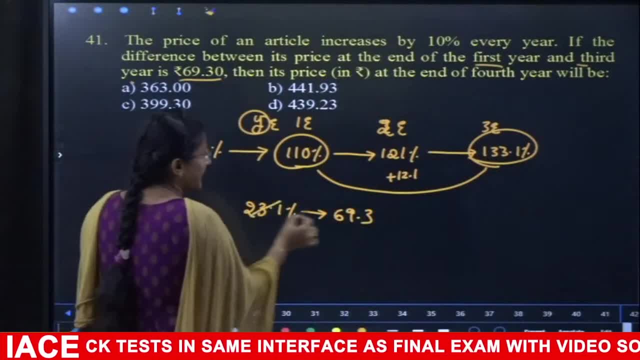 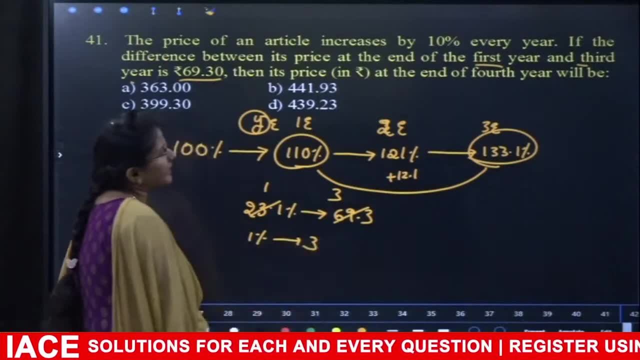 value each and then the cc9.3. it exactly cancel ever many times, three times can. so what person to value 3i net, like the question on the four year end of the courier, on the four period, any circuit upcoming one thirty three point one matter extra: the money. 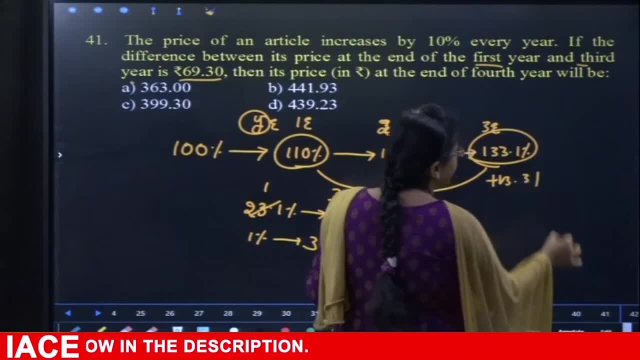 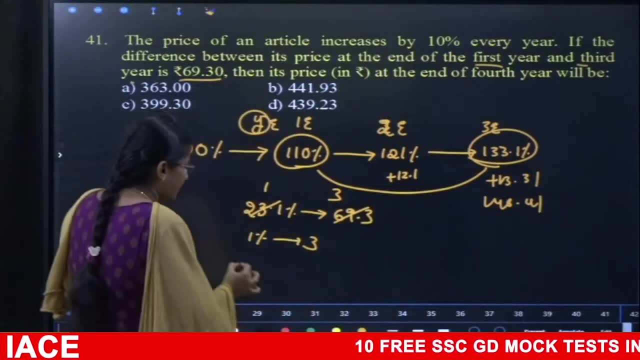 ten percent at challenge, actually thirteen point three, 110 percent actions at late date. so to tell you, one forty six point four, one percent, so one person in today, one point one forty six point four, one percent percent value will be then simply three to multi, pleasure to me, three to. 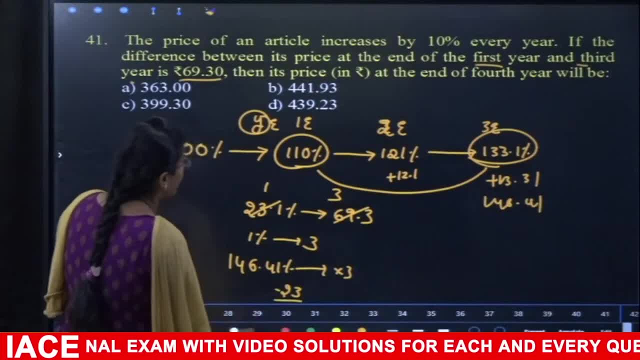 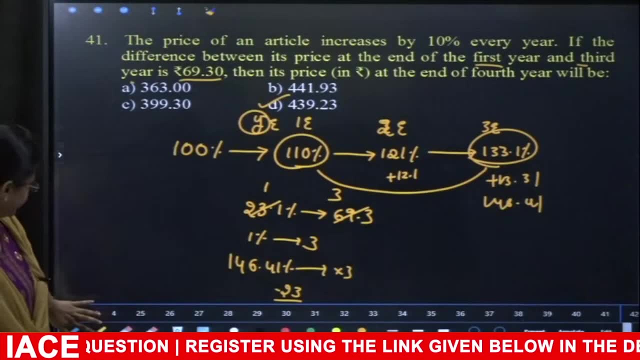 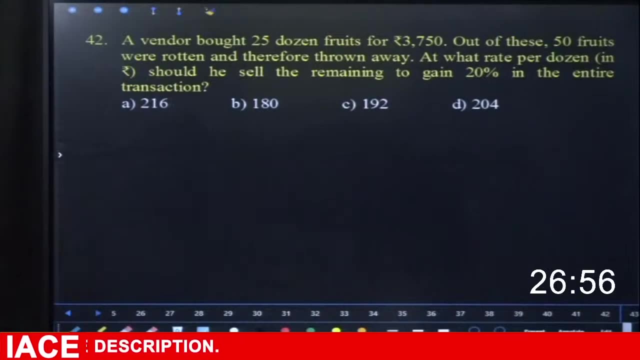 multiply. sister Monica cut a three to you know, does it look? wine to two, three, ocean and a lot of option on the option D for thirty nine, point two, three, okay. next go for forty two, thirty seconds time. oh, please, you okay say: vendor bought twenty five dozen fruit, set three thousand seven fifty out. 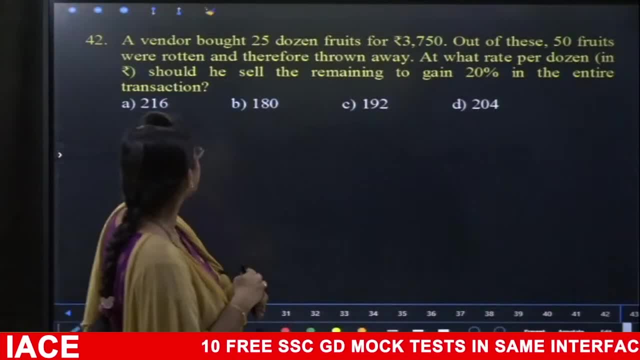 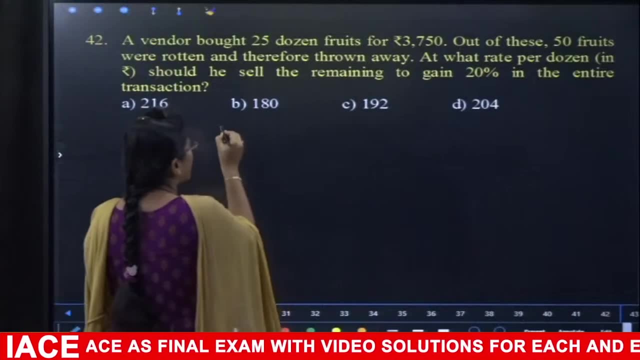 of these fifty foods were wrote in and therefore thrown away. at what rate per a dozen should he sell the remaining to gain twenty percent in the entire transaction? so twenty five dozen fruits and the entire number of fruit. so doesn't get well, get a. twenty five dozens will be twenty five, twelve. so how many fruits? three hundred fruits, three. 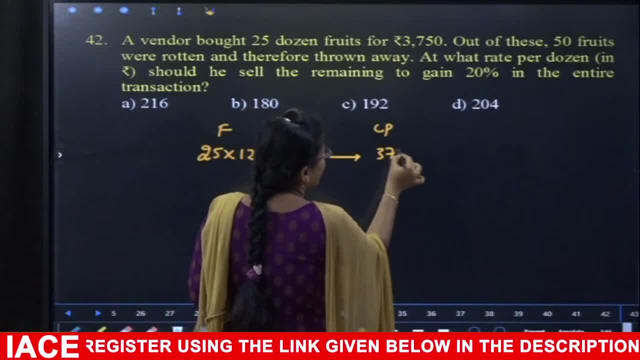 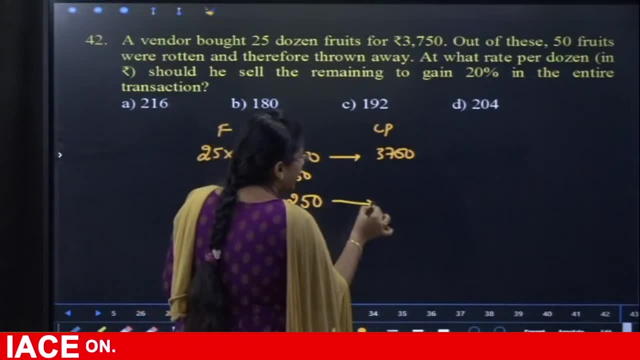 hundred fruits, keep on the cost to present each other and a three, seven, five, zero already in the low money, 50 roten and a party boy. they are thrown away, remaining any fruits and a 250 fruits and a a 250 fruits, me and the cell. 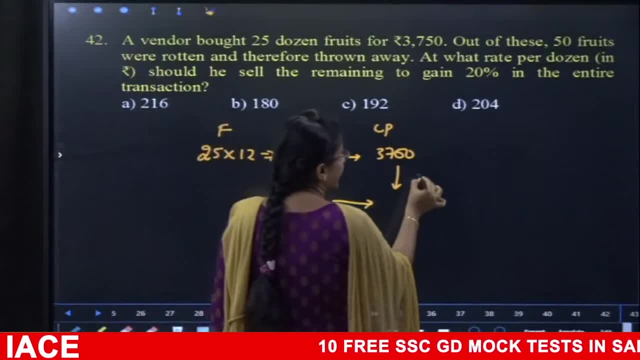 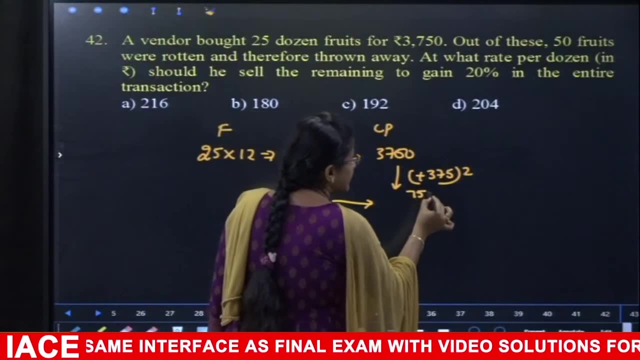 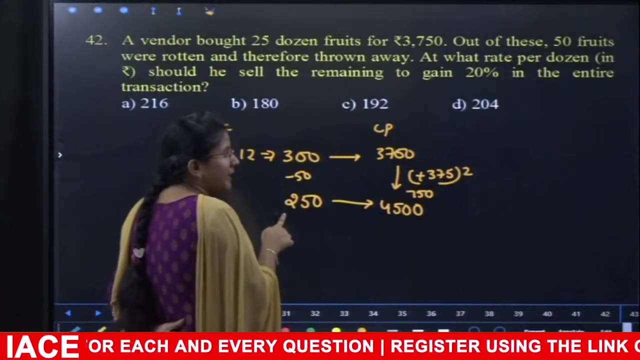 challenge to the twenty percent gain, Ravali, twenty percent gain and take already you know, three, seventy five, double, change the three, seventy, five, zero. we have to be how much? seven, fifty, three, seven, five, zero, key seven, fifty. I just some and a party price on the 204 thousand five hundred and to 250 fruits. 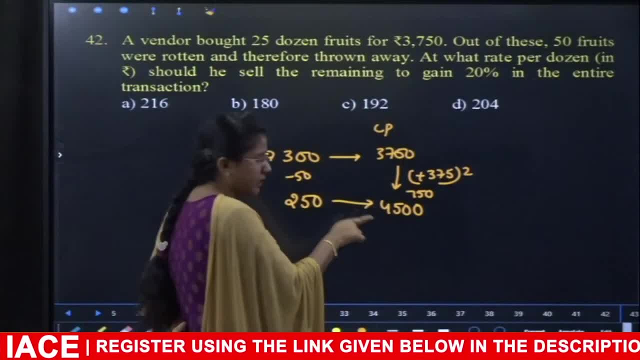 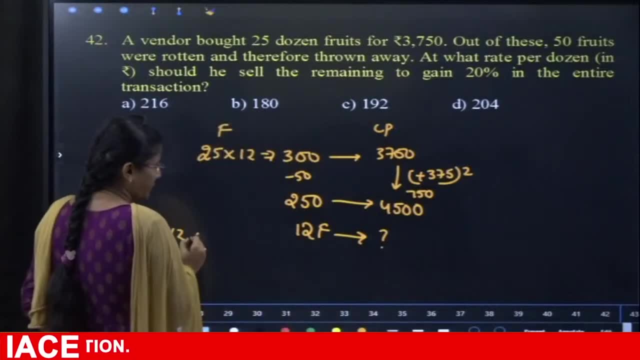 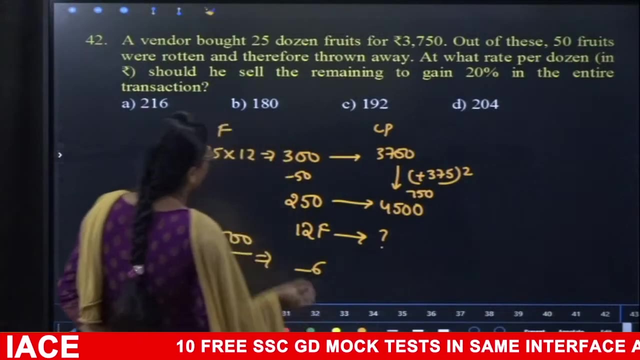 me four thousand five hundred. key fällt up and profit us, and then two fifty people thousand five hundred. I think money doesn't water gotta well free to enter my door chest on. so that will be twelve into four five double zero by 250. so you know, does it. on the new sources, six goes from the six such option of today, um. 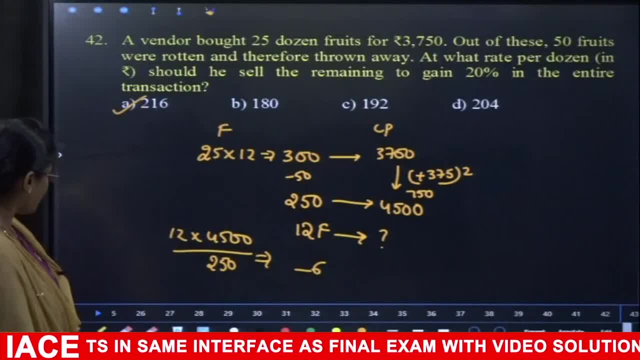 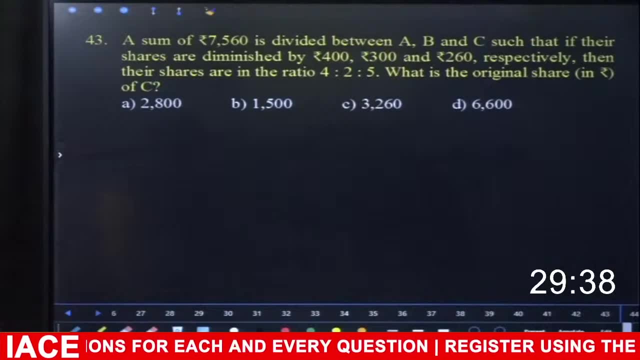 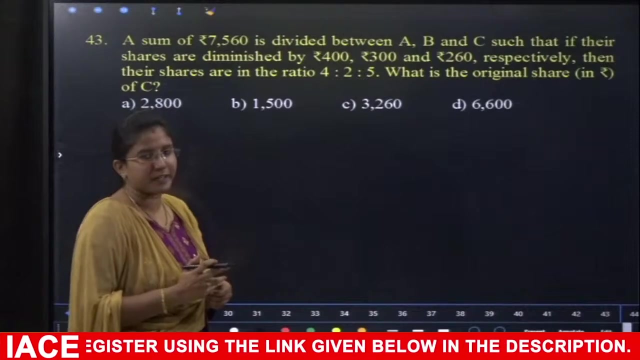 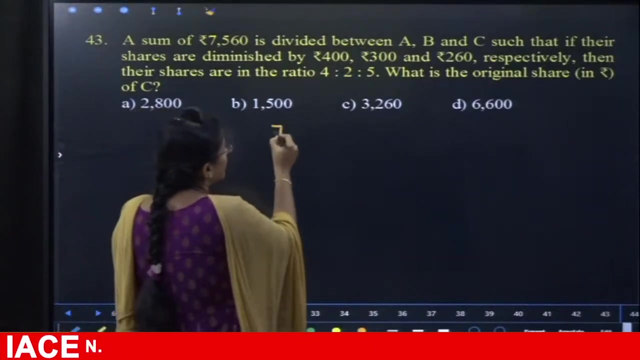 you. that is the 216. okay, next go for next one. 43, 43, try shiny 30 seconds timer please. okay, somehow 7560 is divided among a, b, c, such that if their shares are diminished, diminished and decrease over them, so amount each in the total amount. 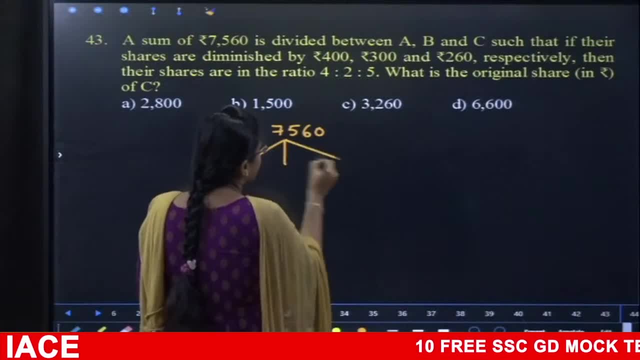 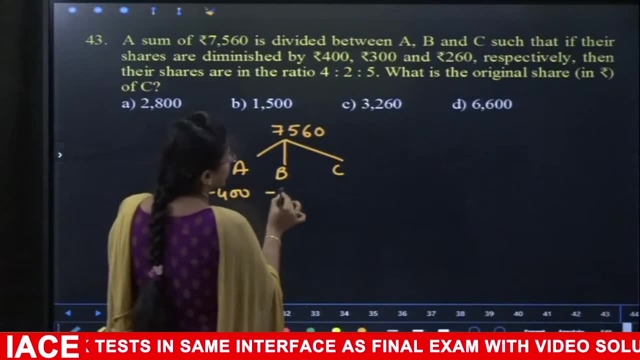 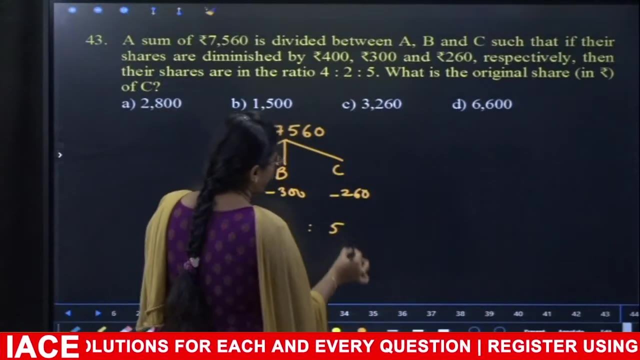 will be 7560, we'll end the money. divide chasm until we divided among a, B, C, such that while a shares me mission to reduce chasm and the an inch of a 400 being each, 300 seen into 260 deduct chases, they while reminders ratio alone and a 4 is 2. 2 is 2, 5 total amount. 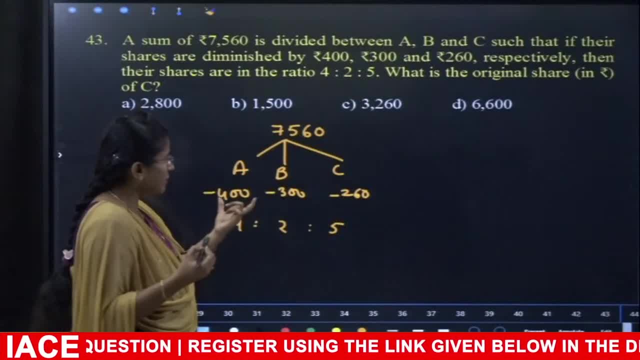 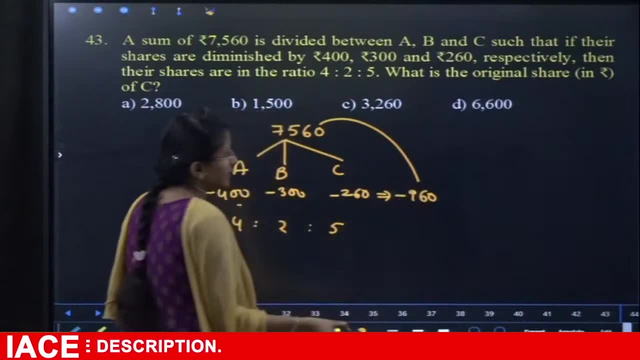 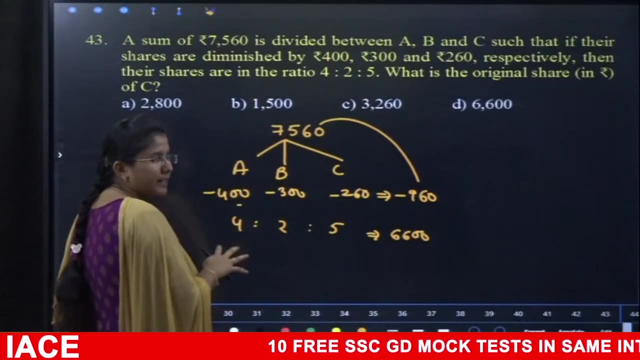 to the government in the launch amounts overall call. if you did a chaser them, so overall you could 400, 300, 700 plus 260. overall got 960 for 7560. launch is 960, deduct chases, not like the remaining amount. that is a 6600, so 6600 erasure. 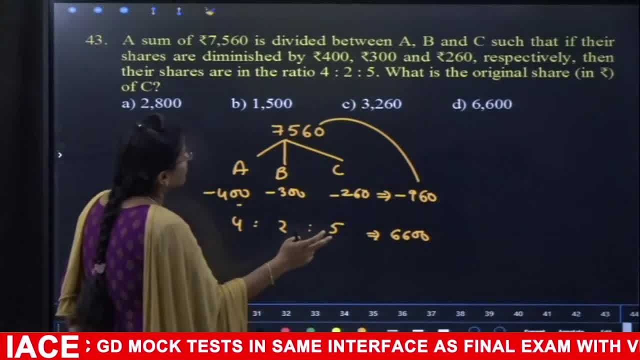 low divide chasm model. so 4 plus 2, 7, 4 is 2, ratio is 4 is 2, 2 is to 5, 6, 4 plus 2, 6 plus 5 total: how many parts? 11 parts, 11 parts. 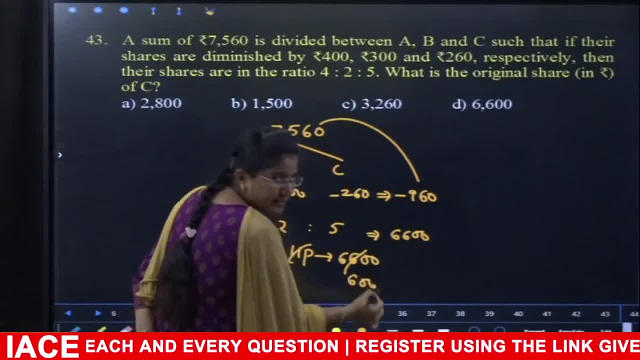 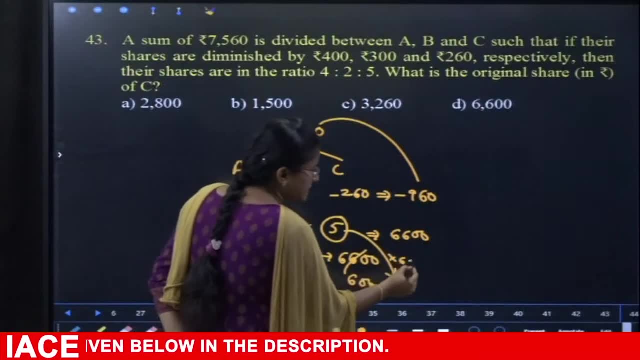 6600, I did. and what is the value of one part, one party, 600, all these three major question, the gobbledy original share of C озера, so you can remind, rent on and a five into six hundred. that is what, 3,000, 3,000 to deduct, chaser, there were the amount 30 original. 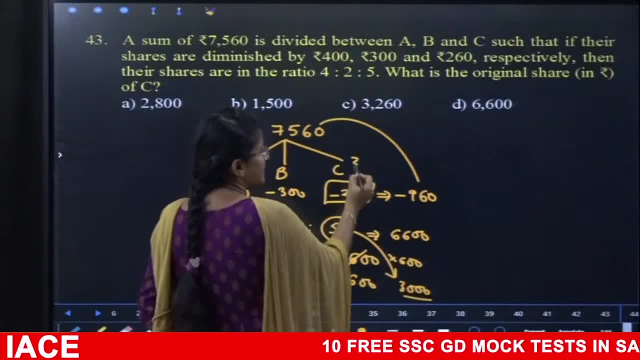 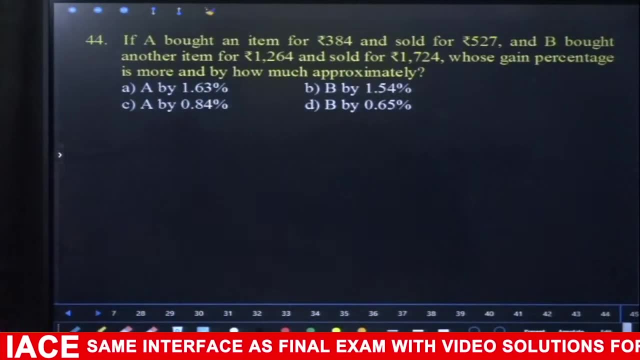 etiquette ka, but they are two, six, to my mind by system. so I just answer: is three, two, six, zero option. okay, next 44, try shine Andy. 30 seconds timer, please you. okay, your time is up. question is the easy question: a profit person days, calculate chassis and the ever kick coach in the ever Kimura, Jeff Ali. but 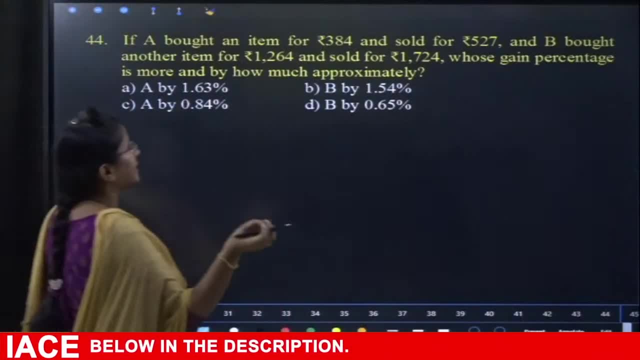 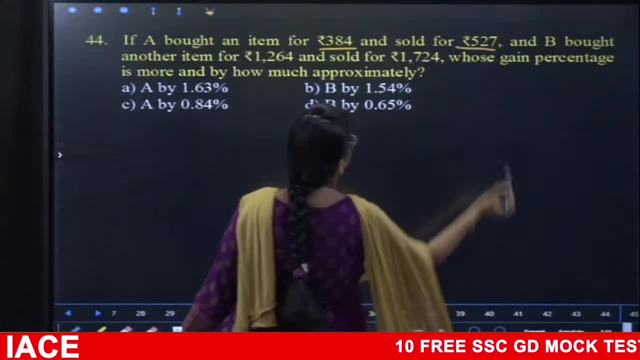 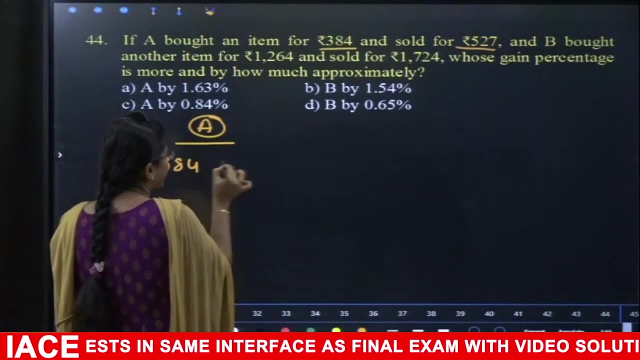 numbers are bit odd: consume calculation, low monkey costs, flexible, cancel out shares in the movie. so here, if we a bought 380 for 84 rupees and sold for 527 rupees, so a the group some money in cheer cost price, which is, you know, to cost price is 380 for and selling prices by 27. next to be the 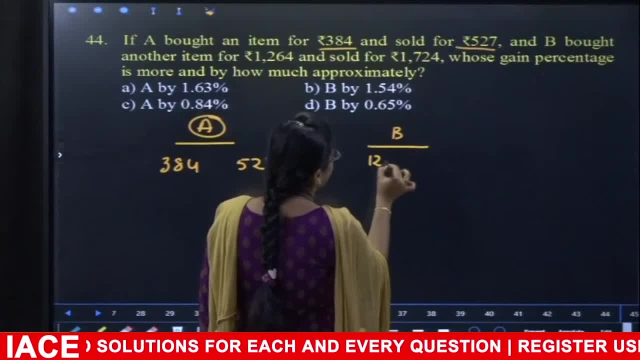 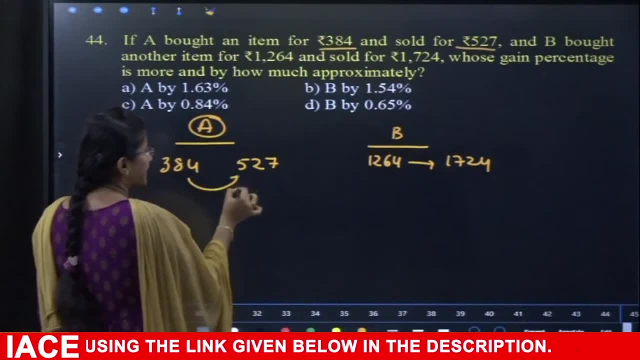 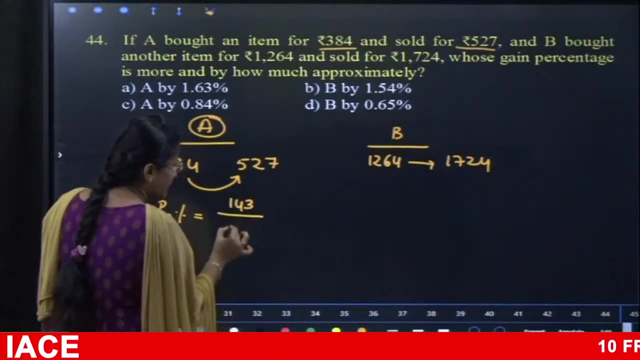 other coaches are key. be bought it for 1264 and sold it for 1724. so be a key profit of chimney. be a key profit of chimney. so profit person days calculation up to profit percent of a will be different student. I make a difference money given 43 by cost prices, some 384 into hundred. next you could. 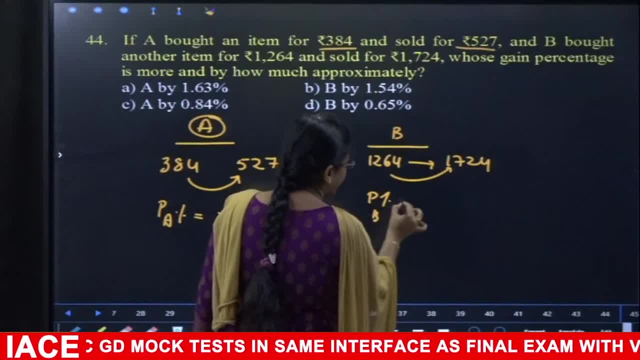 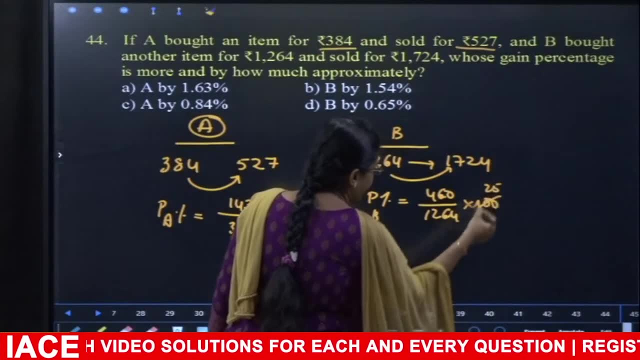 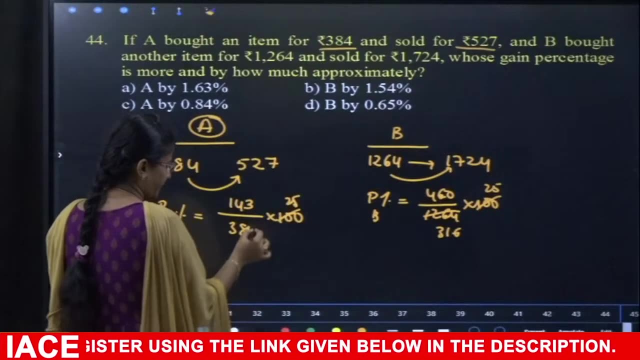 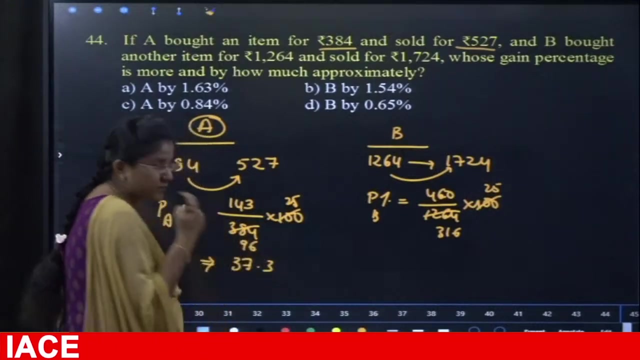 difference which money for 60, difference home the profit person of for be will be. that is of 450 by 1264 in 200. so the common follow loco one time for all right mainstream mêmes Св 7.3 a loss and handy kauphongir. 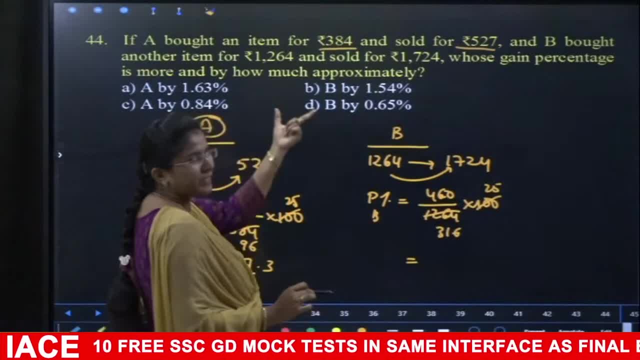 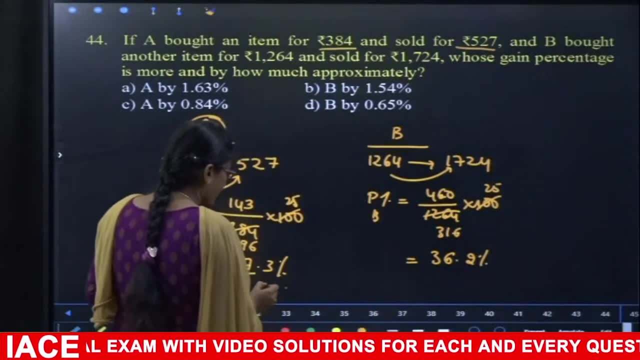 are you? If we look at the digits we can keep the answer nearby. So here it is 36.2%. So the difference is: if the profit percent is more, then the A is more, So the difference will be nearest to 1.. 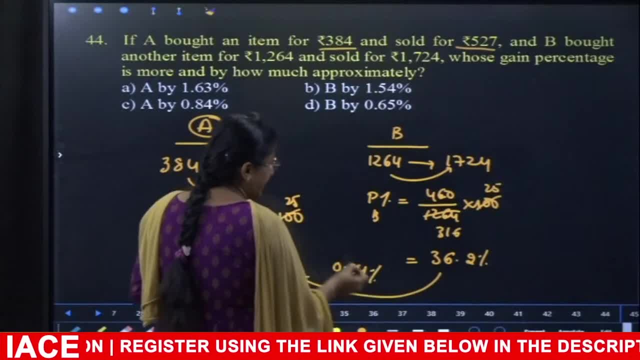 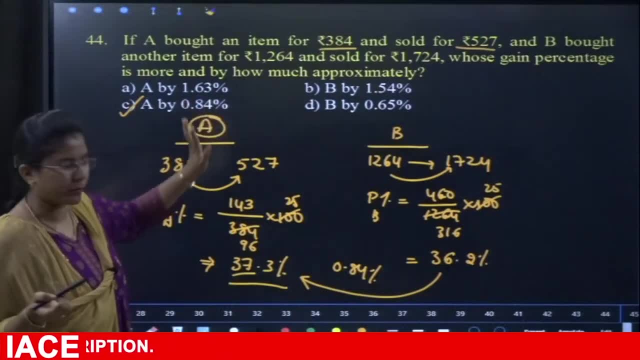 There is only one option, that is 0.84.. Option A, where the profit percent is more, is nearest to 1 multiple, That is 1 is 0.84.. Okay, Next question: 45.. Try 45 for 30 seconds. 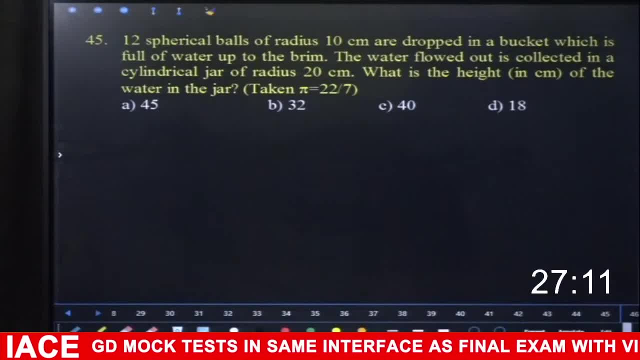 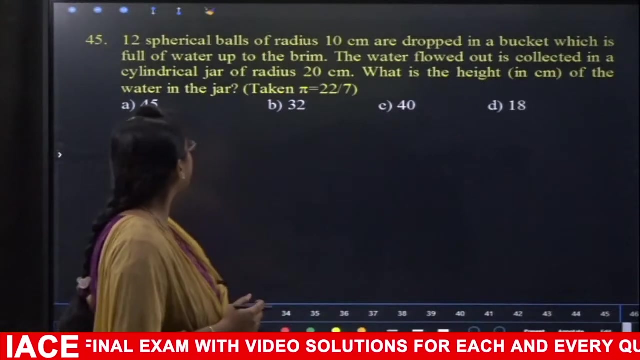 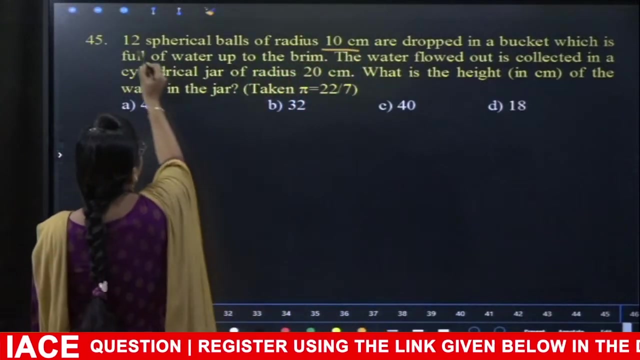 Timer, please. Okay, So 45.. Your time is up, So 45 is the consideration bit. 12 spherical balls of radius 10 centimeters are dropped in a bucket which is full of water. 12 spherical balls means 12 spheres. 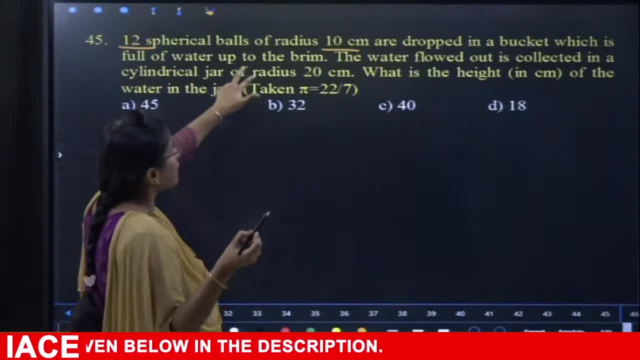 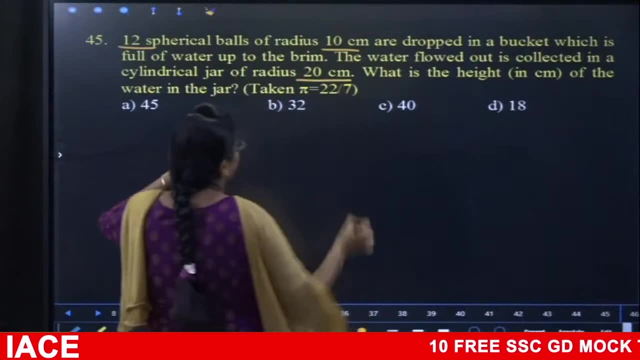 Its radius is 10.. So when we drop a bucket full of water, water flowed out and it is collected in a cylindrical jar of radius 20 centimeters. The volume of the balls is the same as the volume of the water which comes out of the water. 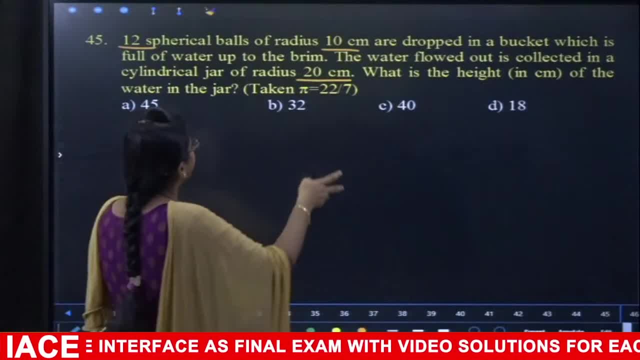 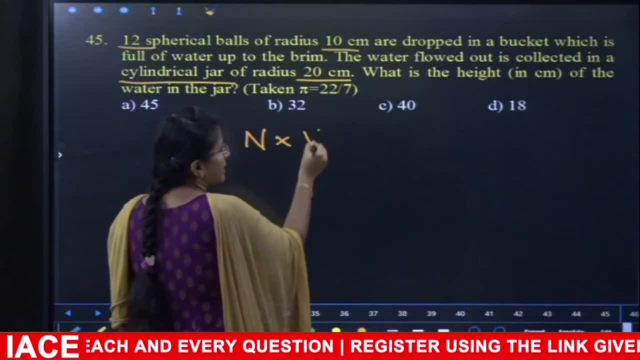 So we should not look at the figure of the water. What did he say? He said it is a cylindrical jar, So use nothing but A. Any balls means any balls. So the volume of the sphere should be equal to the volume of the water which comes out of the water. 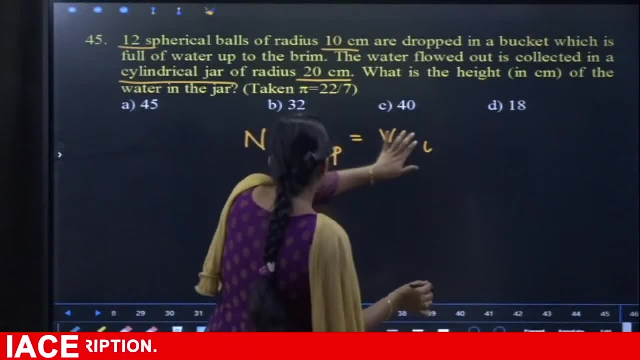 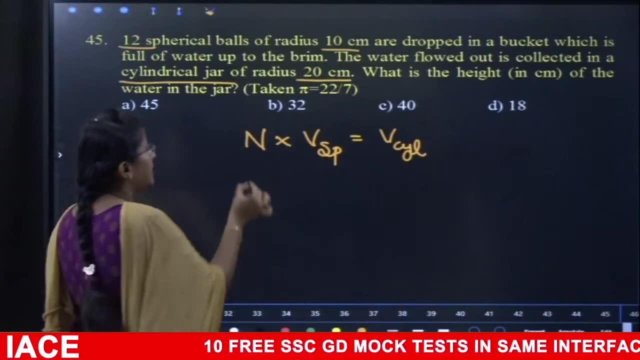 The volume of the figure in which you are filling the water, That figure. That figure should be equal to the volume of the cylinder. The volume of the cylinder should be equal to the N volume of the sphere. So N value has already been given to us. 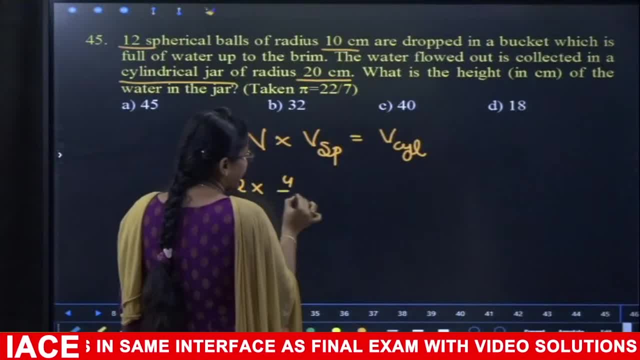 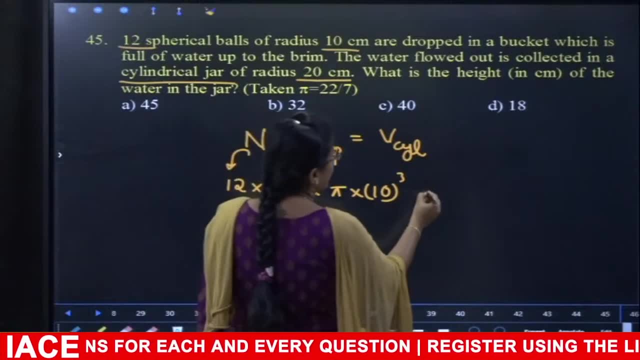 That is 12.. We know the formula of the volume of the sphere. What is that? 4, 3rd pi r cube r is given as 10. 10 cube, Okay. Next, the cylinder volume value is pi r square h. 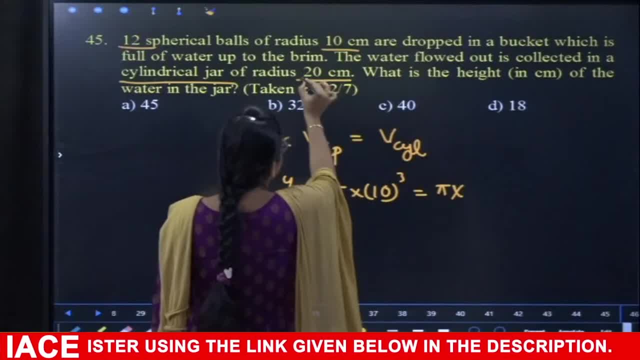 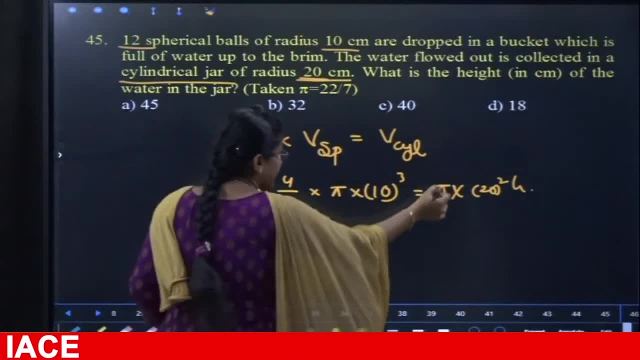 Let us keep pi as it is. It will get cancelled. What is the radius given to the cylinder? 20 square. He is asking for the height given. He is asking to find out the height value. He will find out. So pi will be cancelled out. 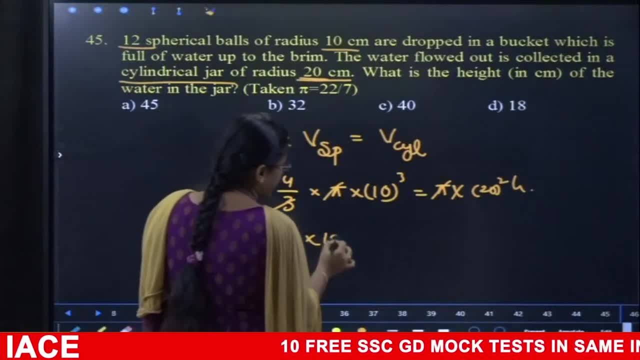 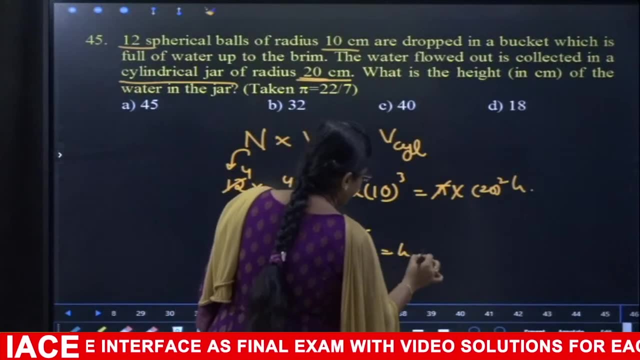 And next 3. This will be for 4 times, So that is 16 into 1000. by height, h will be There 20 square is there 400.. If we cancel out the zeros, that will be answer 40.. 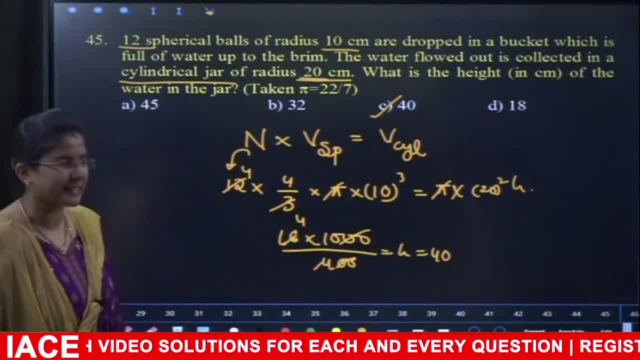 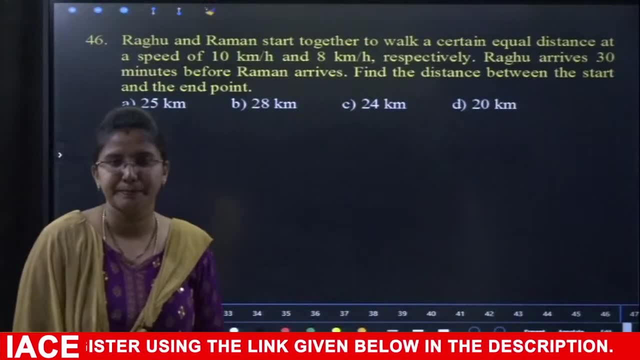 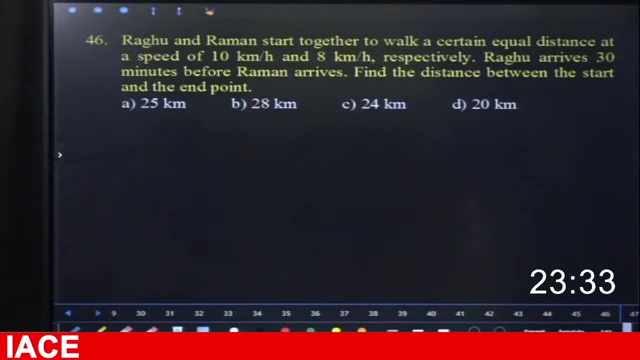 Height is option C, 40.. Okay, Very easy equation. Next we will solve 45.. Try 45.. 30 seconds timer, please. Okay, Your time is up. Very easy equation, Simple equation From time and distance. Raghu and Raman start together to walk a certain equal distance. 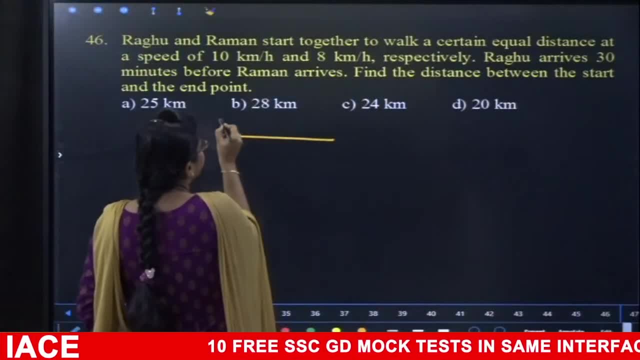 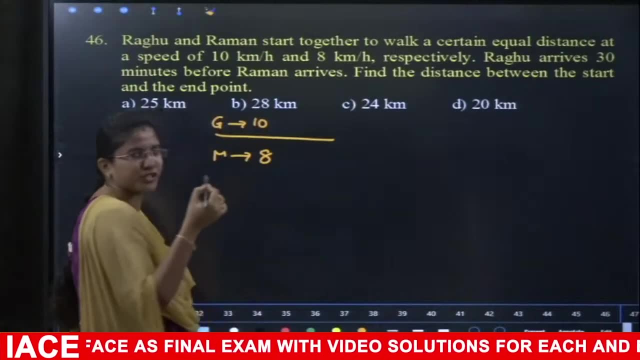 Distance is equal to power. a certain distance Raghu traveled at a speed of 10 kmph And Raman traveled at a speed of 80 kmph. I am denoting Raghu with G and M, So speeds ratio is same distance. 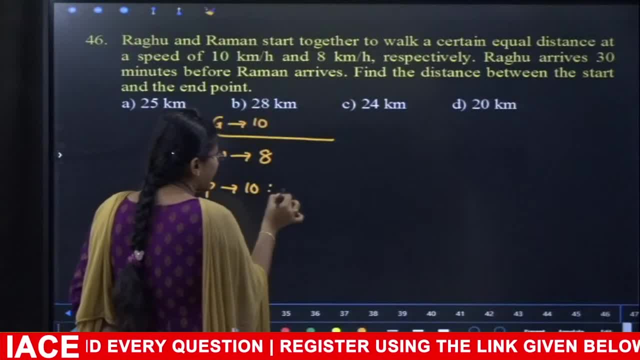 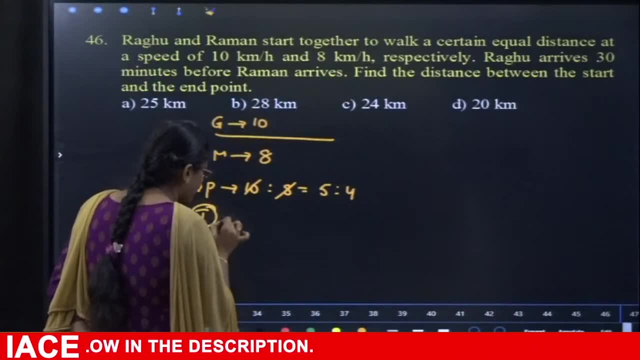 So their speeds ratio is 10 is to 8.. What is the ratio? 5 is to 4.. If speeds ratio is 5 is to 4, their times ratio is inversely proportional. That will be what 4 is to 5.. 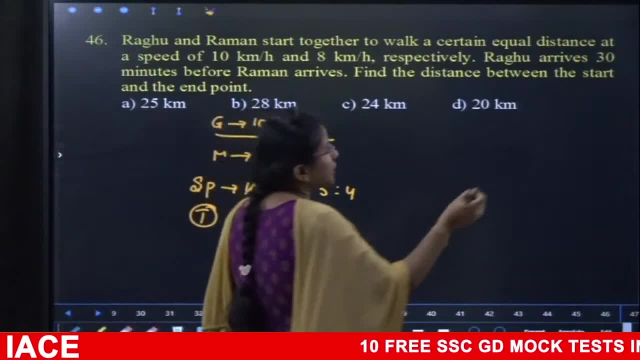 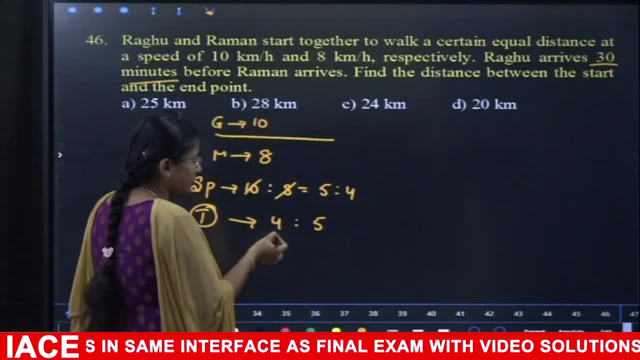 To cover the same particular distance. Raghu arrives 30 minutes before Raman. Raman is half an hour ahead of Raghu. So how many parts did Raghu go earlier than Raman? How many parts did he go earlier? One part. 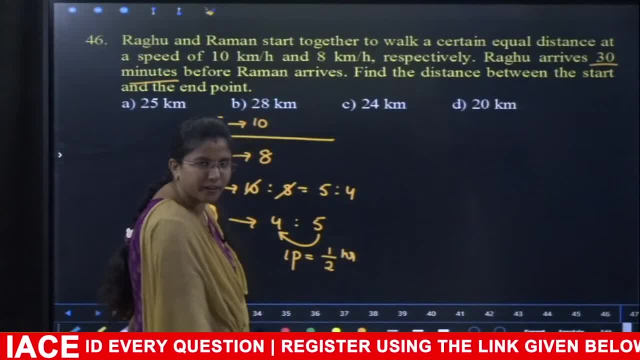 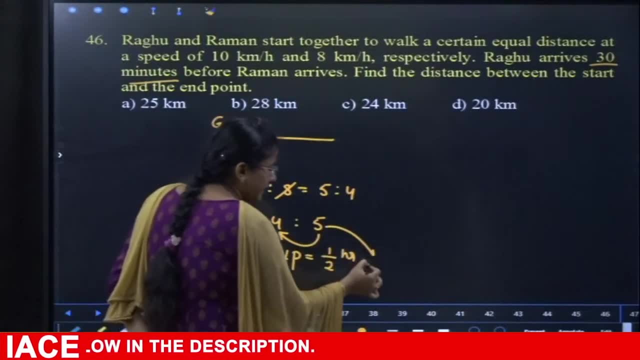 How many hours does one part equal to 30 minutes is half an hour. One part is half an hour. So how much time did Raghu take? 4 into half, that is 2 hours. And next, how much time did he take? 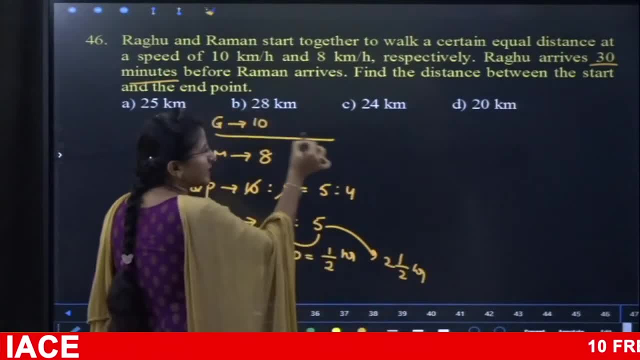 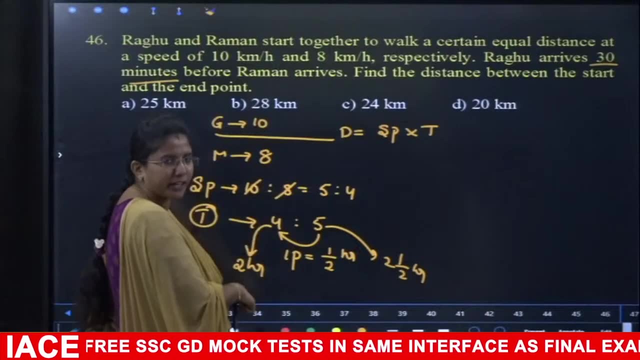 2 and half hours. So, since he is asking the question of distance, we know the distance. What will we use? Yes, Speed into time. Who will take the speed? Multiply by the time taken by them, Since I am taking Raghu. 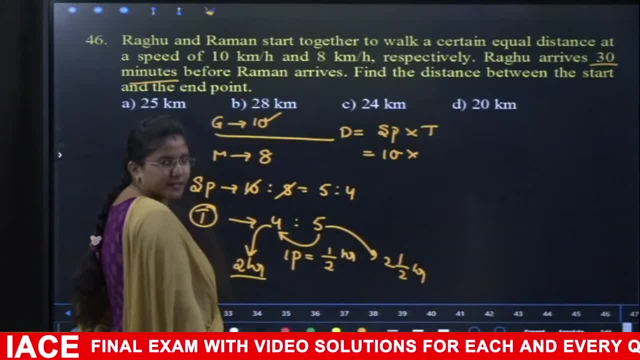 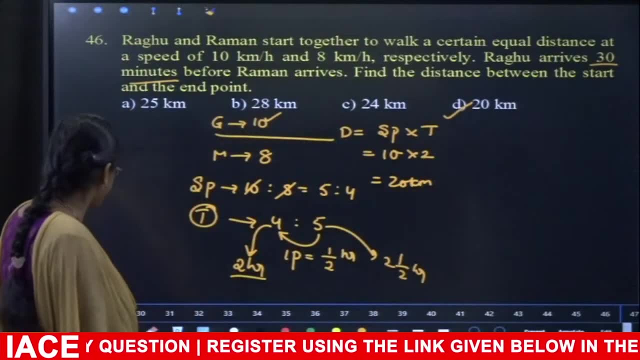 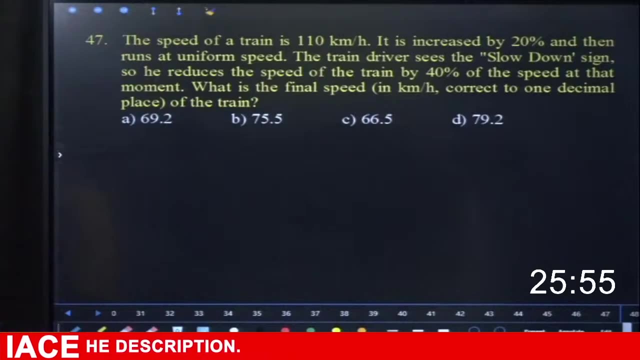 speed is 10 and time he takes to complete the distance is 2.. 10 to's answer is 20 km. Option D: Okay. Next Go for next one, 47.. Please try 30 seconds timer, please, Okay. 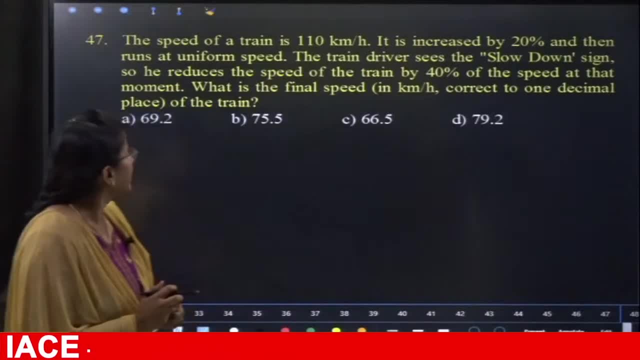 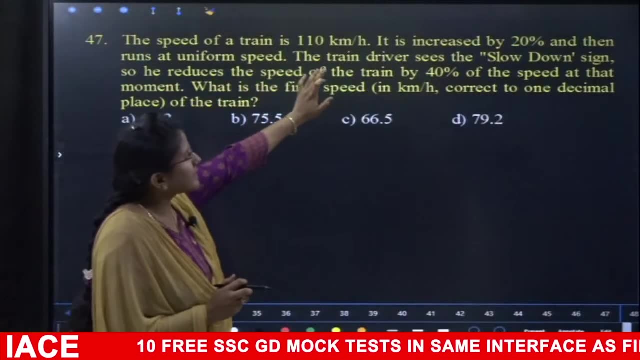 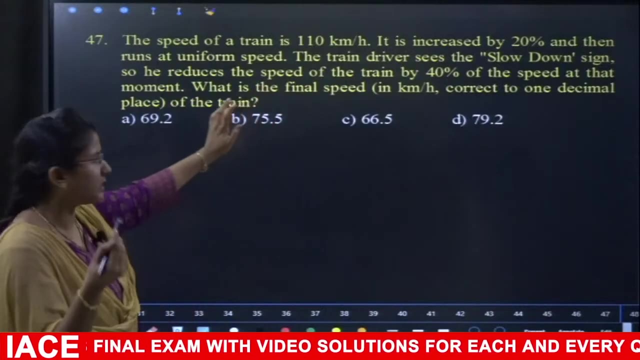 Okay is up. so here: speed of a train is 110 kmph. it is increased by 20 percent and runs at uniform speed. train driver sees the slowdown sign and reduces the speed of the train by 40 percent back in time and distance of train, so can't listen to me. I mean later in the local number, each other 110. 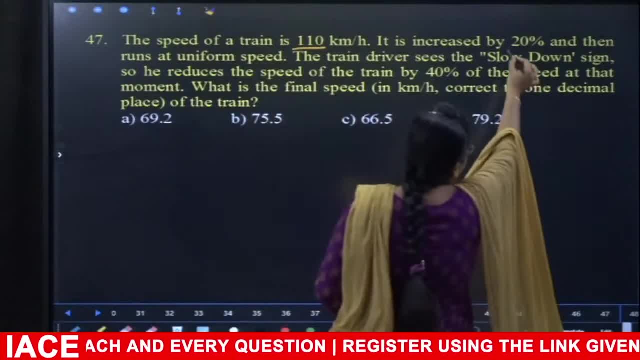 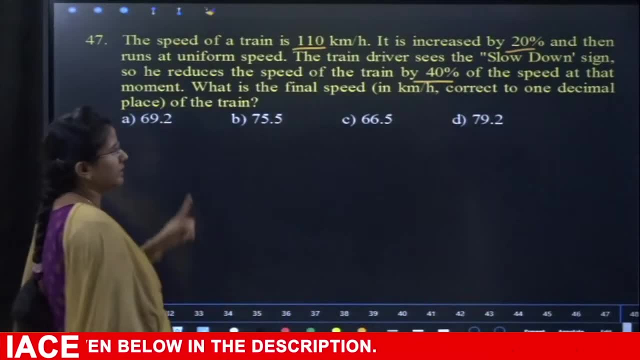 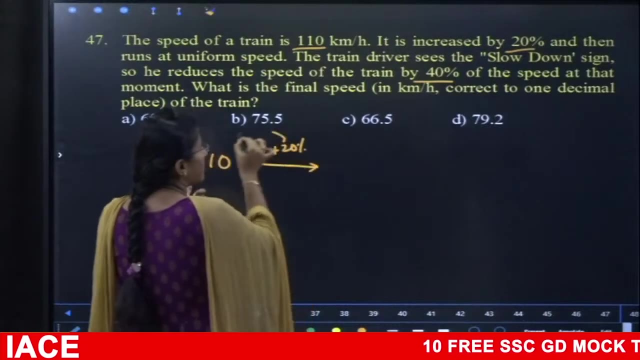 kph speed. me then the first, it is increased by 20 percent. another other, Ratha. he then reduces it by 40 percent on a number each. a first 20 pinch to them throughout 40, second a month. a Danny final speed of a do to not cover T initial 110 kmph. Medha man, 20% increased. a state 20% value on this. 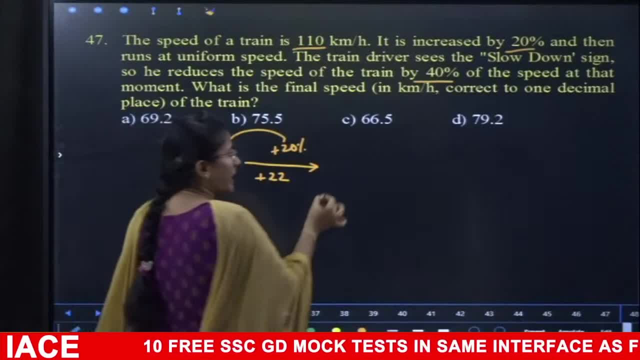 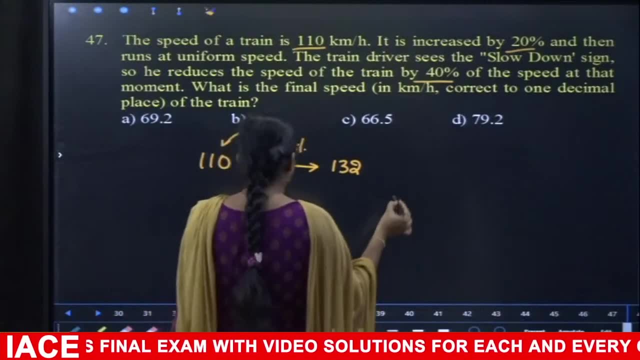 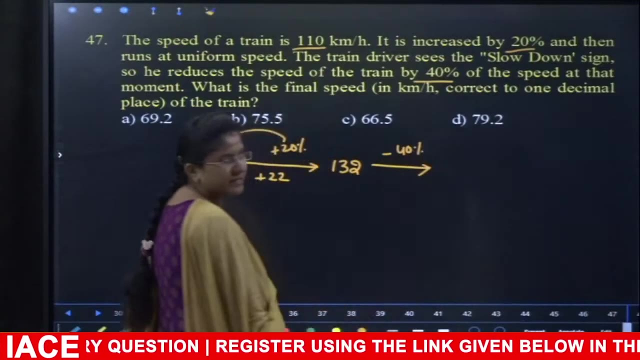 will be how much? 20 to 22 our chest and the speed of Nandi, 132 a 132 kph me. these are in ancient modern day. he told us to reduce it because of a slowdown signal. to say I do say sad that get shadow minus. and the person that gets Charlie party person that gets Charlie 40% value on this. 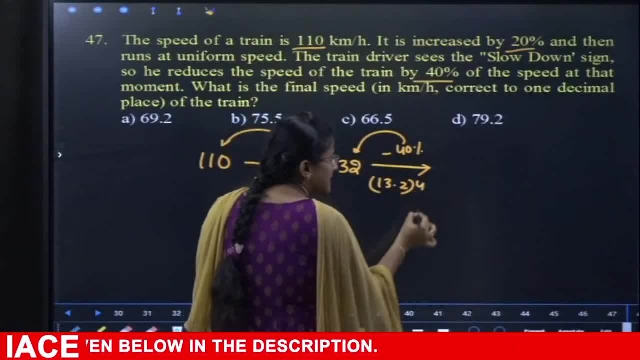 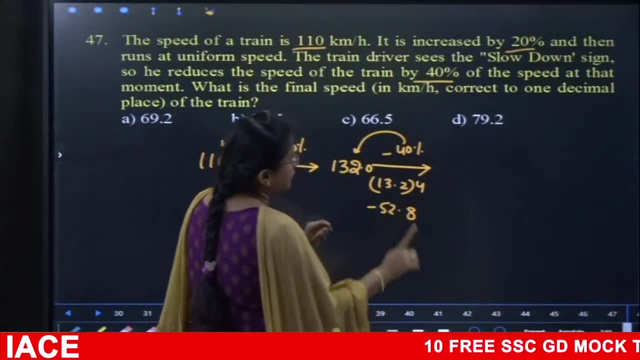 will be 10 percent at a 13.2. only four times a circuit, as that's the 52.8 that the child of the minus system unit. is it a manicure zero? and to me the rate of 22 and options are in the comparison I got in one chair is in. 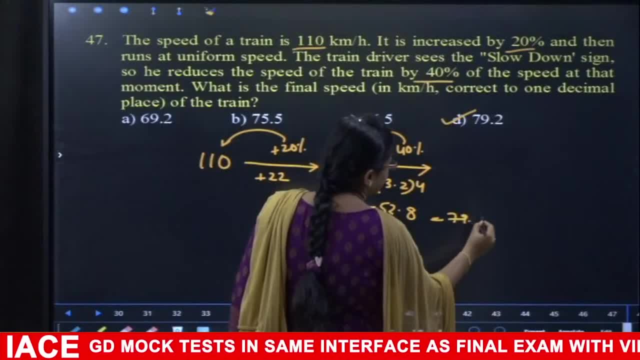 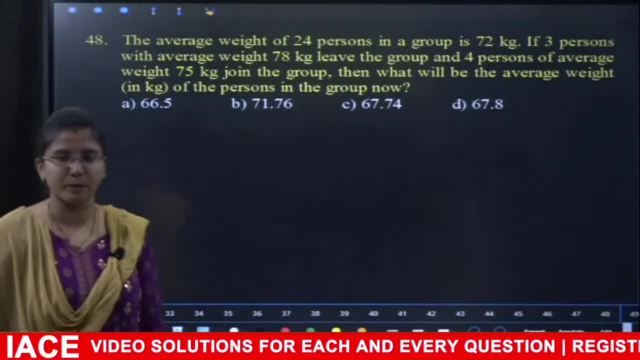 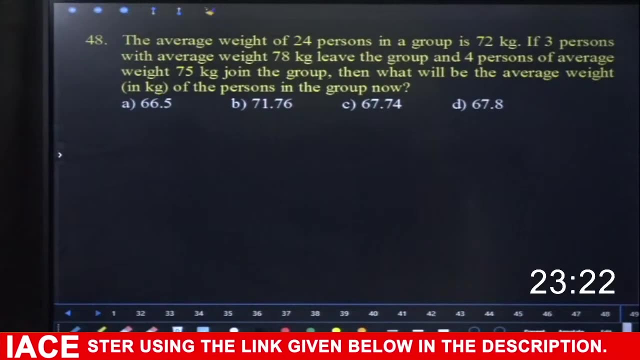 the option: 79.2 minus Chester cancer: 79.2. okay, go for next one: 48 30 seconds time. oh, please you. okay, your time is up so I will just topic ninja question: only a group of people: normally key average rate of damage. okay, your time is up. so average rate of stepping in question on the group of people: normal key average rate of. 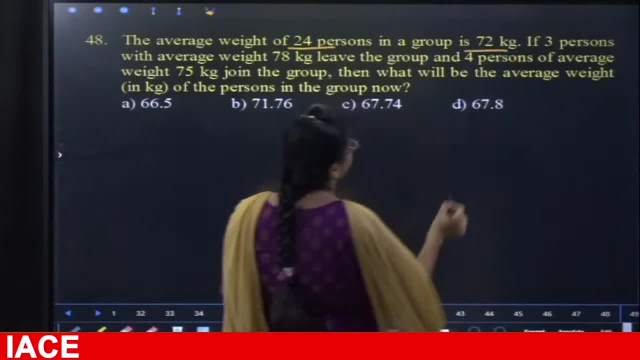 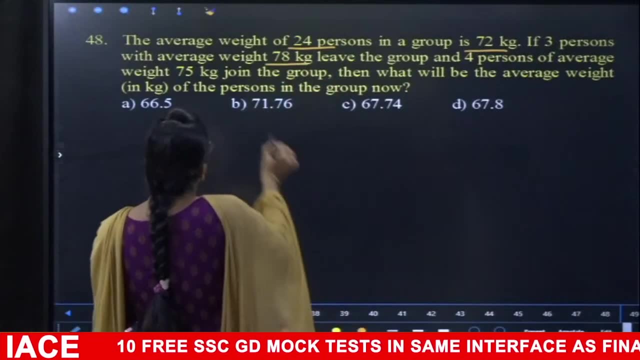 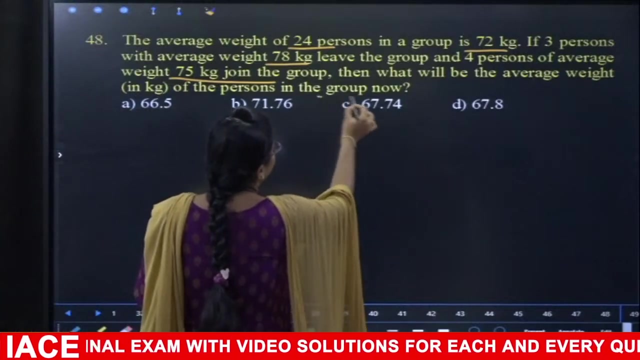 If 24 persons is given as 72 kgs, if 3 persons with average weight of 78 kgs leave and 4 persons with average weight of 75 kgs join. some are exiting and some are entering. what is the average weight of the group now? 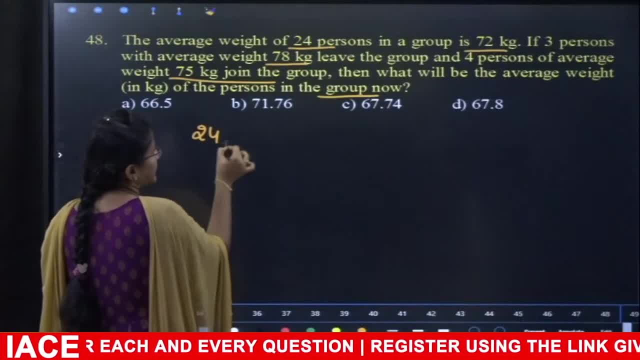 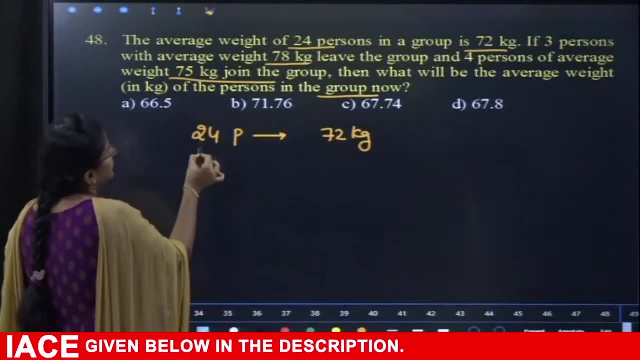 They are asking: what is the remaining person's average weight? So let's write that First. there are 24 persons starting. What is the average weight of all of them? It is 72 kgs. So, from these 24 persons, if 3 persons with the average weight of 78 kgs leave the group, 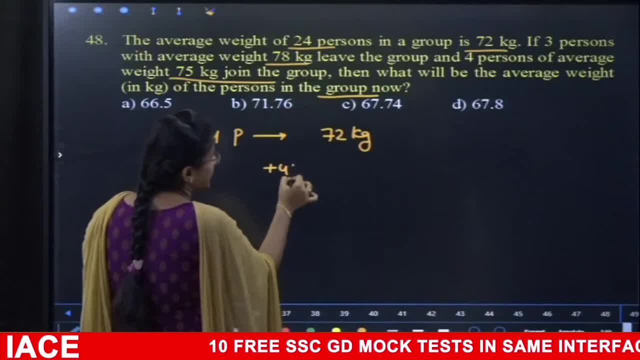 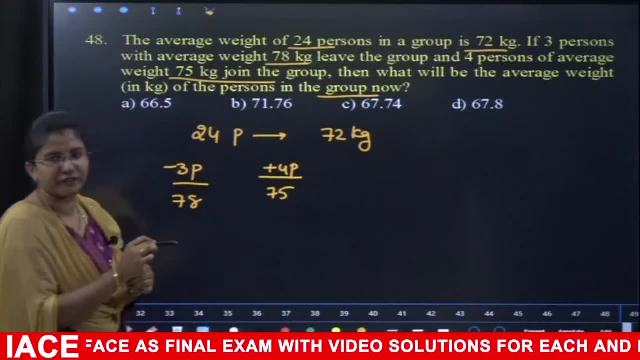 3 persons are leaving from this group and 4 persons are joining. The average weight given to them is 78 kgs. The average weight given to these 4 persons is 75 kgs. This is the information in the overall question. 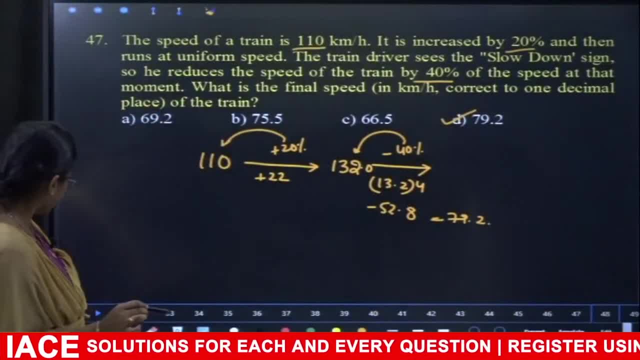 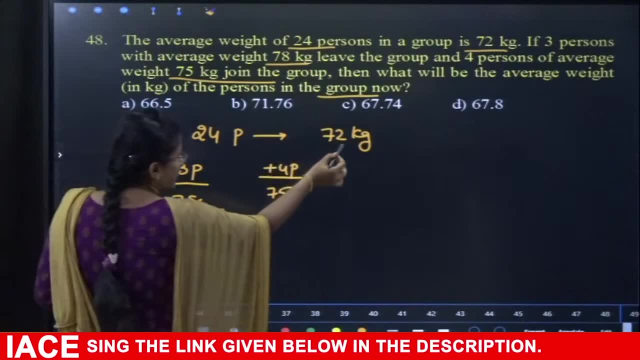 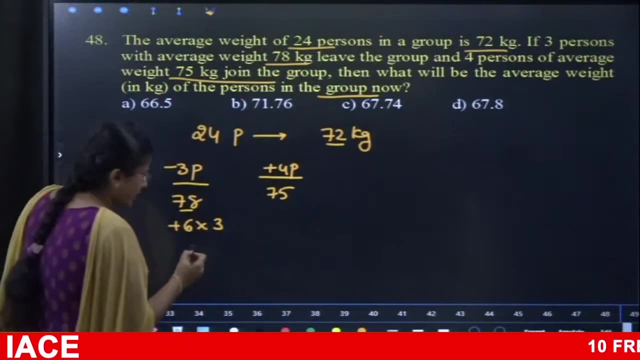 So we will just compare with the initial average and find out the deviations. So if we compare with these 72 persons, 78 kgs is an increase. How much extra is there? Each person has 6 extra. How many people have these 3 persons? 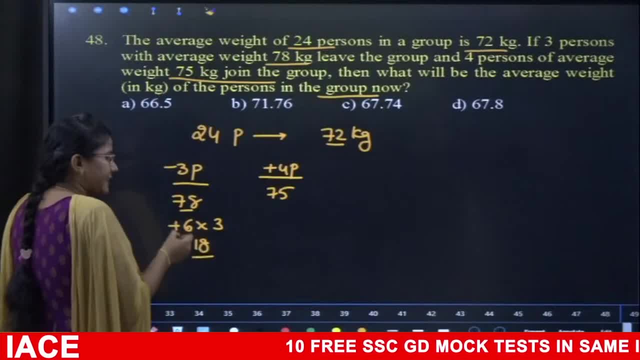 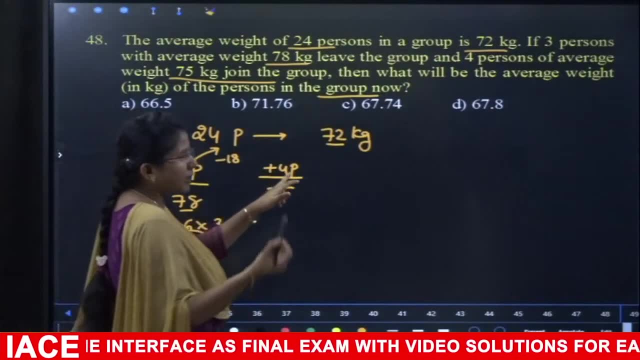 So the total extra value deviation is plus 18.. This extra 18 will be exited from the group. It means minus 18.. So we will take the extra 18.. Next look at the 4 persons joining. The average weight given to all of them is 72 kgs. 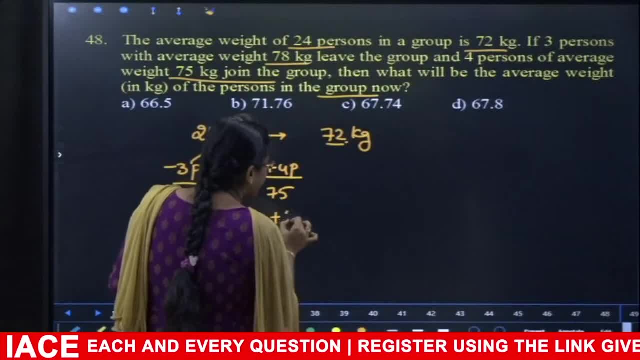 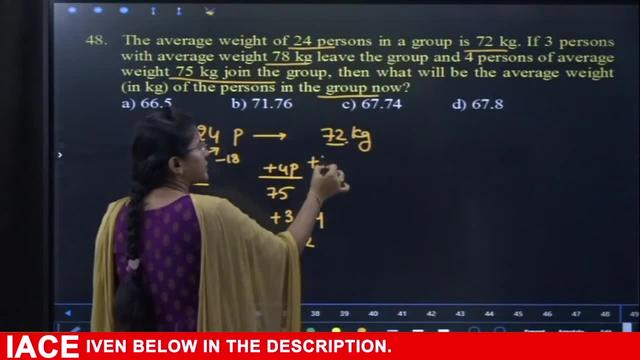 They have extra. How much extra is there? Each person has 3 extra. How many people have extra? 4 members have extra. How much is the total of 3 x 4? 12.. Since they are joining, it will be plus 12 here. 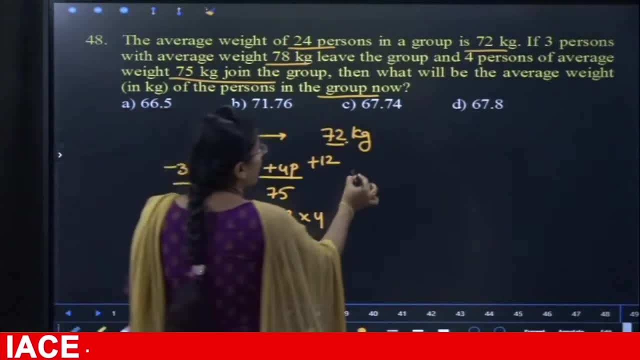 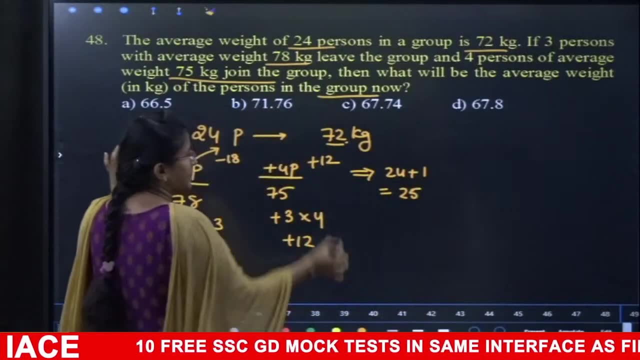 It will not be minus. So if 3 people are going and 4 people are coming, one will join overall. So one will come to the 24 already. How many people will be the total? 25 members. Look at the deviation. 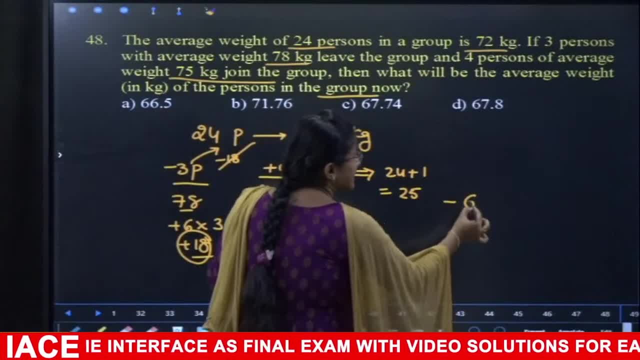 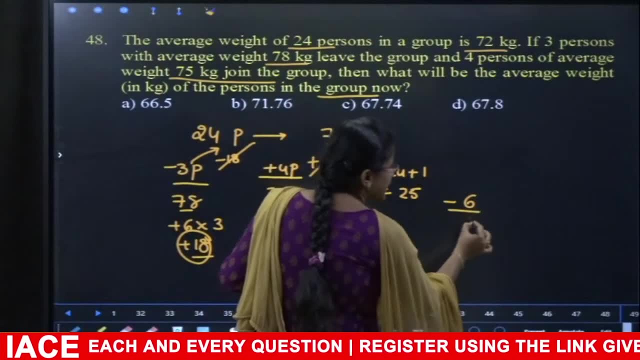 Plus 12 minus 18.. The overall deviation is minus 6.. 6 is reduced from the already available average. How many of us have to deduct 6? equally In total? we need to take out that 6 from how many members? 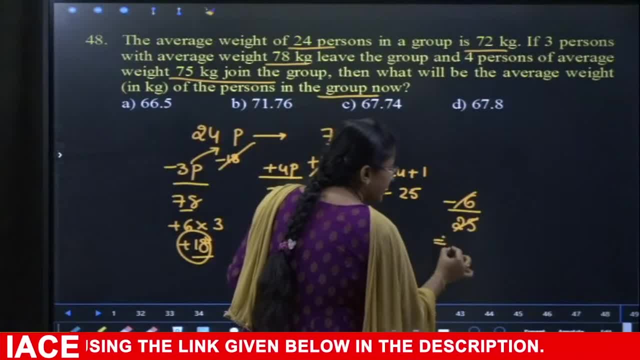 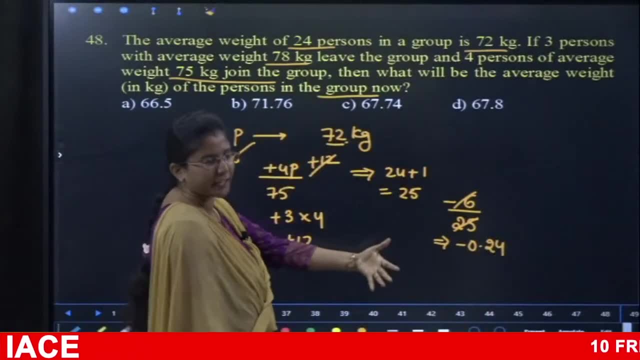 25 members. How do we divide equally From each one 0.24.. We have to subtract 0.24 from the already available average of 72.. So what will be 72 minus 0.24? 71.76.. 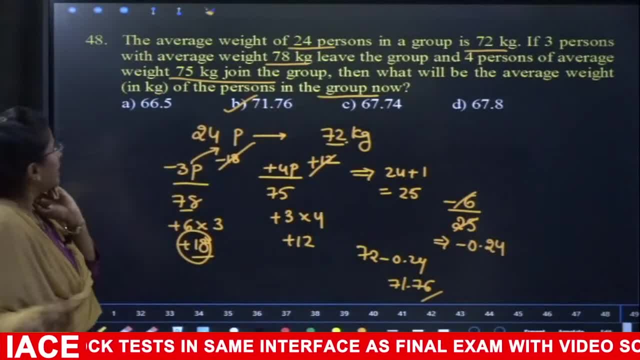 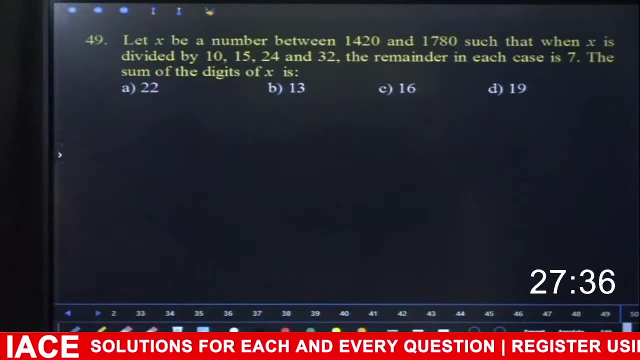 The answer is option B. Okay, Next We will go for next one: 49. 30 seconds timer. please Try it. 49. 30 seconds. Verify the amountФ. Okay, so your time is up. This is the LCM HCF table. 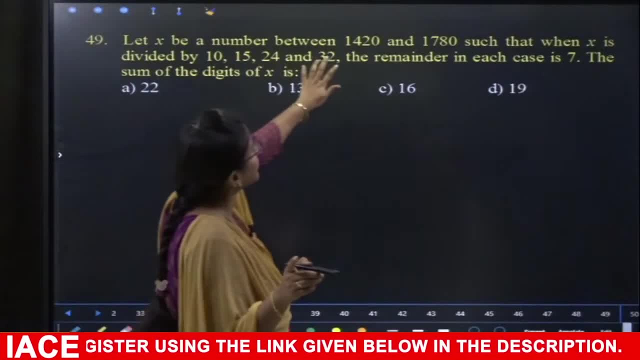 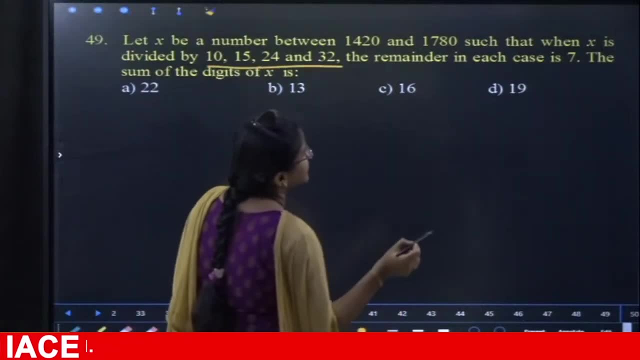 Let's see the LCM. It is enough. if you do the LCM, A number between 1420 and 1780, such that when x is divided by 10,, 15,, 24 and 32, the remainder in each case should be 7.. 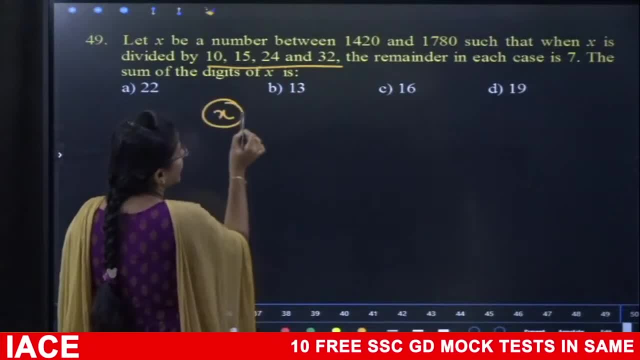 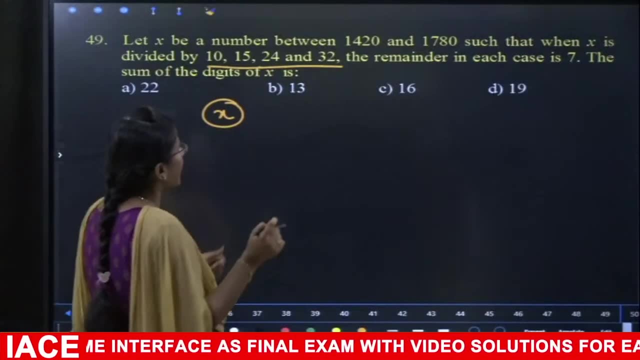 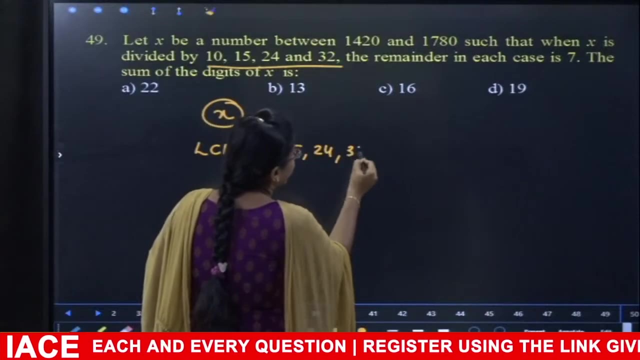 So there is a number x. If we divide that number by 10,, 15,, 24 and 32, there should be a remainder of 7.. That should be in that particular interval. So if we take the case that the remainder should not be there, if we divide by 10,, 15,, 24 and 32- with any number- 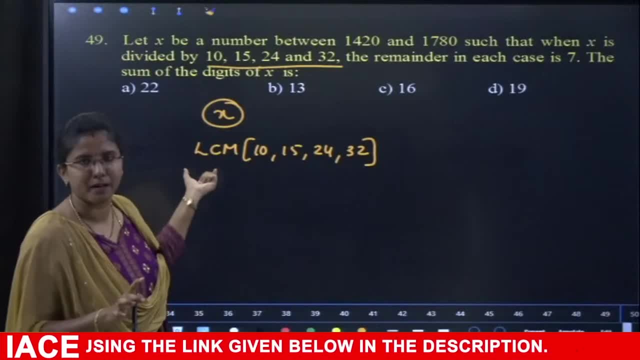 if the remainder should be 0, that is nothing but LCM. We will find out LCM After that. we will increment it in the interval. he asked 2 times, 3 times or 4 times? how many times it is how many times? 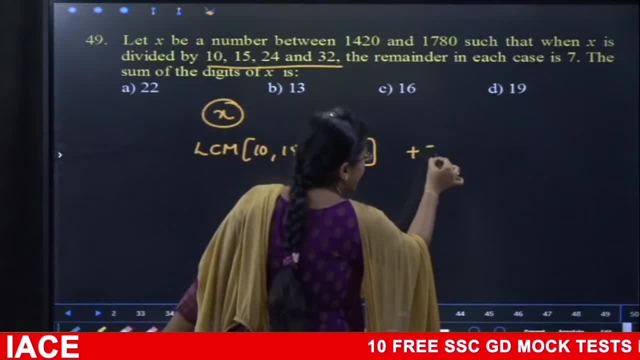 Since he is asking for the remainder, what should we do with the remainder? We will add 7 at the end and it will be enough. So for this particular number, I will take LCM as 32.. 32,, 24,, 2,, 8.. 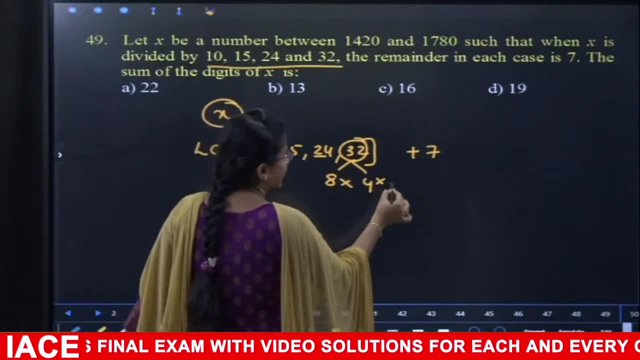 Since it is a multiple, I will write it like 8- 4s. How many times will 24 be? It will be 3 times for 8.. Since 15 should be 5 for 3, 3 x 5.. 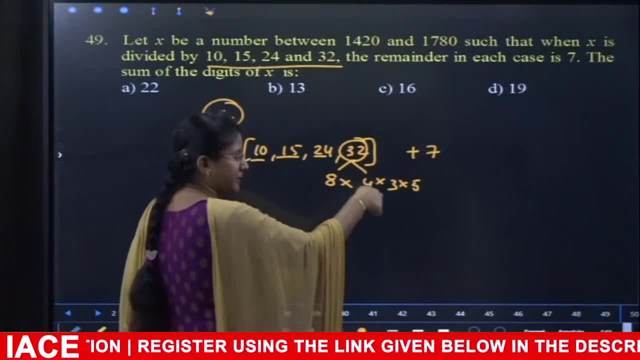 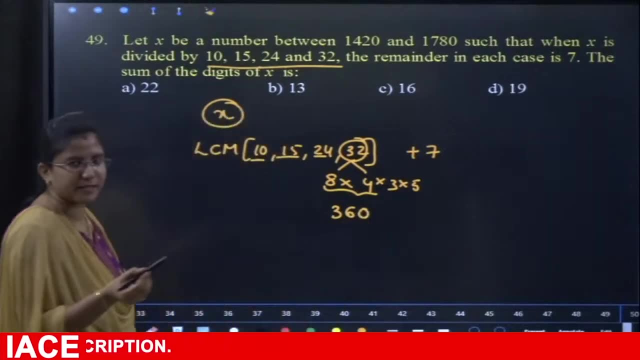 10 is already in this multiplication. 4 x 5 is 20.. 10 is already there, So here it is. 24 x 3 is 70 to 5.. Sir, that is 360.. LCM of the given number is 360.. 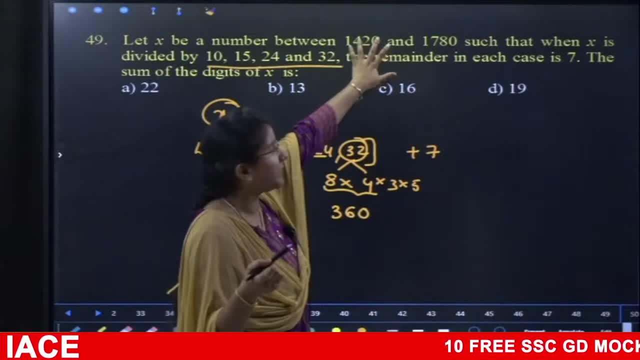 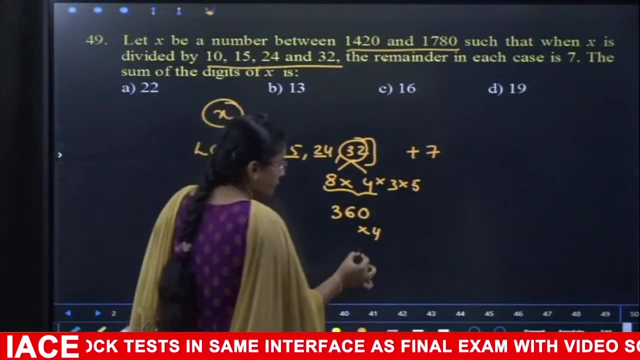 Since it should be in this interval, we will decide it as double or triple. So if we want to come to this interval, if we do it 4 times, it will be enough. 5 times will be more. If we do it 4 times, it will be more. 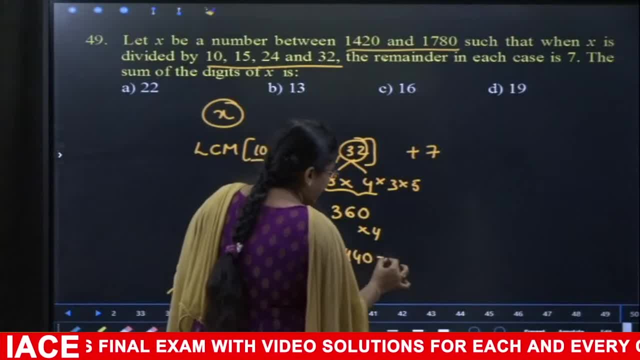 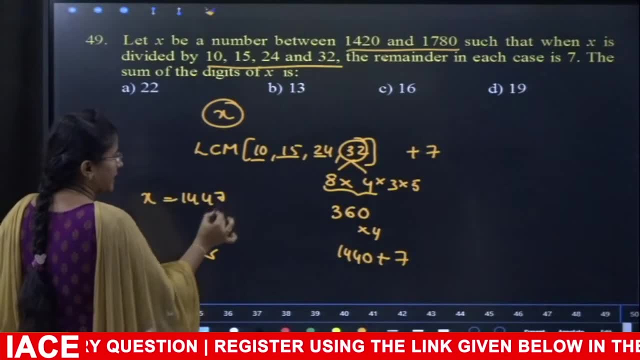 That is, 2, 4 x 3 is 12.. 14, 40. Last we told you to add 7.. We will add 7.. So that particular number x is 14, 47. We have to study the sum of the digits. 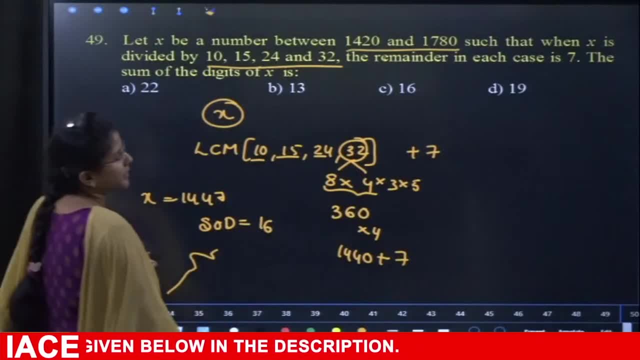 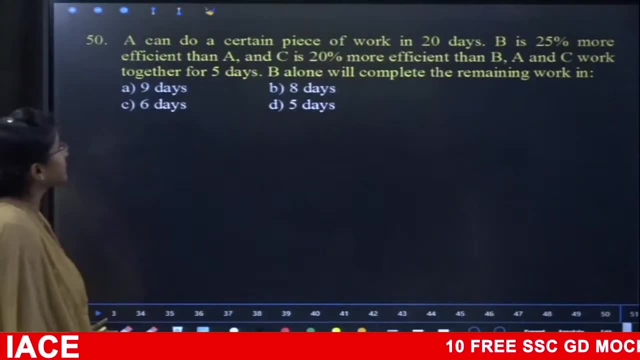 How much will it be if we add the sum of the digits 16.. So option is 50.. Next go for next one: 50.. 50.. One minute timer, please. 10. 1., 1.. 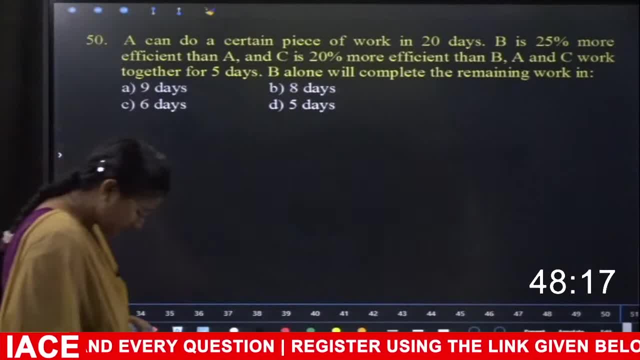 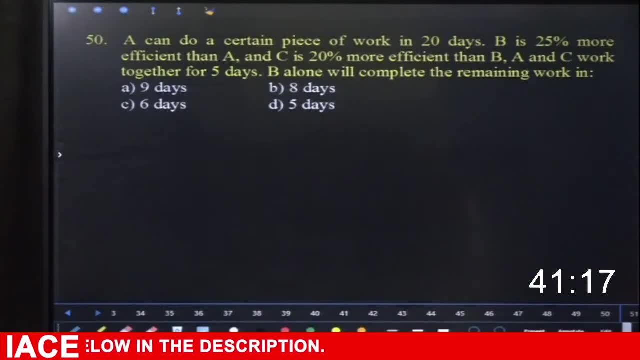 2., 3., 2., 4., 3. 0. 1. 2, 0.. 3. 1., 1., 1., 3., 1. 1. 1.. 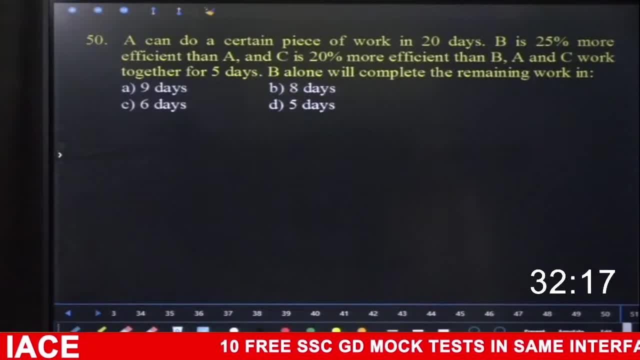 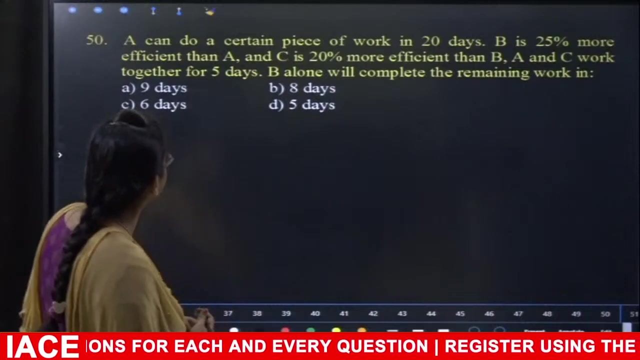 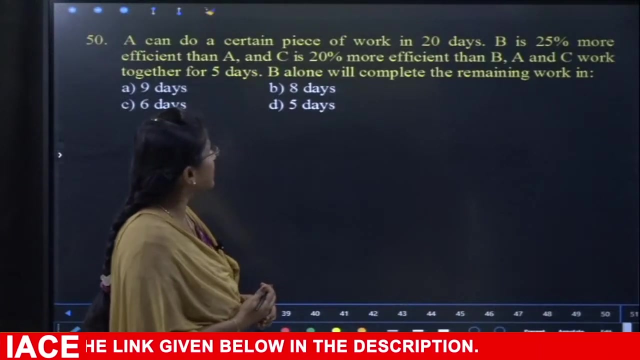 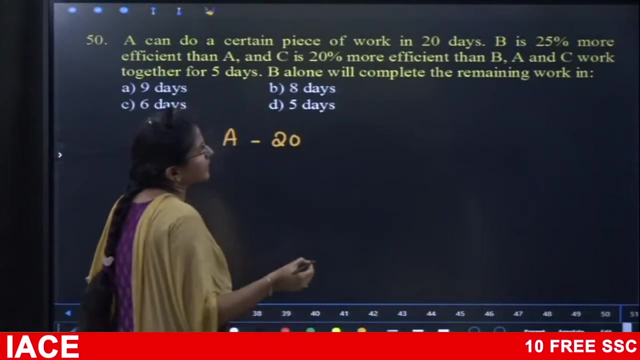 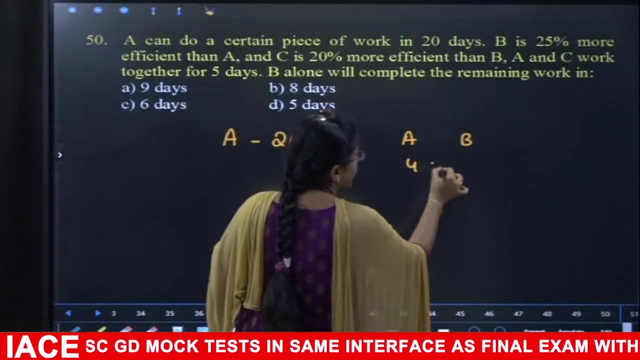 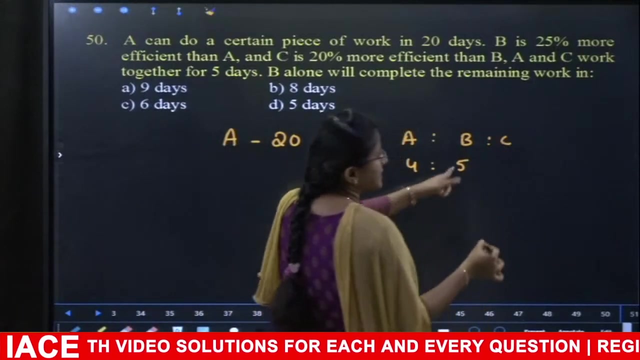 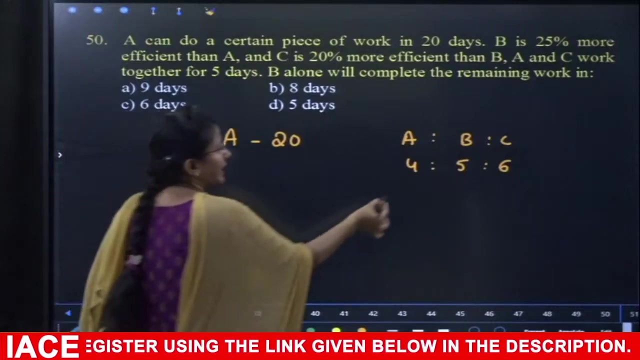 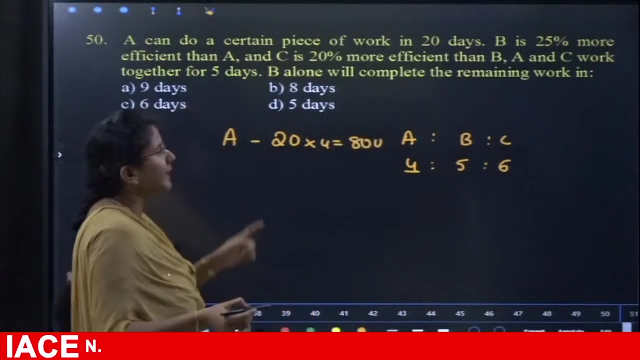 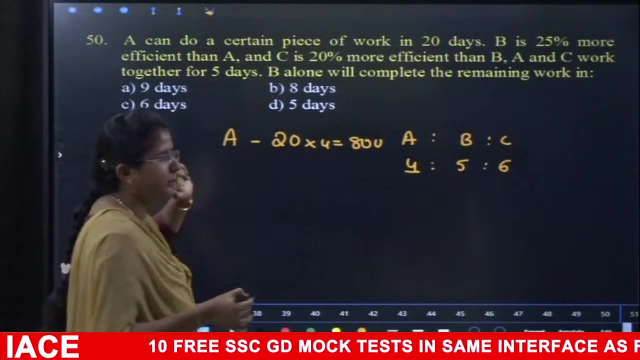 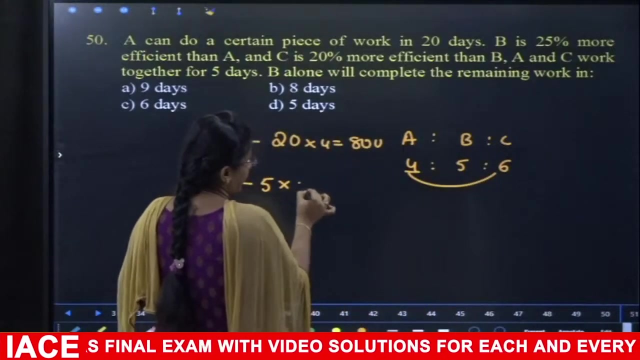 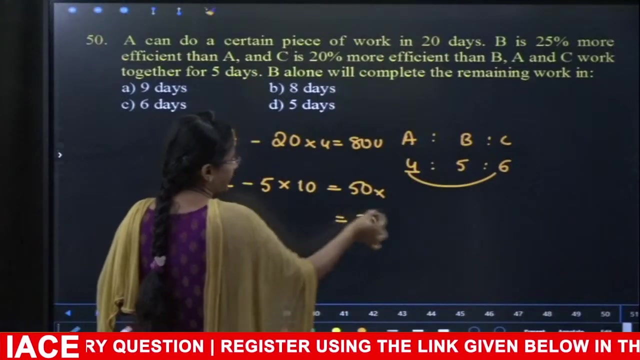 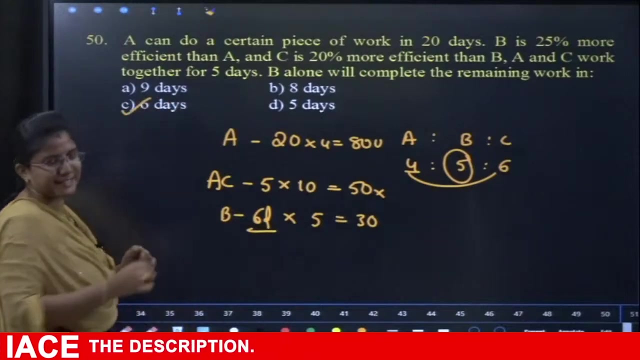 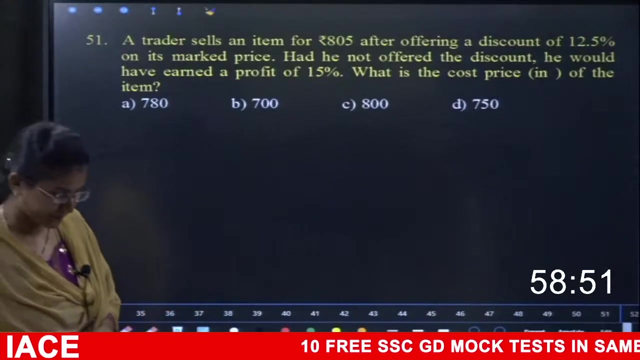 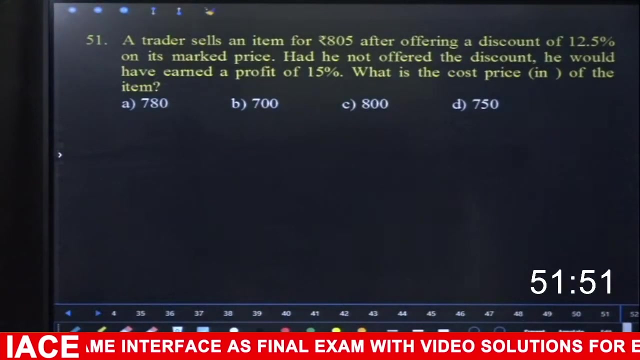 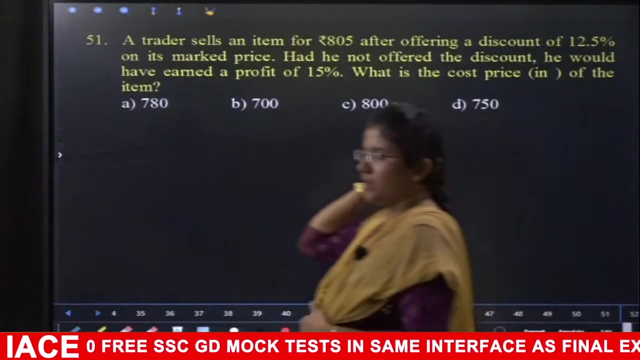 1., 1., 2., 2., 3., 3. 1.. Thank you, Okay, your time is up. Okay, your time is up. Okay, your time is up. Thank you, Okay, your time is up. 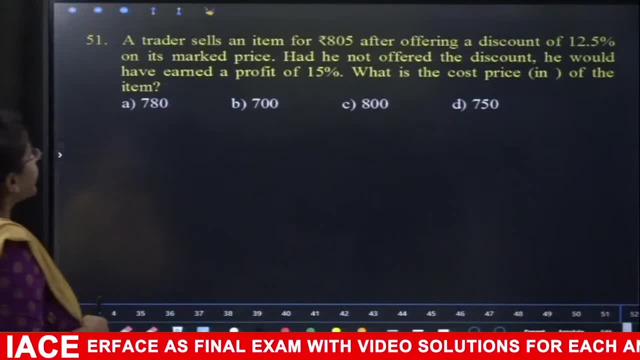 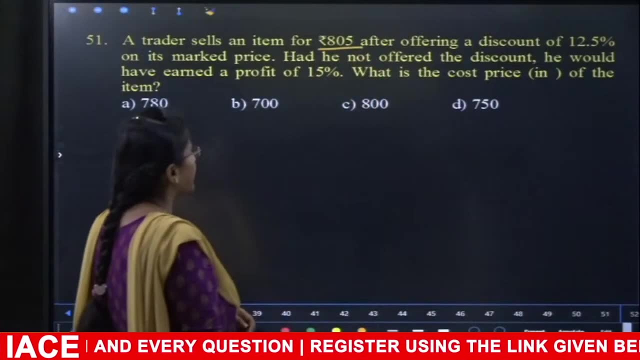 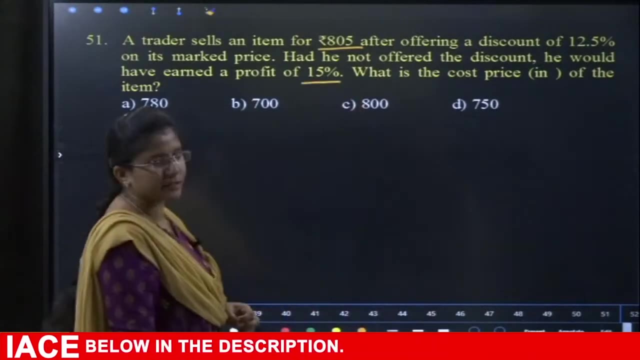 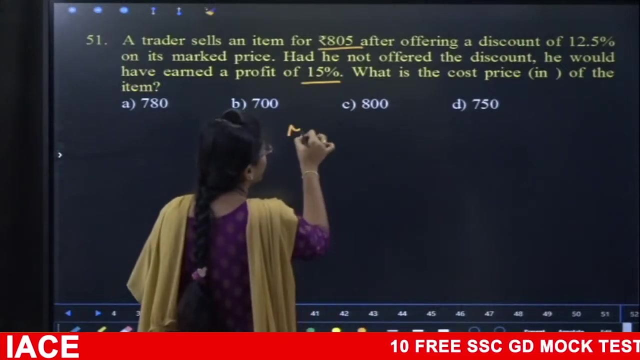 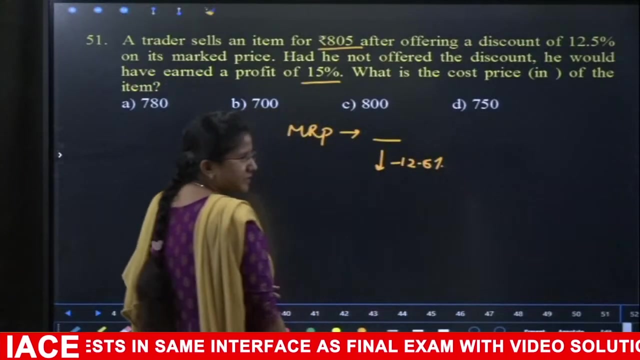 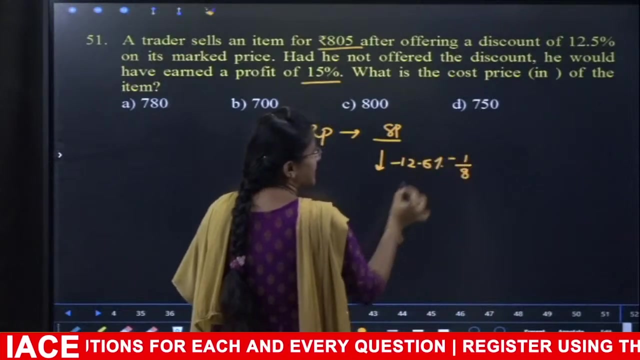 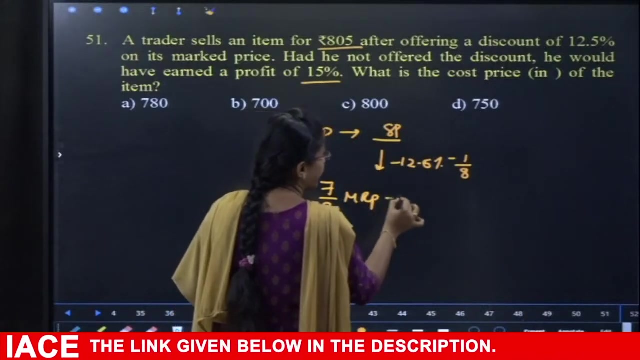 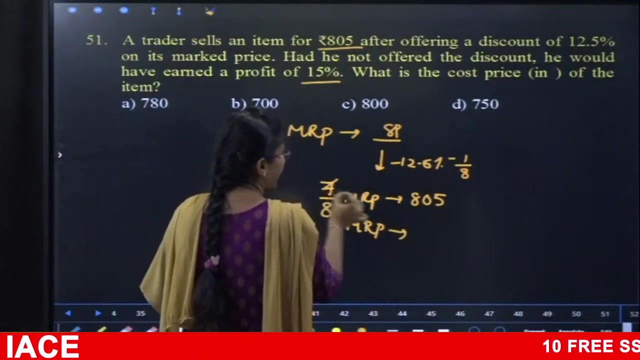 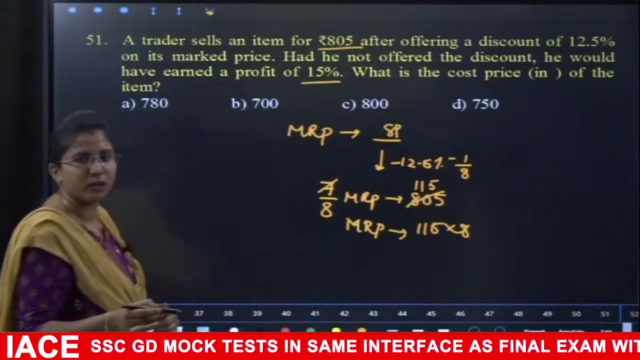 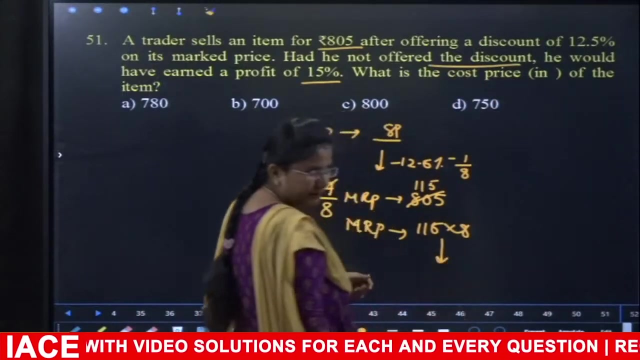 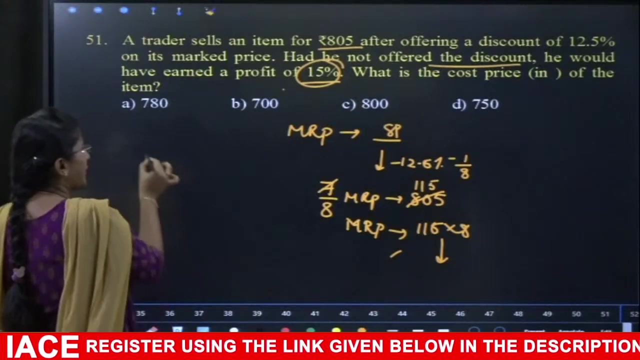 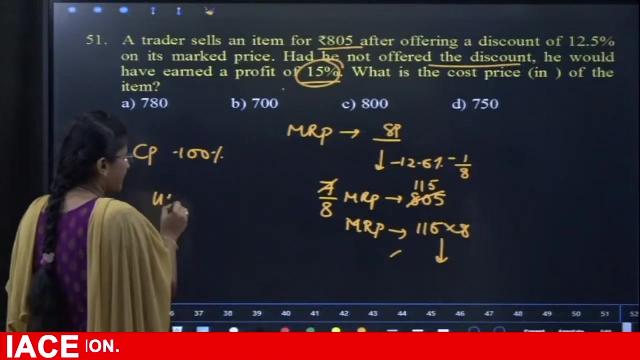 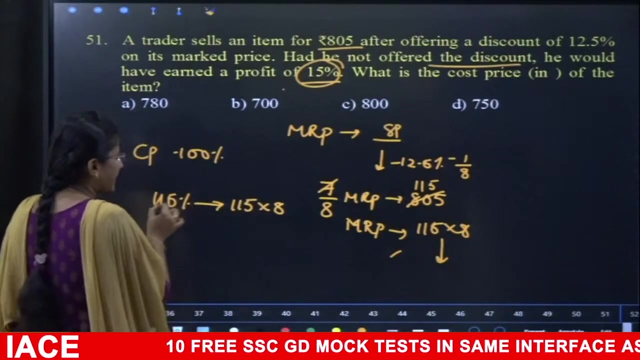 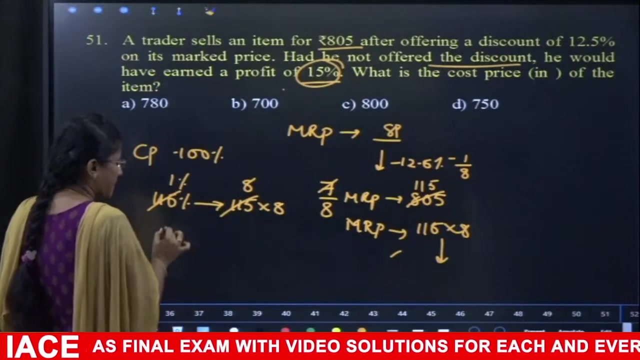 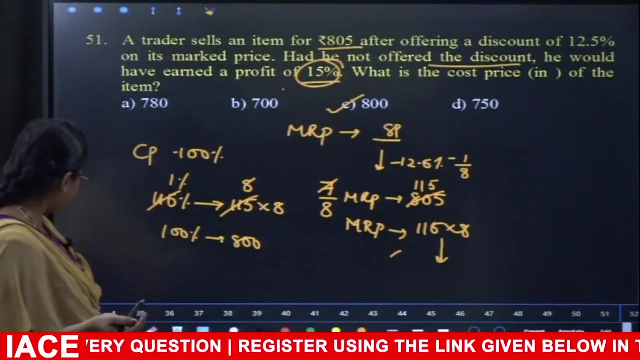 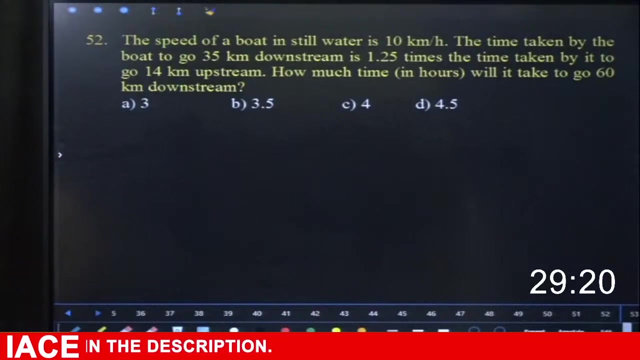 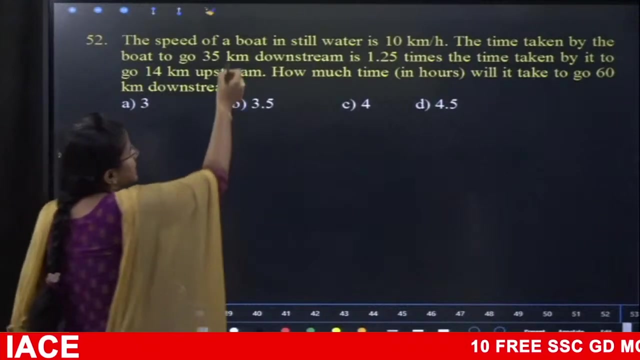 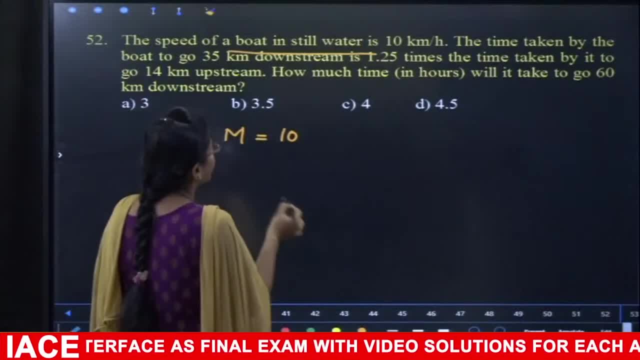 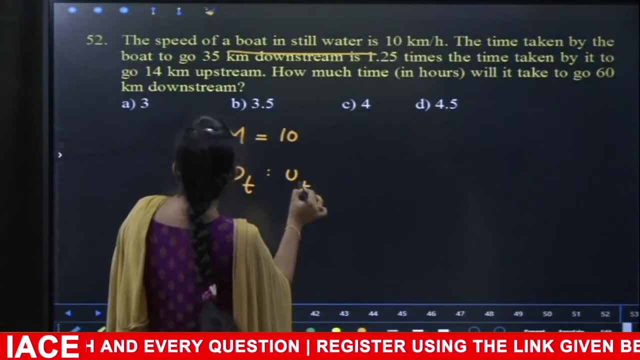 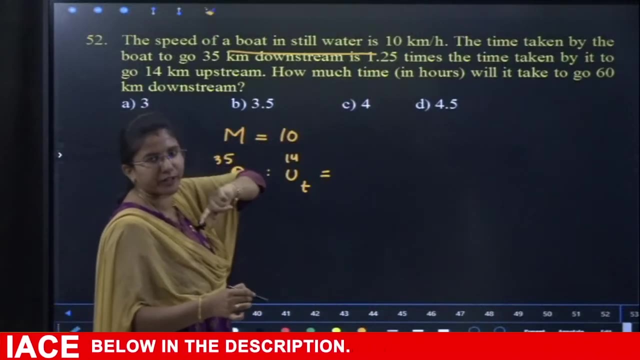 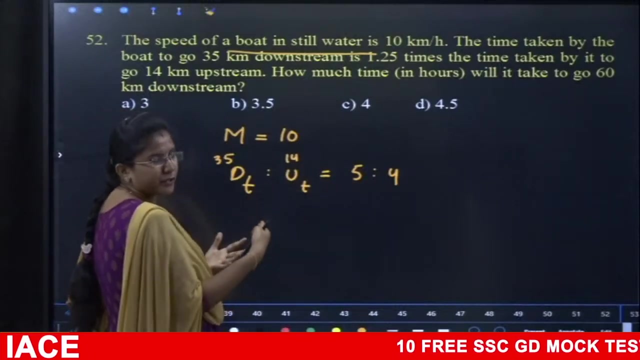 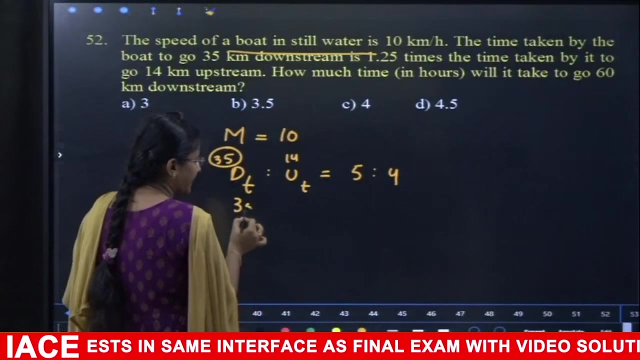 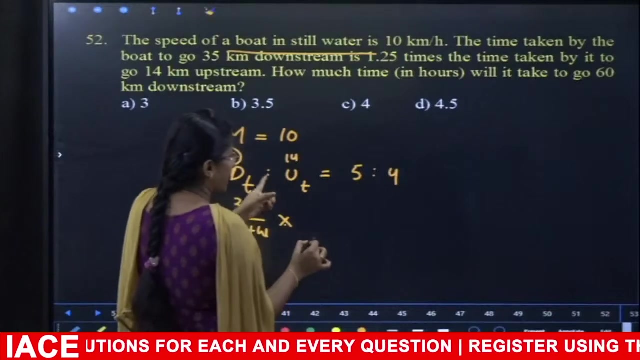 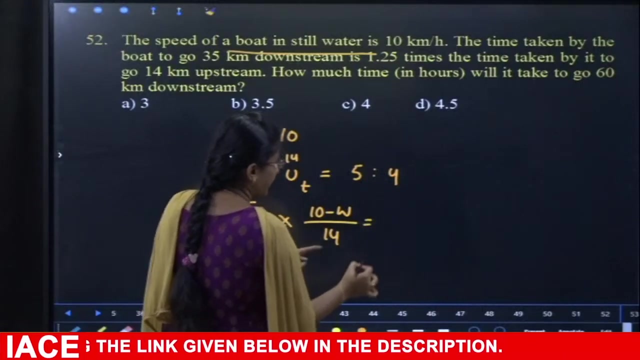 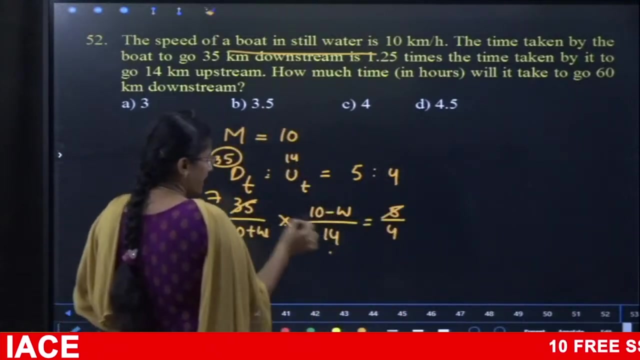 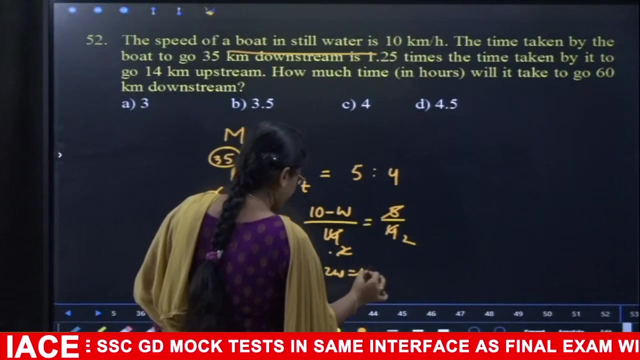 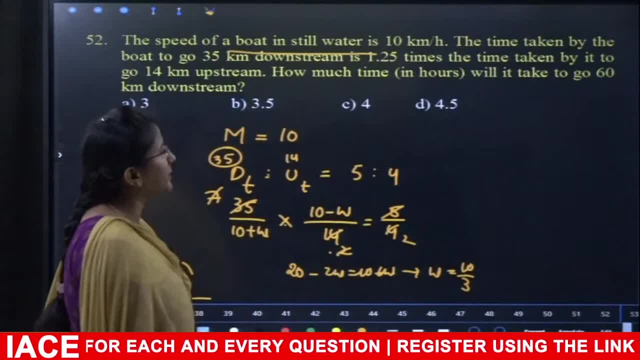 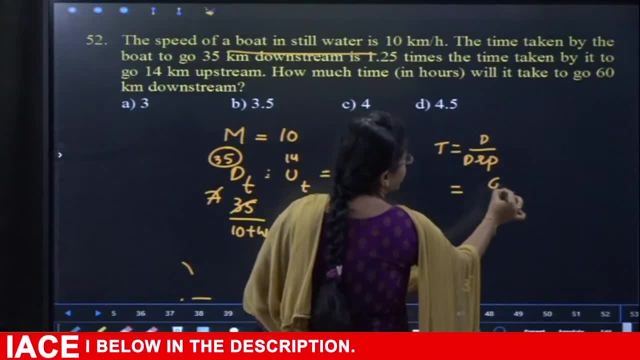 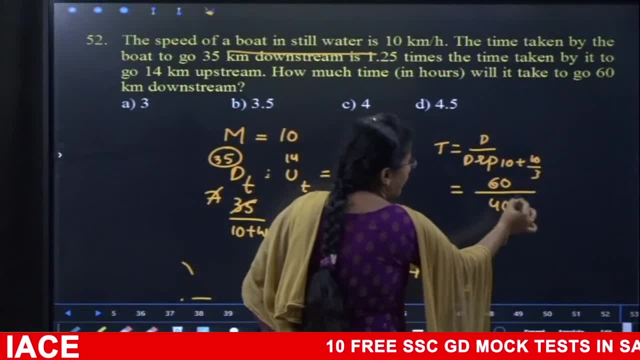 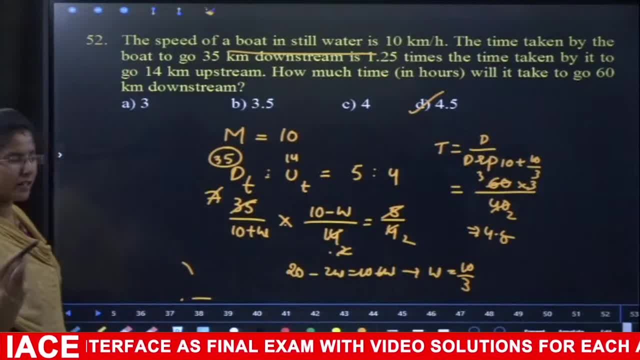 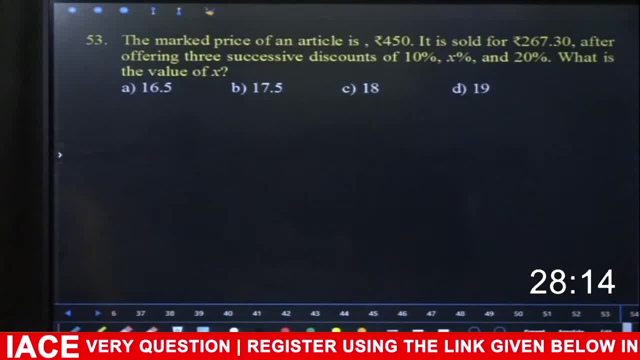 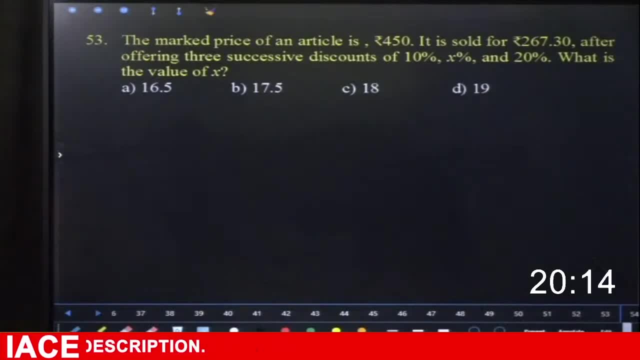 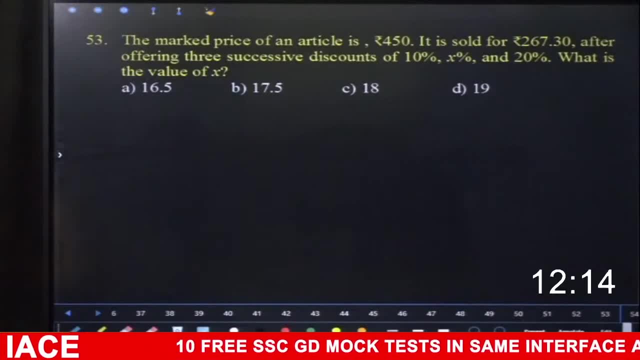 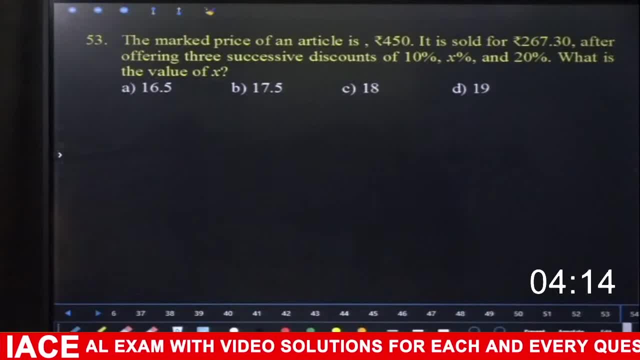 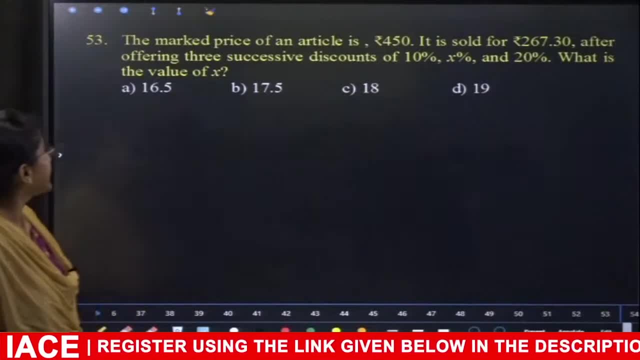 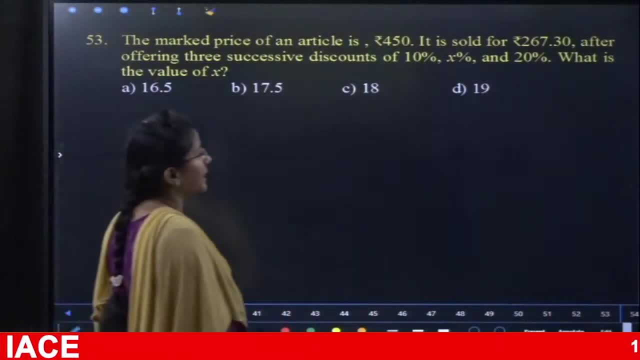 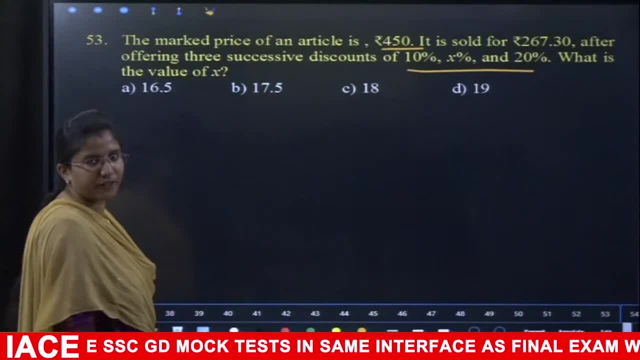 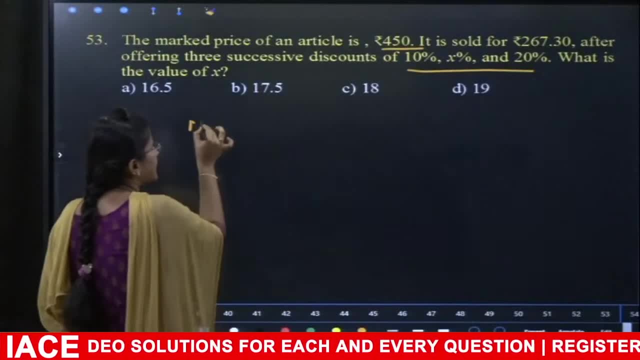 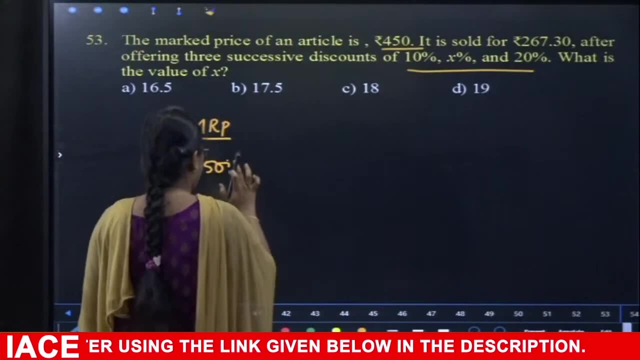 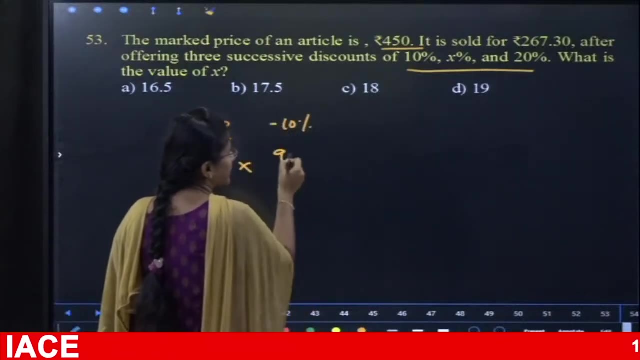 Okay, your time is up. Okay, your time is up. Let's write it normally like this: MRP 450. given this will be for 100% On this 100%, so we'll calculate First. we gave 10% discount, so minus 10 means how much percent should we reduce 90 by 100. 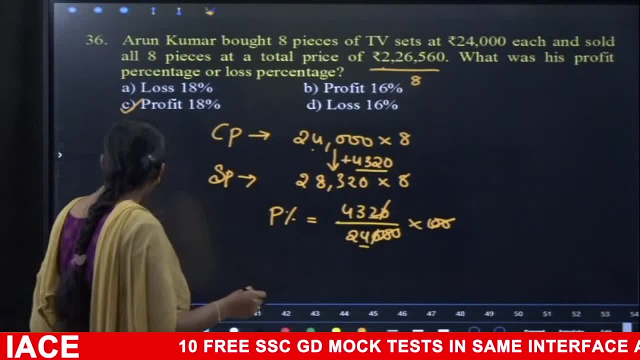 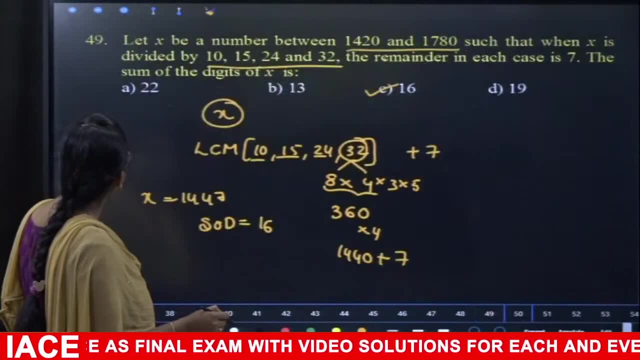 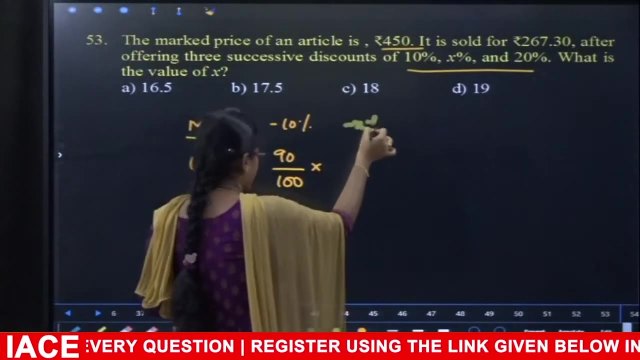 If we give X percent on this, the value we got up to here will be 100%. So the value we got up to here will be 100%. On this, 100%, we gave X percent discount, So we gave X percent discount. so 100 minus X by 100. 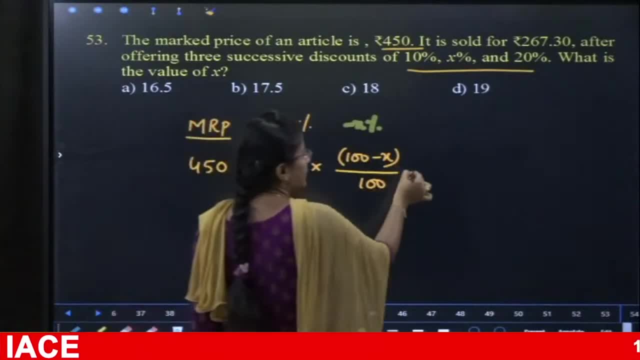 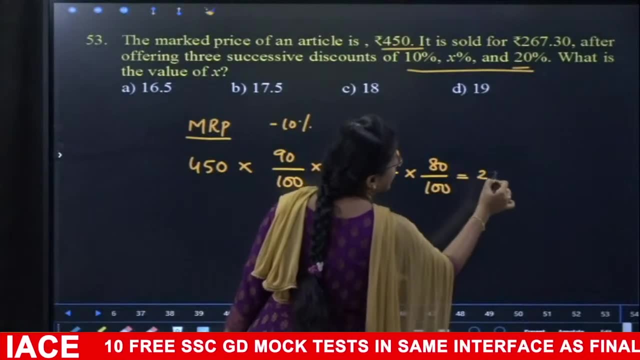 We'll write percentage as divided by 100.. Here the value we got up to here is 100%. This time the final discount we gave 20%. that will be 80 by 100.. Equal to what is the selling price given. 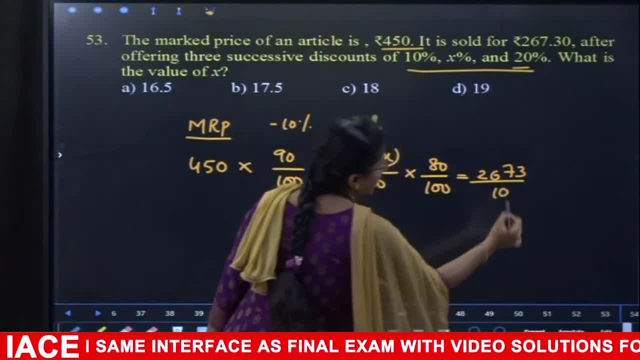 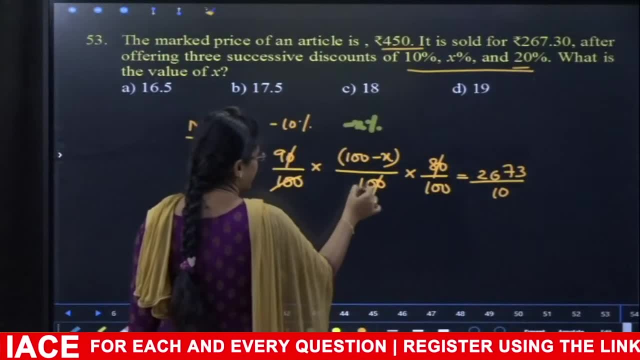 I'll write it by 10 instead of 2,, 6,, 7, 3 points. Cancelation is normal. If there are zeros on us, we'll write zeros, We'll cancel out zeros, Next 45 and this will be for 2 times. 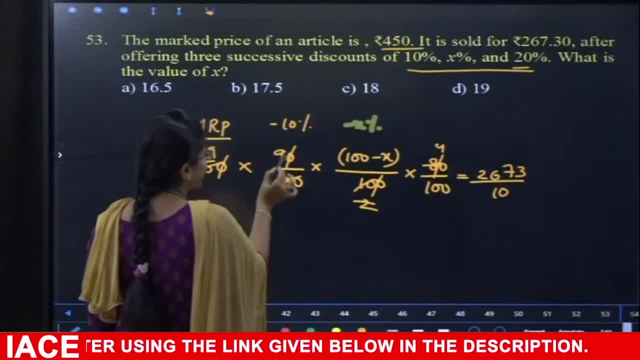 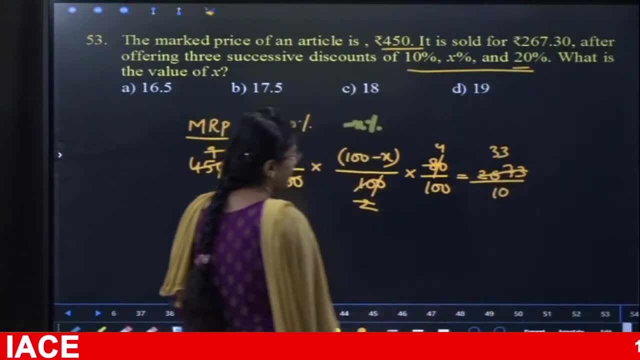 This will be 9.. 2 and 8 will be 4 times. So 9 x 9 is 81.. 81 is multiple Directly. it will be cancelled In 81,. this 2, 6, 7, 3 will be cancelled for 33 times. 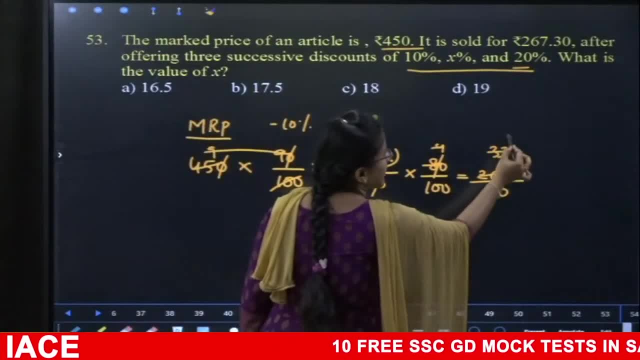 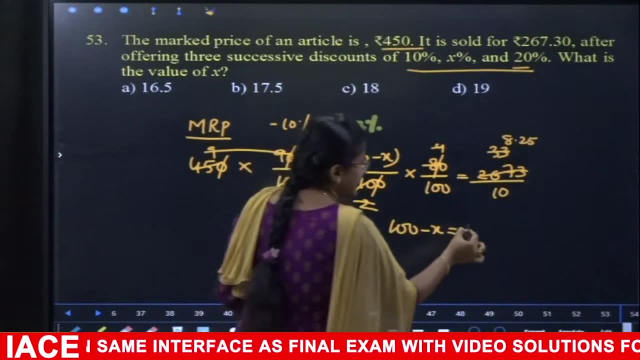 If we look at it overall, the balance will be 4 only 4, this will be cancelled out for 8.25.. So overall, 100 minus X will be zeros. If we multiply all these, we'll get 82.5.. 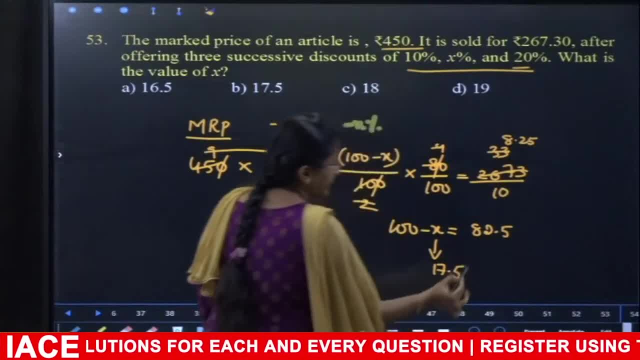 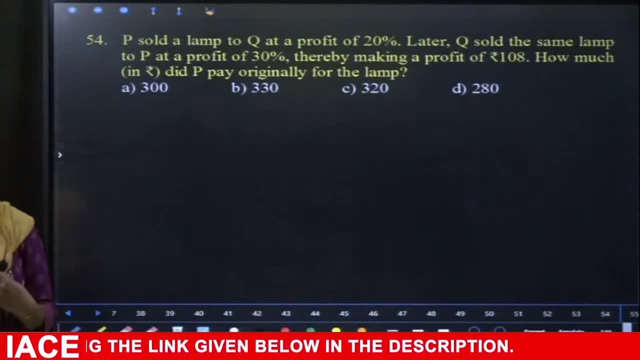 And everyone. what will be discount X value? It will be 17.5.. That's options B: 17.5.. Try the next 54 for 30 seconds. ok, Nextкий 54, leaving 158.42 가격. 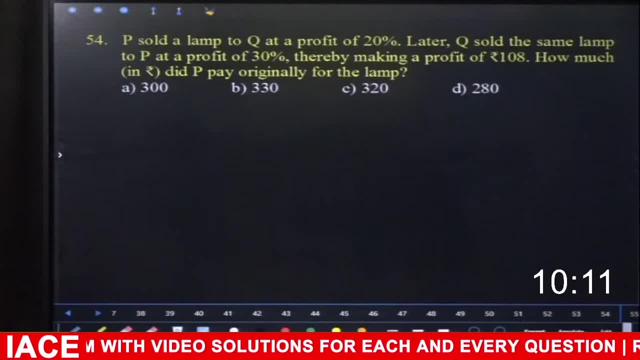 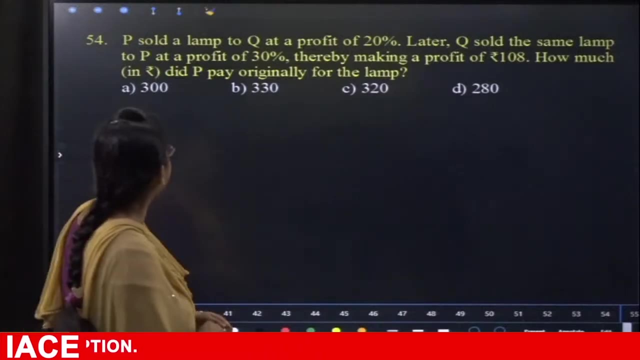 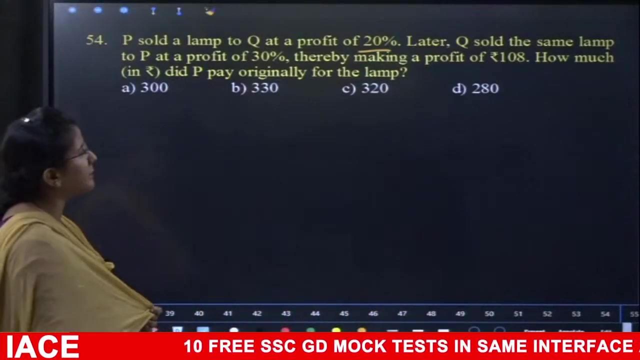 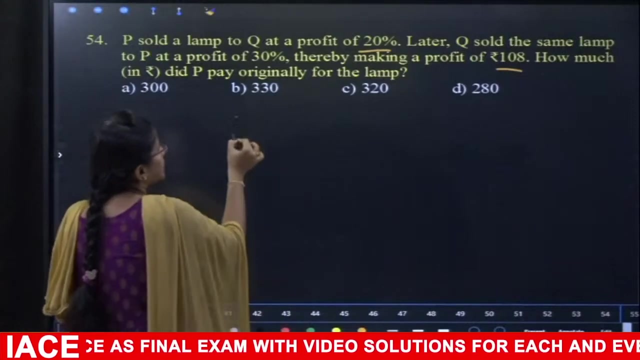 okay, next, next equation 54: p sold a lamp to q at a profit of 20 percent. latter q sold the same lamp to p at a profit of 30 percent, thereby making a profit of rupees 108. how much did p pay originally for the lamp? p reduced the profit to q, ie 20 percent, profit q again. 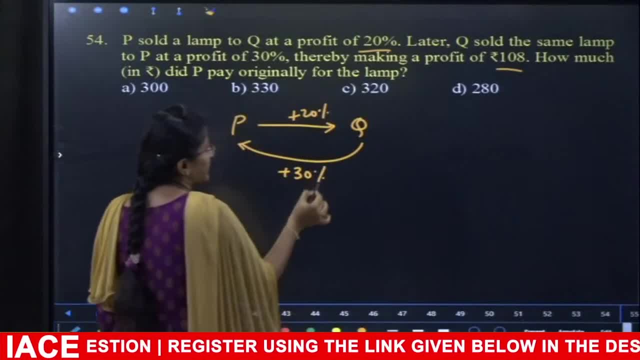 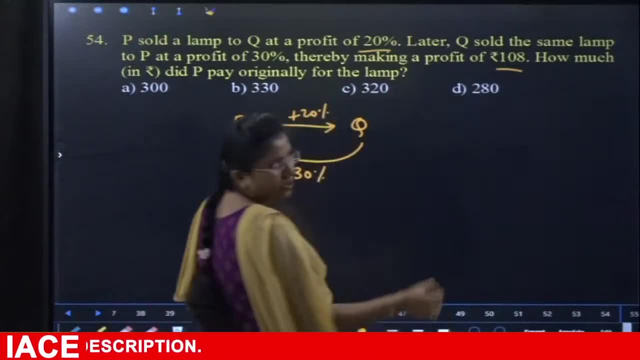 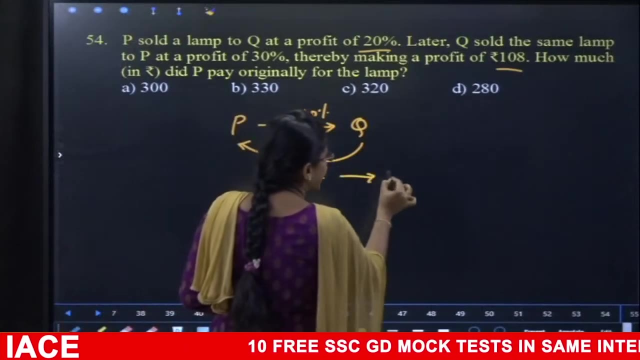 returns to p, sell 30 percent to p. first of all, to the 30 percent value he gave in this equation. how much profit did he give? 108 rupees Q people have a profit of 30 percent of the same amount he gave. that 30 percent value is 108 rupees. 30 percent 108 means 100 percent. 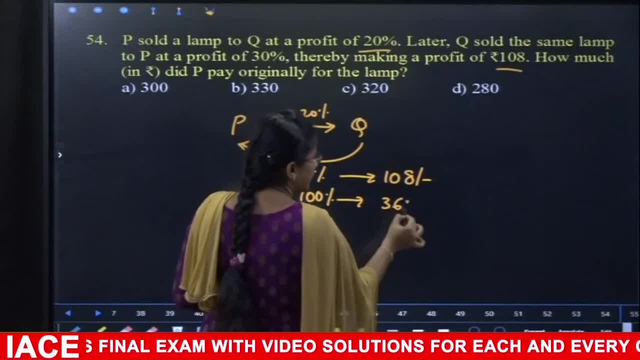 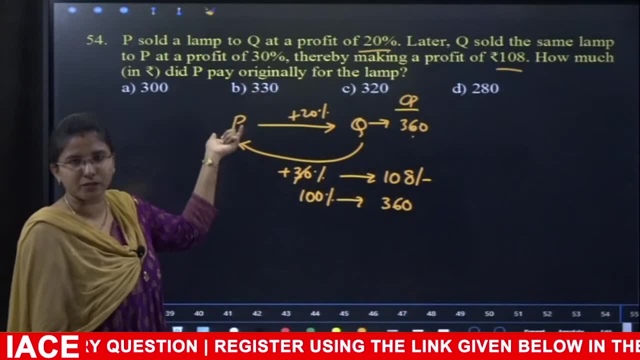 value. 30 percent value is equal to 108 rupees. 40 percent value is equal to 108 rupees. 40: 10s means 36.. 100% value will be what? 360.. So Q cost price is 360.. This is the selling price of P for 360 rupees. 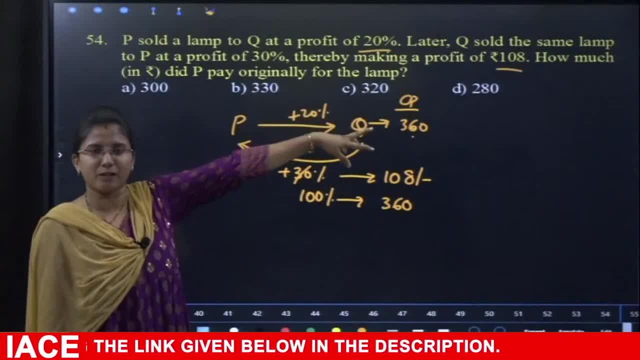 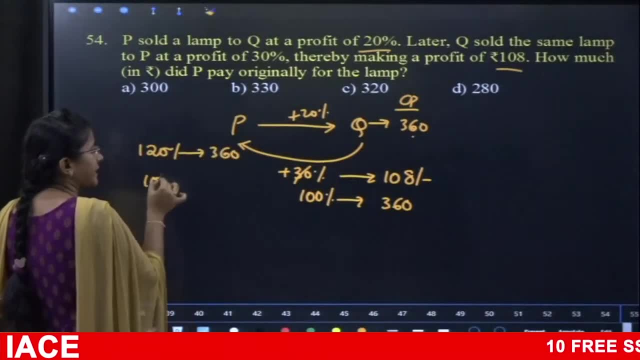 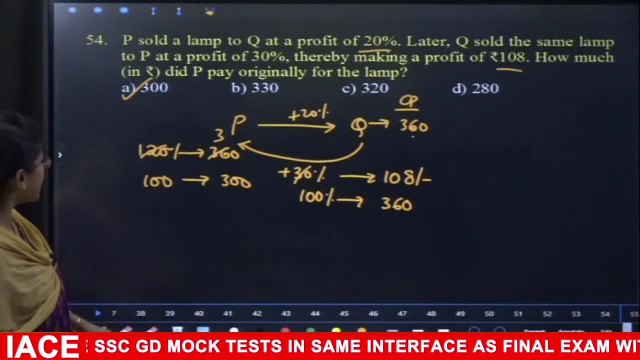 The value added on the 100% value is 360. So here we can write it like: 120% value is 360. Then P's cost price is also 100%, right? So this will be for 3 times Cost. price of P is 300 rupees. Option A: Okay, Very easy equation Next: 55.. 55. try J&D 30 seconds timer, please. 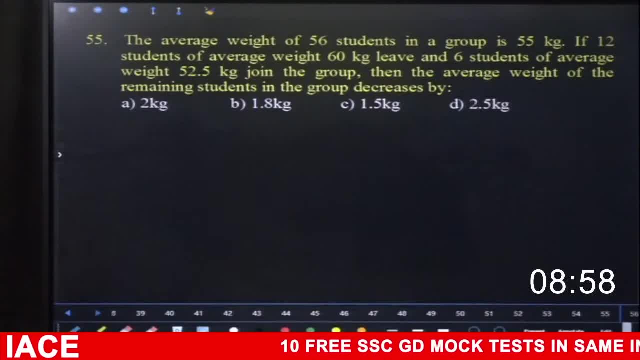 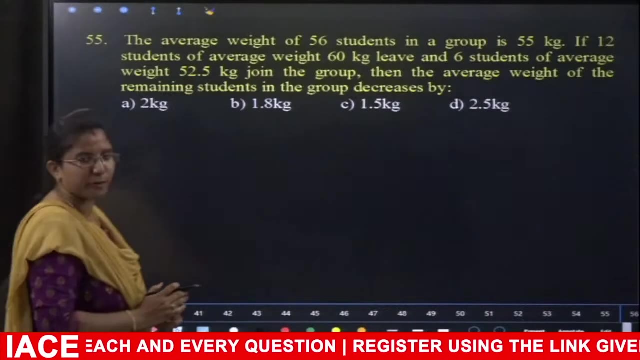 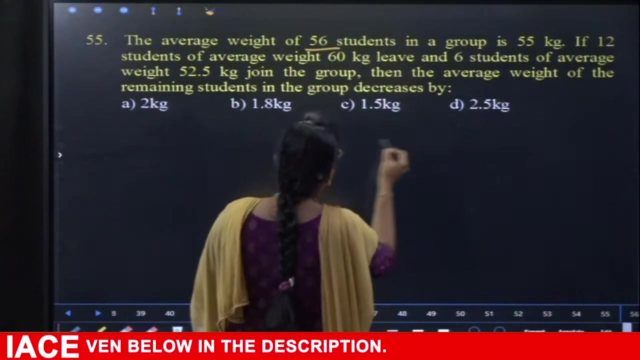 Okay, So your time is up. So average is topic mentioned in the question. So till now we got only couple of questions working. This is the same model. The average weight of 56 students in the group is 55 kgs. 56th students average weight is 55 kgs. 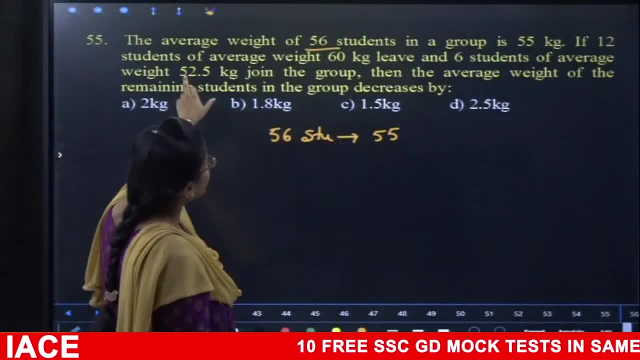 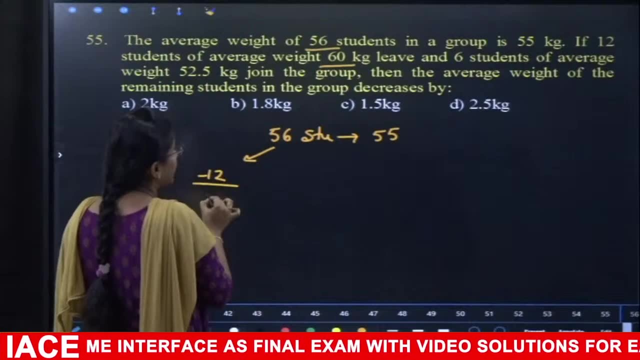 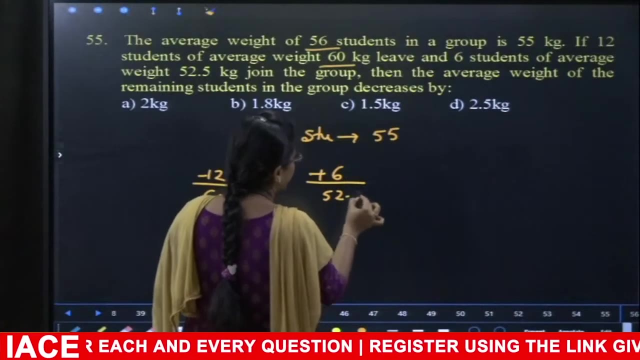 So, from these 56 students, 12 students of average weight- 60 kgs leave. they left with an average weight of 60 kgs and 6 students joined with an average weight of 52.5 kgs. Similarly, we will see the deviations in the process and verify whether it is increasing or decreasing. 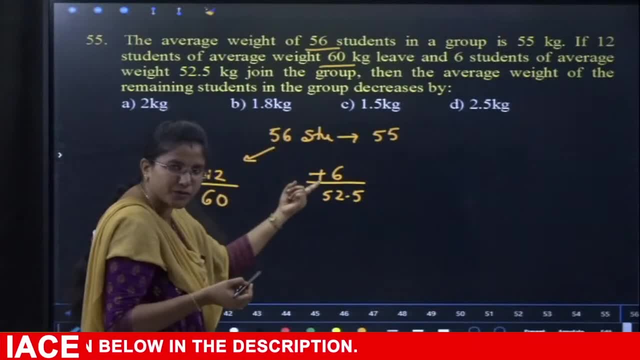 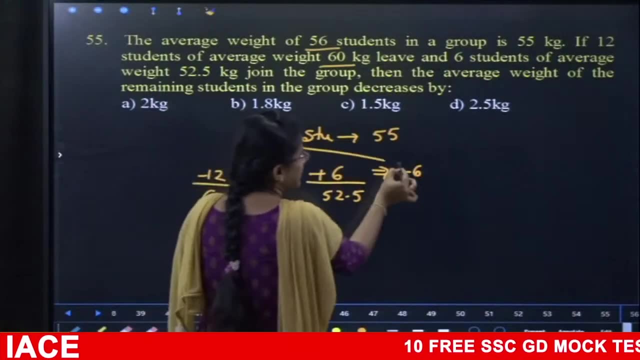 So from these 56 students, 12 students are leaving and 6 students are joining. So overall, if we see the change in the members, it decreases to 6 members. If we decrease 6 members from 56, how many remaining members will be there? 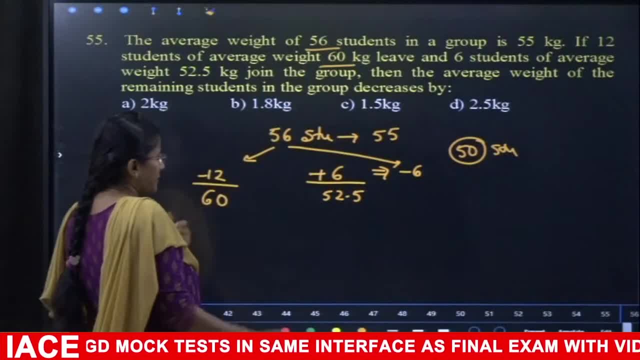 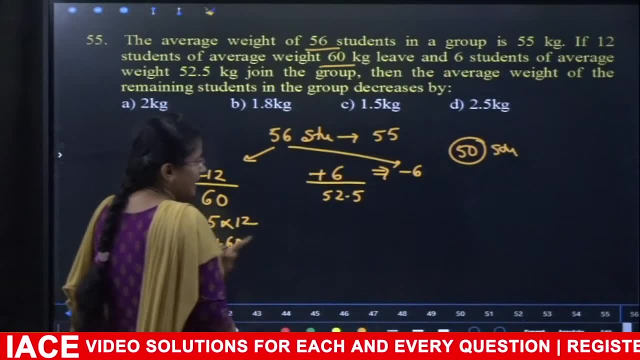 Students will be only 50 members. So if we compare with 55,, 60 is extra. How much extra For each of them? it is 12 members. So the extra weight for the overall is 60.. Next, if we compare with 52.5, it is 2.5 less than for 6 members. 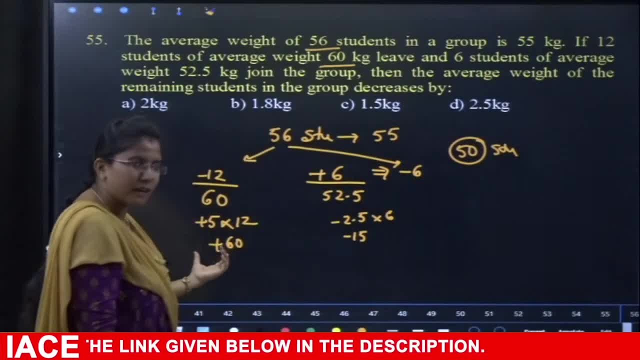 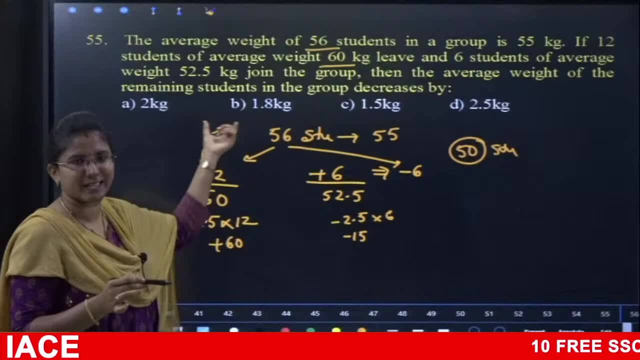 So how much has decreased? overall, It is 15.. For those who are leaving, it is 60 extra. So when these people went out, left out how much has decreased for us From the already existing average. the sum of 60 is reduced. 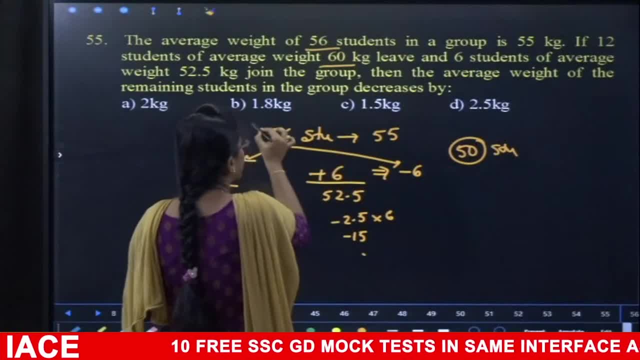 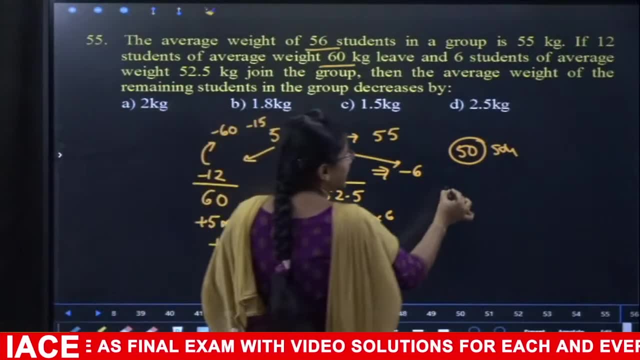 Since they also have a decrease, what is the average due to them? also, The sum of 50 is overall. From these it is minus 60 and from these it is minus 15.. So, overall, how much has reduced from these two? 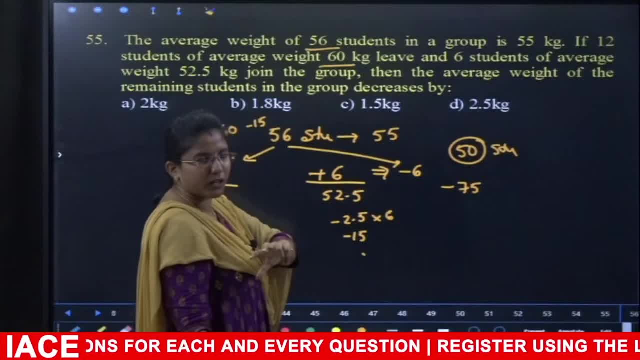 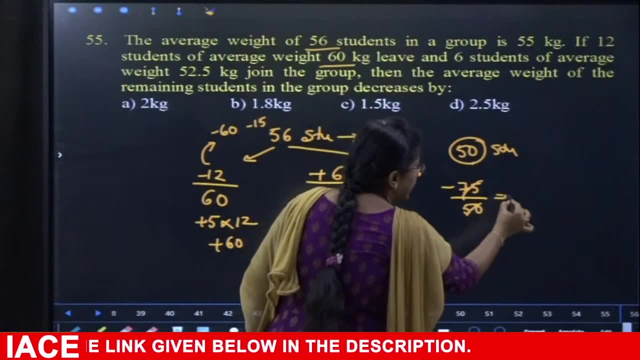 75.. Equally, from how many members should we subtract that 75? From 50 members. So, taking out 75 from 50, 50 members, that is what 3 by 2, right, 3 by 2 is minus 1.5.. 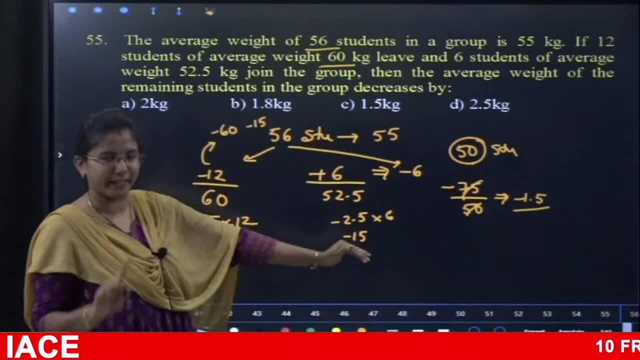 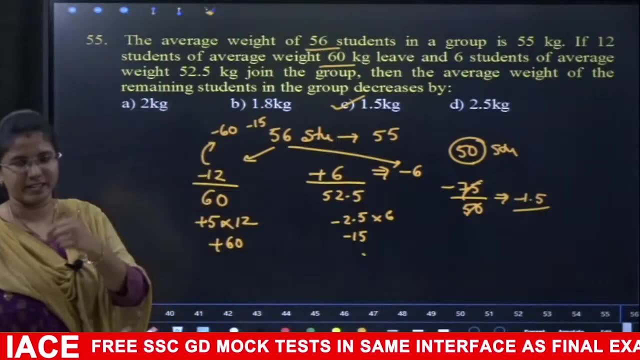 So by making changes like this, the average is reduced. How much did you ask? You didn't ask for change, So it is decreased by how many kgs Minus 1.5.. It is decreased by 1.5 kgs. 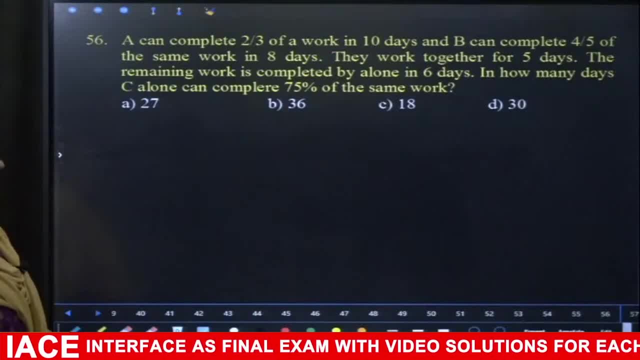 Is it okay? Next 56.. Try it 56.. From the topic of time and work: 30 seconds Timer please. Okay, Okay. So next A can complete 2 3rd of work in 10 days. 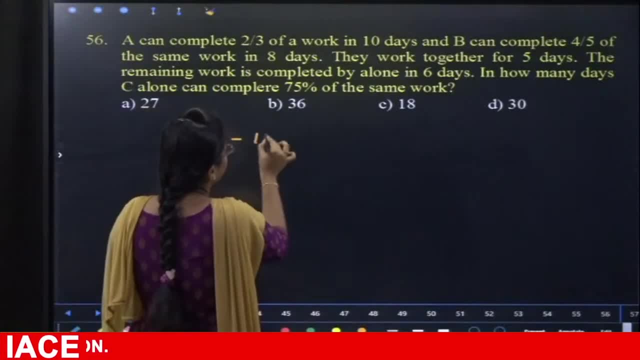 So if 2- 3rd work is completed in 10 days, it takes 15 days for A to complete the total work. 2, 1, 10, 5 times then 3, 15,, 3, 5 is 15.. 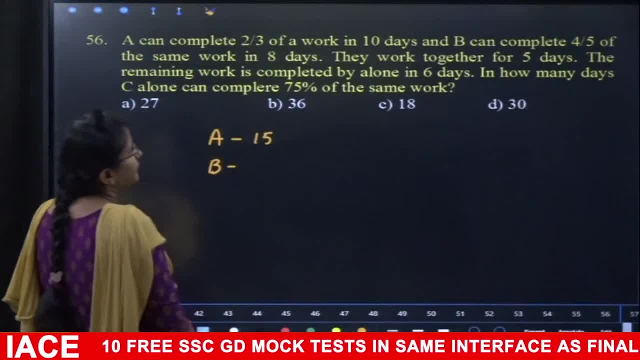 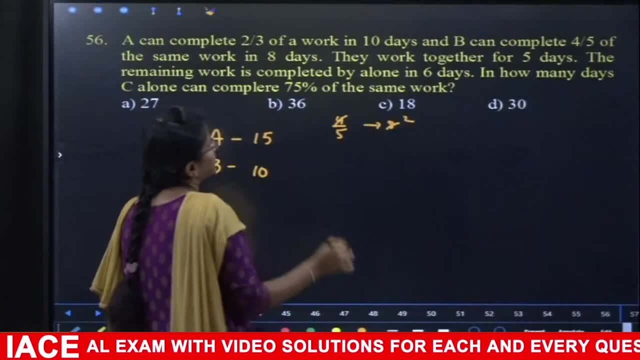 B can complete 4 by 5th of the work in 8 days. 4- 5th work in 8 days means it takes 10 days to complete the total work. They work together for 5 days and the remaining work is completed by alone in C days. 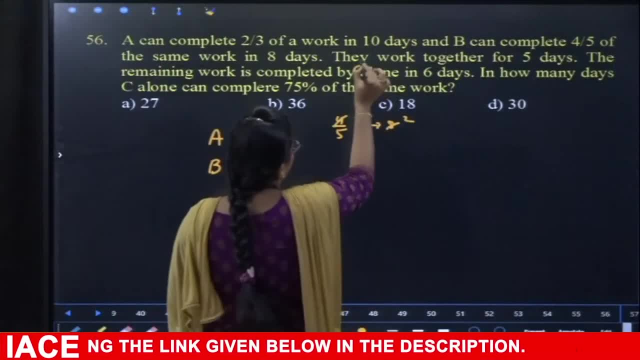 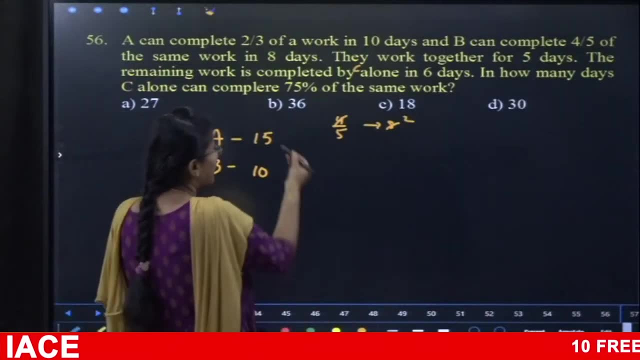 In how many days C can complete 75% of the same work: 15, 10.. I will write 30 units of total work for 15- 10.. 15, 2 times and 10 is 3 times. So, after filling up the efficiencies, since A and B worked for 5 days, A and B worked for. 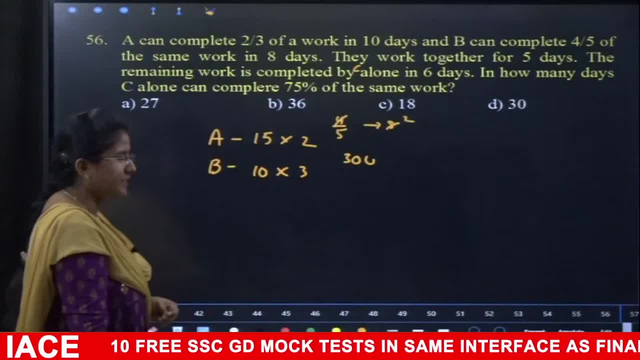 5 days, so 2 plus 3, 5 total 25 units of work will be completed. The remaining work, with balance, is only 5 units of work. The person who completed those 5 units of work is C completed, So C is missing. 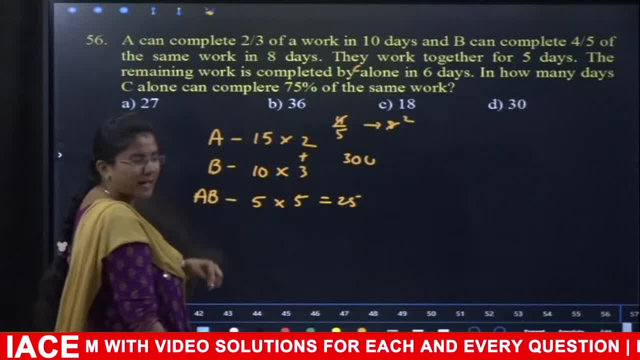 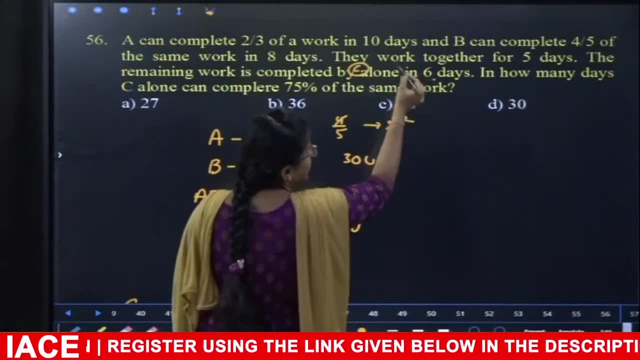 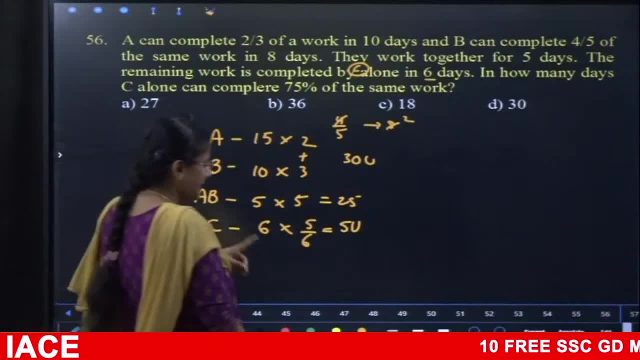 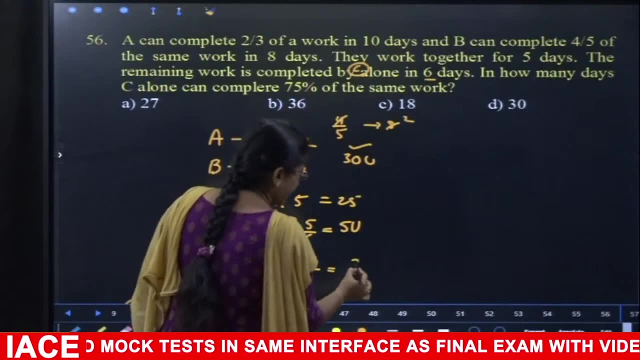 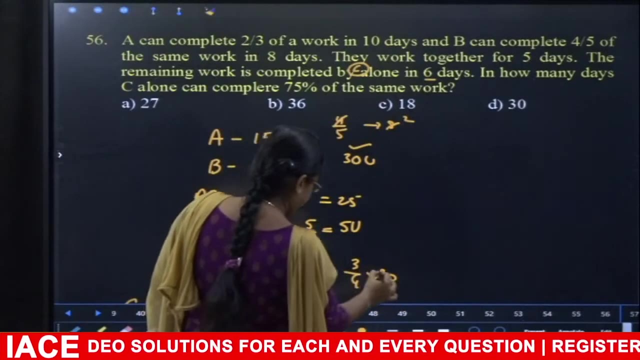 This is the C. what needs to be completed with 5 by 6 efficiency. How many percent is in the previous work? Just 75%. 75% is 3 4th of 30. How many days will it complete C work? 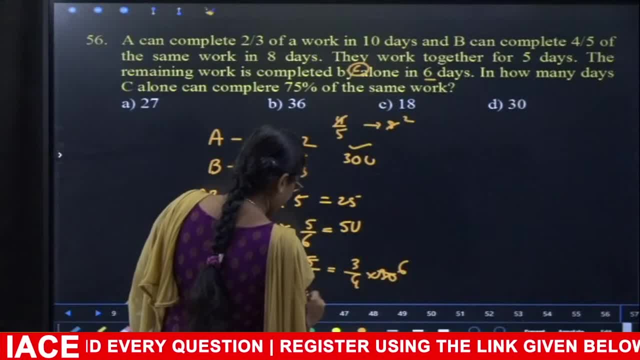 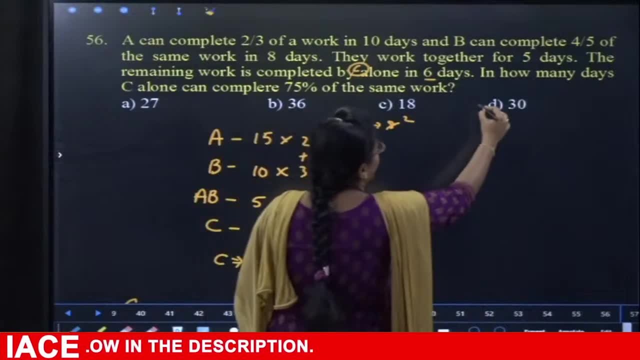 This will be six times. Number of days will be taken will be 18 times each 3.. 6 by 4. That will be answer 30.. 75 percent Already in that. we will do 3 fourths. We have to complete that work. 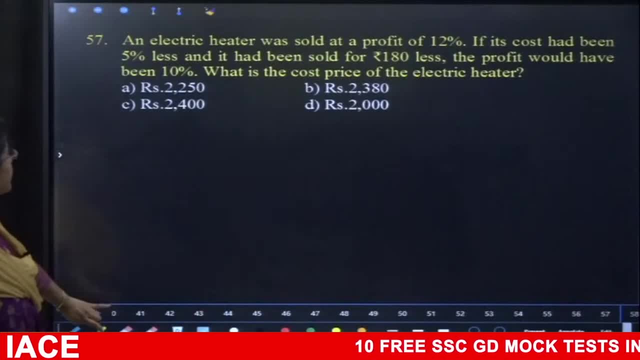 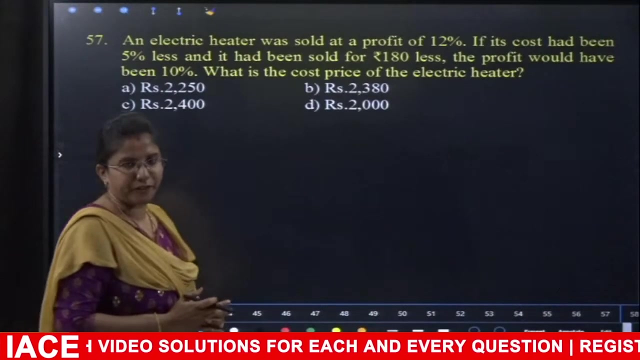 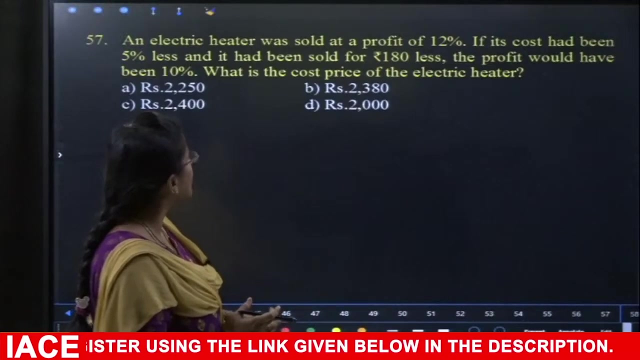 Option D, Next 57. Try 57.. 57.. 30 seconds timer, please. Ok. So here profit and loss question again. 57. An electric heater was sold at a profit and loss question. If its cost had been 5 percent less and it had been sold for 180 rupees less, then the profit would have been 10 percent less. 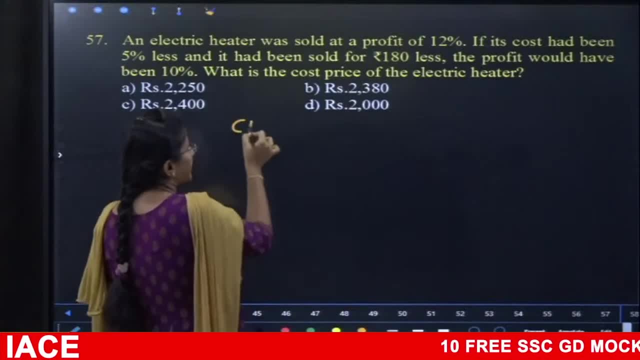 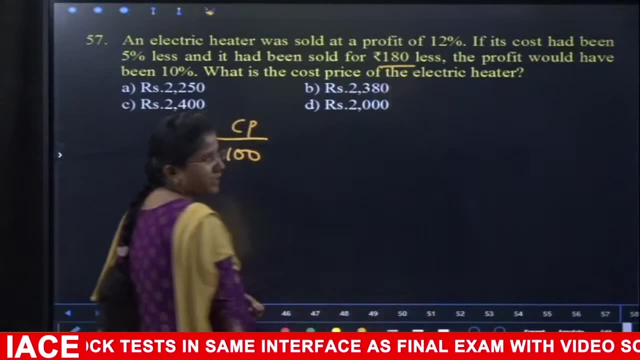 What is the cost price of the electric heater? Here, to find the cost price point, we will take any number. I am taking 100.. If the cost price is 100, then I will see how much difference I will get. So let's compare the variation. 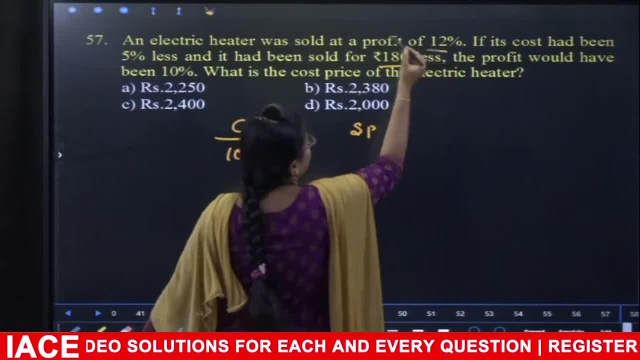 If the cost price is 100 rupees, then the selling price is sold at a profit of 12 percent. So what is the selling price? 1., 12.. And the selling price here is the selling pret, Lucien, at 10 percent. 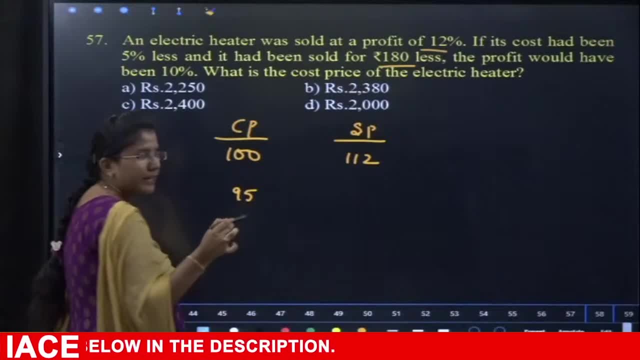 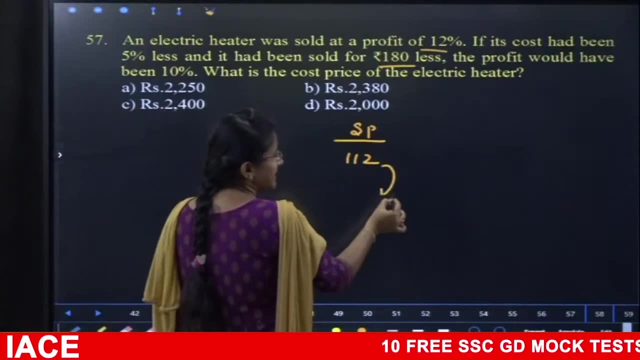 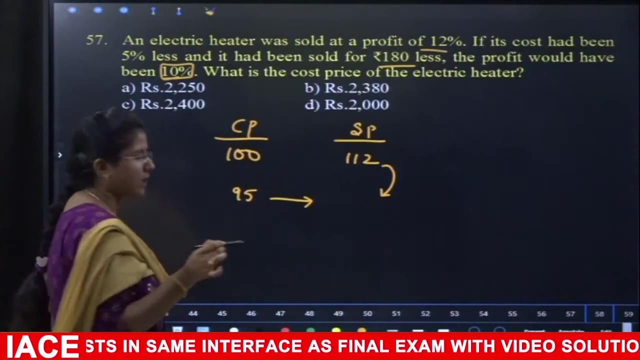 Let's see Next. if the cost had been 5 percent less at that point, so by saving that, putting 5 percent is 75 percent. after this, if it had been sold at 180 rupees less from Census, it has increased to 3.5 percent. This is a good score either way. If the profit percent had been 5 percent less, how much will it be? I have to save it to 90, 5 percent. And if the cost had been 5 percent less, what should I be able to do? if the cost had been 5% less, then I should try to take the cost half. 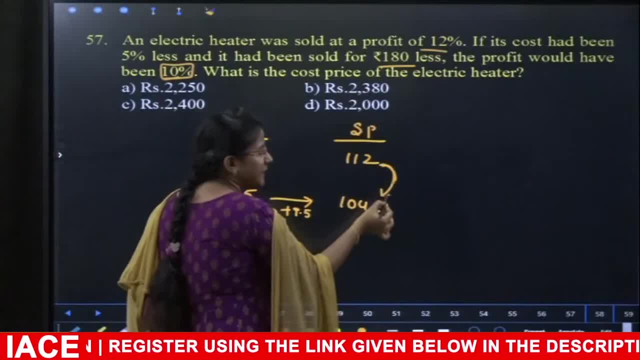 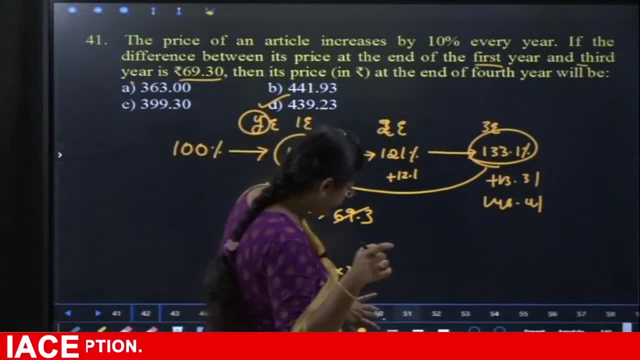 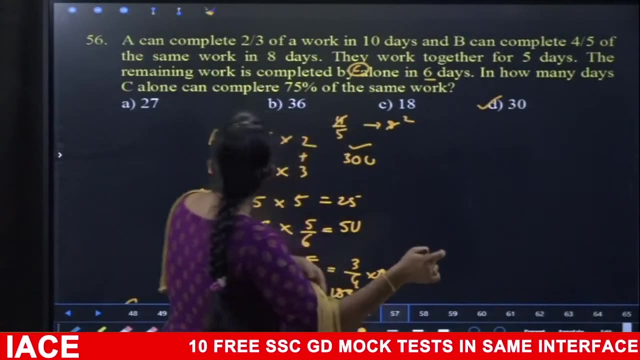 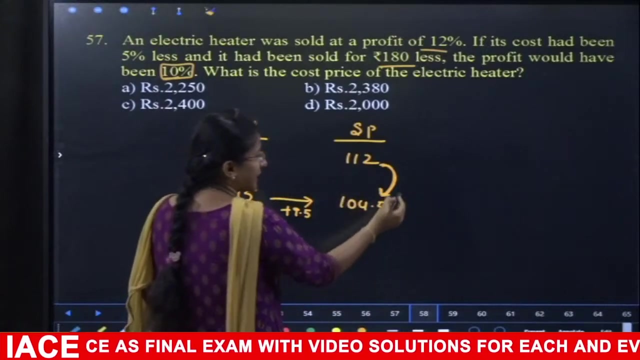 means when I take the cost price of 100 rupees, I get the deviation. I will compare how much it is. So the difference between 104 and 112, The difference between 104 and 104.5 and 112, is 7.5. 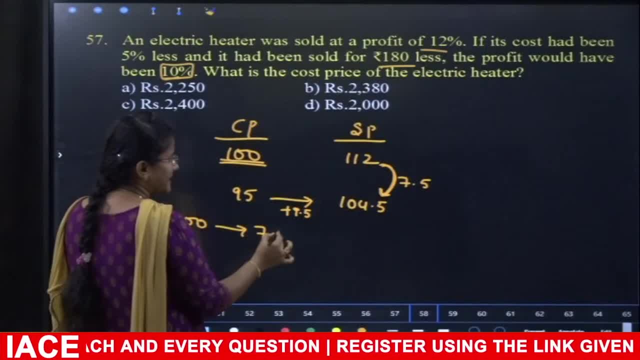 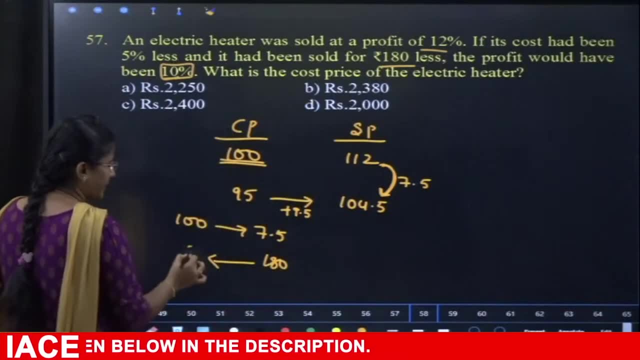 If I take the cost price of 100 rupees, I get the deviation. I will compare how much it is. If I take the cost price of 100 rupees, I get the deviation, I will compare how much it is. So the answer will be 180 into 1000 by 75. 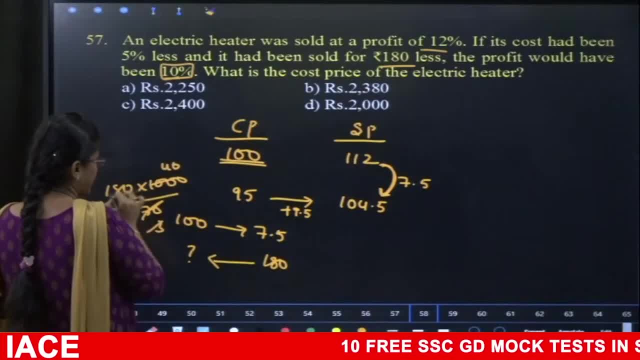 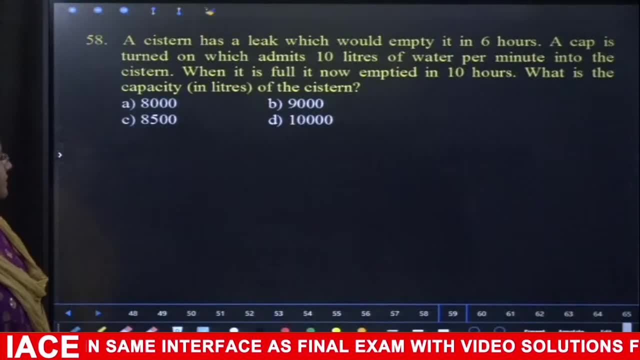 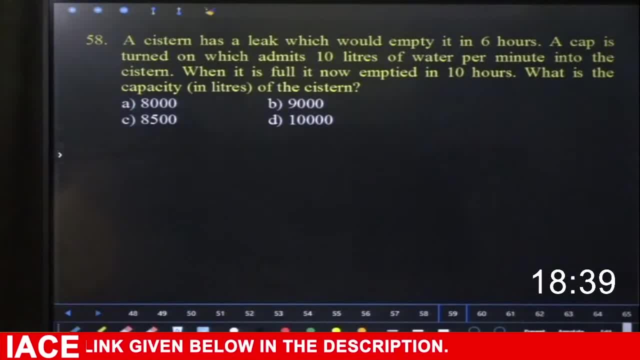 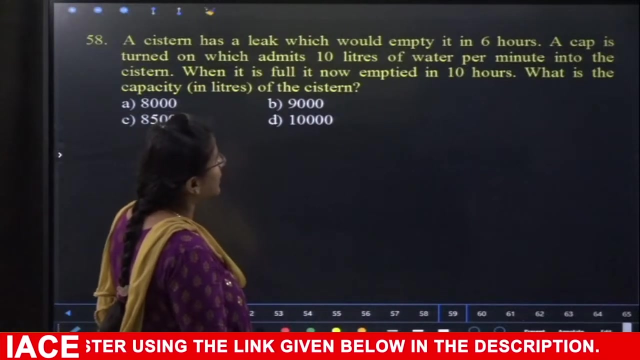 Try 58, Try 59, Try 51, Try 52, Try 53, Try 52, Try 53, Try 54. Try 55, Try 56, Try 56, Try 57. Okay, your time is up. 58. A system has a leak which would empty it in 6 hours. A cap is turned on which admits 10 liters of water per minute into the system. When it is full, it now emptied in 10 hours. What is the capacity of the system? 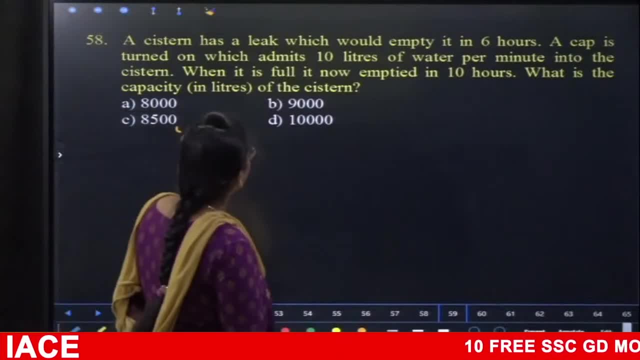 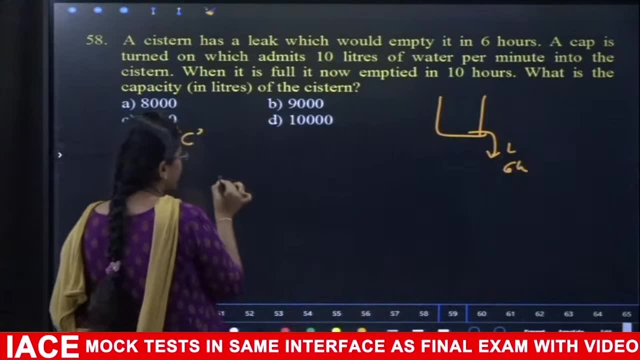 What is the capacity of the system in that place? If there is a leak in the system, how many hours can that leak be emptied? This particular leak can be emptied in 6 hours, So we can do an indication like inlet outlet or inlet leak from it. 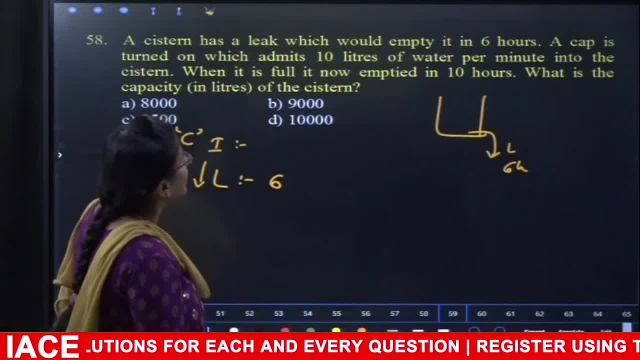 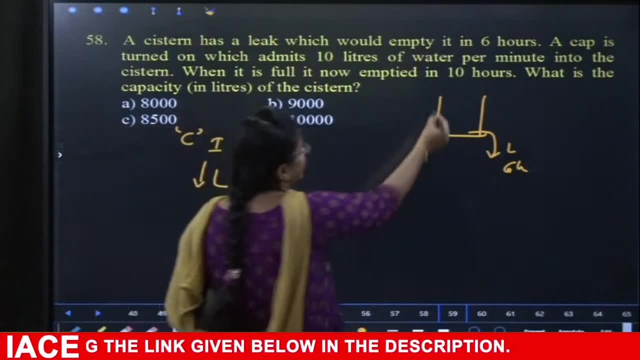 What is the capacity of the system If a cap has a system has turned on which admits 10 liters of water, a cap has turned tap at the top of the inlet. What is that doing? For 1 minute, 10 liters of water is turned on. 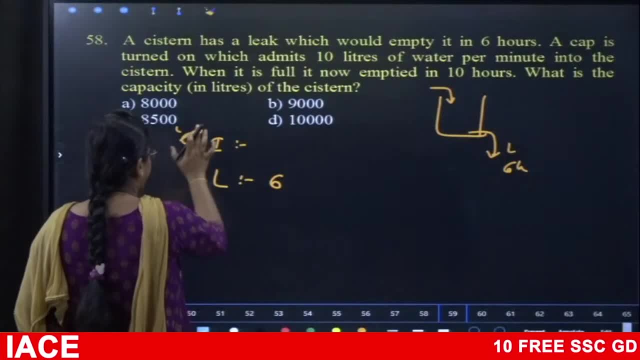 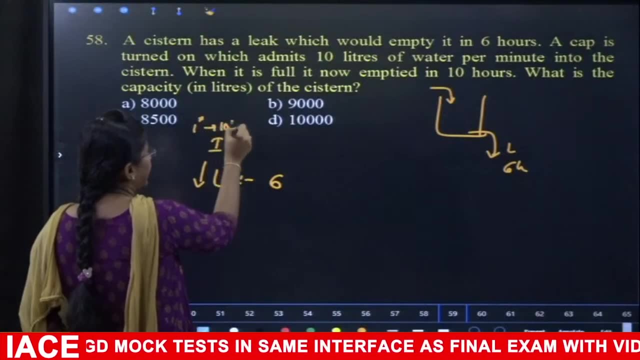 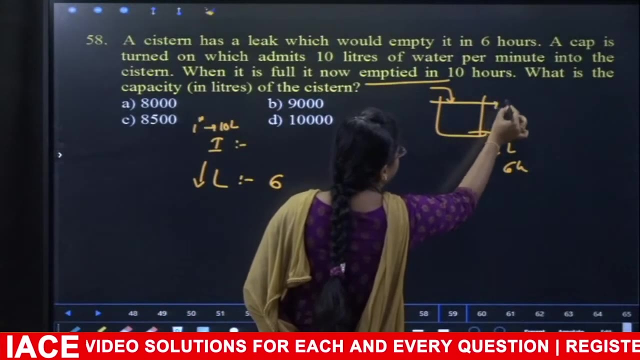 What is the capacity of the system? liters, so one minute, 10 liters. so one minute, 10 liters. one minute, 10 liters. next, when it is full, it is now emptied in 10 hours. okay, well, a tank is on the full life. I will not like the inlet to. 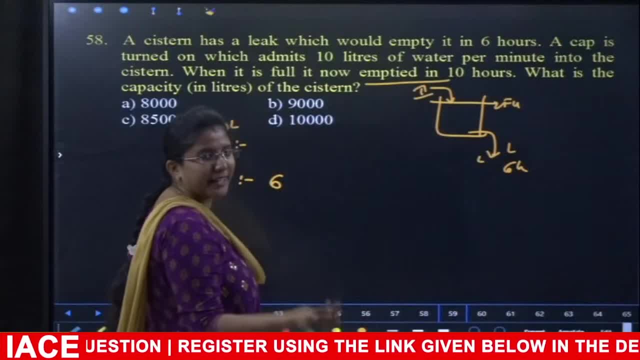 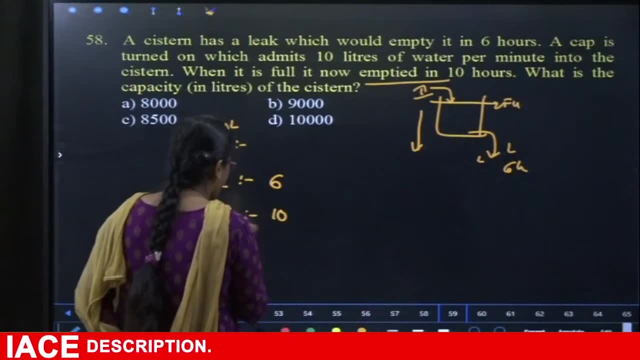 e leakage you're into parallel. you have a chest up, bro, in our slow tank empty out on the shepherd and a national time to empty out on the ten national tank inlet and the outlet ten national tank empty of children on a only leak, matrimonial to success: the empty shaker do in light photo. 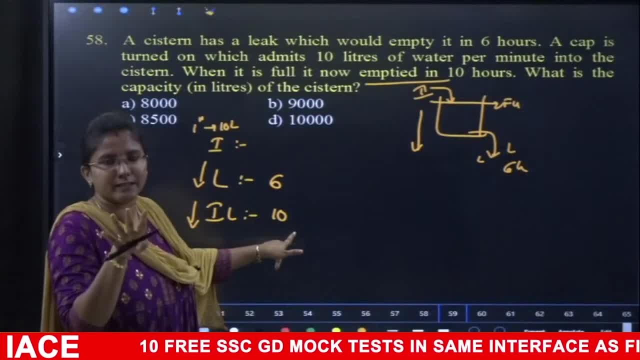 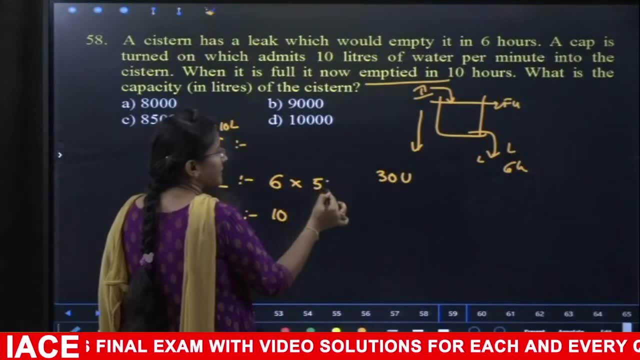 on the wall and extra in our time but in the day for us overall gain, our 10 hours, six. and then I take tank as some 30 units on turn. 30 units on that lady leak will empty. how many units for one or five units? inlet outlet, caliphate, any units modern leak out in? I only three units a. 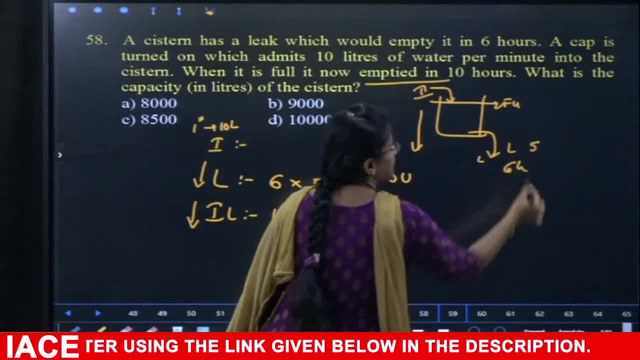 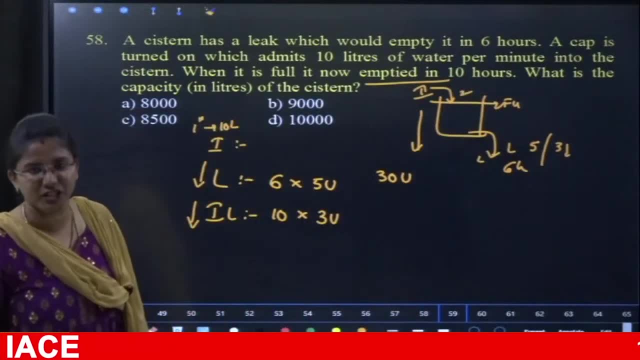 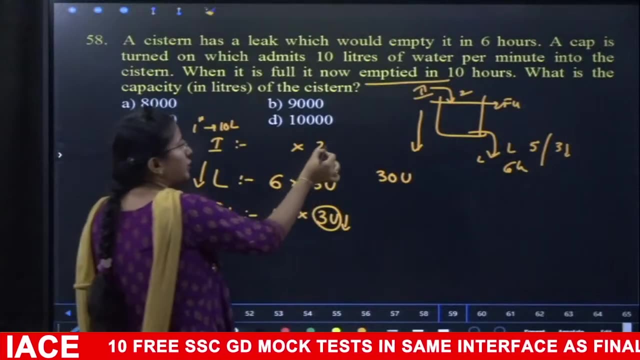 legal leak of a tea. five units empty circle capacity in the inlet outlet in about only three matrimony by together nine times are going down and take over two units of water and any let it fill chest. oh darling, so I could have money. because to Rastan, so to minus five will be open day, minus three, open another. so you could do. 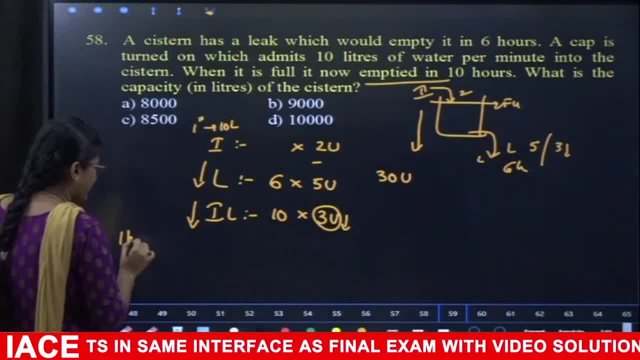 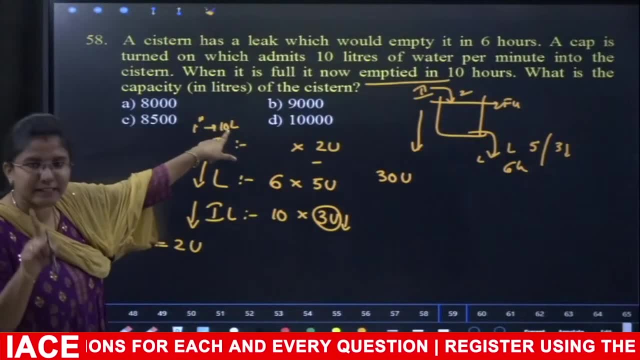 you know. so efficiency, which in the front a one hour coaching and the one are can units to units. so, Connie, it's in the car. one minute I can take. one minute you can tell you leaders. one minute you can tell you to say the one are one, aren't a 60 minutes, see minutes. cover tail, open the. 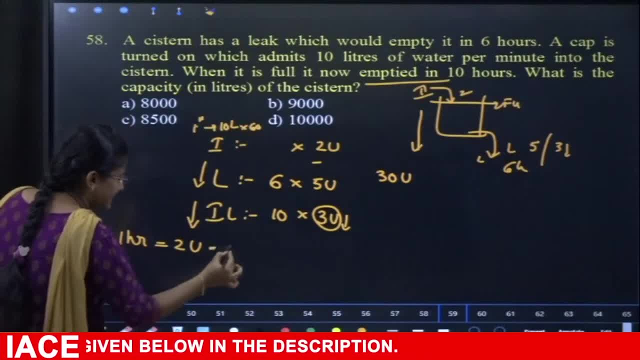 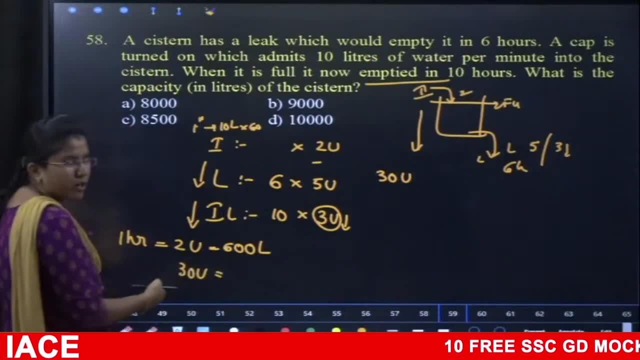 ending to 60 oh and 60 cent, and the tank load two units of a value, 600 liters, on my man upon the total time to 30 minutes cada capacity into total this window, so doing to 30, 30 dollar and a 15 times. 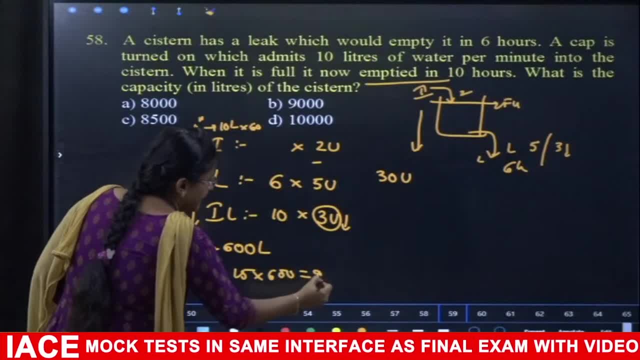 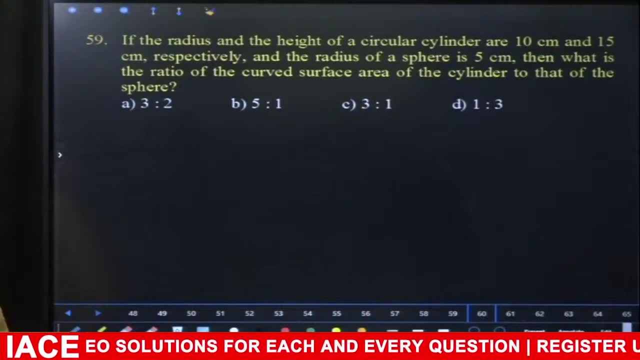 science are 15 into 600. answer. and then the 9,000 liters. answer. option D: okay, next, go for move. for next one: 59. try sharing the media. the 30 seconds timer. please get go. we're gonna let you guys do Q and A with your unique. 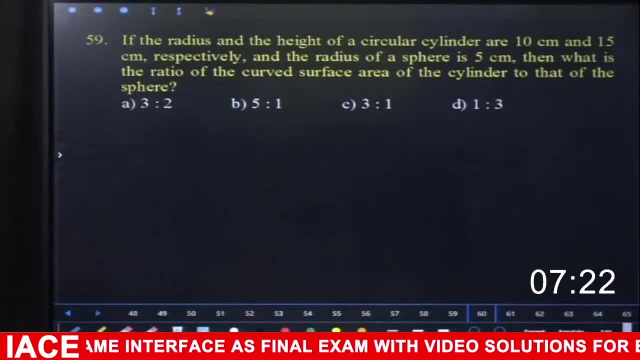 so get excited all together over the course of 30 minutes. You guys just head time in five. one an hour up on that won't take up time forever. Okay, Do another looking at the share center for a couple of minutes. tone will get all the other gens that in the chat and we'll take over the break up and ending. 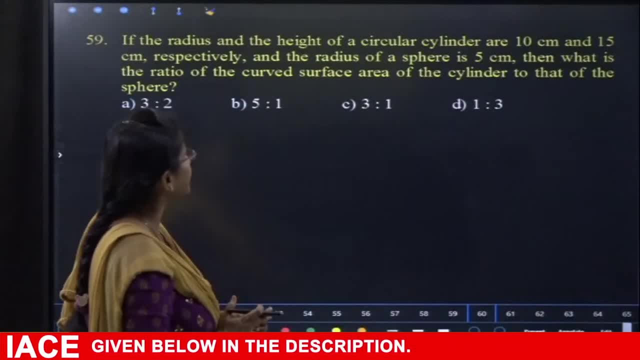 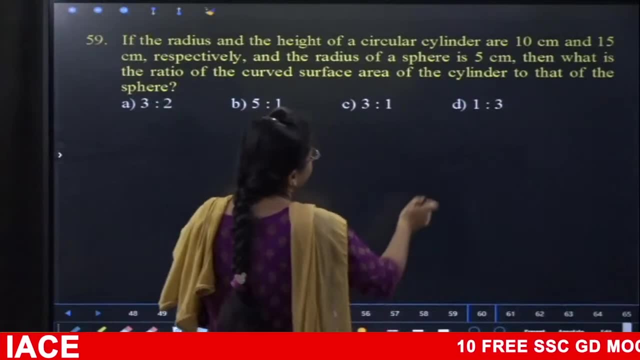 up. So here the question is very easy. If the radius and height of a circular cylinder are 10 centimeters and 15 centimeters respectively, and radius of a sphere is 5 centimeters, We have numericals in 10,, 15, 5.. What is the ratio of curved surface, area of cylinder and curved surface? 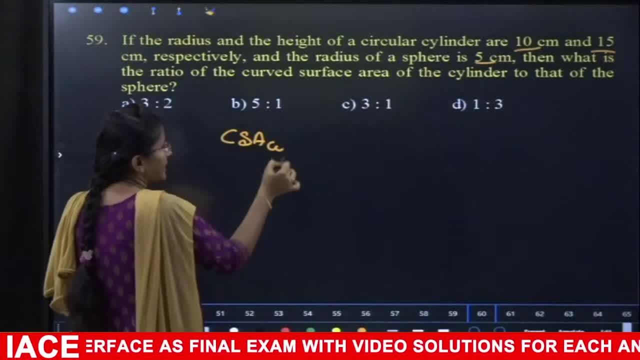 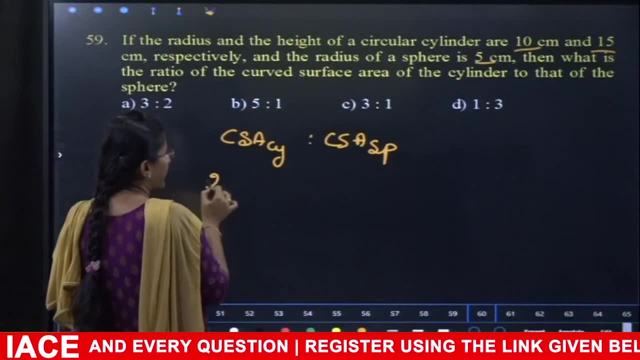 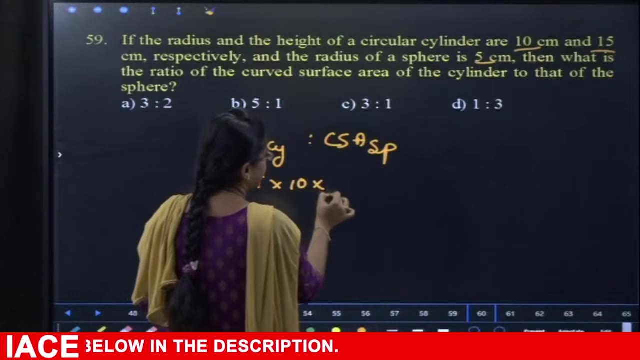 area of sphere For the curved surface area of cylinder. and for the curved surface area of sphere, we have to find out the ratio. For the curved surface area of cylinder, formula 2 pi, r, h 2 pi. How much is the radius? It is 10.. How much is the height? 15.. Is to 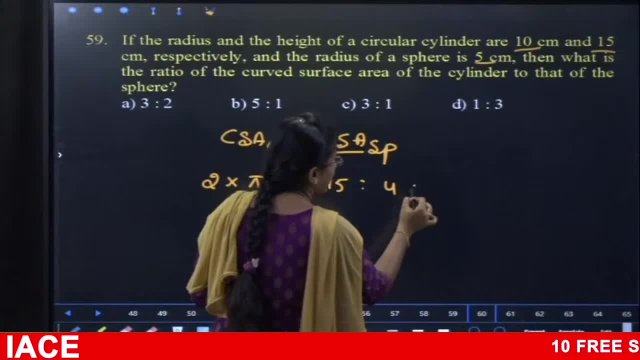 Give radius to the sphere. What will be the curved surface area of the sphere? 4 pi r square r square is given to us as 5 square Pi and pi cancel out 2 and 2 times. So next here. 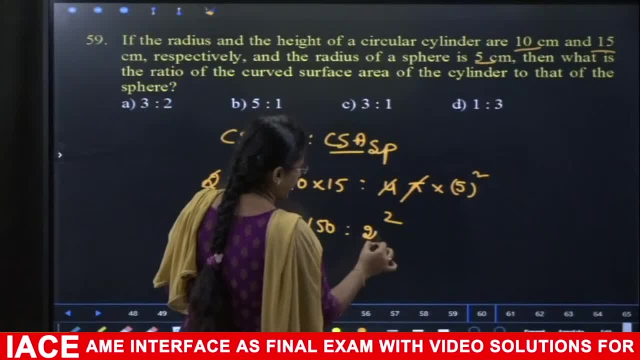 we have: 150 is to 20.. 25,- 2 is 50.. 25,- 2 is 50.. What is the ratio of 150?? 3 is to 1.. Option C: 3 is to 1.. 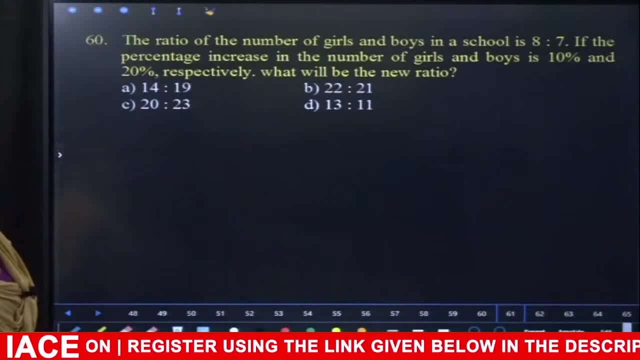 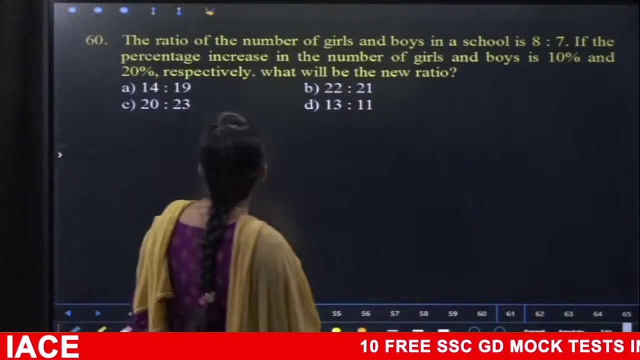 Very easy bit. Next 60.. Try 60.. This is also very easy. 30 seconds time, please. Okay, Your time is up. This is also a very easy equation. You can answer within seconds. The ratio of number of girls and boys is 80 to 7. And the percent is increasing The number. 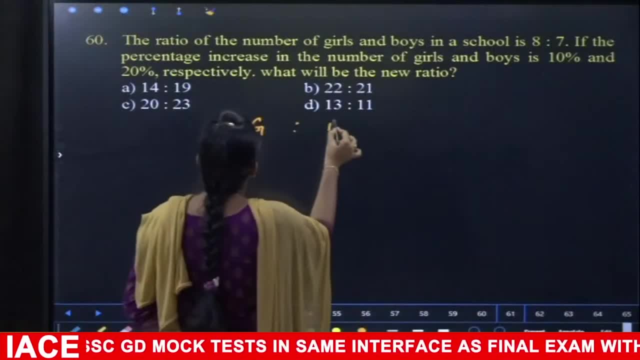 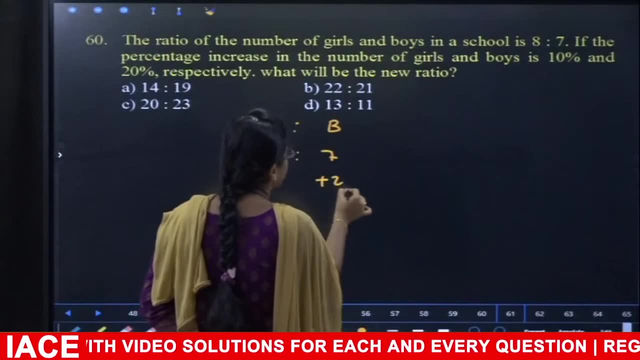 of girls and boys is 10 percent And 10 percent. He gave the ratio of 80 to 7. Girls increased by 10 percent and boys increased by 20 percent. We don't know the initial values. It is 100. 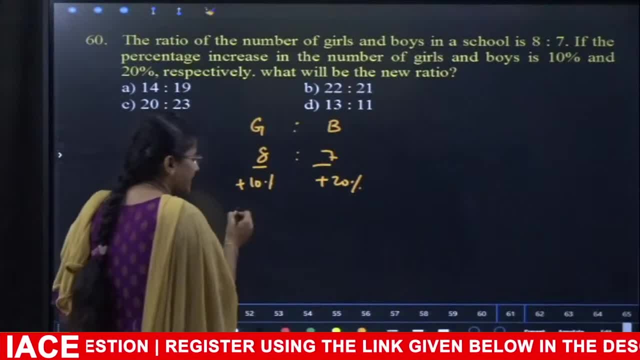 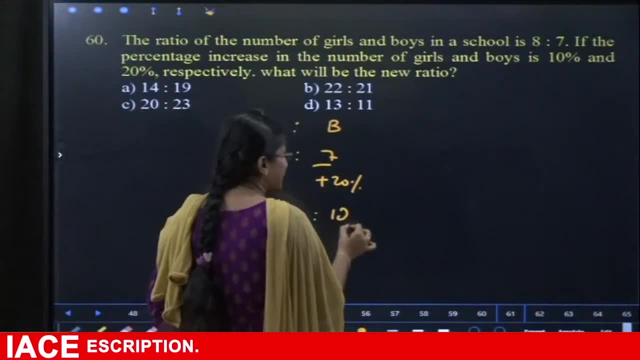 percent. If we increase 10 by 100, how much is 100 plus 10? 110 into 8.. He asked the ratio again. He wrote that If we increase 100 percent by 20, what will happen? 120 into how many parts? 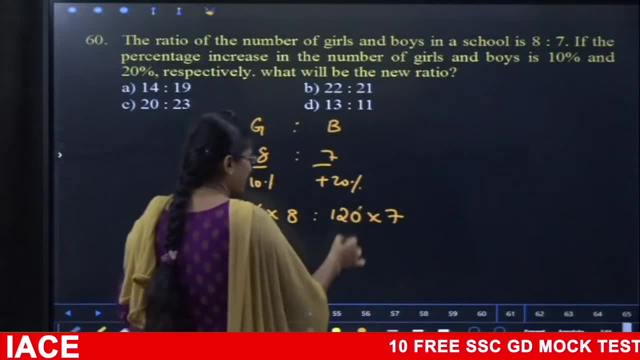 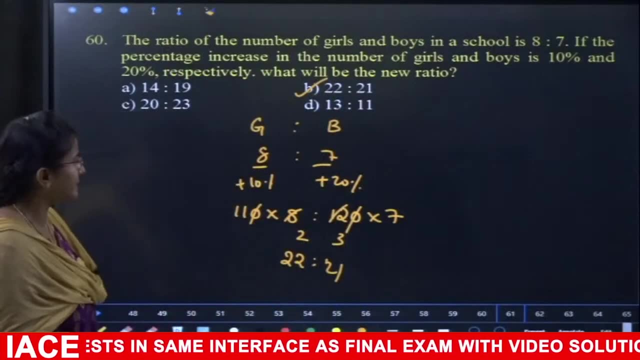 7 parts. Simply, we will write only this. So if we cancel out 0s, this will be for 4, 3s and 4 2s. Answer 22 is to 21.. Option B: Okay, Next. Go for next one: 61. Try 61.. 30 seconds. 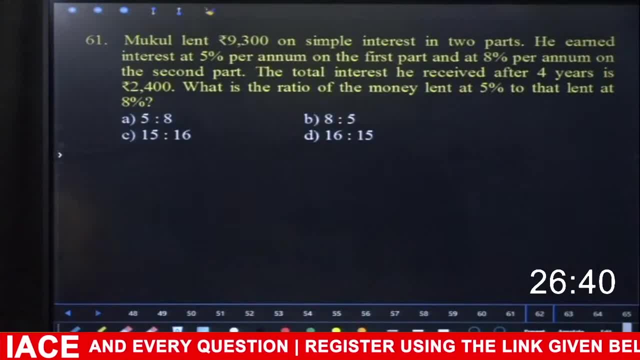 timer please. This is the highest time limit given, So for the last five seconds it is based on 1.. After that, calculate how many parts of girls and boys will have this particular value. So what we have is a 3 plus 2, 6 plus 3, 3 plus 3, 2 plus 2, 2 plus 3, 2 plus 2 plus. 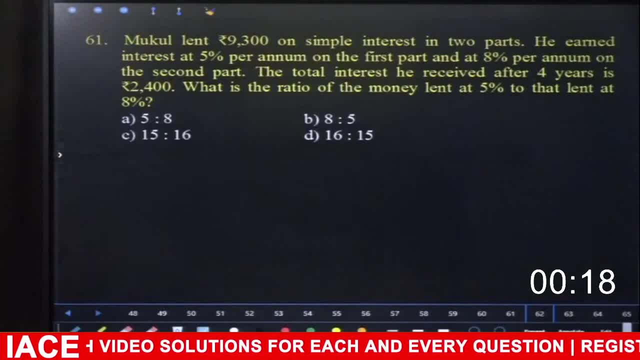 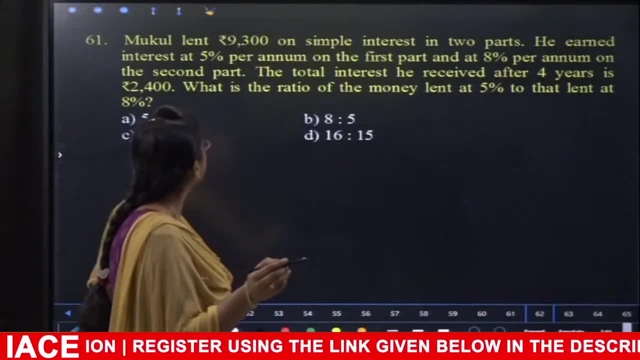 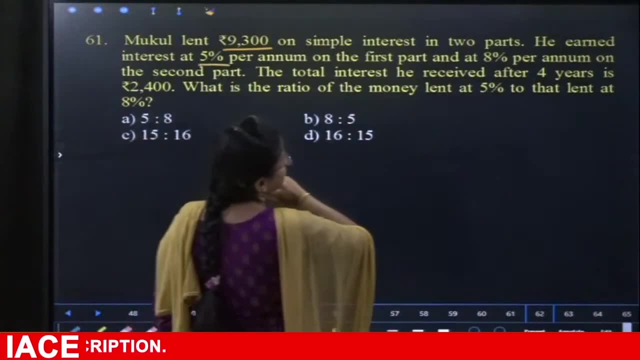 So this question is easy. We will use the allegation for this. Mohan lent 9300 on simple interest in two parts. He earned interest of 5% on the first part and 8% on the second part. Total interest he received after 4 years is 2400.. 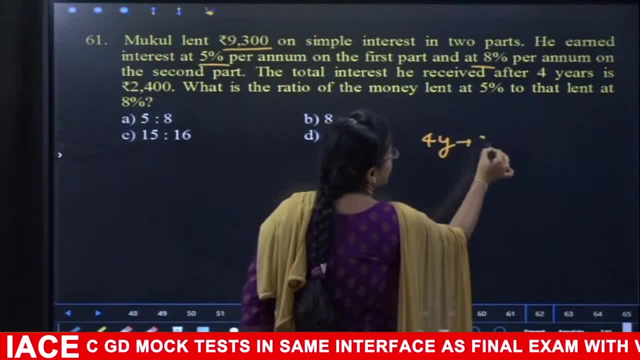 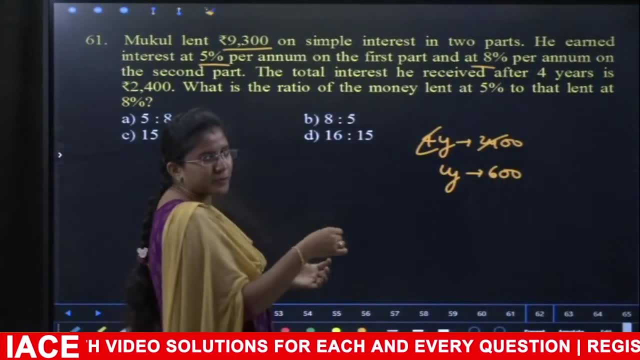 Since it is a simple interest, we can write it once. If 2400 interest is earned in 4 years, what is the interest for 1 year? 1 year it is what It is: 600.. He did not give rate of interest percent to this 600.. We will find it out ourselves. 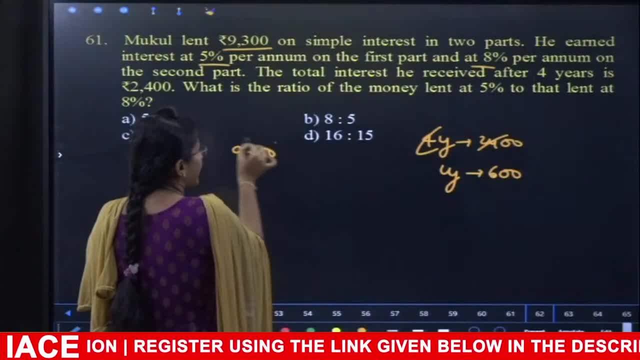 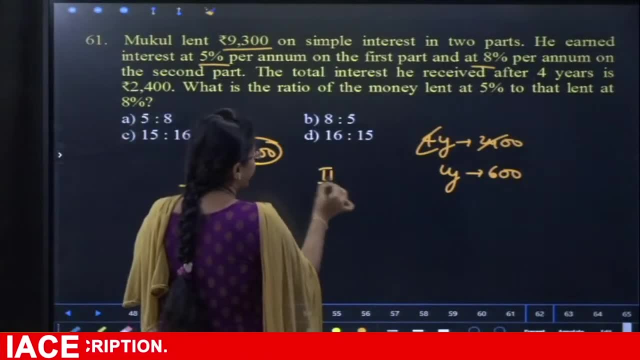 So total interest amount he lent is 9300.. In that the rate of interest he lent in the first part is 5%. In the second part he lent at the rate of 8%. Here we will find out the middle part to give the overall allegation. 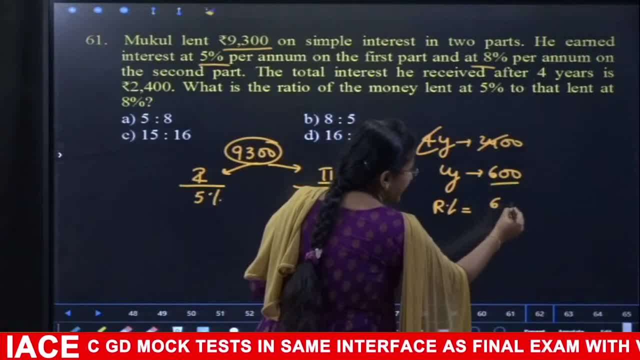 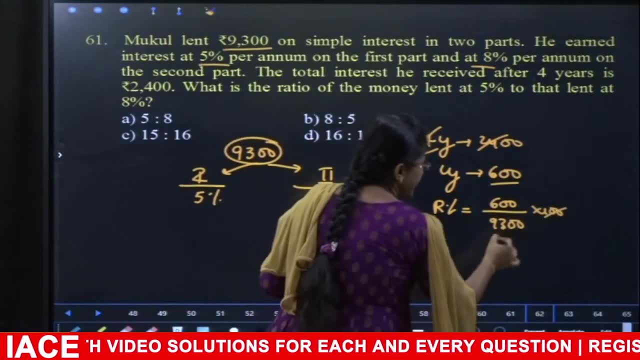 So to find out the rate of interest: interest is 600 for 1 year. The principal he gave is 9300.. How much percent is there overall? We can write it like this Here: if we cancel out all the zeros, it will be 600 by 93.. 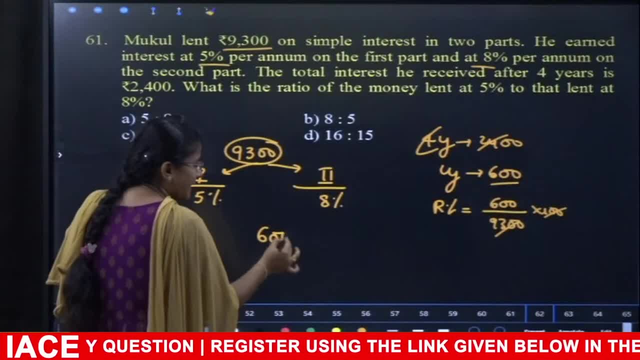 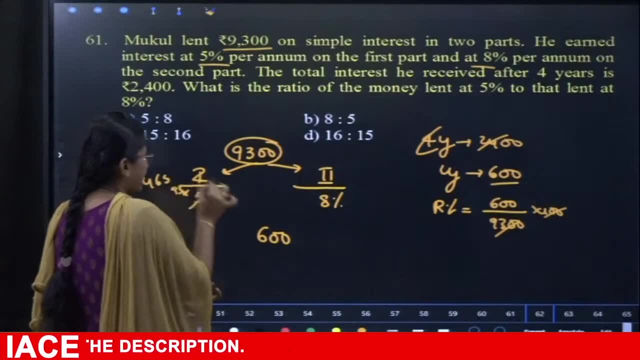 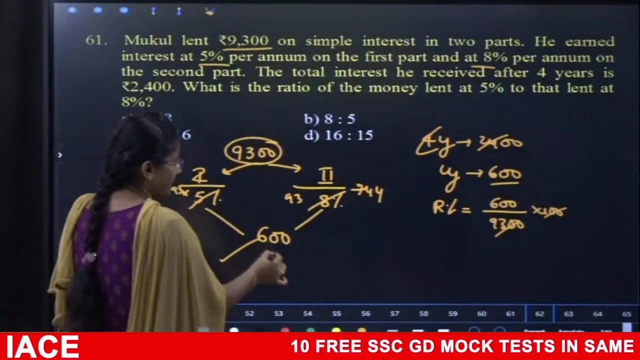 Since it is a fraction, write 600 here and multiply the denominator 93 here. So 93 into 5, that will be for 465.. So the same 93 into 8, that will be for 744.. So here, when we write the allegation, the difference is 744 and 600 is for 144.. 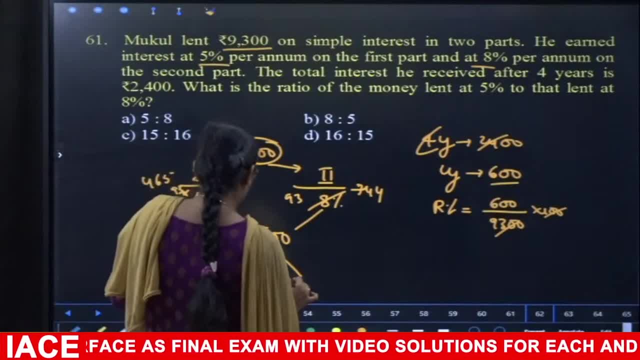 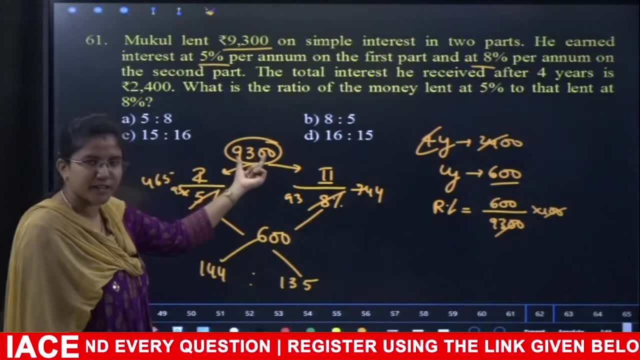 Next 465 and 600 is for. that is 134.. 35.. So the ratio, how many parts are there in the first part and how many parts are there in the second part? The whole 9300 is divided by the ratio when we use the allegation. 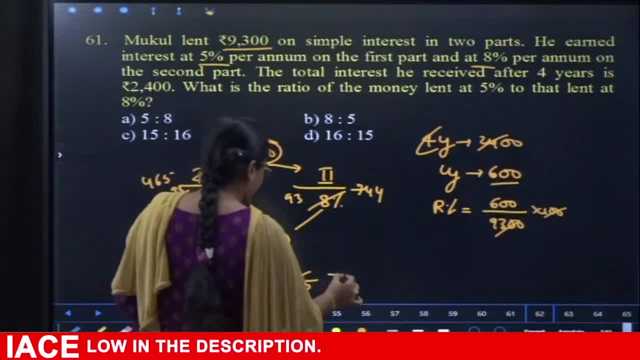 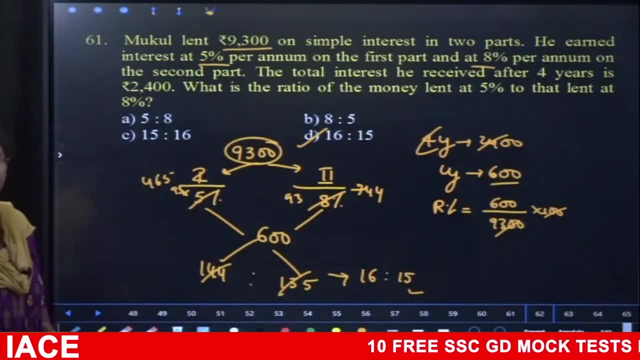 So here 144 and 135 cancel out in 9. How many times in 9? 16 times. So this is 15 times. So the ratio option D, 16 is to 15.. Okay, Next. 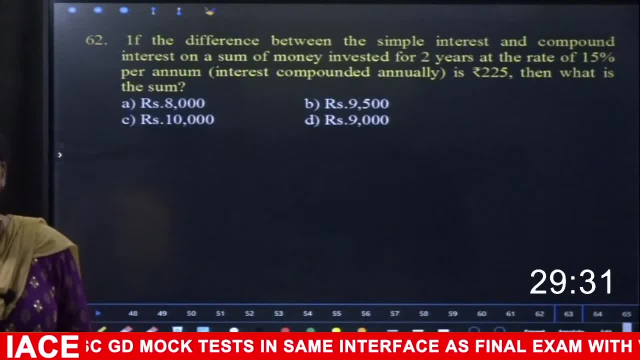 Go for the next one: 62. 30 seconds timer. Next, Go for the next one: 62. 30 seconds timer. Next: 31. 31.. Your time is up, So this question is a very easy question. 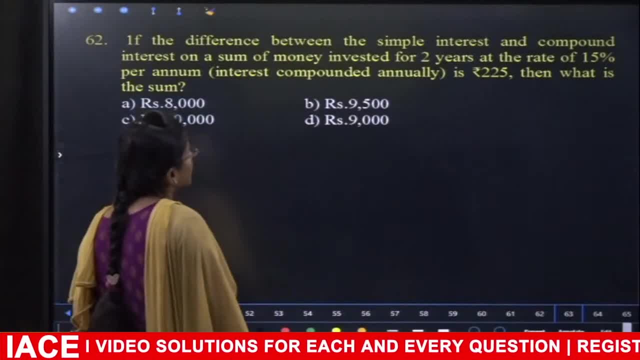 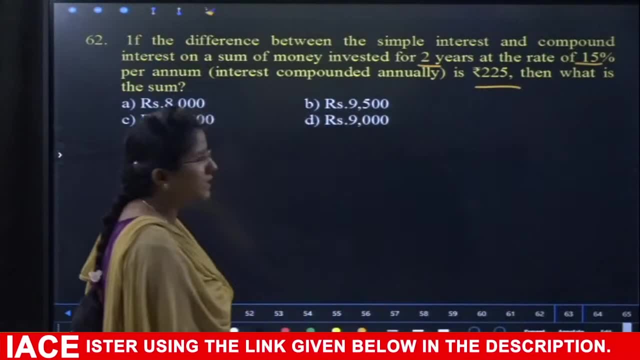 He gave a difference. If the difference between the simple and compound interest, or a sum of money invested for 2 years at the rate of 15%, is 225 rupees, then what is the sum? He is asking the principle. So, since he gave the difference, 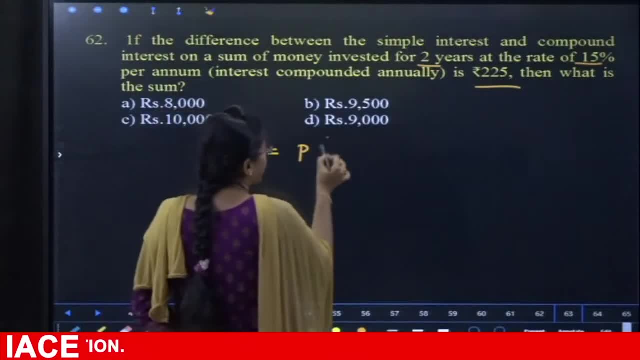 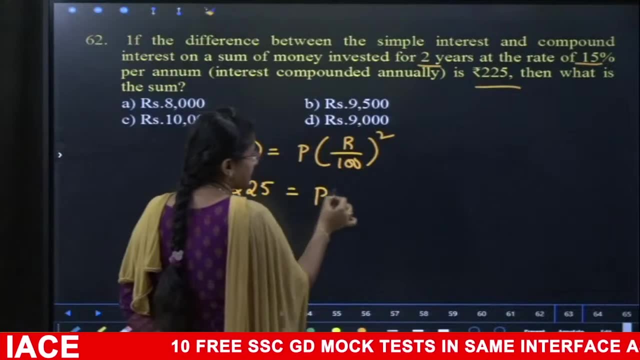 for 2 years. we will use this formula. What is the difference equal to P into R by 100 whole square, So difference already given in the question 225.. We have to find out the principle. He gave the rate of interest at 15%. 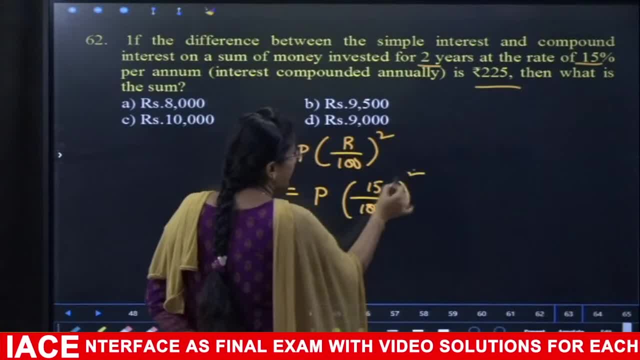 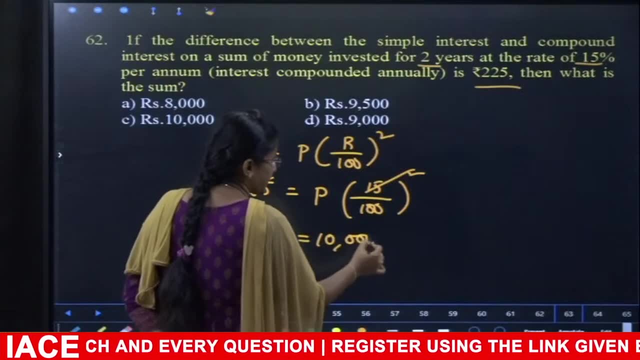 by 100.. Whole square, 15 square, will be 225, right 225, 225. cancel out 100 square is what Answer? Principle is 10,000 rupees, Okay. So option C: Okay. As simple as that. 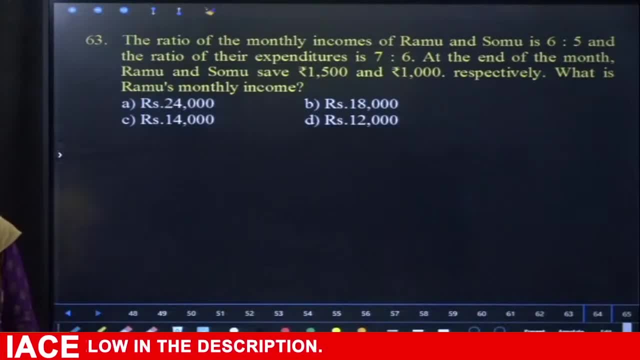 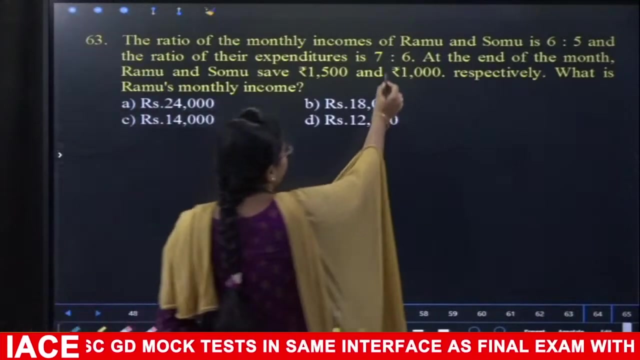 Next go for next one: 63., 63,, try 63,. ratio of monthly incomes of Ramo and Soma is 6 is to 5 and the ratio of their expenditures is 7 is to 6.. And the 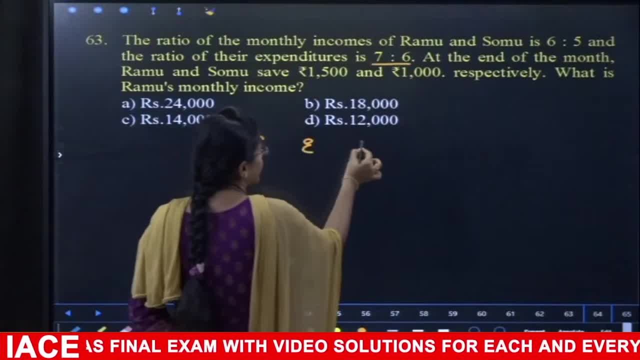 same ratio of monthly incomes of Ramo and Soma is 6 is to 5.. Savings is 1500. Incomes expenditure saving. So income expenditure saving relation, always income equal to expenditure plus saving is written Incomes ratio. 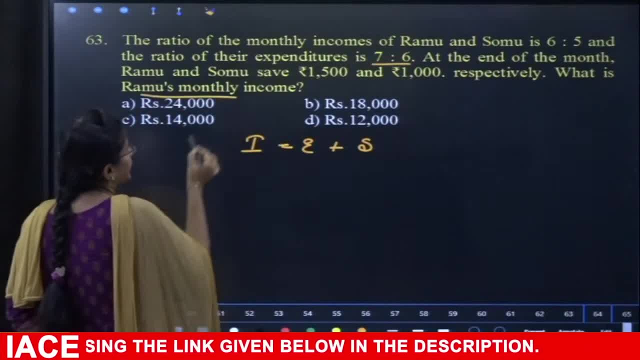 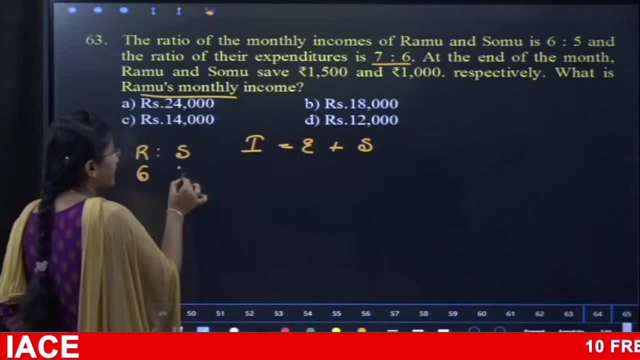 already given to Ramo and Soma. Question is: Ramo's monthly income is how much? So we use X or P for incomes. So incomes ratio is given to us as 6, 5,, 6 is to 5.. That is 6X. 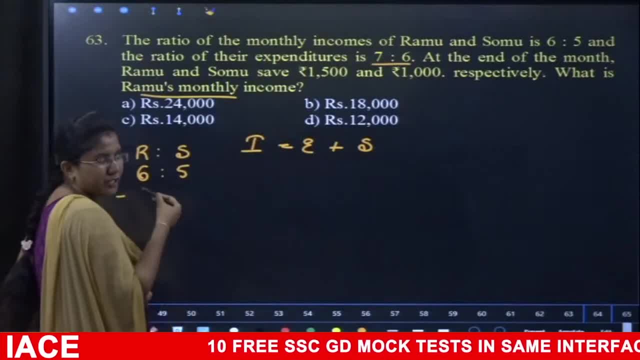 and 5X incomes. If savings are deducted from these incomes it will be expenditure. How much savings should be deducted here for Ramo? 1500 should be deducted. So this is the ratio of savings. How much should be deducted here for Ramo? 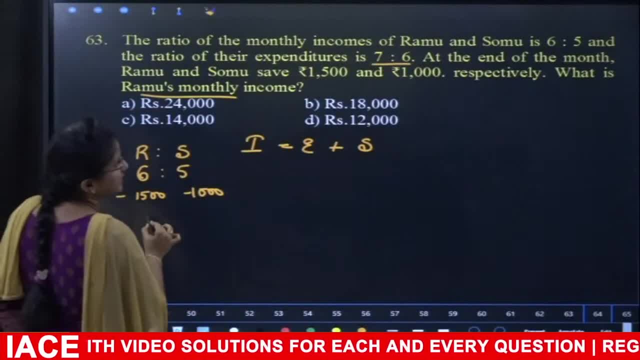 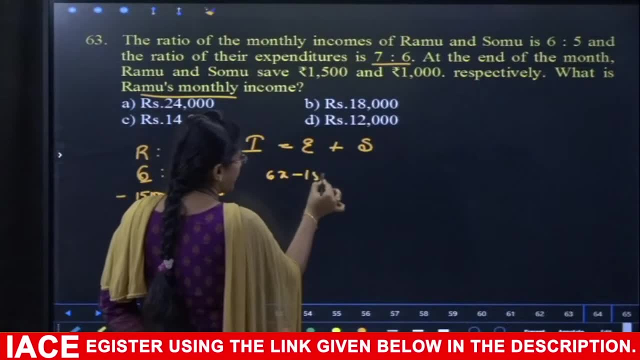 1000 should be deducted. If savings are deducted, how should be the expenditure ratio? It is 7 is to 6.. We use this only 6 parts and 5 parts: 6X minus 1500 by 5X minus, saving 1000 rupees. 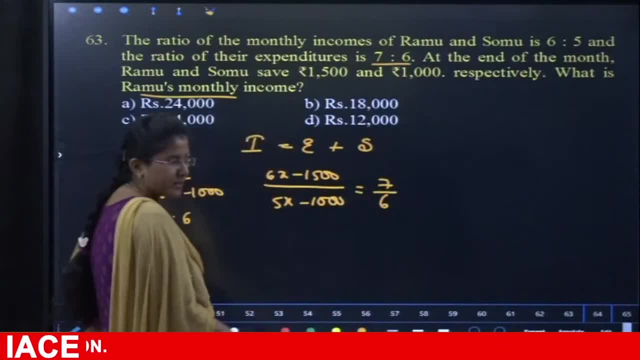 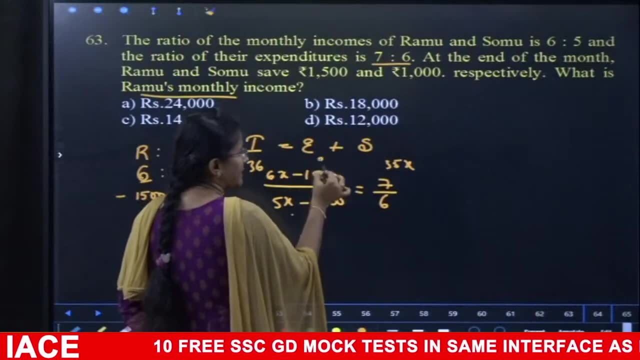 how should be the ratio of expenditure? 7 is to 6.. Here we have: 6X is 36X and 7X is 35X. The difference is X. Next here, 15X is 9000.. Minus 9000.. 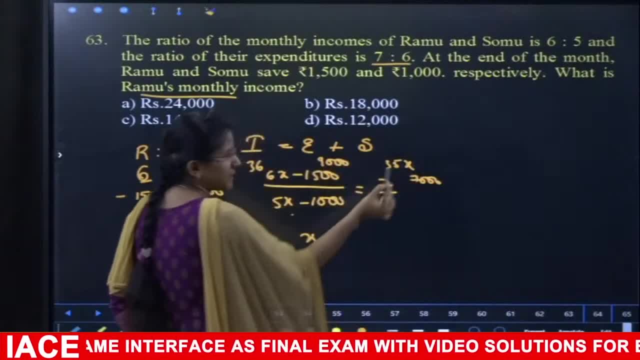 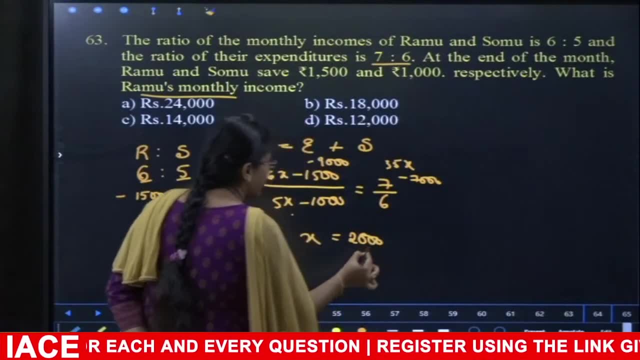 On the other side it is 7000.. On this side it is minus plus 9000. minus 7000 will be 2000.. So X value is 2000.. So what is the income of Ramo? 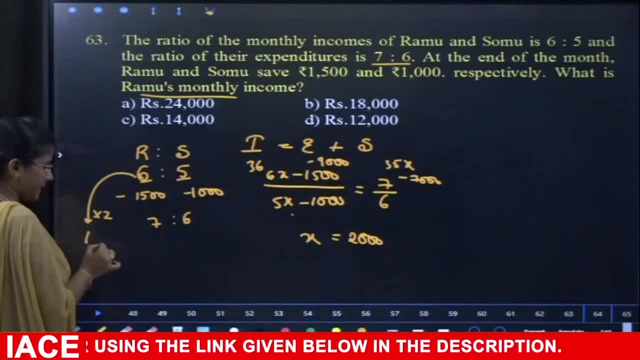 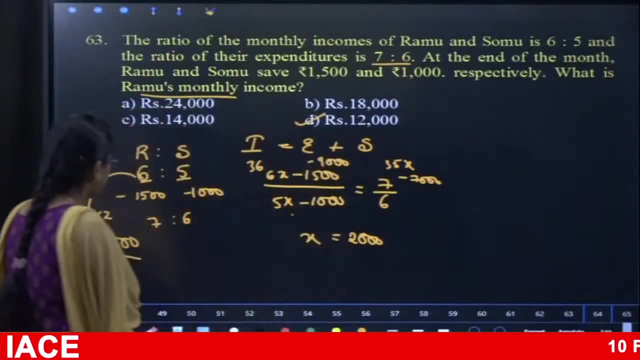 Ramo has 6 parts, So 6X is 12000.. We will do either option verification or normal solving. Option D: Next 64.. Go for 64.. Next go for 64.. Next, go for 64.. 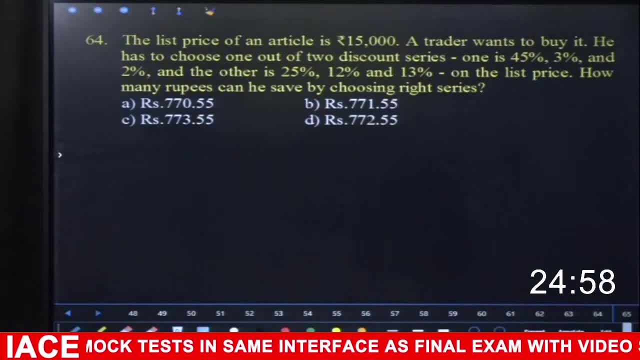 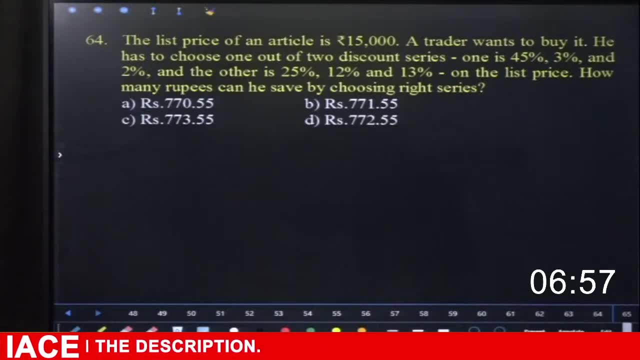 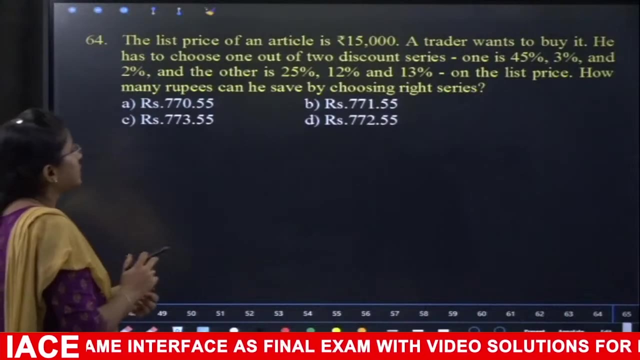 Next go for 66. Ramo has 66. Then textbooks account is optimistic. Rach �аты uncomмат bi Sugat Pasik Taise. This is a bit time-consuming for us In our calculations. it is not that time-consuming. 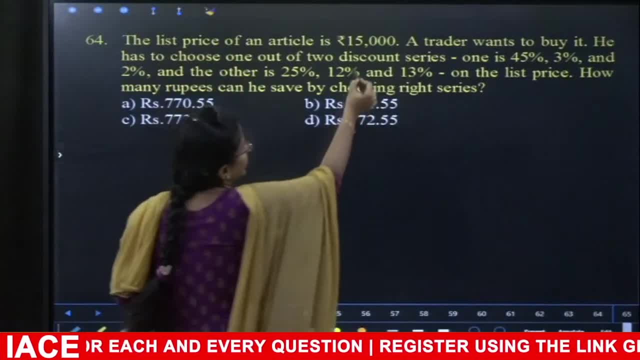 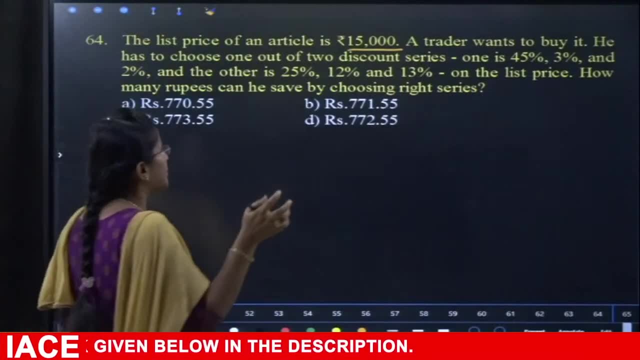 We can put a tricky option for this. List price of an article is 15,000.. A trader wants to buy it. He had to choose one out of the two discount series. He gave two types of discounts here: List price or market price. 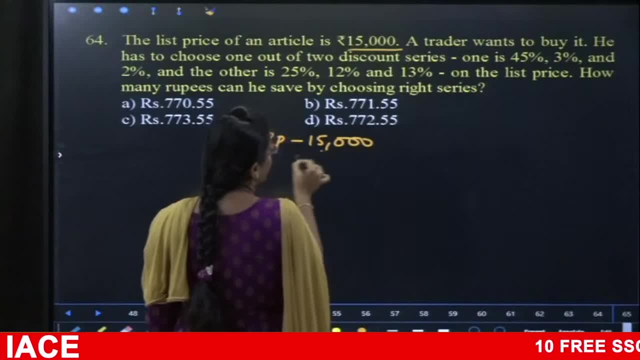 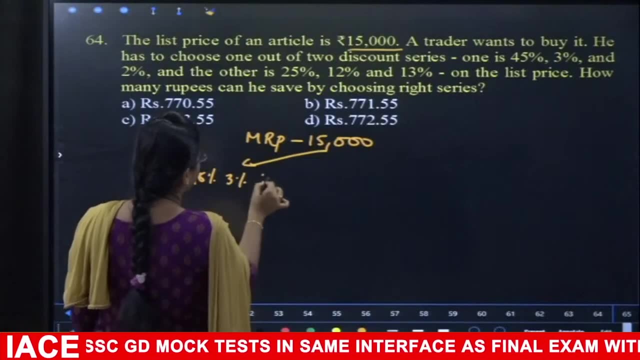 MRP is given as 15,000.. On this 15,000, the discount series given to us. the first discount series given to us, 45%, and then 3%, and then 2%. Next, the discount given to us on the same 15,000,. 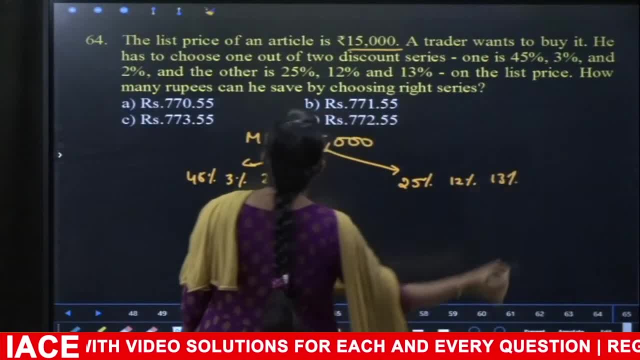 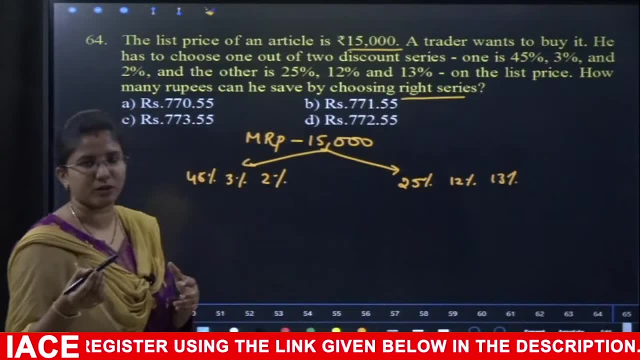 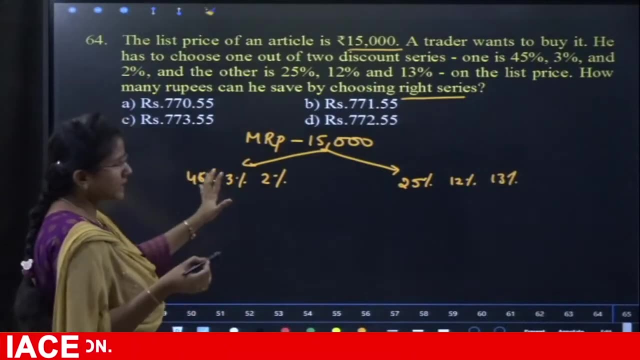 25%, 12% and 13%. Then how many rupees can he save by choosing the right series, The price at which the right series gets the highest discount? He is asking how much he can save by taking that discount. We write the selling price. 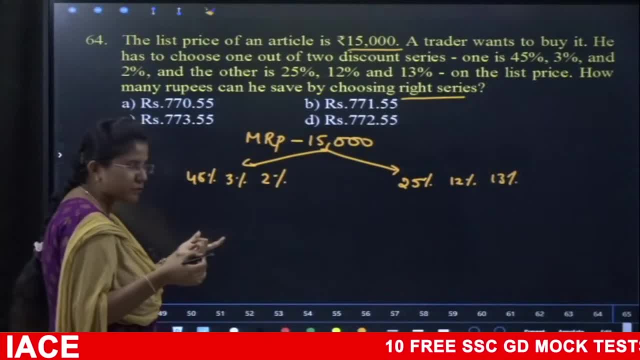 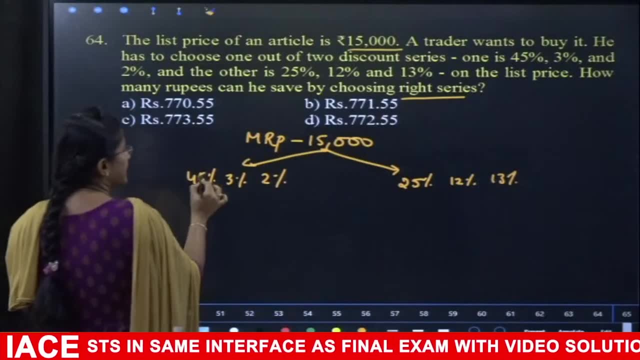 It is to differentiate the selling price. If the selling price is 2000 and 1500 is given there, how much will be saved? That is the difference. So when we write the selling price, we write it as a series, as there are 45% and 2% here. 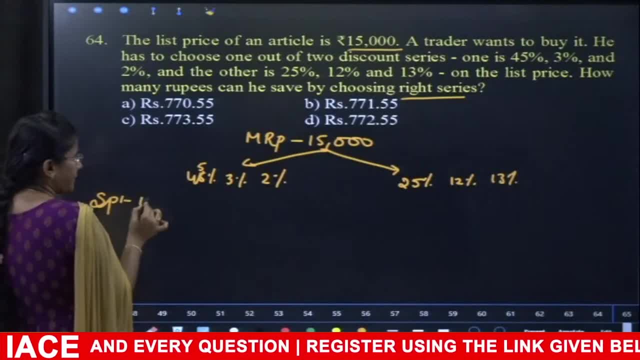 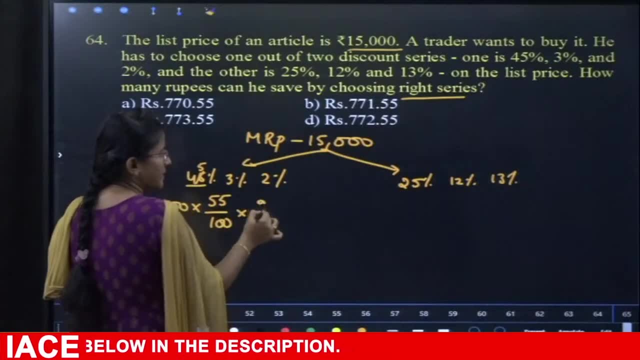 So here the selling price on the first case will be 15,000.. How much is the remaining discount of 45%: 55 by 100.. How much is the discount of 3%: 97 by 100.. How much is the discount of 2%? 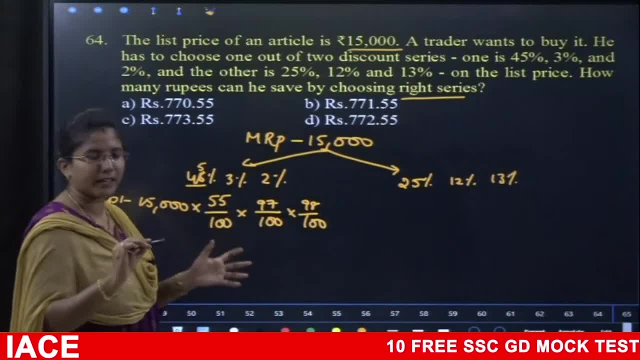 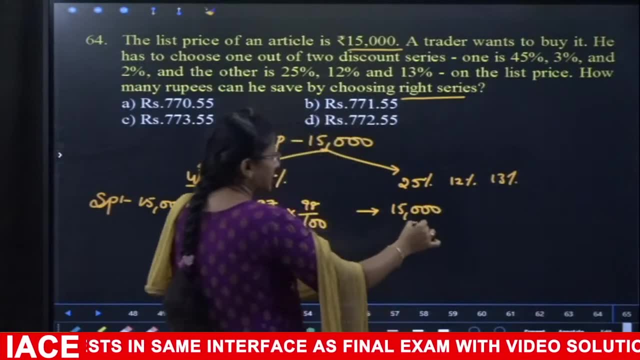 98 by 100.. Here our calculation is very tough, But since he asked for the difference, we can check multiple and give the answer. The difference is 15,000. on the same amount, 25% discount is 3 by 4.. 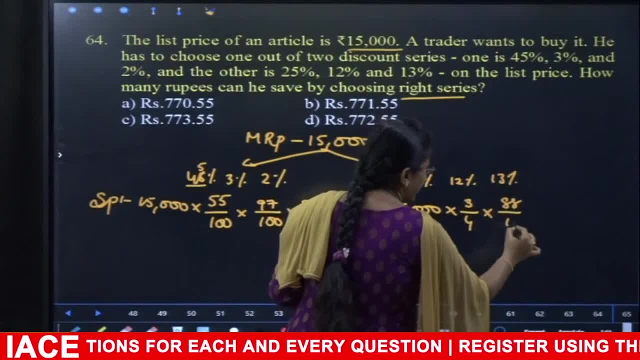 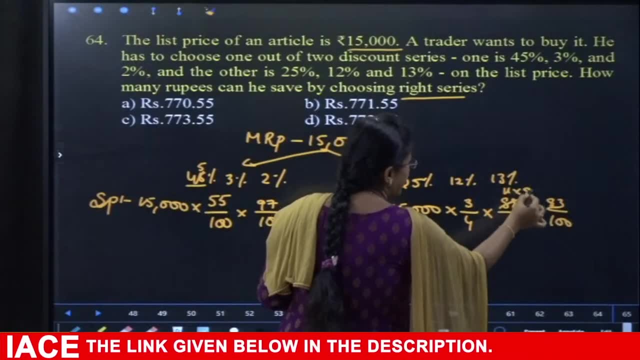 75% will be there. 12% will be 88 by 100.. 13% will be 83 by 100.. So here 88 can be written as 11 by 8.. When we cancel out with 8 and 4, we get 11.. 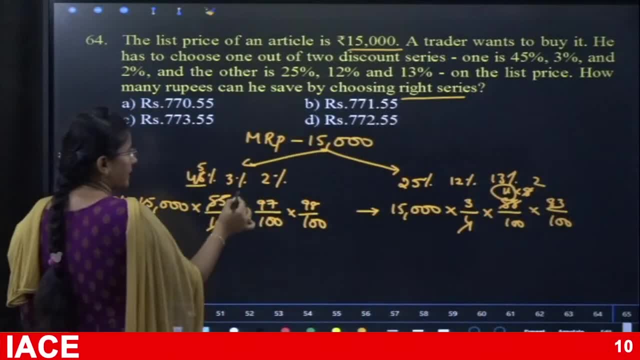 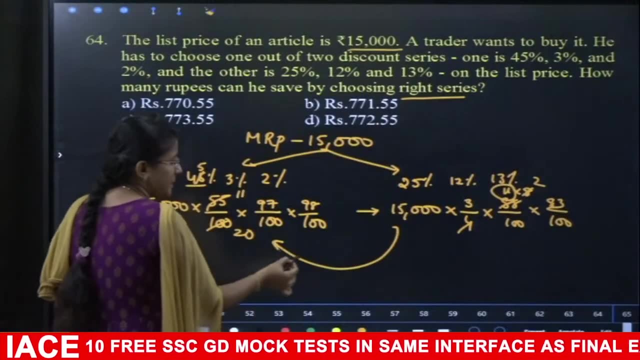 Next, like that, this side also, 55 by 100, is 11 by 25.. 11 times or 20 times. Since he asked for the difference, the selling price here and the selling price here. In between, the difference will definitely be multiplied by 11.. 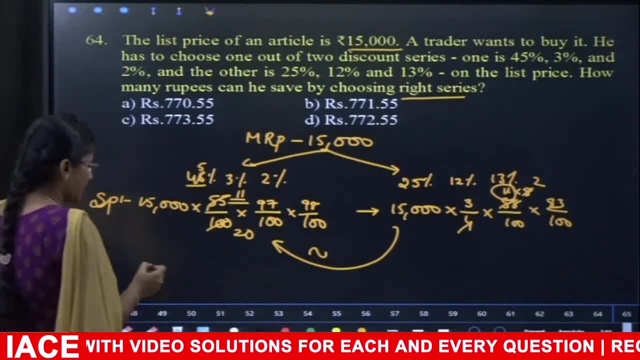 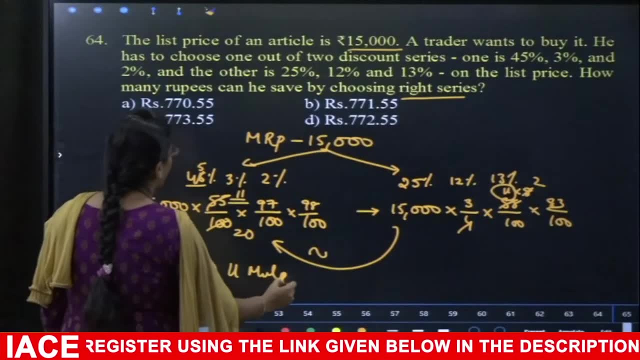 So, without doing any other calculations, without doing any other questions, the difference between the selling prices should be 11 multiple. What is the difference between the selling prices? Keep that option. So what is the option? There is only one option, option A. 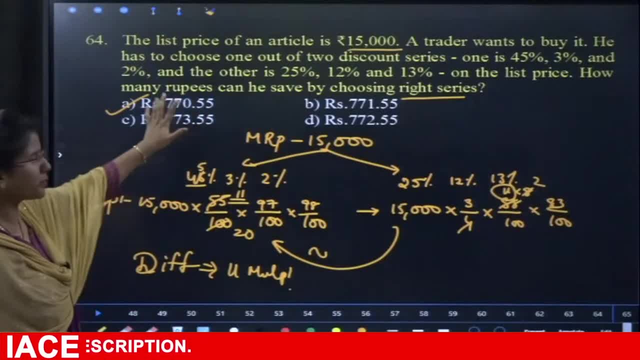 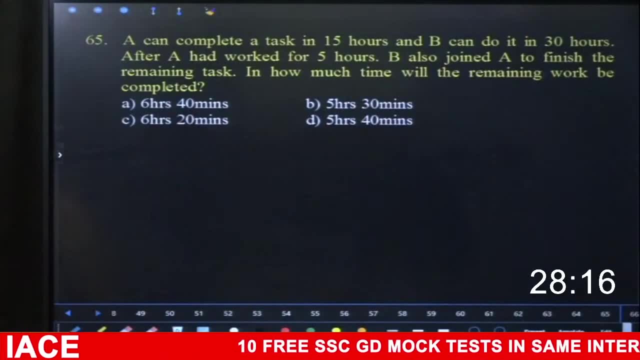 770.55.. Is it okay? Option A is the answer for this. Next, go for 65.. 65, 30 seconds timer, please. Okay, our time is up Time and work. question A can complete a task in 15 hours. 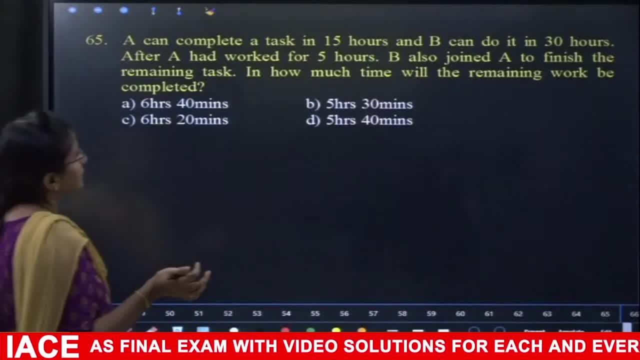 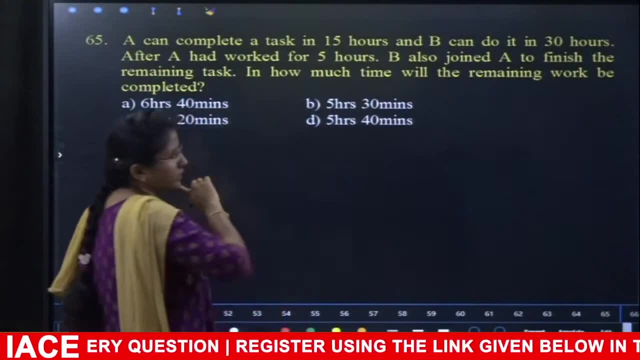 B can do it in 30 hours. After A had worked for 5 hours, B also joined to finish the remaining task. So next, in how much time will the remaining work be completed? So, since all the numbers are small and easy, 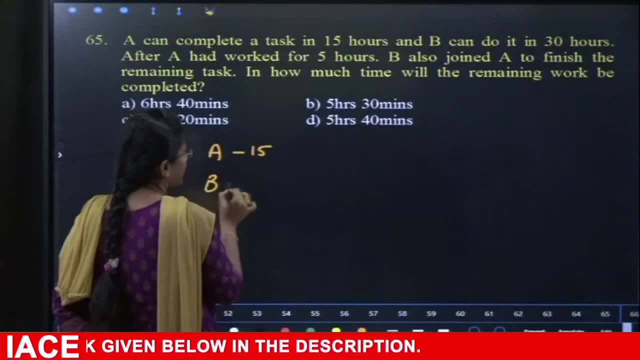 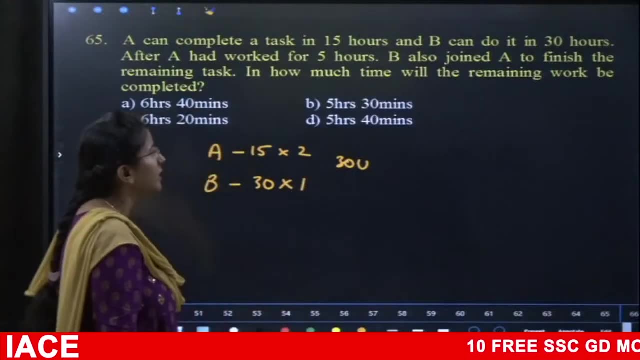 so A can complete the task in 15 hours and B can complete the same task in 30 hours. 15 and 30, total work completed: 30. Like that, efficiency of A: 2, efficiency of B: 1.. Next, A worked for 5 hours. 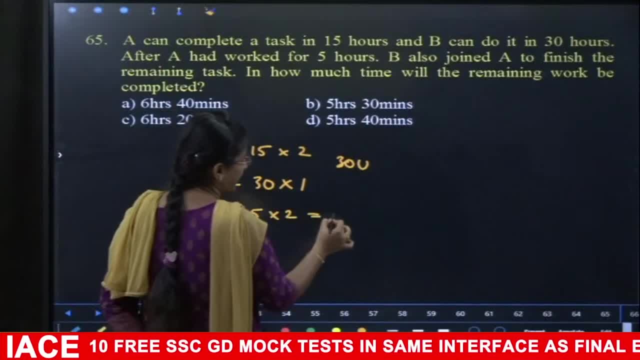 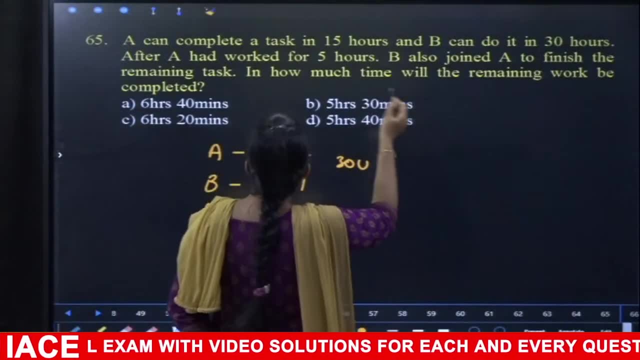 So A worked for 5 hours, 5 into 2, total 10 units of work will be completed. Remaining work will be balanced with 20.. Who should work these 20 units of work? In how much time will the remaining work be completed? 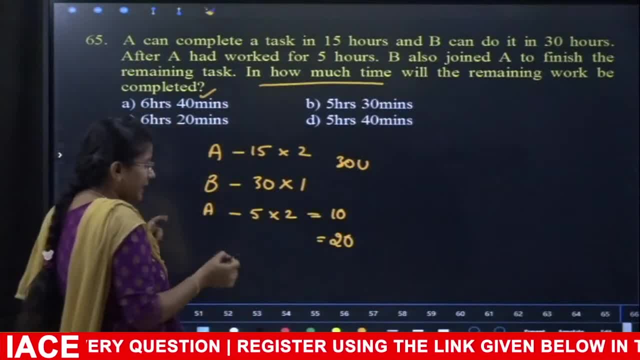 A and B. Now, after A worked for 5 days, B joined to A. B joined means A and B will work together. If both work together, 2 plus 1 for 1 day, total 3 units will be completed. 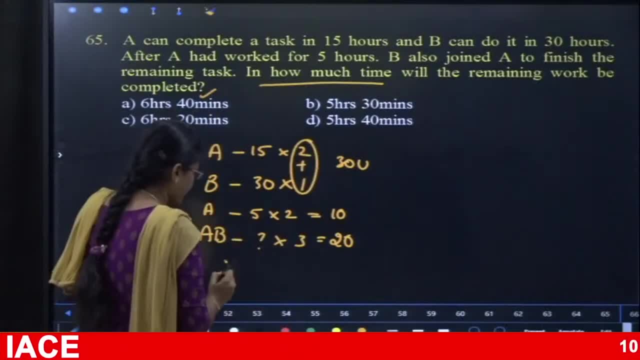 If we want 20 to be completed, how much time will it take? So 20 by 3 will be answered. 6 hours will be included. Above 6 hours, we have 2 by 3.. 2 by 3, 2 third of an hour. 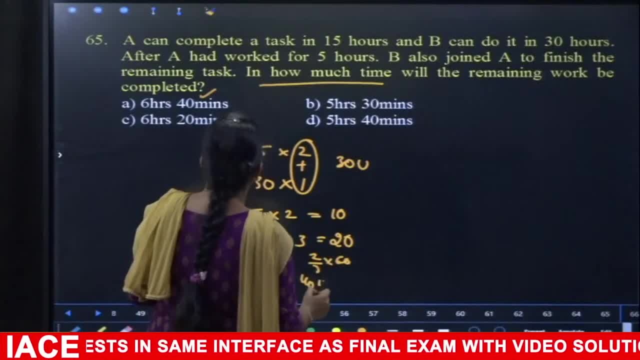 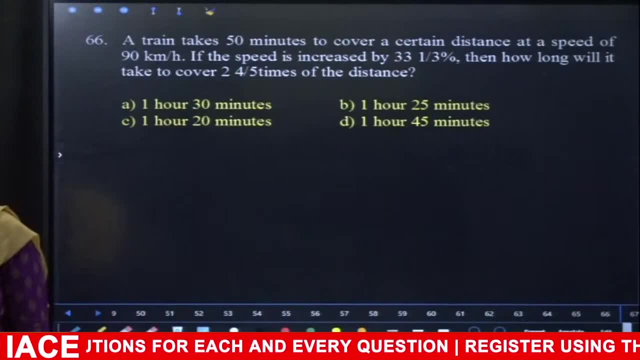 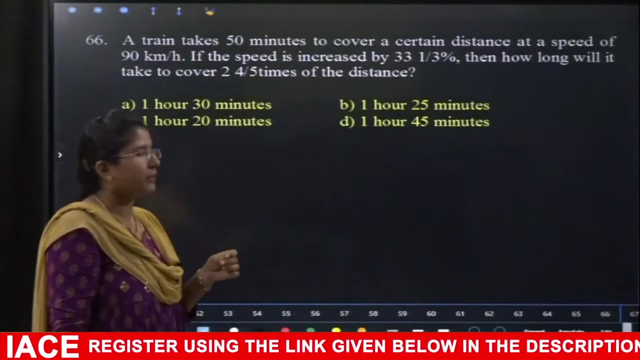 How many minutes? That is 40 minutes. Answer: 6 hours, 40 minutes. Okay, option A. Next try, 66th question. okay, your time is up, so again time and distance question came. a train takes 50 minutes to cover a certain. 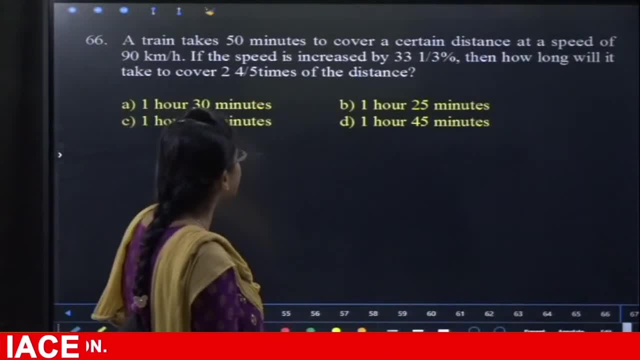 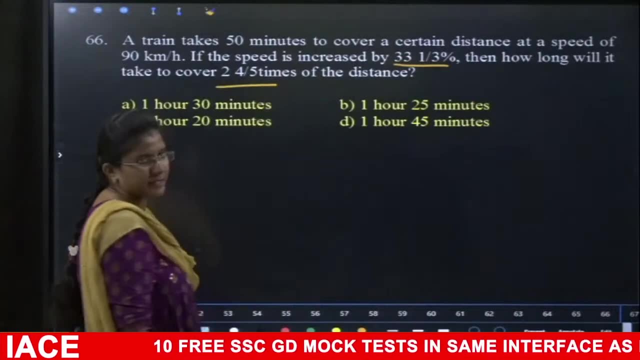 distance at a speed of 90 kmph, if its speed is increased by 33, 1 by 3 percent, and how long will it take to cover 2, 4 by 5 times the distance? how long is the question? it is a question on time. 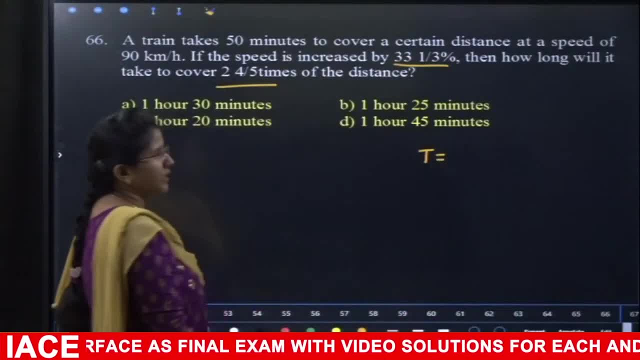 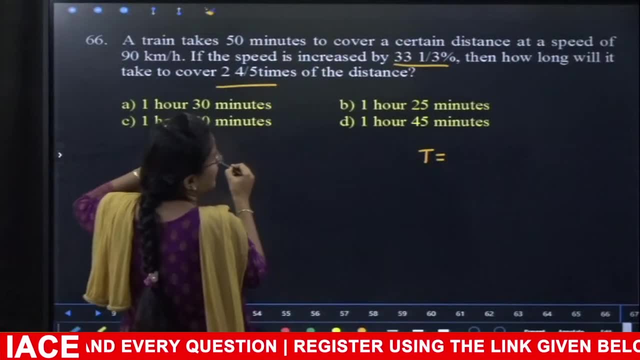 how much time will it take? first we will find out the distance and then we will change the speed and distance. so the train takes 50 minutes to cover a certain distance at a speed of 90 kmph. that means the distance covered first is speed into time. 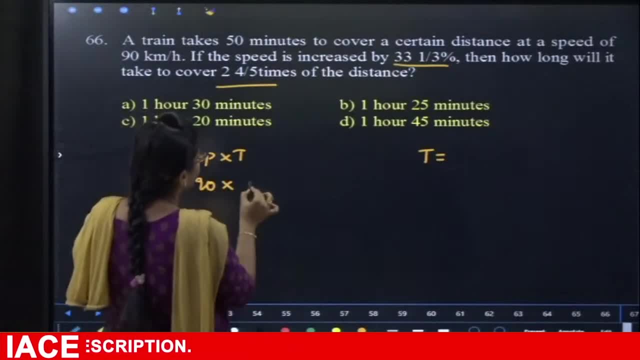 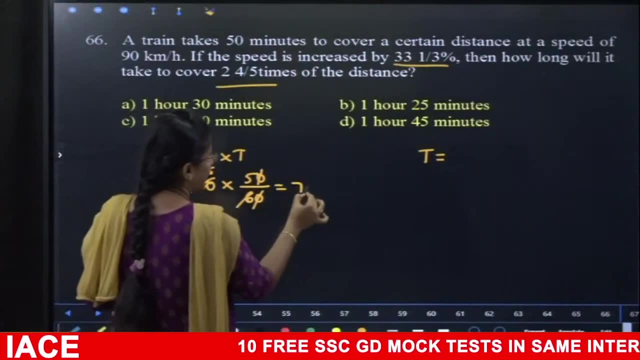 speed is what? 90 kmph into how many minutes time? 50 minutes time that means hours are 50 by 60. that will be for 6 and this is 15 times that is 75. for this distance: 2, 4 by 5 times the distance. 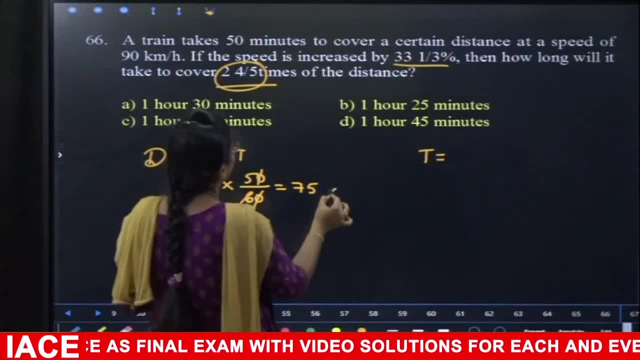 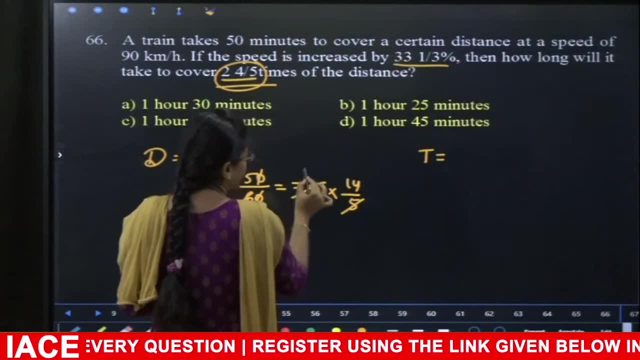 he is asking us to take there. that means 2, 1 by 4. we will do it here. 2, 4 by 5 times means how much? 10, 10 plus 4, 14, 14 by 5. so that is here 5, 20. 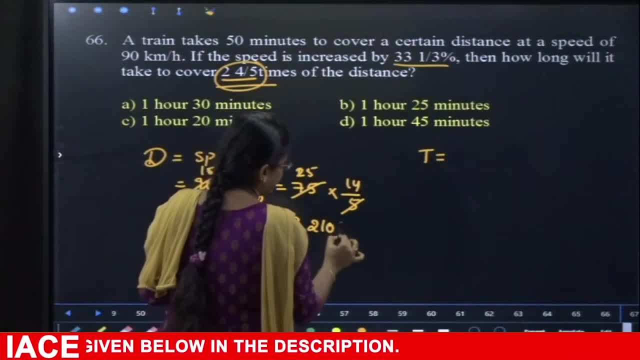 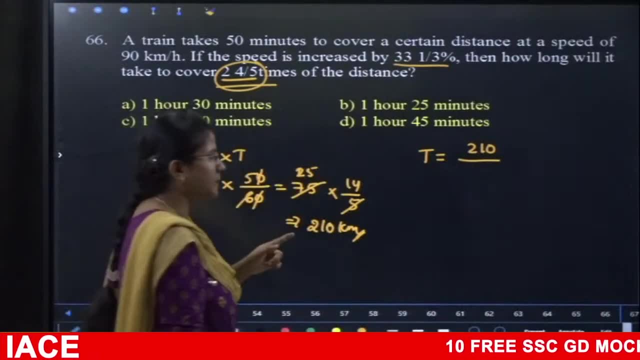 sorry, 15 times. that is 2, 10, 14, is 2, 10 km to cover these 2, 10 km of distance. how much time will it take? time equal to what we will write. distance by 70 kmph speed: we will write: 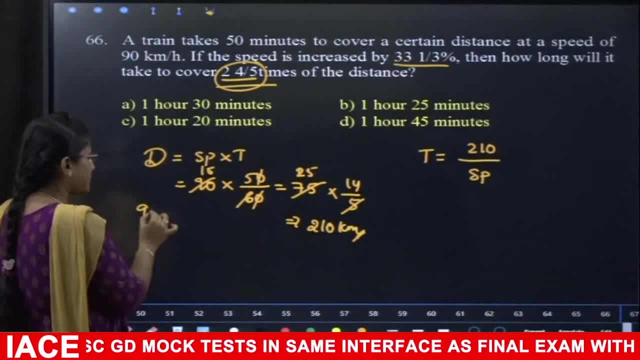 we will write speed. so, as we have taken the speed till here, you do not take 90 kmph and increase it how much percent? 33, 1 by 3, that means 1 third should be increased. 1 third of 90 will be 30. 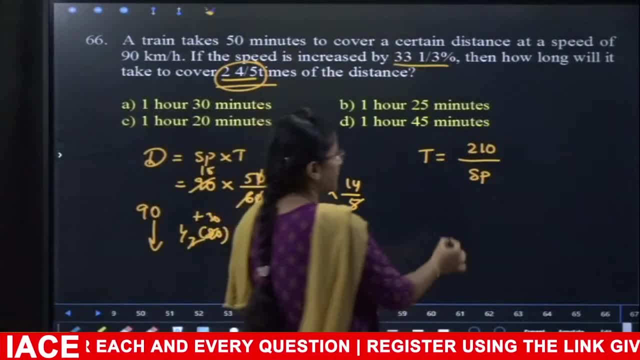 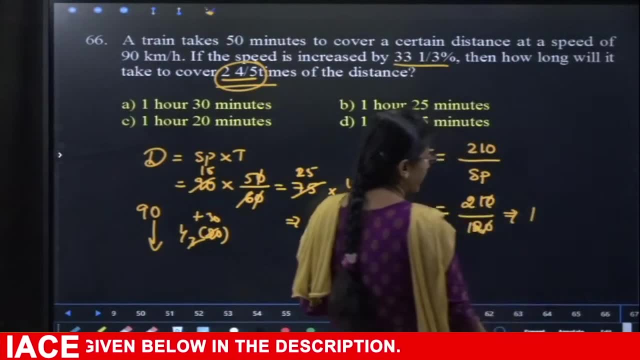 how much will be increased by 30: 120, ok, 2, 10 by 120, 120. so 21 by 12, 21, 12. one time is cancelled, remaining 9 by 12. 9 by 12 means 3 by 4. 3 by 4 means how many minutes 45 minutes. 1: 3 by 4 means 1 hour 45 minutes. 1: 3 by 4 means 1 hour 45 minutes. 1: 3 by 4 means 1 hour 45 minutes. 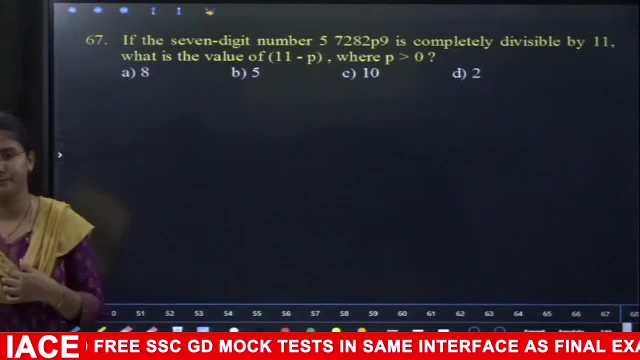 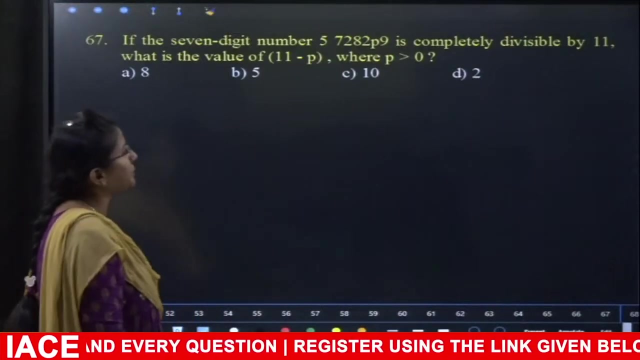 next. let us go for next one. 67. easiest question: 30 seconds timer. ok, ok, your time is up. this is very easy question 67: if the 7th digit number- 5, 7, 2, 8, 2, p, 9- is completely divisible by: 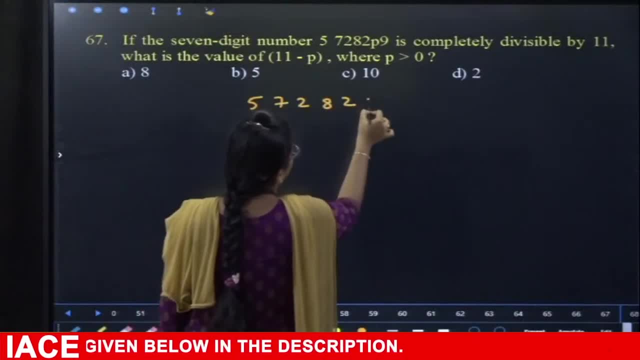 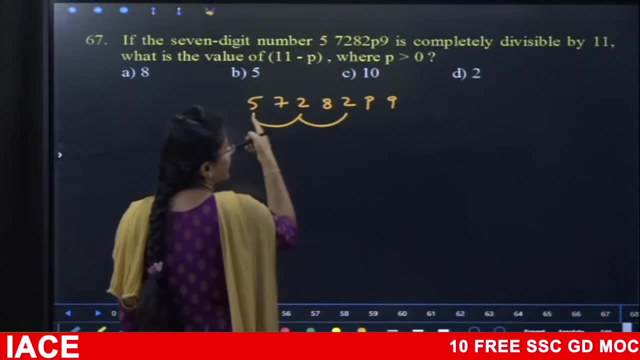 11th, or divisible by 5, 7, 2, 8, 2, p, 9, 11th, or divisible by alternate digits, sum 0 or 11, or 11, multiple can be said so here. alternate digits: 5 plus 2, 7. 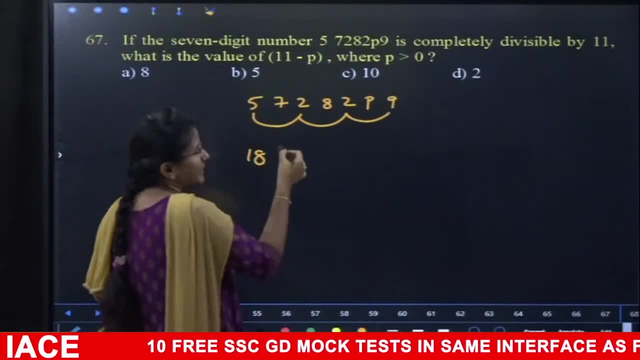 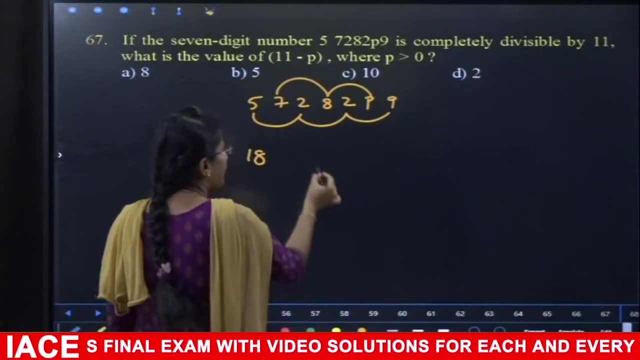 and 9 plus 9 is 18. one alternate set sum is 18. next alternate set sum is: 7 plus 8 is 15. 15 plus p here already 15. is there p value? definitely there is no chance of double digit. so p value. 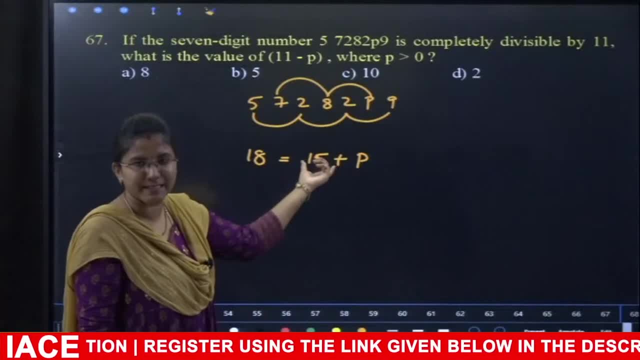 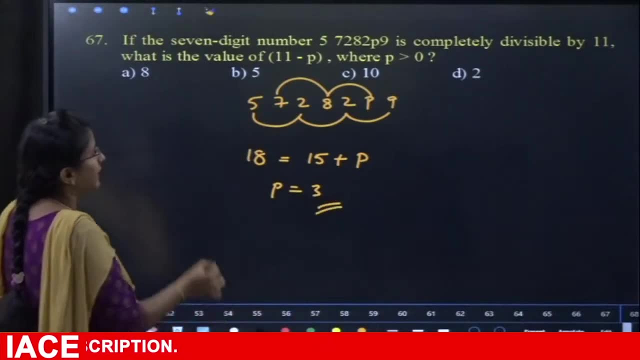 2 to alternate digit, sum will be equal. when 0 is there, then sum is 0. so here p value will be 18 minus 15. how much is it? 3 question is: what is the value of 11 minus p? so 11 minus p. 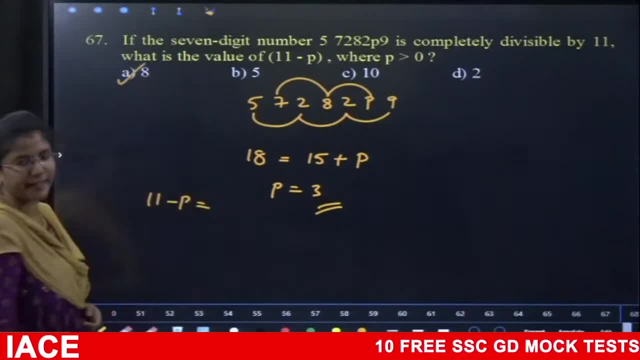 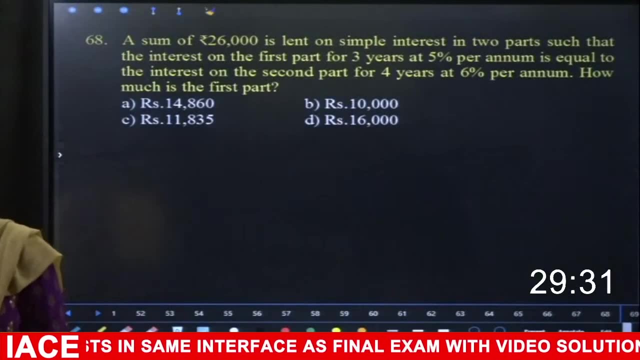 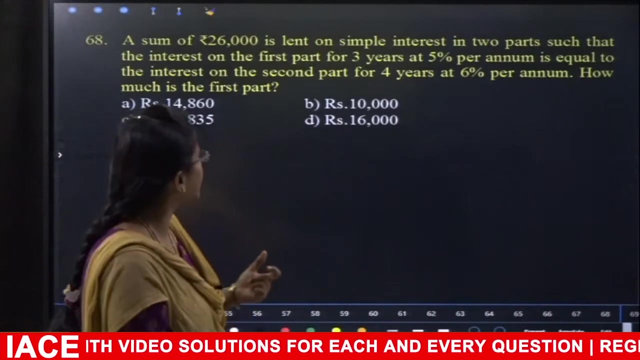 11 minus 3 is answer option a: 8. ok. next go for next one: 68, 68. try 30 seconds timer, please, ok. ok, this is also very easy question. very easy question. your time is up. see 26000 rupees. we have lent. 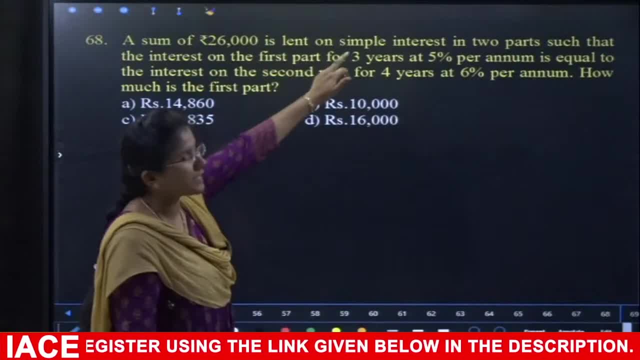 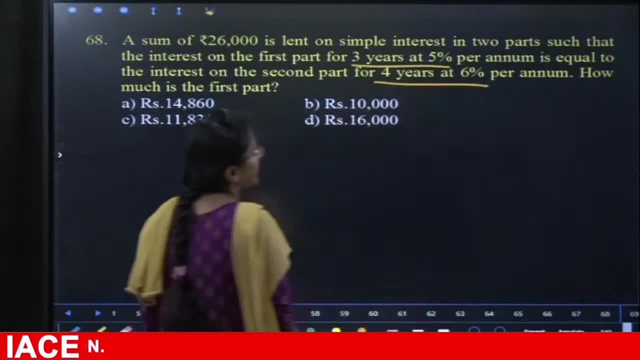 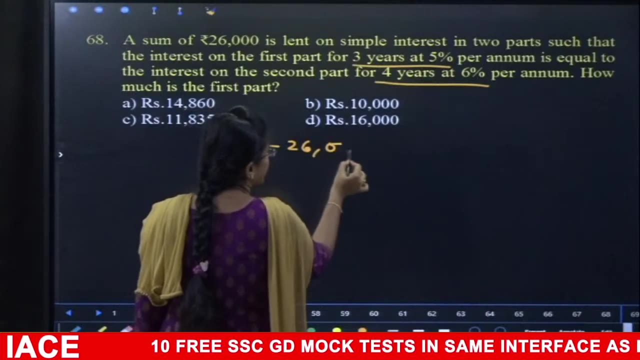 in simple interest in two parts. so in first part, how is the simple interest of 15 percent for 3 years? next second part, 4 years? 6 percent interest is also same, means we also do equal. so total principal given is 100 percent 26000. 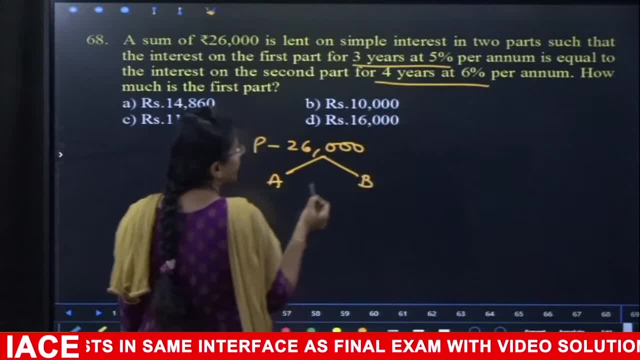 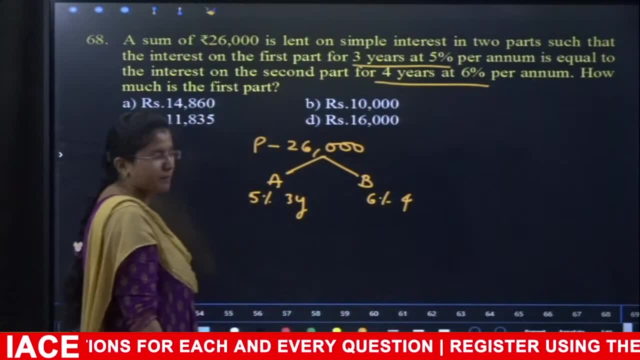 this 26000 I gave to first part a and b. this is 5 percent per year. how many years? 3 years here, 6 percent per year. how many years? 4 years? so simple interest: every year: 5, so 3 years. how much is 3, 5? 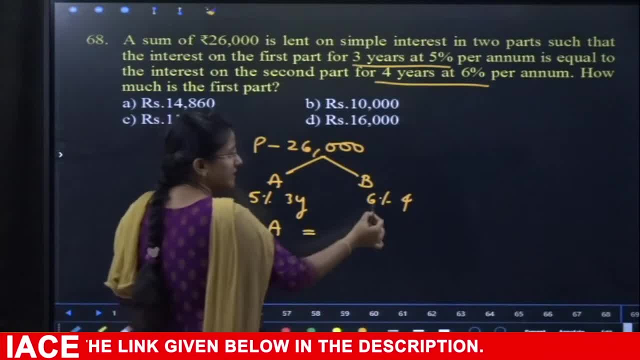 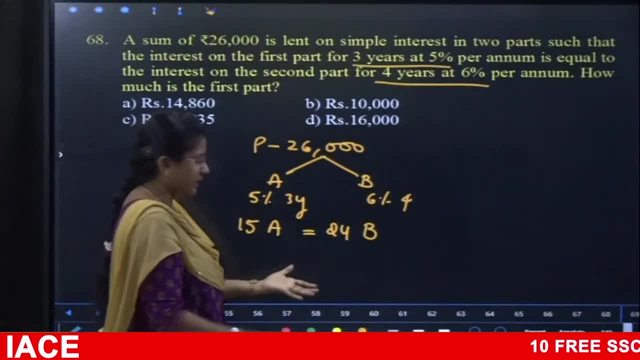 15. 15 percent of a is equal to next 6 into 4 every year 6, so 4 years. how much is 6, 4, 24 percent of b percentage by 100? next, next 15 and 24 will cancel out for. 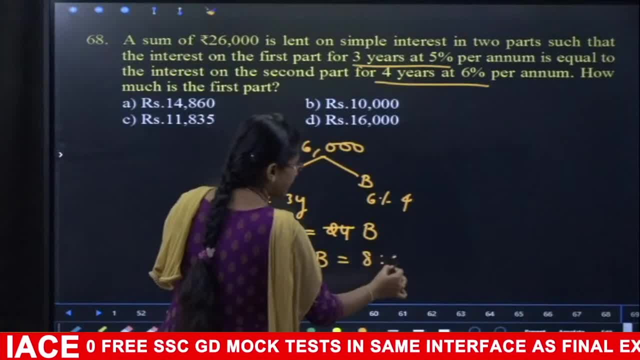 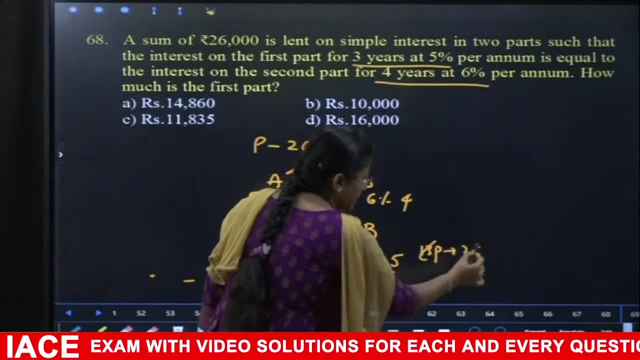 ratio directly: a is to b. what will be 8 is to 5 a. 8 parts b, 5 parts 2 together total how many parts? 13 parts. 13 parts is 26000. then what will be 1 part value 2000. 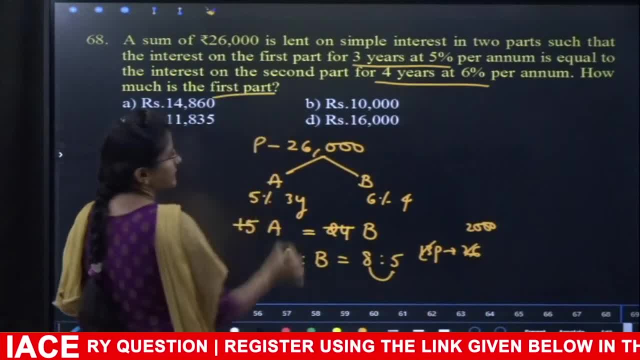 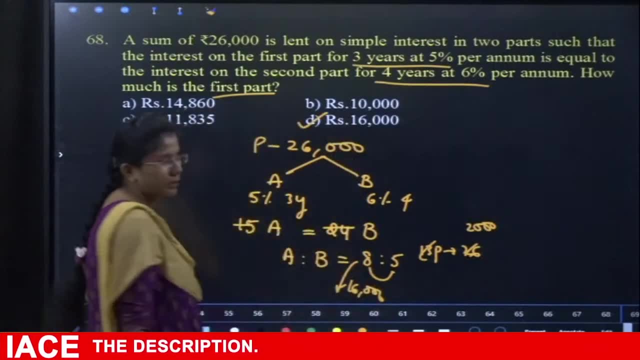 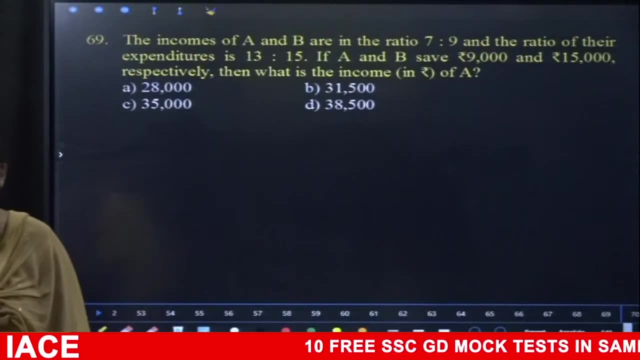 so what we are asking is: how much is the first part? how much is the first part? we have 8 parts, so 8 into 2000. answer will be 16000, option d: ok, 16000 next. then we will. we will write now have. 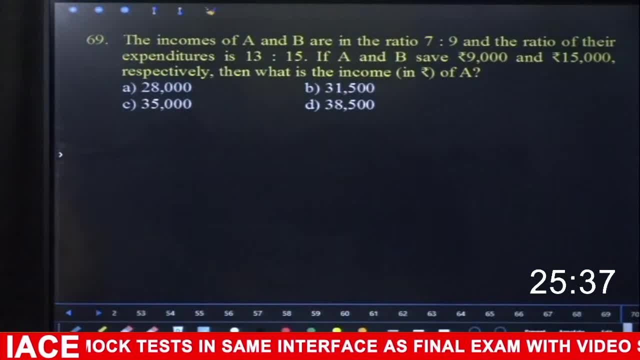 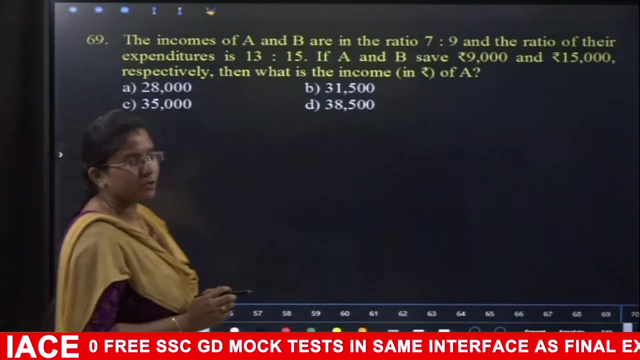 another 4 equal to 5, 6, 7, 8, 16000. so 3, 8, 6, 6, 7, 8, 9, 8, 9, 11, 23, 13, 13, 1, 3. okay, incomes of a and b are in the ratio 7 is to 9 and the ratio of their expenditures is 13 is to 15. 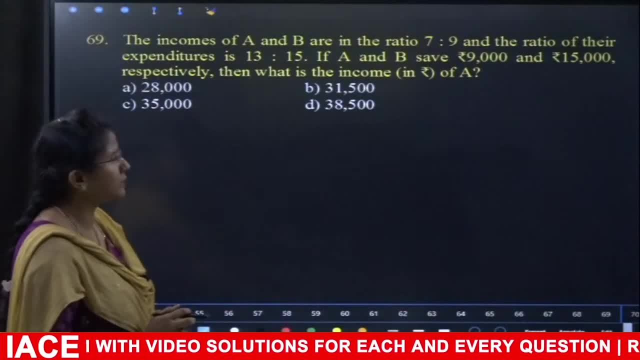 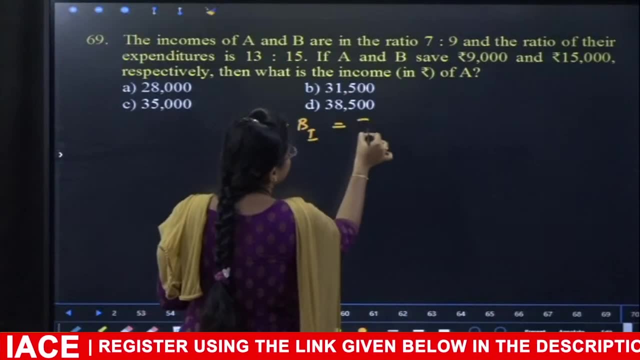 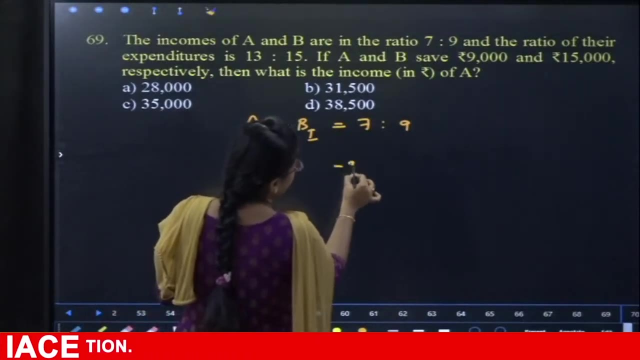 if a and b save 9000 and 15000 respectively, then what is the income of a incomes ratio is given initially, income of a and b are in the ratio 7 is to 9 and from these savings amount is given. saving c is given, a saving is a 9000 and b saving is a 15000. 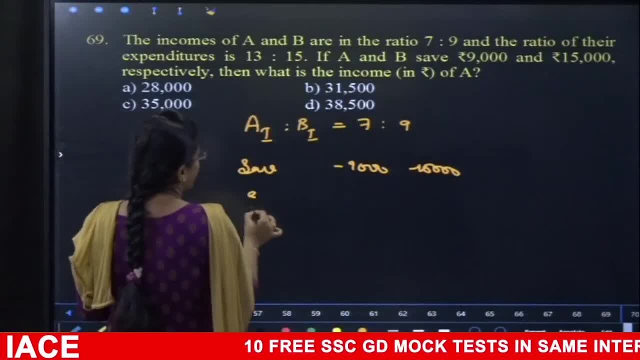 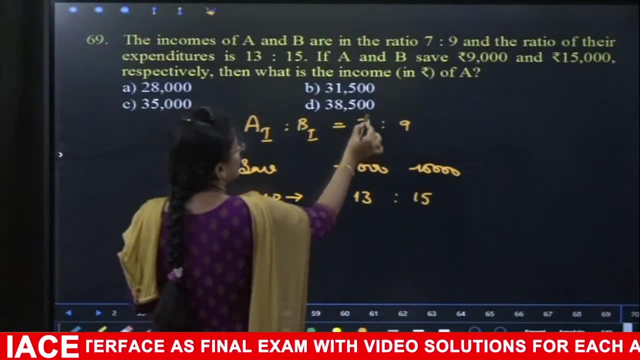 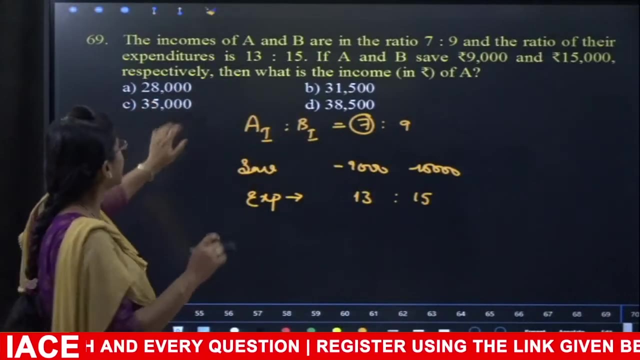 after deducting these remaining expenditures ratio from the income, the savings expenditure ratio is given already. 13 is to 15. we are getting income of a and b. so we can solve the previous problem of our normal equation, or because of a and b. we need 7 multiple. so we have a chance of getting 7 multiple, either 28 or 35. 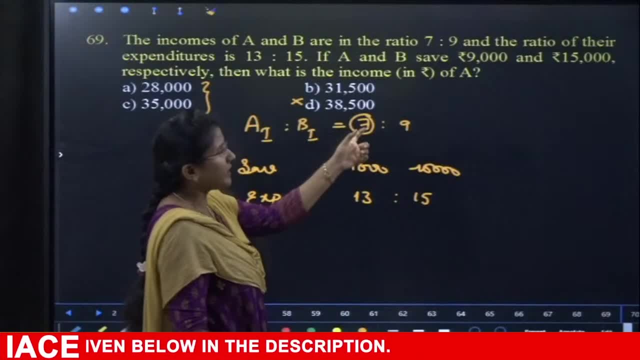 so there is no chance of getting i, so we check. so there is no chance of getting i, so we check. 7 go for 28 or 35. now if I take 35000, 7 parts 35000, so 1 part 5000. 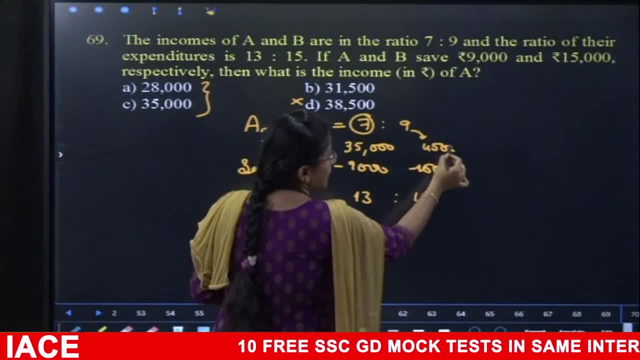 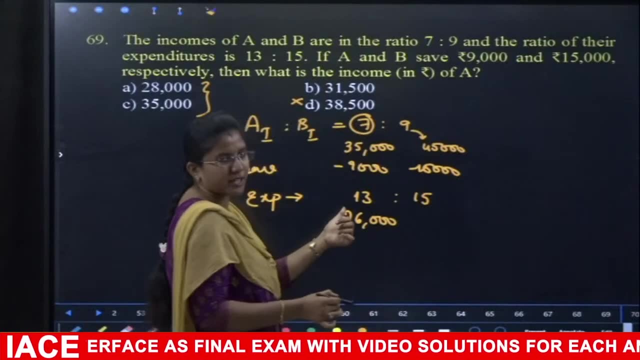 so what is the value of 9 parts? 9? 5 is 45000. if we deduct 9000 from 35000, remaining is 26000. if I get 26, then there is a chance of getting 13 in 2. verification go on. 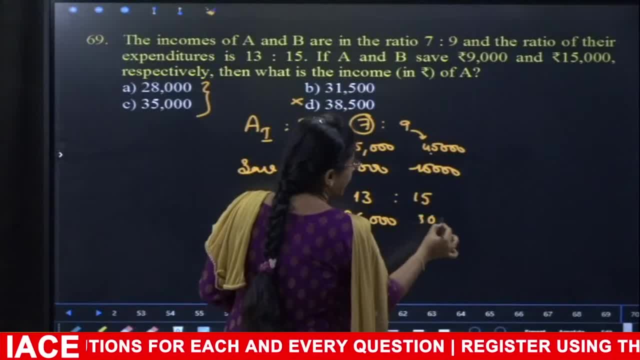 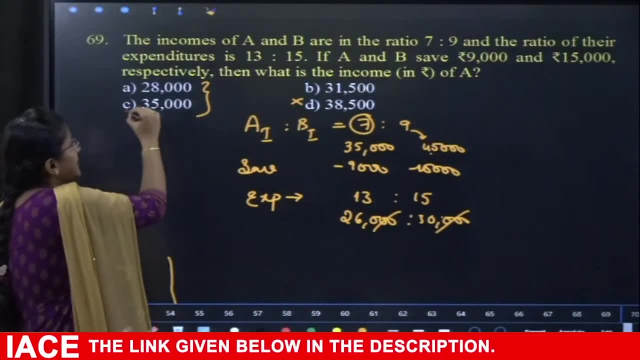 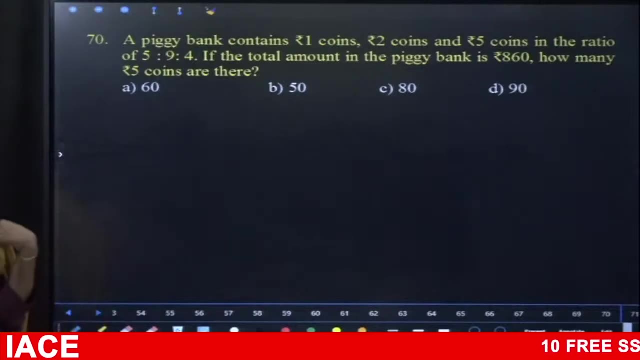 or else we will stop 15 from 45. remaining is 30,000. so what is the ratio of 2 is 13 and 15 in 2? table 13 is to 15 will be satisfied so option. so what is the ratio of 2 is 13 and 15 in two? 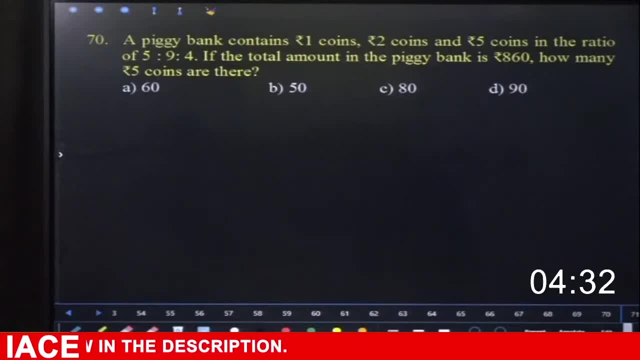 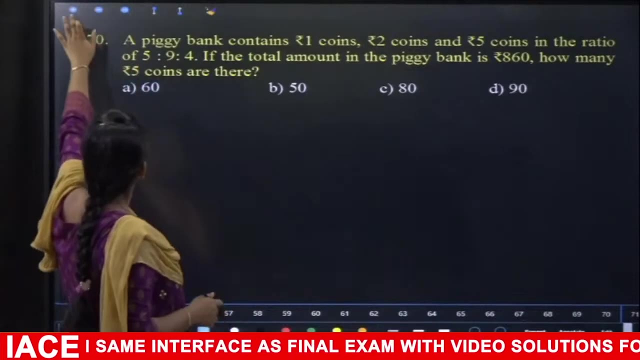 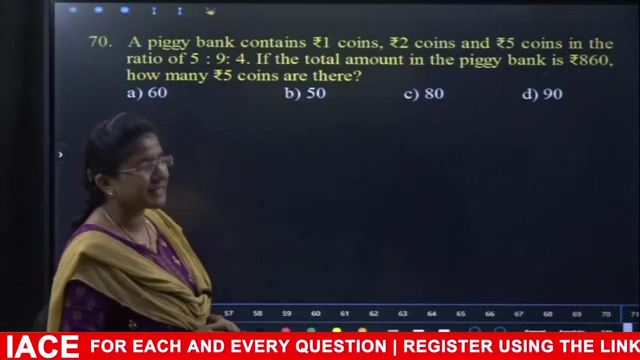 okay, so here the question from ratios topic. a piggy bank contains 1 rupee, 2 rupee and 5 rupee coins. in the ratio 5 is to 9 is to 4 and the total amount in the piggy bank is 860 rupees. then how many 5 rupee coins are there? so in a piggy bank this denomination of coins is given what all coins there are: 1 rupee and 2 rupees and 5 rupee coins. next it is given the ratio of the coins: 5 is to 9, is to some 4 and the total amount in the piggy bank is: 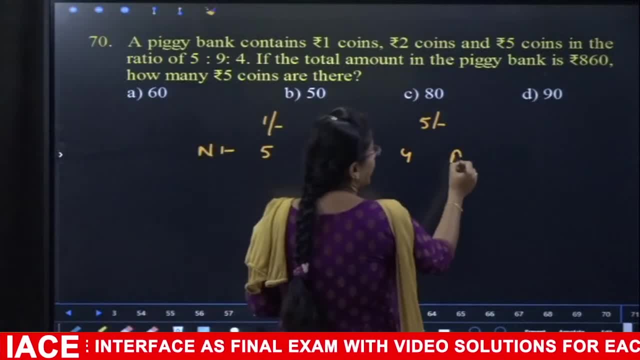 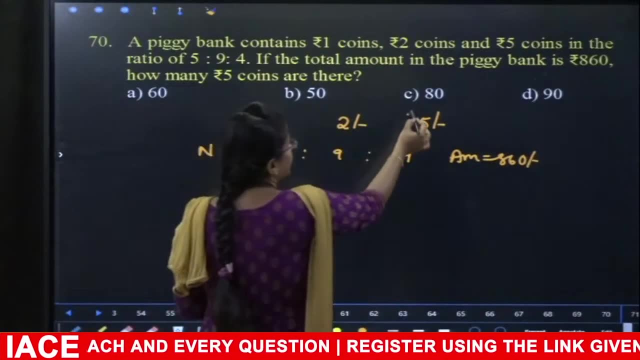 rupees. he has not told how many coins are there. he has told the number of rupees. the amount is 860 rupees. then how many 5 coins are there? how many 5 rupee coins are there? he is asking now. please do answer the question. 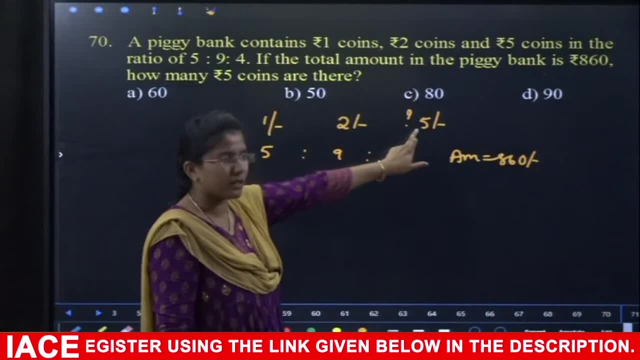 so the first question is: how can you find out how many coins are there? the second question: When you ask a question like this, go for that number. if you ask for 5 rupees, check here. if you ask for 2 rupees, check here for the parts. 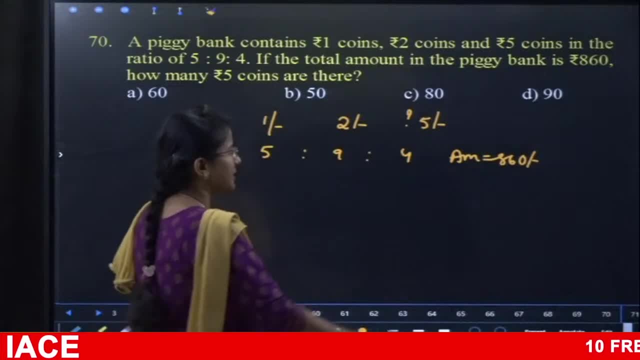 Since he asked for 5 rupees, we have 4 near 5 rupees. What should be the option for which it should be multiple? It should be multiple for 4.. Exactly, this decimal should not be written. So there are 4 multiple. there are 2 questions. 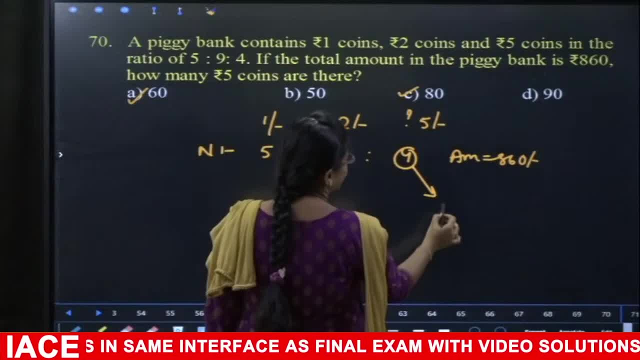 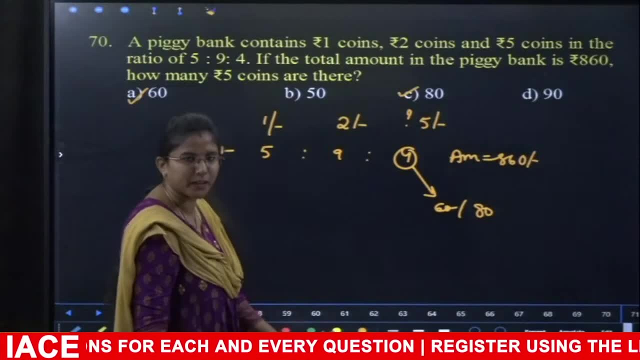 One is 60 and the other one is 80.. 60 or 80. This is 15 times and this is 20 times. If we check, the amount is 860.. We will check if it is enough. So 4 is 60.. 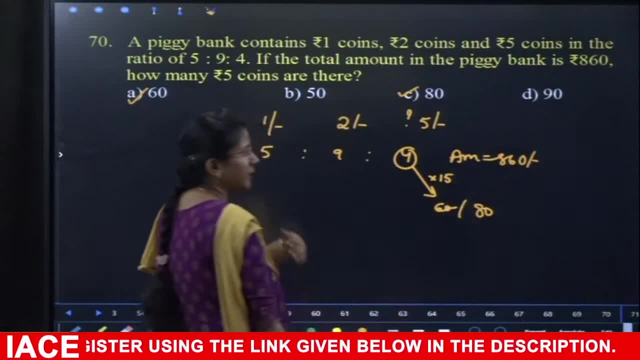 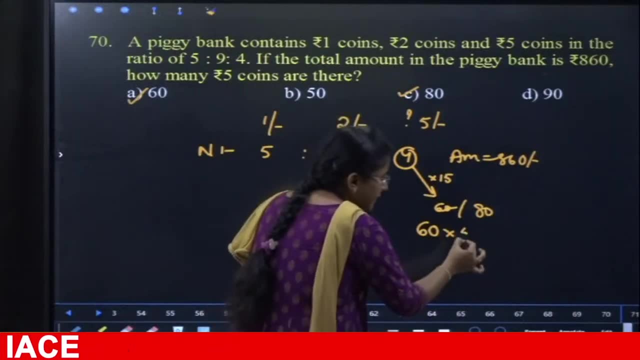 If there are 60 coins, what should be one part? It should be 15.. So if there are 60 coins and 5 rupees coins, each coin has a value of 5 rupees. Since there are 60 coins, 60 into 5 rupees, what is the value? 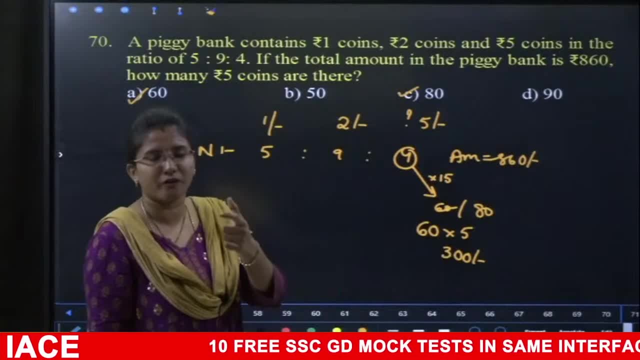 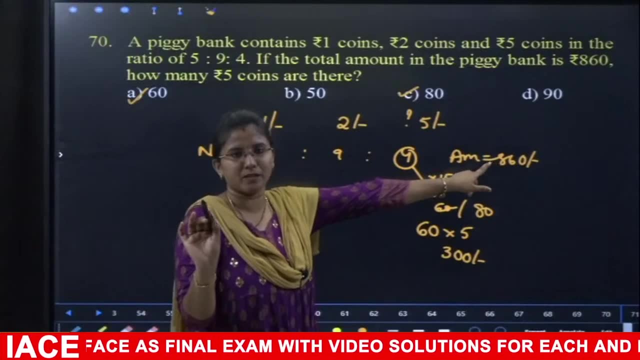 300 rupees. In the previous denominations the maximum value of the coin is 5 rupees coin. If 300 rupees comes from that, we cannot reach 860 because of these two. So in that verification we do not have to check 60, we will eliminate it. 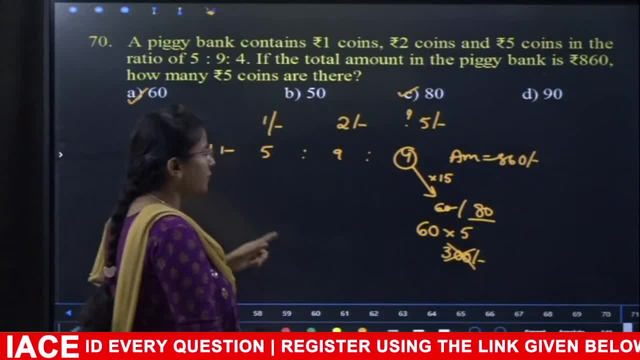 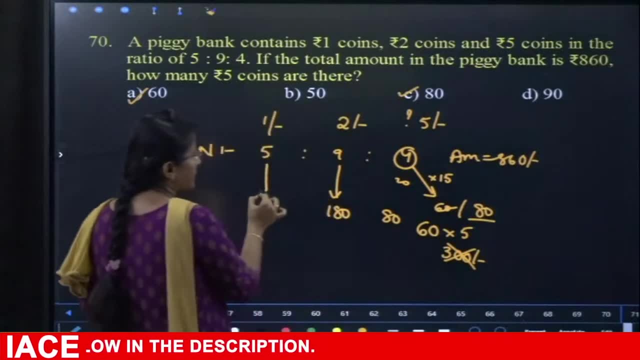 Then go for another multiple: 80 is there, So 480 means how many times 20 times. So there are 80 coins and 920s. There are 180 coins and 520s. here There are 100 coins. 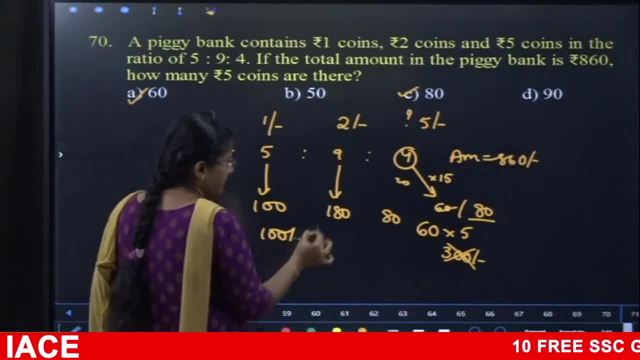 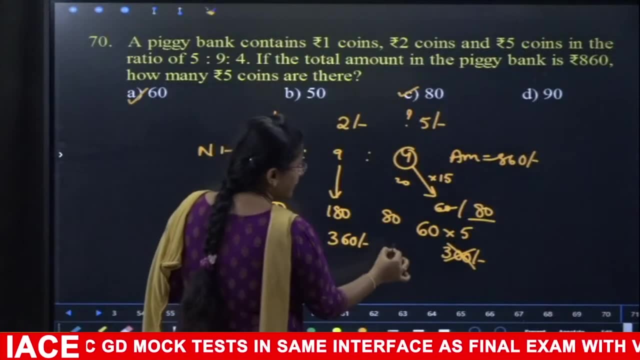 If there are 100 coins for 1 rupee, how much is it 100 rupees If there are 2 rupees and 180, how much is it? 360 rupees? Next, 5 rupees If there are 80 coins, how much is it? 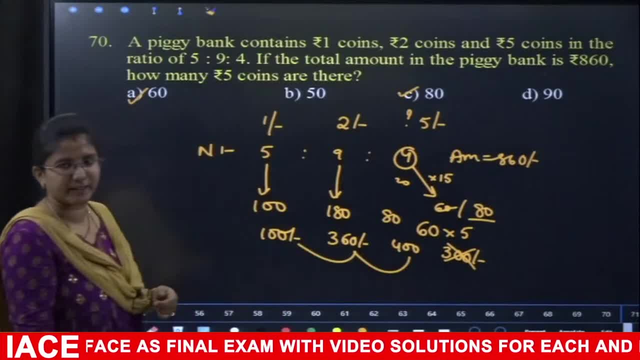 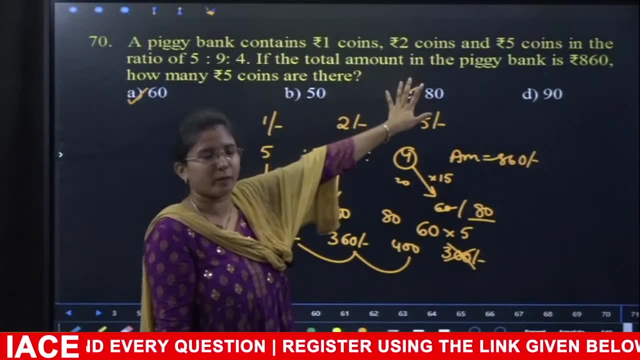 400 rupees. So if we add all these and check, we will get 860. clearly We have taken this process off. If there is only one multiple, the same answer is given directly. If not, we can check and put the answer in the verification. 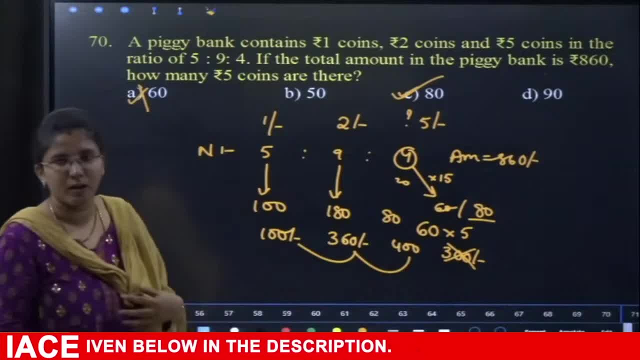 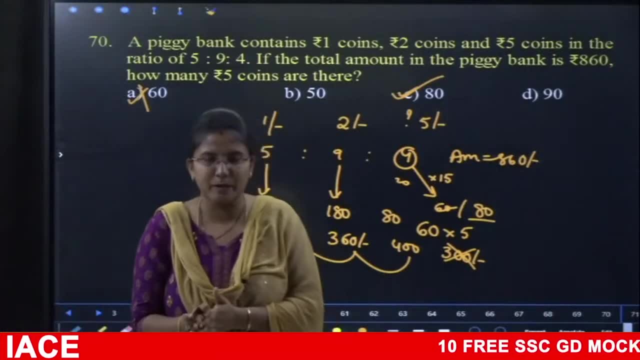 So it is option C, not option A. Okay, So till here we have completed 70% of the paper. from quantity to aptitude. We have completed 70 questions in the overall 100.. Remaining 30 will be. 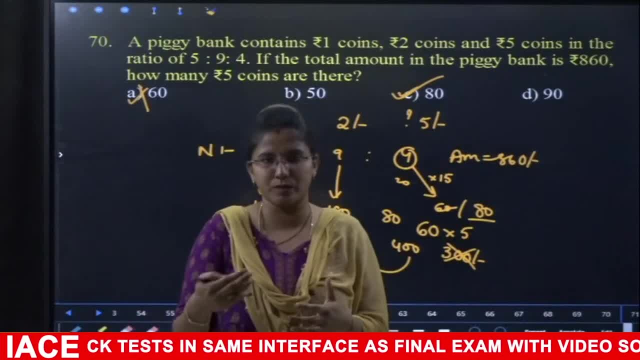 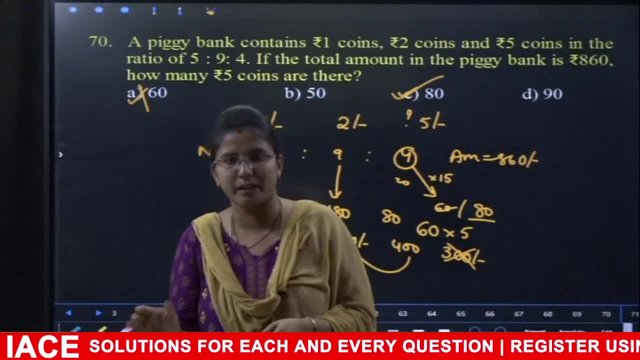 We will provide a PDF format for this in the evening. In that remaining 30 questions There will be maximum repetitions. Some questions will have repeat same models. New questions will also come. Try with the base. So your workout for the complete perfect quantity aptitude marathon session will be: 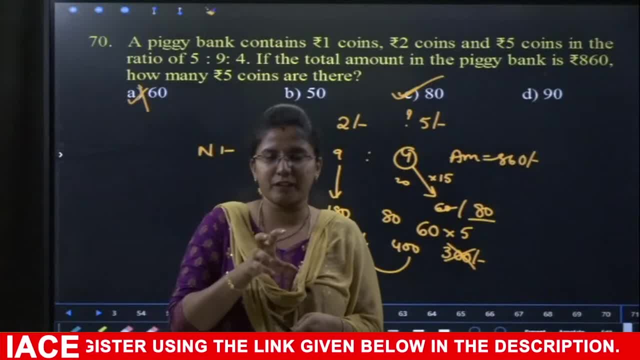 cleared. So we have completed 70. Remaining 30 will be a workload for you. Try it. And then the questions in these marathon sessions. if we are covering these models, if we are practicing rigorously, we can surely clear the elementary mathematics section. 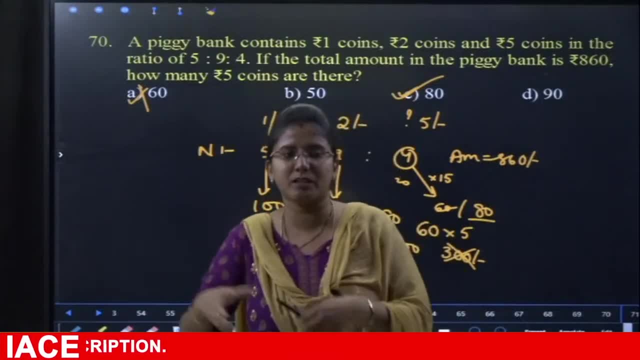 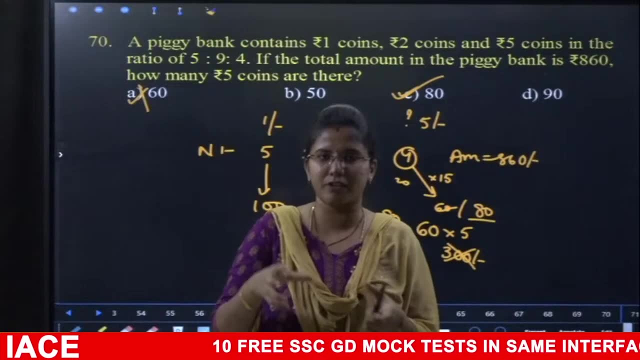